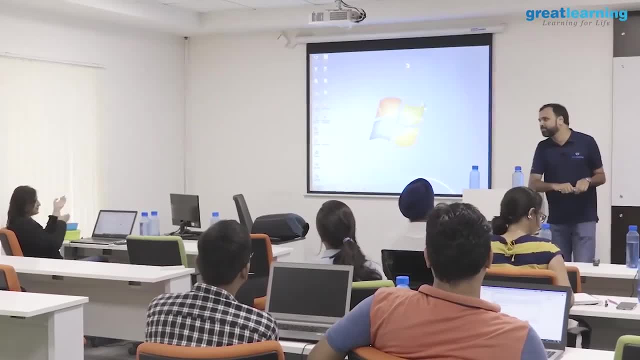 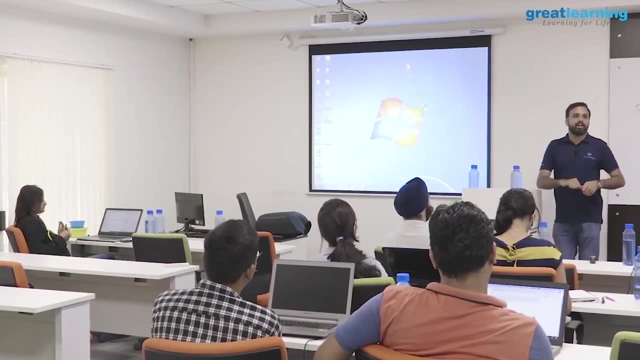 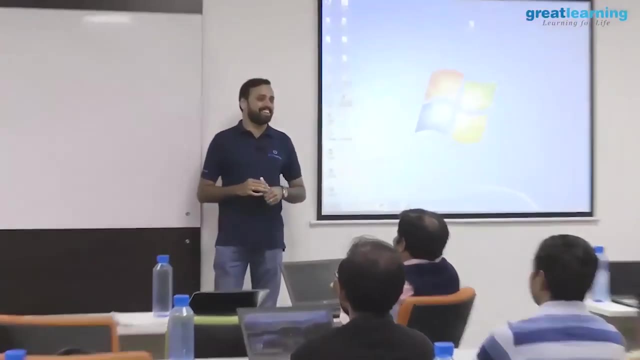 Yeah, If I have to say, Because the base anyway is we have a big data team who is creating data and investing into the lake. Okay, Who else? Who else is bold enough to say that I'm coming from the field? Don't worry, I'm not going to ask any questions or anything like give me the definition, or something. 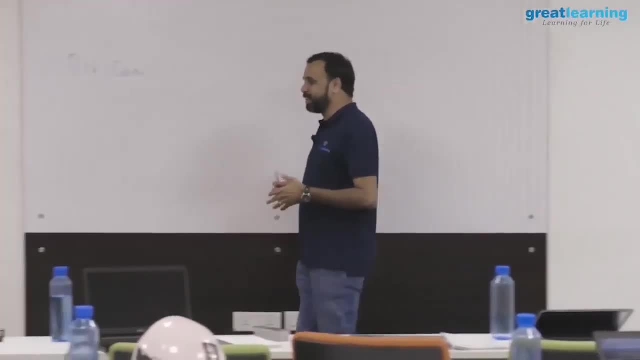 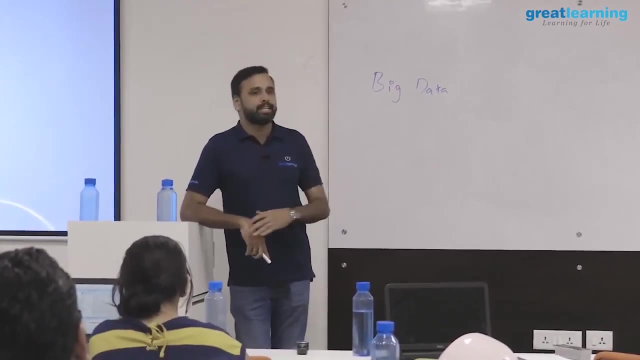 Nobody is there from big data domain. Okay, Probably not. I mean, I don't blame you. Maybe you're already coming or you're already part of something related to big data, But maybe you're not completely convinced that you're working on big data, right. 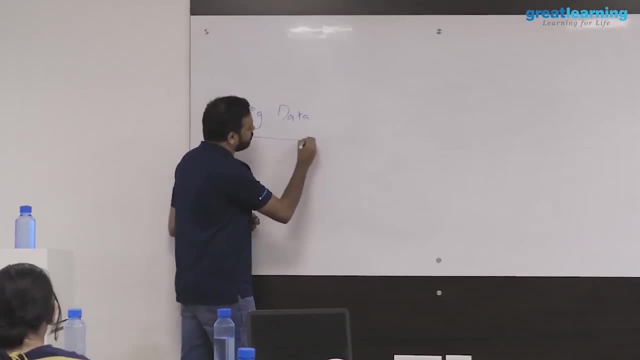 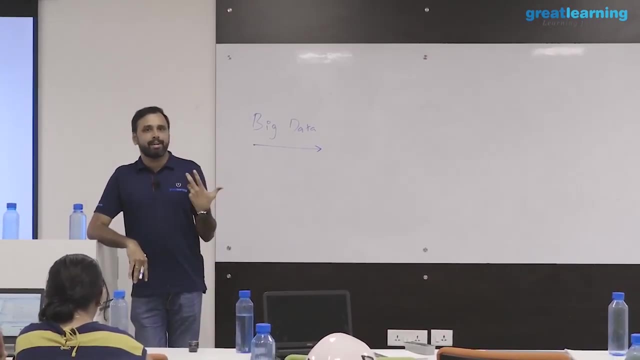 Okay, So this term is actually a very elusive or how do I say? It is a very relative term. So big data. this term was very popular, I would say around eight years back or 10 years back. Even today it is very popular. 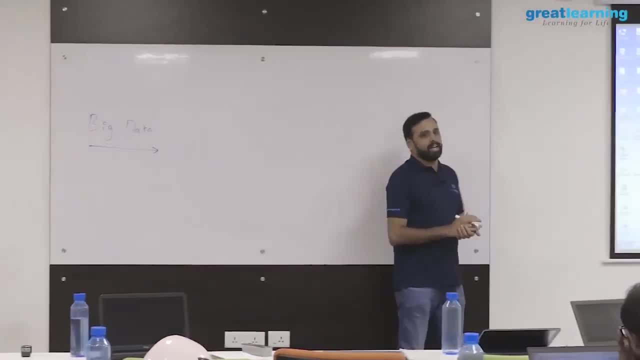 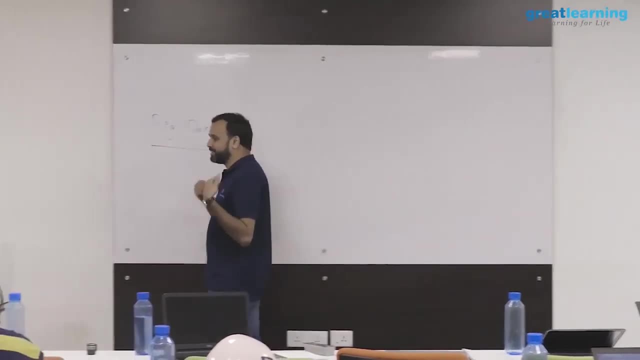 But the meaning has changed a lot. Okay, So, So, when you started working in big data, it was when somebody said big data, it was like: oh, that's something really great stuff that you're working on. But today, when you say that you are in the big data domain, that's like: oh, it will happen anyway. 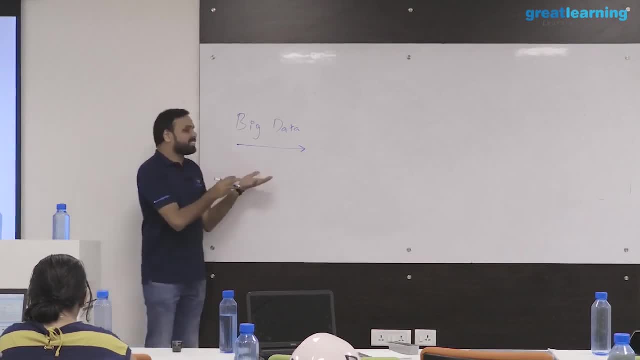 So something like that. So before we understand what is big data, or what is industry aspect of big data, et cetera, et cetera, you need to have a slight idea about what is the world without big data. Right? So before I talk about big data, I have to tell you what is the world looks like without big data. 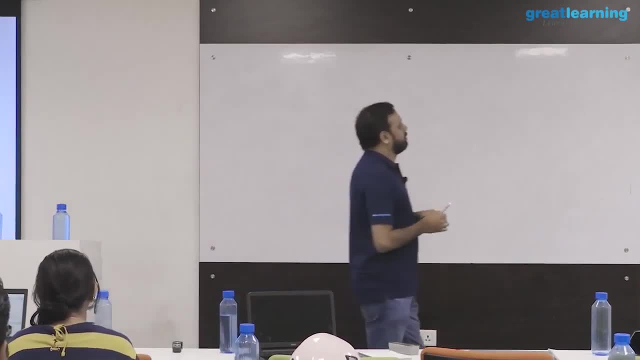 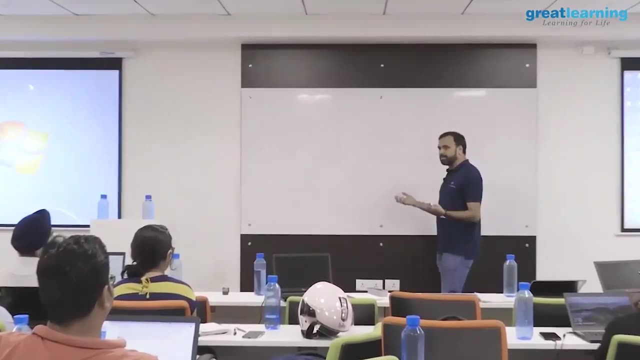 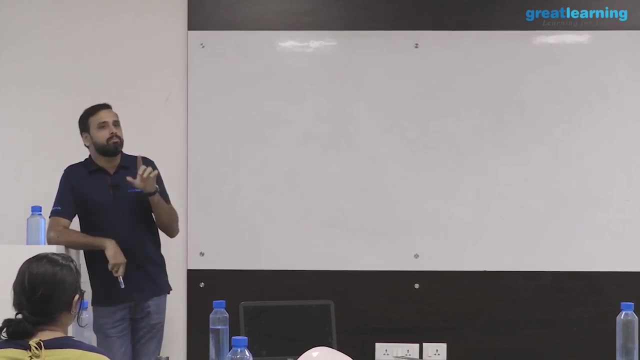 So, traditionally, if let's say you're working for a company I don't know- ABC Corporation, any company, Right? And let's say this company is having a lot of products, Right? So let's say I was with this company called insurance company AXA, 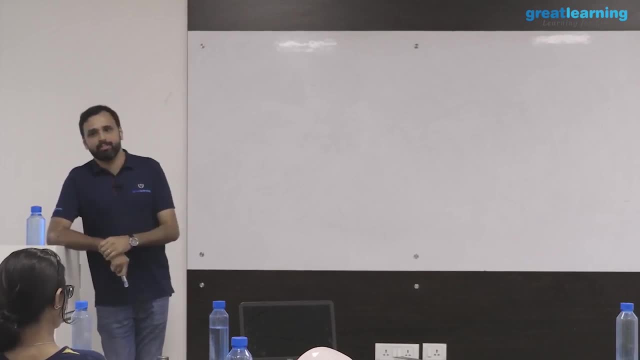 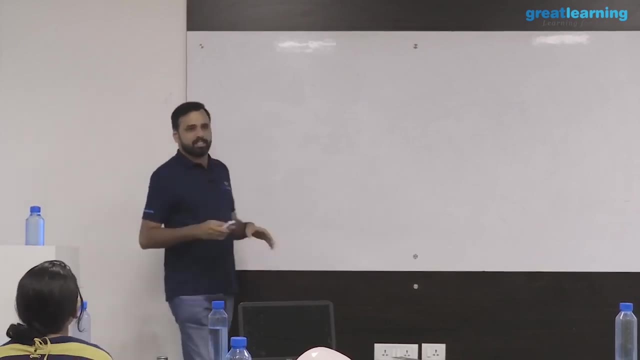 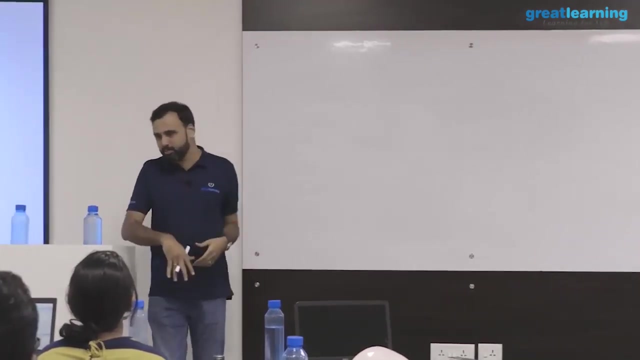 Right, That is AXA, Right, Right, And they have been working as a consultant for some time, So they are in the life insurance business, Right? So take an example of AXA, just as an example. Okay, So this company, what they do, so they have a product called life insurance which they sell to all the US customers. 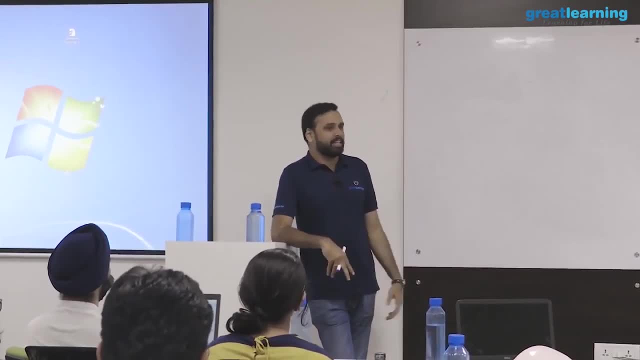 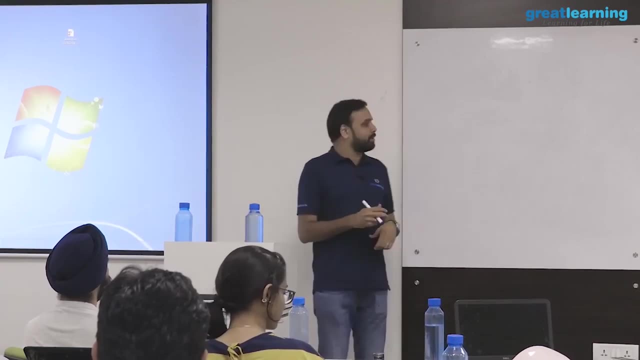 In US insurance is big deal, Not like in India. In India, even if you hit and die, nobody cares about insurance. But in the US it is million dollar business Right. So AXA has a lot of customers in India as well as in US. 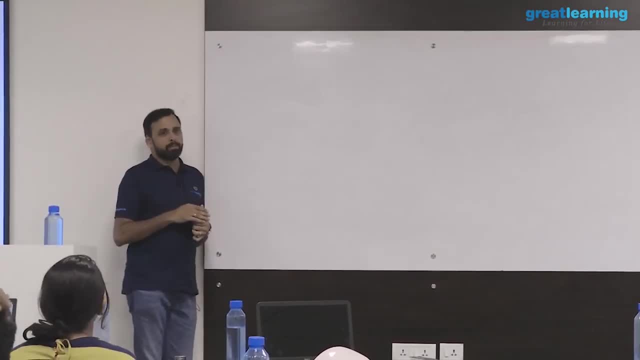 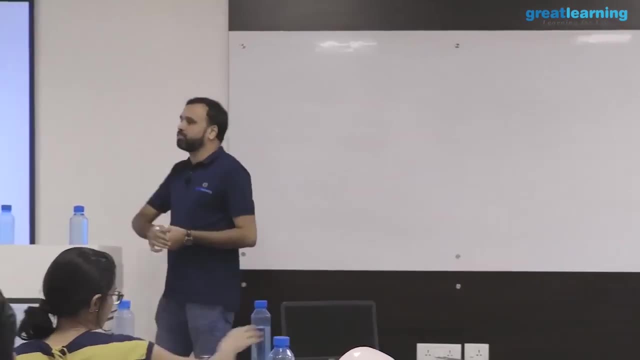 So in US, what they have done? they have a platform where people visit and buy insurance. So you have a portal where you can log in and say that I want to buy an insurance for my bike or myself or anything like that. Right, 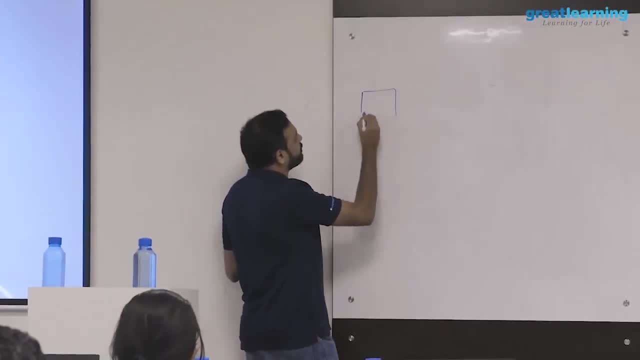 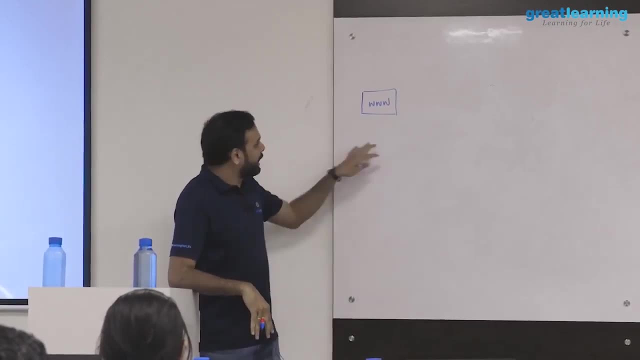 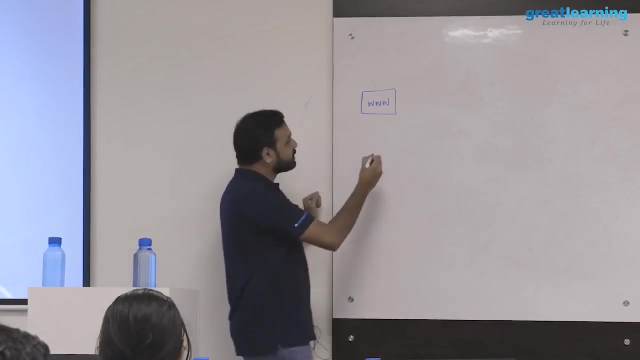 So basically they have a website kind of thing. Okay, From there, people actually buy insurance, Right? So if you're buying an insurance online or if you go to them and physically purchase an insurance copy, these transactions that are happening in the website are actually handled by an RDBMS system. 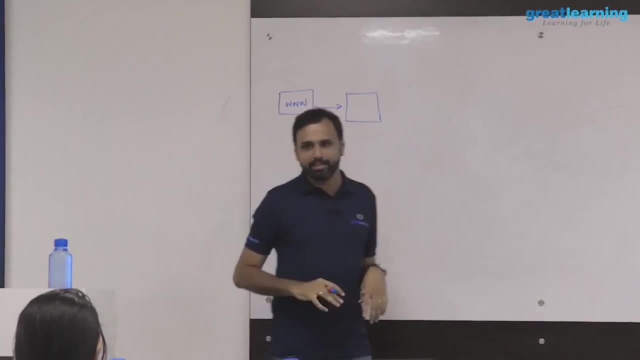 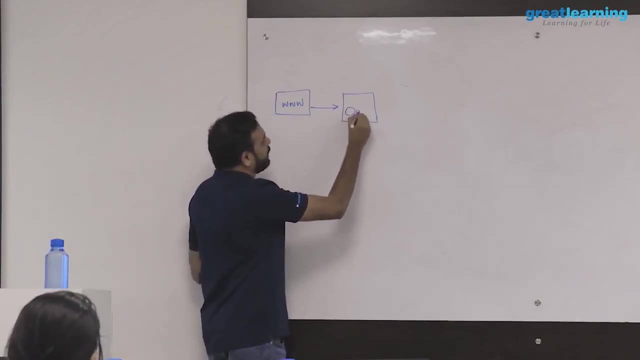 So I'm assuming that you at least know what is a database and all Right, So I don't have to tell you what it is Right. Okay, So AXA was actually using Oracle to handle all the you know, insurance transactions. 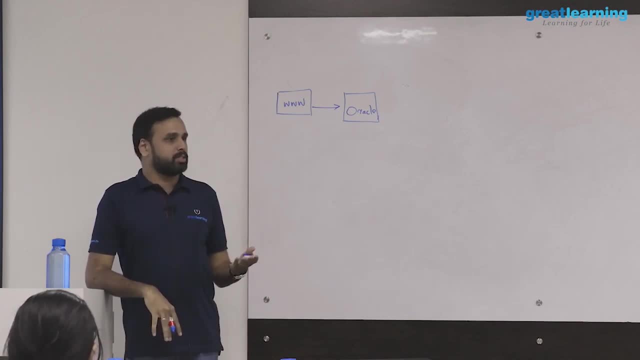 So if you pay some money to their insurance Or renew your insurance, anything that you do- this website will take care of it, And all the data that website has is being dumped into Oracle, So Oracle is their database Point number one. 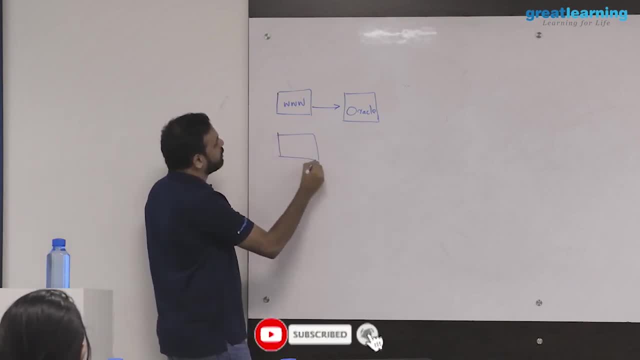 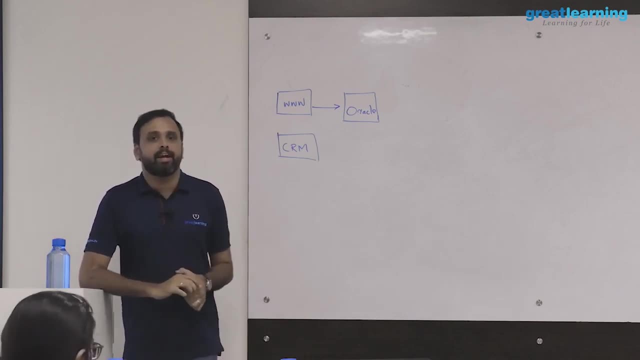 AXA also has a customer portal. They call it as their CRM. It's called the Customer Relationship Management System, Wherein they keep details like the customer's name, age and ethnicity. you know all this customer related information, So the CRM also dumps the data. 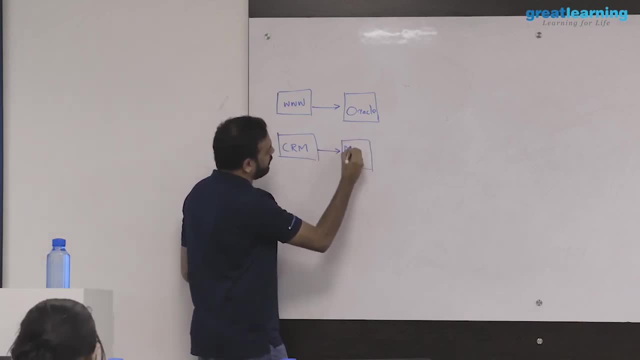 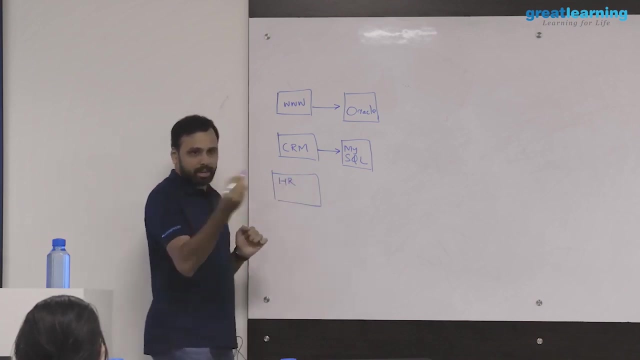 But CRM is using MySQL, for some reason, another RDBMS, So CRM is using MySQL, Right. And then they have an internal system which is used by this HR and other folks. They have an internal application, software application, where employee data and HR data and all this is getting managed- their office data. 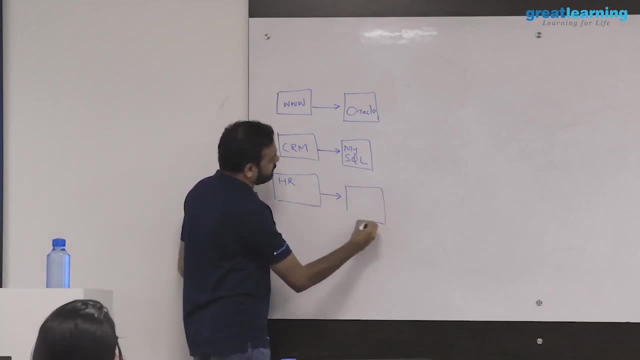 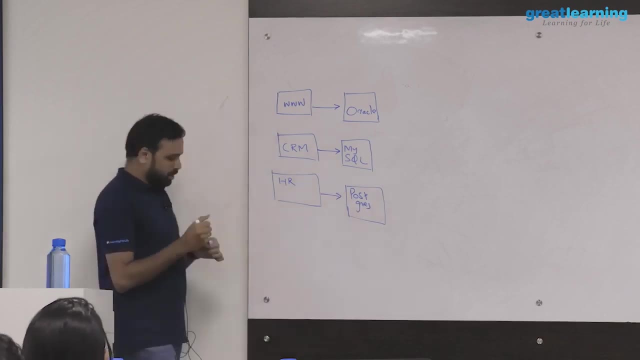 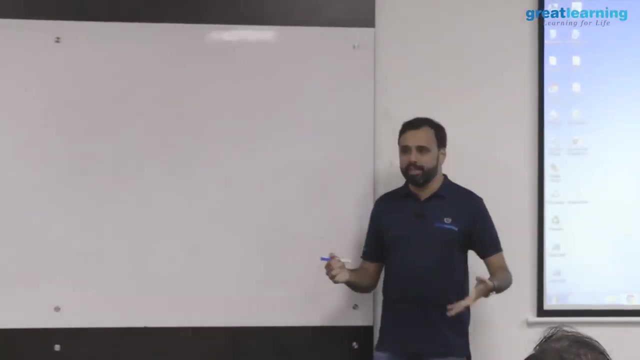 And this is using some other RDBMS. So let's say, this is using- I don't know- PostgreSQL, Just as an example. So you see the problem right. This is not a new problem, But in the traditional world, one of the problems that we have is that if you look at any organization, they will have multiple applications, not one application. 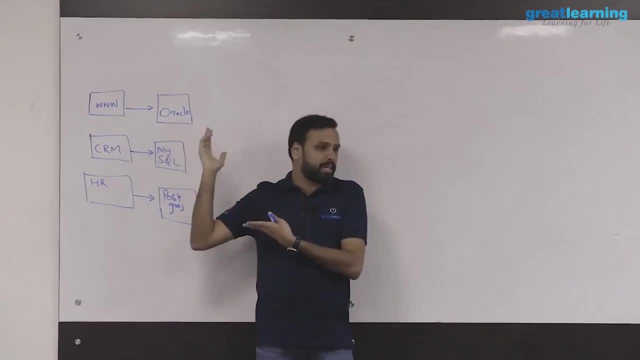 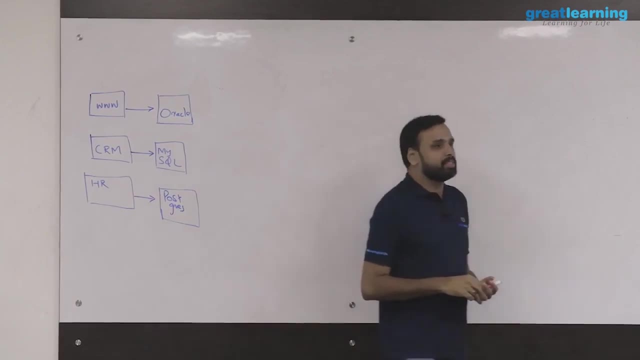 And each application will be probably using a different database, Right? So this guy is using Oracle, This guy is using PostgreSQL, Right? And now what happens? if you are the CEO of AXA or some big shot in AXA, you want to pull a report. 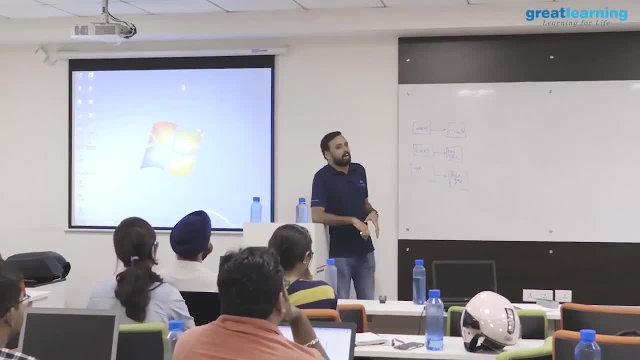 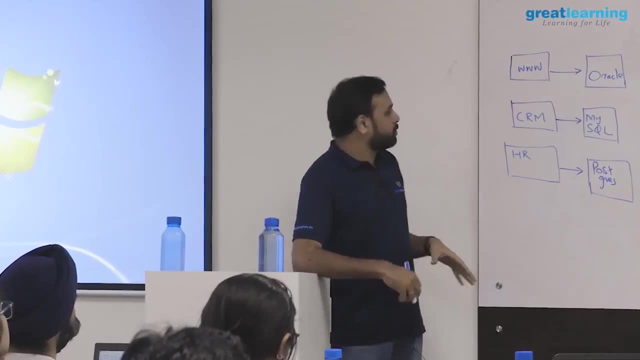 Right. So you are basically interested in understanding how many customers between 30 to 50 age group have bought an insurance from this country, et cetera, et cetera. So to pull that report you actually need the data from all these guys. 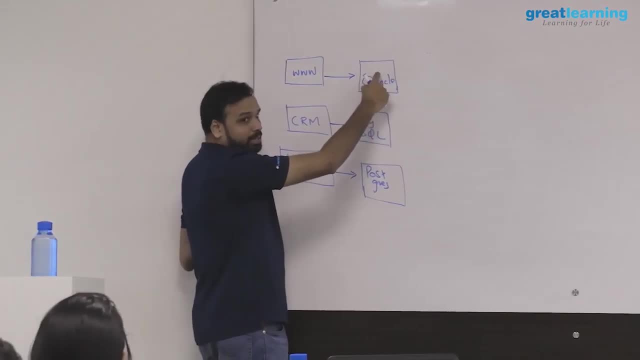 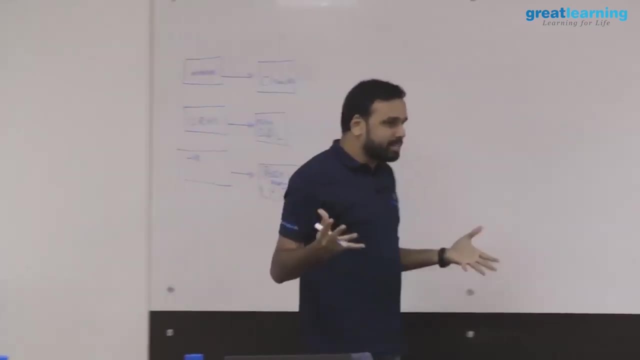 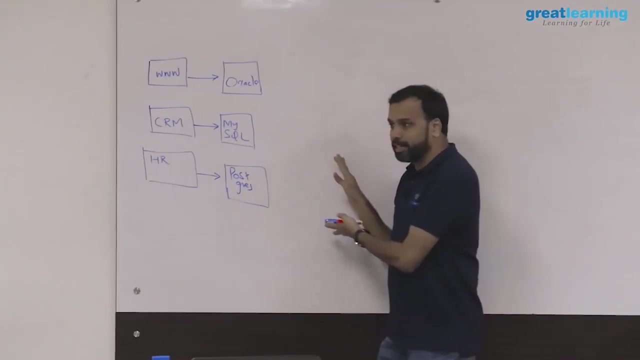 Because your transaction data is in Oracle, Where the customer data is in MySQL and some other data is here. So if somebody needs to do some sort of analytics or want to get a report combining all this data, the only way is that I need to get all the data from these three guys, which normally is not possible. 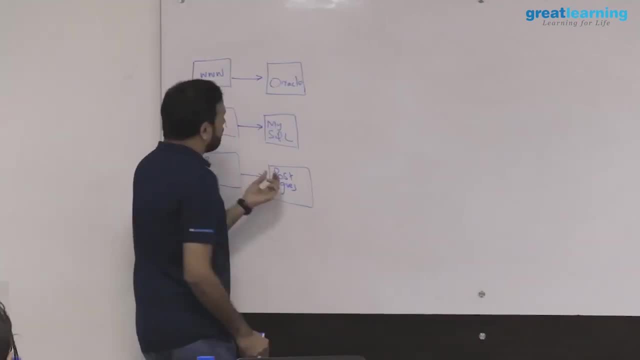 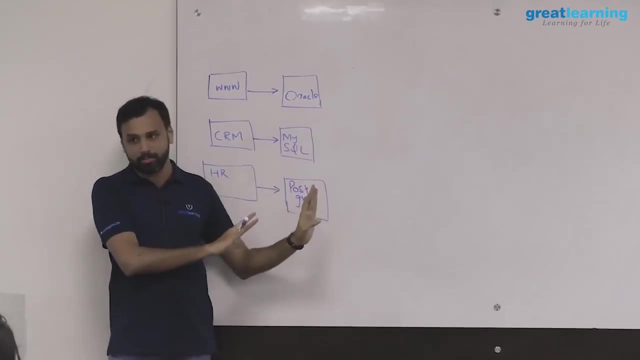 Why it is not possible? Because usually these databases are very busy. They are serving their customers, Right. So this database is very busy, This is busy, This is busy. You can't touch them. That is where, in the traditional world, we do something called ETL. 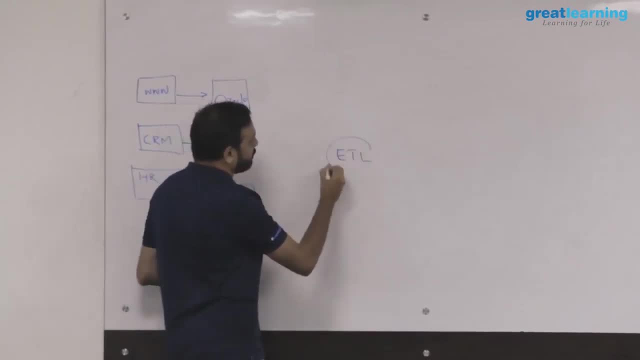 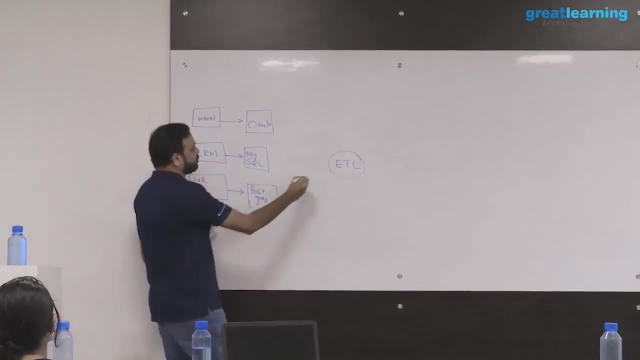 That is something called ETL. Maybe some of you have heard about it. Okay, It stands for extract, transform and load. So basically, ETL is a tool. You connect this with all these sources And you say that, hey, pull the data. 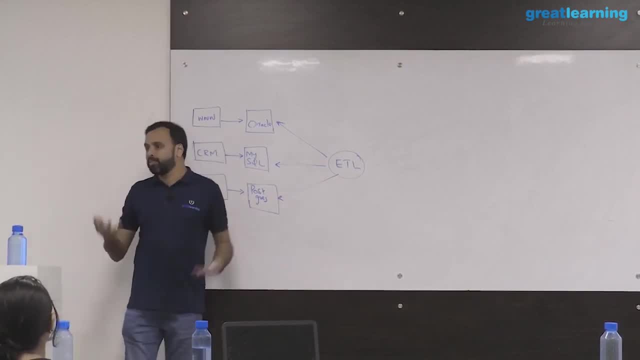 Right, So every day, at, let's say, midnight 12 o'clock, an ETL job will run And at midnight 12 o'clock all the data from these guys will run. All the data from these guys will be pulled towards, let's say, a data warehouse. 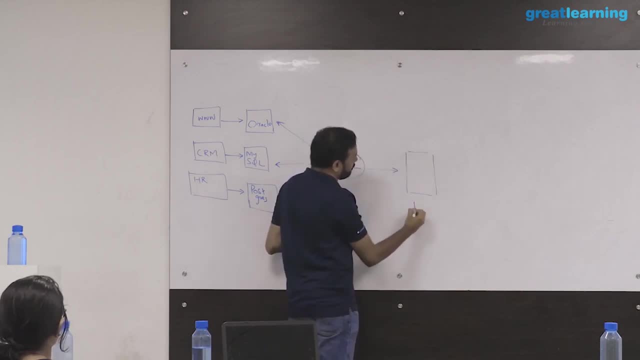 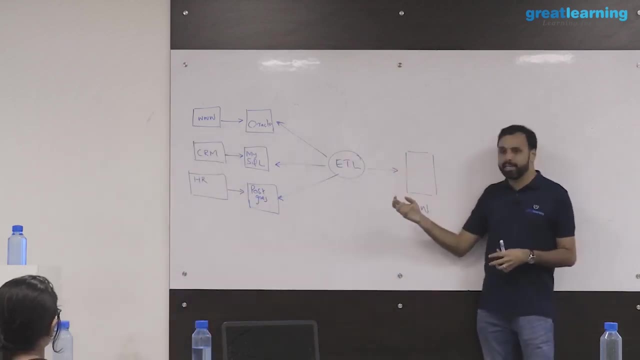 So here you are going to have a data warehouse. This is called your data warehouse. So basically, the data warehouse is a place where all this data is getting dumped Right So that you can look at the data and analyze the data- Very simple. 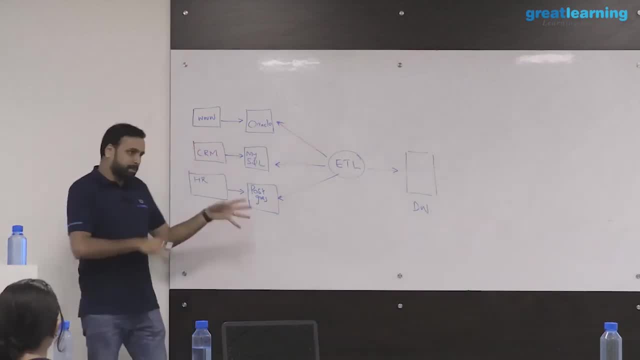 Right Now, and this is something which has been happening in the industry for like past 30 years. It's not something I invented, Okay, This is something that is already there in the industry And people were using this for quite some time. 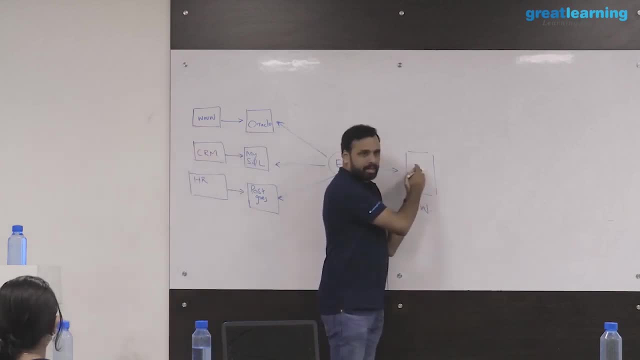 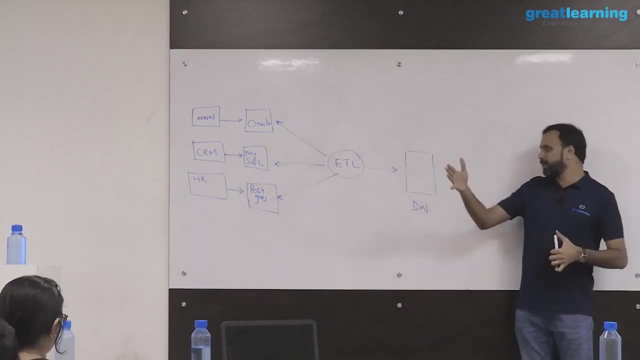 Now, once you have all your data here in your data warehouse. the beauty is that this data warehouse is internal to the company. That means the external customers are having no access here, And I can connect my business intelligence tools- things like Tableau. 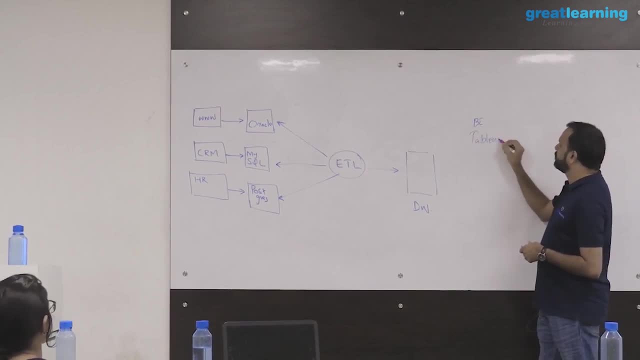 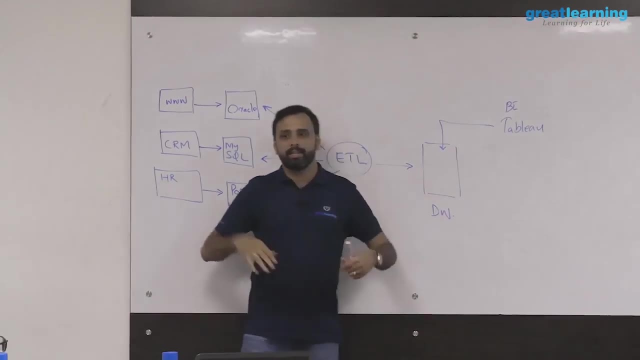 I think you're learning Tableau in your course, So I can. you completed Right, So you can just connect your Tableau to a data warehouse and then create visualizations. Right, You completed Tableau, So you very well know this. 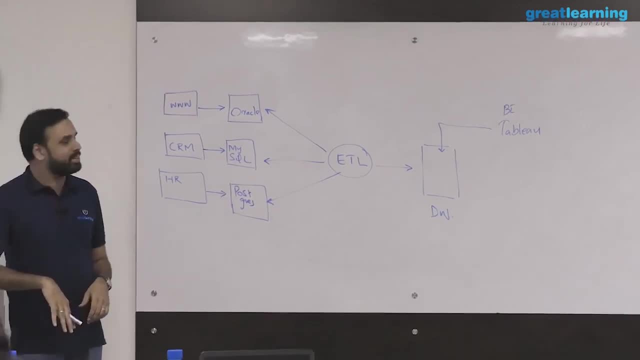 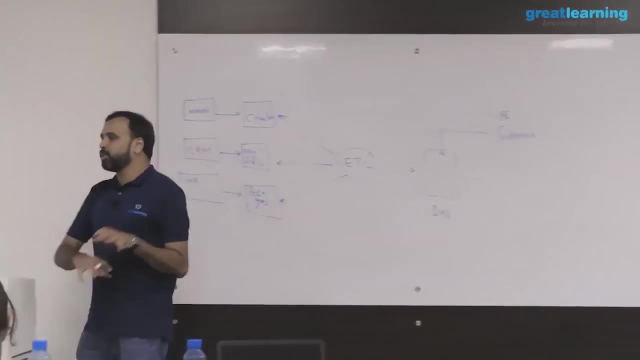 I mean this exact picture, Right? I don't have to tell you, by the way, Right? So Tableau is one of the tools which you can use to visualize your data, Right? And so this is how the industry has been working for quite some time. 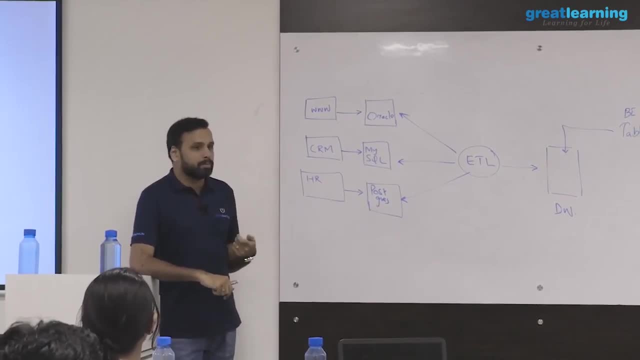 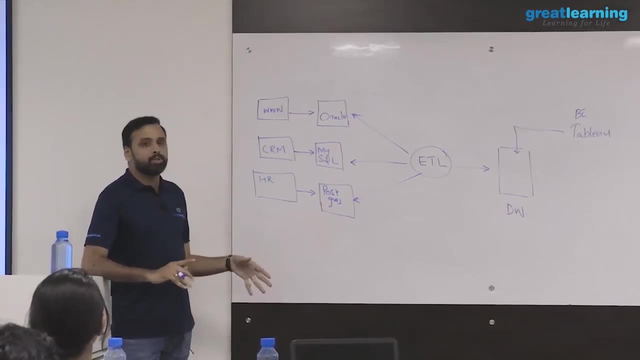 And this is perfectly fine, No troubles. But the real problem is: so this was a nice diagram in 2002 or 2004.. I don't mind. But when I go to 2010 or 2015, if I fast forward, my problems are bigger. 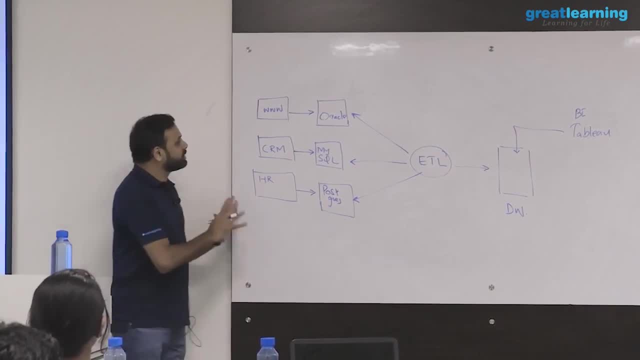 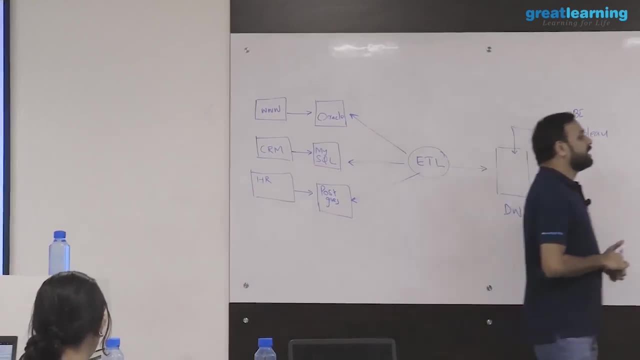 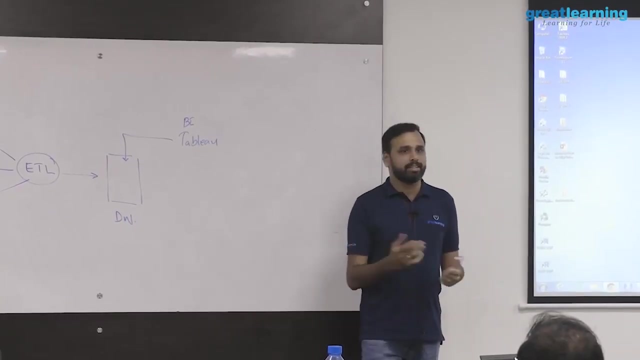 So one of my problem is that I don't just have data in my database, I have data everywhere, Right? For example, when was the last time you actually went to a mobile shop and purchased a mobile phone? I don't remember. I order it online. 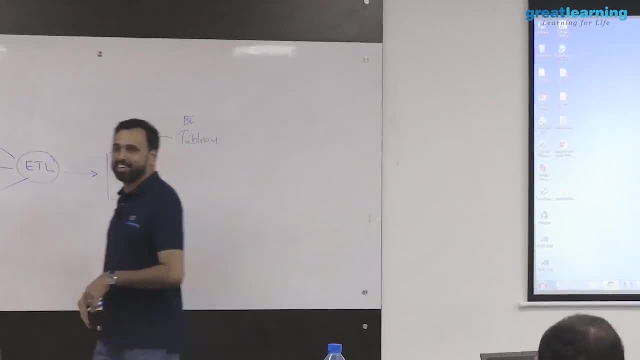 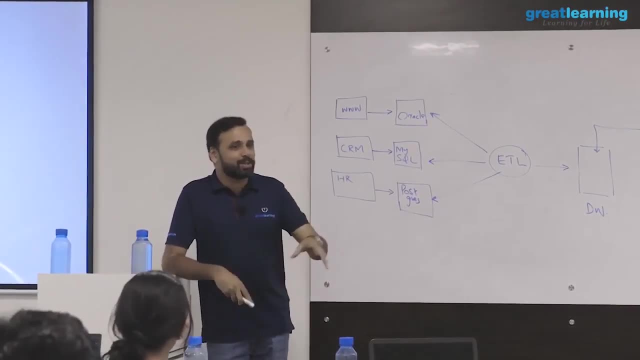 Right, And practically you are all Bangaloreans, I believe at least. So you order everything, starting from groceries to rockets, online, Right? I mean, I'm not from Bangalore, so we still go to show, but you guys order everything. 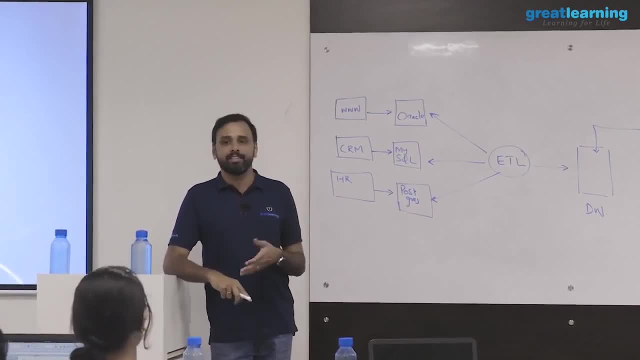 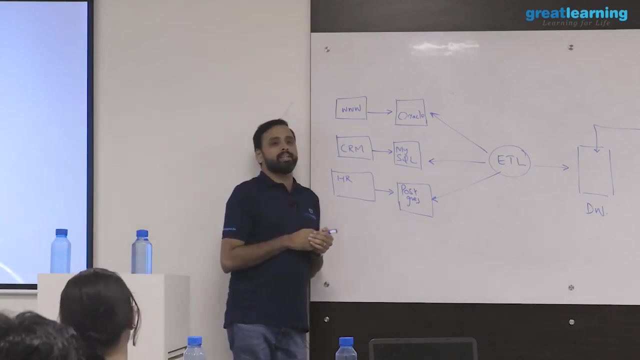 online, Right. So what does that signify? If you can order everything online, that means all the businesses are online and all the customers are also online. Everything is online these days, Right, So that means that also means that I was also working with Flipkart for quite some time. 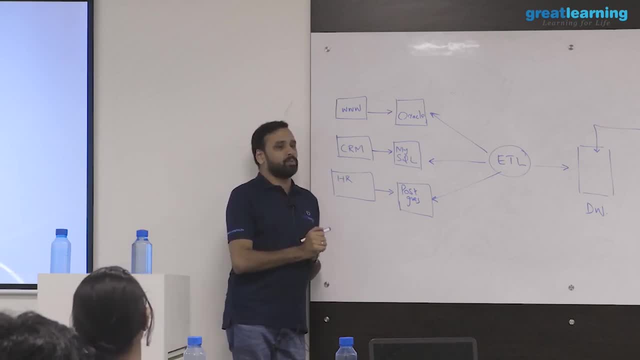 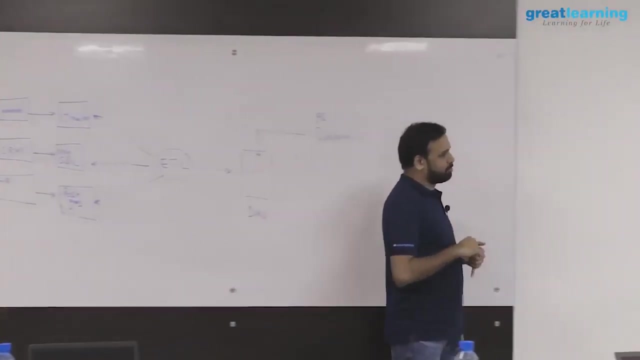 Flipkart was one of my customers Right, So I had the chance to work with them for a variety of their use cases. So if you look at a company like Flipkart, their major revenue is actually from the website, I mean, or the app. however, you purchase stuff from Flipkart. 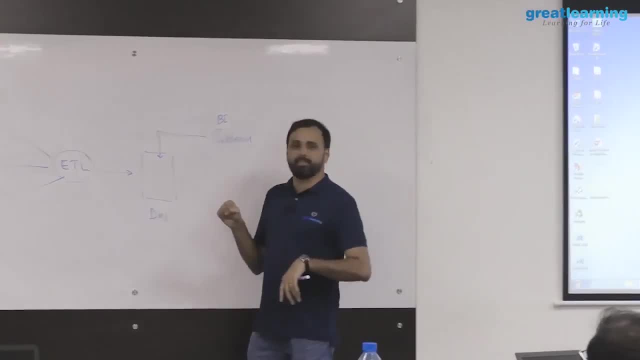 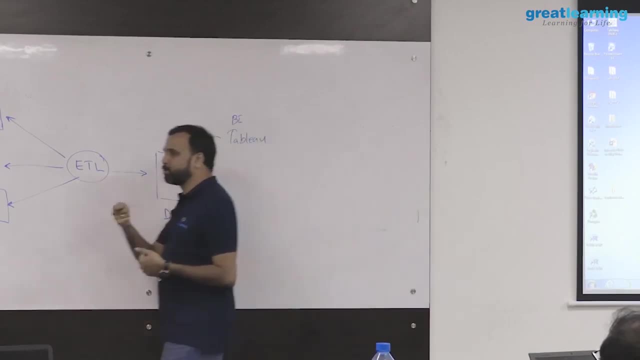 So what they do the moment. let's say you open Flipkart's website, either online or either on your laptop or the app. they start tracking you. From which IP address are you browsing? Which city are you browsing? How much time you are spending on a product page? 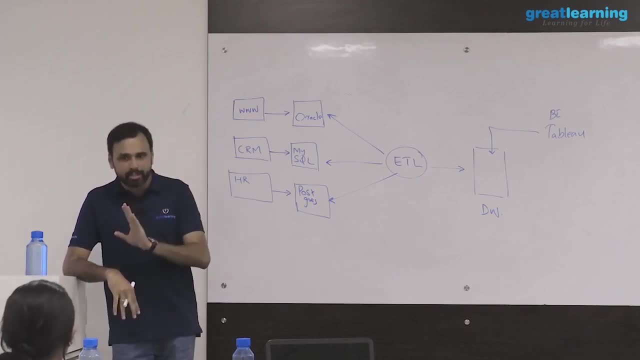 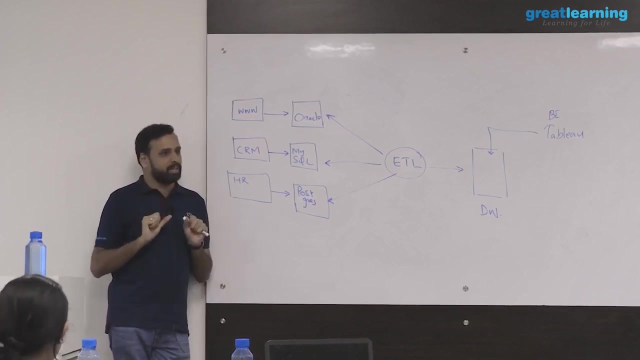 Which items you are zooming, Which items you are adding to cart. All this activity you do is being captured, So this is captured in multiple ways. One: they collect all the log files. So whenever you browse the website and leave, you create log entries. 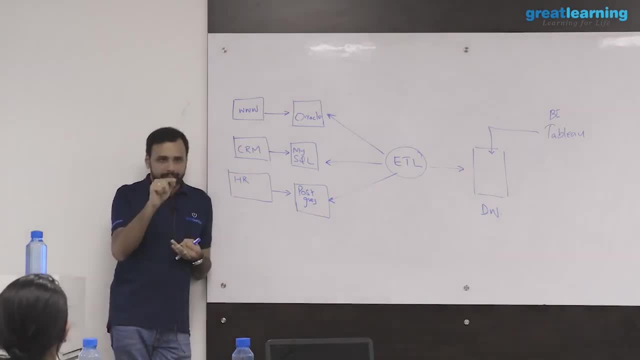 Second thing, there is something called clickstream data. The moment you click that's called clickstream. It will generate a report: which icon you clicked and what was the effect, etc. So clickstream data, then log data. they capture for every customer. 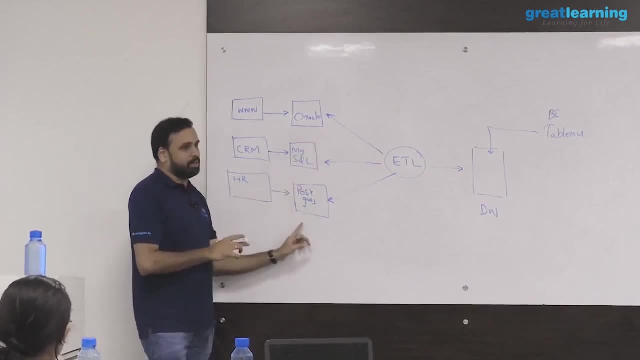 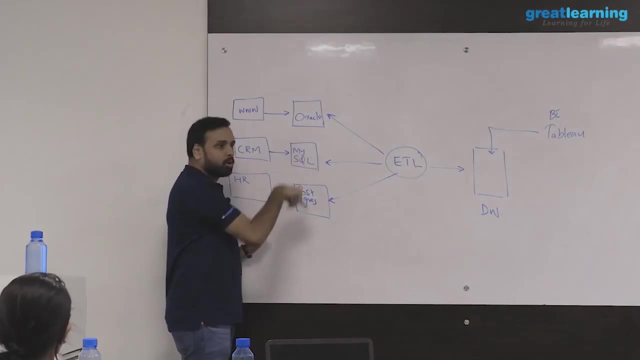 Now I don't really have a way to dump any of that here. Clickstream data and log data are not really something which I can fit in a table. RDBMS table- It's not row column format. I don't know what to do with that data. 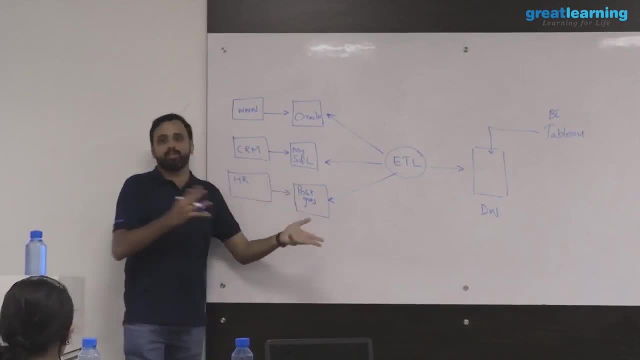 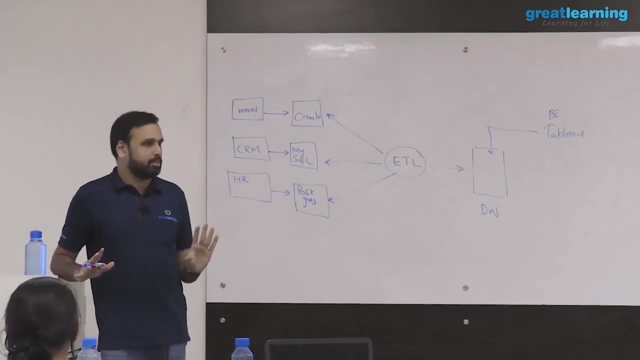 Question number one. So my traditional architecture may not really work in case of Flipkart, Point number one. And every day they have millions of log entries, practically Millions of log entries, So that data is coming in and they don't know what to do. 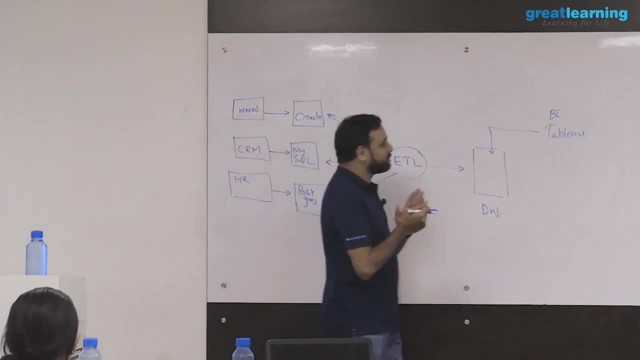 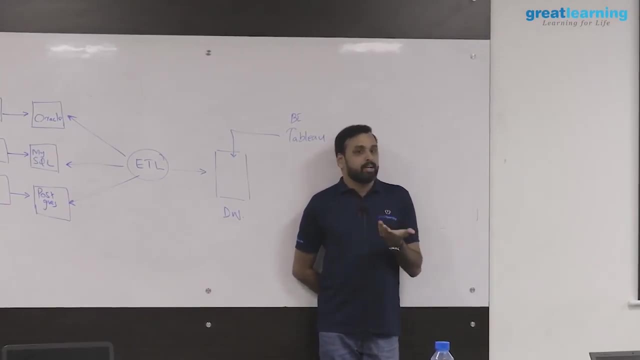 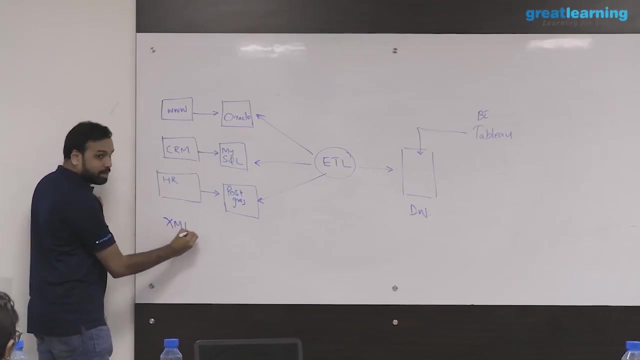 And from the app. they also collect the data like how much time you are using the app and a lot of statistics about the app, the way you use your app- right So that data they collect in a format of XML. The data comes in XML format, not in the normal row column format. 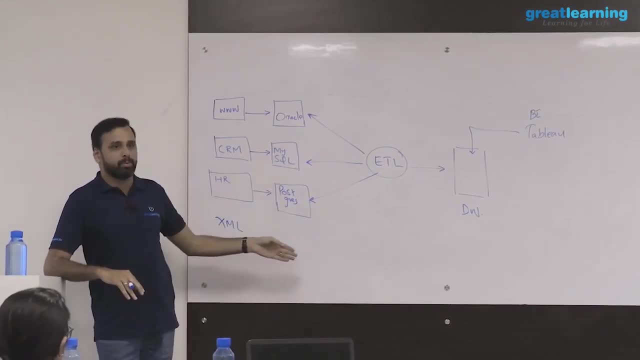 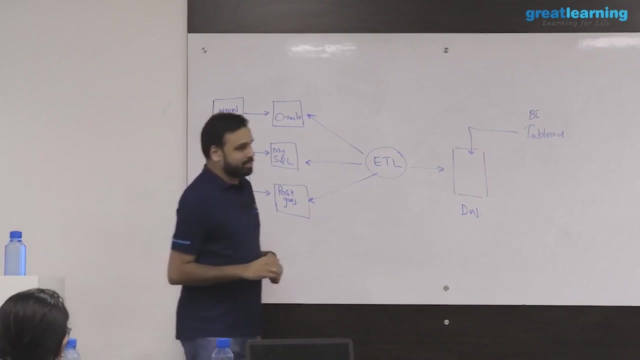 So that data also. I cannot put it anywhere here. to put it very simply, Then, Flipkart also collect a lot of social media activity right Around the city, around India, as such Like. so it is Diwali right. 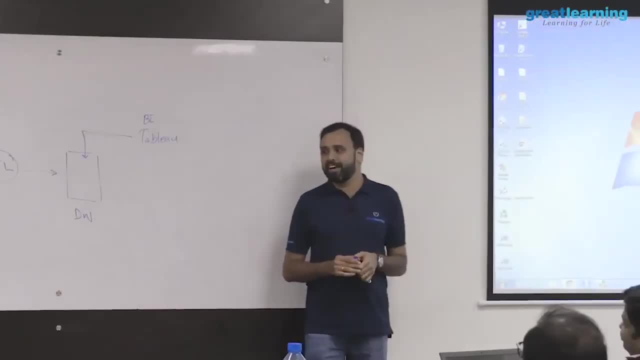 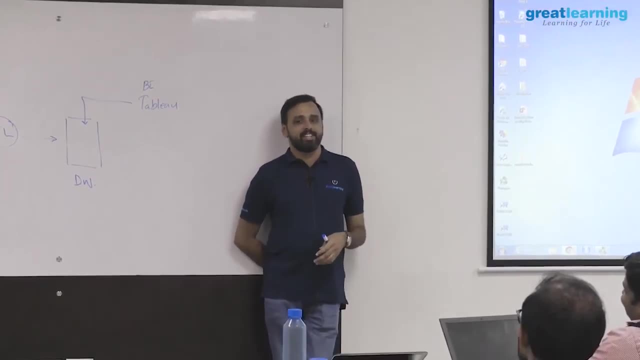 Or it was Diwali. Diwali is over, right? So during the Diwali season they conduct this. What do you say Sale festival? What do you call it Big billion days? So basically a way to empty your pockets, right? 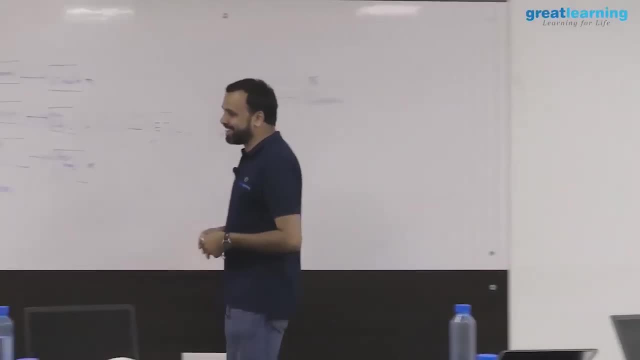 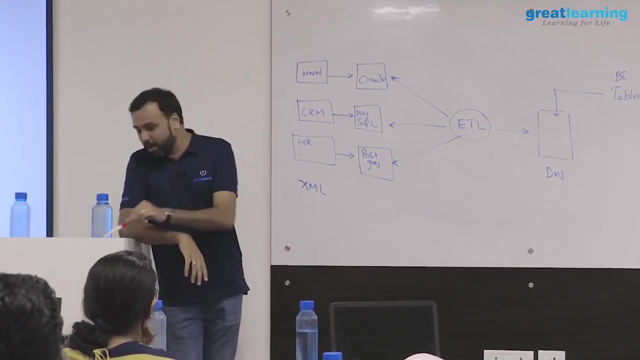 So, to put it in a nutshell, but they call it as huge discounts and profit for them, right So? but how do these sales things happen? So, when big billion days were there for the first time, I was at that time, I was working. 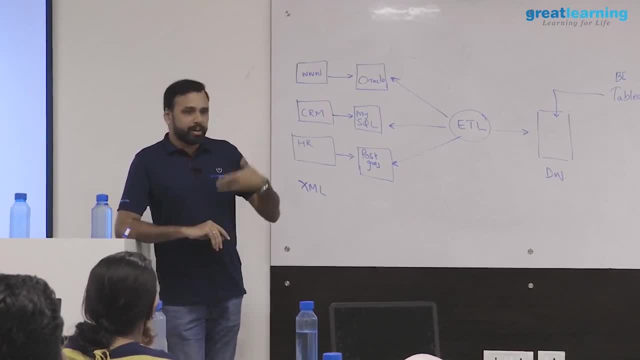 for Flipkart for some time. So what they do is, first they will analyze the market, So they will look at the trends and also what people post in social media, and all to understand what is the interest. So they will generate something called interest token. 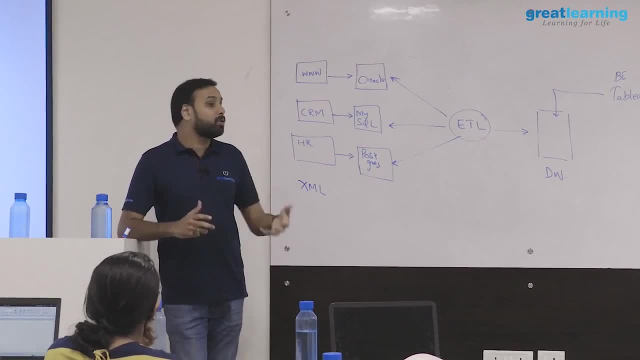 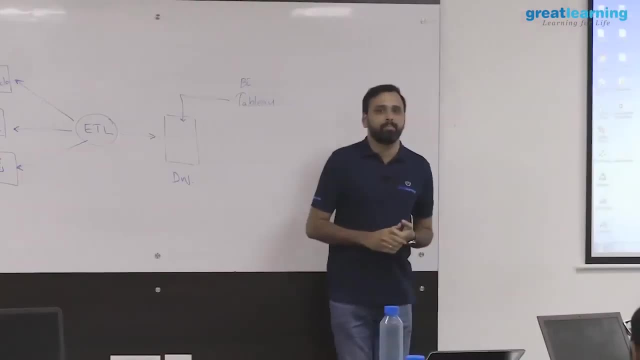 So that means what you guys are really interested. How do they generate it? They will send you mailers and websites. So let's say there is a new phone getting launched- Apple iPhone. what is that? X, something? XR? Okay, the next iPhone, right. 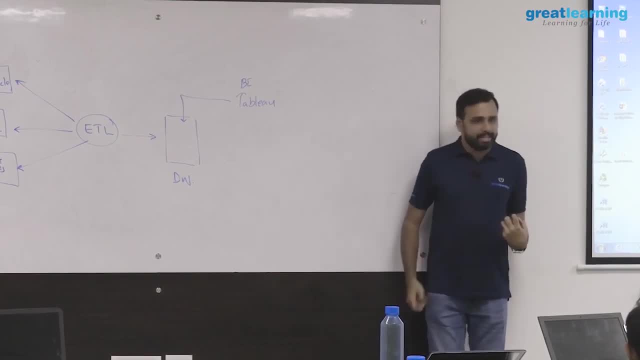 So they will collect social media. They will collect social media data from Twitter and Facebook: whether this particular model is trending, how many people are really following this model, how many people really like this model, et cetera, et cetera. 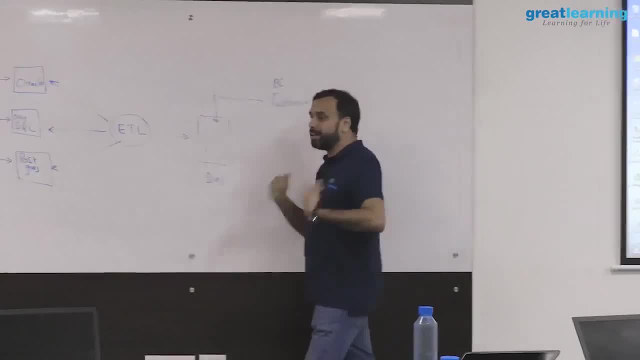 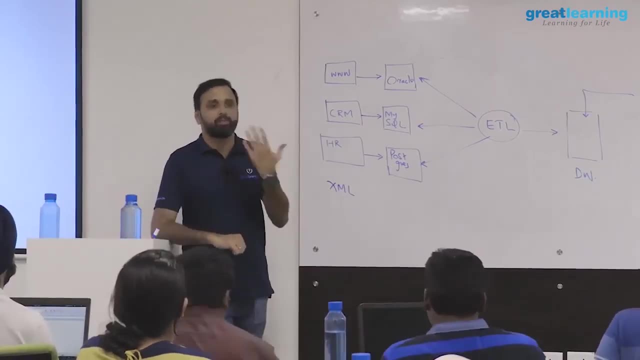 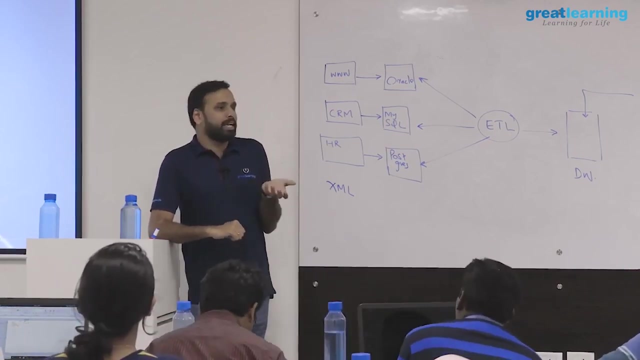 So first they capture all this data right, And then they decide on the actual day of the sale what they should sell, on how much amount they should sell, et cetera, et cetera. So if you are looking for something like big billion days- the amount of data they collect- 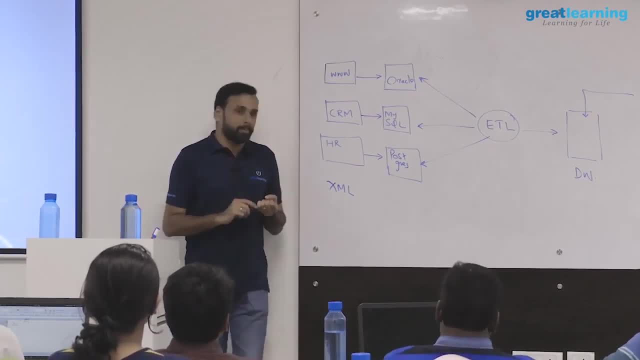 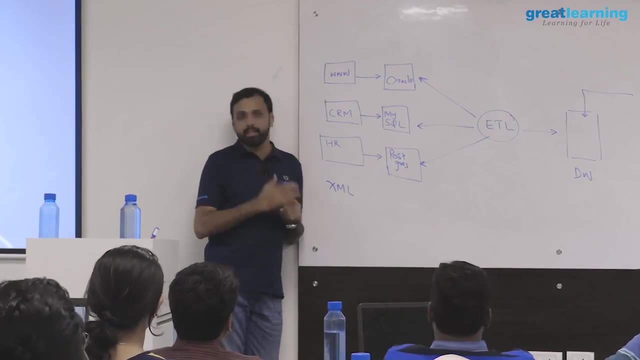 capture is in terabytes actually, So that comes in the format of images. If you collect from, let's say, public feeds in Facebook and all, and news articles, comments and tweets, The Twitter data right, the tweets that you can get in JSON format. 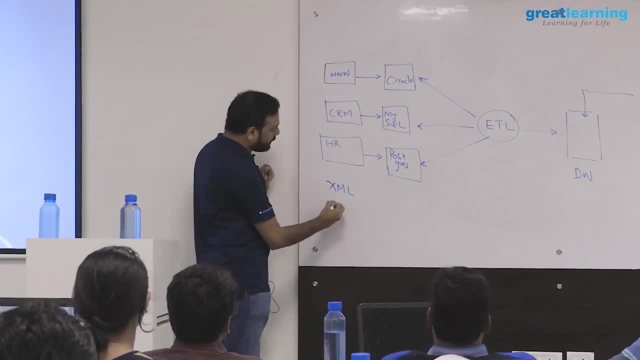 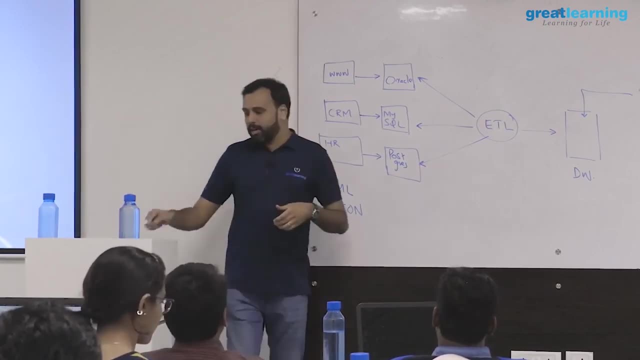 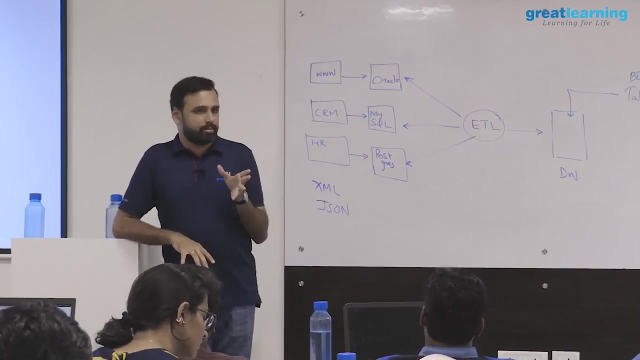 There is a format called JSON Twitter data. you can typically get in JSON format- This is key value pair- again right And then from Facebook If you are planning to sell, If you are practically downloading the data, it comes in a typical format called graph. 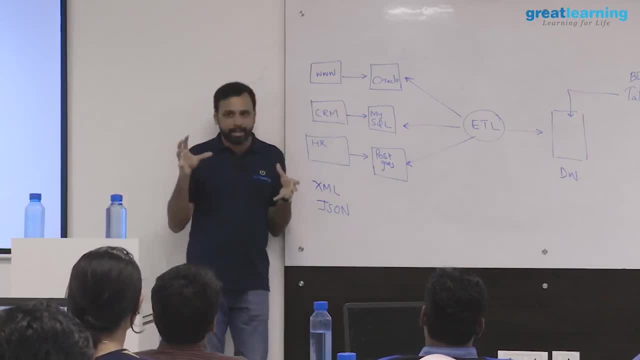 graph format. Facebook uses something called a graph API to represent the data, So it pretty much is like a graph: the data comes in And then the text data, like what people commented, what people wrote, what news article they read, et cetera, et cetera. 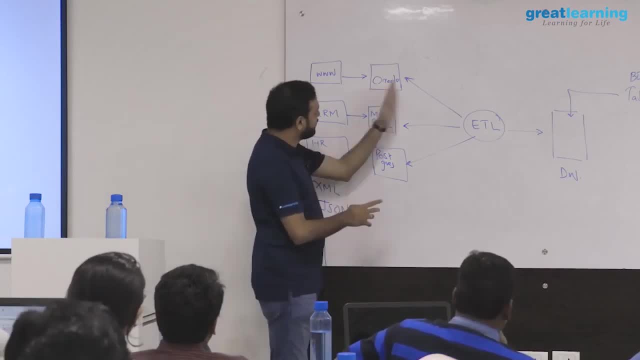 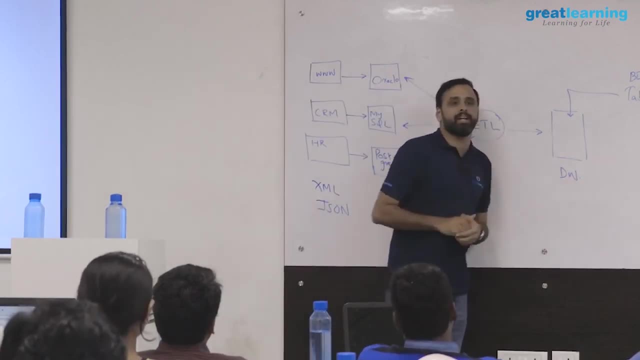 So if they are getting all this data, first of all they cannot feed it in this such a structure. If they are able to feed it, if you dump it in a data warehouse, you have no ways to analyze this kind of data. 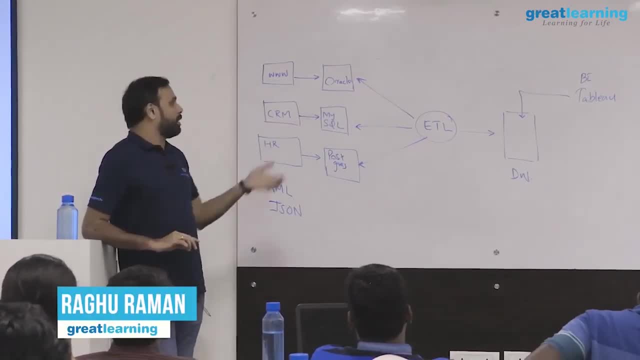 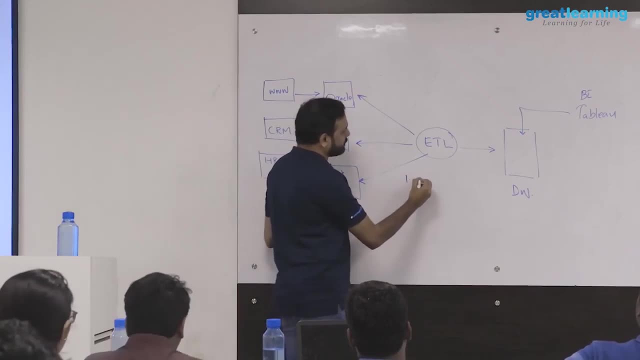 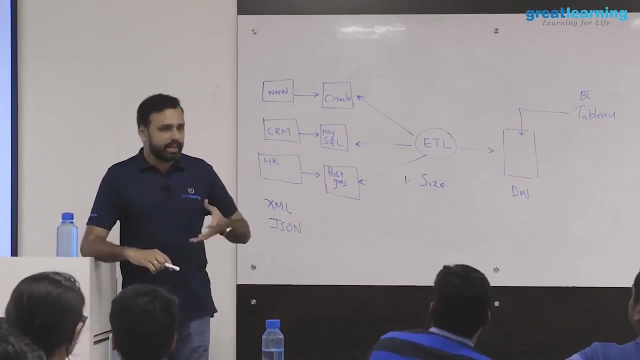 So the problem that we face today, or what I would like to call as big data, is that, first of all, when you say big data, one thing that matters is size of the data, Size of the data. So the industry has changed in a way that today, every business is online. 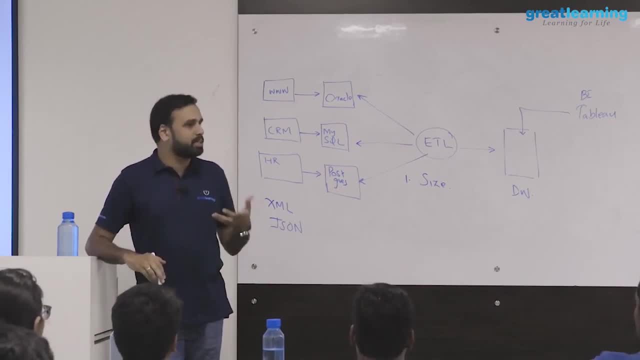 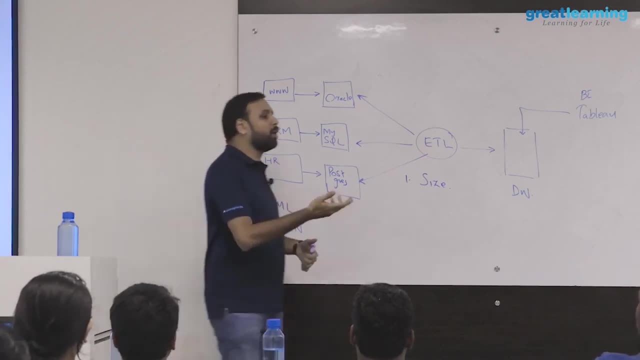 And people want to collect more data. They want to collect more data about the customers so that they can understand their customers better. So previously, if I'm selling something, I will have a shop and people will just walk into my shop and they will buy something. 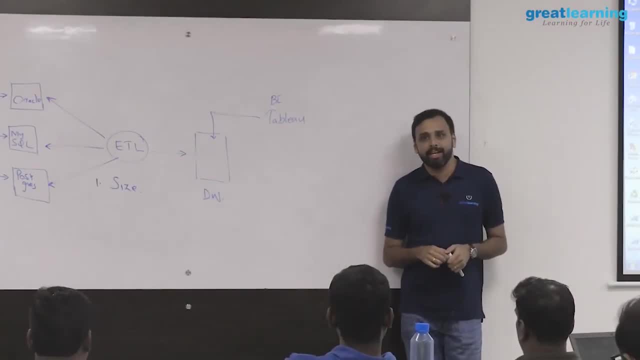 I don't really care. So today it is not like that. I can show ads and catch people. Even if you're purchasing something from me, I can recommend products to you. So if you go to Amazon or Flipkart, you can see the recommended items based on the previous. 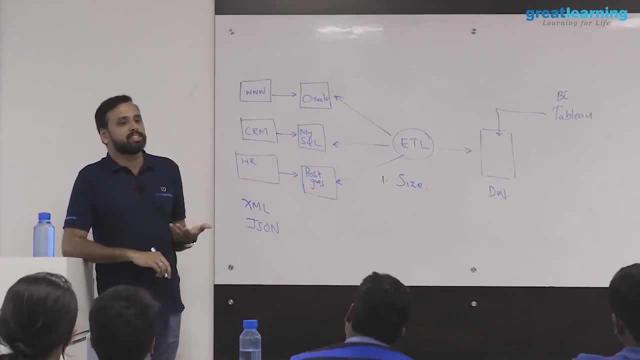 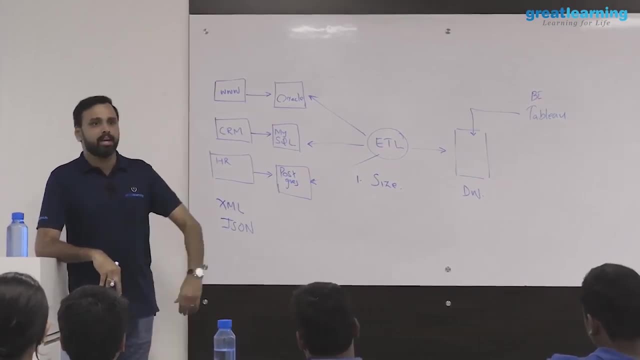 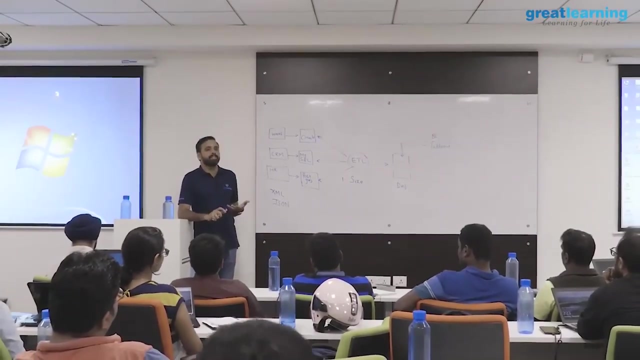 items you bought right. So today, since businesses are online, you can gather more data from customers, with or without their knowledge, And using this data, you can do analytics and understand your customers better. So to do that, the first thing is that you capture the data. 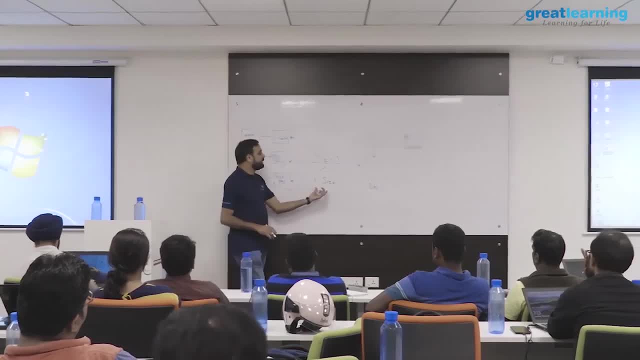 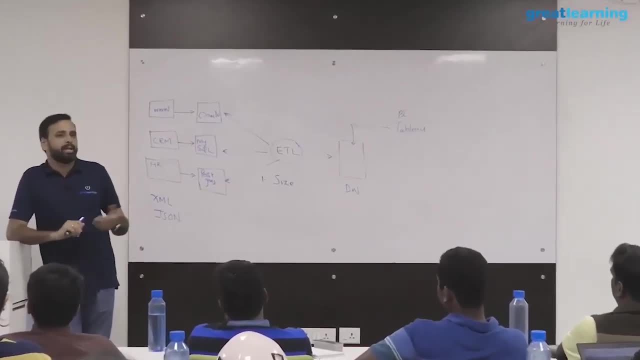 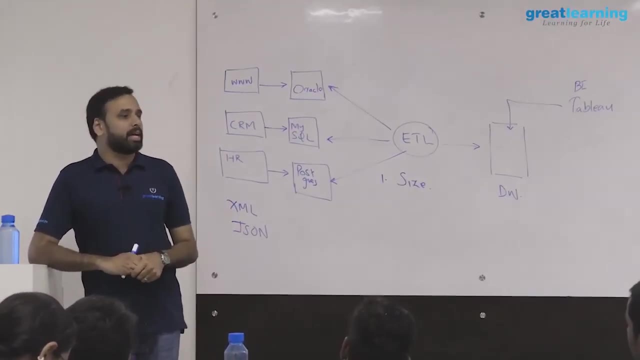 So when you capture the data, the first thing is the size of the data. So if I'm talking in the megabyte or gigabyte spectrum, that is okay, Anybody can handle. But when I go to terabytes and petabytes of data, your traditional systems cannot actually. 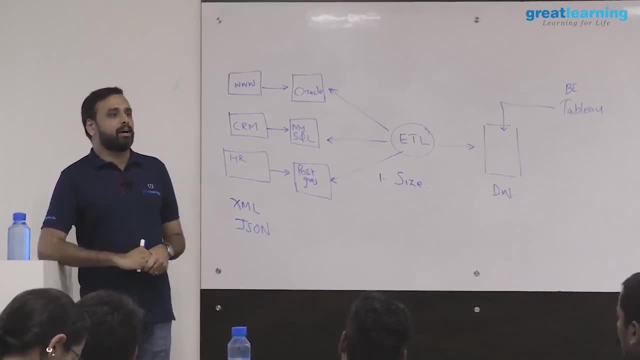 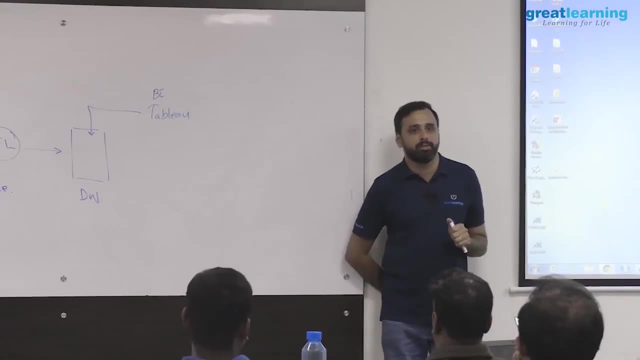 store the data. That is a problem, right, Like this cab company, right, Uber. Uber collects 80 terabyte data every day, 8-0.. So in a month they are collecting what 800 times 3, right. 2,400 terabytes of data every month. they collect Why? Because all this data is related to which route you are taking, how much time you spent on traffic, who was the driver? did you give him a one star or a five star? 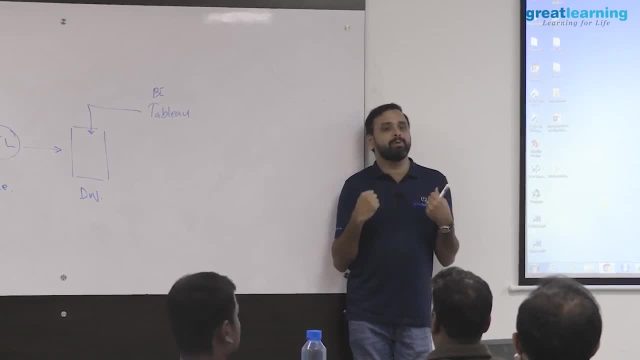 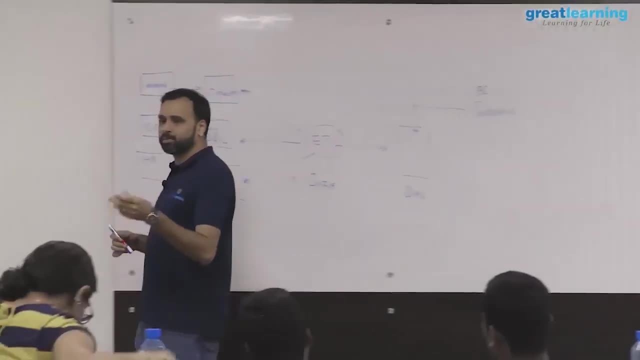 All the statistics is collected And that will help Uber to analyze and predict what is going to happen. This search pricing, right, You see, this search pricing. Sometimes, when you open the app, they say two times, three times. So how are they able to do search pricing? 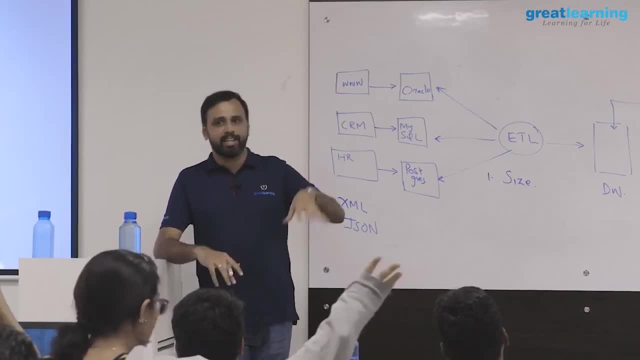 That is based on analytics. Uber knows that. let's say, in Bangalore, In I don't know- Whitefield, They give it to the driver. also, I have seen Uber drivers. Yes, They will know from this area if they drive to. 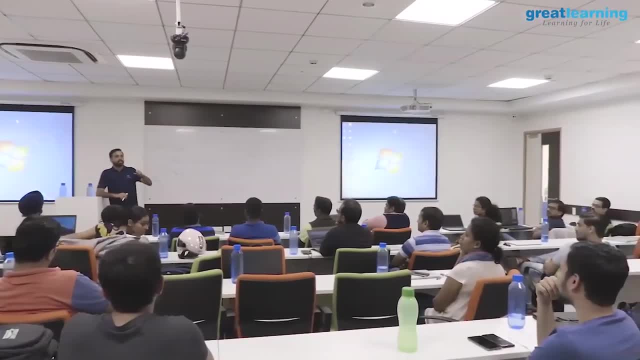 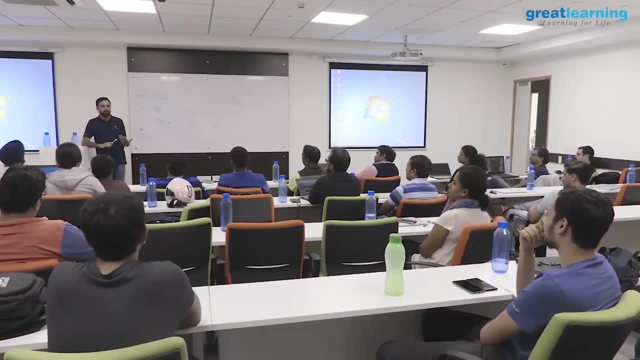 Yes, They will have eyes on searches Exactly. So that is done because their algorithm is so perfect. It has all this data to you, know, churn and predict what is going to happen. So they know at what day, what point, how many drivers are required. 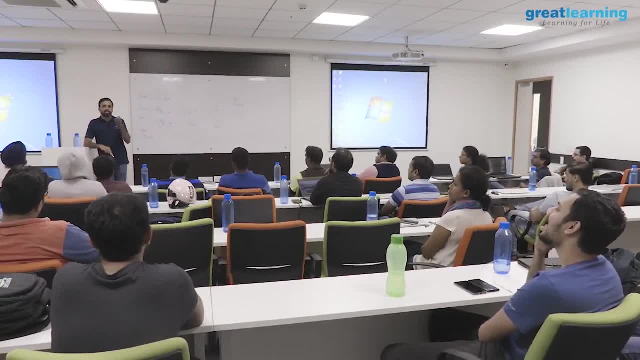 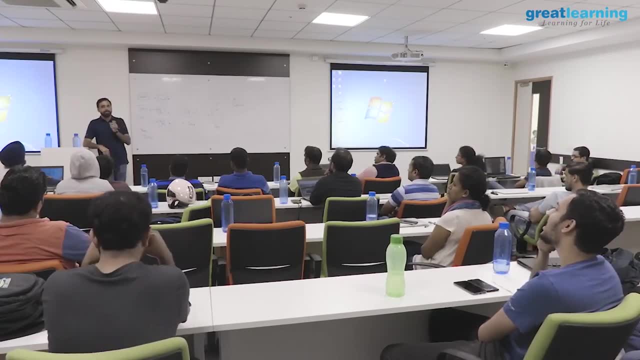 And even when you call an Uber driver, they will know. When you call an Uber driver, there is an algorithm running to decide which driver should come to you. It's not random. So previously it was random, Now it is not random. 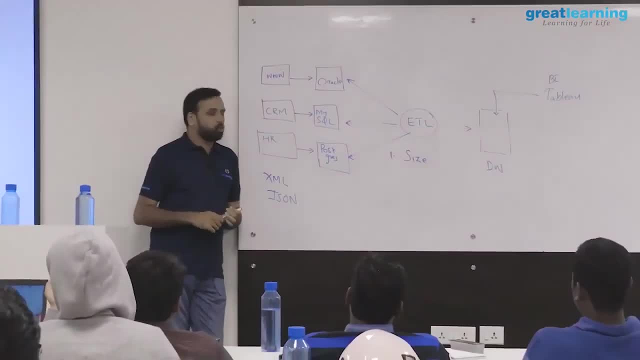 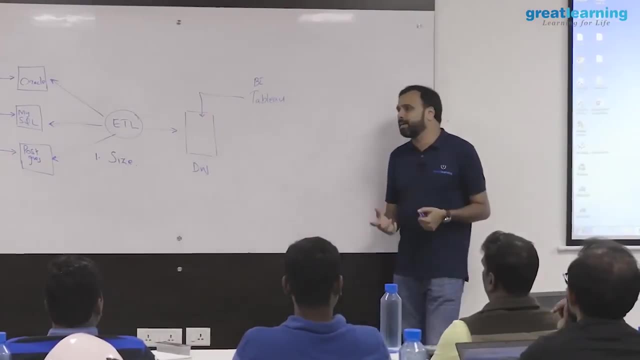 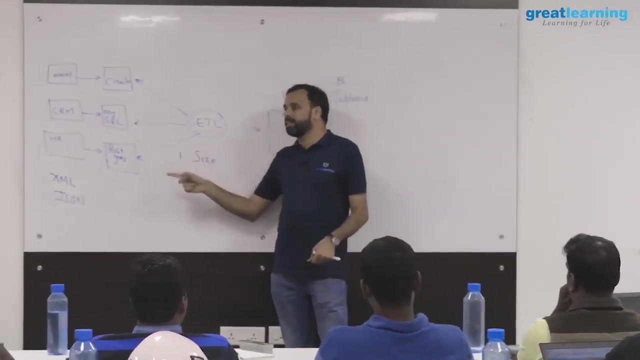 They run analytics and decide which driver has to come to you. So Uber is just one example. Every company does. Flipkart also collects a huge amount of data. Any ecom company, banking company, retail company- everybody collects data. So my first problem with data is the size of the data. 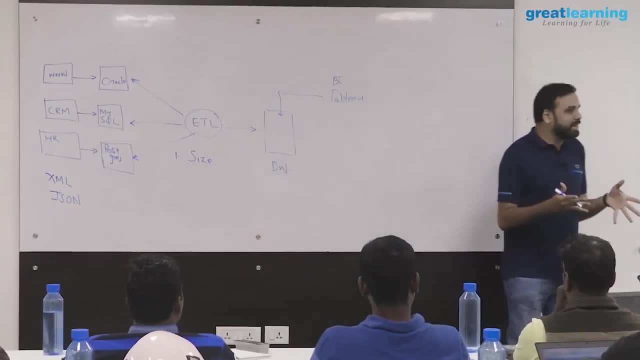 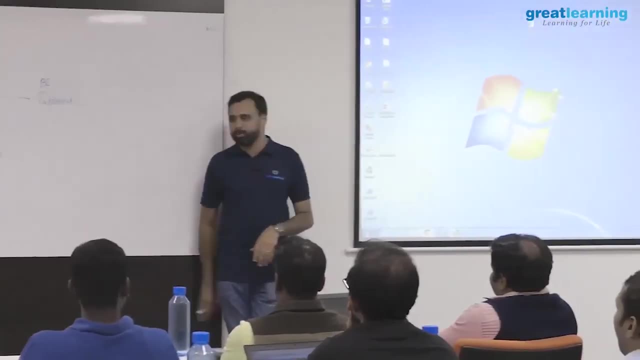 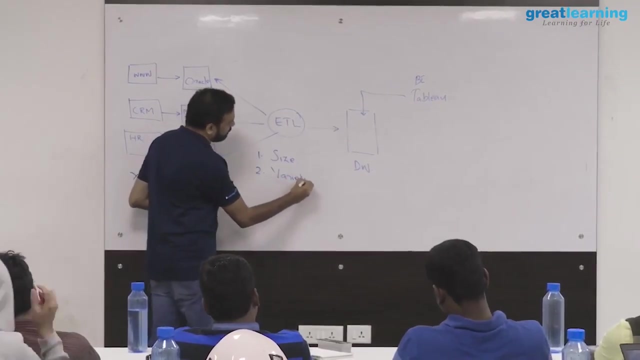 Forget anything. If you're getting 80 TB data every day, where are you going to store it, right? So that's my first problem. I need to figure it out. Okay, No problem. The second problem that I have is called variety of data. 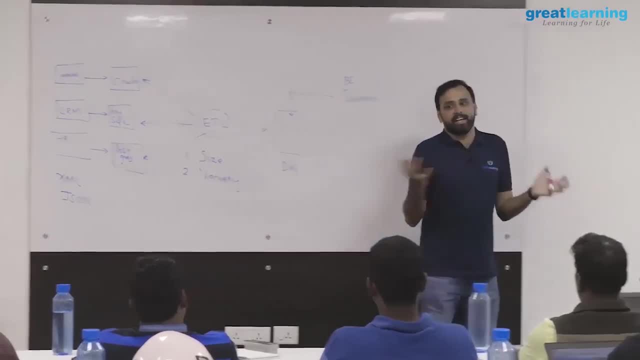 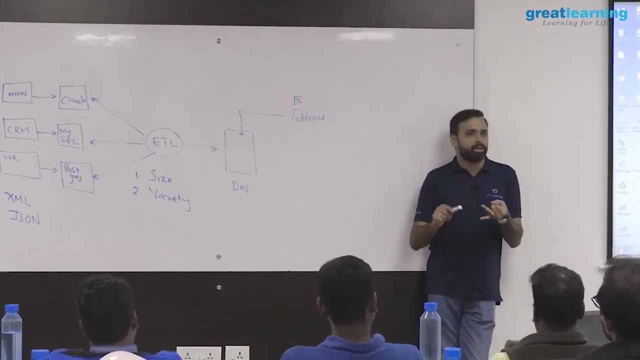 Meaning. not only I'm getting 80 TB of data, I'm getting it in all formats right. I have location data, I have latitude and longitude, this kind of data. I have text data, I have image data. So how am I going to make sense out of it? 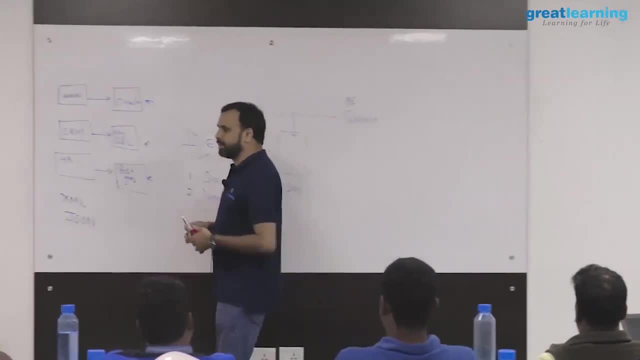 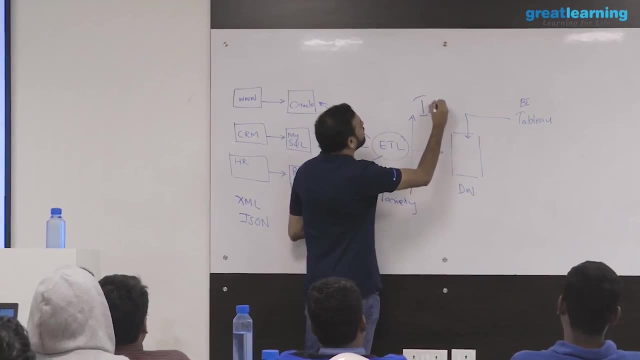 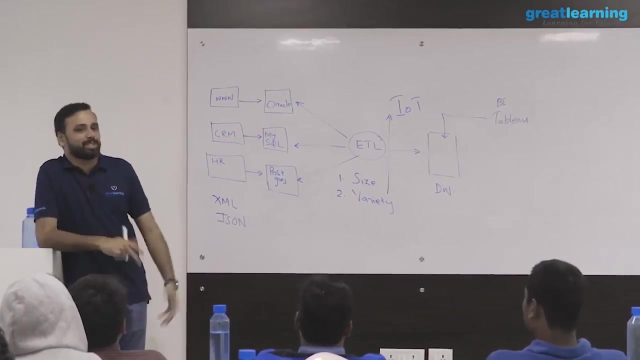 And one latest- I will not say latest recent- culprit in this variety is your IoT devices. You have this almost practically useless home automation systems right, Which God only knows why people are buying. I don't know. Probably it is cheap, right. 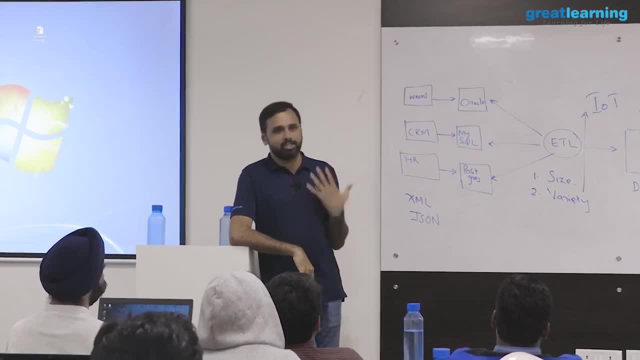 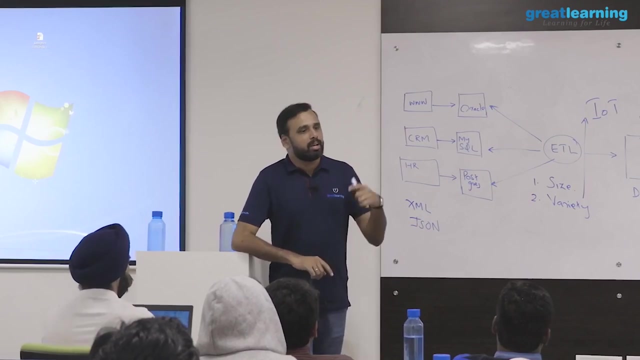 All these IoT enabled devices right. They generate a huge amount of data. Now I'm not just talking about home automation systems, sensors, particularly So thermostat sensors, And we had a customer in Japan, So in Japan, what they do when somebody buy a flat or house that has a lot of sensors? 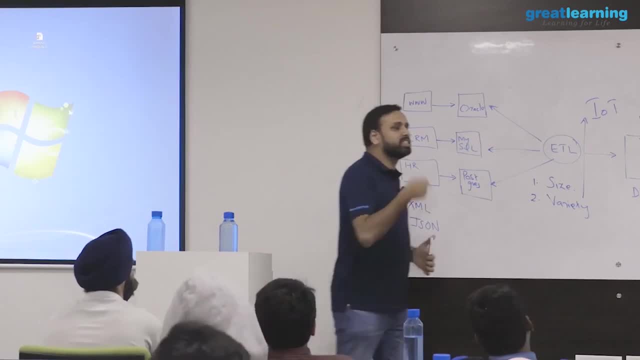 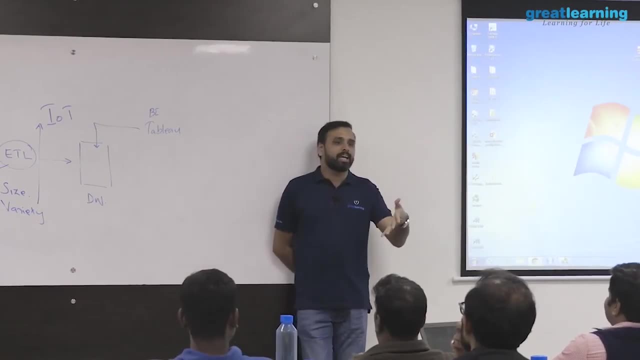 as per the government regulations. So the person who is selling the flat right He is responsible for the flat. For example, if I'm selling the flat to you, if something happens to a flat, I'm responsible, not you. So that's nice actually. 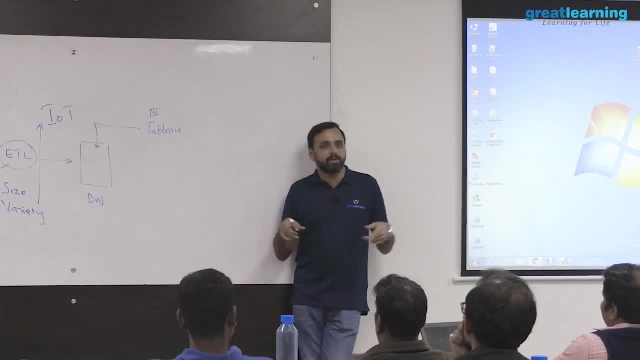 So this company actually monitors the flat, because a lot of earthquakes and all happen in Japan, So every house has around 300 different sensors. They sense everything And this data is streamed into a system where it will do analytics: understand what to do, what not to do, et cetera, et cetera. IoT data. 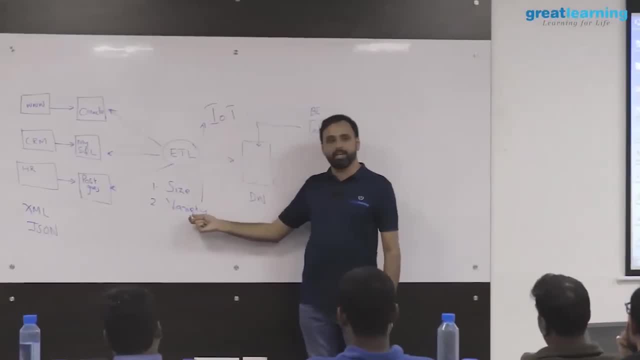 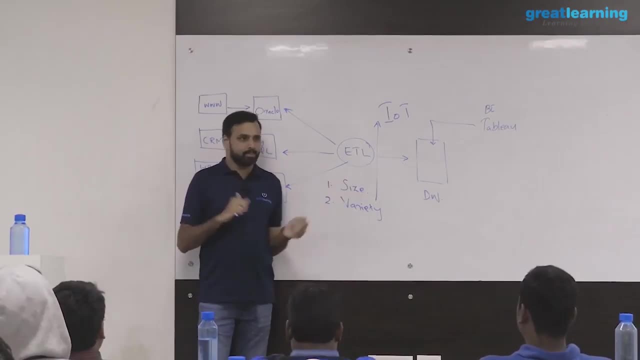 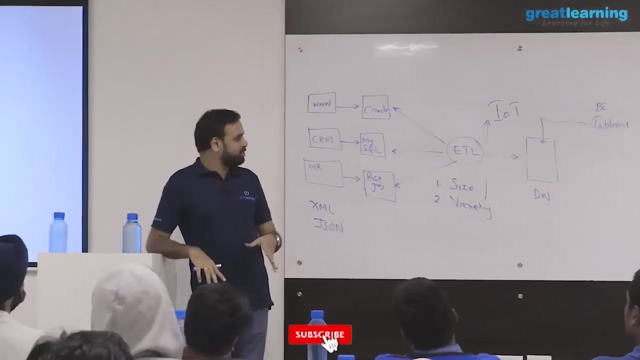 So a lot of Internet of Things or IoT data actually accounts here for variety. So size is one factor when you talk about big data, Second factor is variety. So what will I do if I start getting 100 terabytes of data every day? which is of different? 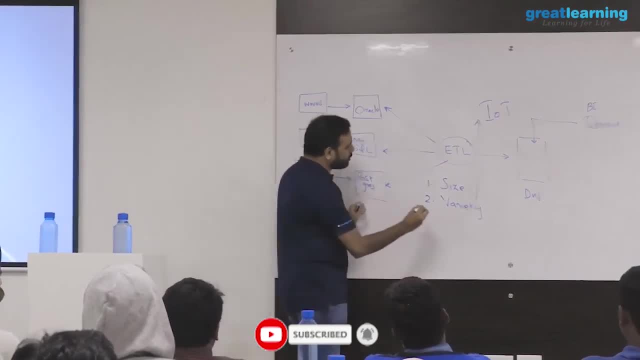 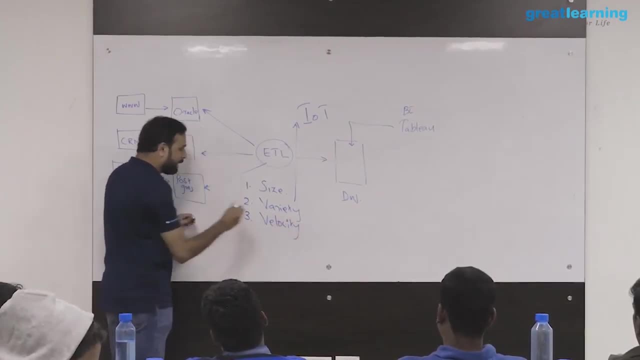 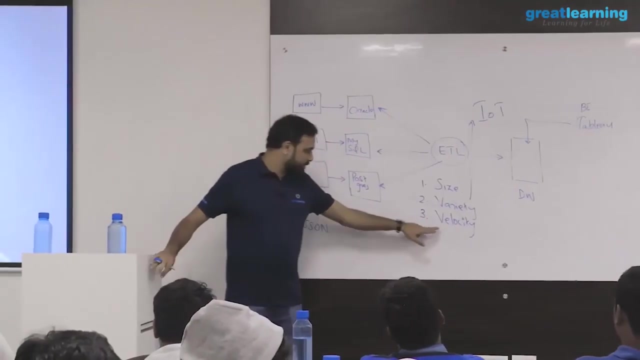 different type. What will I do? And third and most interesting point is something called velocity. So this is an area where I am working recently: Velocity- Most of my work actually is in this side right now because there is a lot of demand for this. 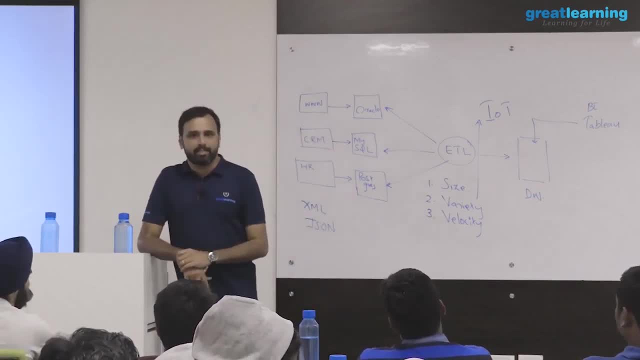 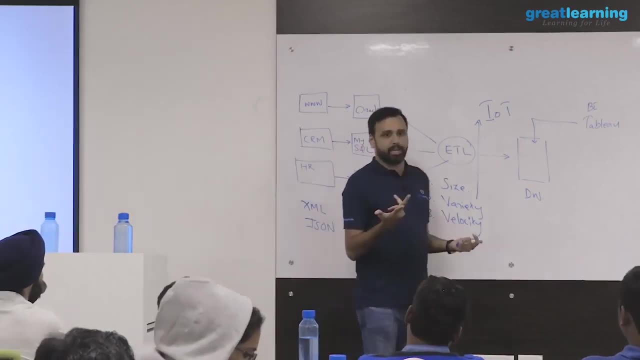 Velocity is actually real-time analytics, So this was not so popular before, but now this has become very popular. Why this has become very popular? So, to give you an example, I don't know. So let's say you are using a credit card. 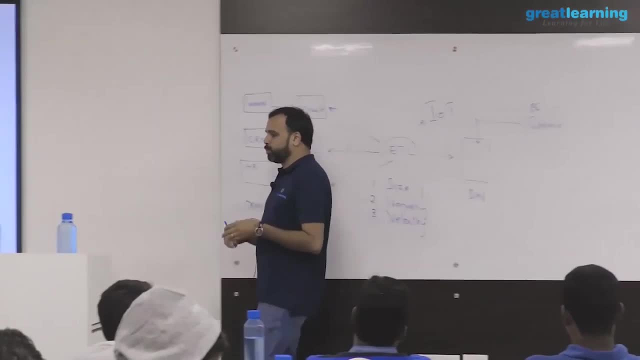 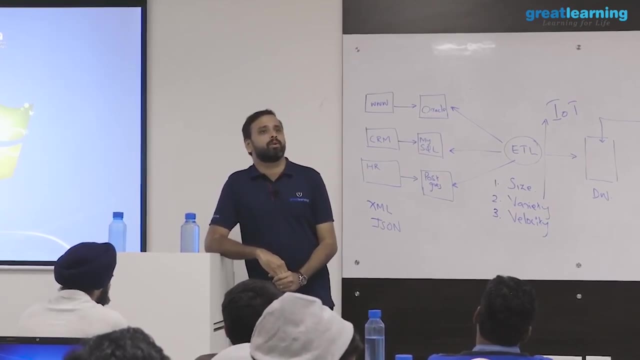 So you go to Appendix, You go to a place, you swipe your credit card or you swipe it online. right, Let's say you are swiping for I don't know one lakh rupees. You swipe your credit card for one lakh rupees. 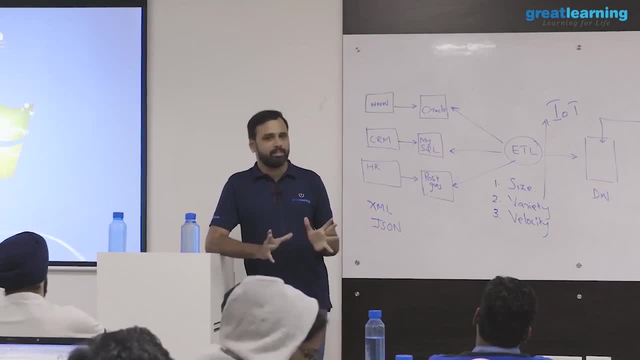 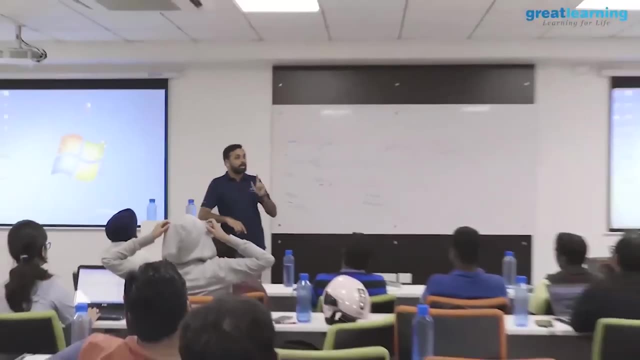 What will happen? Transaction happen, then what will happen? Nothing will happen. Message. we will get then what You get a call, You get a call. Have you ever noticed Message is different? I will tell you. Message will be automated. 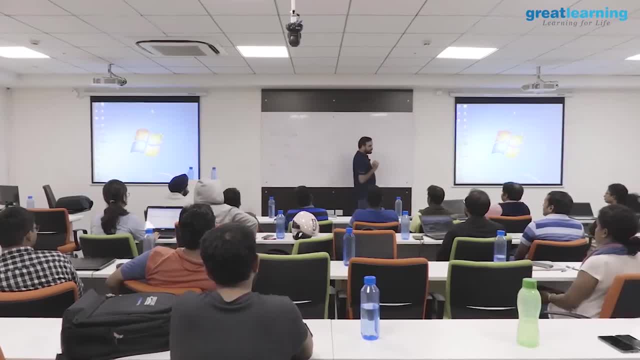 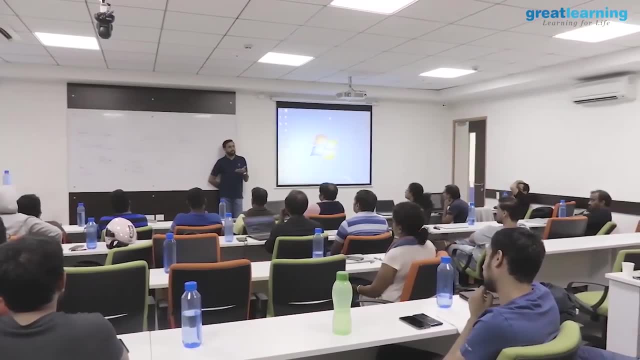 Even if you are swiping or not- I mean debit or credit- you will get a message. You will get a call from the customer agent, right? He will say: did you actually swipe, Right? And if yes, do you want to convert to EMIs? et cetera, et cetera. 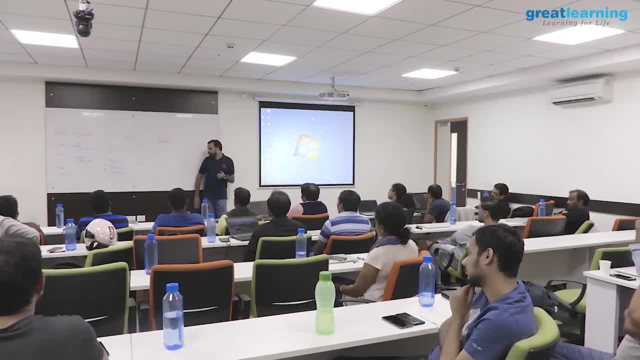 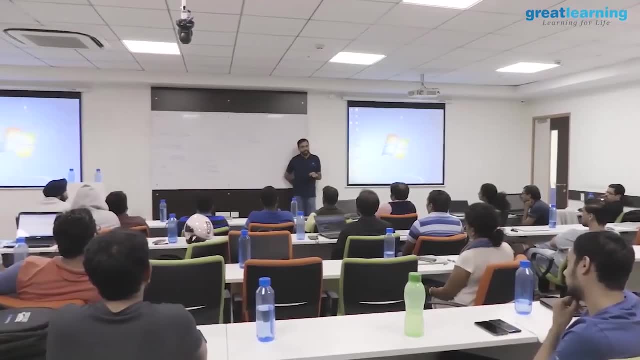 How this is working right. So back in 2013, we had implemented this for Citibank. I was part of a project where we were working with Citibank. Now it is not a big deal, but in 2013, it was a big deal actually. 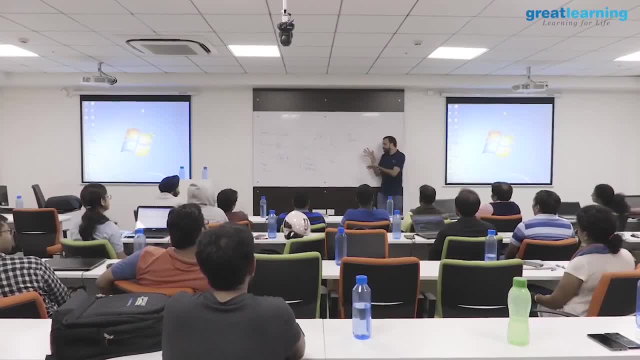 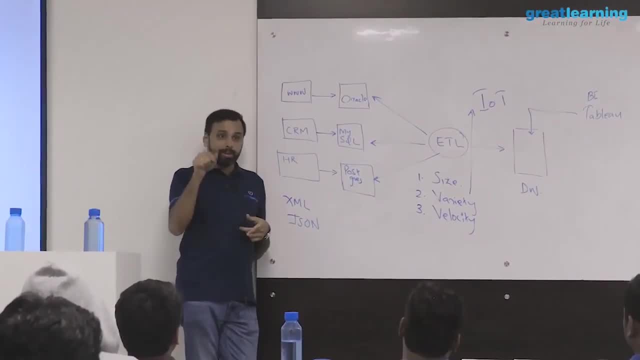 So this is called real-time analytics, meaning there are specialized systems which can handle this. What happens is that all your swipes, so the location where you are swiping, how much you are swiping- all these checks are done to initiate the call. 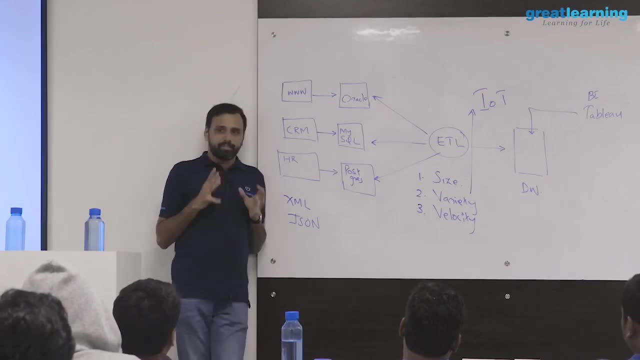 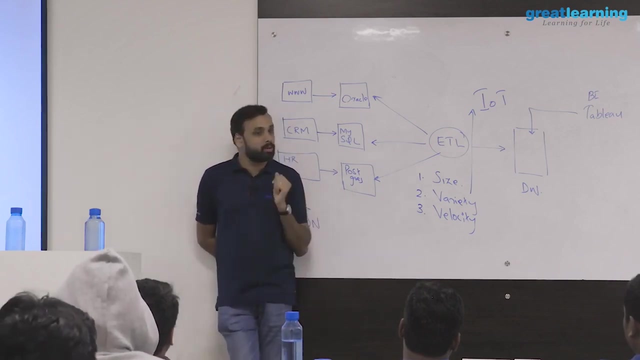 Now that is not the interesting part. Every minute, actually, millions of swipes are happening. So you need a system which can process, let's say, one million transactions in real time and then apply the logic and then say whether somebody should call the customer or not call the customer. 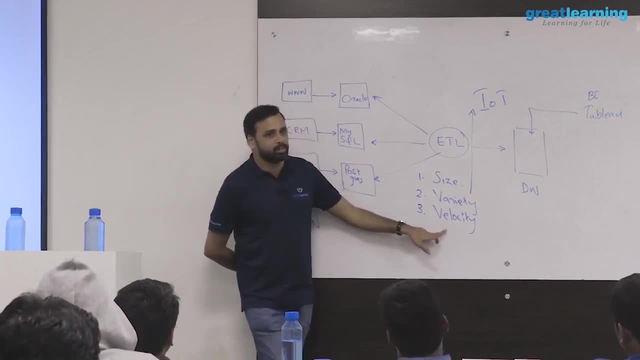 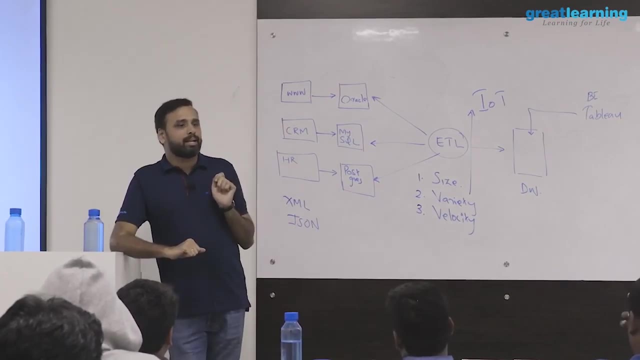 That is the velocity part. So this is a very interesting thing actually: real-time data analytics Again. second application is your sales. So one point is that, let's say, Flipkart is declaring a sale, So how it works in the backend is that they will decide they are giving off on mobile phones. 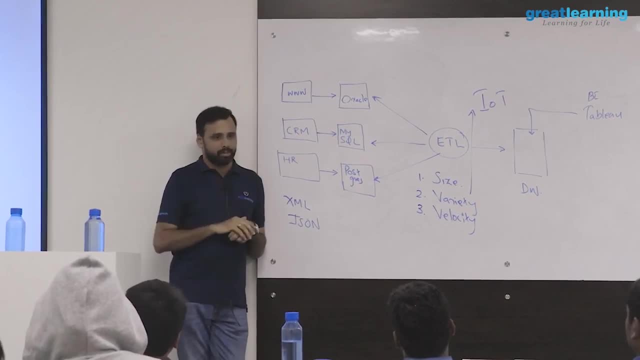 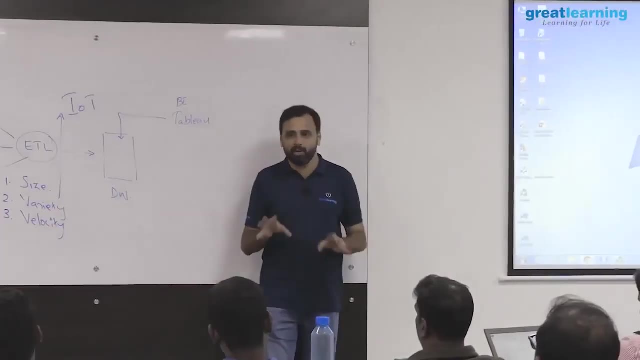 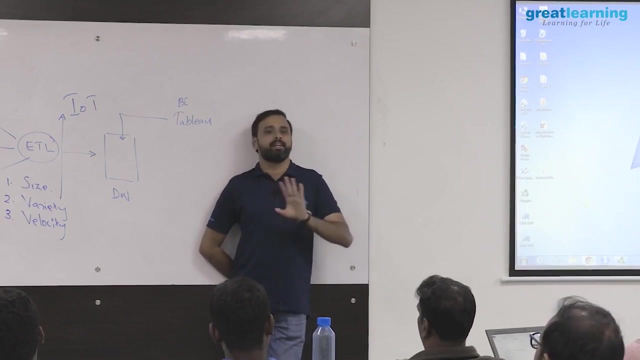 They will say: we will give you 30% off On mobile phones. But in reality Flipkart has no clue which phone people will buy. They will have some clue, but not a complete picture. So the ad will come saying that okay, today you log in, you will get a mobile with 30% off. 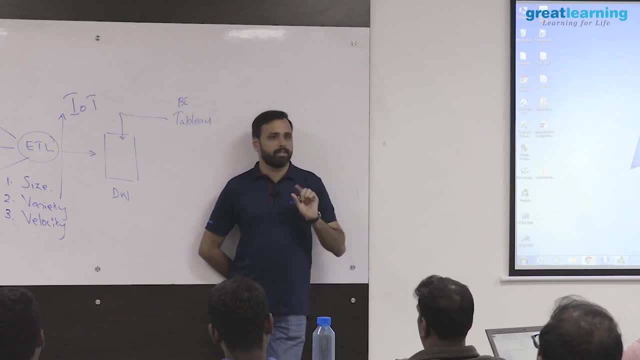 But which mobile? you don't know Some mobiles you will have fixed discount. That's a different thing. Then what they do on the actual sale day. when you log on to the Flipkart website, they start analyzing your data in real time. 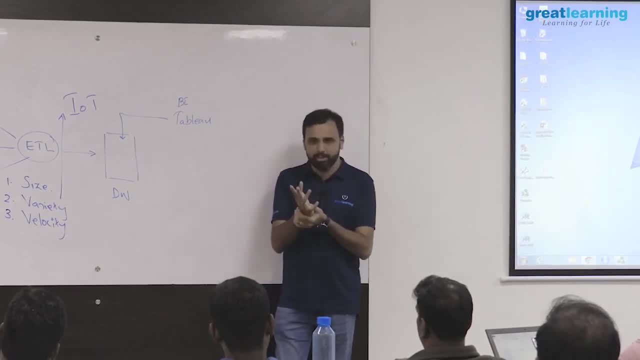 How many customers are searching for, let's say, iPhone. In that, how many are buying iPhone? So, if they figure out that total 100 customers are there, 80 of them are searching for some particular mobile, Let's say Xiaomi or any other mobile. 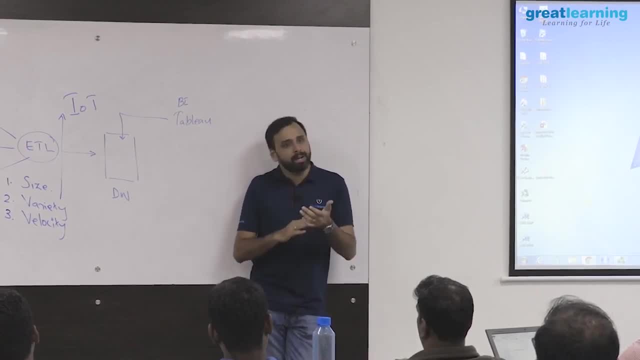 They know that they have to boost the sale of this product. So automatically you see the offers changing. After some time they will have more offers on this particular mobile. So that is a decision which has to be taken in real time. You can't analyze that data tomorrow and say that okay, I will change the sale. 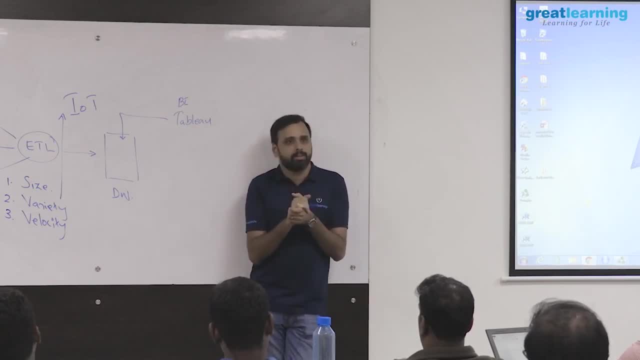 That does not work. So probably within minutes, or let's say within half an hour, you have to understand what the customers really want and adjust your sale- Again velocity. So real-time analytics is a very interesting field And we do a lot of sentiment analysis. 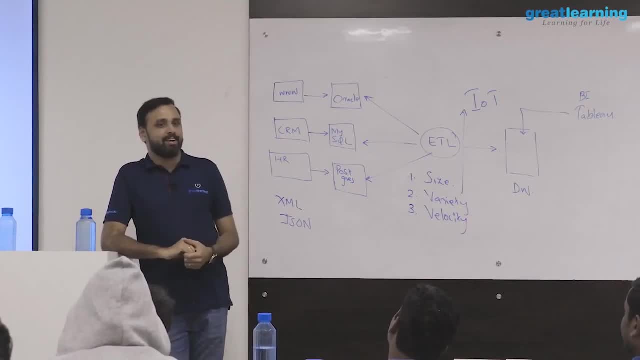 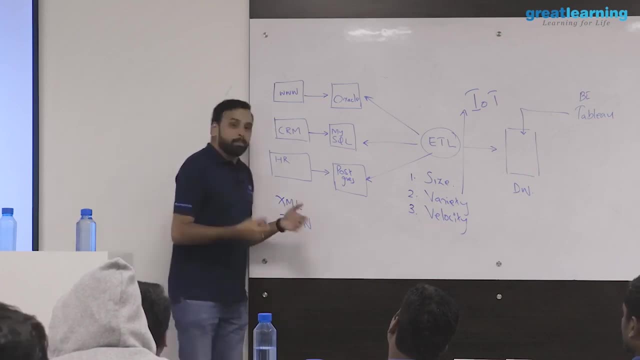 So how Pagzo of Hindustan and all are getting a very bad review is because of this. It is actually a bad review. I'm not saying that. What I'm saying is previously people were like they will release a movie and that's it. 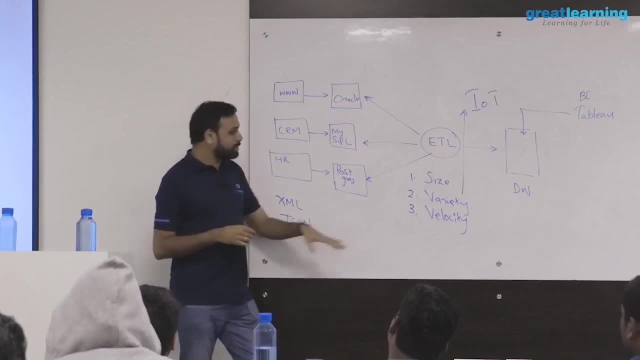 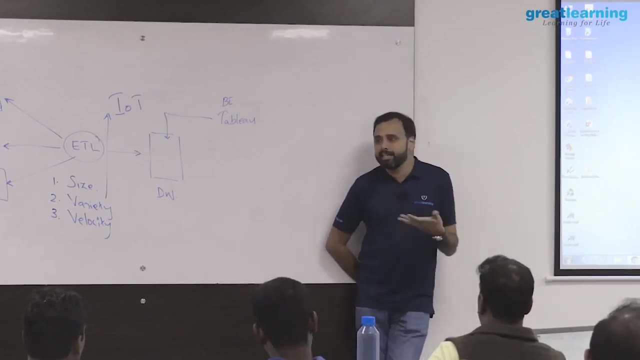 Maybe people will watch the movie or don't watch the movie. So now it is not like that. We do a lot of this thing called sentiment analysis. Like you, will start collecting social media data about how people feel about the movie. Are they posting positive reviews or negative reviews online? 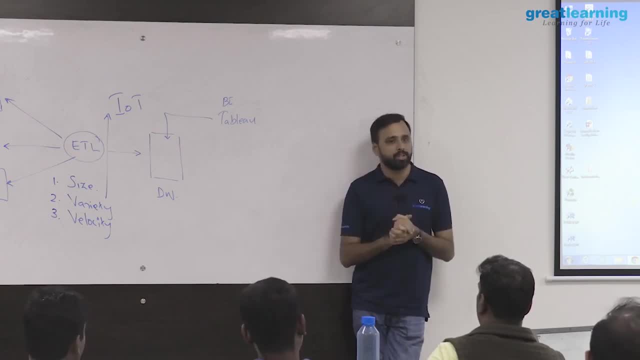 And then you will collect and understand in real time what is the position of the movie. So let's say the movie is getting a one-star rating, Then there is really nothing to do. But if the movie is getting a three-star rating, you can probably push some more advertisements. 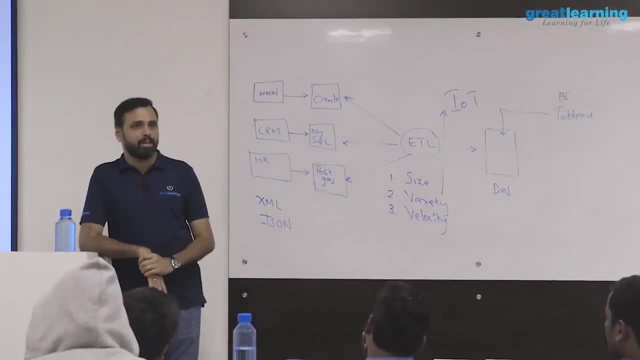 spend some more money. People may actually like it. We don't know- And sentiment analysis on when things like demonetization happened. It was very interesting, So we did some POCs at that point in time. Two years back, demonetization happened. 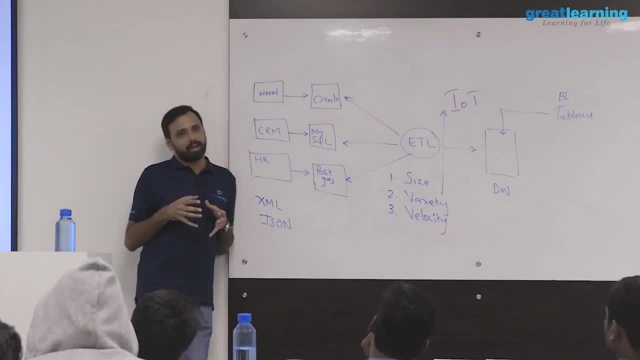 So people wanted to know how people felt about the movie. People wanted to know how India feels about demonetization. Some people supported it and some people opposed it. So one of the ways is that you can collect the data from social media and online blogs and all. 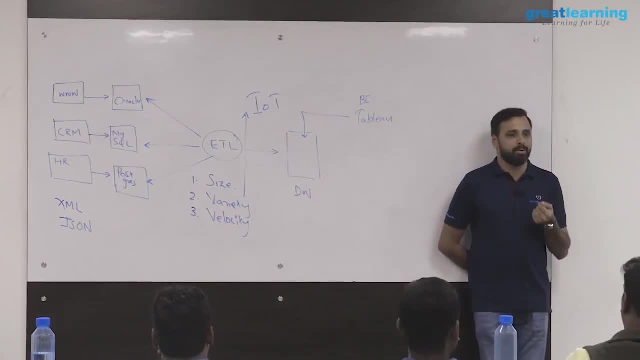 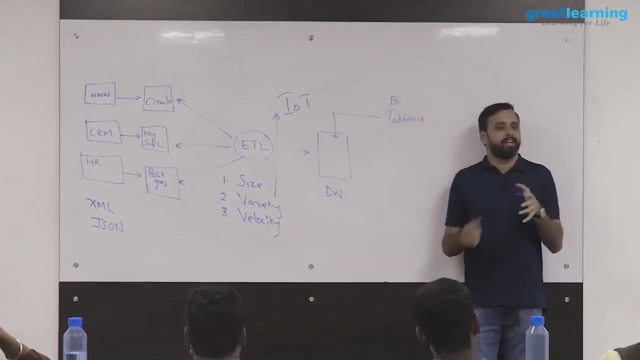 Then analyze it And then predict how people are feeling about a particular event. So all of that are related to velocity, Because you are not analyzing the data that was already there In real time. you are collecting the data And keep on analyzing the data. 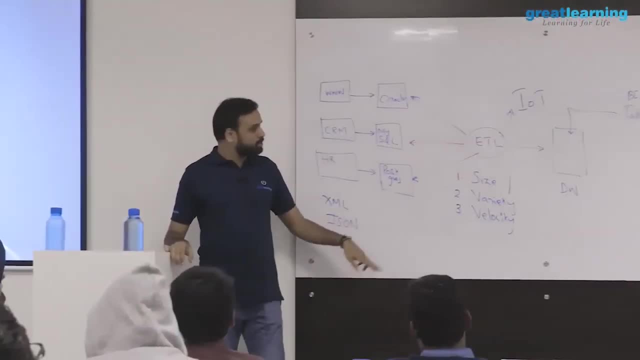 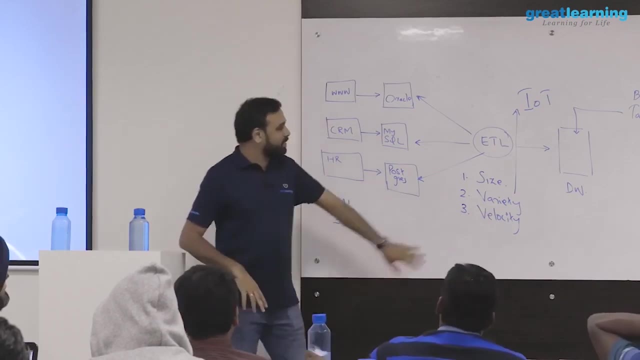 So there are systems which can do this, Velocity. I will tell you what can do this. But there is a factor. So typically, when somebody says big data, these three attributes are there. That's my point. So you have size, You have variety. 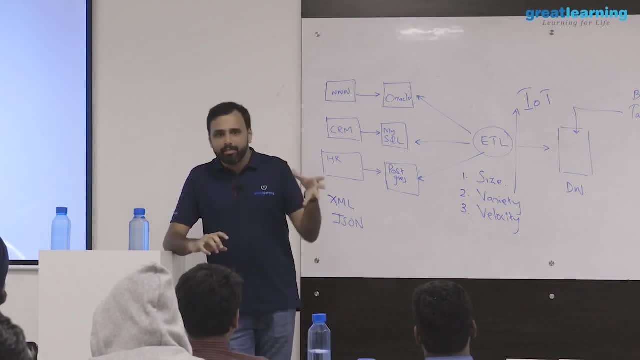 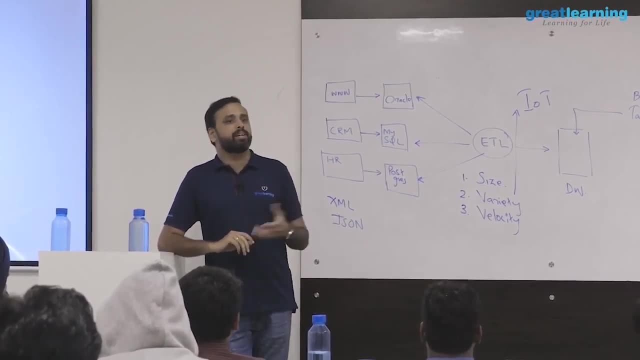 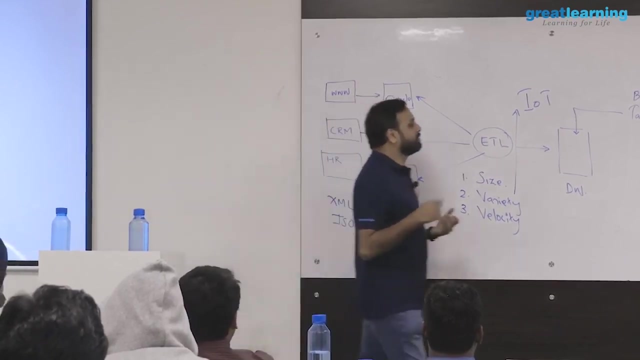 You also have something called velocity. So if all these three factors are there in any data analytics, you are doing So typically. we are talking about a big data scenario right Now. the question is that you are normally familiar with machine learning, and all right. 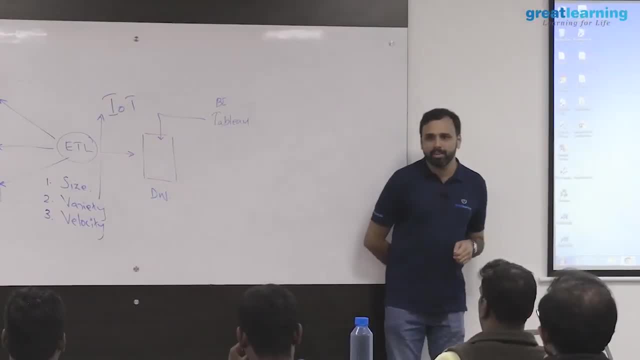 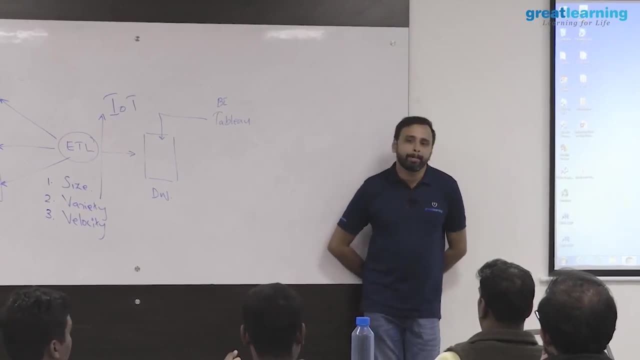 Because I think you are learning what machine learning. What did you cover in machine learning? Clustering, Shutter width Clustering, k-memes, Data mining and so on. Oh, data mining, k-memes, clustering, So to build a machine learning model. 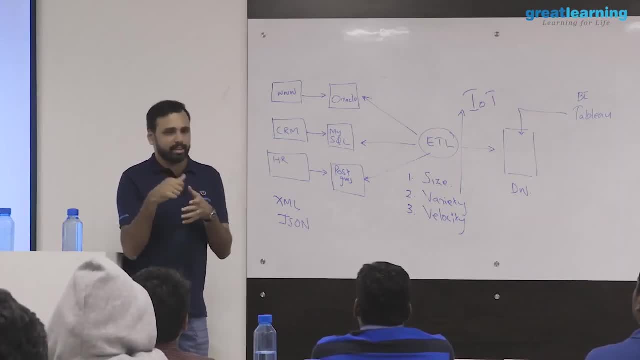 You need some data correct. First you need some data. Then you will use your exploratory data analytics, EDA, And then filter the data And that is how you, step by step, build your machine learning model. But the data you are feeding is very less. 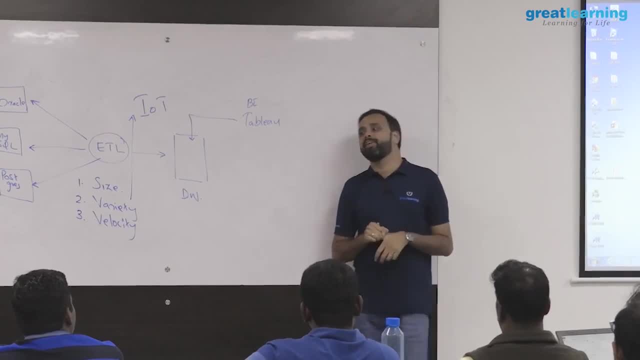 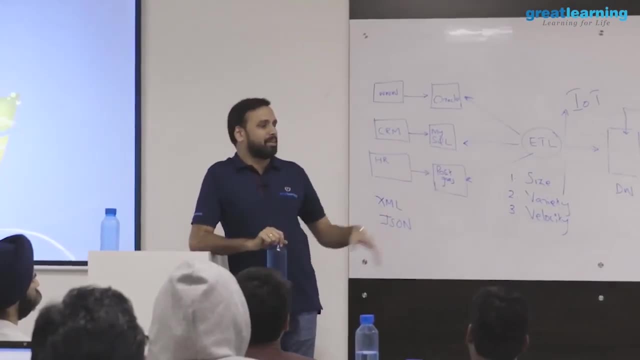 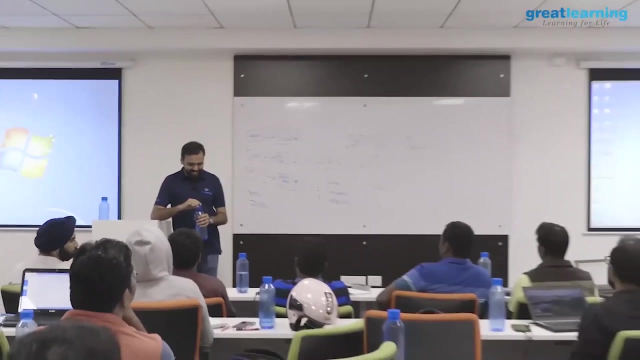 Normally when you are learning right. So let's say, I want to predict the property prices in Bangalore by 2020.. I want to know what will be the market rate. What technique will you use in machine learning? Let us see how many of you are really learning machine learning. 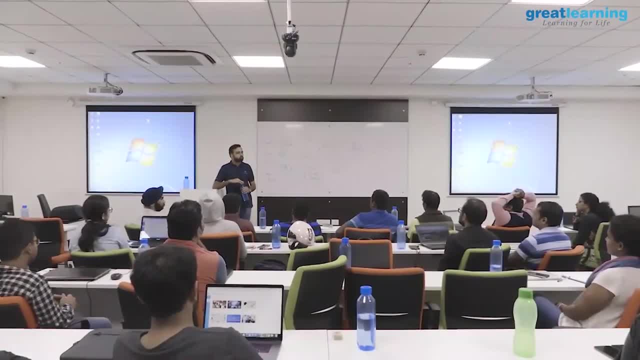 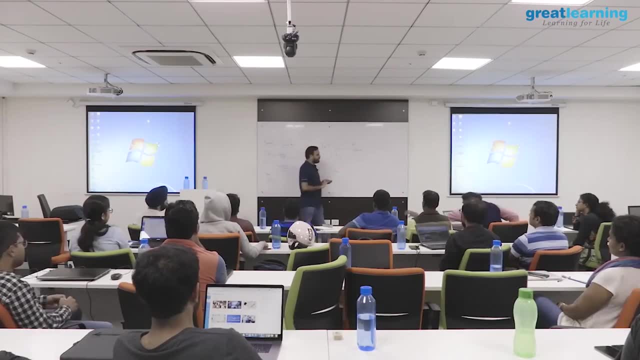 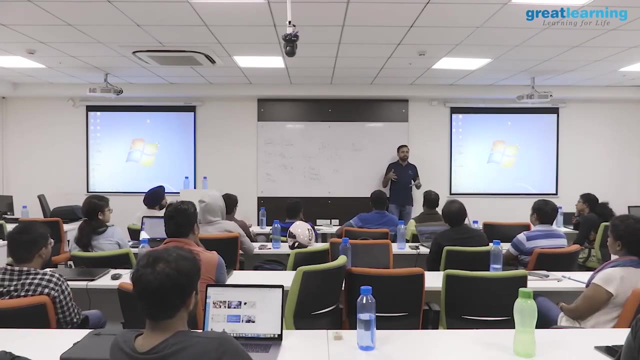 What technique will you use? Supervised regression, Yeah, so you can use many, but regression, right. So let us say regression. So to do regression you will use some data for sure. So probably the data is the Bangalore property prices, right? 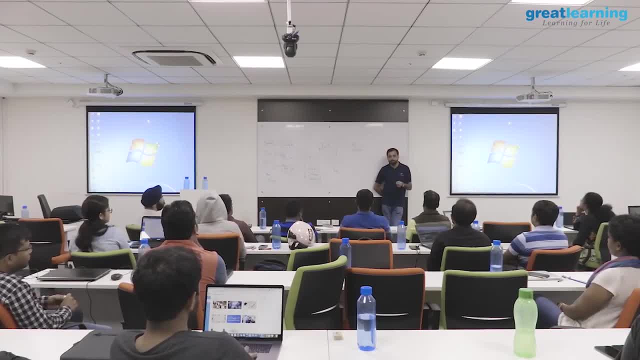 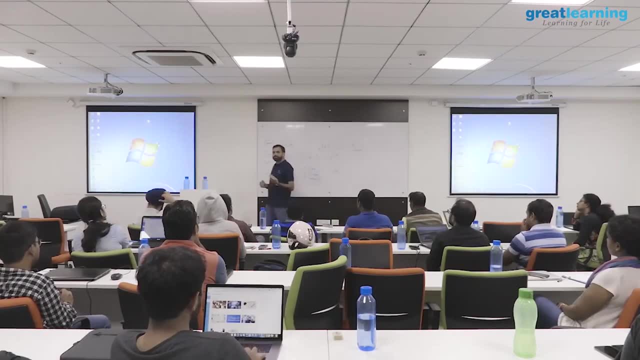 And maybe a lot of other things which can influence the property prices. right, That is how you make machine learning. That is how you make machine learning models, right? So normally what people do, or people were doing, they will use either their laptop or desktop or a server. 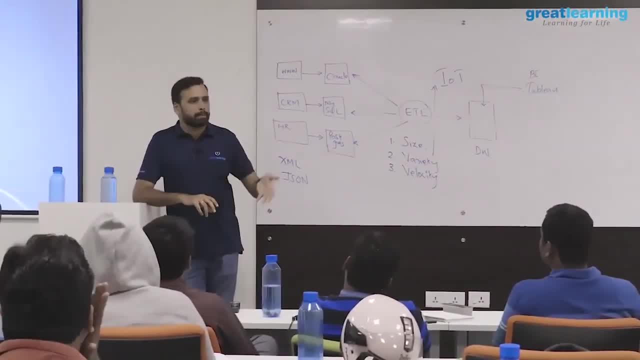 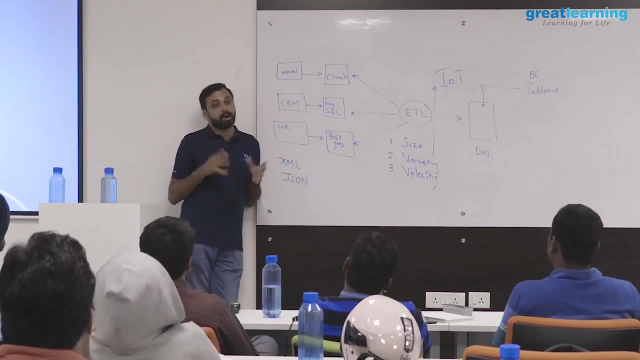 where they will build a machine learning model and then apply this and predict it. But imagine if you can train your machine learning model with, let's say, 1000 terabyte of data. That will be so powerful Because it is learning from 1000 terabyte worth data. 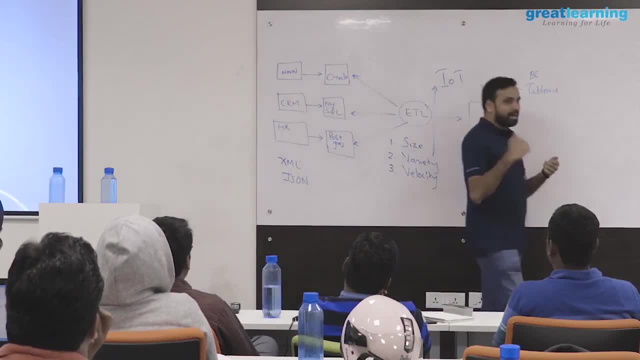 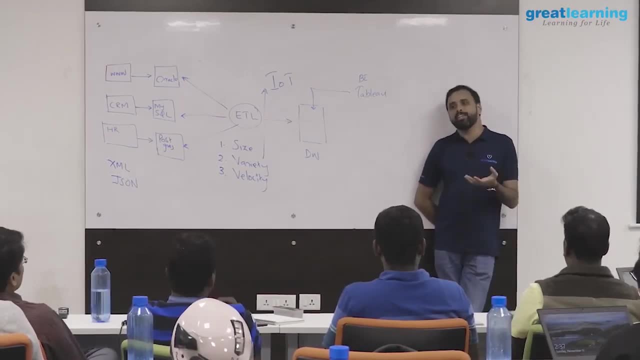 So if you want to do something like that, that is where you can blend machine learning with big data. So all that you are learning right now, for example, R right R. normally, when you create your model, you are creating on your laptop, right? 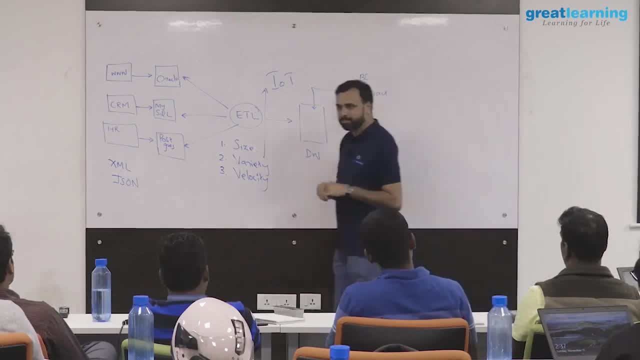 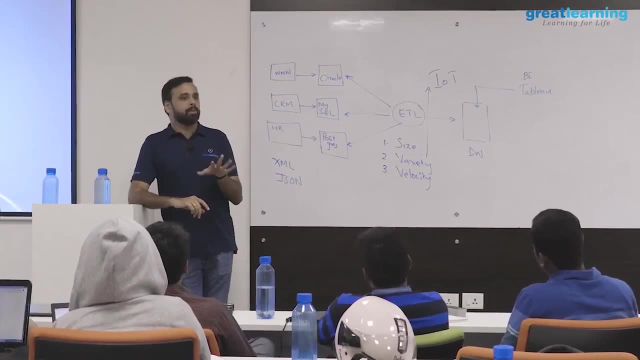 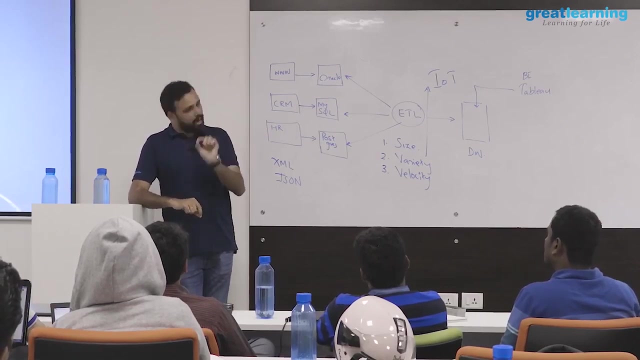 But you can also run this in a cluster. When I say cluster, group of computers, right, Not one computer. So one framework which is very popular for this is Spark, of course. So Spark has a module called Spark R. If you use Spark R, the advantage is that you will be writing same R things, no difference. 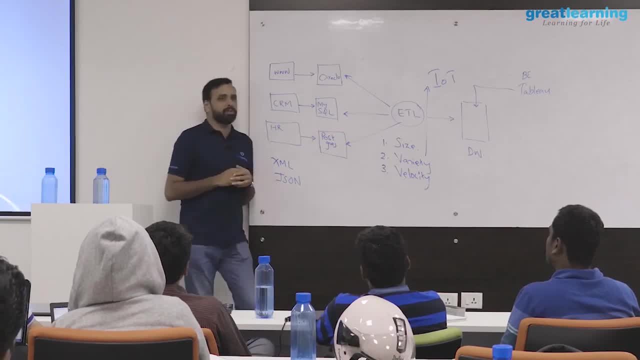 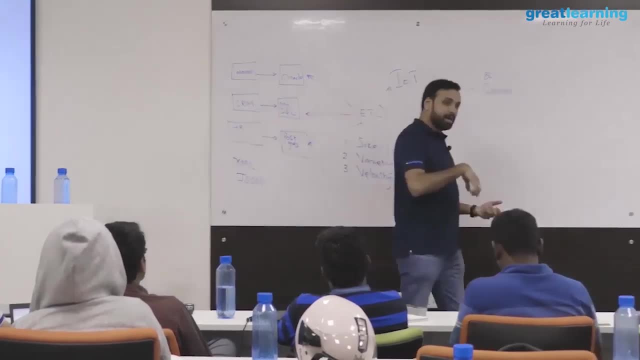 But rather than you build your model on your laptop, you will be building your model in a cluster of thousands of servers. So imagine creating a machine learning model which will learn from, let's say, 10,000 terabyte of data. That will be so powerful and so accurate, right? 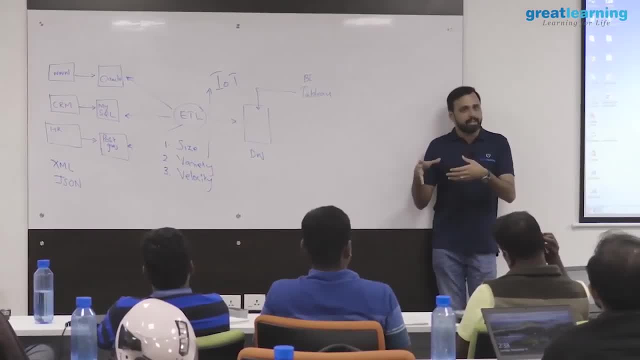 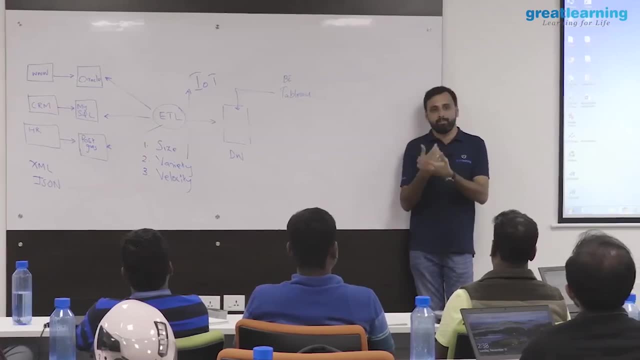 So I am not saying that everybody does that Right, But if you have a situation where you need to feed a lot of data, then you can actually blend big data with machine learning, Right? So they are not. machine learning and big data are not like two different concepts. 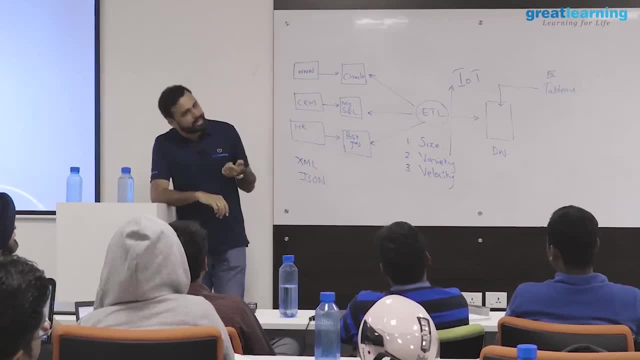 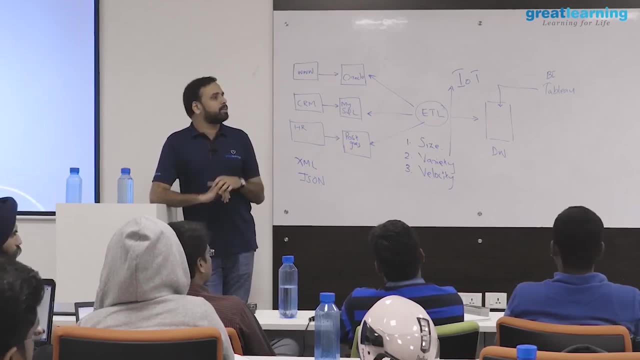 So machine learning requires data And that data. if that data is huge, then you can use big data technologies to solve your problem. So I think we were doing that in one of the batches, not the BA-BI course. In another course we are actually doing that. 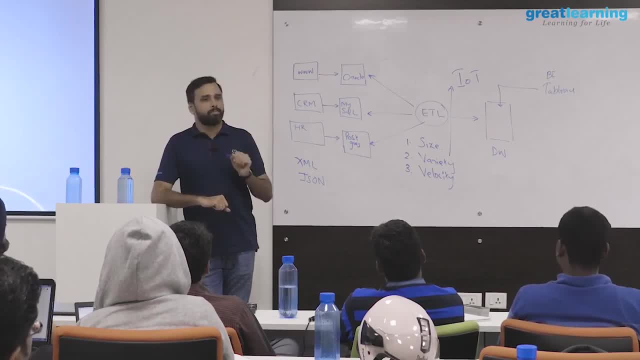 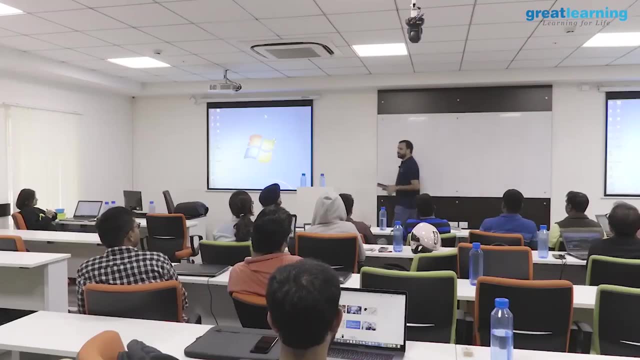 We teach ML and AI And we also use a bit of big data to clean the data and understand the data, etc. Right, Correct, I understood the point. So the question is like if you are doing velocity, then infrastructure cost has to be very high. 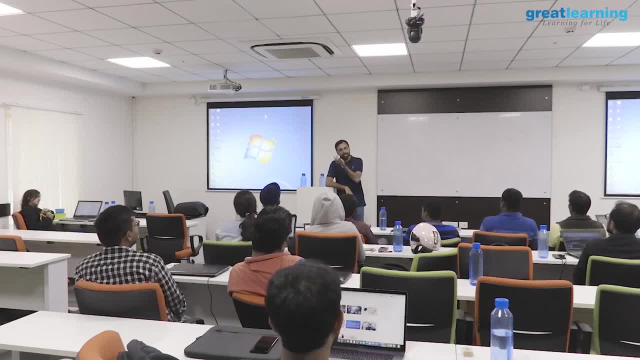 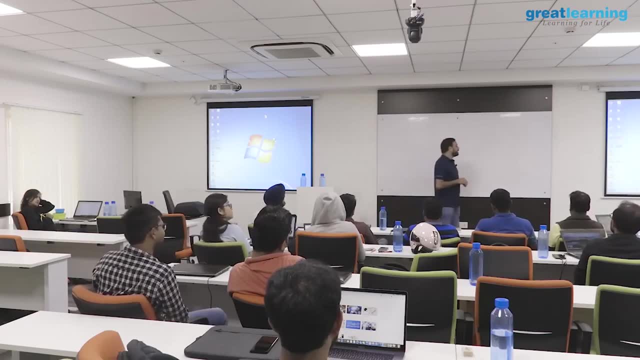 So there are multiple ways to answer that. I will answer that So yeah, so not even velocity, Even if you remove velocity from the equation. even if you simply want to store big data, it has to be costly. Infrastructure cost has to be very high. 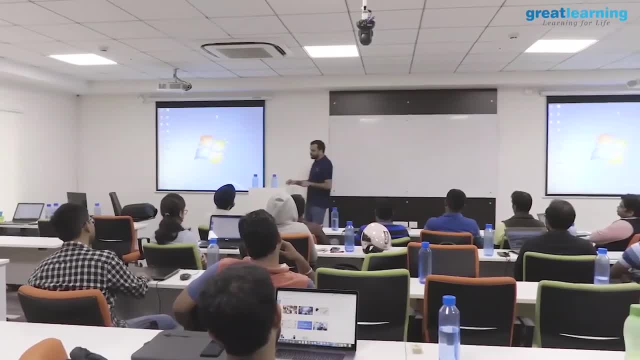 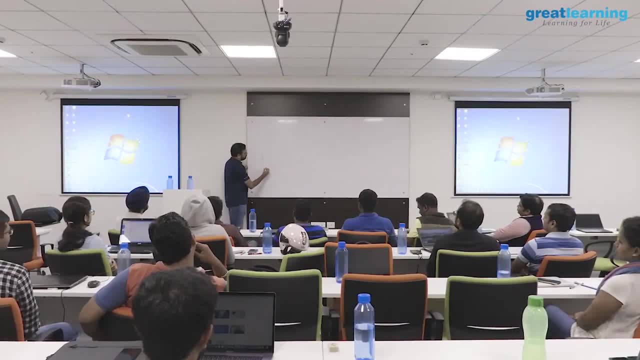 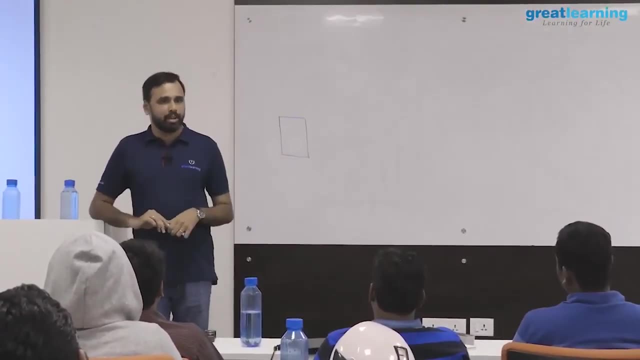 So the question is: if I want to store huge amount of data, what should I do? So if I take a machine right, This is a server, Normal server. No rocket science, no hi-fi stuff- Normal server. This will contain something called a hard disk. 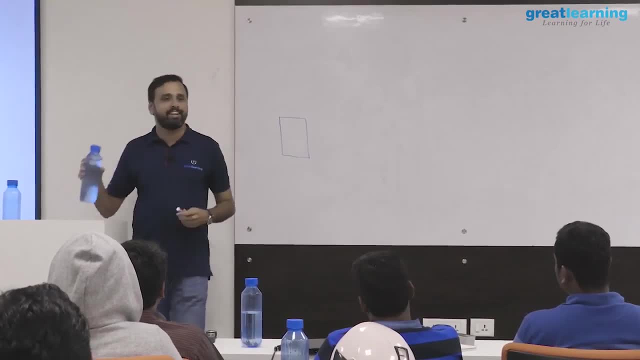 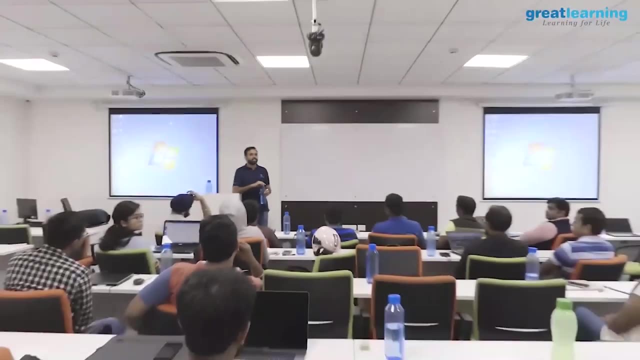 You know that? And what is the maximum capacity of a hard disk in a server? What do you think? 5TB, I don't know, I am just asking. 10TB is the limit, 10. So 10 is the limit. 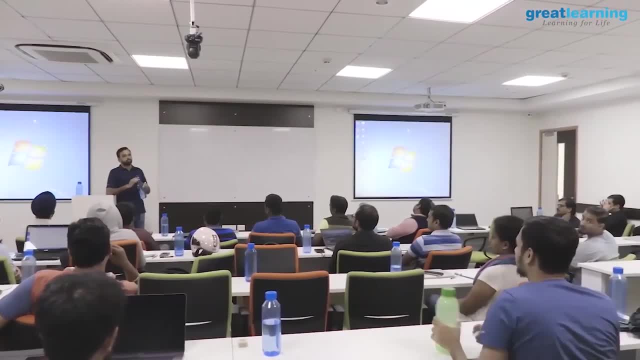 Physical number. 10TB is the limit You can't get 20.. 1TB is 10TB, So you can make a rate. You can make a rate, So a rate 10.. Okay, 80 hard disk. 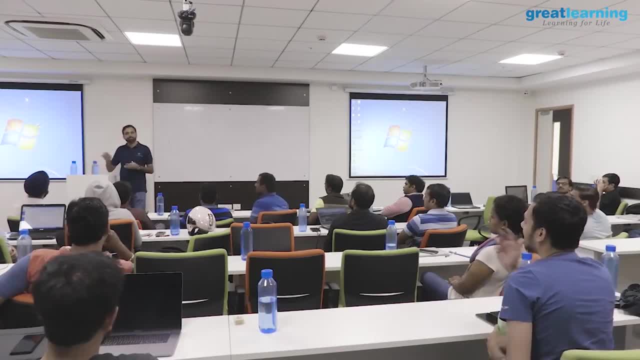 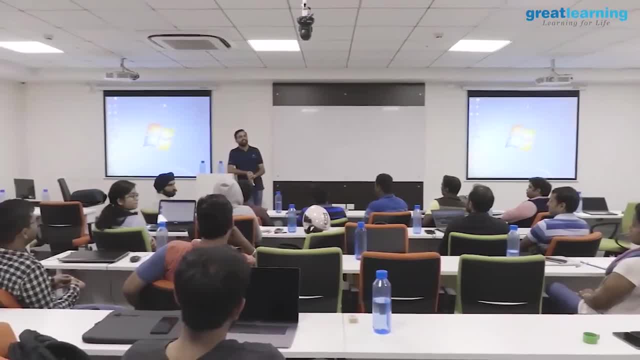 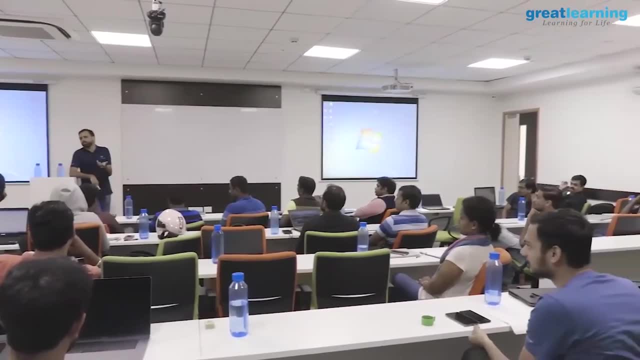 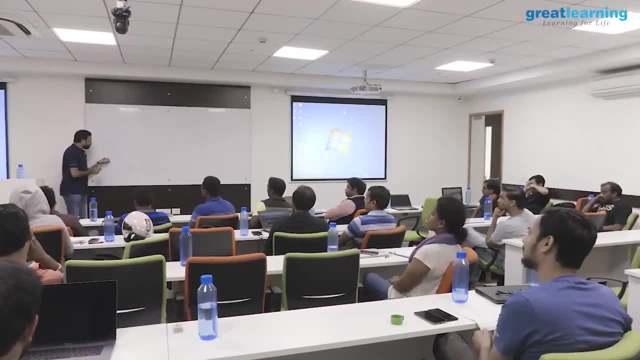 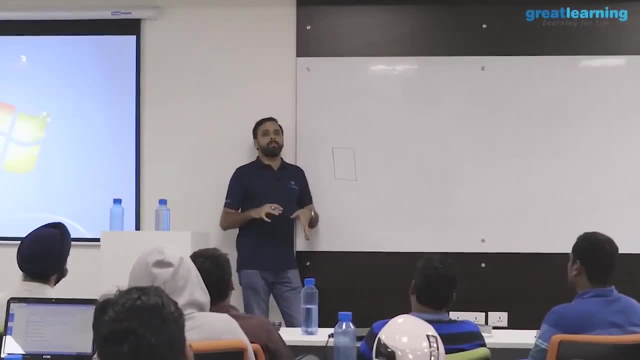 So the The point is, if I take one machine, there is no way I can dump all my data. So this is gone. I am not going to use one machine, And some people argue that. so in every, not this batch, okay. 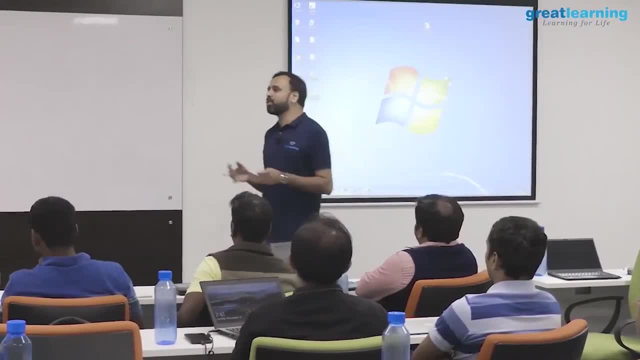 So typically when I take big data. so one of the cool feature about big data is that anybody can learn big data. There is no prerequisite. So typically when I take big data, I can learn big data. So people will be from different, different background, right. 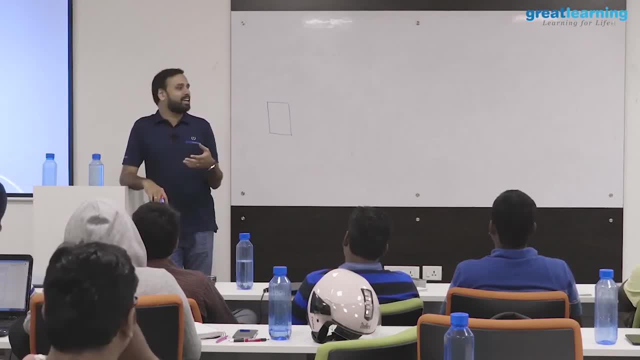 So one of the things: that in every big data batch there will be somebody from storage background, Like some guy who has ruined his career with storage. you know He worked in all the data centers. you know in and out of data center. 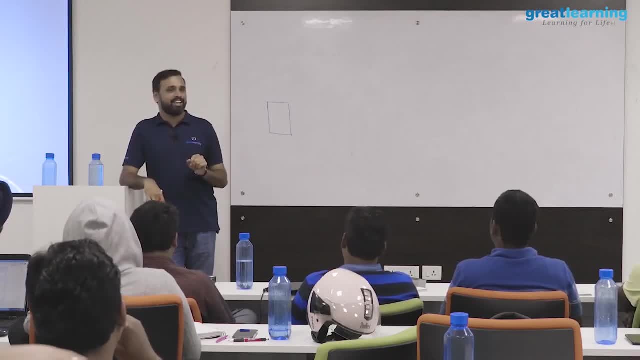 So he will always argue saying that storage is never a problem. Okay, You bring your NAS SAN, So he start drawing stuff. Okay, So there is NAS and SAN. Well, I am not against storage. Even I have worked with EMC. 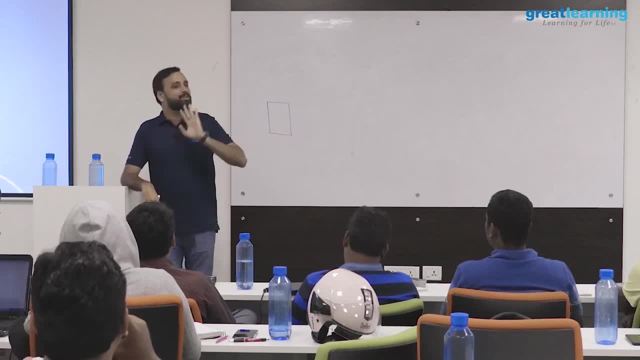 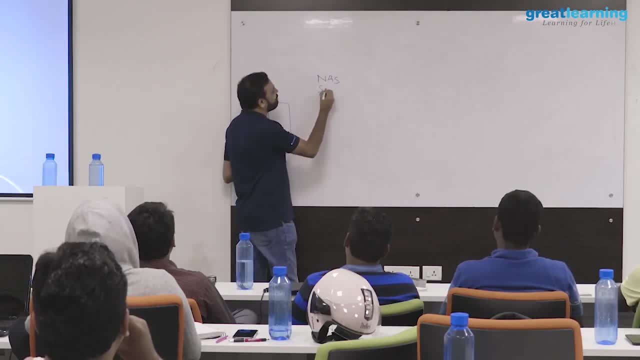 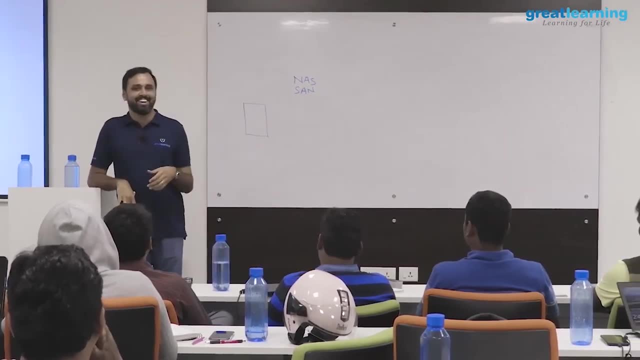 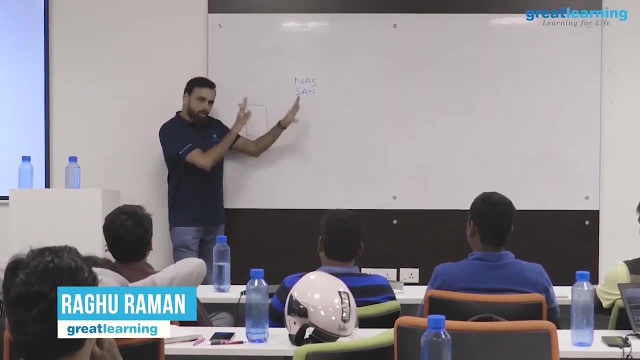 I am just kidding, So don't get offended. if you are a storage guy, Okay, I am just kidding. So yeah, I agree, There is something called network, attached storage and storage area network, which are like storage boxes where you can store any amount of data. 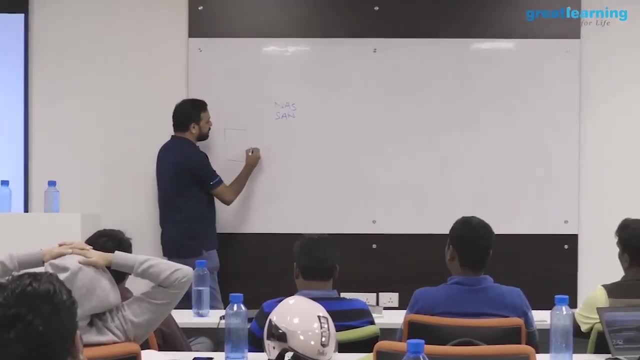 But that will not solve my problem, because I can connect the server with the SAN- let's say a storage area network- and in the SAN I can probably store any amount of data. And that will not solve my problem, because I can connect the server with a SAN. and let's: 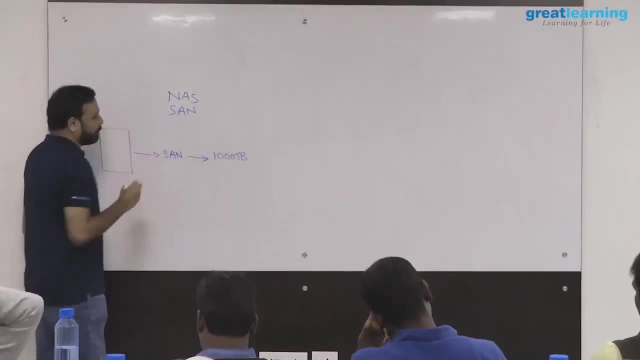 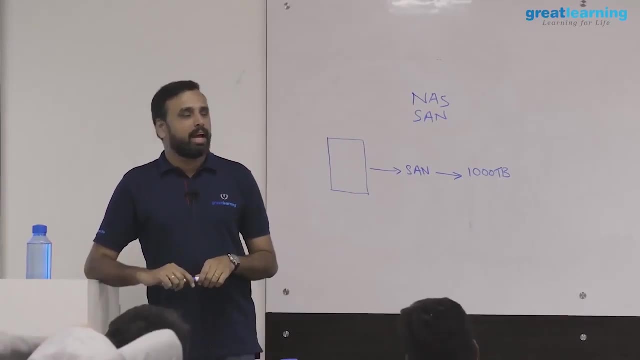 probably store 1000 terabyte, no doubt. But I can only store, I cannot process. SAM can be used for a variety of other purposes, actually to store the data right, And NAS also. I mean NAS also does not work, So this part is gone. So the question is that what? 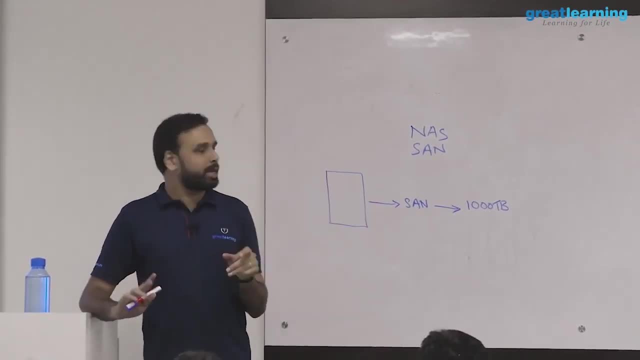 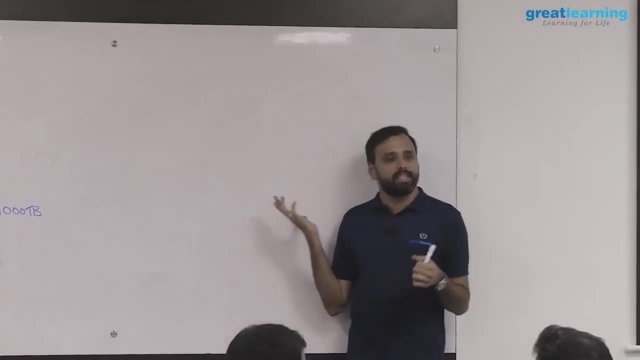 people were actually doing when they had data right. So I showed you the traditional architecture where the data warehouse was there, right. The data warehouse is nice, but the only problem it is costly right. So data warehousing is actually a very nice concept You can store. 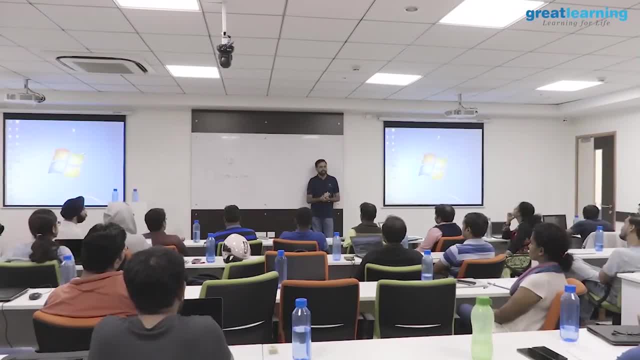 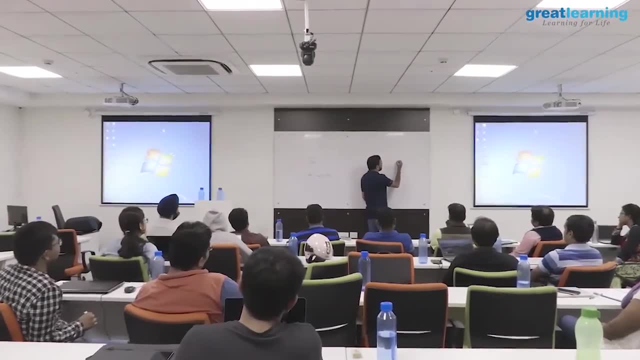 a good amount of data, even 1000 terabyte, more than that you can store. But the only problem: it is very costly. So we have vendors like Teradata. So there is a vendor called Teradata, Greenplum, Netizar. there are many vendors actually. 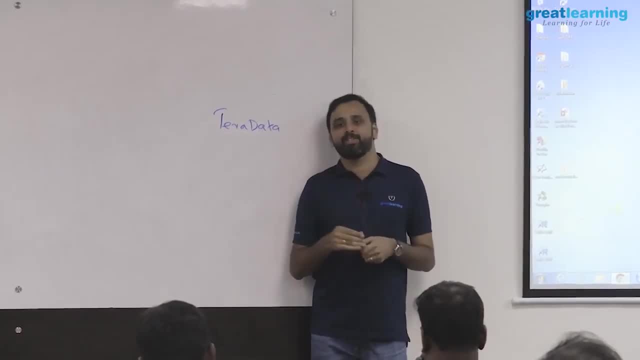 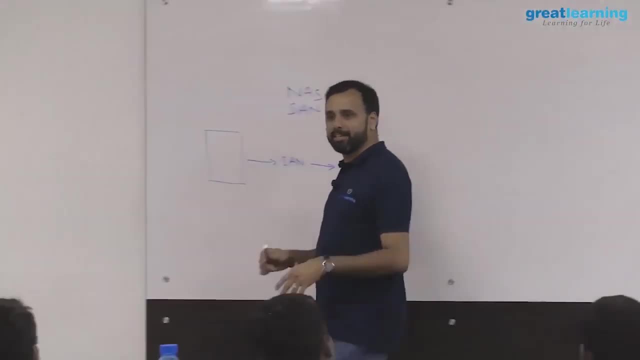 But I cannot pay you, So that is a requirement. So they will come back to us and say, sir, we have an excellent solution, this will work for you. What is the solution? You store 500 terabyte rest. you archive. They will give, they will sell an archival. 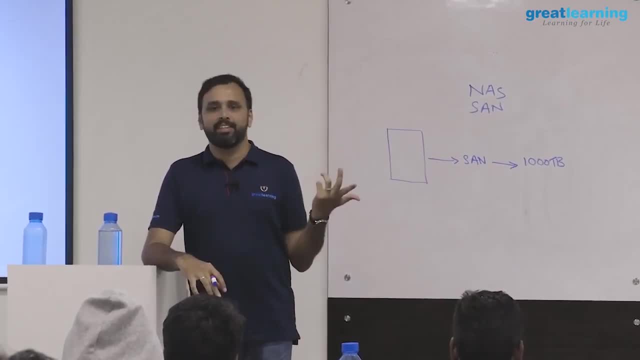 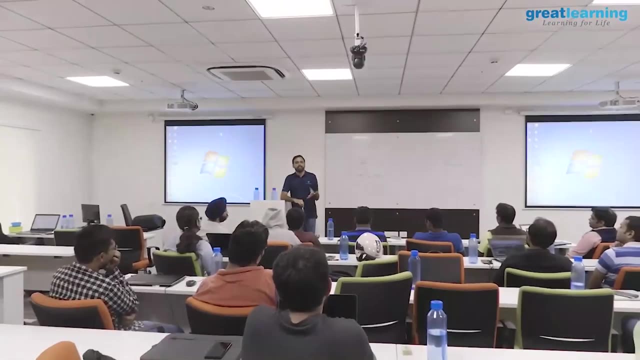 solution along with that. What is the problem? If you archive your data, then what? You cannot use it. You cannot get it for real-time analytics right, Exactly. So that is what people are actually doing, So they will archive majority of the 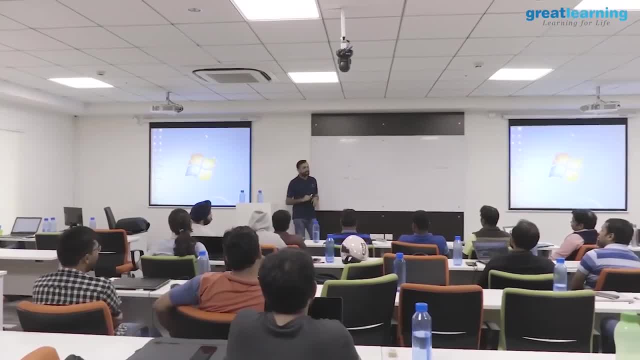 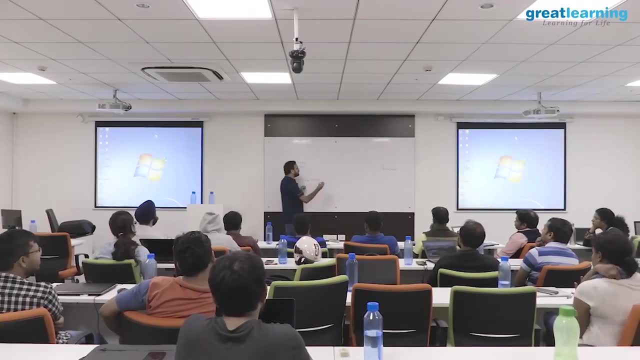 data, remaining data- you analyze. whatever you get, you analyze right. So now, when it comes to the big data technologies, what we usually do is that in the big data technologies, instead of taking one machine, we take a group of machines. So I will just 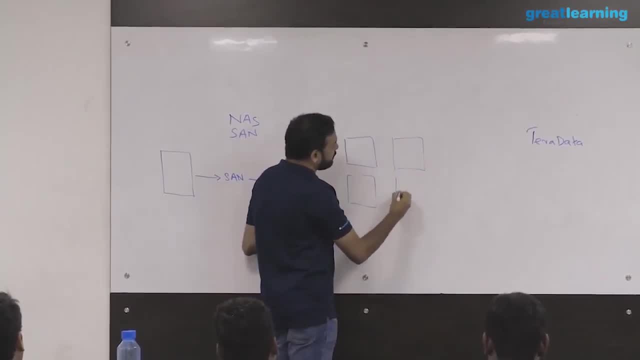 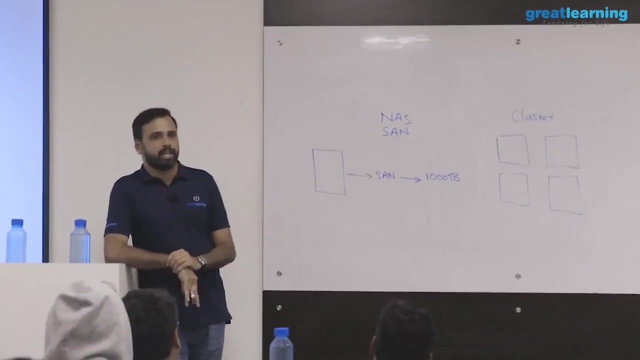 draw four machines. that is not the number, But we take a group of machines and we create something called a cluster. A cluster is nothing but a group of machines, to put it very simply, And let us say we are taking four machines as an example. So I take four machines and 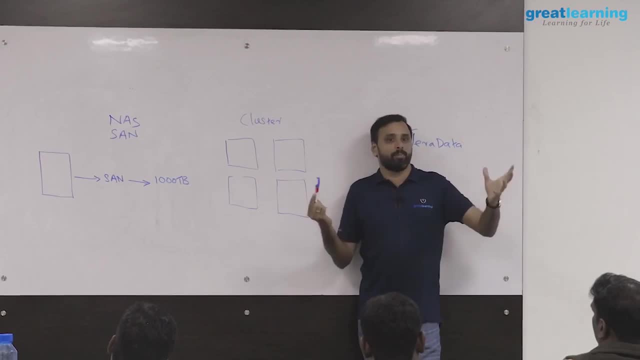 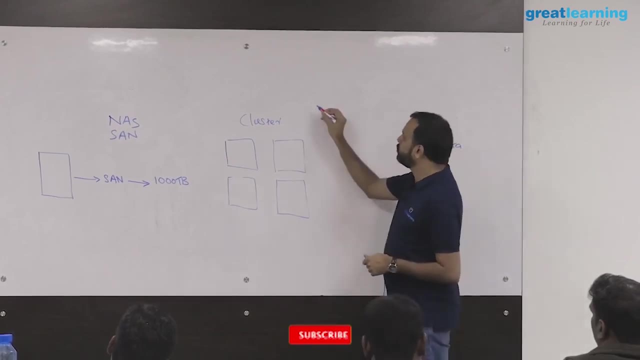 then I form a cluster. So the question may be that how do you form a cluster? Will it come out of thin air? No, You have to use a framework. So that is where this thing called Hadoop and all are very popular. So there is something called Hadoop. Hadoop is 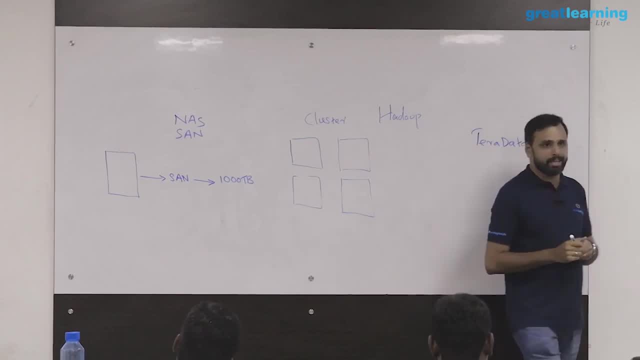 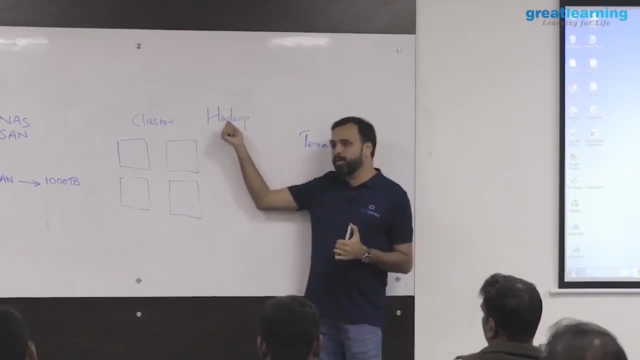 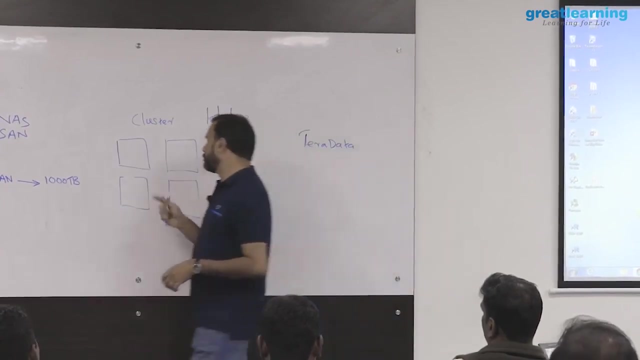 probably the most used big data framework in the world. as of now, Hadoop is a platform. So if you are using Hadoop, what you can do? you can say: take four machines, install Hadoop in all of them. you have a ways to do it Once you install Hadoop in all of them. 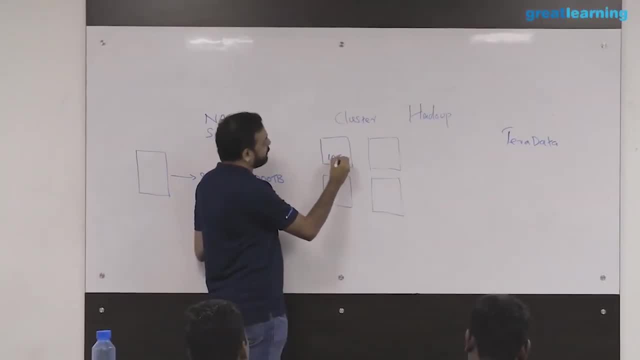 what Hadoop can do is that, let us say each machine is having 10 terabyte of hard disk, it can project a total storage of, let us say, 40 terabyte, combining all these four machines- hard disk. Not only that, it can start from here. you can start with four machines and 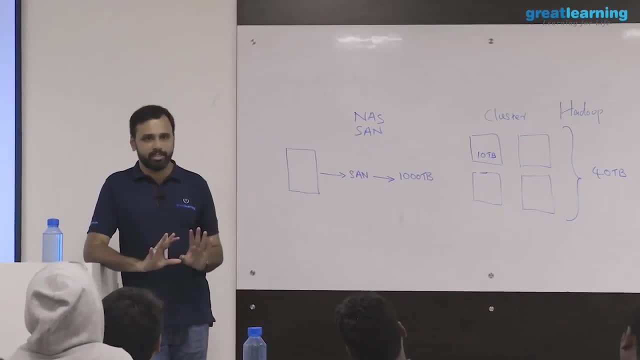 you can expand to 40 or 400 or even 4000 machines Without disturbing the cluster, So you are never going to run out of space. So the more data you have, you keep adding more machines, And I am talking about a very typical setup. 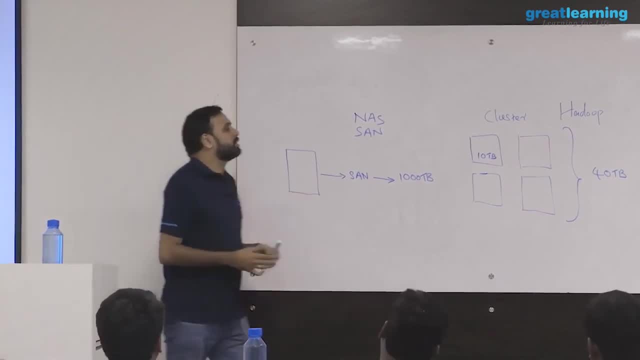 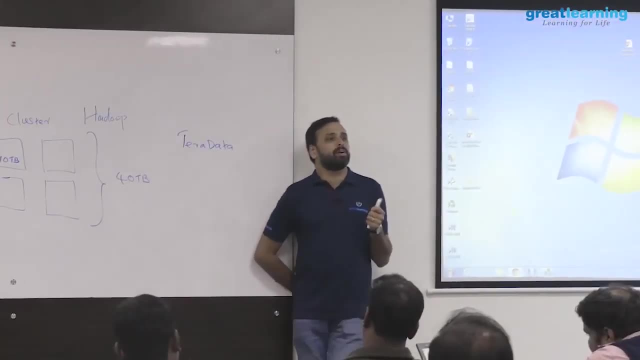 So normal Hadoop clusters are anywhere between 50, 2000, 2000 nodes. For example, there is a company called 24 bar 7 nearby in Bangalore. They are a call center BPO company. They do a lot of analytics, 24 bar 7.. They have a Hadoop cluster. they run 60 nodes in the 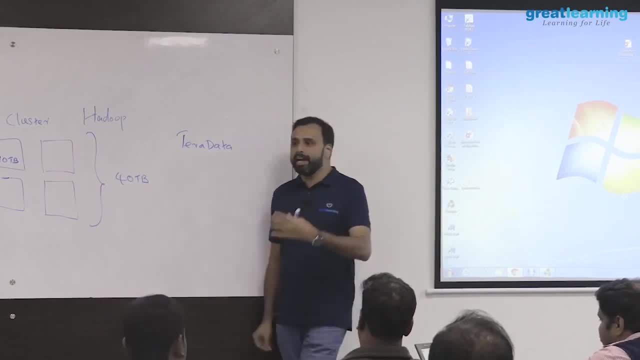 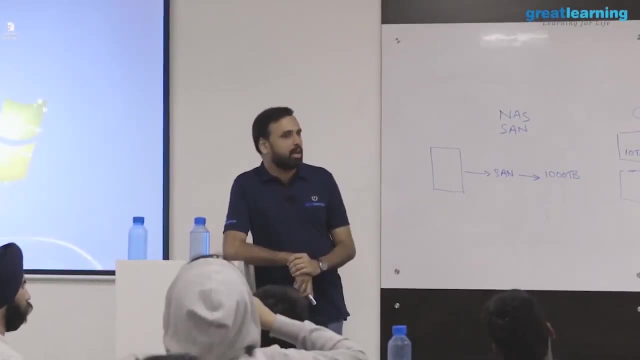 Hadoop cluster. that is their setup. On the other hand, Bank of America has a Hadoop cluster that is 2000 machines, because Bank of America is bigger, of course, and they have huge amount of data. So now you may ask building this setup to. 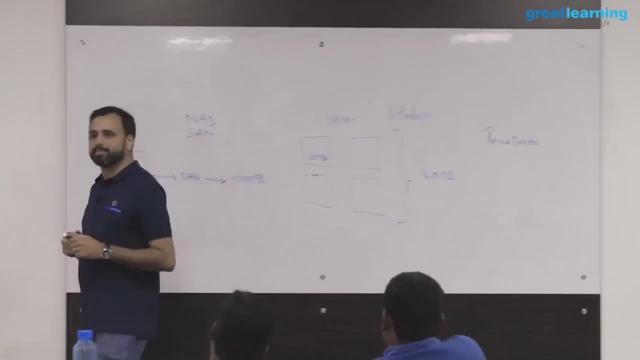 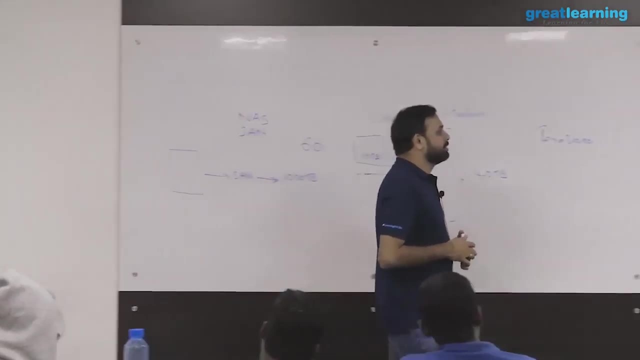 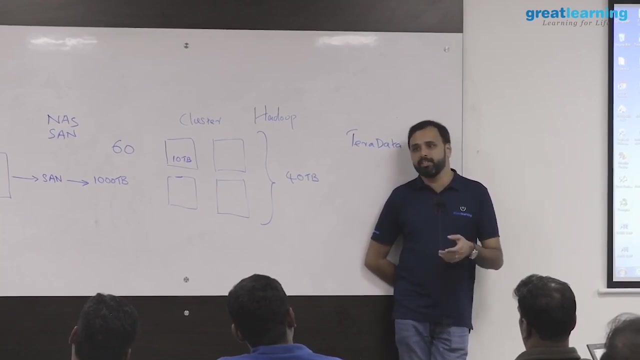 store my data. still, I have a cost problem. So if I am building a 60 node Hadoop cluster, imagine, are you really investing money for 60 nodes? Yes, In that case, how? this is cheaper. because you have to buy 60 machines, you have to connect them, electricity and everything. 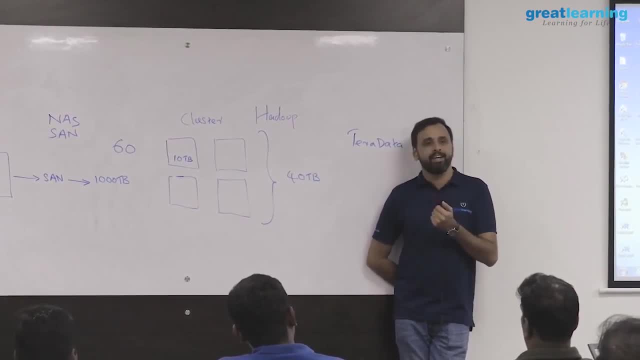 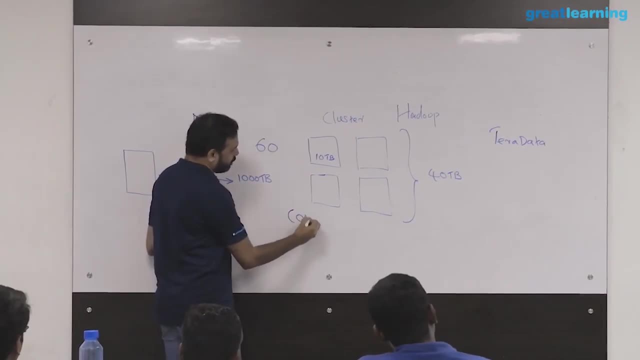 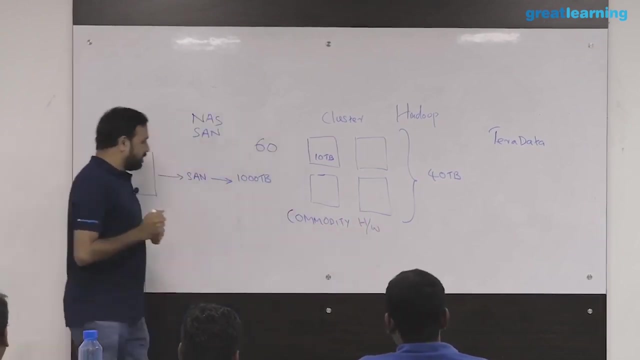 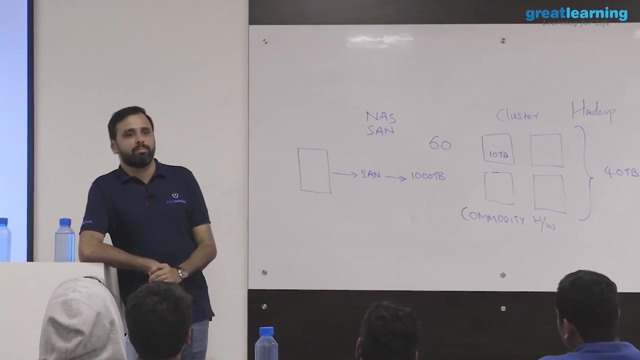 So that is not really a cost effective way to do. It is cost effective because all these machines I am using, they are commodity hardware. There is something called commodity hardware. Commodity hardware means cheap machines or assembled machines or second hand machines. 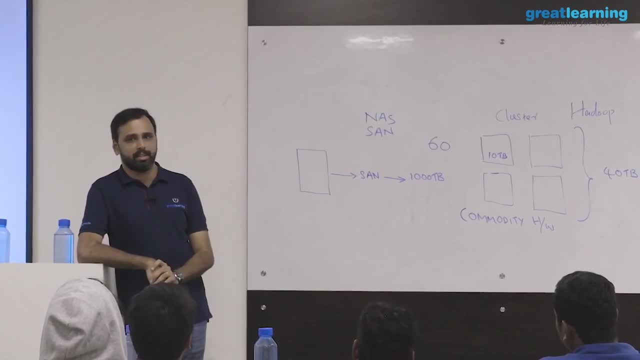 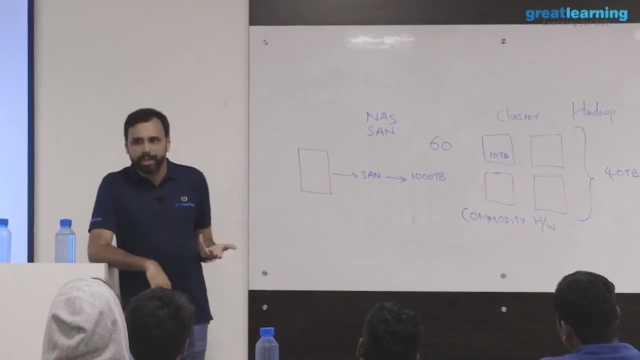 You are not building enterprise grade systems. So point number one: you are not going to invest a lot of money for hardware. So the philosophy of Hadoop says that if you are building a Hadoop cluster, find the cheapest machines possible and build it. That means 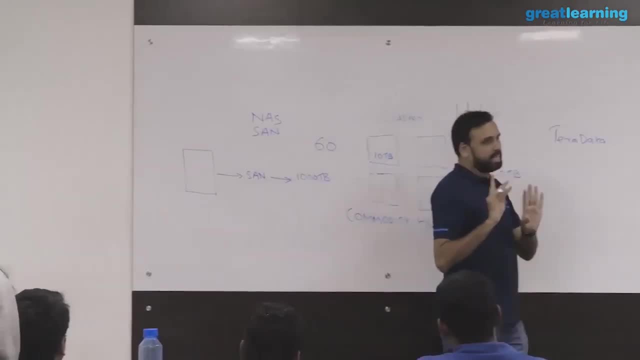 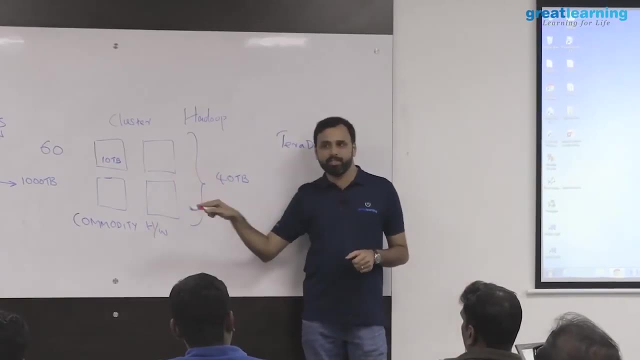 these machines are not really reliable. They can crash, they can go down at any point in time because they are not really reliable, And there is a way- Hadoop will take care of it. So that is a different question. But you are not really going to invest a lot of. 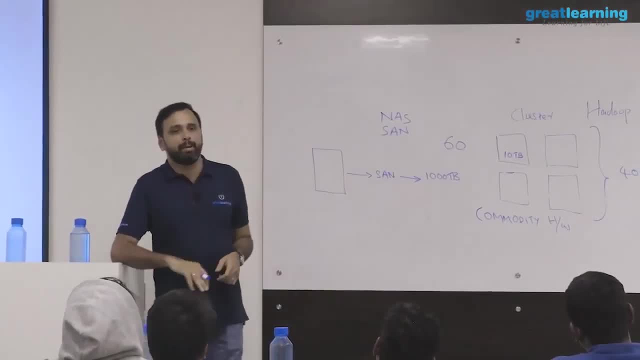 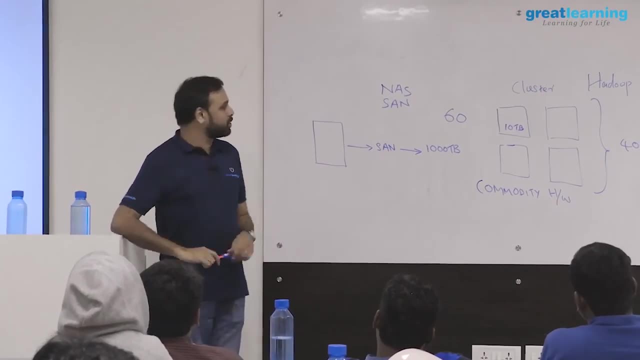 money into buying hardware. You are not going to buy like 60 IBM blade servers to build a Hadoop cluster. Then you will practically run out of money. end of this thing. So the machines are commodity. Now I should also tell you what is happening in the industry. 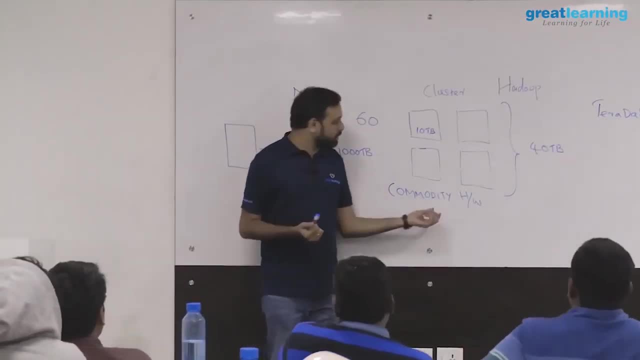 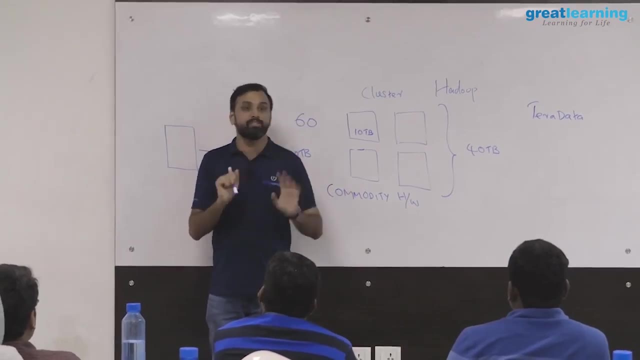 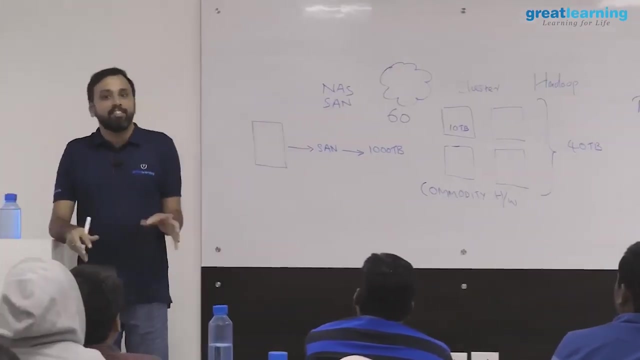 So what is happening in the industry? So this is probably the theory which I was teaching like 10 years back. Even now it is valid, But now there is a huge difference. This is the difference: Cloud Everything is on cloud Everything. I mean, I am not kidding, It is. 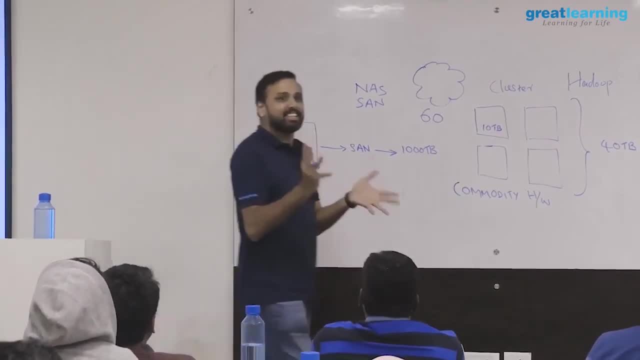 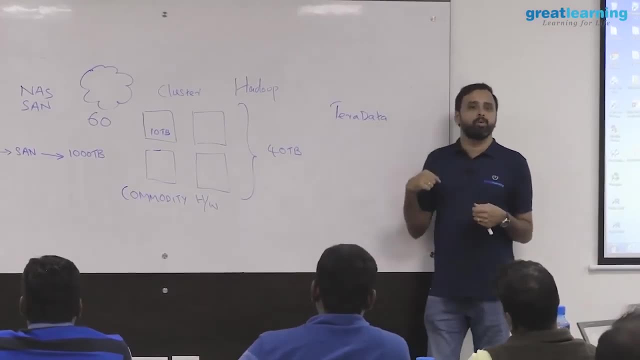 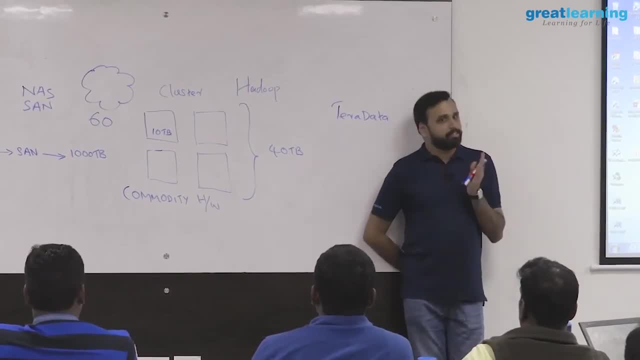 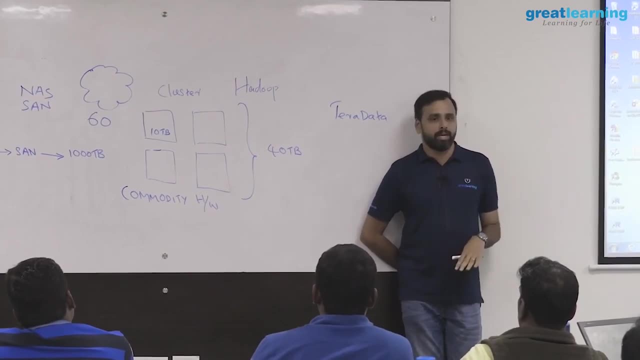 On-premise clusters are very rare. In fact, I have seen very so. I also work with this company called GE General Electric. Their entire platform is on cloud, including their financial data- lake finance data. So previously people had these concerns like: if I want. 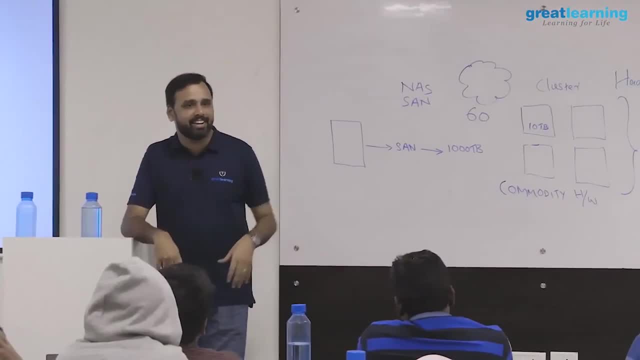 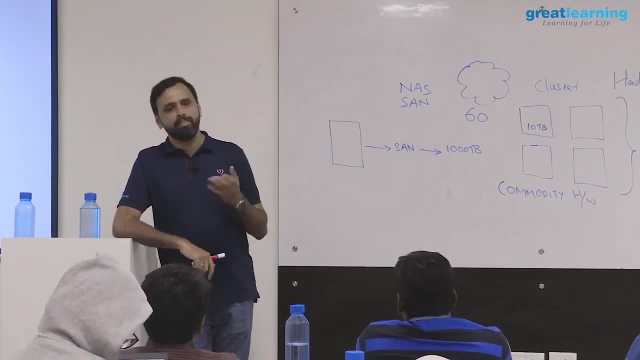 to go to cloud. what will happen to my data? Some hacker will hack in. Those are all concerns. It does not matter. It is over 10 years back. you can ask that question. Everything is on cloud now. I mean different vendors will have their different perspectives. Some people 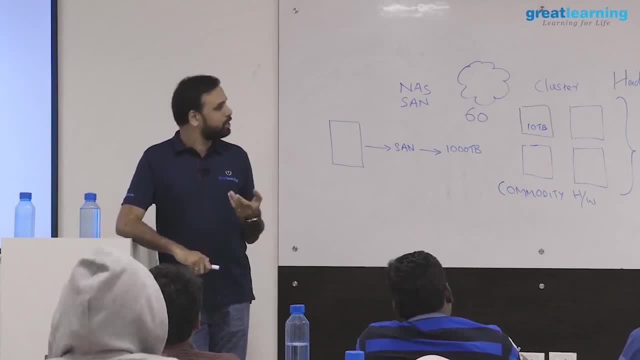 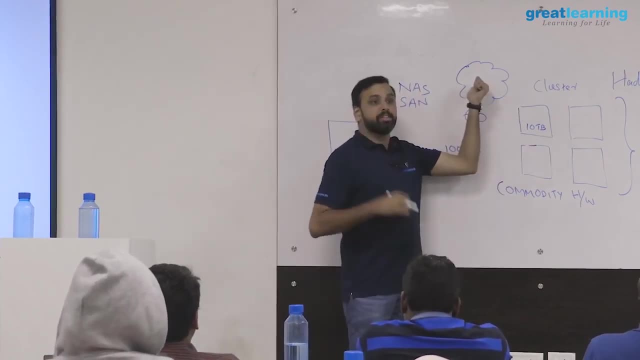 will still say that due to security reasons, I do not want to go, But majority of the people have migrated, So most of these clusters are now in the cloud, which means, again, it is cheaper. You know how cloud works, right. 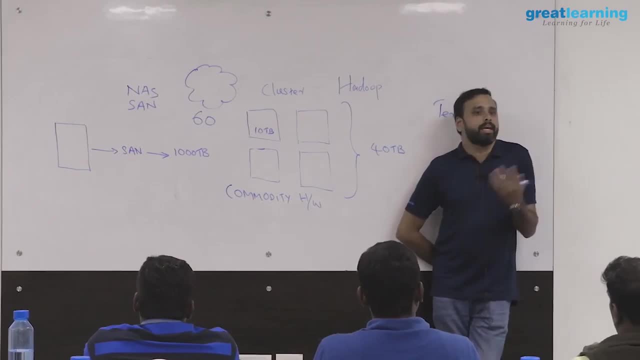 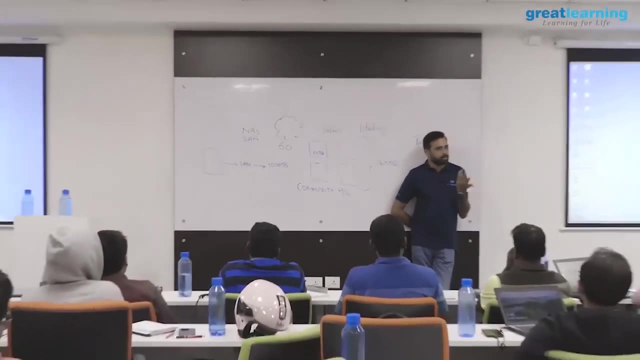 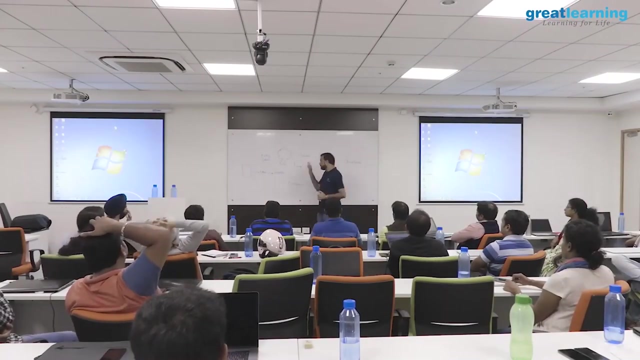 It is a pay as you go service, So you can get any type of machines you want and you only pay hourly basis or whenever how much you are using, right, So, and you can resize your cluster. all these advantages you get. So, and so that is what I am saying, So in. 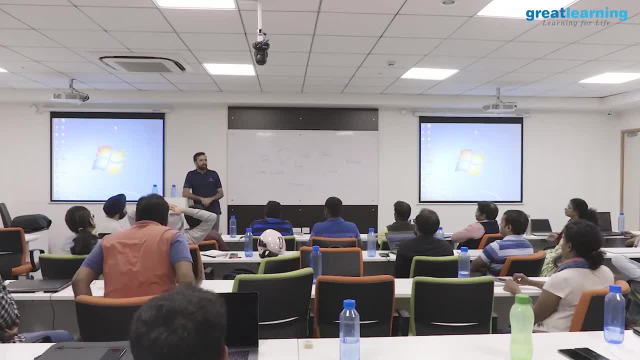 the very recent days, I have seen a lot of customers migrating to cloud or using cloud-based Hadoop infrastructure. I will show you this practically So. ideally I am supposed to talk for only theory stuff, And that is fine, But I also thought I will show you something. 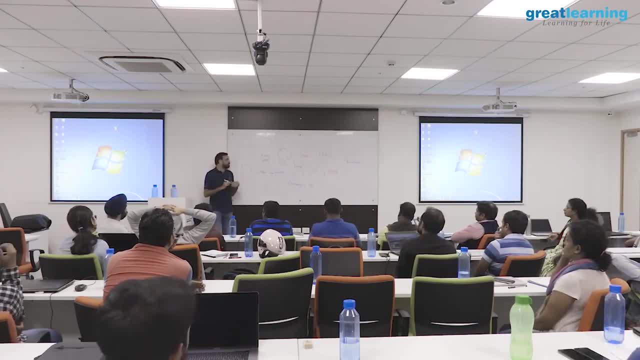 just so that you can understand, I will show you a cluster which we already have And I will also show you how easy it is to create a cluster in the cloud. Anybody can do it, It is not a big deal. But if somebody wants to build a cluster, how you can actually do, 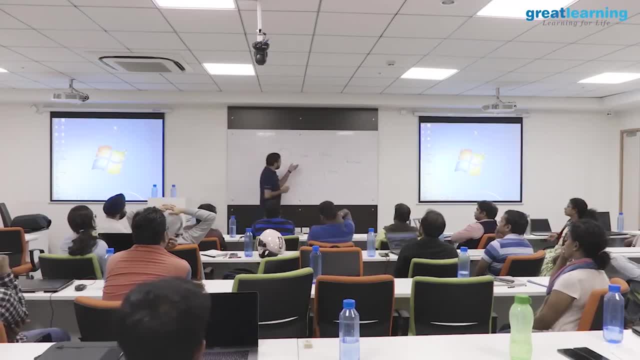 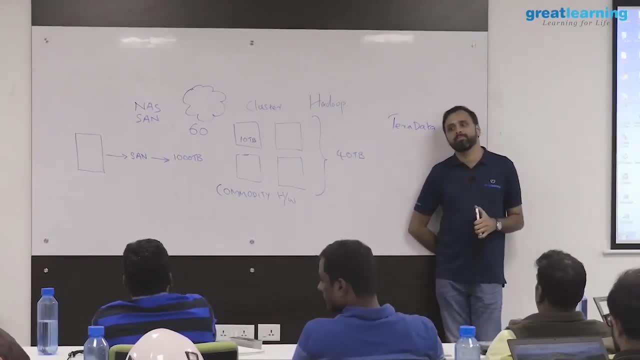 it. I will show you that right. So these factors will actually bring down the cost of your hardware, So you are not really spending a lot of money. So it is like you know somebody else is giving the service and you are just taking. 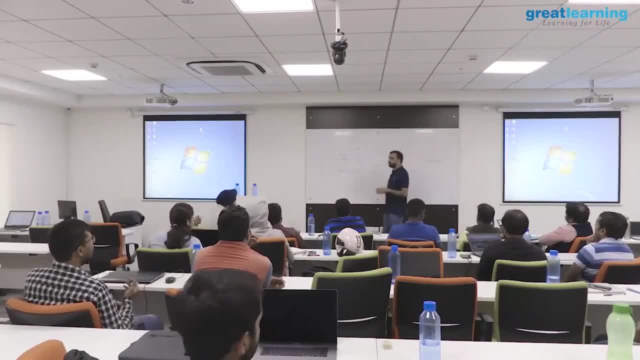 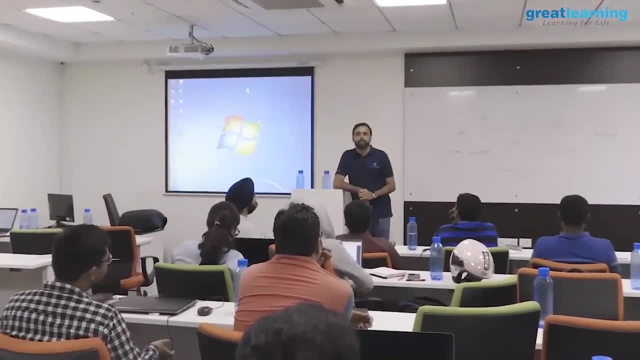 it Cloud? Yeah, like Amazon, for example, Amazon Web Services, Amazon Web Services Or Google Cloud or Azure. Anybody You sign up with them, They have that machine, They have that virtual informant and everything Exactly So they have their data center. 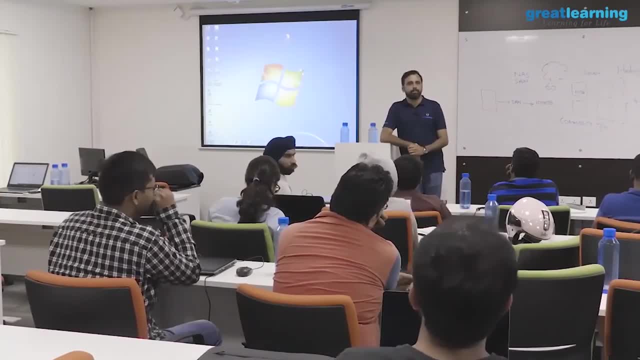 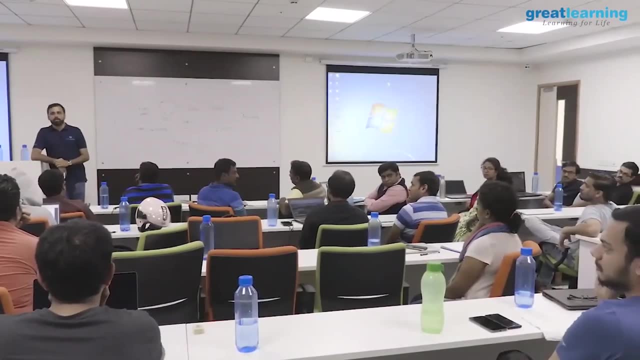 And you can. yeah, I have just started. You can send my company. So we pay around 40,000 rupees for 20 terabytes of the company. So the thing is that you just go to them and say that you can get the service in different. 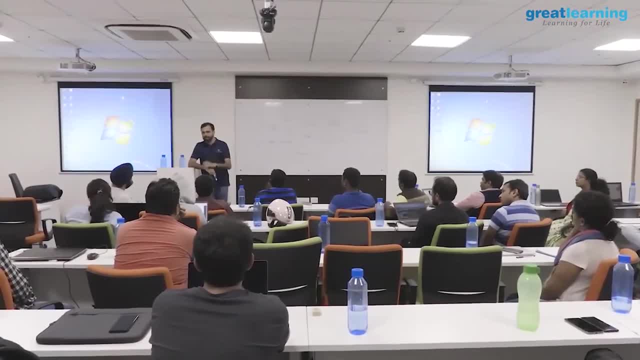 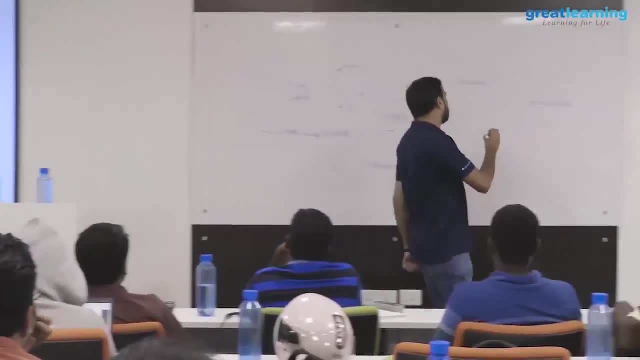 ways You can get compute service, storage service or anything as a service. And another term which people use a lot is something called data lake, And that is also very popular. There is something called a data lake. Well, this is not a lot to do with. 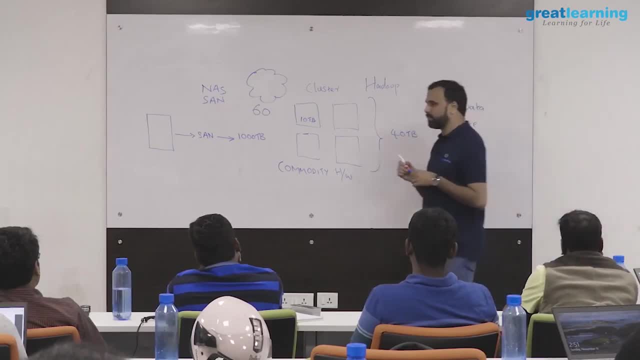 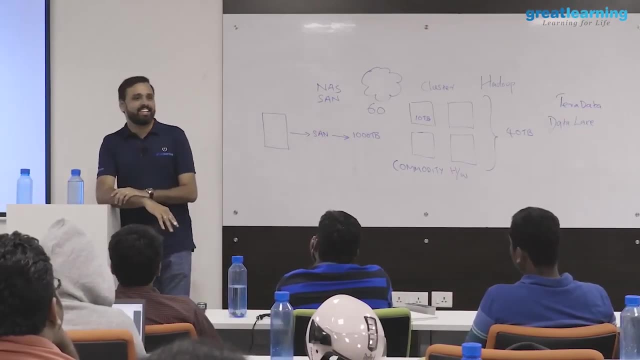 big data, but I just thought probably there is something called a data lake. Okay, I do not know how to define a data lake, to be very honest, because the technical definitions are very difficult to understand. A data lake is a common place where you get all the different. 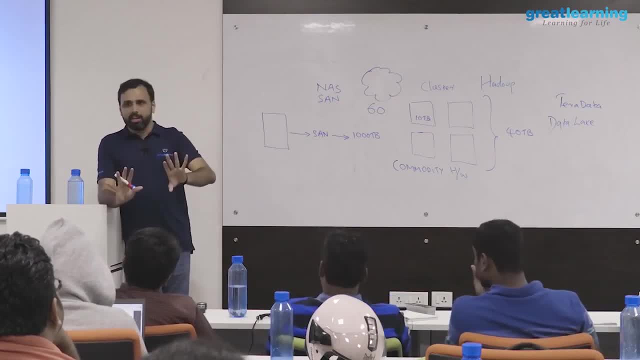 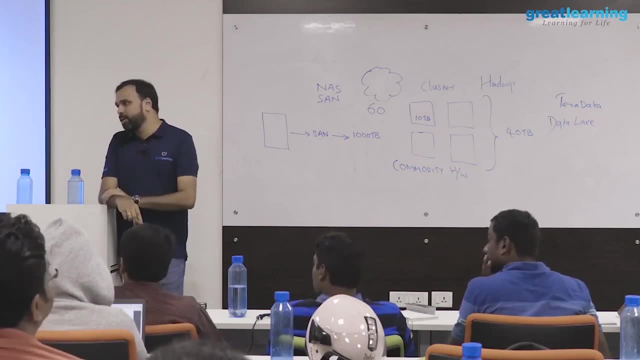 varieties of the data in its original glory. So basically, you can build a data lake, Like I think you are working on a data lake on Azure, right? So you get all the kind of different data. So these cloud platforms, what they do, they will offer this data lake. 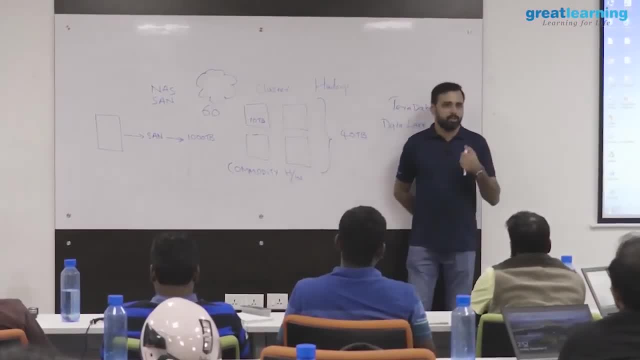 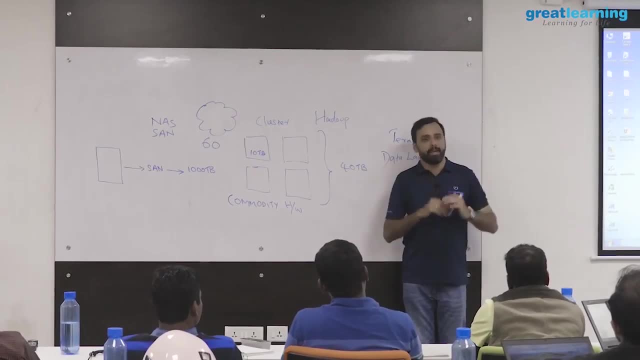 as a service like Azure or Amazon. So they will say that we will give you this data lake. Okay. So they will say that we will give you a data lake. What is a data lake? Nothing. They will give you the data in its original format, all the data in one place. From there, you. 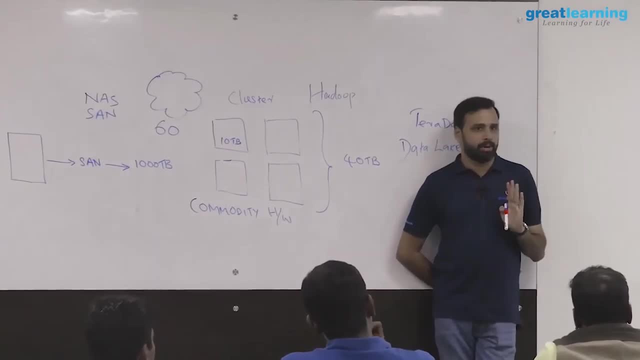 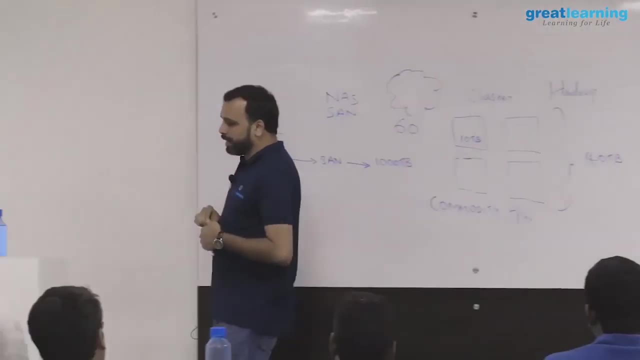 can start taking your data and doing whatever you want. So it is a common platform where all the data will lie. That is called a data lake. Yeah, So data warehouse is more or less like for structured data, Like you have tables. 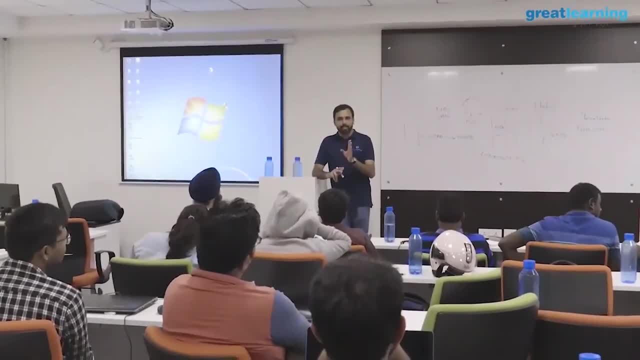 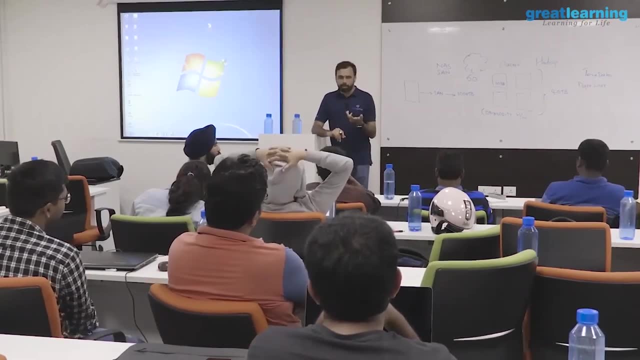 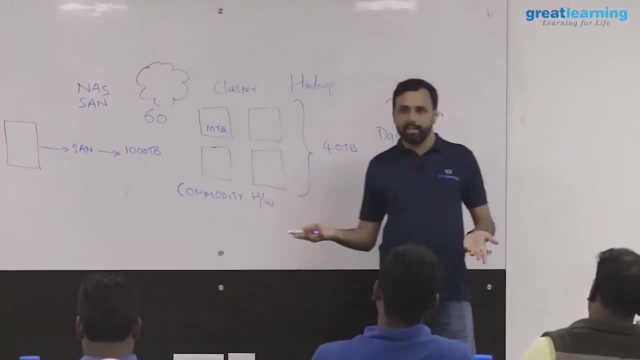 and then you write SQL queries. So data warehouse is always confined to structured data And as well as you are more or less writing SQL queries on the data, And a data lake is a place where you also have structured data and unstructured data- Any type of data that 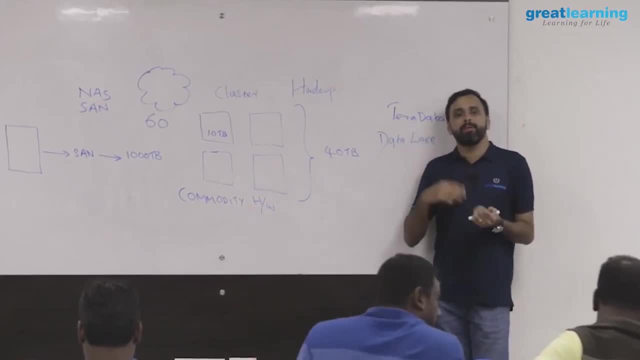 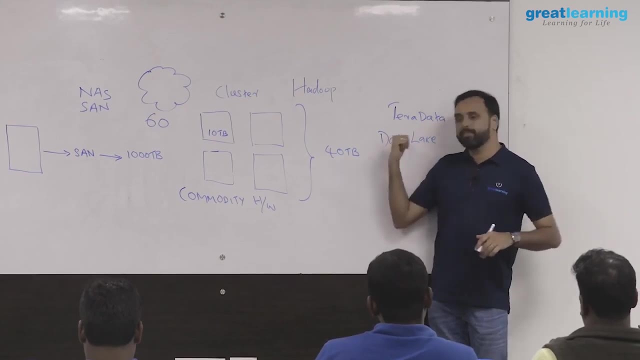 is coming from different, different sources And then people can connect with a data lake and make use of the data. So probably if I am a guy who is coming from SQL background, I can connect with a data lake And I can say: create a table and I just want to query. 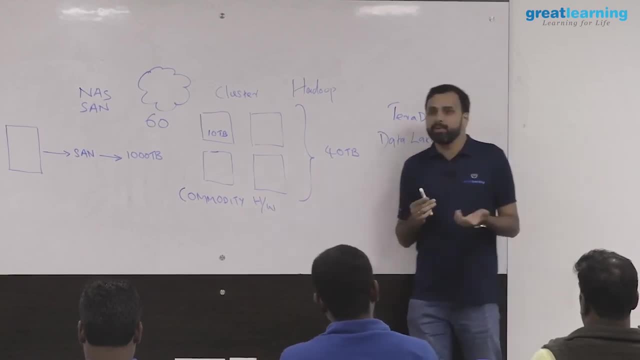 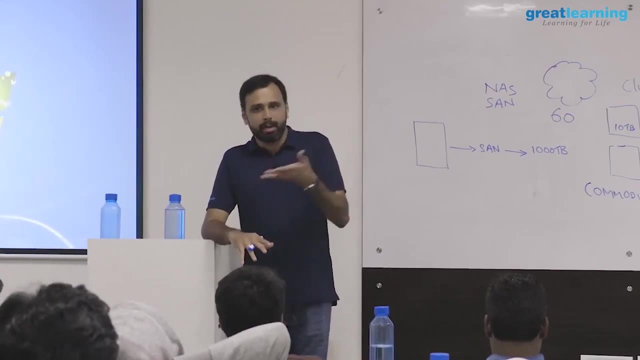 the data. But maybe, if I am coming from machine learning background, I don't want to write a SQL. I can say: read all these text files and I want to do my EDA and then build my machine learning model or something. But basically, data lake is a place where all your data lies. 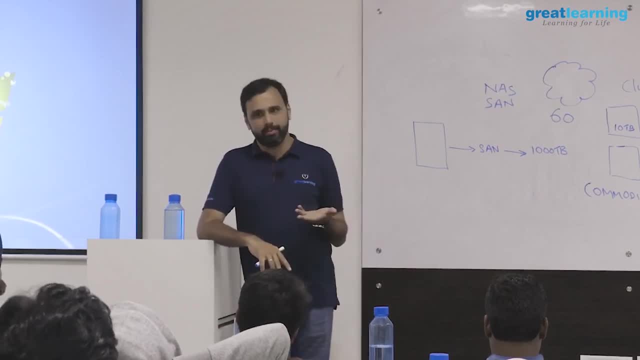 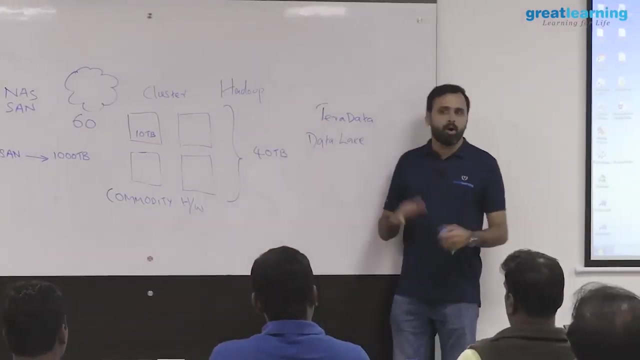 in its original format, And then you decide what to do with the data. So it is a service that is being offered these days. All the cloud vendors offer it as a service, basically. So I am more familiar with Amazon Web Services than the other cloud vendors, But all of them. 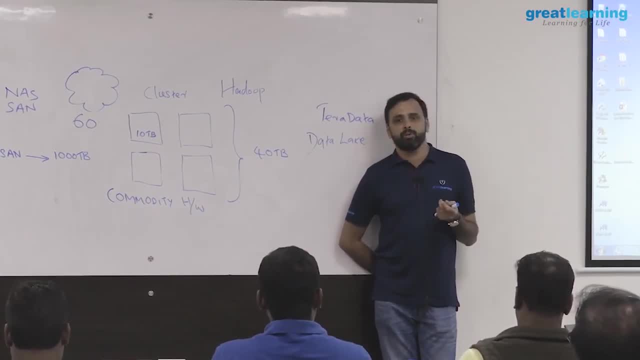 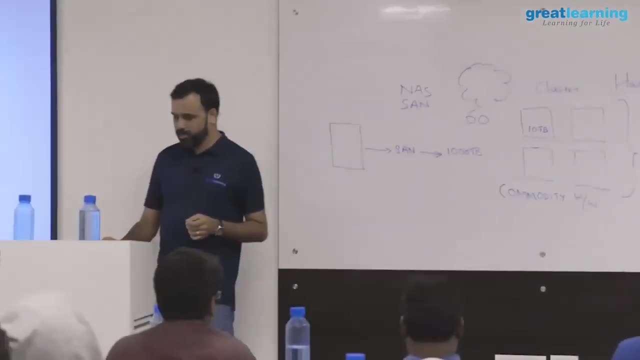 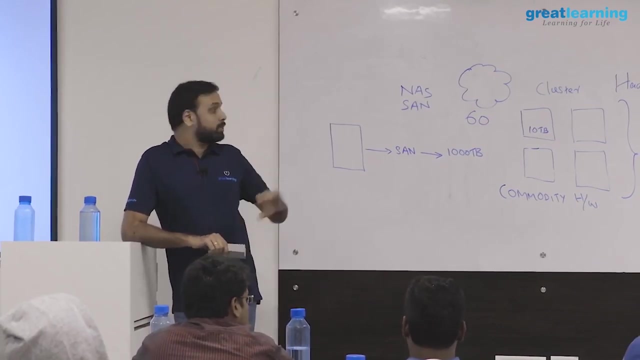 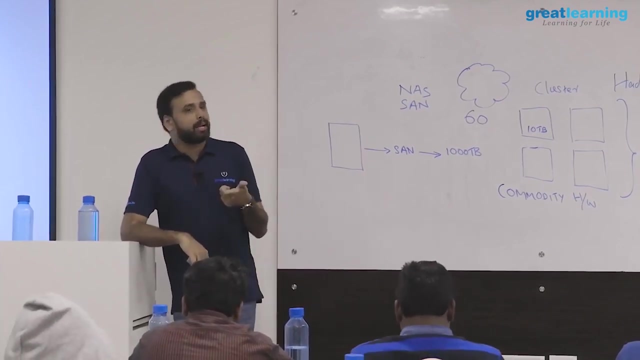 are having similar ways of doing it. Like you also have Google Cloud, Microsoft Azure, IBM, all these cloud vendors, right, Yeah, So there is no archiving in this platform. It is available, readily available If you want it and archive. Now that is what. when you go to the cloud, you pay for the data. 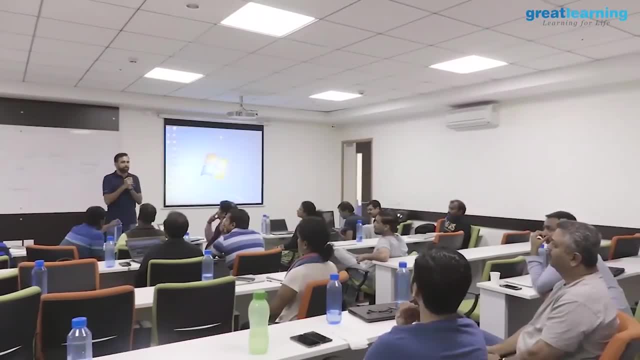 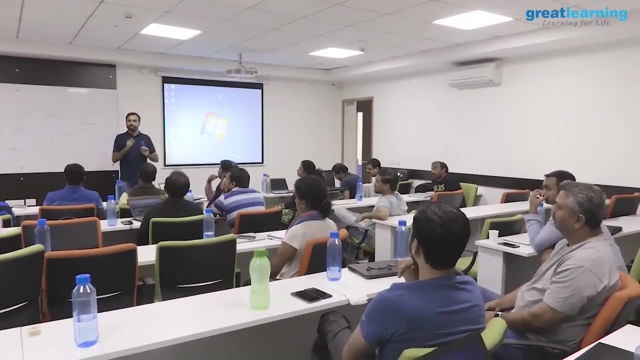 and you pay for something called the storage handlers, like how they are storing the data, So you can decide. So if I go to Amazon, Amazon has something called S3. That is the storage, primary storage, And that is the cheapest storage Amazon gives you. So Amazon. 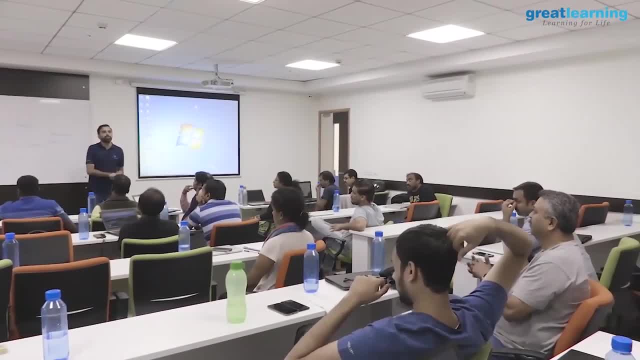 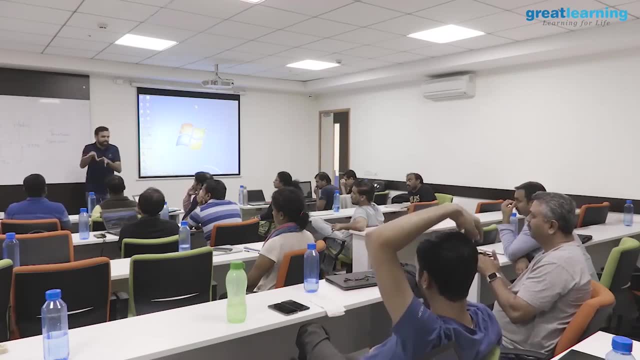 will tell you that, hey, you know what? all the data you want to store, I will give you S3. You dump all the data in S3. But what they don't tell you is that then, once you start dumping the data, they will say that in S3, I will give you three options. One: 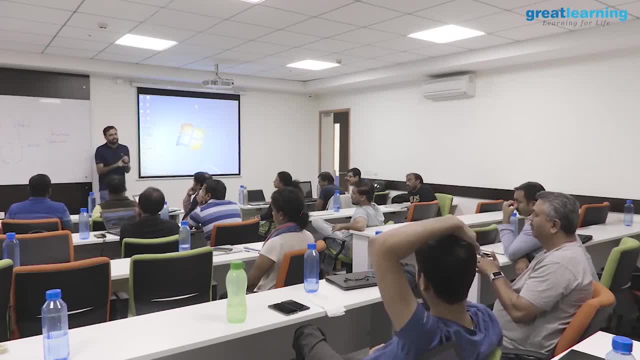 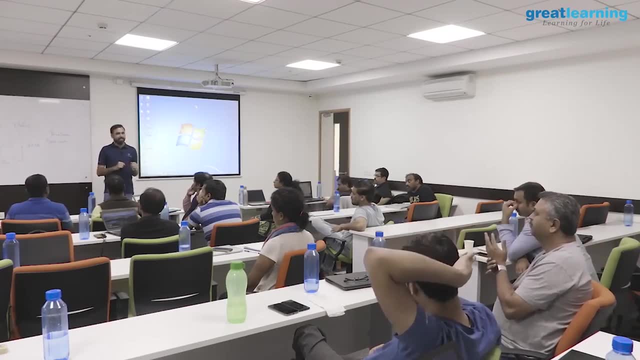 I will give you three options. Do you want in magnetic hard disk, Do you want it in SSD, Or do you want something else? If you want SSD, I will charge you more. If you want magnetic, I will charge you less. Okay, So still, you figure out. okay, you want magnetic, But again. 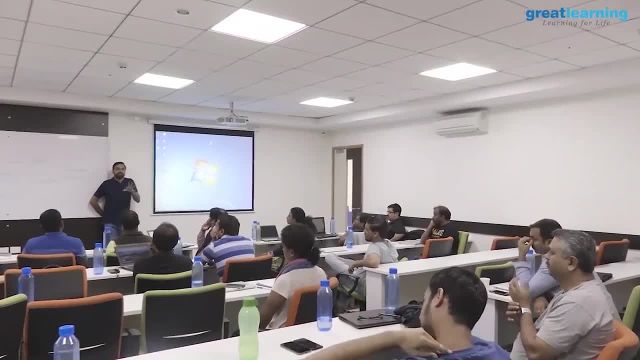 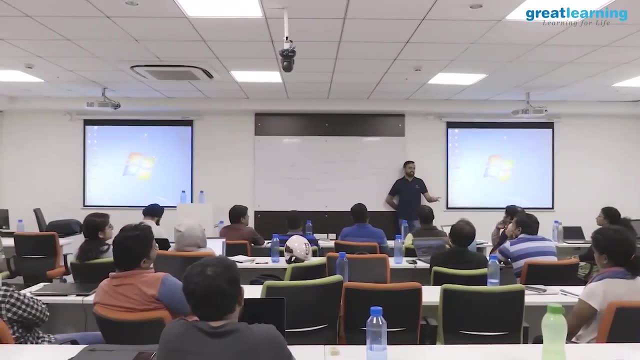 you are getting a lot of data. So then Amazon will say that, hey, your data is very high and I don't know where you will be able to pay, So we will give you an option. We will ask you to archive the data. We will give you Glacier. Glacier is their product for. 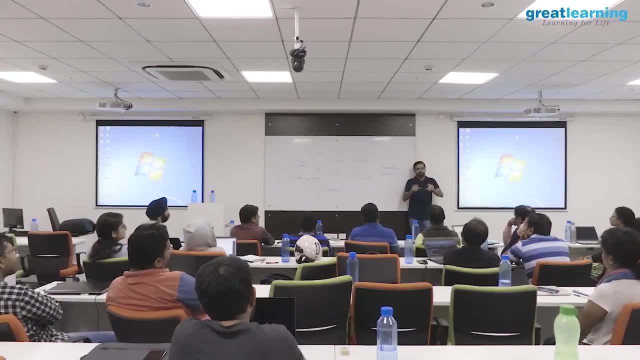 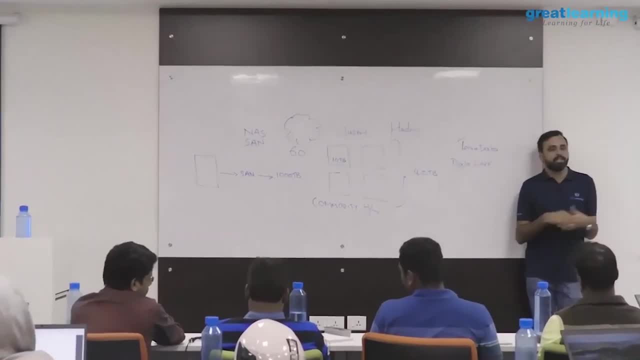 archiving. So they will say that in S3, we will keep your data. But if you want to keep the data, but if the data becomes one year old we will automatically move to Glacier archive the data. So Glacier is cheaper, So the customer can decide. So there is. 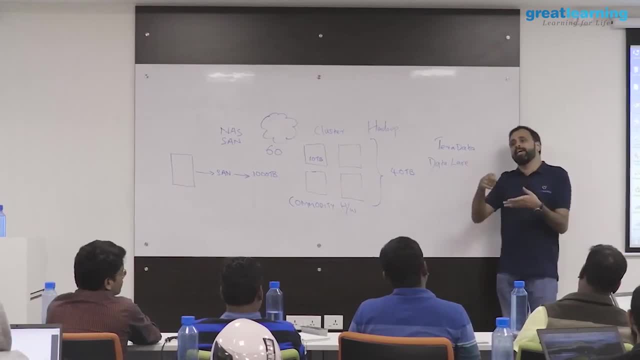 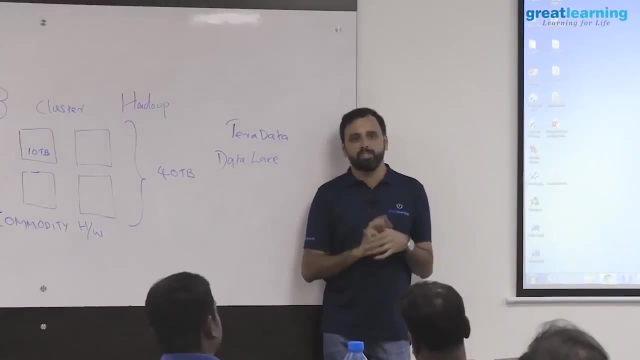 something called lifecycle policy. Customer can decide: if my data becomes one year old, what should I do with it. Should I delete it? Should I move to archive? Should I keep it here? Charges will be there, And what the cloud providers do not tell you, because we 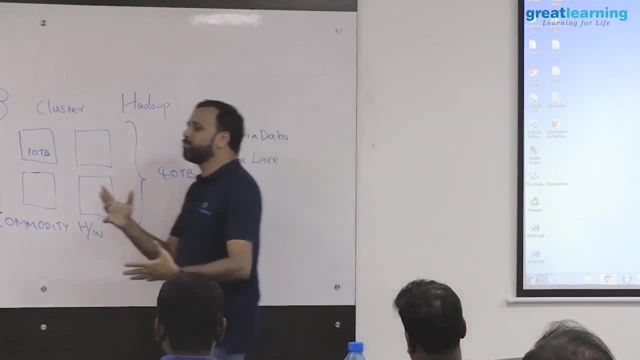 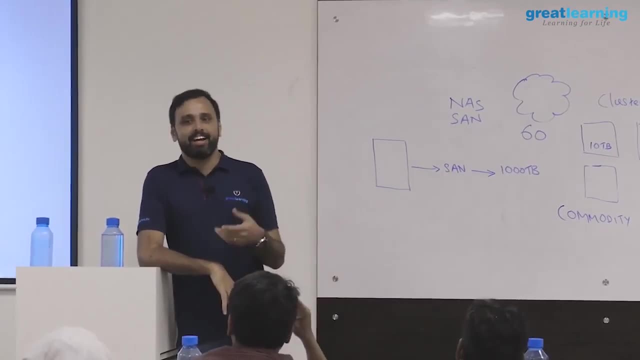 had a lot of bad experiences, is that everybody moves to the cloud, thinking cloud is the best solution, But in fact it is not. It is not And in fact it is not cheaper. This is not in fact. Yeah, And and the biggest thing is that if you are keeping your data in cloud, 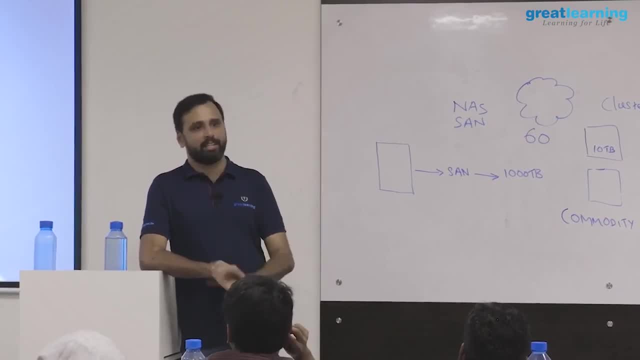 for uploading the data. there is no charge for downloading you. you will be charged. So in majority of the cloud platforms, when you upload the data, it is free. Free in the sense you have to pay for the storage. But if, let us say, I uploaded a picture somewhere, 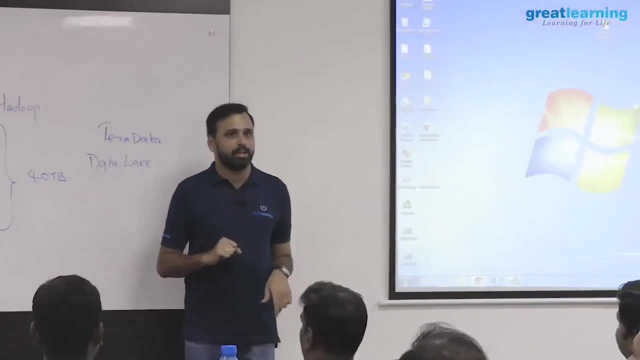 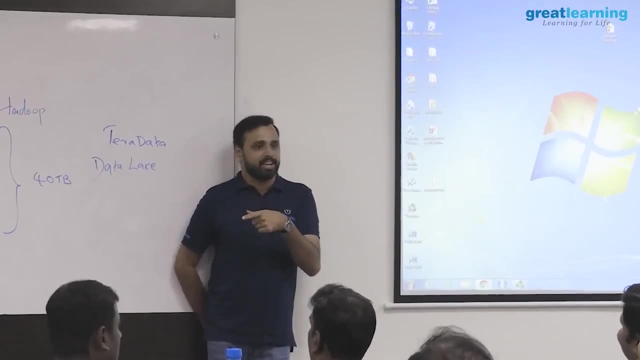 and if, let us say, one million people viewed the picture, then it is free, right. Then they will charge for this 1 million views because that is a data transfer out of their cloud, right? So these charges you will not see. unless you see your bill right. So then you're like: what did I say? So you will come back and say I'm just paying S3 only $500 and you give me a bill of 5,000?. That is the remaining data transfer charges. 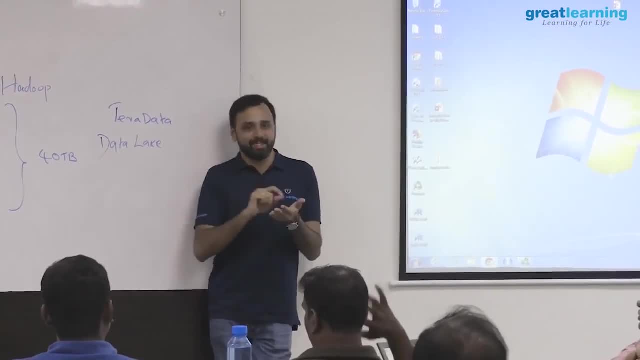 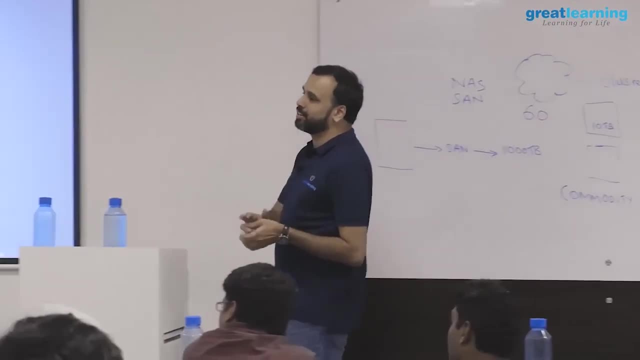 So then you start learning. okay, there is data transfer charges, okay, So then you start quoting. So we had a lot of bad experience with this. I mean, all the- Are you running a cluster or they charge? Running cluster, for sure, they charge. but for data transfer they should charge, I guess. If you're so, let's say you're keeping the data in some platform and if you're taking it out of their cloud, they will charge. per amount of data they will charge. 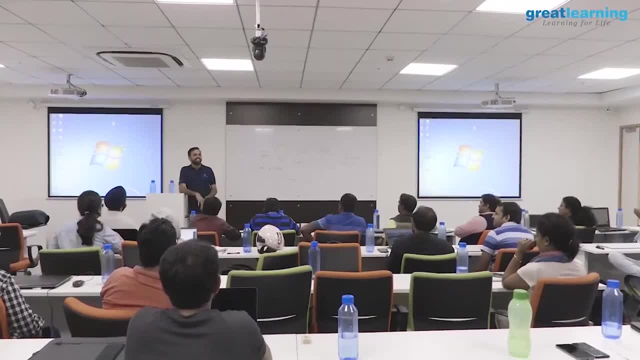 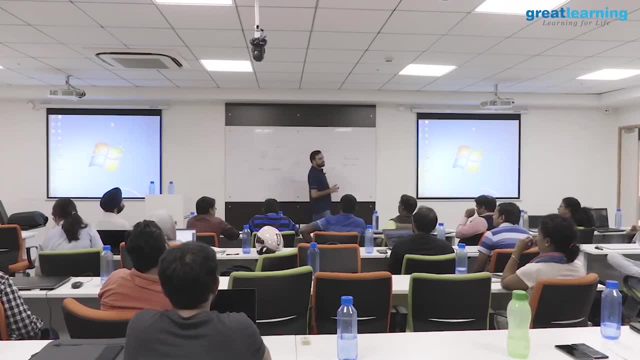 Let's figure it out, right So? nobody has any clue how this is working. So, end of the day, you pay the bill, right So? but data transfers are charged in the cloud. usually That is how it is. I think, what is happening with the cloud. is more than the cost. it's the elasticity, The manageability of the data center, and the infrastructure has become more costly up there than the hardware itself. So now these cloud companies are actually giving you the hardware plus the manageability, which is much cheaper. 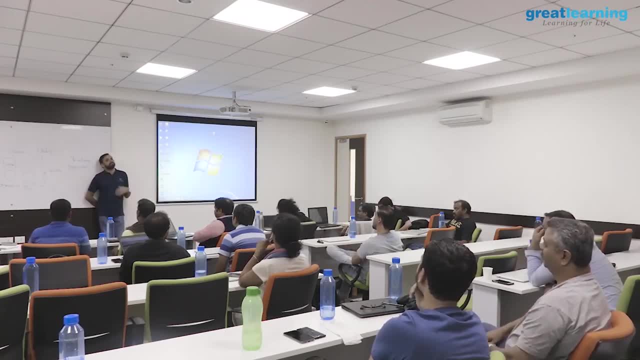 So that's where the benefit of the cloud is coming in. So, like O'Reilly said, one of the advantages of cloud is elasticity, Which you cannot get on-premise, Like all of a sudden you want 100 machines. you cannot buy it, you get it on the cloud. 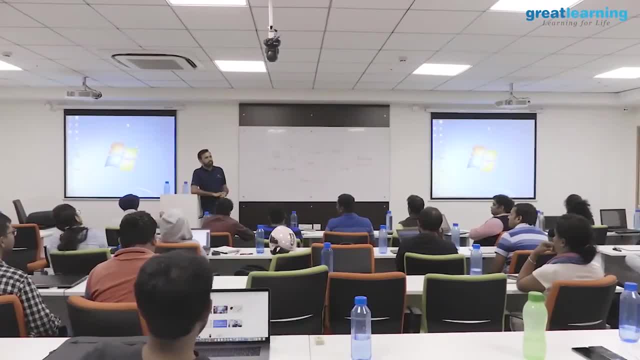 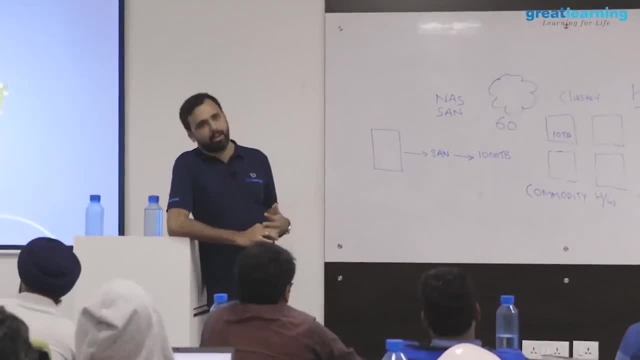 The second thing is the manageability part, where everything is managed by the provider for sure, right. Yeah, speed and all are also fine, And you get numerous services free on the cloud, So they're fine. I mean, I'm not blaming the cloud, everybody's on the cloud. 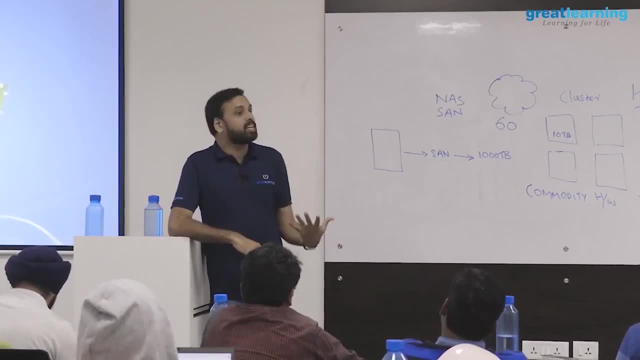 So there is no way to blame it. But a lot of hidden charges are there which people don't understand When they learn cloud, they don't know how to do it, So they don't know how to do it. So they don't know how to do it. 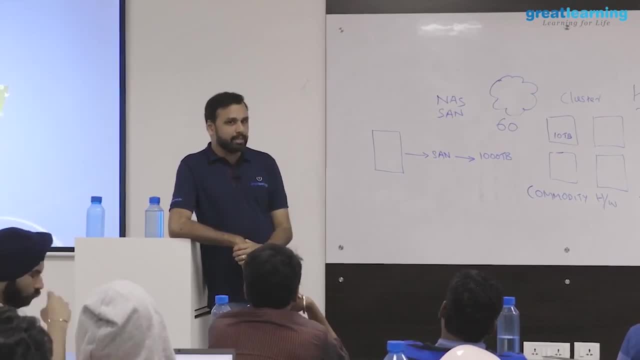 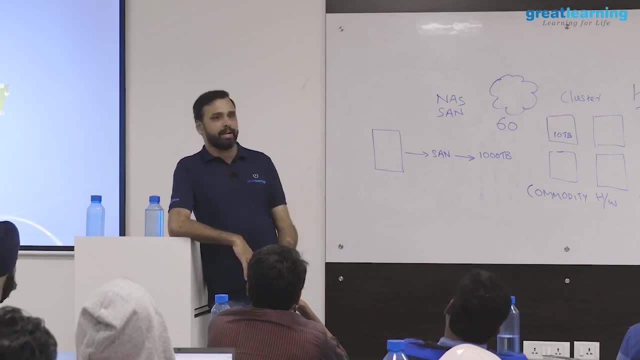 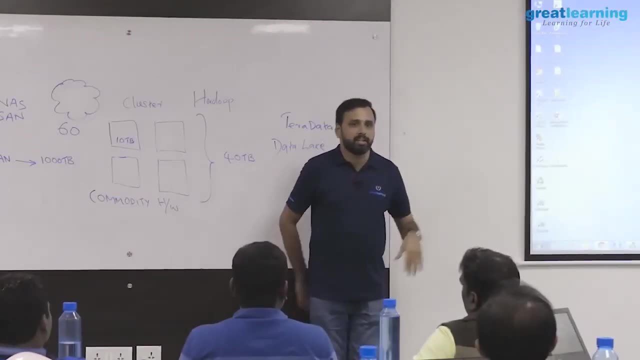 So for a lot of times we had experience like we personally fight, we were using Amazon. But that's the story with every vendor. Sometimes you fight with them and say that you know I'm going to another vendor, So they will say they'll go for three months. 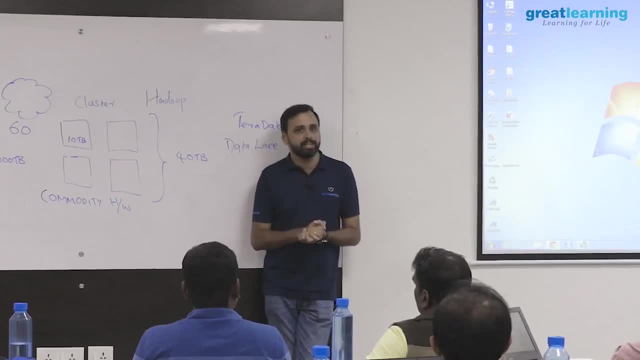 So in these three months, you understand how to cut down your charges, But, end of the day, it is much cheaper than on-premise. You're building something. on-premise is very costly- your own data center and all right. So, but yeah, but cloud always becomes a topic. 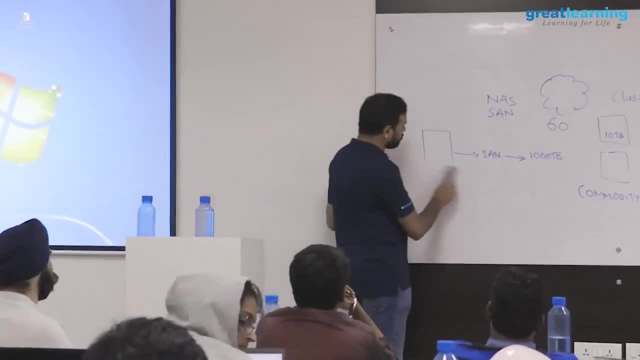 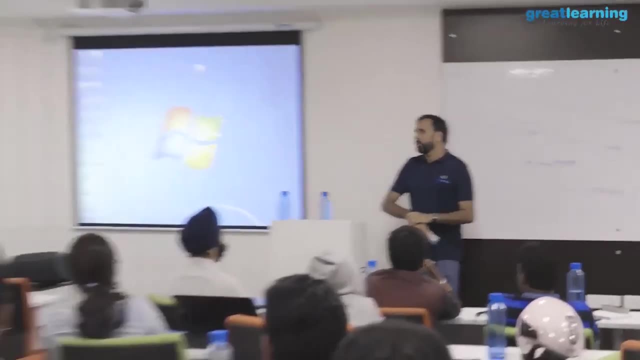 even when you are discussing big data, and all right. So in this case of Amazon, did they have they need to have huge amount for the storage? Yeah, exactly, They have, they have. They have big, big aircrafts. 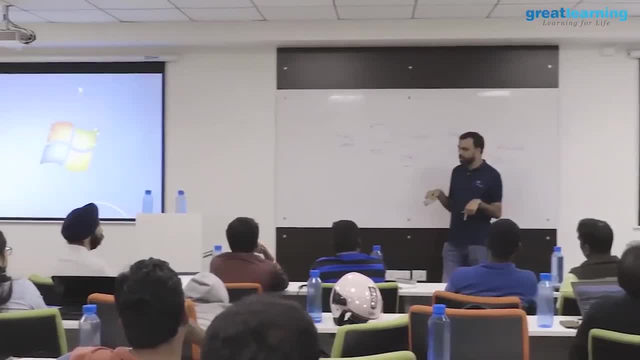 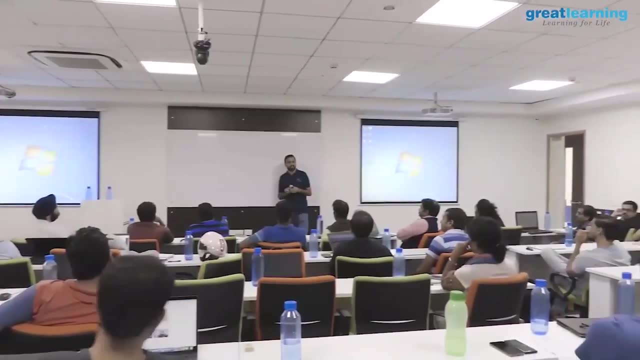 So Azure data centers are the size of a football field actually, And they have I don't know how many hundred plus like that server farms they have. So this Amazon S3 is a very interesting service, because your entire Instagram and Dropbox is on S3. Think about it. So what will be the size they are handling? Entire Instagram and Dropbox is stored in S3. And that is just like the equivalent percentage of storage in Amazon of S3. That is just two clients, So S3 is probably the most widely used storage service. in the world. Nobody can beat it because they started first For enterprise. Azure is more reliable For public access, S3 is more, because it's a very cheap action, drag and drop kind of Azure also. So now, yeah, sorry, 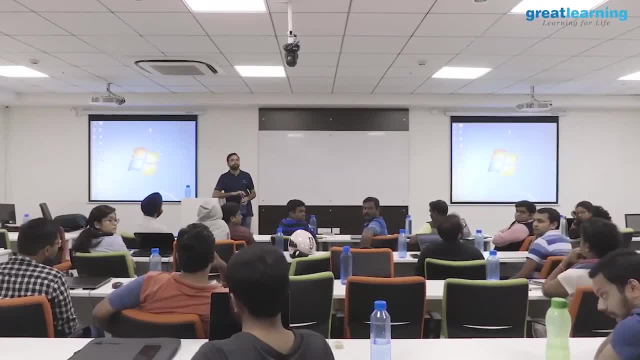 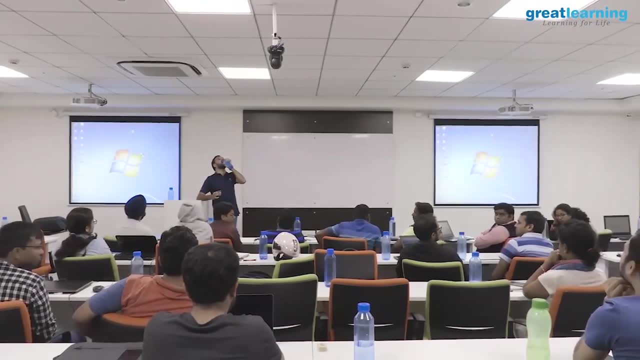 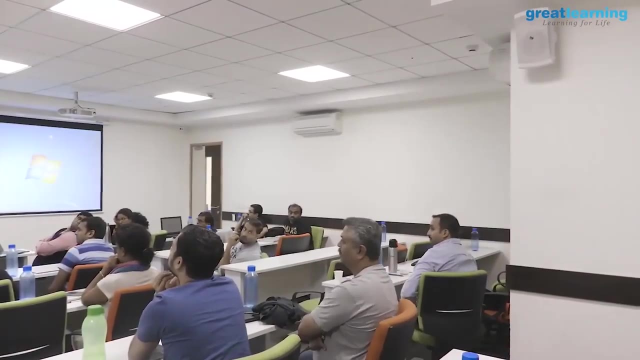 For startup companies, for them to stand up and try to get you know data out. probably try to get the data. Is there any kind of if you're seeing the 10-year evolution of how data is transformed? is there any benefit analysis? that is kind of there that. 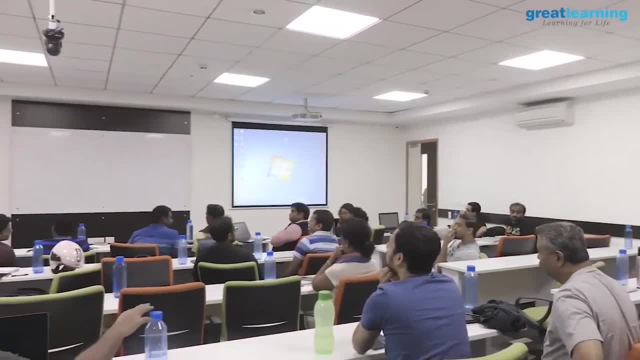 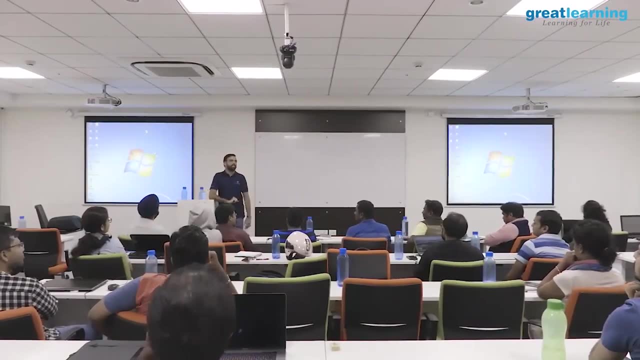 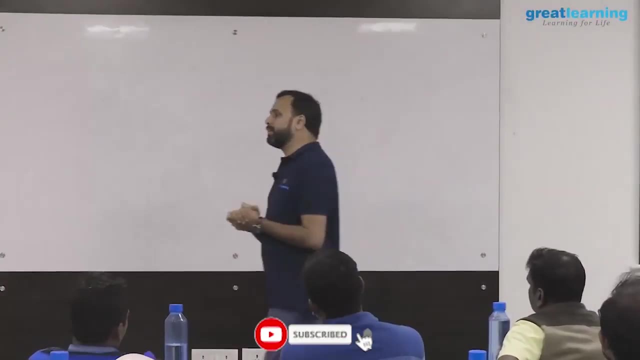 okay, that means that they can probably let these startup companies kind of invest in that. Yes, So the? so previously, what startup companies used to do? they used to build their own hardwood cluster and all which was very costly. Now, in the cloud perspective, 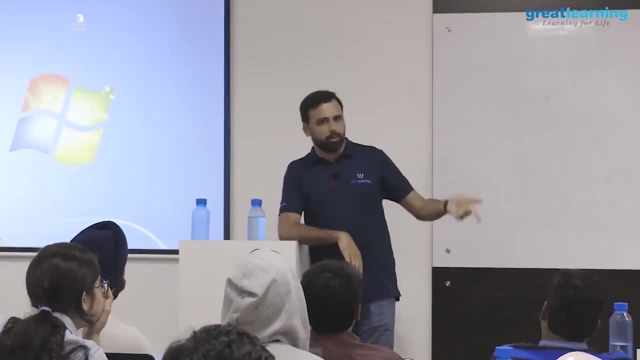 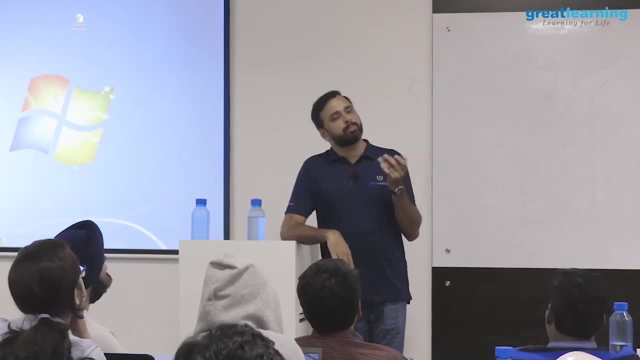 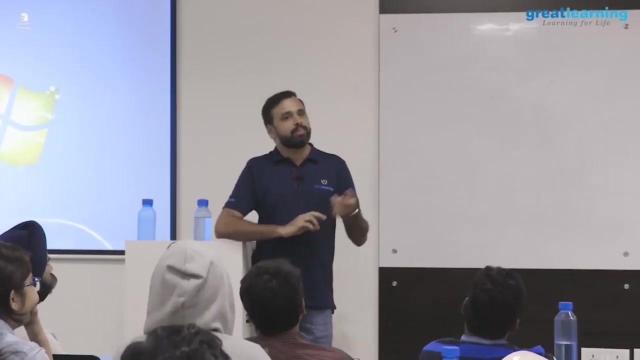 there are some solutions, which I will show you. one solution: I was about to show that Amazon has a solution called EMR stands for Elastic Map Reduce, wherein that is specifically for, like startup companies or companies who do not want to run a full-fledged hardwood cluster. 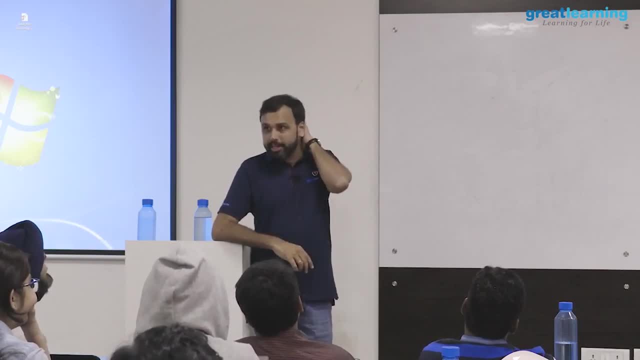 So we had a customer. it was an Australian client. They were an e-commerce website company. They were a startup. Their problem is they are already in Amazon, Their website, everything is in Amazon and they have a lot of data stored in Amazon. 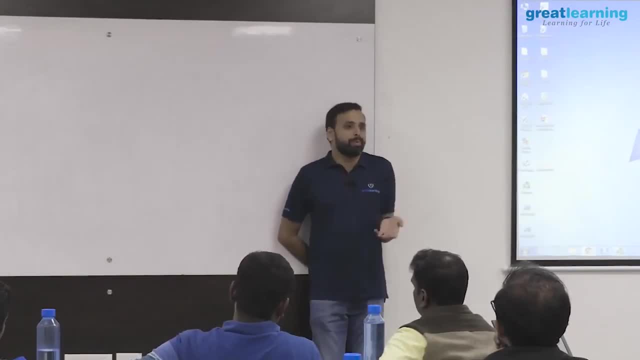 So they're happy with the storage. but now they want to use Hadoop and Spark and all for analysis. So that means they have to create a cluster which they're not ready, because they don't want to spend a lot of money in creating a cluster and analyzing the cluster and all. 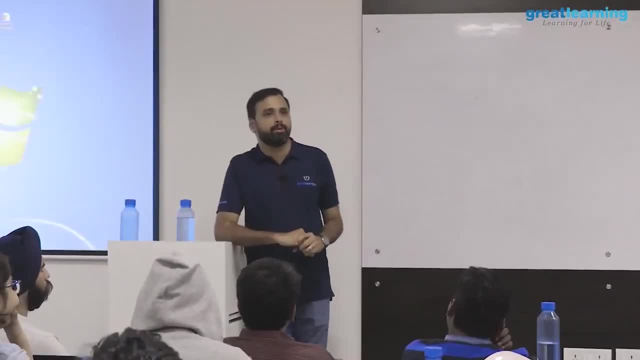 So that is where the solution called EMR can help you. EMR is actually a disposable service, meaning you go to Amazon and ask Amazon that I want a Hadoop cluster in five minutes. So Amazon will ask how many machines? You say a hundred machines. 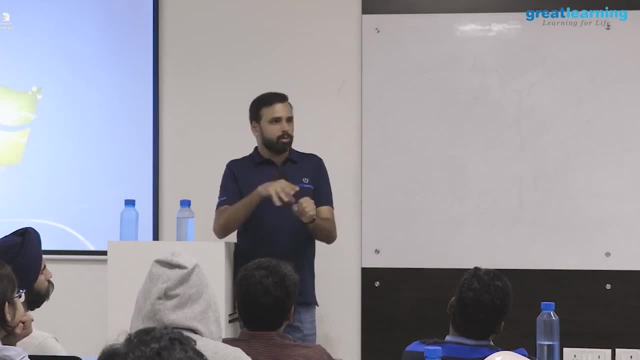 They will create a Hadoop cluster, install everything and give you, let's say, a hundred machines in five to 10 minutes. And let's say you get the cluster, you run it for one hour. In this one hour you analyze whatever you want to do. 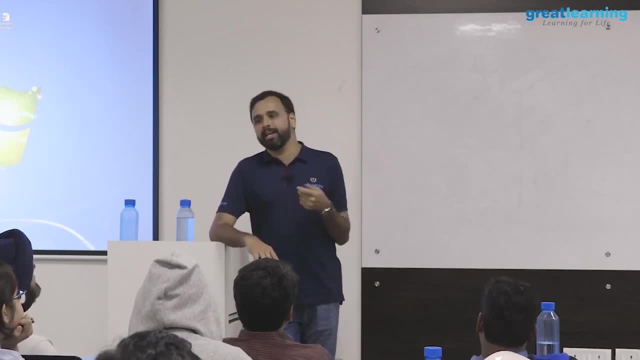 You do analytics and all delete it, terminate it. So it is like a disposable service And you're paying only for one hour, Very cheap, Because otherwise I have to manage these hundred machines throughout the year. that is not required. So Azure service is called HDInsight. 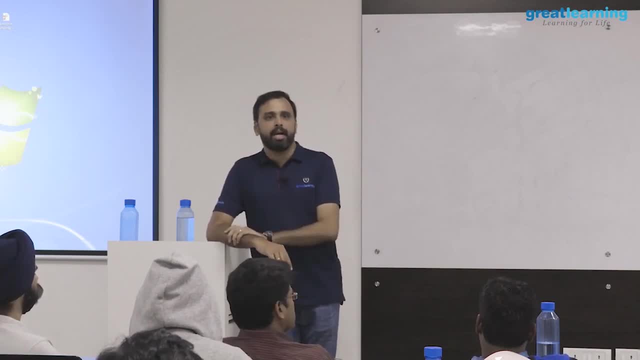 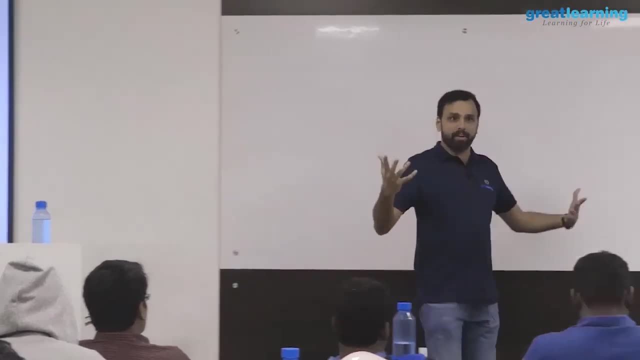 Maybe you could have heard about it. There is a service called HDInsight, very similar, And Google Cloud has Dataproc, that's also similar. So they are like clusters which can be created on the fly and you can keep them for a shorter period of time. Maybe two days, three days also, But there is no way you can stop them. Once you create them, you have to delete them, Unless there will be huge charge. So for ad hoc analysis, like startup companies and all they do this. 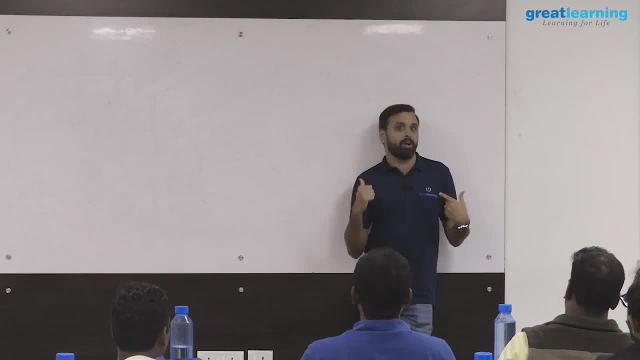 And another advantage is that normally, when somebody is creating a Hadoop cluster, you need the knowledge How to install Hadoop, how to set up Hadoop, which people may not know. right In this, Amazon will do everything for you. 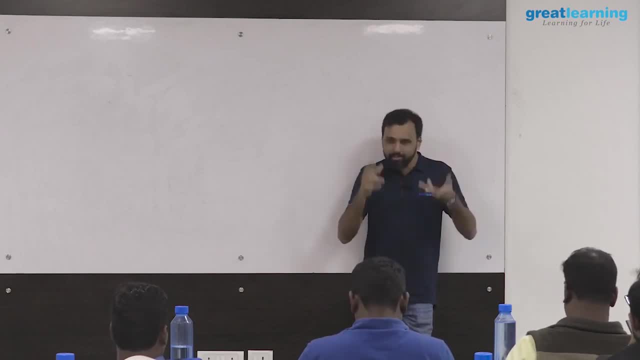 So you just need the knowledge of a developer right And everything will be installed and configured and given to you. You just have to use the service. So you practically do not need an administrator. So it's a very manageable service. I'll show you how to create an EMR. 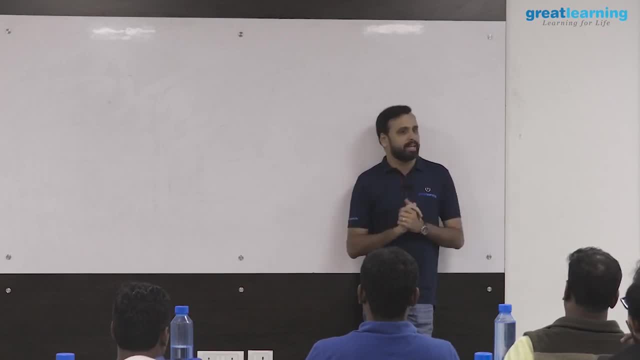 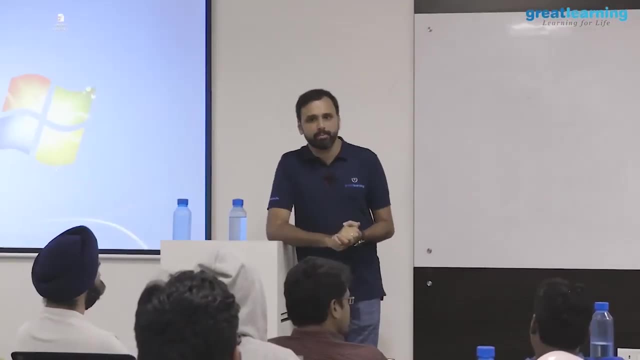 it's very easy to actually to do And then you can start playing around with it. So you can see this, which even some of my previous clients were interested in doing because they were not ready to run a full-time Hadoop cluster. 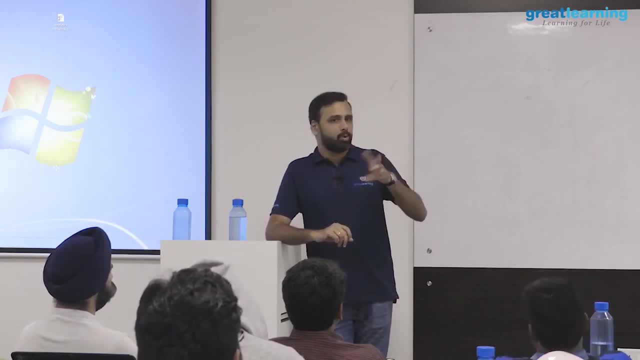 So they wanted. whenever they want, they will create it and they will do the analysis. Then they will delete it. End of the day, Man. Yeah, that is where we are wrong. Startup companies, it's not that much. They don't have that much data. 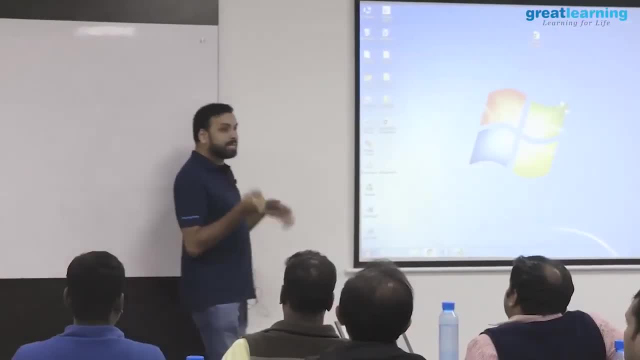 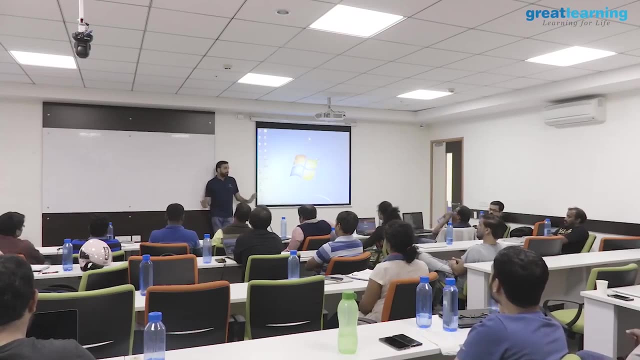 No, that is where we are wrong: Startup companies. they don't have that much data. that company may not have fixed data, but it will have a lot of public data. So they want to analyze the social media trend. right, That is common for everybody, right? 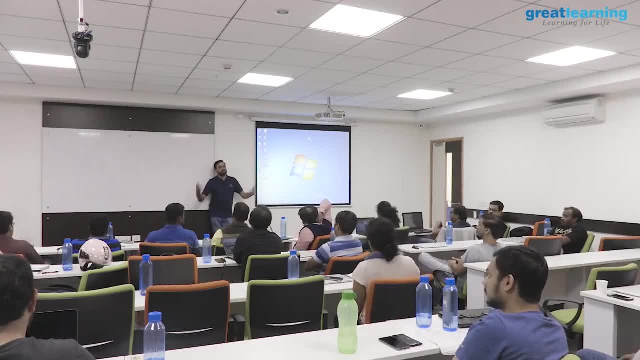 So the social media data will be huge which anybody can download. but to download that and analyze that they need a Hadoop cluster. So they can create something like this on the fly, probably a small cluster, analyze it and then delete it if they don't want data. 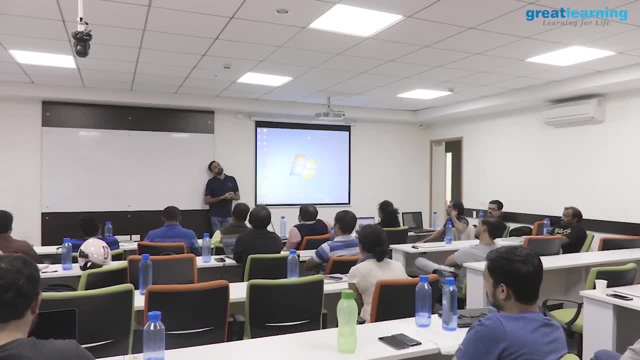 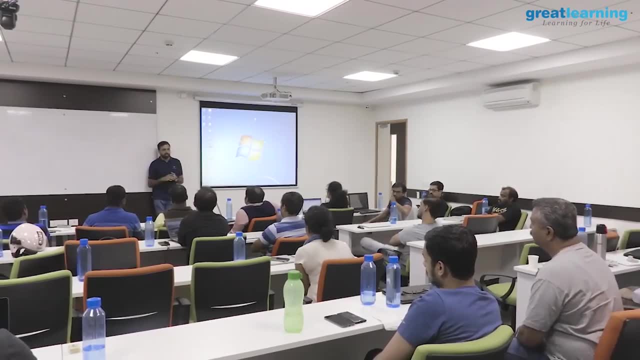 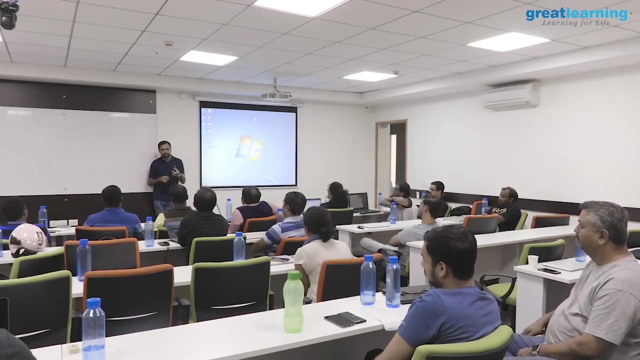 So one use case. I'm saying So. a lot of people are there who are interested in analyzing a lot of public data. right To predict what is happening, what is not happening, et cetera. right, In this great learning, we had a project, not in BABI. 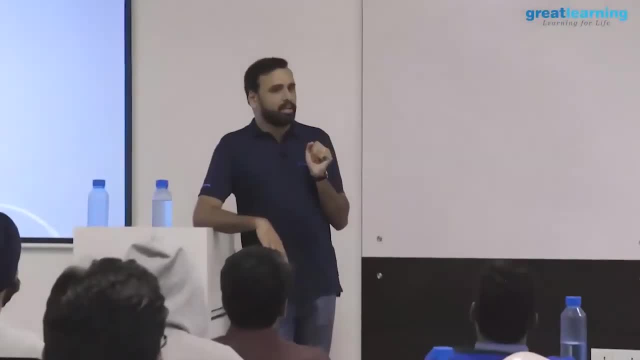 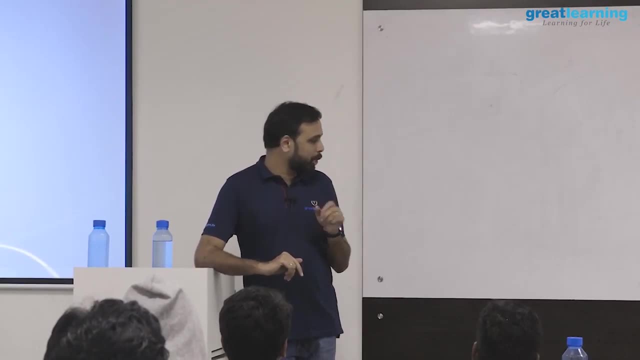 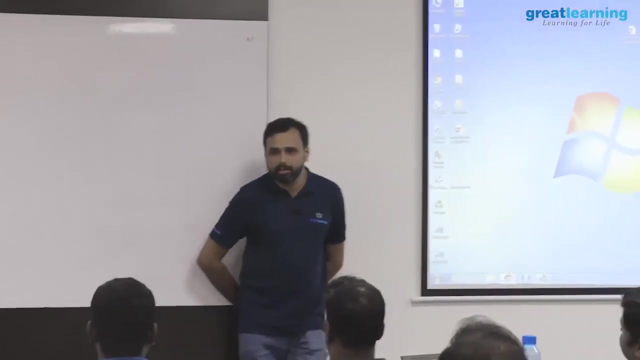 We have an AML course: artificial intelligence and machine learning. There people have done a project of judgment summarization This low, what do you call crime? right? So you have this: judgments by the Supreme Court and High Court, and all right. 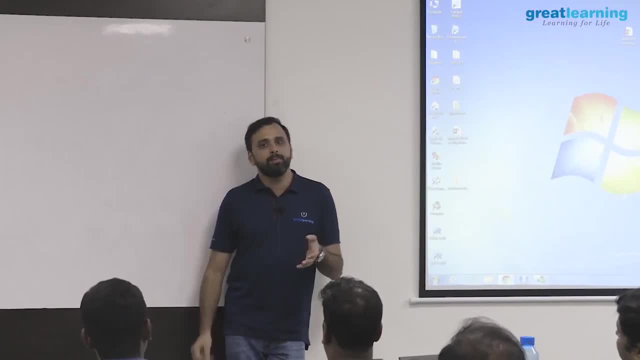 So what happens when the judgment comes right? The judgment is very big, like 200 pages, 300 pages, So let's say the Sabarimala verdict or something happened. So if somebody want to read it, it's like 300 pages. 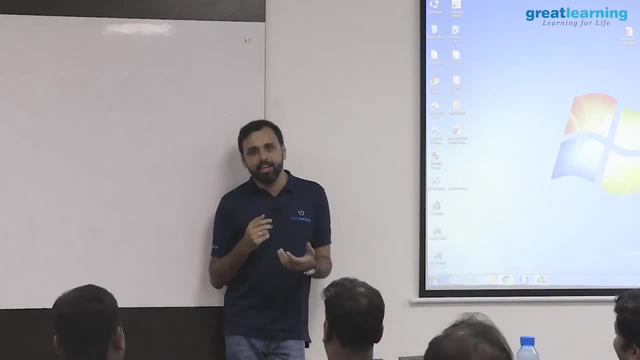 You can't read. I mean you can, but you have to spend a lot of time. So they built a machine learning model which will summarize. it will summarize into one page. The system will automatically read basically text, analytics, and then it will summarize to one page. 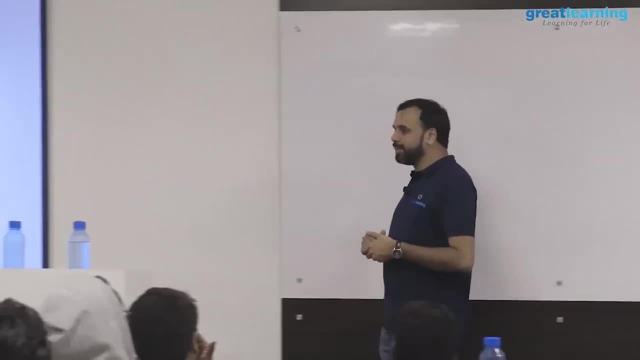 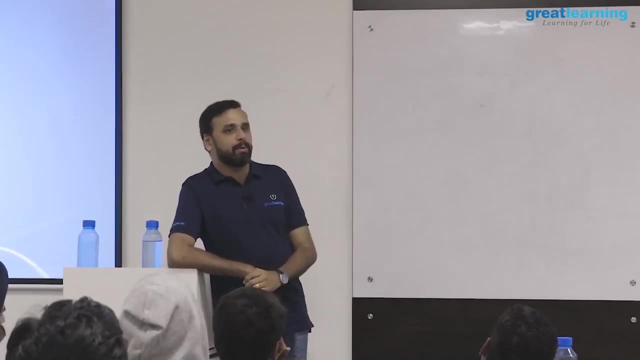 So they did it as a part of their project here And I think then they moved to you know, building it as a company. They started it as a startup company Because that idea was very interesting. They got funded also, I think. 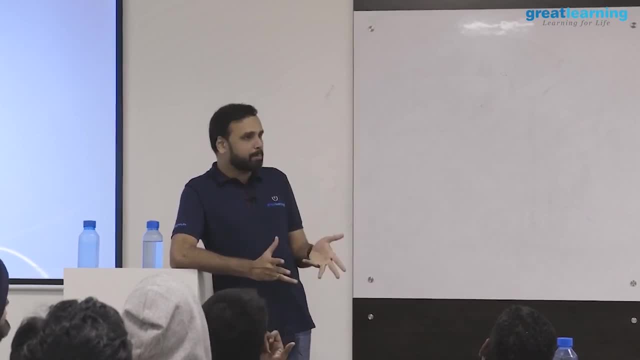 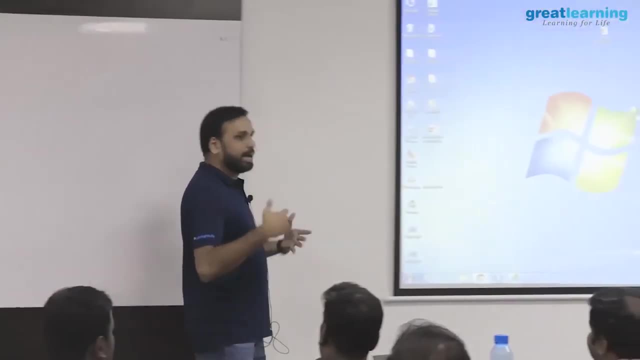 Now these guys were getting. so what I'm saying? it's a startup company, but they were having huge amount of data. They were collecting the low related data from India and US and so many other countries. So the amount of data they were getting. 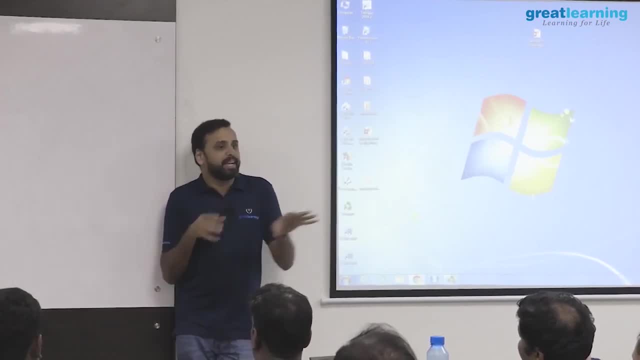 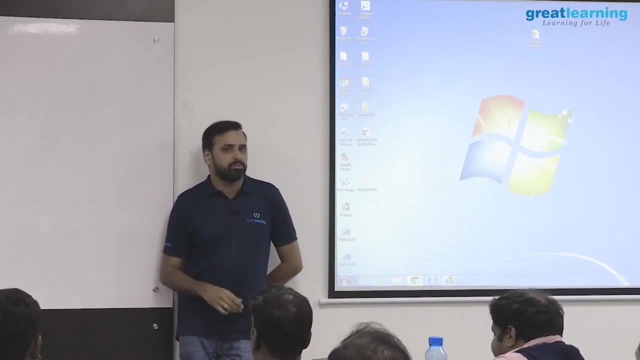 were very huge actually. So, even if it's a startup, the data they wanted to manage was very high actually. So they had discussed with me some solutions: whether we can use data warehousing or something to store the data and then later use it and all. 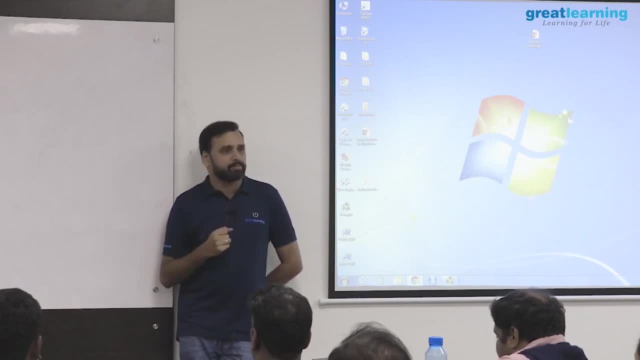 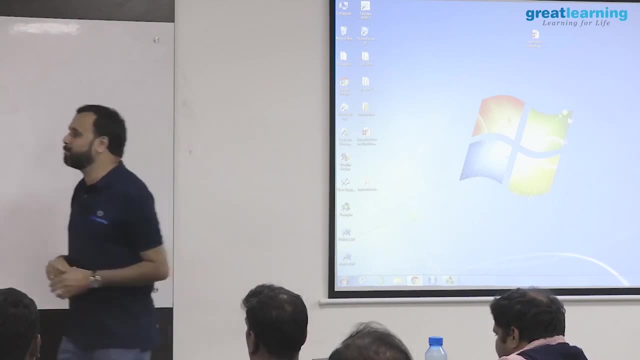 We had a short discussion, I think we started the company. it's in Chennai, The bash was in Chennai And I think the company is also in Chennai. That's very interesting. You guys also have a project right Now. I have to actually talk about the. 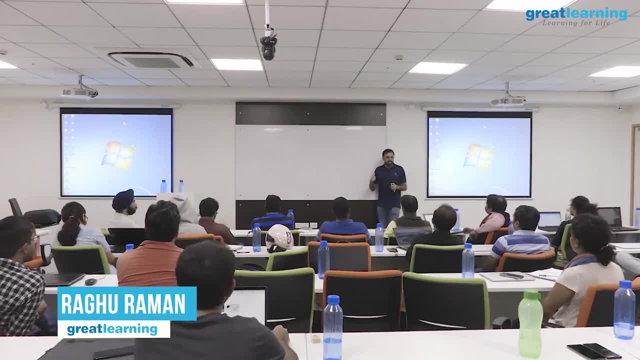 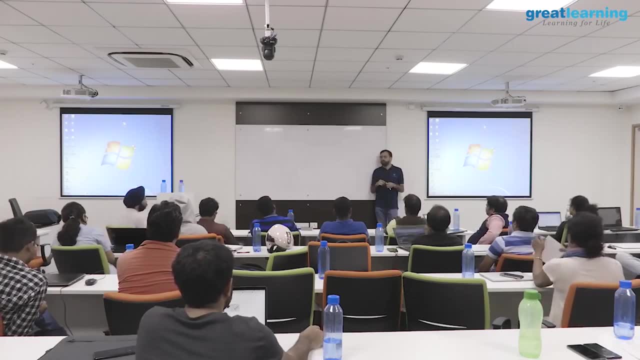 something called big data ecosystem. So, rather than talking in general, I have to tell you what are the products we use, where we use them and why we use them right. And you need to have a rough idea about them, Like if you hear the name, you should say: 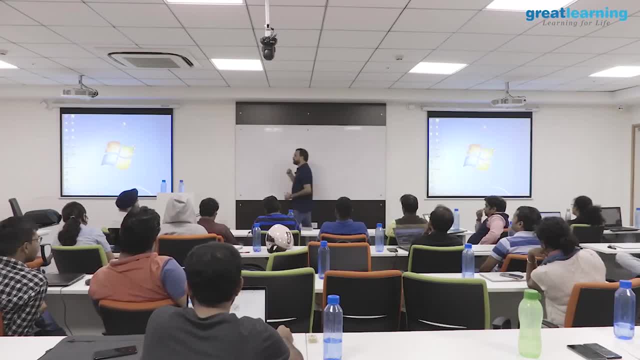 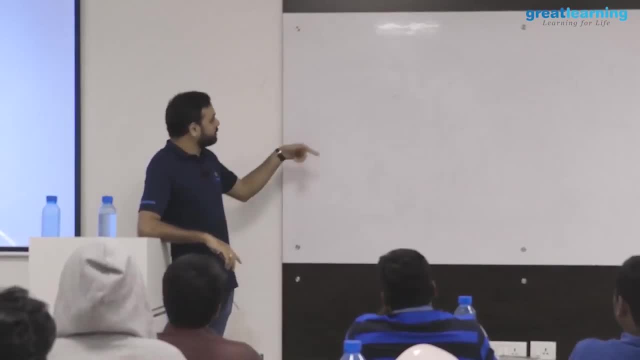 okay, this is what I'm using Now. in order to explain that what I'm going to do, I'll pick up a use case That's better. This is the use case which we were working and that will cover most of the products. 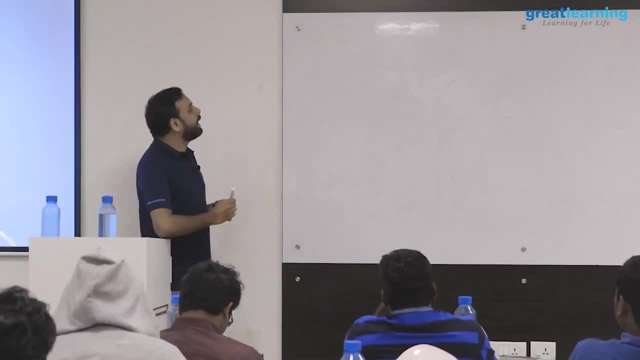 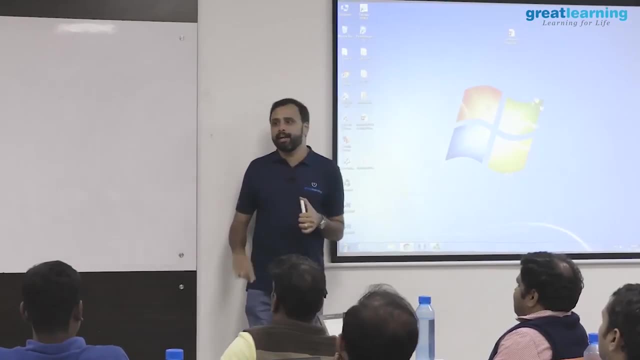 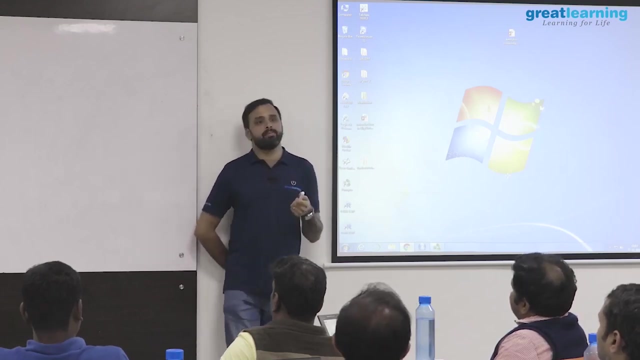 at least majority of the products right. So the use case we had was the migration of ICICI bank in 2012.. ICICI bank had migrated from the traditional platform to Hadoop back in 2012.. And at that point in time, my company was the major consultant for them to migrate. The migration actually took two years. It took two years Almost, And later the support was changed. I was also part of the team which did the migration. I didn't do the complete migration or something. 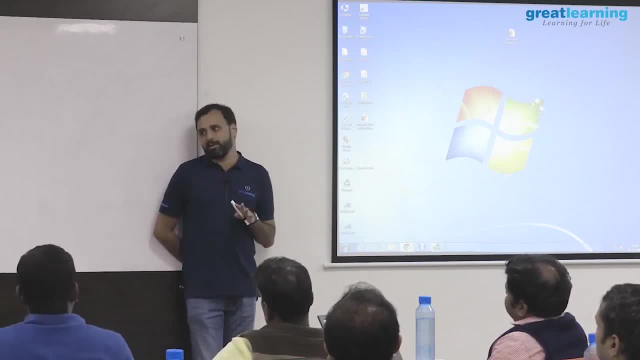 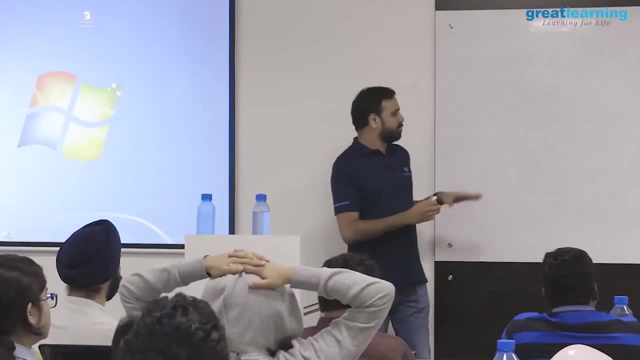 but I knew how it was happening, like which were the parts which were migrated and all. So I'm just going to take the same scenario so that we can understand what are the- you know tools that are actually involved. right, So you are migrating to Hadoop. 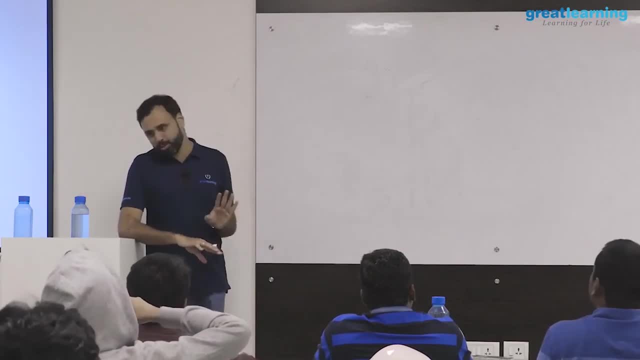 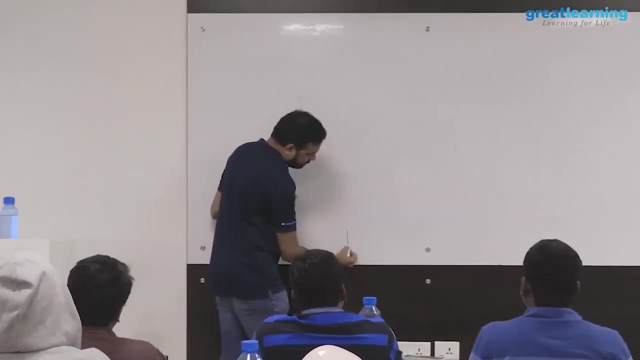 So that means, Hadoop is there. So first thing is that Hadoop is there for sure, because for managing that data you have Hadoop. right In Hadoop you have something called HDFS. I'll just write it here: 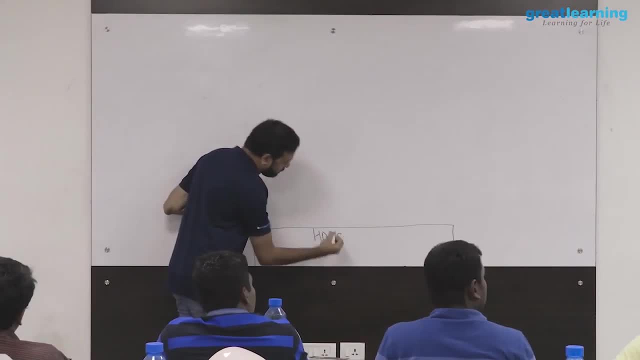 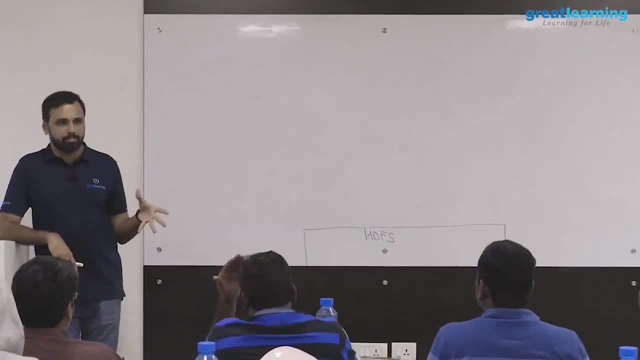 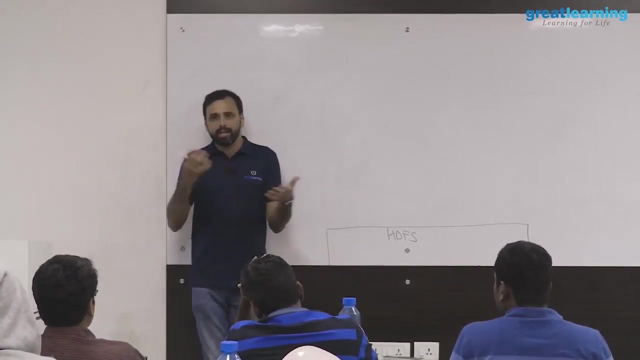 That's something called H-D-F-S. So HDFS stands for Hadoop Distributed File System. Basically, this is the file system which helps Hadoop to store the data. So when you build a Hadoop-plus system, Hadoop cluster, let's say you are using 100 machines. okay, 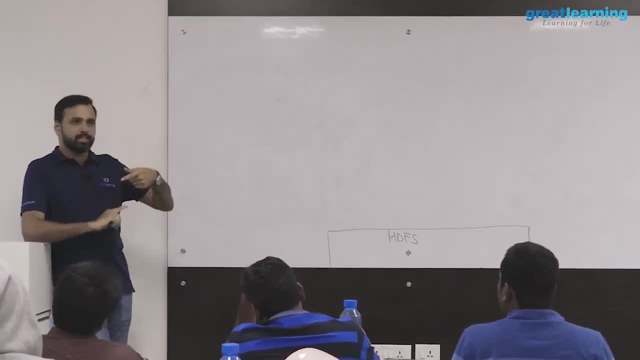 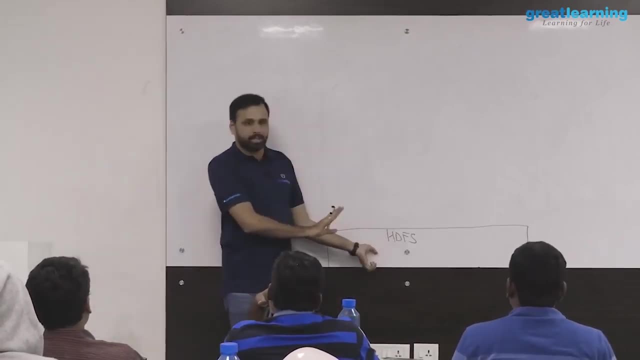 What Hadoop will do. it will combine all these 100 machines into a single file system called HDFS, right? So I'm just drawing HDFS here, just to tell you that Hadoop is there and the storage part is handled by HDFS. 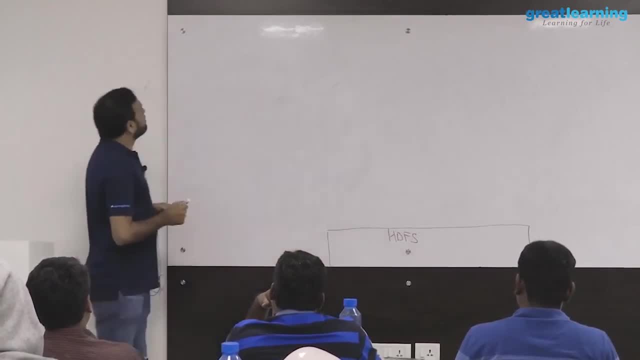 And imagine we have a cluster there. okay, Now, the first challenge we had was that ICICI bank had this core banking. Core banking is where all the transactions are there, you know credit, debit, everything right- And this core banking data was actually in an RDVMS. 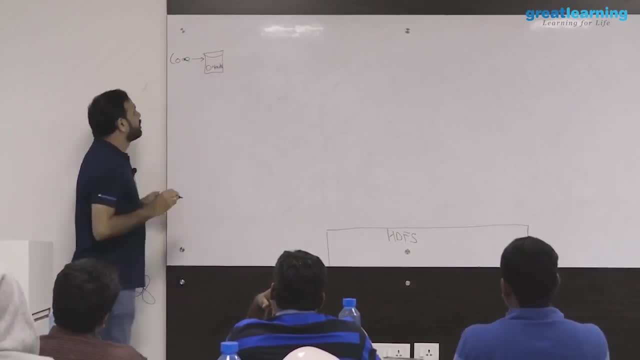 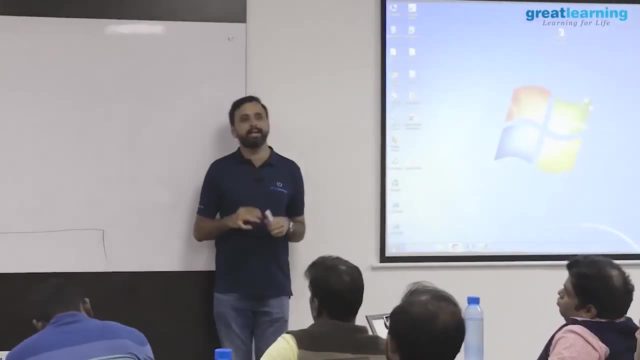 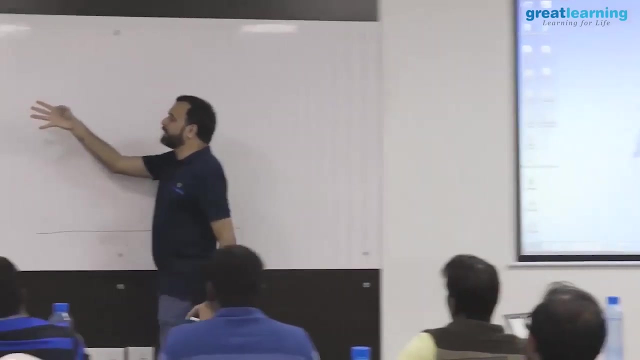 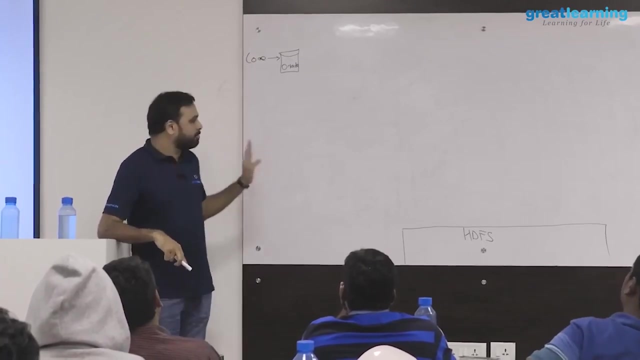 that was Oracle, So they were using Oracle to store all the core banking data and Oracle is very reliable and all you know that right Now, our challenge was that. so they already gave us the backup of this data. We already had the backup, like last month till date backup data and all. 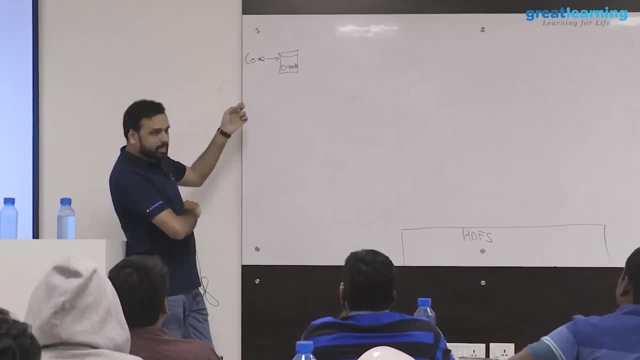 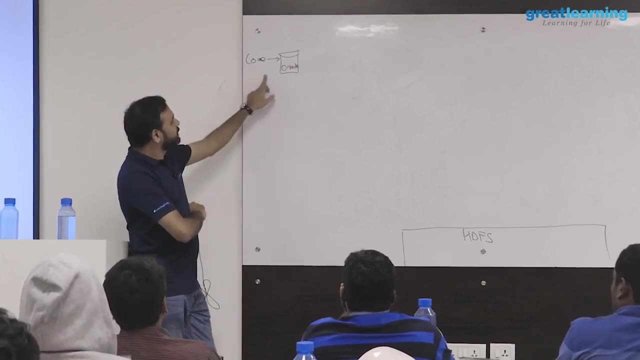 And we copied that to Hadoop. that's not a big deal Of only this, because we had to combine the data. actually, I mean but But don't you have even an algorithm system with them? I was not actually in this part. 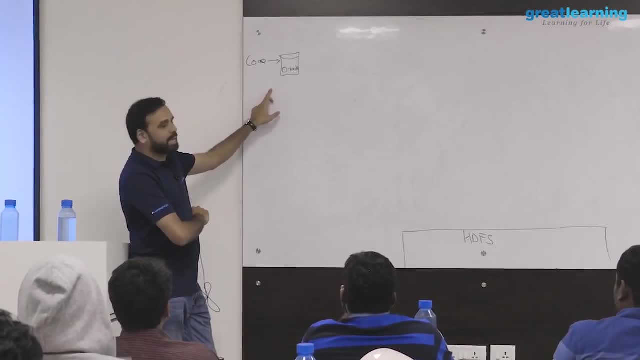 I was not involved in their core banking migration So I didn't know the exact size, but they were migrating There was. so this was done in phases actually because it is a very complicated migration. So this was done in phases actually because it is a very complicated migration. 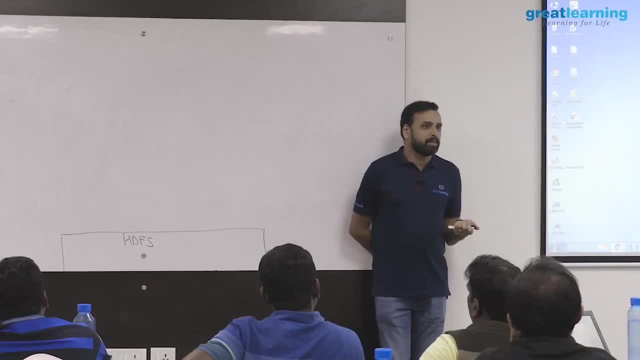 So this was done in phases actually, because it is a very complicated migration, So we had a lot of people working on them And I was actually part of a technique called Kafka. There is somebody called Kafka. I was managing Kafka queues. That was my role. 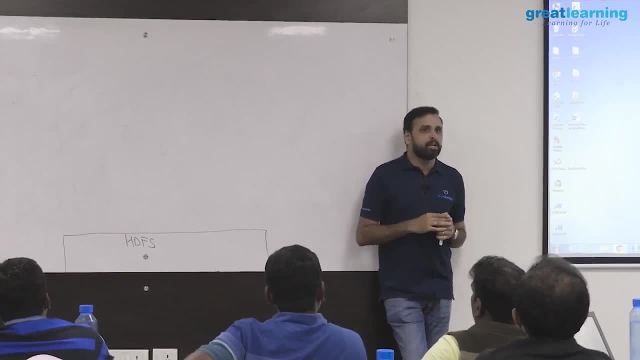 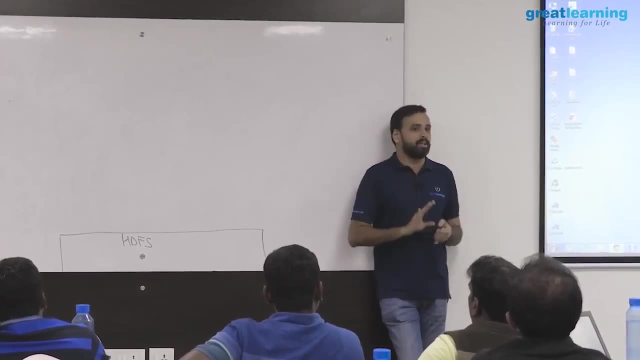 So I don't exactly remember what was their DB size, but the backup was easy, because they will give you the backup, you will copy it, that's done. But then their requirement. they came up with something very weird, What they said. so this migration will happen in a way that 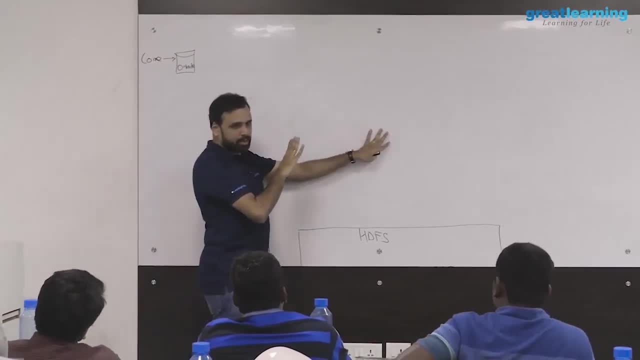 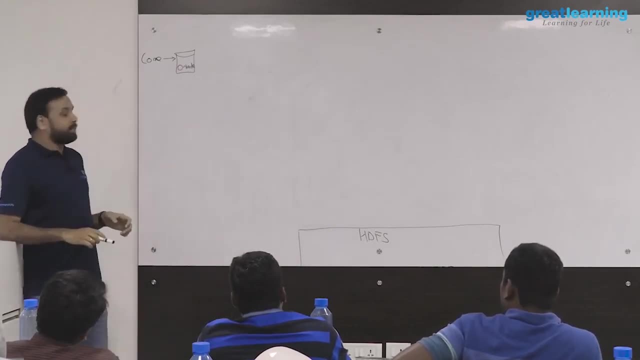 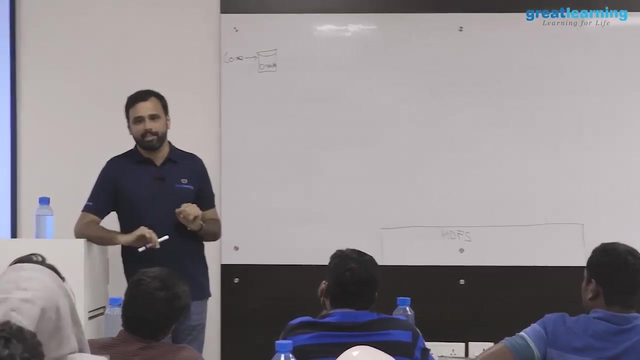 you will migrate all the data from here to Hadoop Right, And this system will remain. Now, one thing you need to understand is that nothing on earth can replace RDBMS in another 100 years or 1000 years, give or take. 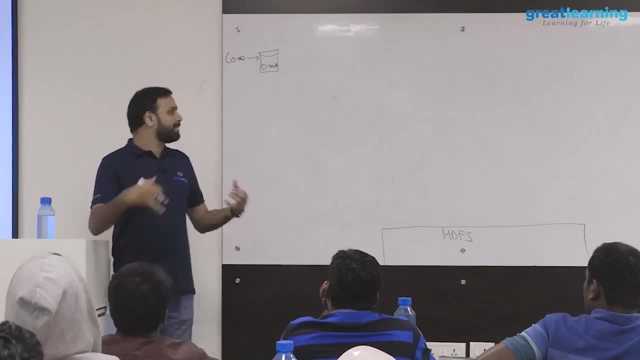 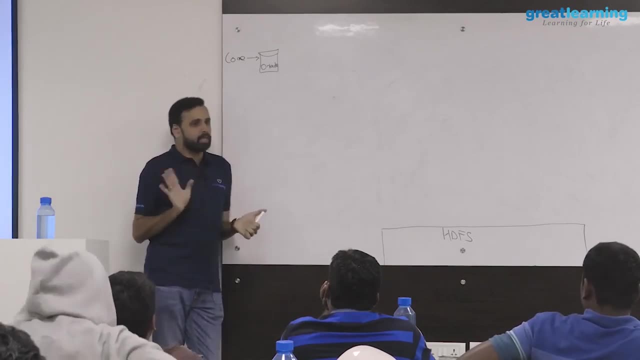 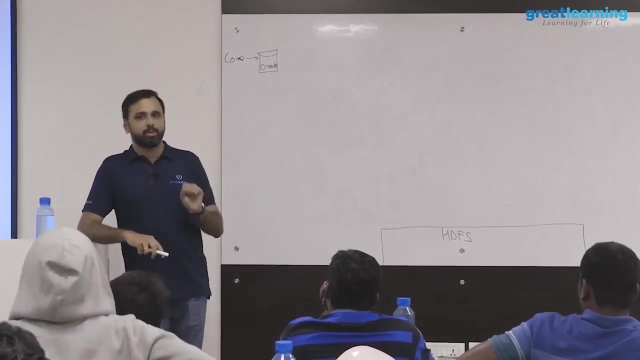 So many people have this question. Okay, so now big data is there and so many other technologies are there, That means RDBMS is losing its significance? No, absolutely not. Nobody can replace RDBMS, Because RDBMS is the only system which gives you consistency. 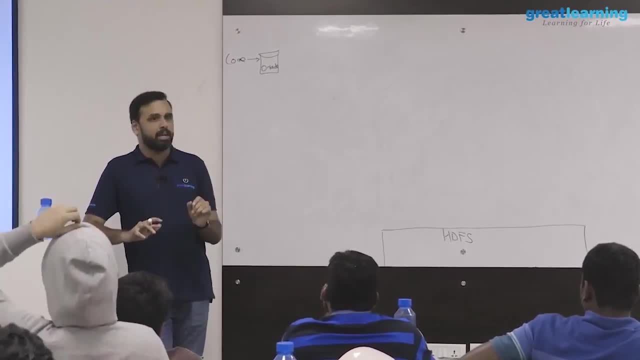 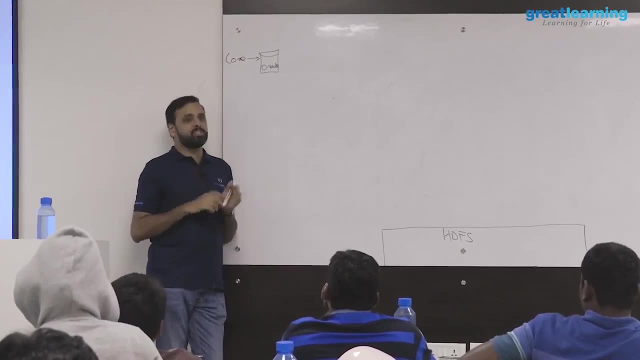 You know what is an RDBMS anyway, right? Acid properties. So for the core banking, still they are using the same or actual DB And nothing can beat it. There is no system on earth which can beat it. But the reason they are still using it because 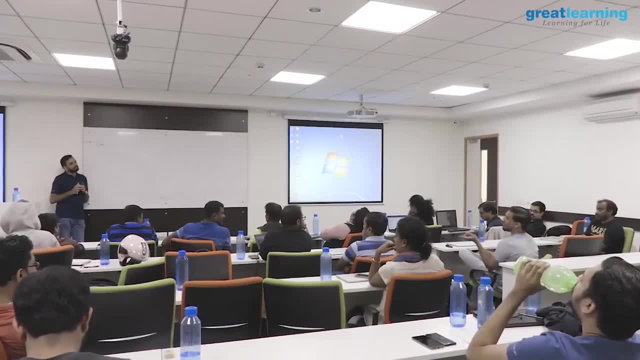 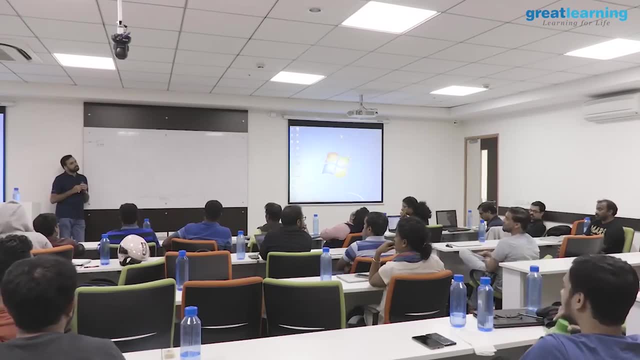 if somebody has to migrate one of the databases, it's law of time and effort and money Fine. But if today somebody creates a new application, they will not choose to use the RDBMS. RDBMS- yeah, That's right. 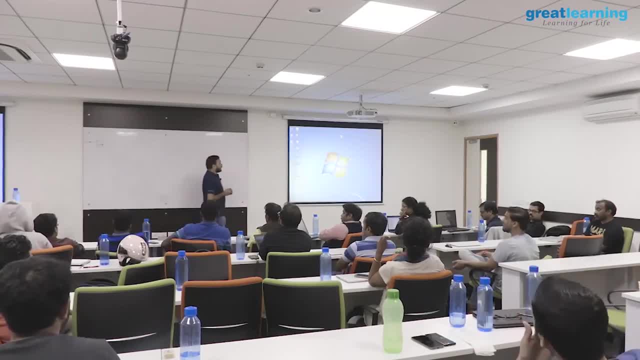 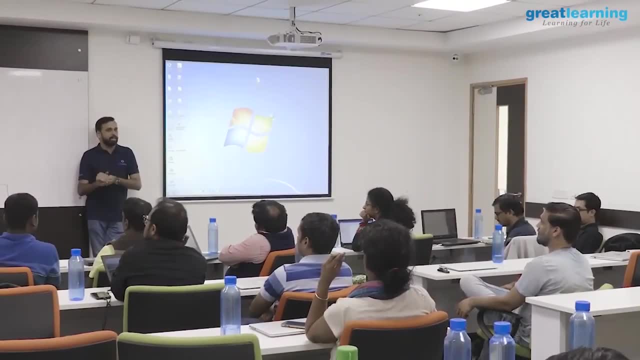 They will use the NoSQL database. There are much more reliable NoSQL databases out there. No, I will come to NoSQL in a moment, But I feel still they will use RDBMS. We will use NoSQL, for sure, But for a different set of aspects. 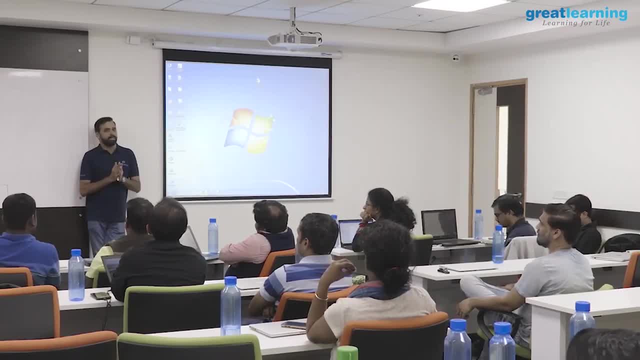 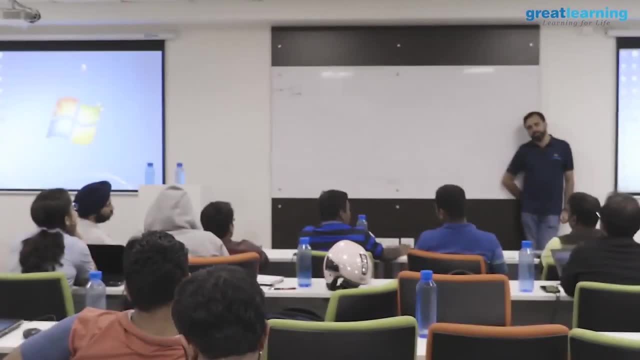 If you are creating, let's say, a financial database, you still prefer RDBMS. Let's say we are moving from HANA. HANA is a node-based database company. They won't provide you database Correct Because of huge volume variables. custom mode. 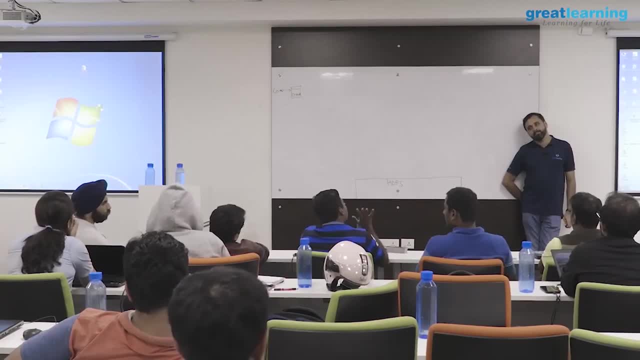 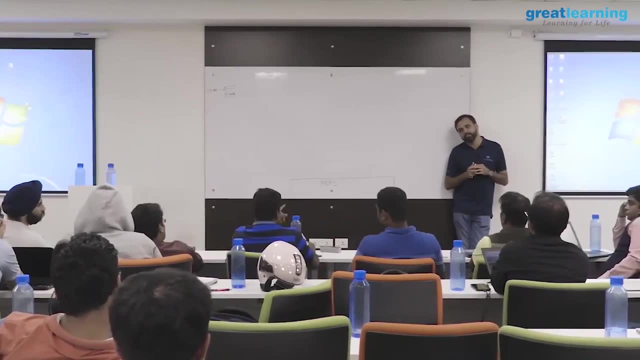 SAP has already moved Even all SAP customers. they are forcing to move to HANA. Right, But HANA is again like normal. what you say table-based database- No, it's not a table-based, It's a clustering-based database. 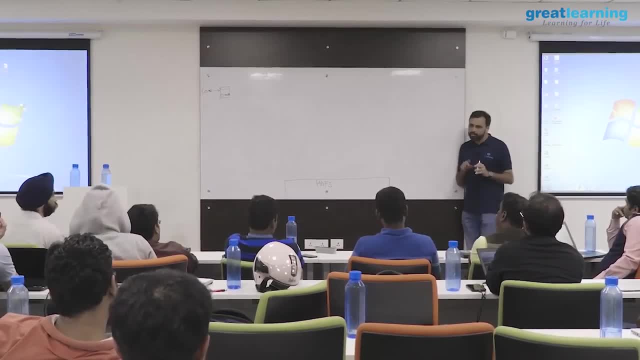 They won't provide you database. Correct Clusters are there, But at the end of the day, you are using SQL only. right? I don't see it. SAP uses their own retrieval procedures from their site. Okay, They write the queries. 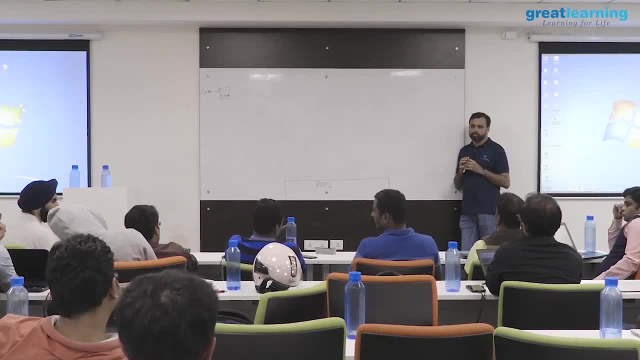 Queries and all. See, the backend will not be open for you. So there is a code name. I mean ABAP. you know right, ABAP, Yeah, similar kind of code position for that. Okay, You can't directly touch the SAP databases. 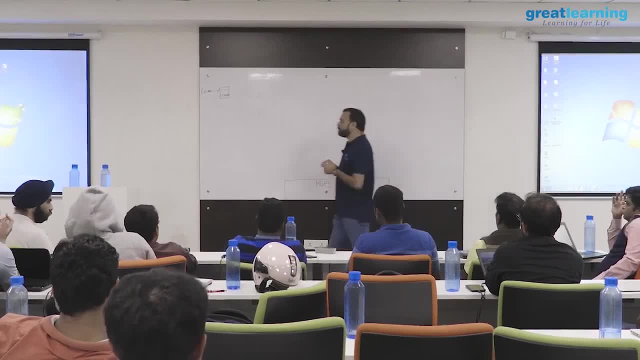 Now my point is: if you look at financial data right In financial data, your problem is with consistency. Right One thing is consistency and all the asset properties: atomicity, consistency and all. And RDBMS is the only system which provides asset properties. 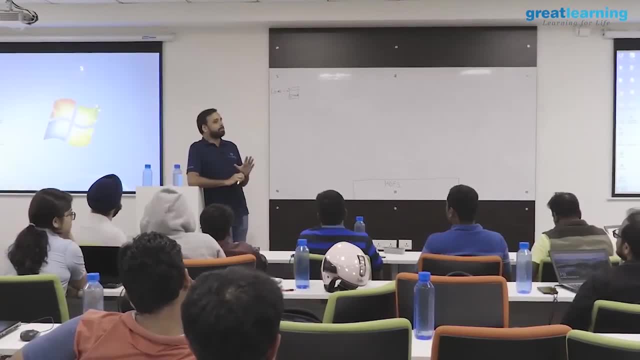 Right, Yes, And RDBMS is the only system which provides asset properties. Right, Yes, And RDBMS is the only system which provides asset properties. Right, Yes, And RDBMS is the only system which provides asset properties. 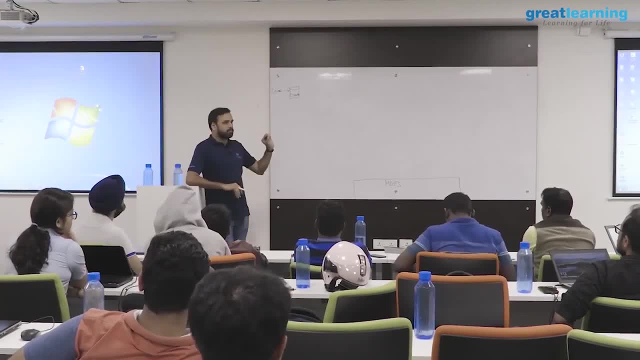 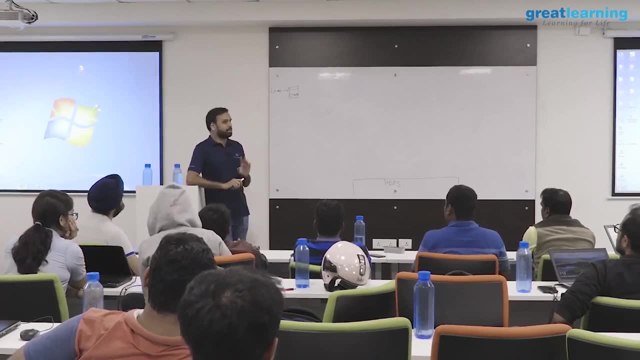 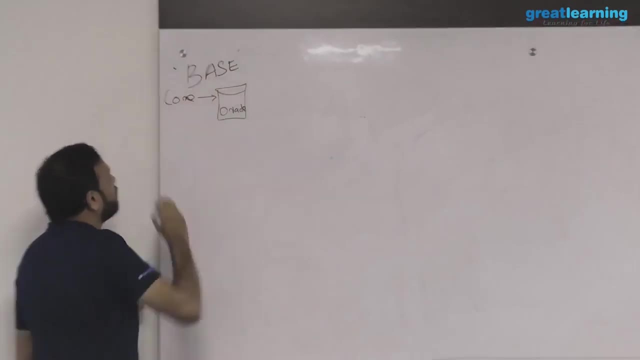 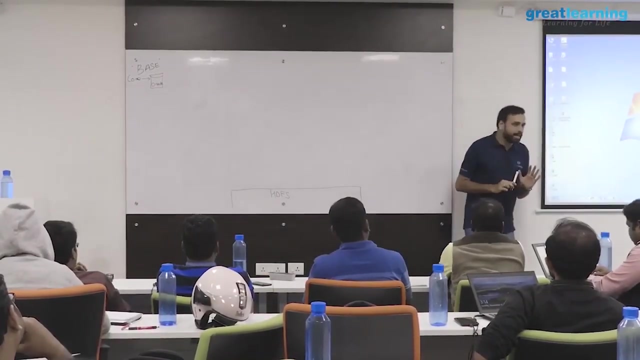 When you go to NoSQL. NoSQL actually does not work on asset properties. There is something called base. NoSQL works on something called base properties. Well, it is different. I mean, NoSQL is also reliable, But if you go to financial side, people don't actually prefer NoSQL. 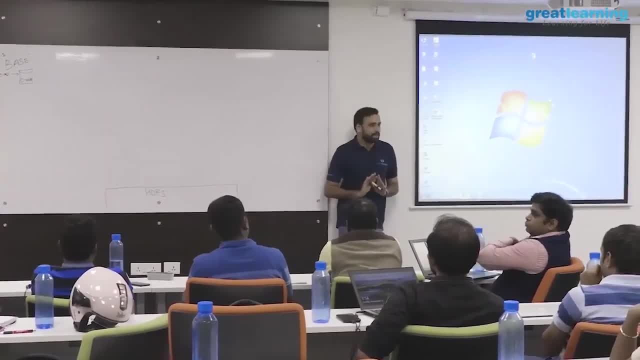 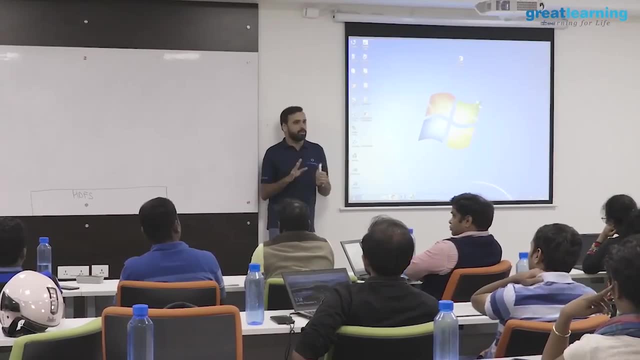 Mostly either RDBMS or not, the pure RDBMS Right, Pure NoSQL that we say, like MongoDB or Cassandra, those things. So ICICI bank and many of the financial customers still use either DB2 or or any of the RDBMS. 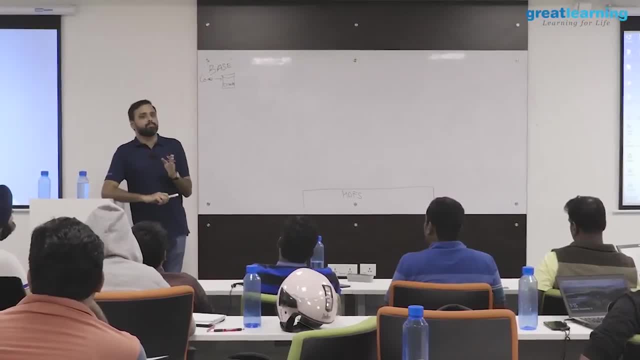 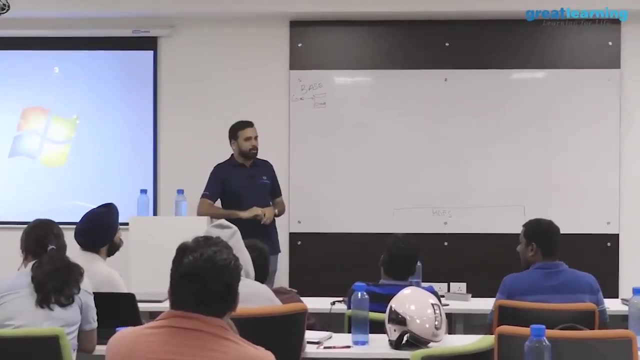 systems. So what they wanted to do. if a customer is again the same situation, swiping his card in a particular merchant, and if the amount is more than a particular amount, he should get an SMS with an offer. say: you bought jewelry for one lakh rupees the moment you swipe. 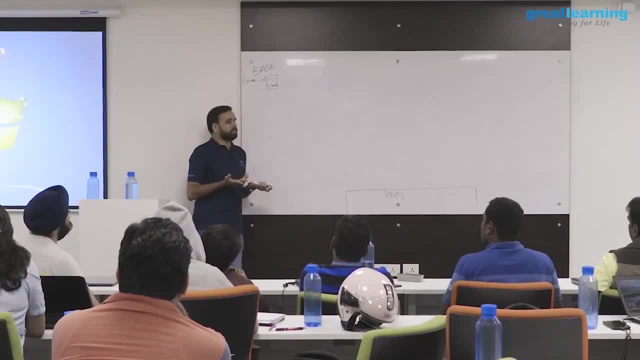 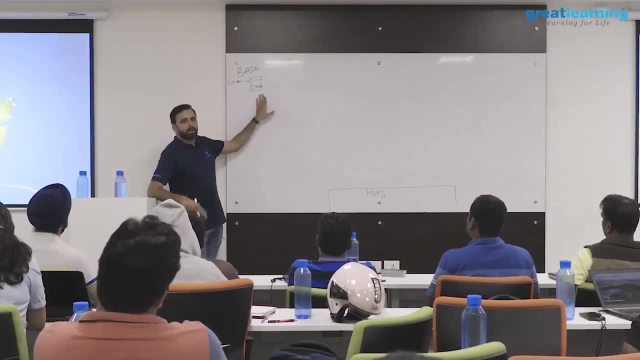 you should get a message. You should get a message saying that again, if you purchase jewelry, you will get 20% or 30% off. That was very new at that point in time. Now, whichever new data comes in Oracle- probably every day midnight or something- we will 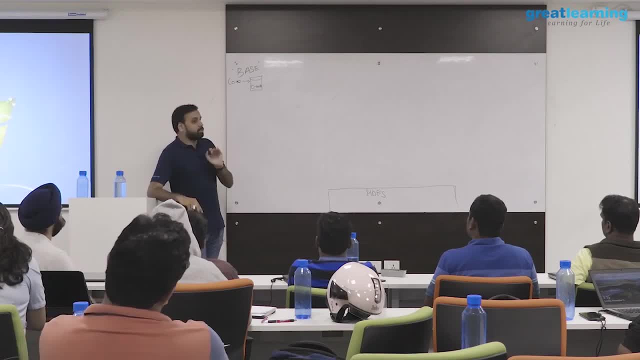 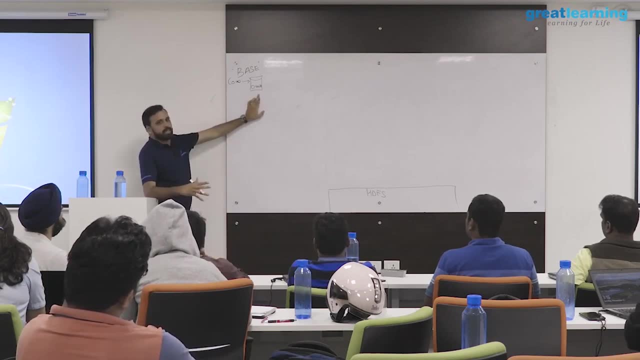 copy the data- Not a big deal. But then the bank said, No, no, that's not our requirement. Whenever there is a transaction happening here using a card- not an online transaction using a card- that transaction has to be captured in real time. 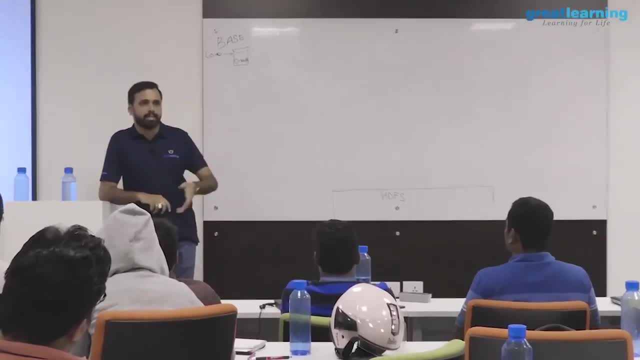 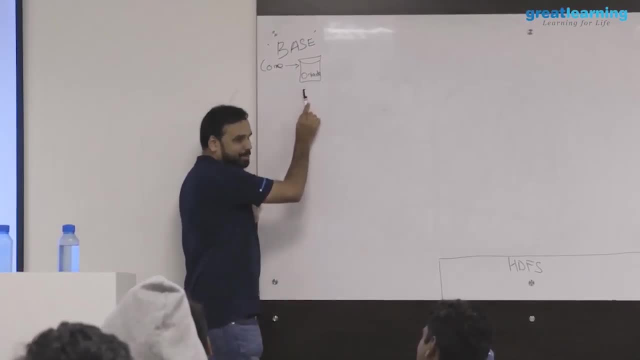 Right, And then a decision has to be made whether you should contact the customer or not contact the customer, etc. Now the problem is this: Oracle is their core banking database And they will not allow you to touch this. Nobody will allow you. 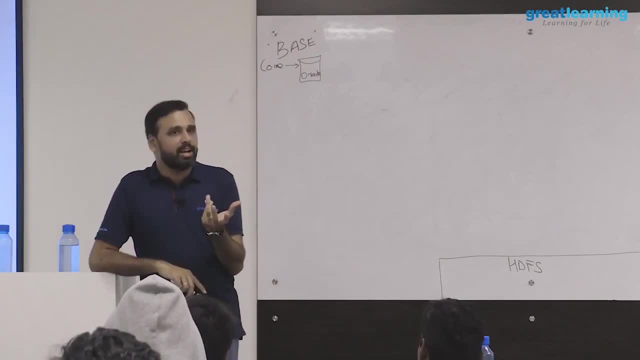 Correct, Because that is their primary database where everything is happening. And we agree the condition that you are migrating to Hadoop and all, but they will never say that okay, we will open our Oracle for you. you can come and do whatever you want. 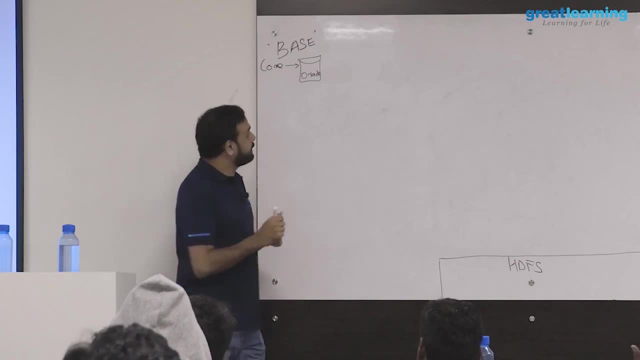 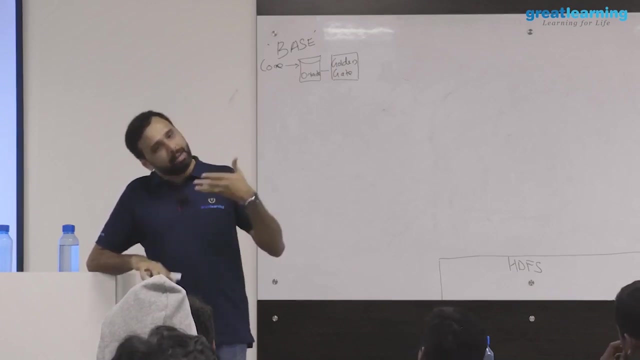 No, So the point is they were using this guy called Golden Gate. You might have heard about it. There is somebody called Golden Gate. Golden Gate is basically sort of like a replication system, that replication management that Oracle does. It is a proprietary product. you pay millions only for Golden Gate, but very reliable. 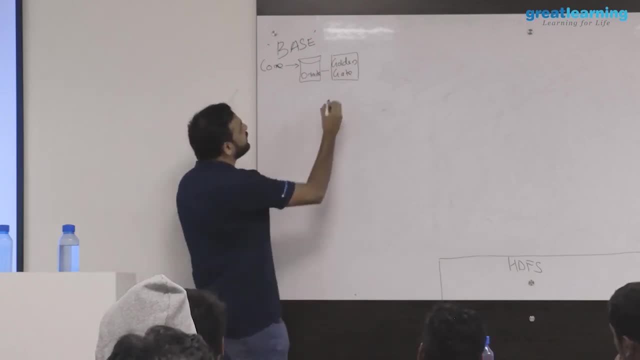 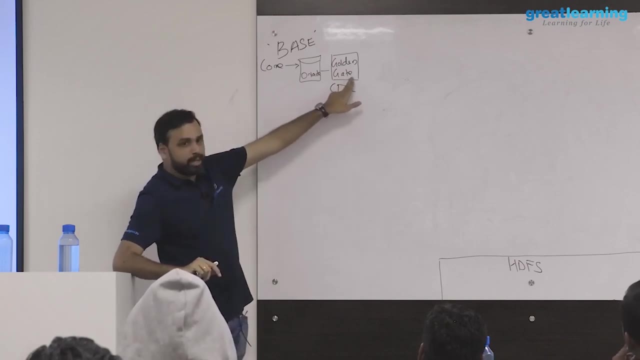 Right, So Golden Gate comes under the category of CDC. have you heard this term change data capture Meaning? what is this Golden Gate doing? If there is any modification in data here, a log file will be created here for that. 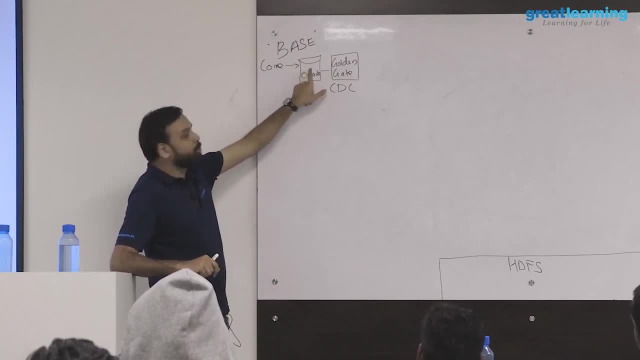 So if somebody wants to understand what is happening here, you go and ask this guy. He will give you a log and if you can read and understand the log, you know what is happening. So if I have the backup and this log file, I know what is the current state of things. 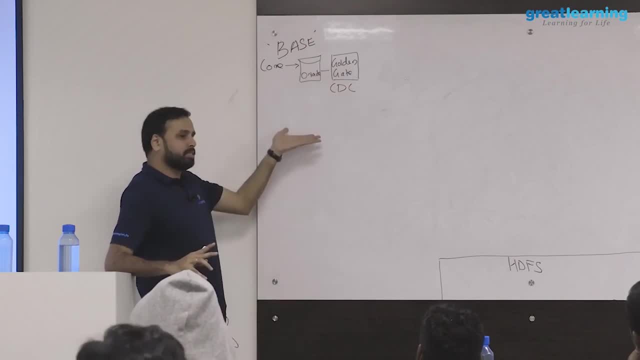 So you have to see this data and then you can use this data to understand what is happening in the current state of the db. And this is very common everywhere. It is not only in this situation, it is very common. Lot of people use cheaper CDC solutions. 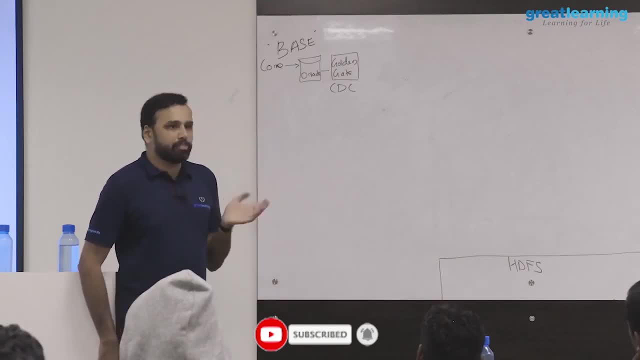 Golden Gate is very costly. In fact GE and others. they use a very cheaper CDC, not Golden Gate. GE uses Green Plum as their data warehouse. Green Plum is their data warehouse and for replication they use- I forgot the tool's name- but it is very cheaper, not like Golden Gate. 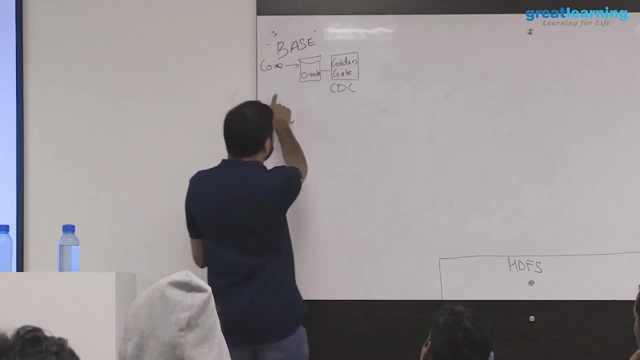 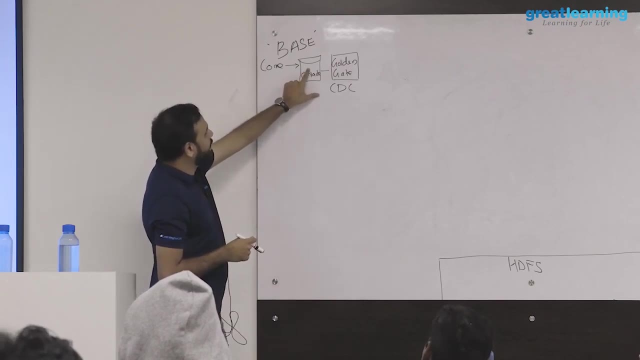 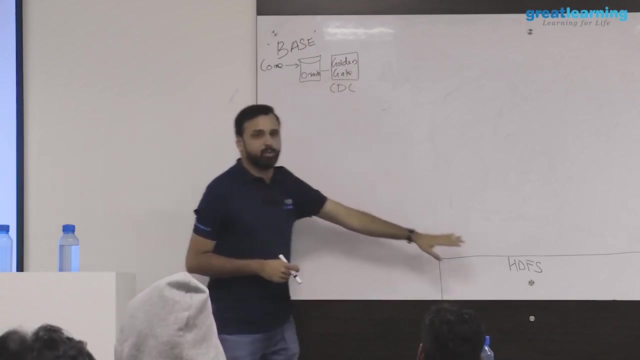 But ICICI bank was actually using Golden Gate and CDC. that means the data warehouse is really efficient. Now, if somebody is swiping their card, the data comes here and immediately. I have a log file here. So I need to figure out a way to get the log file from here to my Hadoop right. 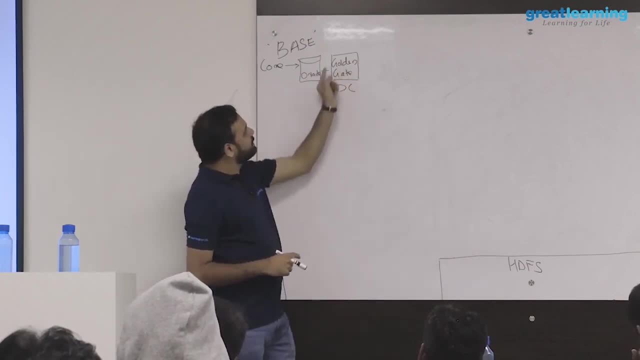 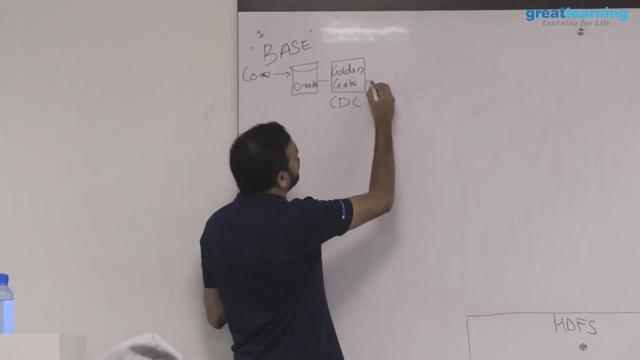 So I need an effective way in which, whenever there is any new log data getting generated here, I need to bring it here. That is where I will be using a tool called Flume. So this is important: Flume, Apache, Flume. so when you discuss Hadoop, it is like you are discussing about a mobile 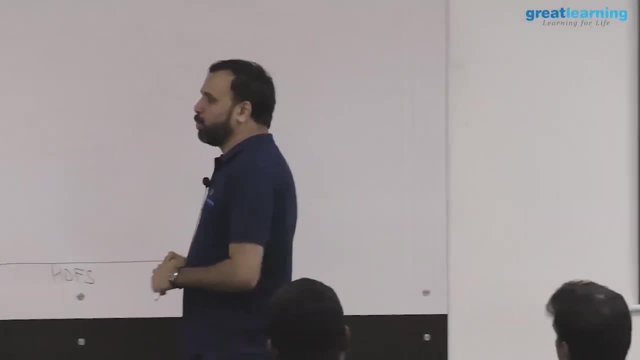 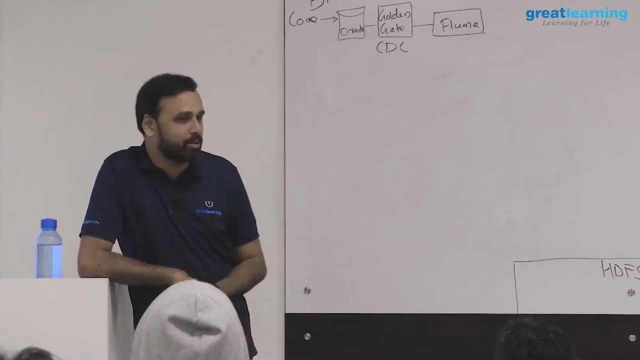 phone. So let us say, somebody comes to you, okay, who was in the jungle for like past 30 years, who has never seen the light of the day, right, He comes to you and say that he looks at your smartphone and he is asking: what is this? 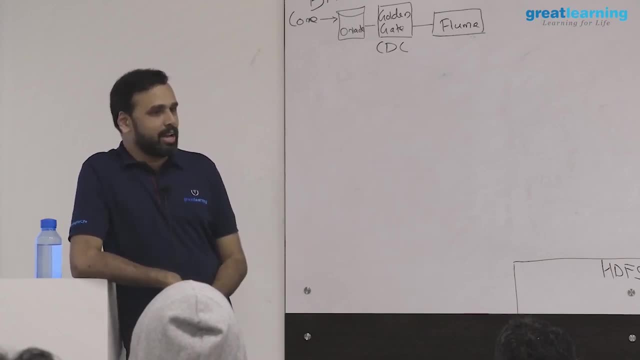 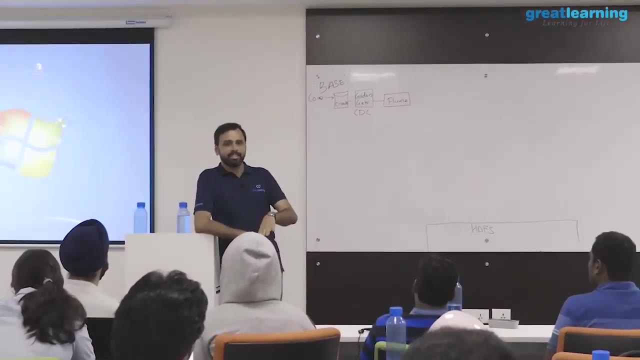 So you will say it is a smartphone, okay. and he will ask- so let us say he is a bit intelligent or something- he is asking on what platform, and all it is right. So he will definitely say it is an Android phone or an Apple phone. but then his next: 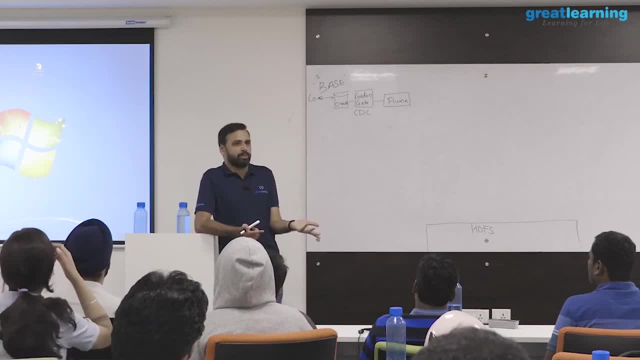 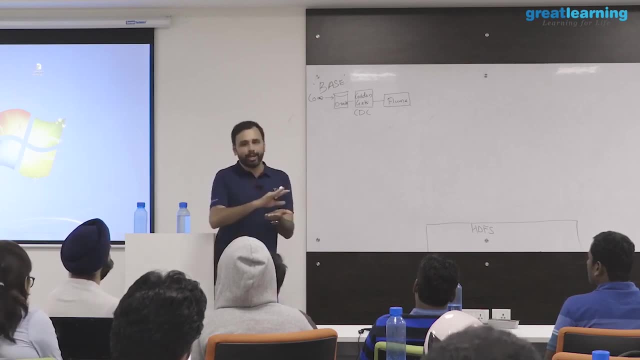 question was: is it just having only Android or Apple? No, So if I look at my phone, let us say I have an Apple iPhone. okay, So Apple iPhone has a platform called iOS, but on the day to day lives, we also use a. 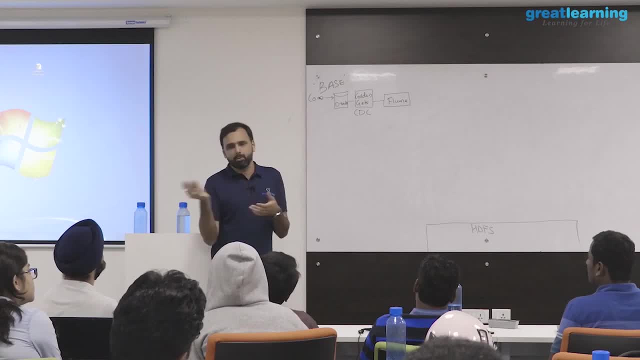 lot of other apps like WhatsApp or Facebook. or to book a cab, you use Hola or Uber. So today, when somebody say a mobile phone, it is a mobile phone. So you will definitely say it is an Android phone or an Apple phone. 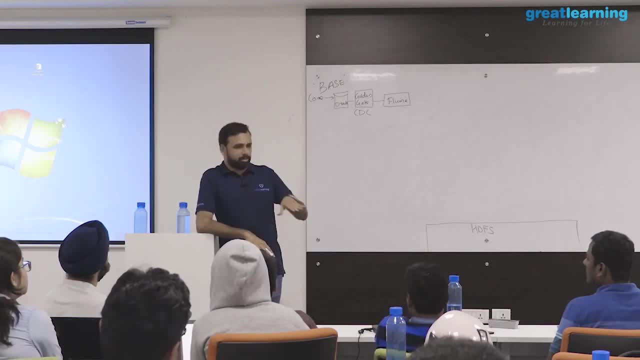 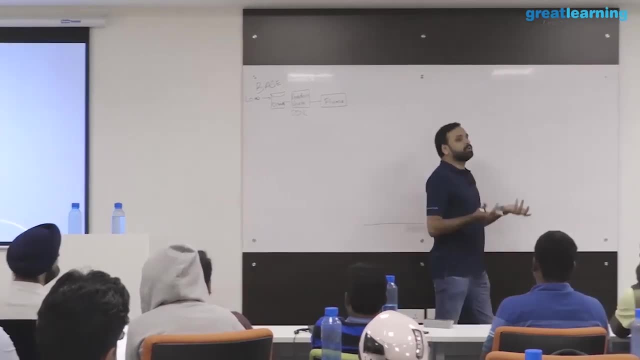 But then his next question was: is it just having only Android or Apple? No, So if I look at my mobile phone, it has a platform and then the apps on top of that. So Hadoop is very similar. Hadoop has a platform where it will allow you to store the data. no doubt about it. 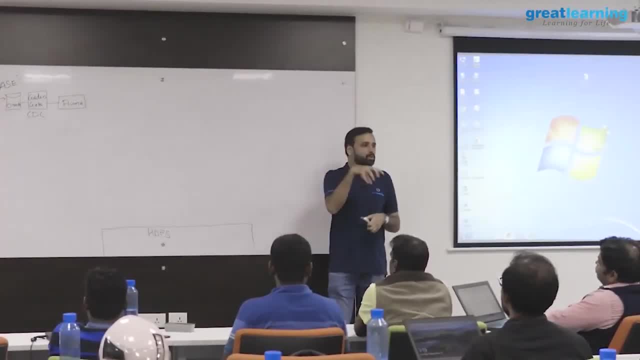 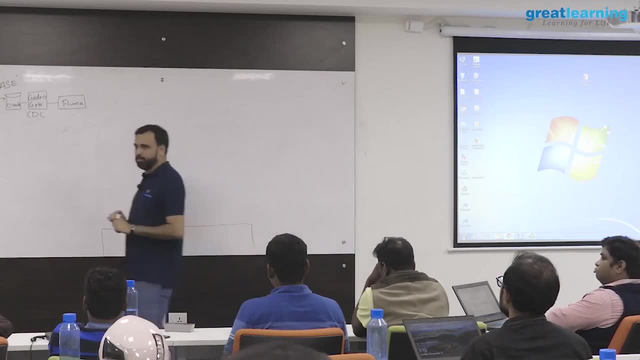 Then it has n number of apps you can use for day to day activities of analyzing and bringing the data. Hadoop alone is not very powerful, because if somebody is using Hadoop only, they are just storing the data and they are not really concerned about analyzing the data. 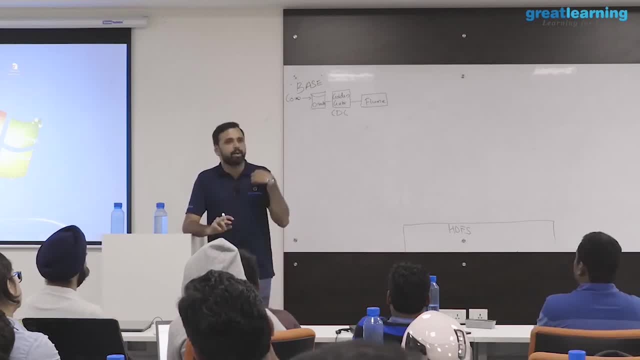 So when you want to feed the data or analyze the data, you need to have a mobile phone. So if you want to feed the data or analyze the data, you use a lot of apps. we can say apps. It is called ecosystem tools technically. 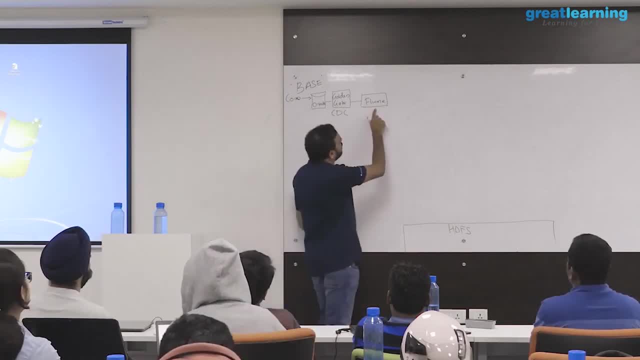 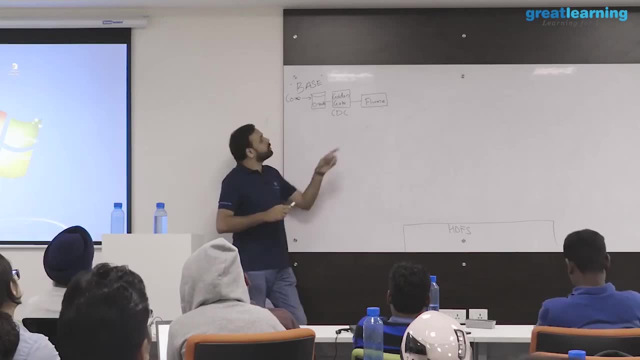 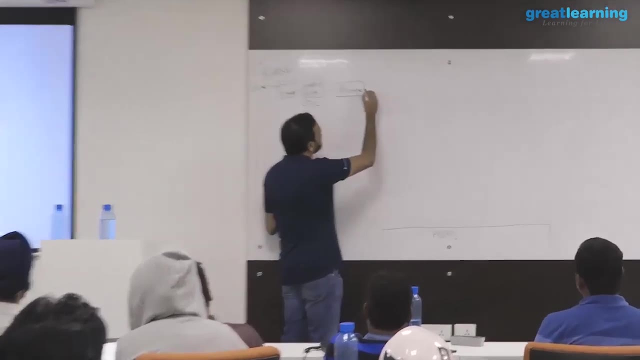 So Flume is one such app or a tool which commonly we find on top of Hadoop. And what is the purpose of Flume? It is used to collect log data from source to destination. So typically if you are using Flume, this guy can take the data and then simply give. 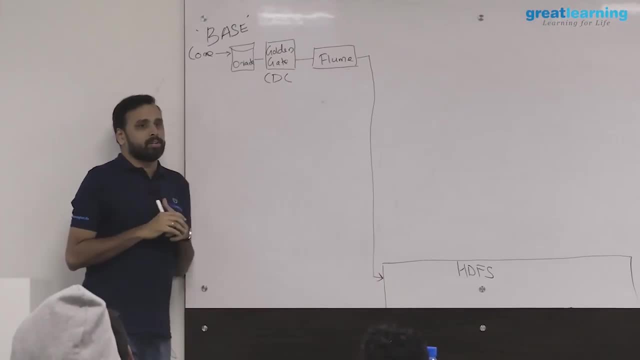 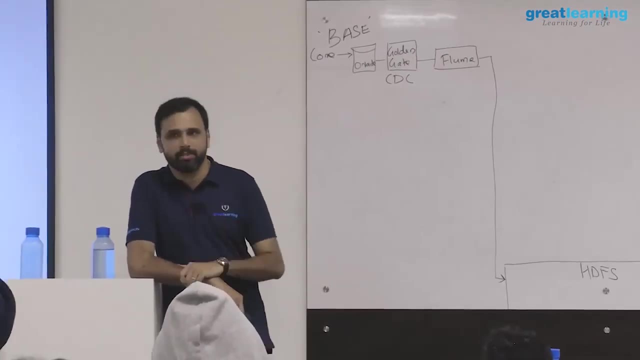 it to Hadoop. So a Flume is an open source project, Apache, even Hadoop is open source. all these are open source products. So no money, nothing free. not 100% is free, but you can say it is free, it is open source. 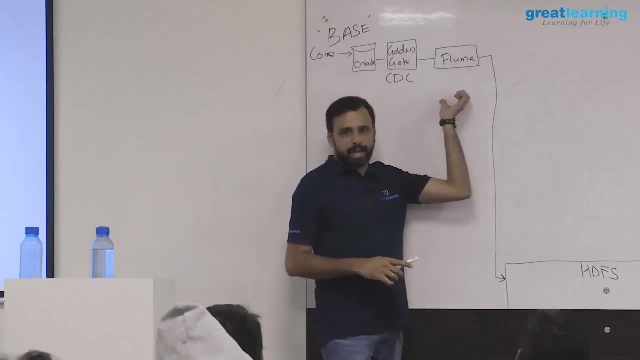 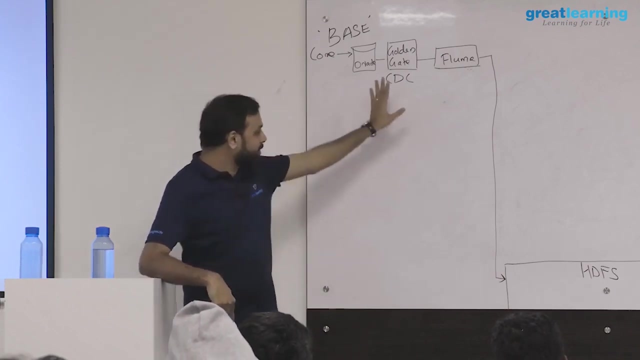 alright. So we implemented Flume so that whenever there is a log file getting generated here, this guy will pull it and he will immediately make it available in Hadoop. But that did not solve the problem. Why? Because my problem was that I don't want to give the data to Hadoop. 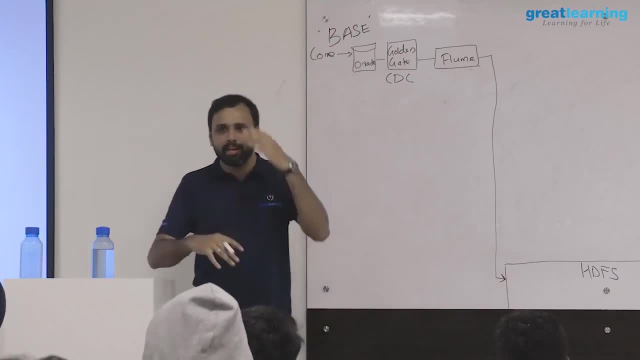 I want to understand whether it is happening in real time And if yes, if this card is for one lakh rupees or something, I want to send an SMS. That is my requirement. So this was not exactly what we did. This is ideally what you can do with Flume. 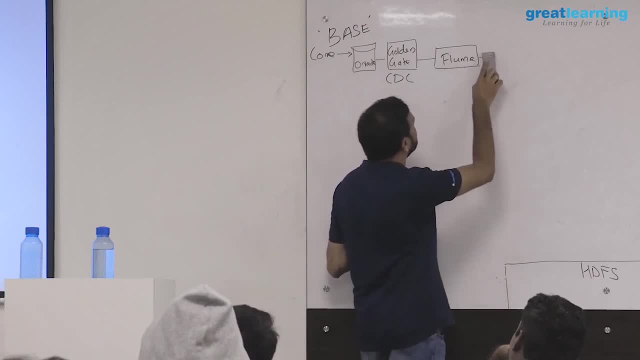 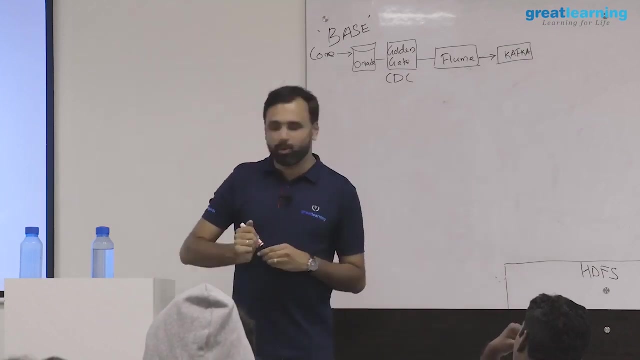 From Flume. what we did? we got the data, We sent the data to somebody called Kafka- Kafka, Another guy. Now I will use a lot of terms, don't worry, So you do not have to be by heart. and like there is no exam where somebody will ask what. 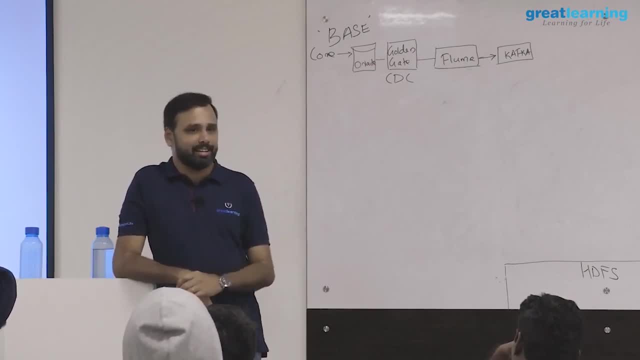 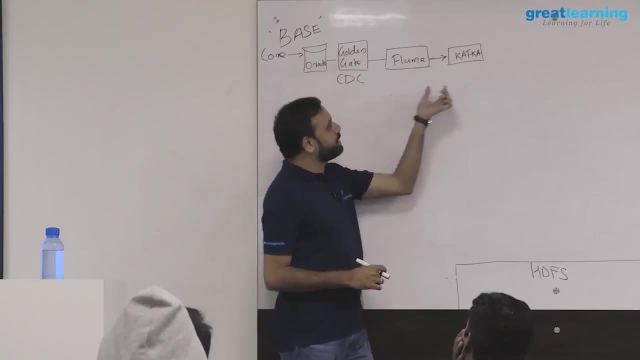 comes after Flume. Is it Kafka or Flavka? So there is nothing like that. So just understand what it is. So, from Flume, what we did, we took the data and sent it to another guy called Kafka. 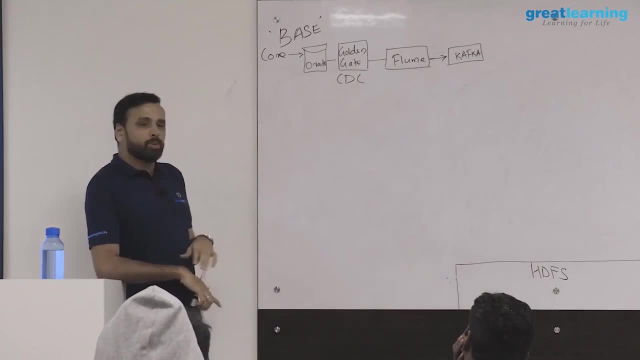 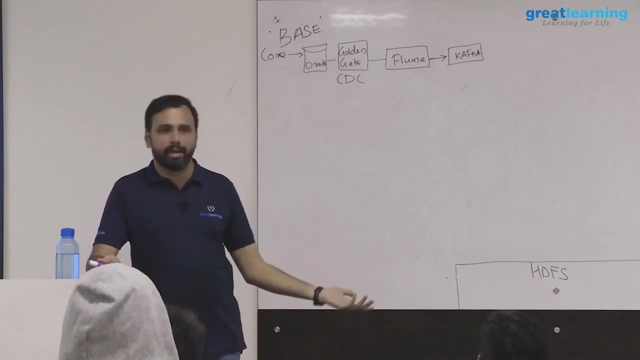 Now, what is this Kafka thing? Kafka is a message queue. Anybody aware of what is a message queue? So when you post something in Facebook, say, 10 people can read it or 10,000 people can read it, as long as it's public to them, right? 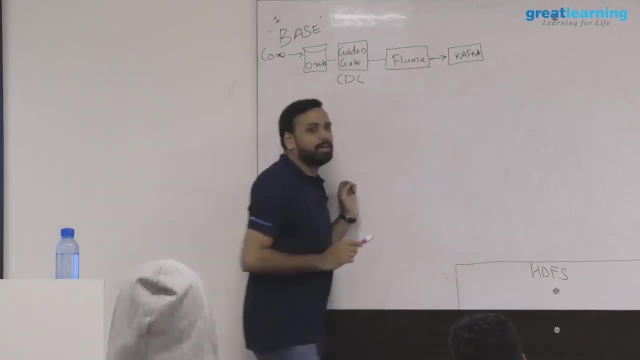 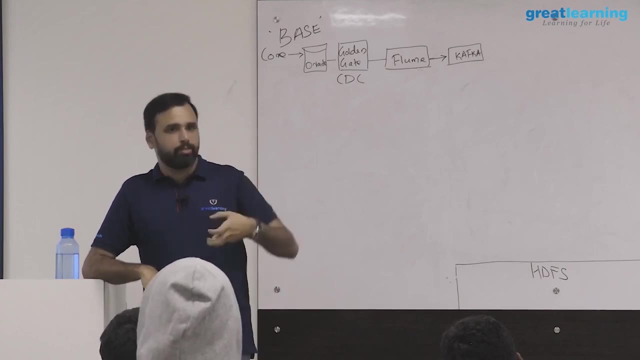 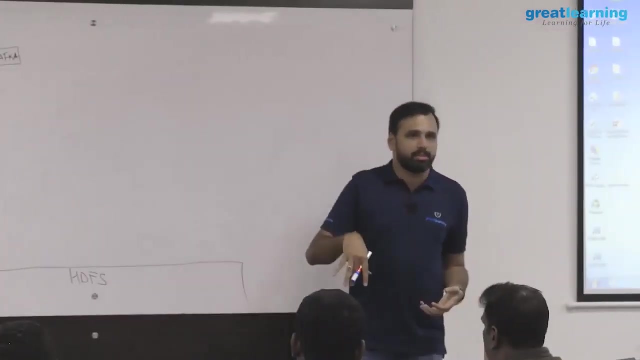 Same way, if I publish my data to Kafka, multiple people can actually read the data from Kafka at the same time. So the industry use case of Kafka is this: So let's say you are having multiple projects in your company. So let's say we split into three groups. 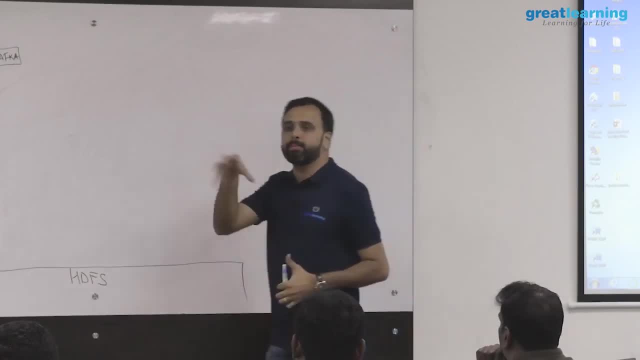 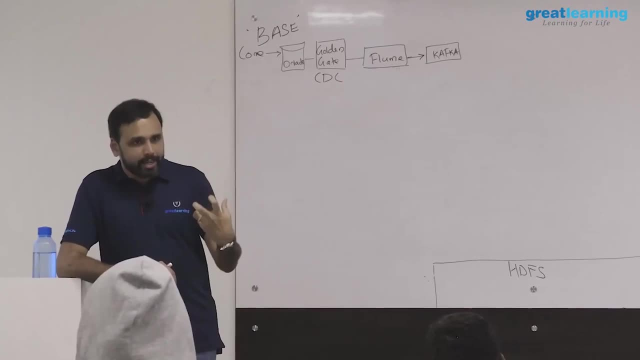 So let's say we are working for a company, right, And there are three projects in the company. All three projects are working on social media data. So what I can do, I can download the social media data and keep it in Kafka. 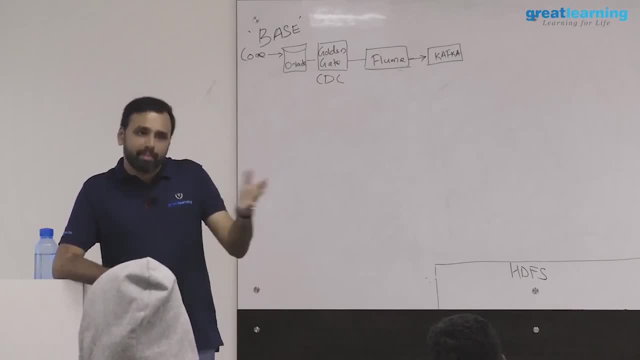 And all of us can connect with Kafka and get the data. So otherwise, what I should do, every team should separately- what you say- connect with social media and get their own data. So Kafka will provide like a common platform. From there anybody can connect and get your data. 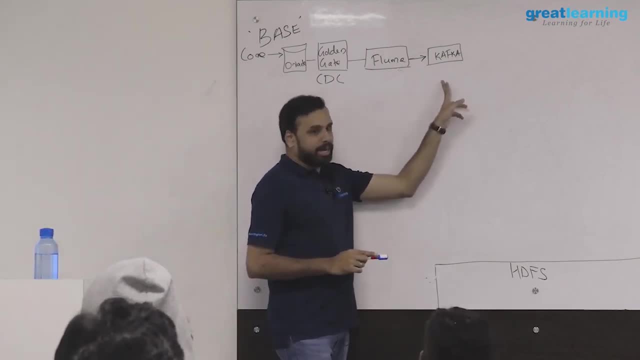 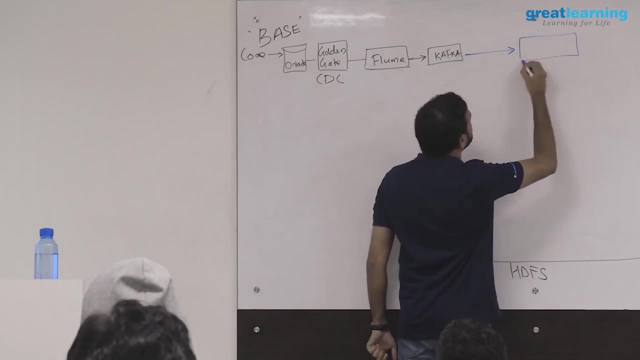 So and Why we were using Kafka, that is a question right? So from FluMetal go to Kafka, from Kafka for doing real-time analysis. we were using something called Spark Streaming. Spark Streaming is the guy who is going to do. 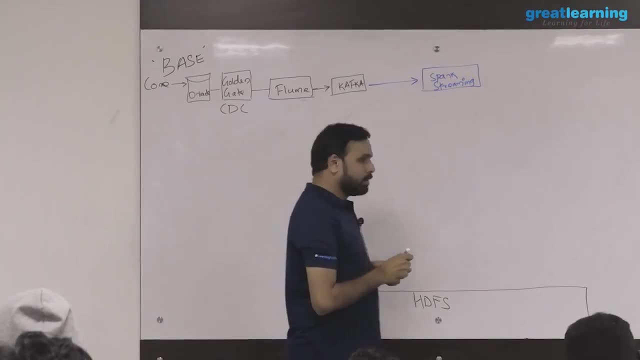 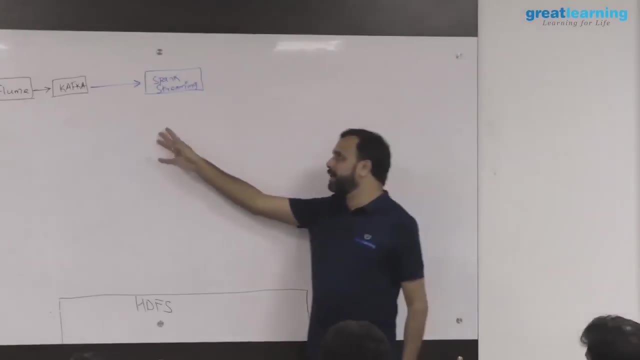 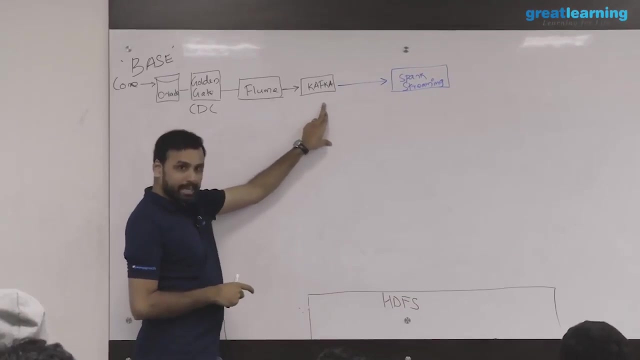 this real-time analysis, Like this guy will read the data and decide you know whether the message has to be sent, not sent. All the analytics is inside something called Spark Streaming Right Now. why I was using Kafka? because once the data is in Kafka, 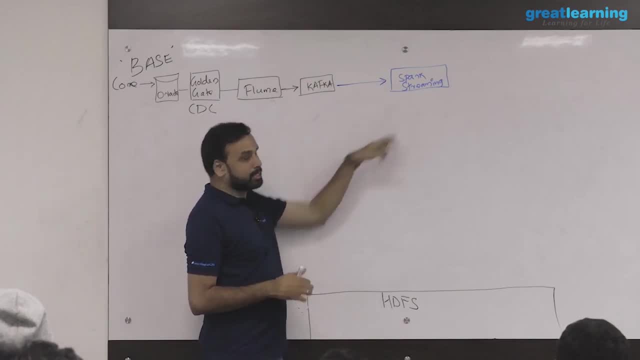 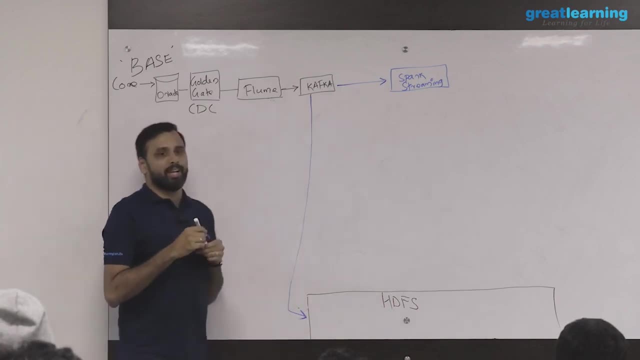 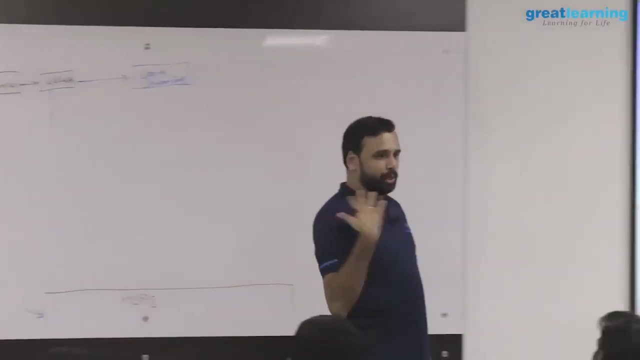 one copy Spark can get to do real-time analytics. Another copy I can send here. that is why I'm using Kafka. Flu is point-to-point delivery. If I'm using Flu, only one Flu- is like you're sending a personal WhatsApp message. 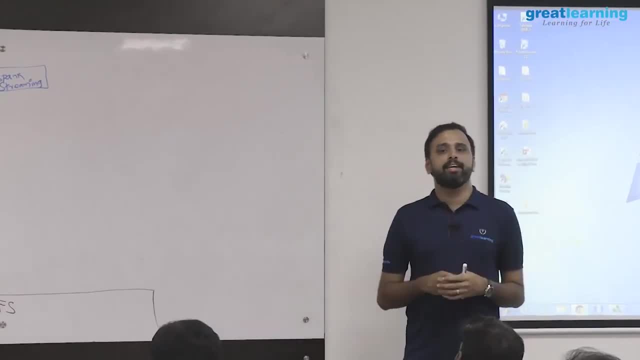 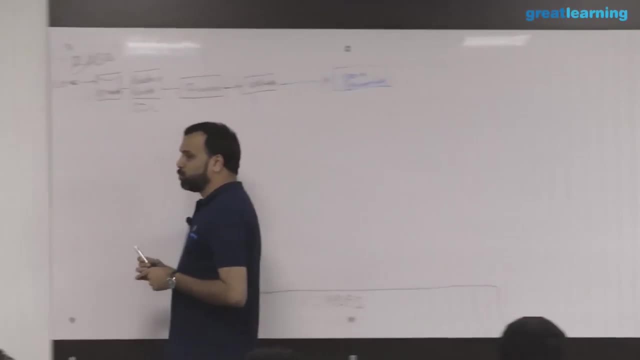 You send it, another person receives it. Kafka is like you're putting something in a Facebook bar: anybody can get it. Also, you are So in future ICICI bank. what they wanted to do? they wanted to build a machine learning model. 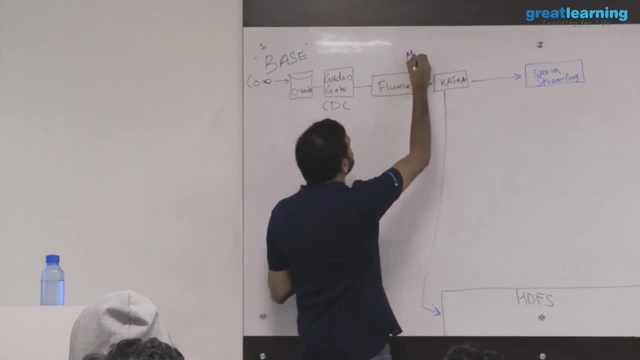 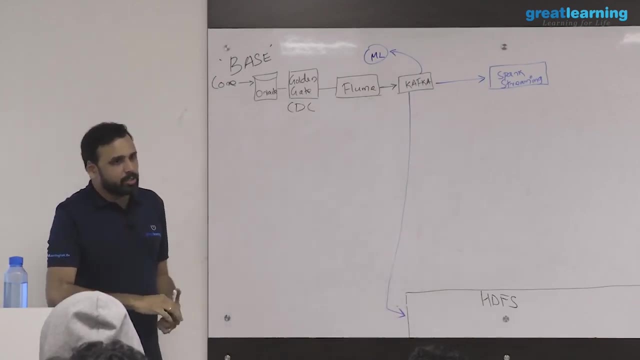 based on this data. So if they're building a machine learning model, the machine learning model also can get the data from Kafka multiple people can consume. So they wanted to expand on this. So that is why they said: from Flume, send to Kafka. okay. 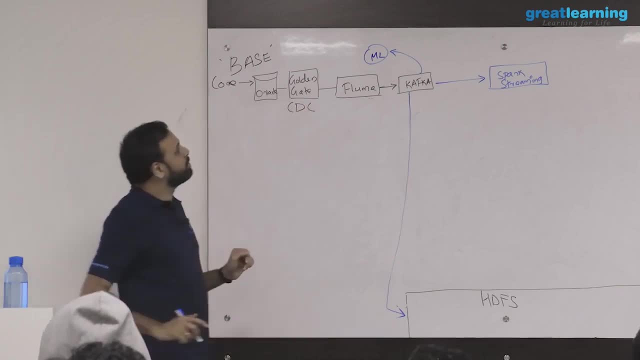 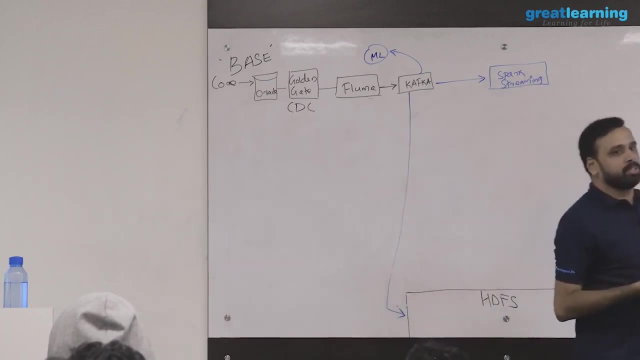 From Kafka. let's say, everybody can consume and get the data. So what we were doing, this will go to Spark streaming. Here all the analysis will happen where somebody should send an SMS, not send an SMS, and Spark streaming will take care of the part. 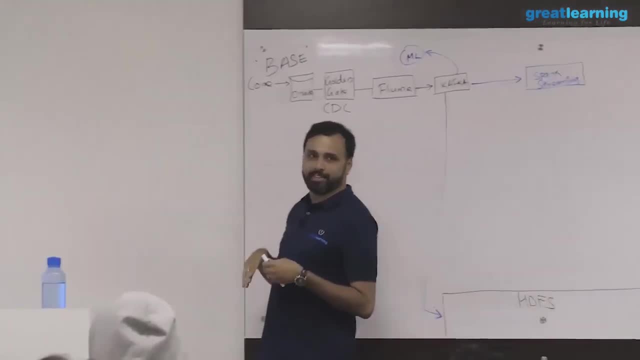 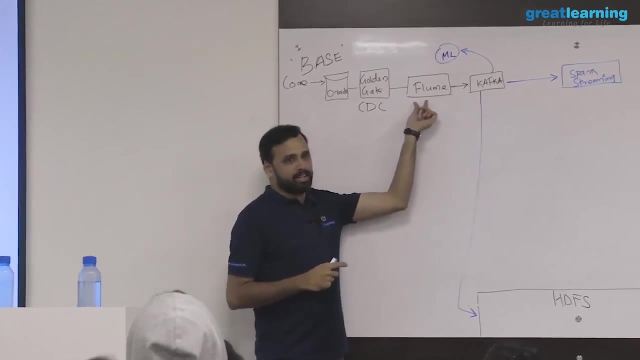 Now the question: if this is so efficient, why are you using Flume right From here? I can directly send to Kafka right. Why do you plug this in the middle Right? that is a question. There is a reason. 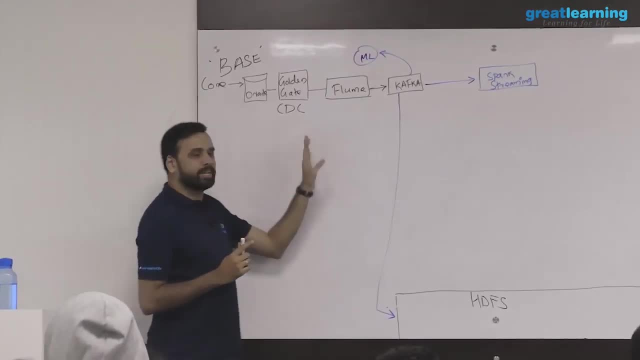 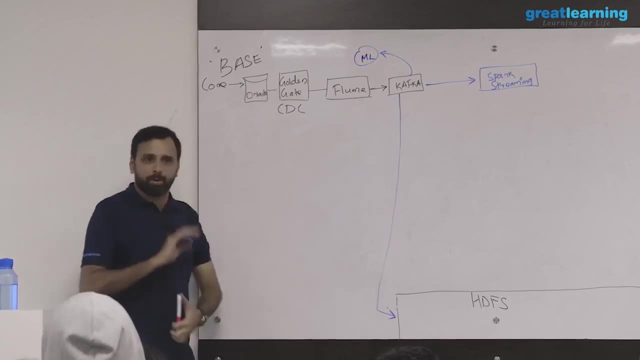 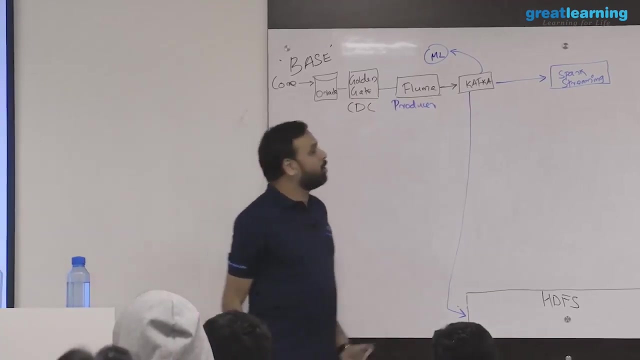 So again, this is in 2012 or 13.. Now the architecture has changed. Kafka is based on something called the push approach, Meaning somebody should push the data to Kafka. It cannot get it, Or in the worst case, or in the worst case. 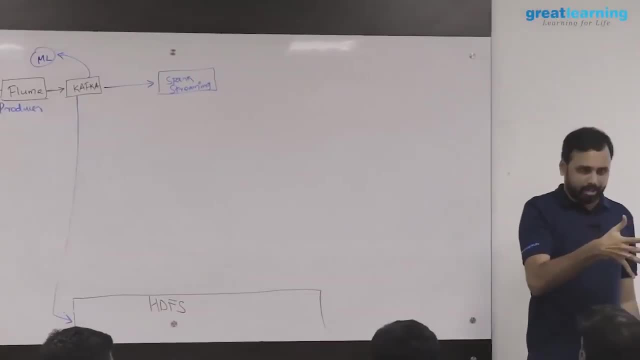 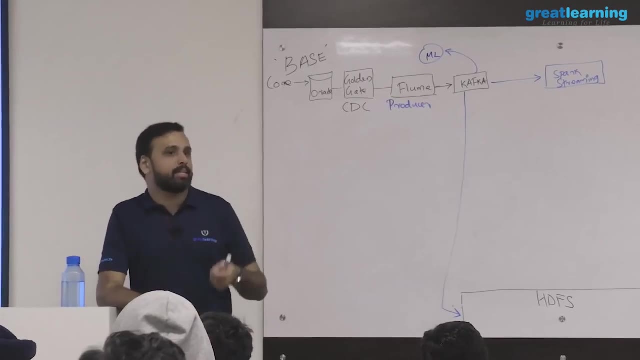 let's say I don't want to use Flume at all, I must stick with Kafka. Then what I need to do? I have to go to this Oracle DB or Oracle GoldenGate, and I have to write a program to push the data, which ICICI then will not allow me to do. 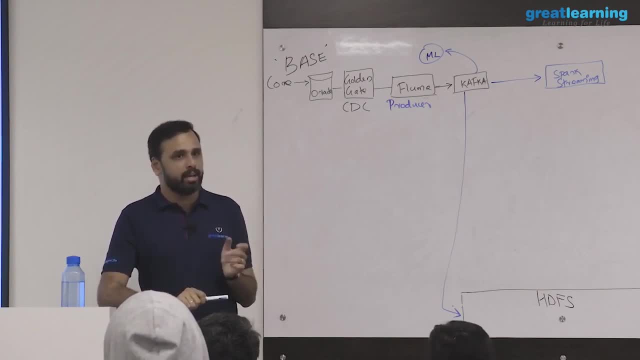 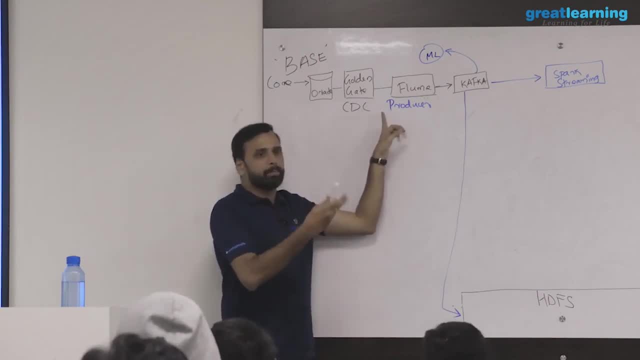 Okay, So Flume is a pool-based approach. Okay So, Flume is a pool-based approach, Which means whenever a log file is getting generated, Flume will automatically pull it. Nobody knows what is happening. Once Flume get it, it will push to Kafka. 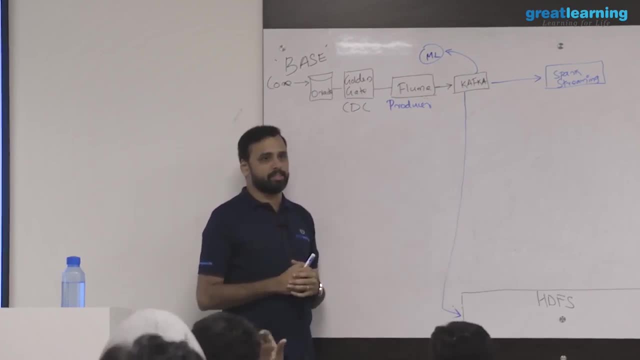 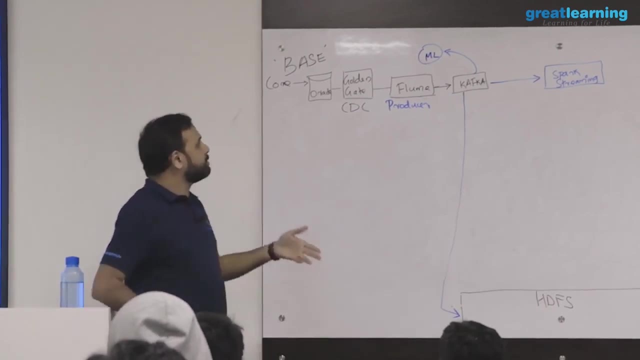 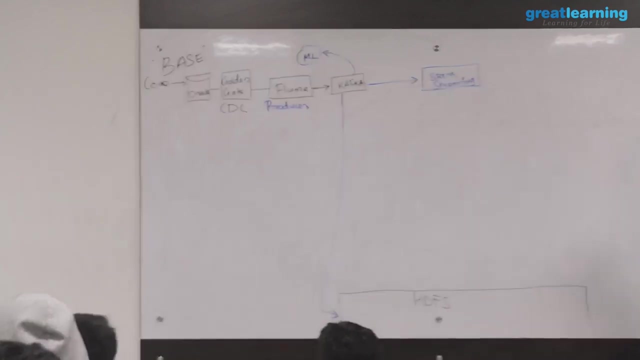 Kafka will get it. Once it is in Kafka, everybody can get it. Now, in the recent changes, like past three, four years, this architecture has changed a lot. In the recent versions of Kafka, Kafka can also pull. now It was not there in 2012,, but the recent versions of Kafka. 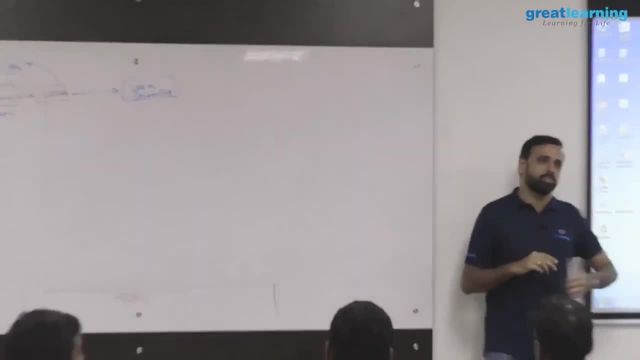 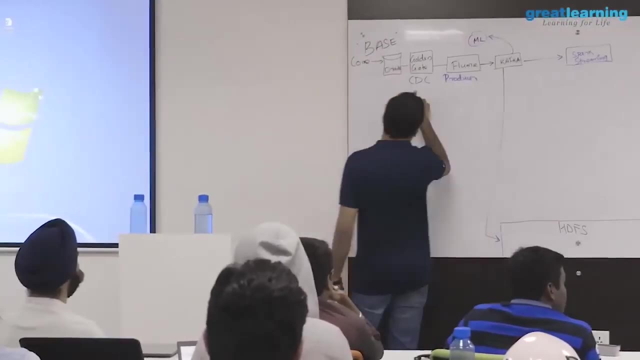 there is something called Kafka Direct where it can pull the data. It is possible to directly pull the data, But yeah, so this was what we were doing. So we were using GoldenGate, then Flume, then Kafka, then it will go to Spark streaming. 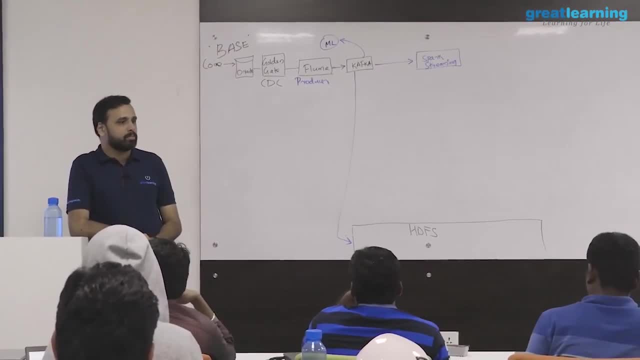 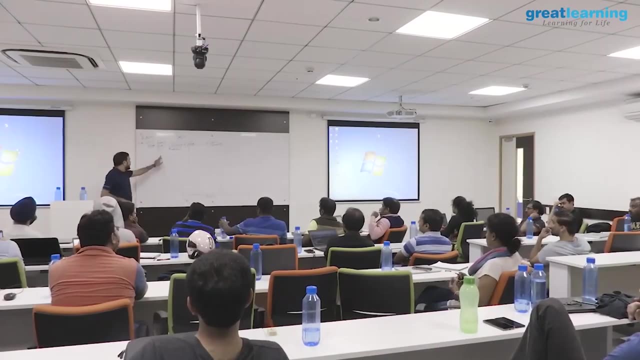 And there the real-time analytics will happen, whatever. So how the data was getting stored in the Hadoop file system, Because the data is coming from the RDB, From GoldenGate. Yeah, Log files, Log files, Text log files. 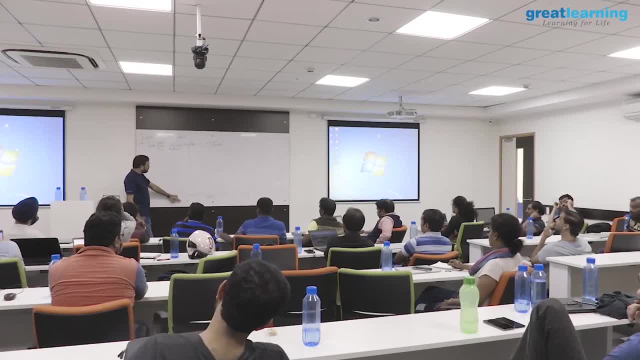 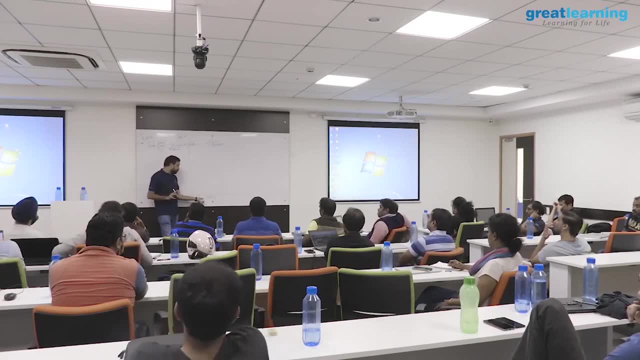 So text log files will go to the Hadoop file system. Yes, yes, yes, yes. And we were doing analytics only on the data. I mean, the bank wanted to do analytics, So they were okay with any format, Because once I have the data in Hadoop, 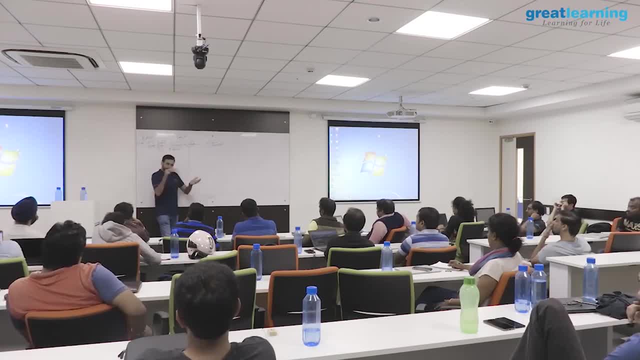 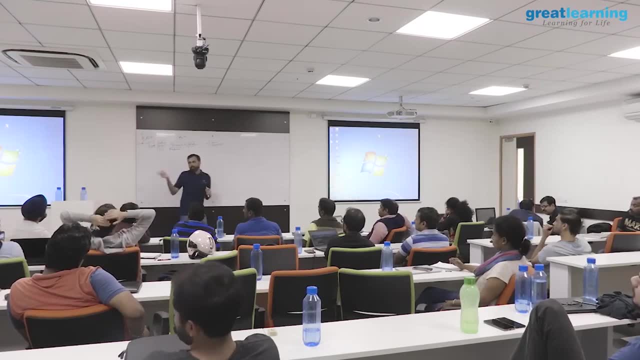 I have different tools which can read the data. So whether the data is in a table format or a text format, I have a way to read it. So they just want the data to be present here. First thing is that Flume is point-to-point delivery. 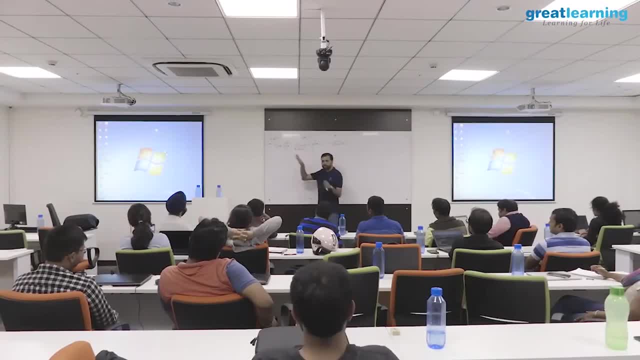 Like it will take data from here to here. It cannot say point-to-multi-point delivery. Second, the difference is Flume is originally pulled back. It is a pull-based approach. I mean you give a source for Flume, it will automatically start pulling the source. 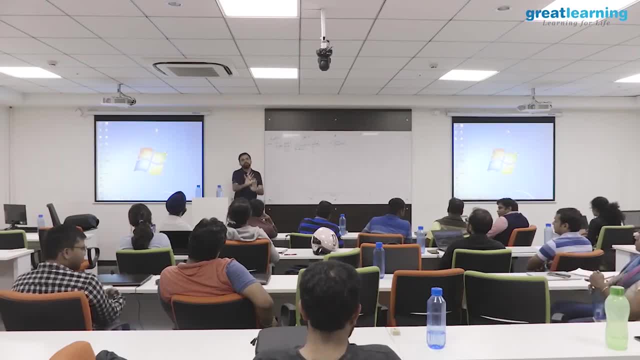 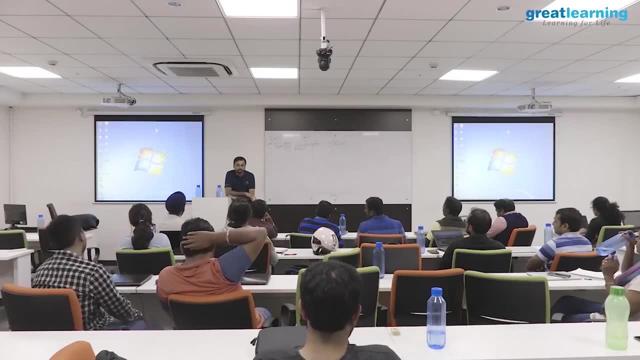 and pulling the data. Kafka is push-based. Somebody should give the data to Kafka. push the data. You need a source which can pull. Kafka is taking pull-based approach, right, Kafka is Taking pull-based approach now. Now it is taking pull-based approach. 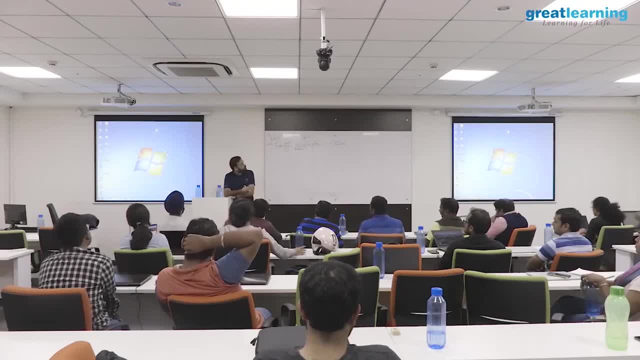 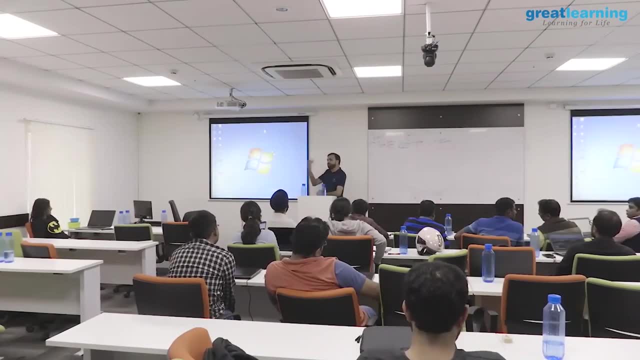 This was Now. it is not using pull-based approach. So now, if I'm building this architecture, I don't need Flume. Kafka can directly pull it. There's something called Kafka Direct, which will actually give me the data directly. I can get the data. 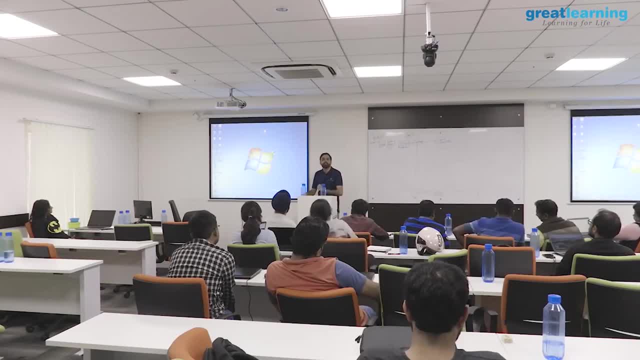 But again, Flume is used a lot these days, So there are situations where you don't need Kafka. For example, my interest is just downloading tweets. Imagine you're building a system where you are downloading data from Twitter- tweet data. I can use Flume. 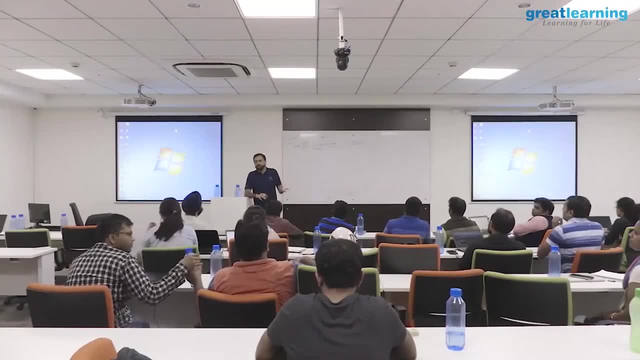 I can say: Flume, connect with Twitter, get me the data. I don't need Kafka. Flume will get the data to Hadoop. Why should I use Kafka? Maybe I only want the data I'm not ready to share. 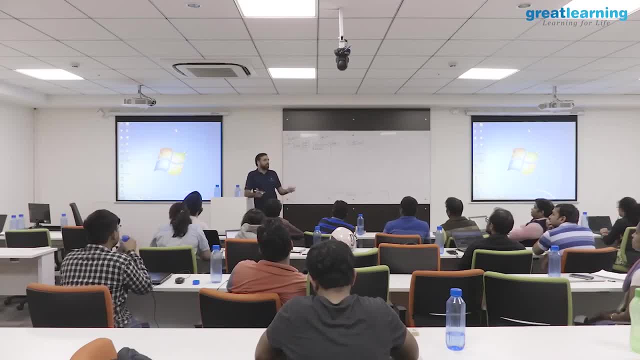 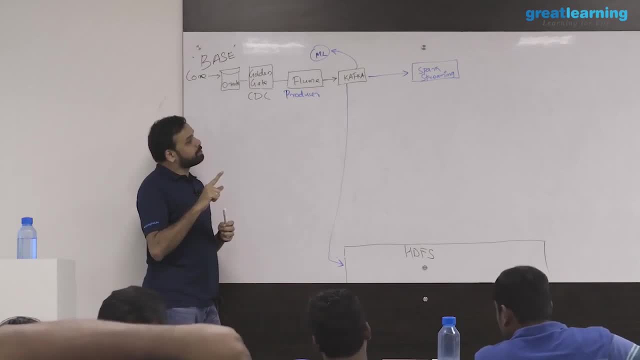 Maybe I'm bad, So I can just say that I use Flume. I don't need Kafka in that place. Yeah, only one input, multiple output. One input, multiple output. Now, Kafka is much more complicated. There is a separate course called Kafka. 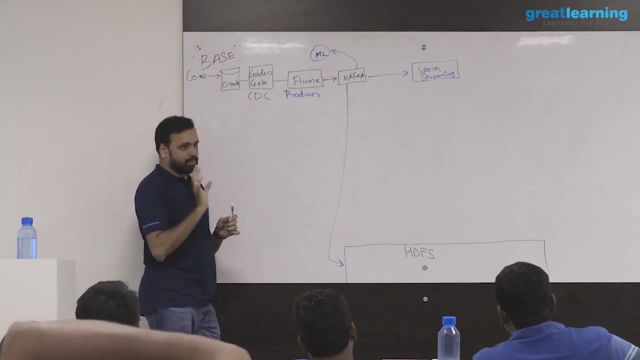 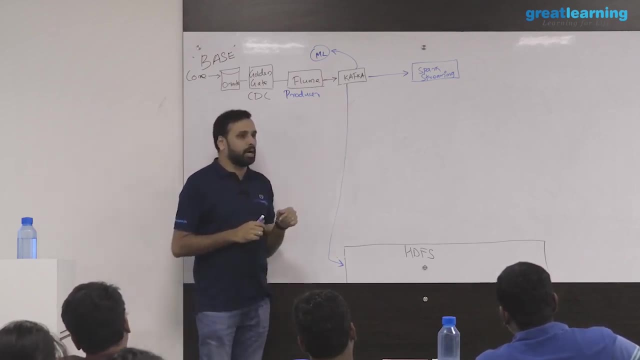 So in Kafka there is something called topic. Topic is like a queue In the same architecture. let's say, somebody else is sending data to Kafka. How do you know the difference? This data is coming, that data. So you'll create something called a topic. 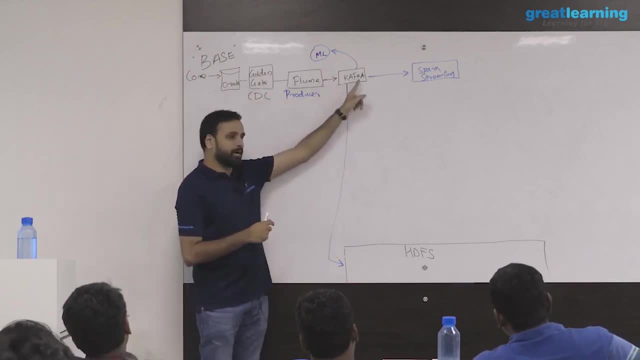 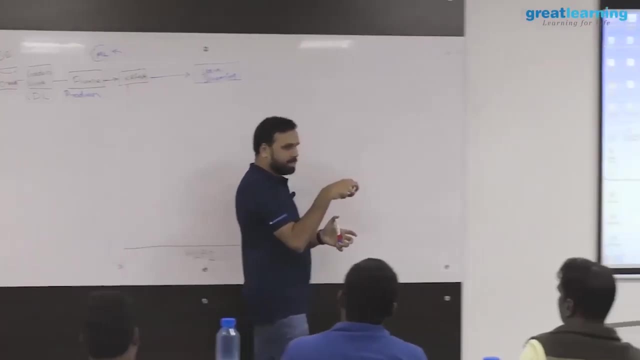 That's like a queue. So if this guy is sending the data, you will say topic one, It will end in topic one. Someone else wants to send, you create topic two, So that will be identified. Okay, so this guy is sending the data. 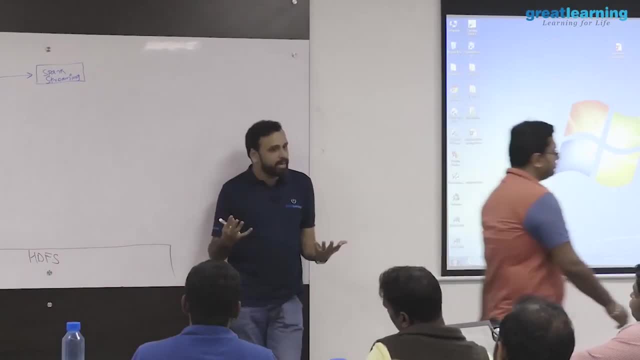 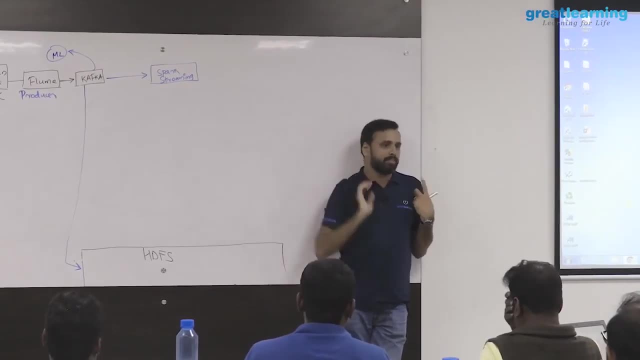 That's in queue one, this is queue two. And then whoever wants to consume the data they subscribe to that queue. I will say: give me all the data from queue one. I know queue one is coming from this side. I will get the data. 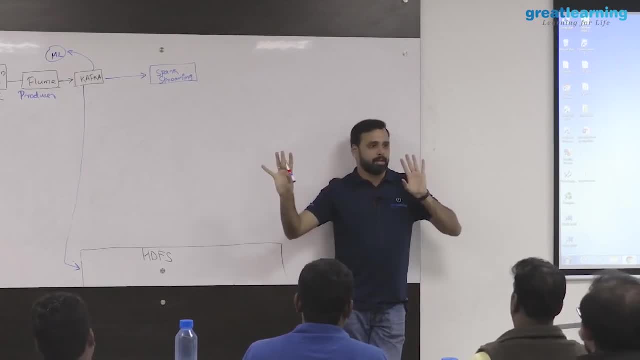 So it is called a producer-subscriber model. Producers are the guys who will produce the data. Subscribers are the guys who will come in. They will connect and say: give me the data. Kafka will hold it in the middle And typically when you install Kafka in a Hadoop, 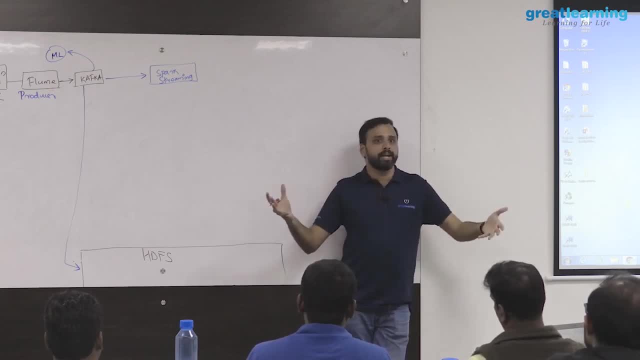 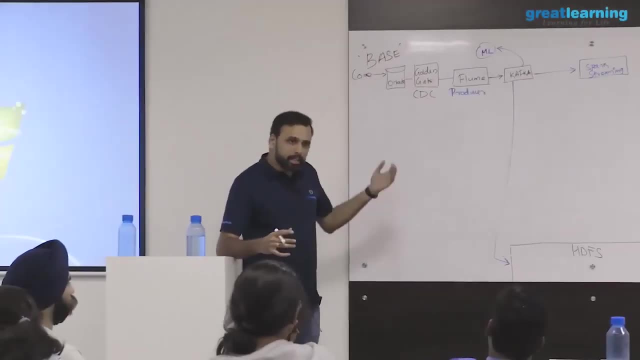 it is installed in a cluster, not one machine, Because it needs to hold this data. You can't predict how many data will come And some of the people will say: I want to hold the data for seven days. So if seven days the data keeps on coming, it has to hold. 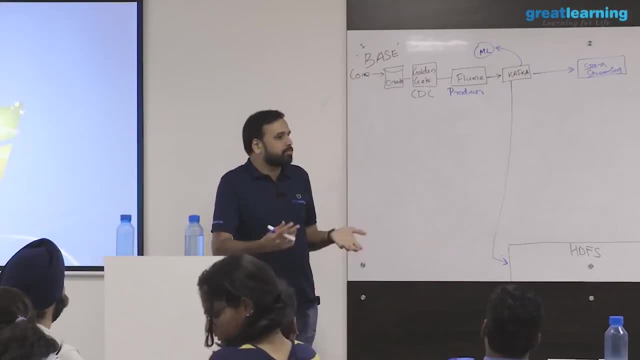 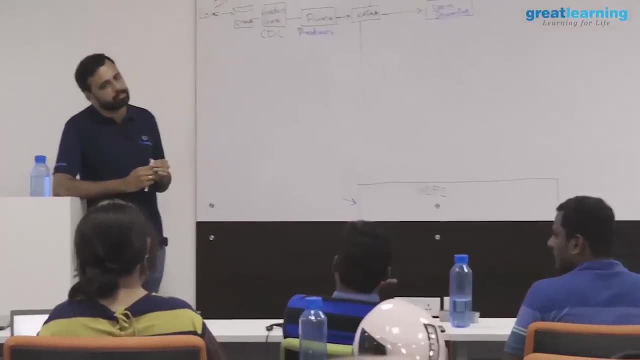 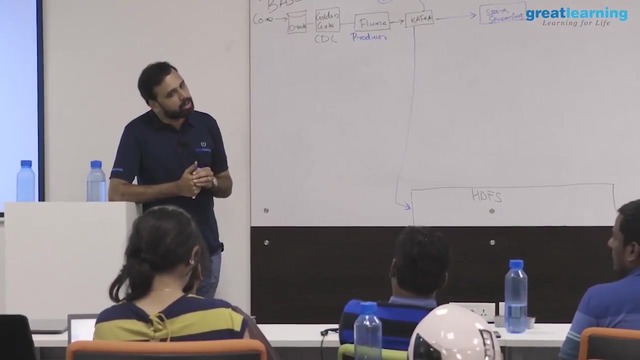 So space is required. So you need to allocate some space for Kafka to hold the data, Otherwise it will not work. Is there any generic services for Kafka? Suppose I want to download Kafka, That means I need to go through Kafka and I need to have some other services to go through. 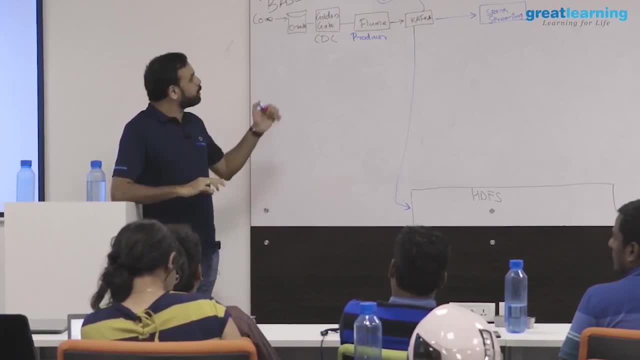 some services. No, no, no, Kafka can work independently also. So even though Kafka is very common on Hadoop, we have customers who are using Kafka independently. For example, there is this Nokia Siemens network: Nokia right, Not the phone. 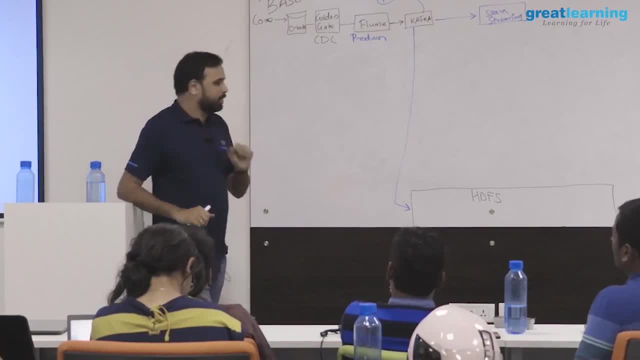 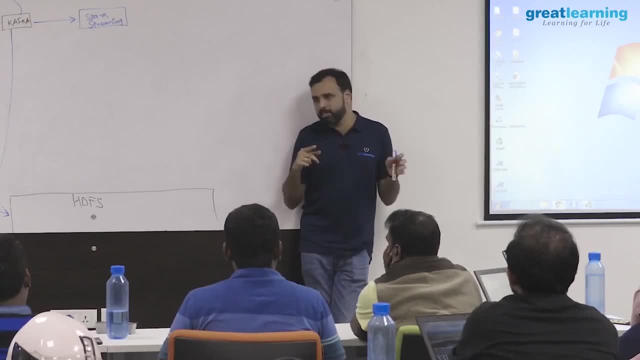 So they have a lot of equipments: Routers, switch tower, etc. So the majority of these equipments are handled by Nokia Siemens Network, in India at least. So we were working with them for one of their projects. So they have this telemetry data. 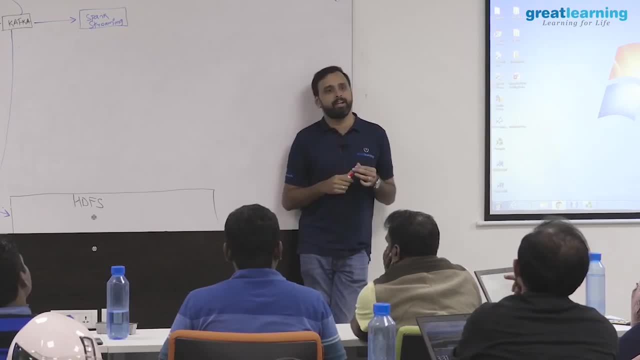 Telemetry data means all these devices will send the data, Like switch router, their current status, etc. etc. That's called telemetry data. So that will come through Kafka. And they are not using Hadoop or anything. They are using the same thing. 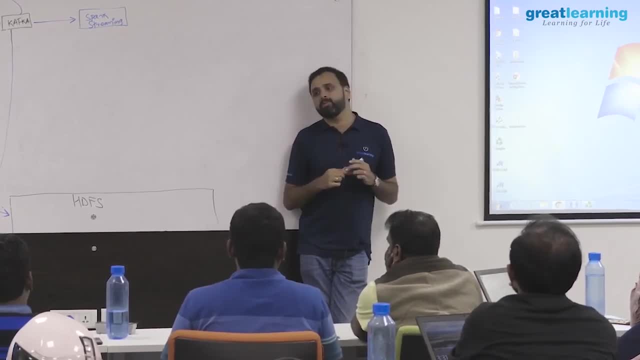 So they have a lot of telemetry data. So they have this telemetry data. And then they have this telemetry data, So they have this telemetry data. So they have all these devices that are used for sending the data. Telemetry data means all these devices will send the data. 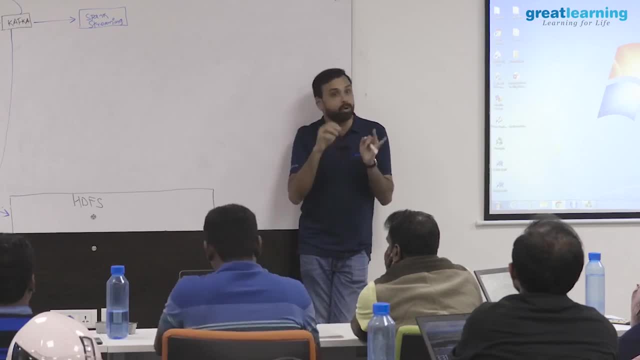 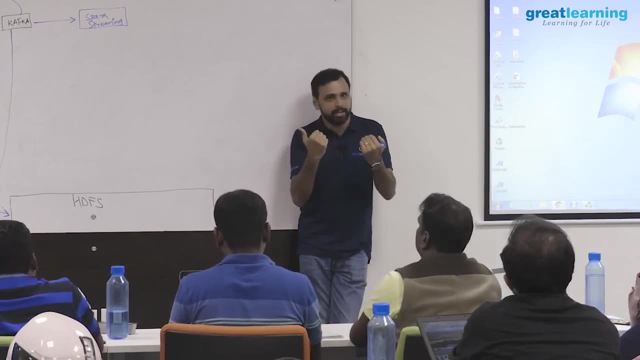 Like switch router, their current status, et cetera, et cetera. That's called telemetry data. So that will come through Kafka And they're not using Hadoop or anything. Kafka is just used to collect all this data. 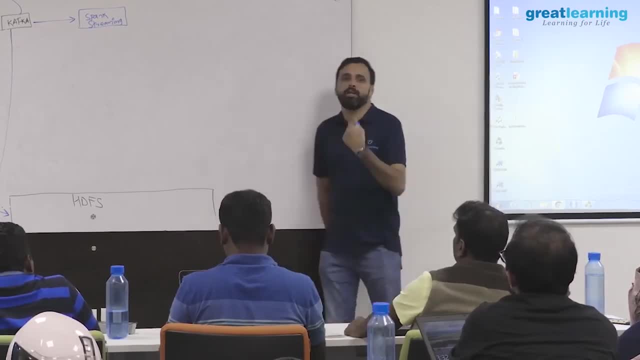 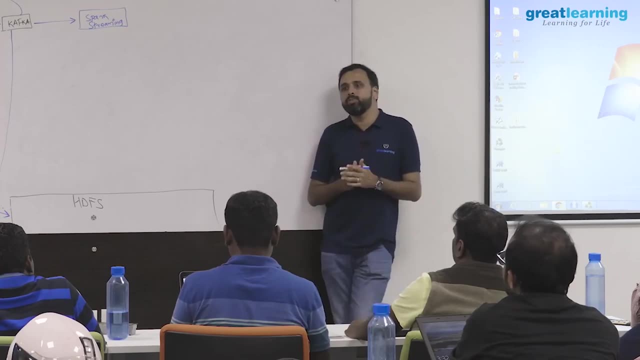 So once Kafka holds this data, they have multiple applications which will read this data and understand the data. So basically, they have a Kafka cluster- They have nothing to do with Hadoop- And that is used to hold all this telemetry data, this telecom-related data, for them. 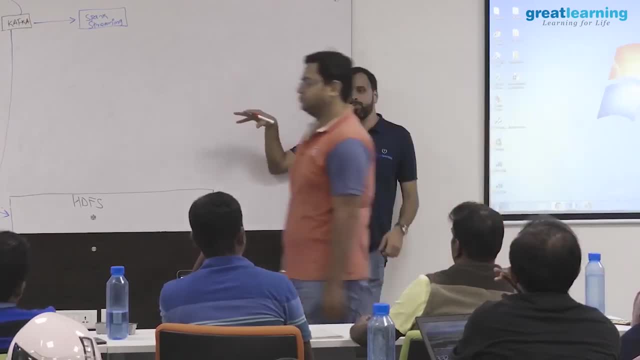 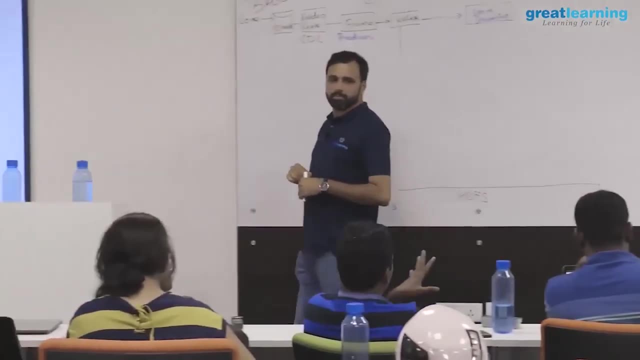 In this example we have Hadoop, So very commonly Kafka is found on Hadoop. because it is a big data platform, You can use it independently also. Suppose if I want to download the tweet data, then what should I do for this? 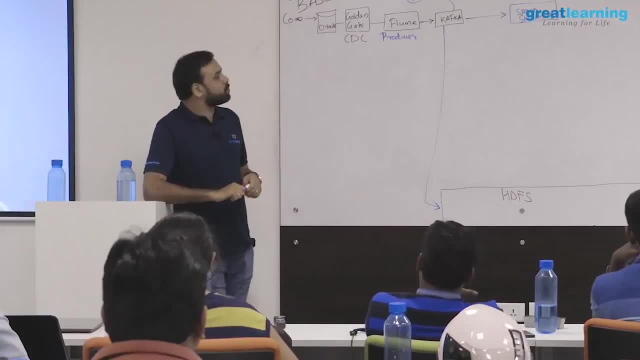 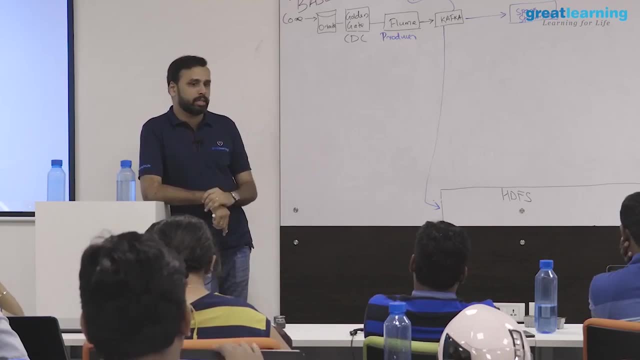 So in this architecture, I mean, if you- Not in this architecture generally, I'm talking about it- So you can use Flume. So I mean, if you're simply interested in downloading the tweet, you won't need to use any big data technology. 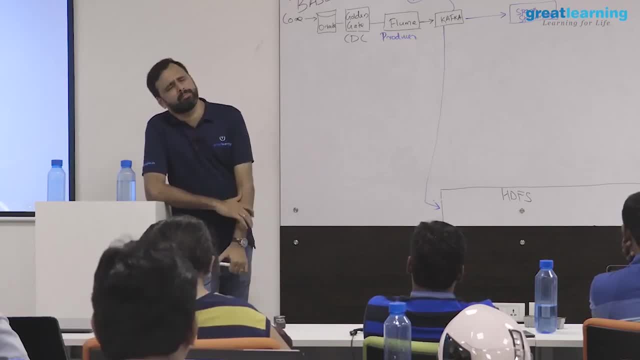 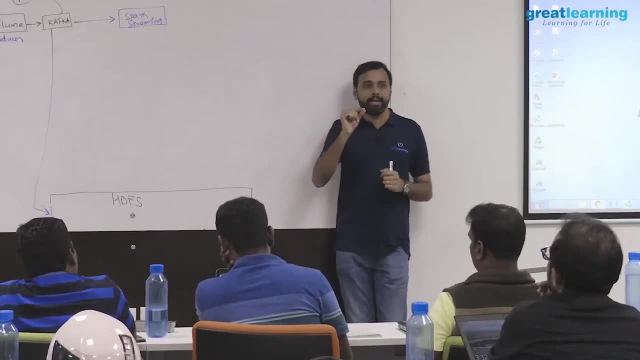 You can get it from this. what you say API, right, REST API. So there is something called REST API Using the REST APIs. so Twitter has some rules. Previously it was very easy to download Twitter data, Like anybody can go and say that. 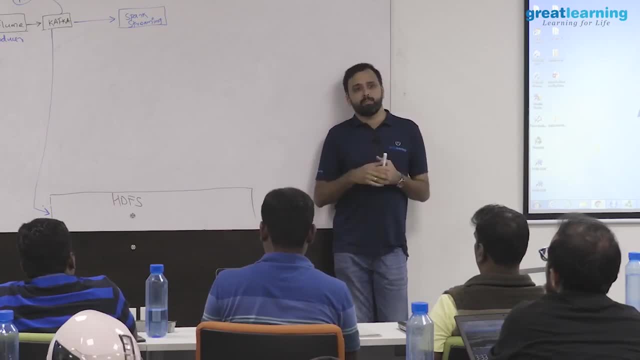 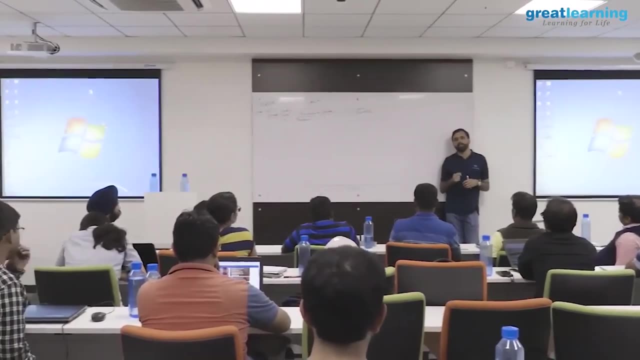 I want the data and you'll get all the data. So now they have made their rules a bit stringent. So you have to sign up for a developer account and then you have to send a request to Twitter. They will ask, like, why you want to create it. 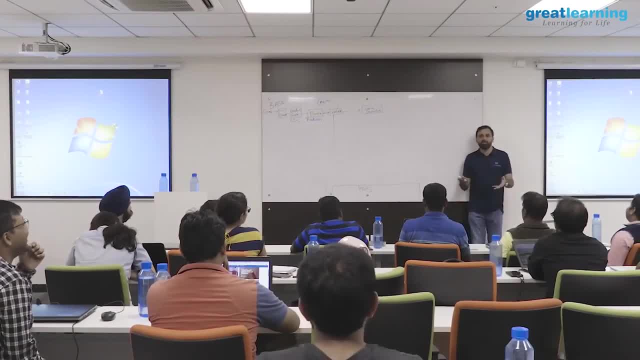 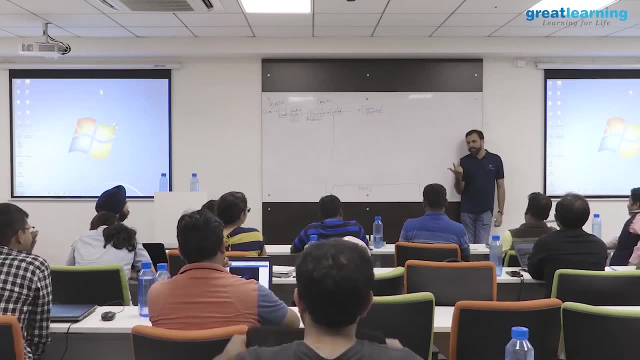 Are you going to bomb the Washington, or something like that. they will ask You say yes or no? And some questions they will ask basically to identify, And then you give all the answers and they will take two days to review your application. 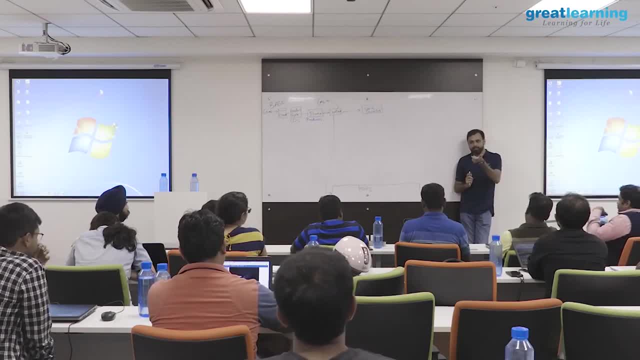 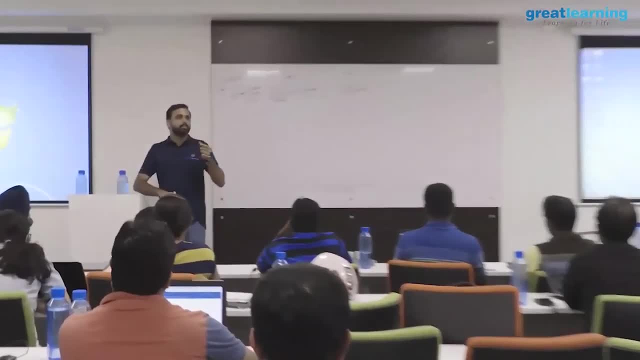 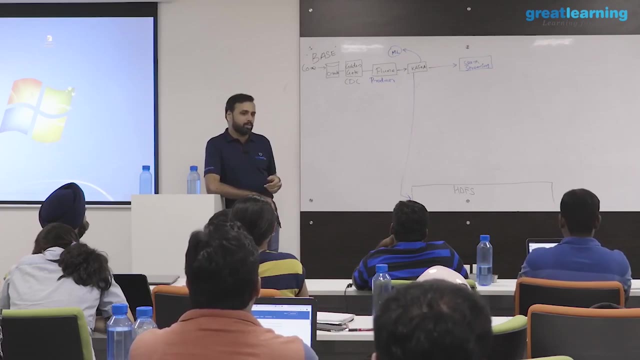 Then you say: okay, you have the access. Then you have to create an application with Twitter And that application will have something called consumer key and consumer secret. It will generate So that is based on your username and Twitter. Using these keys, you can create a simple web-based. 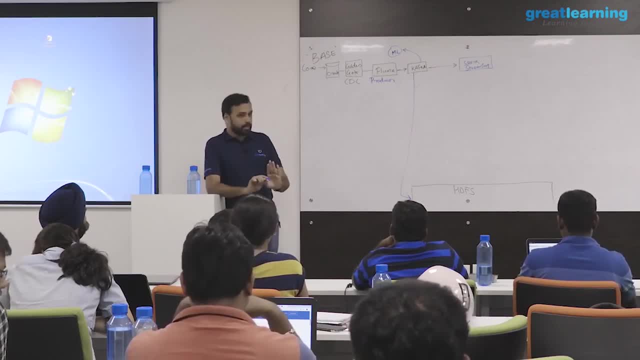 what you say, REST API. Start downloading the tweets- Normal tweets. Now, if you are expecting a lot of- like millions of tweets you want to download and store, probably REST API is not a good idea. I can use Flume. 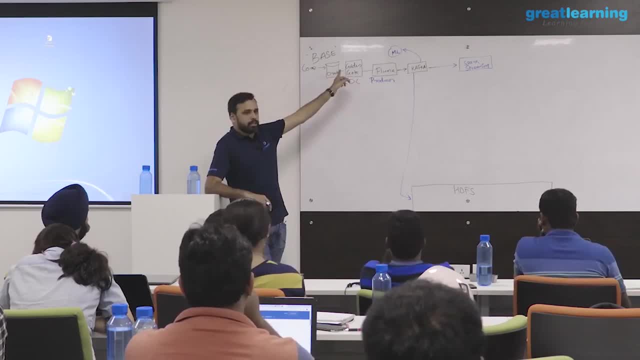 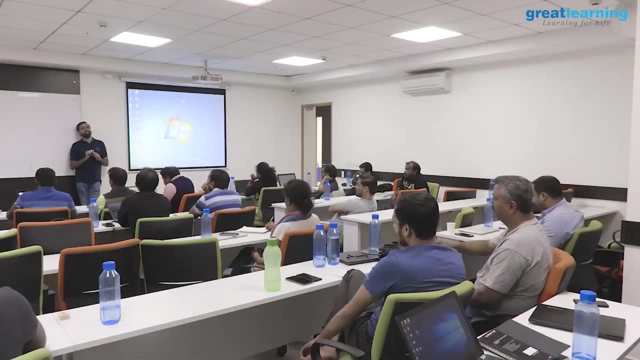 Flume will correct it, So the source will be Twitter Destination. I will say Hadoop. It will dump it into Hadoop, all the tweets that you are getting. So, first thing, they will give you all the public tweets, not private tweets. 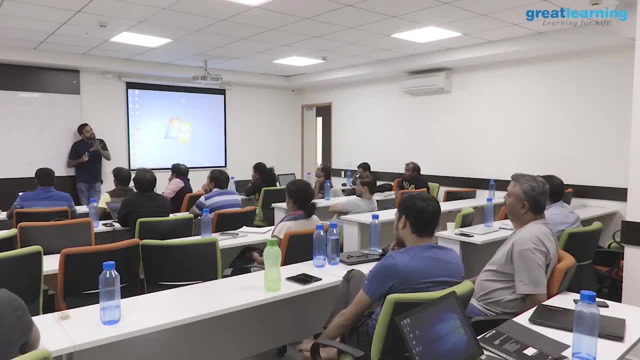 So any public tweet you can access And you cannot- ideally you cannot- go to them and say: give me all the data. That will be overwhelming, Like you will get billions of tweets right. So you can use filters. We use filters. 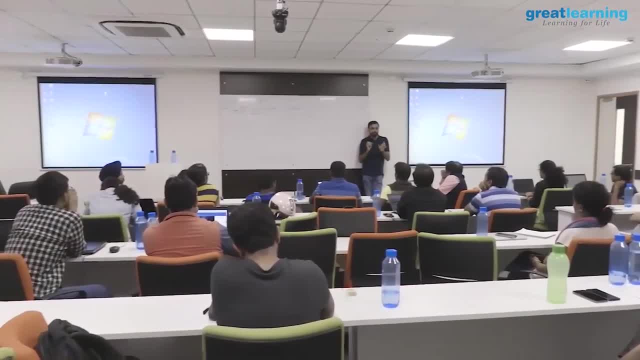 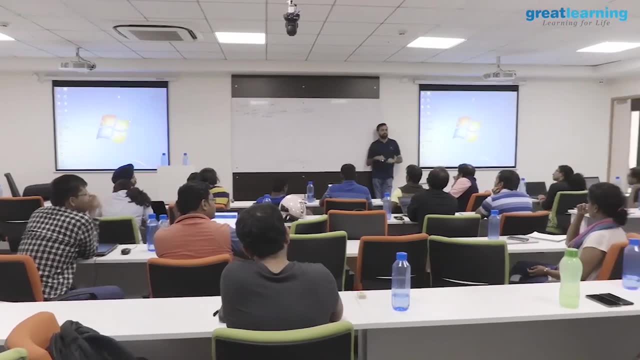 In the filter you have to say what you want. So in the filter I can say Apple, So anything matching with Apple you will get. But the filters are not really powerful because you will get the fruit Apple and the company Apple also. all right. 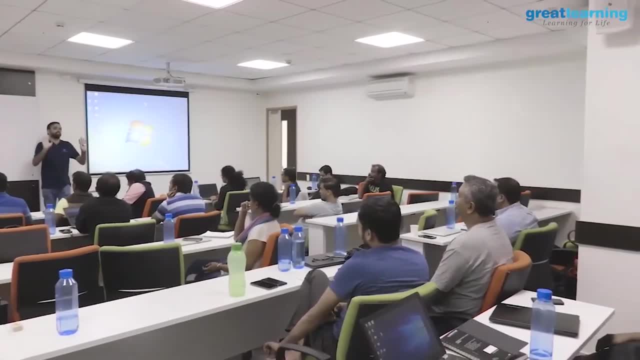 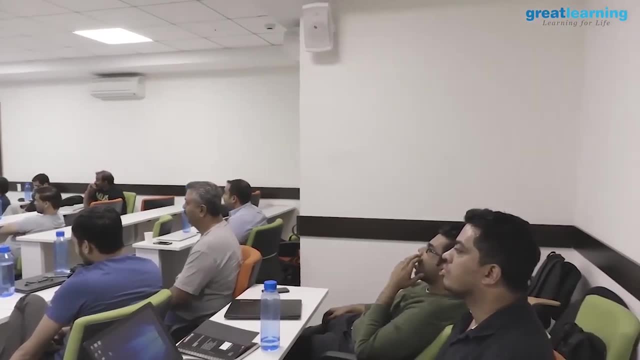 So then then what you do, Because Twitter will say that, boss, this is what I can give you the best. Then you have to figure out from that. okay, you have to write some logic and figure out. This is related to the company Apple. 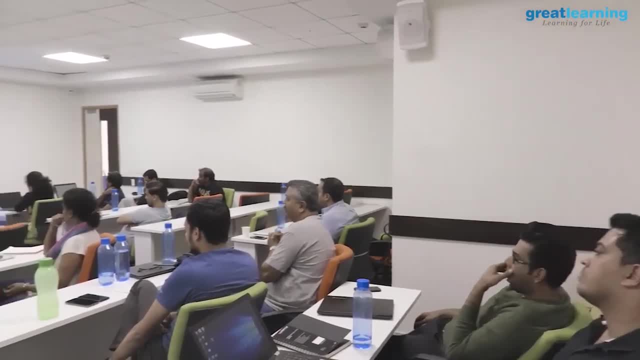 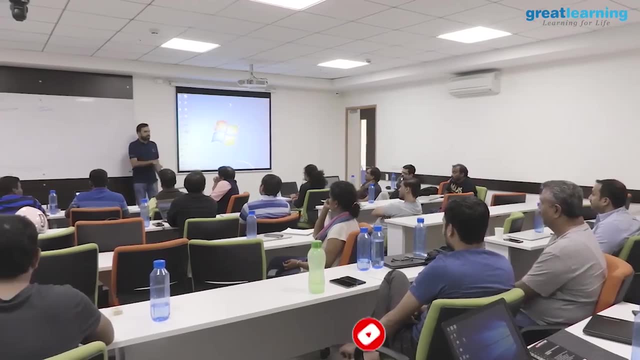 But you get the data. You get the data first And then you clean the data. understand this is company related data and you can get Very rarely people use it. But if I have to send you a tweet which I don't want to make it public, 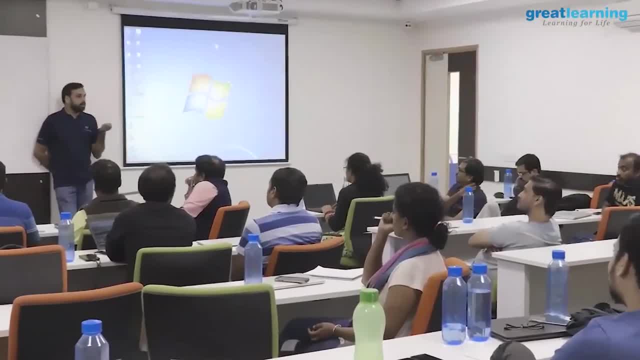 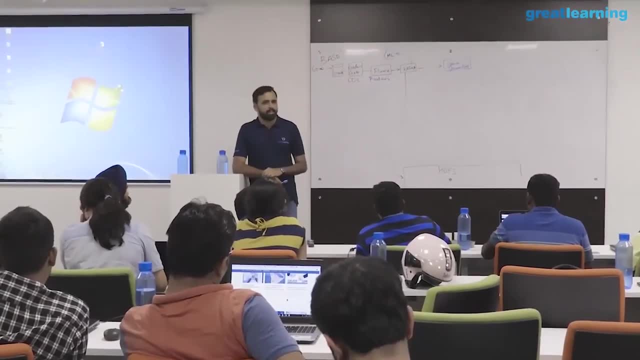 I can do it. It won't be visible So that we will not allow you to download Any other public tweets you can download. Tweets come in JSON format, So we do this all the time. Twitter- Yeah, That's not very common. 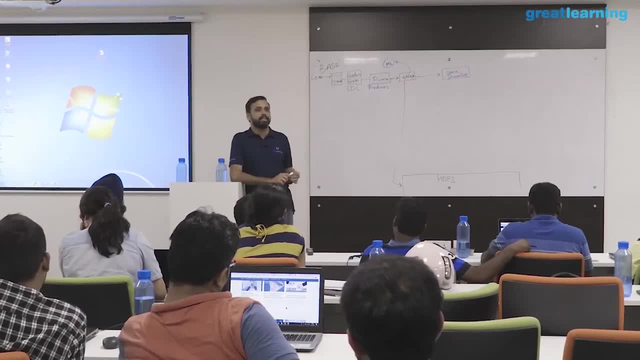 Sensitive analysis is very common, Very common. yeah, Like last week itself we did one on Me Too campaign, Hashtag Me Too. So that was very interesting. So it's very common to do. okay, But I don't. I have the code. 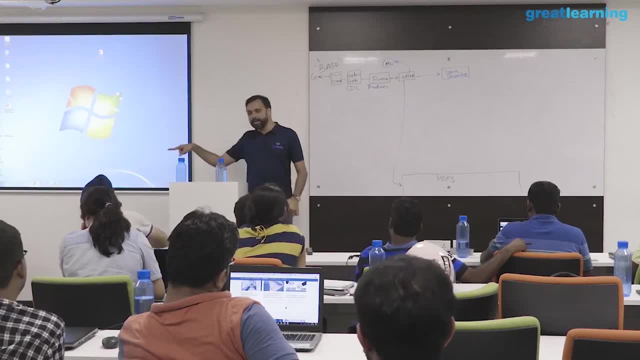 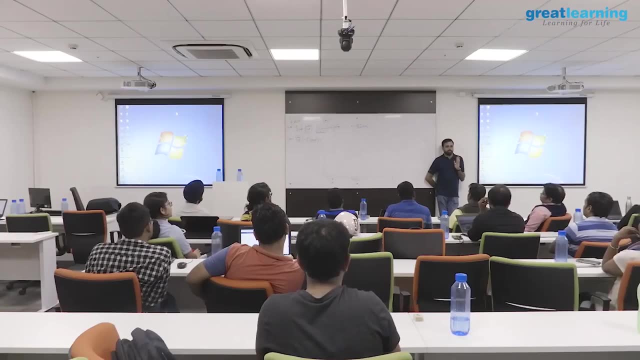 but that's in my laptop. It doesn't work, Like I can't connect. You know you have this machine right, So there's a bit of code. you have to do Quill-based data transfer. So what is the difference? 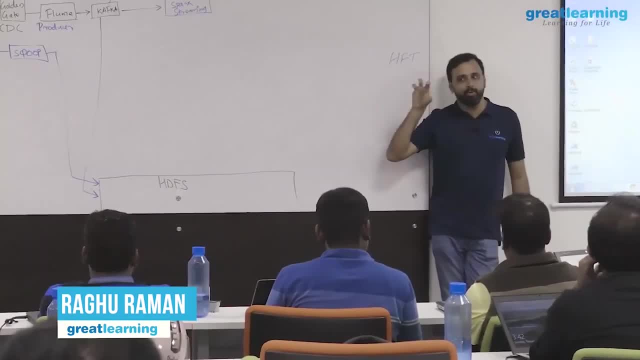 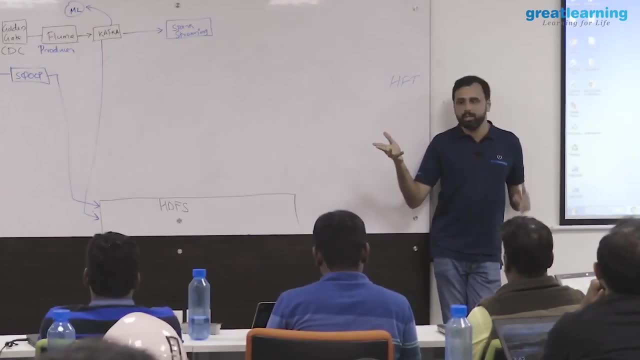 If you're having log files or tweets or any other type of data, Flume will come into picture, or Kafka will come into picture. If you're having RDBMS or a data warehouse, then Scoop will come into picture. typically, Scoop is very easy to implement. 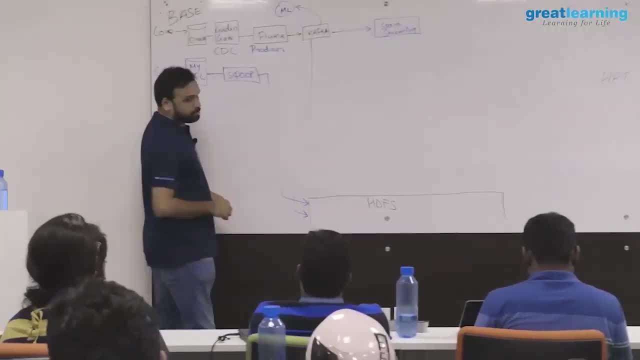 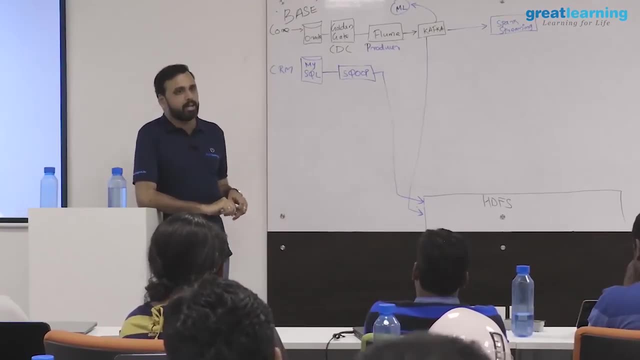 So this guy can actually bring the data from here. So how it stores here, Stores in same place. It's a log file only or No? it is text format by default And you can decide the delimiter Like what delimiter you want to keep. 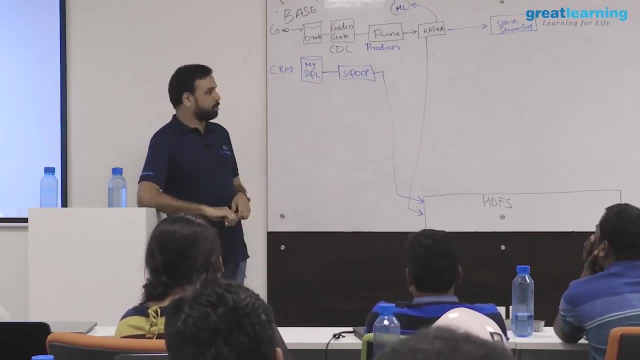 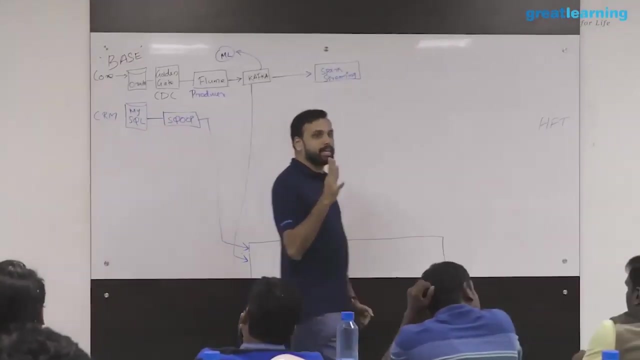 There are also other options. I will explain. So by default it dumps at the text format. Now they have a lot of other data, So primary sources were this okay. Then they had an app, ICC band. This they were giving to their sales marketing people. 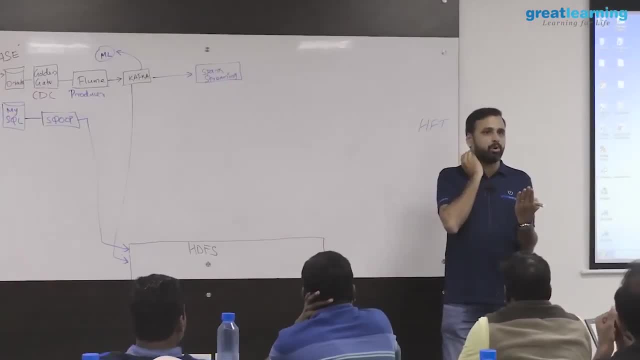 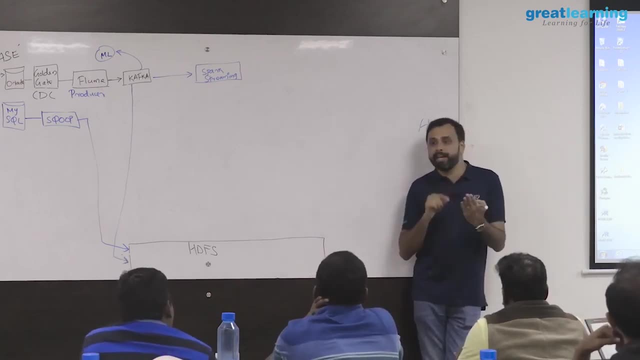 So what this marketing people will do? they will get targets. every day You go and meet 20 customers. They will go to the customer and maybe the customer will join. will not join, So they have to update all that in real time in the app. 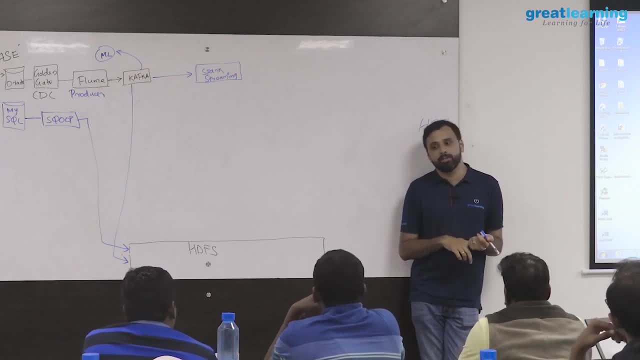 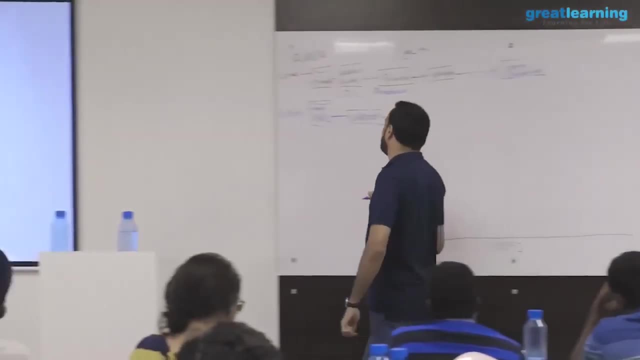 That's an internal app And they have some 3,000, 4,000 employees at that time, as like marketing executors, So this app was actually sending the data in XML format, So they had this app, customer app- okay. 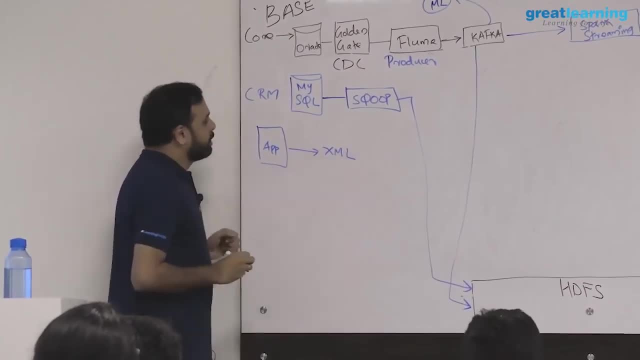 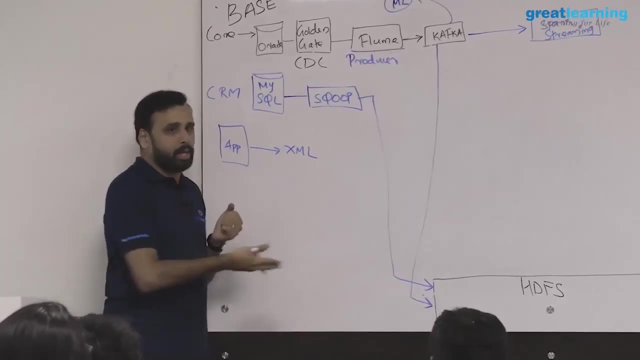 This was sending XML data. Now there is no way to feed an XML data to a root cluster, So there is nothing like scoop and flume. You can manually dump the data. So they were doing a manual dump- nothing fancy, okay. 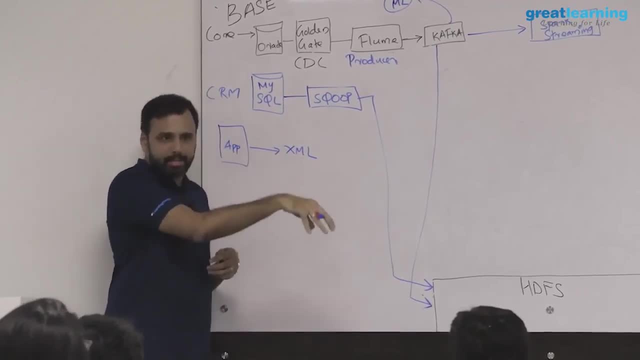 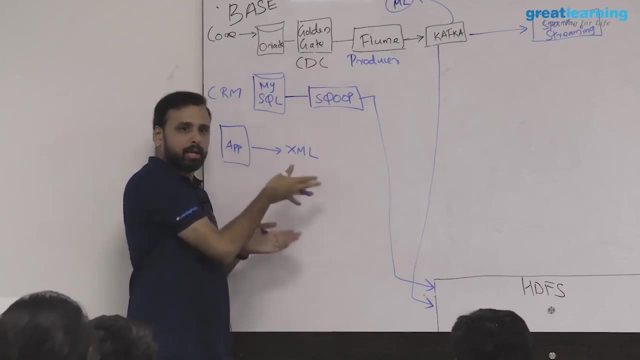 So they had their internal tool which will. so this data will land in one of their servers which will read, and manually you can send the data to Hadoop. So these things are automated manually, which we can send. So this and this data was very small. 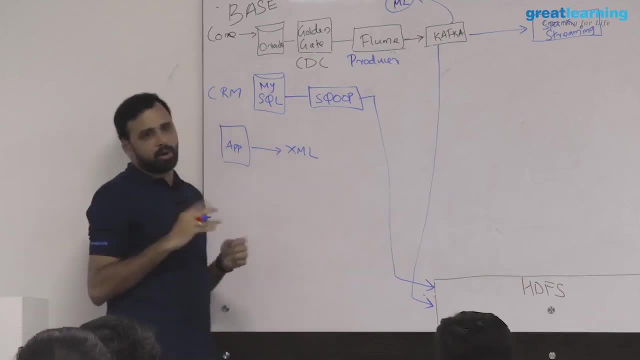 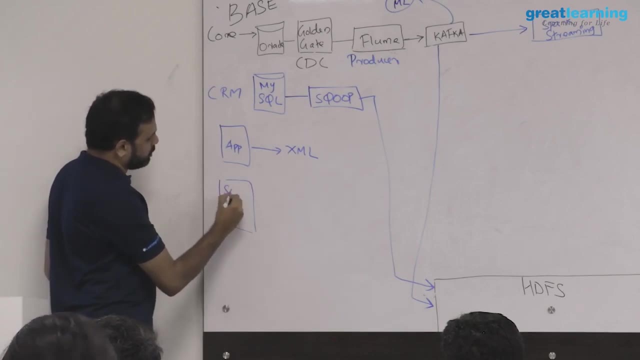 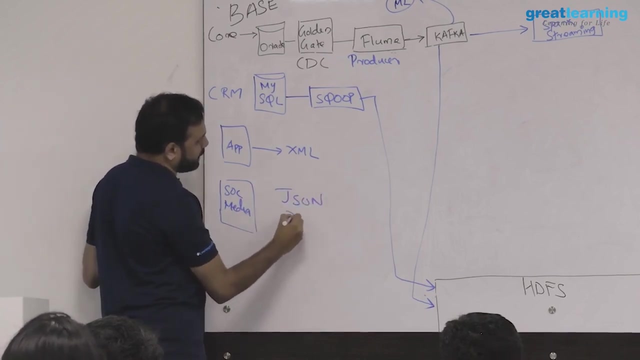 Originally we had a lot of backup, but this day-to-day data was very small- actually not very big- and all right, And they were also having the social media data. So social media data they were getting in JSON format. They were also getting some XML format, okay. 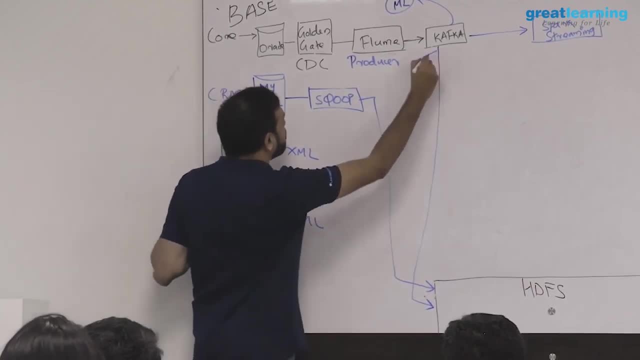 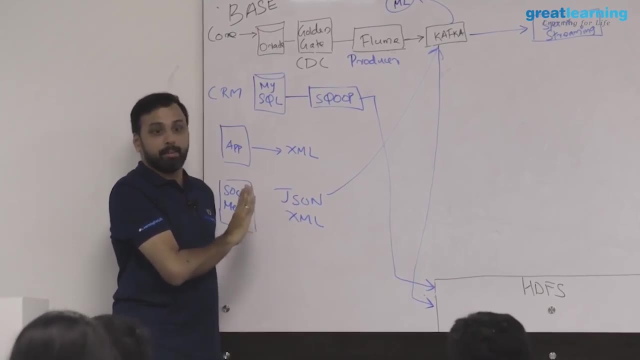 So social media data they were pumping to Kafka. Previously they were not doing anything with the social media data. They were not doing any analytics at the time of migration. So what was the social media data? They had a Facebook page where customers will post reviews. 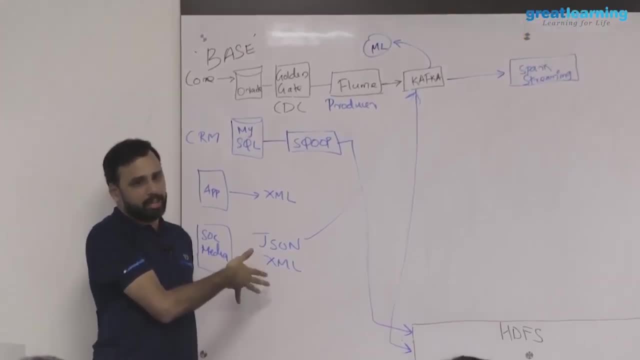 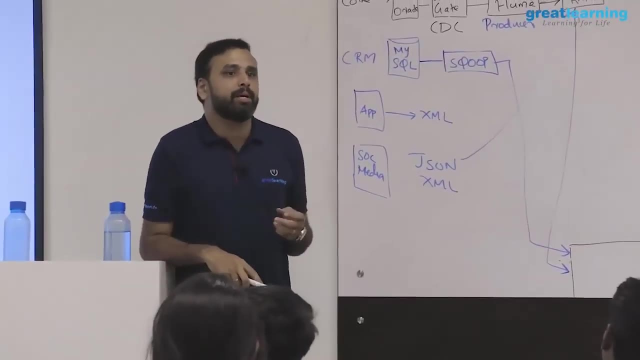 comments, likes and so many other things, So they wanted to do analysis on that. That is one data And tweets and all they were very popular. They were also having a support hashtag, So if anybody is writing to their support. 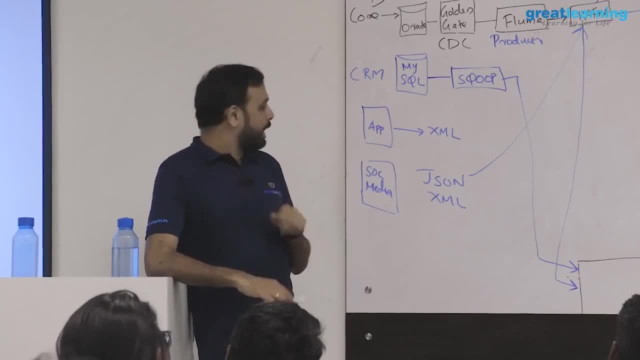 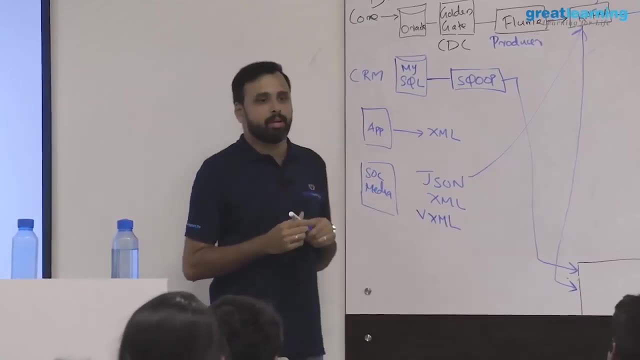 technical support or bank support or whatever they can do that. They were capturing all this And they were also having this voice XML. When you call the bank right, you will say: press one for this, press two right. 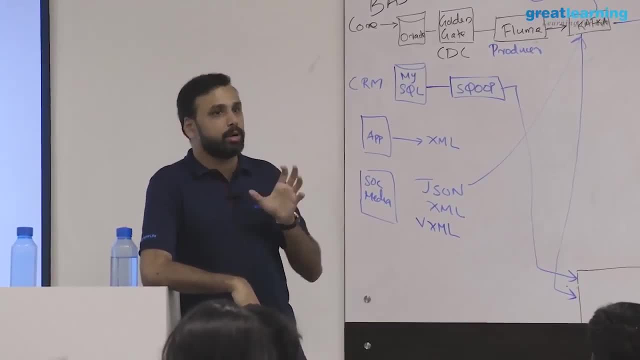 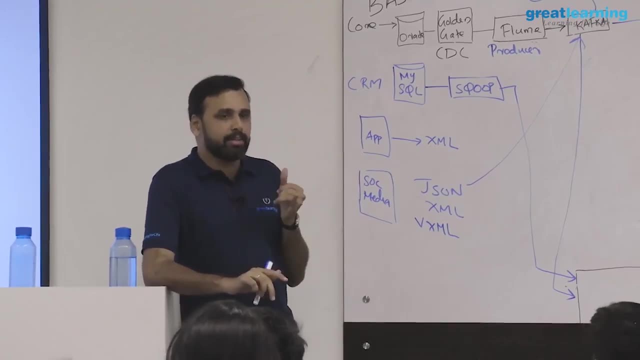 So that is captured as VXML. There is a format called VXML voice XML. They won't store the call record and what you're talking. They will store the metadata: What button you pressed, how long you waited in the queue. 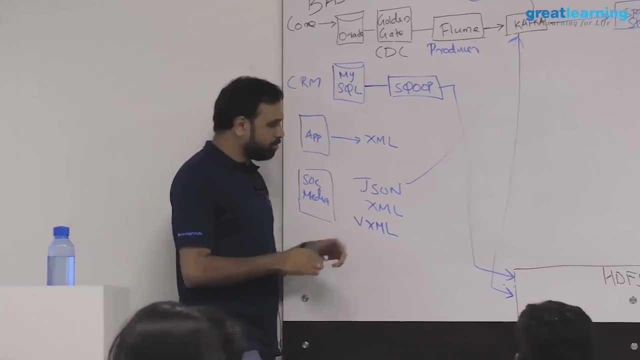 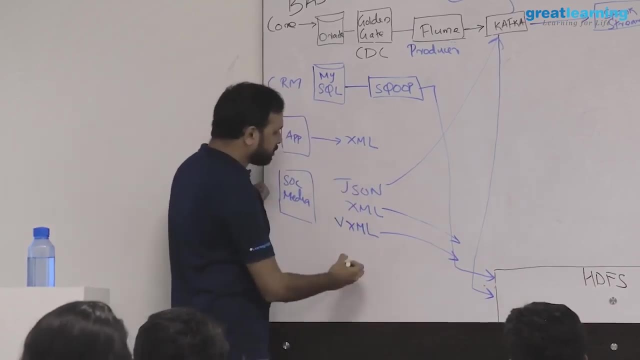 these things right. They have a format called VXML, So VXML and XML. they were directly dumping here into Hadoop. So they had XML, VXML, JSON and some text format data. I don't know what they were using that. 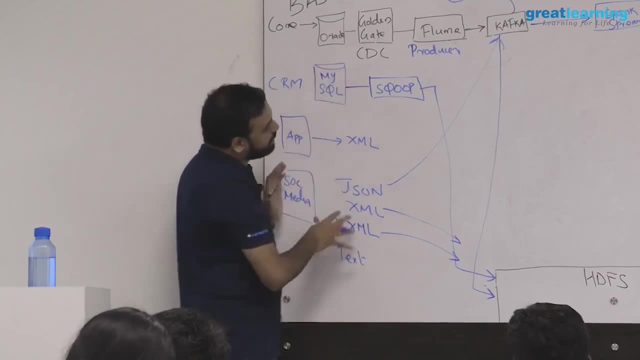 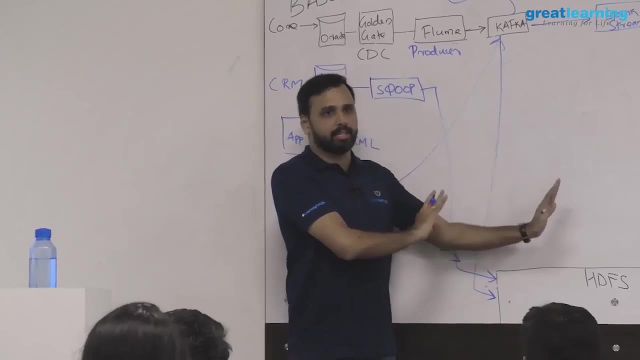 but some text format data also was there. So a variety of data was actually getting pushed to Hadoop, Point number one, right. So this phase is data ingestion, where they're injecting the data. Now, once you have the data here in Hadoop, 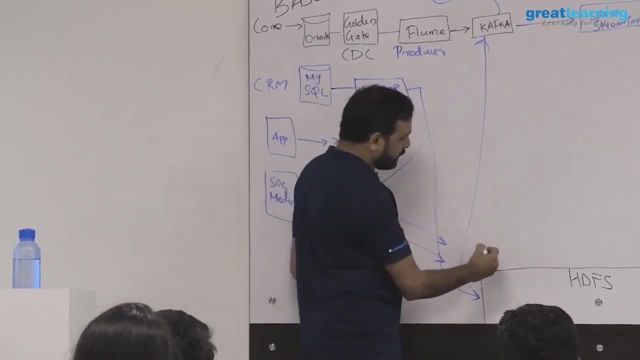 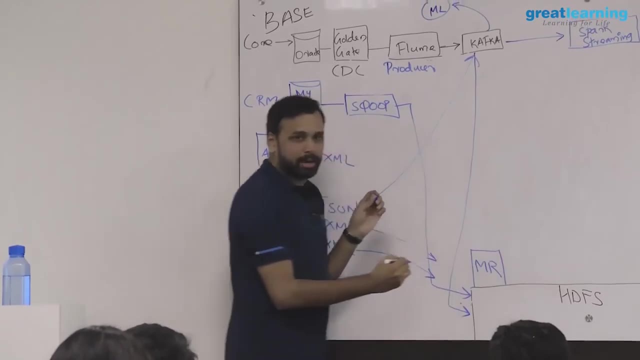 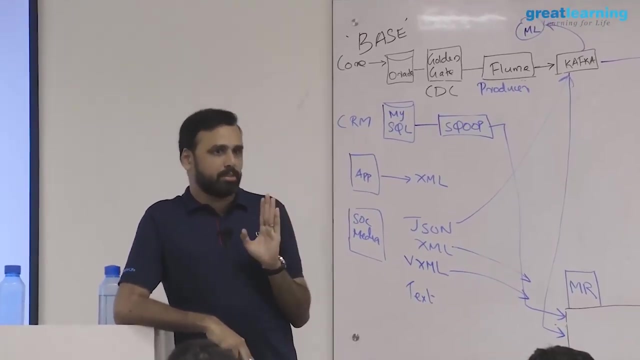 so when you look at Hadoop, one of the oldest ways in which you can analyze the data is called MapReduce, MR. I like it as MR. It's actually called MapReduce, So MapReduce. so Hadoop actually came in 2005.. 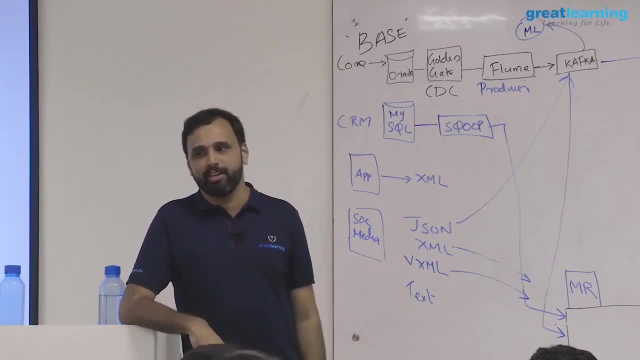 So very old framework. it's not like something very new. Okay, We are in 2018, right, Almost 19.. Hadoop came in 2005.. So in 2005 it came with this framework called MapReduce- Basically MapReduce. 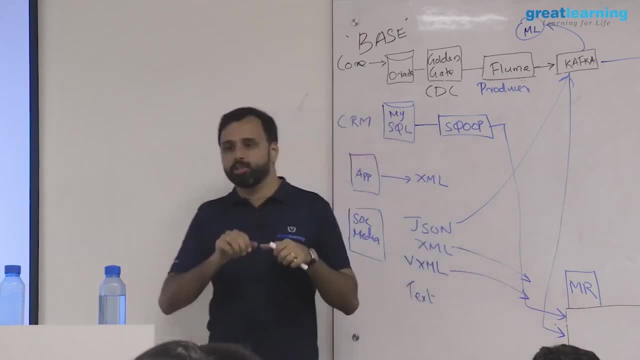 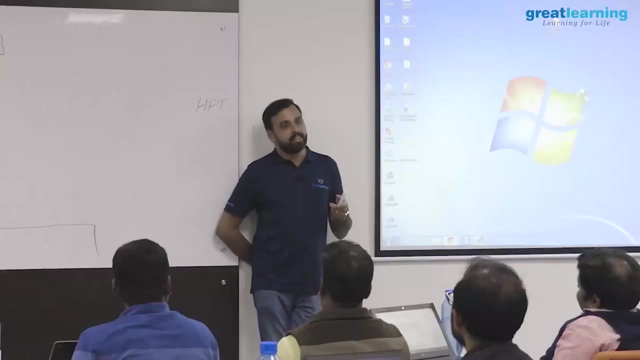 MapReduce is a programming framework. You write something called a MapReduce program which can analyze all the data that you store in a Hadoop cluster And I used to teach MapReduce a lot in the earlier days in the training because MapReduce was very popular at that point in time. 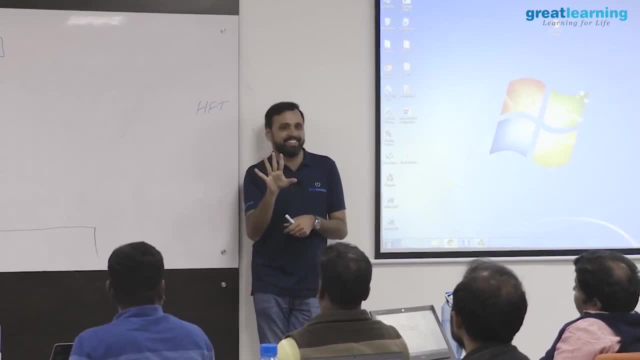 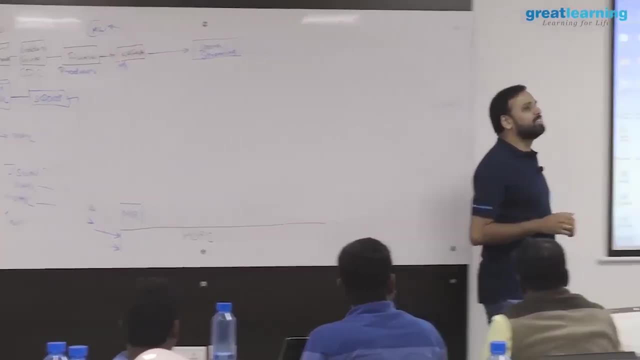 Then, using Java, you write MapReduce program. That is much more complicated, okay, But initial days this is what people were doing: MapReduce program. it was like- and there was a lot of demand for Java developers- Like, if you're a Java developer, you're a big shot. 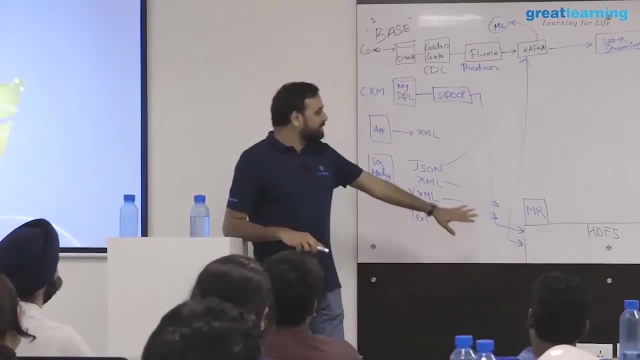 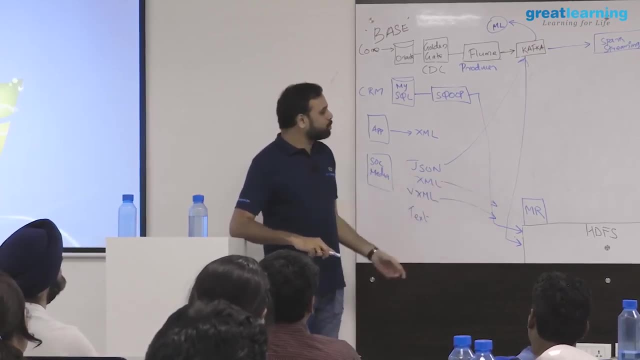 because you can come to MapReduce world directly. right, But nobody is writing MapReduce programs these days. It is over. MapReduce is still there. you can see that nobody writes it, And also MapReduce programs are very slow. If you execute them, of course, you're handling big data. 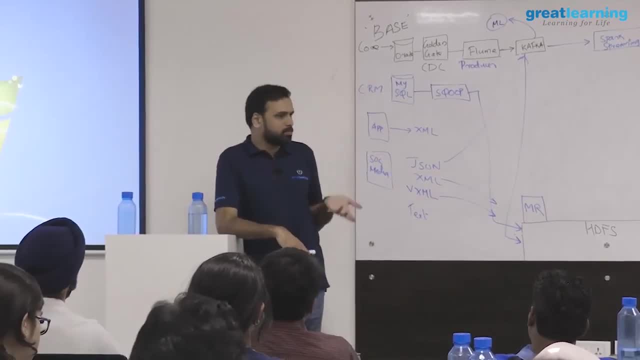 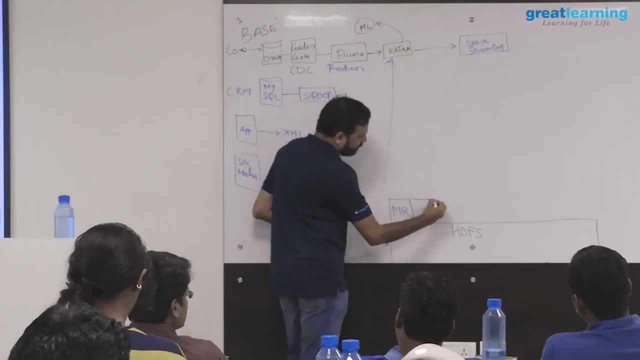 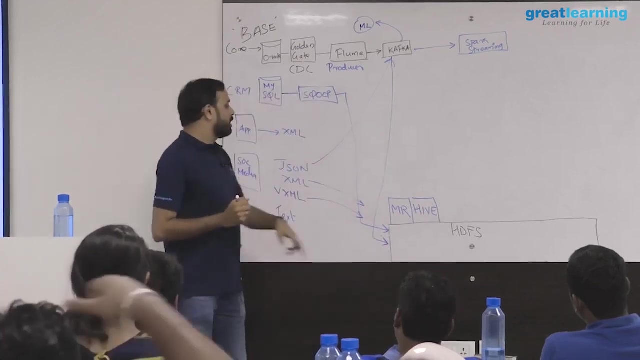 huge amount of data, but it's very, very slow. Running time is very slow and all right. So one way to analyze the data is MapReduce. Another way is that you can use something called Hive. This maybe some of you have heard about, I don't know. 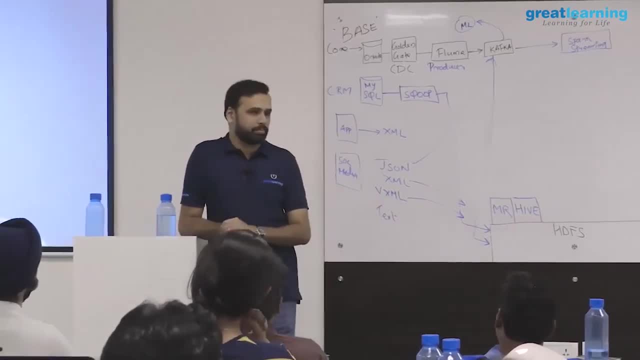 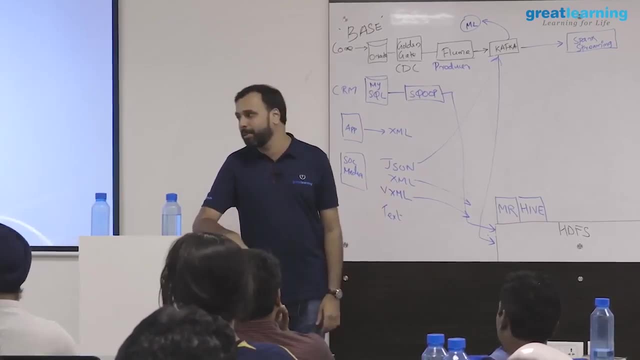 Hive is nothing but SQL on top of Hadoop. So you install Hive, create table, join aggregate, blah, blah, blah. No need to ask me: Yes, same. Well, it is not 100%, it's same. 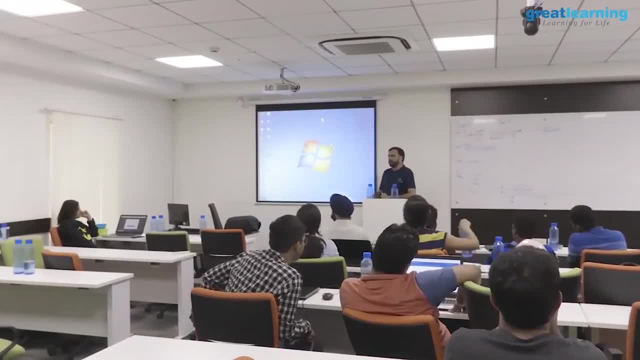 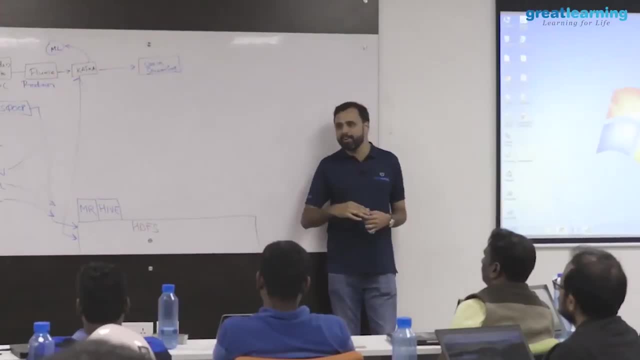 Hive uses a language called HQL, So HLISE language. That is like 99% SQL. Some tools are slightly different Because when Hadoop came into the world, everybody was very happy. okay, Now we have a solution for big data. 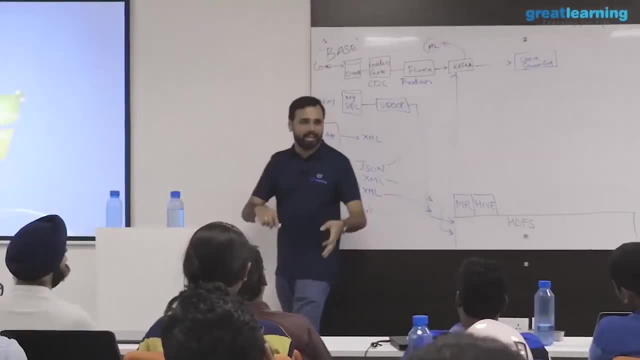 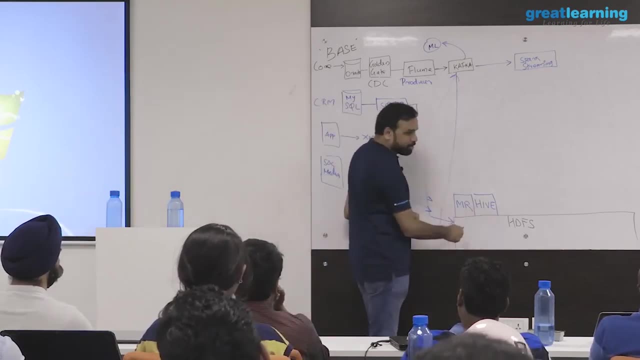 But the moment companies started using Hadoop, everybody was unhappy Because they had to learn MapReduce, which was not very easy. So Facebook created this project called Hive wherein you can, if you structure data like text data or CSV data, you can create a table. 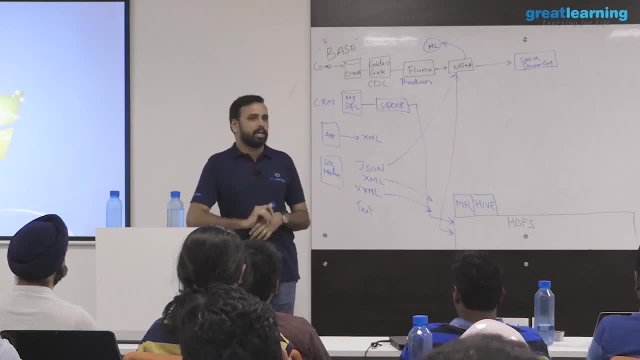 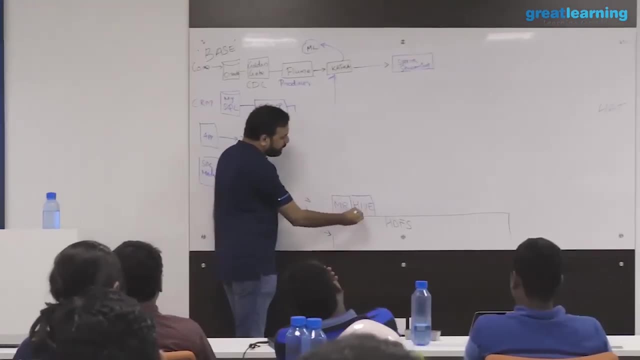 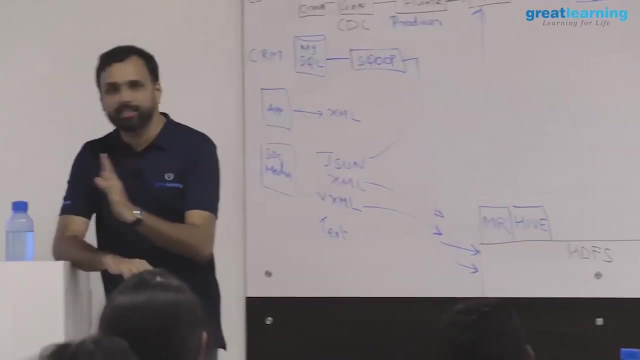 write, join queries and anything that you do in a typical data warehouse. So data warehousing platform, actually. But what you need to understand, Hive will internally convert your SQL queries into MapReduce. it's a translator, It is not direct SQL. 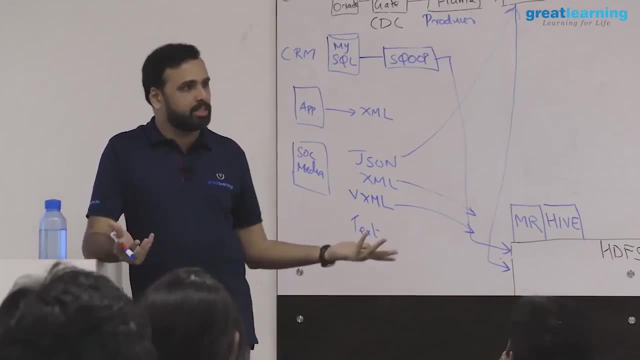 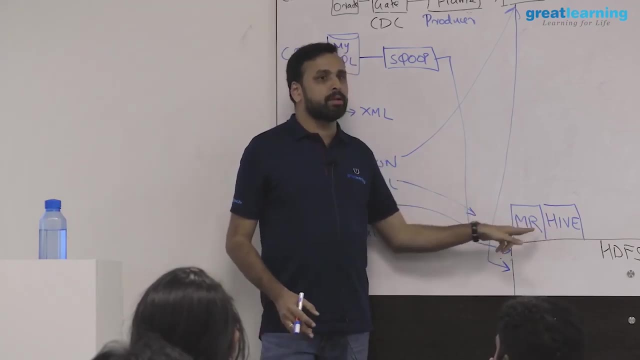 Like if you are using Oracle or something, you run a SQL query. I think it runs as a SQL query right, Like it will push as a SQL query here. no, You write a Hive query and then you check the cluster. 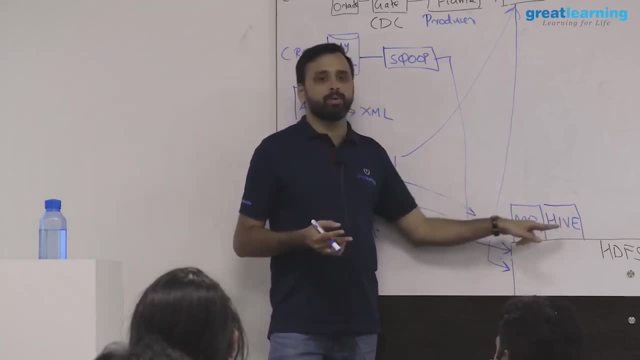 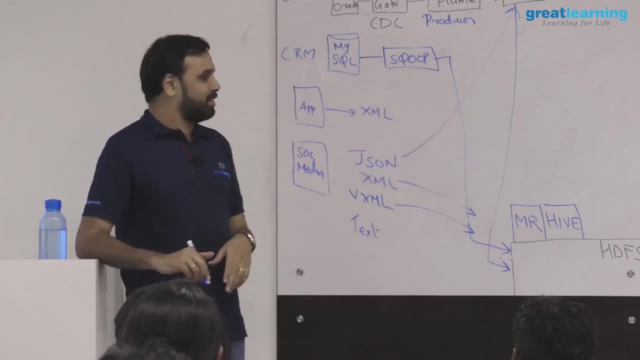 there will be a MapReduce program running, So this guy will convert your query into a MapReduce program. But your headache is gone. you don't have to learn MapReduce, you are happy with it. No, anyway, the slowness of MapReduce is there for sure. 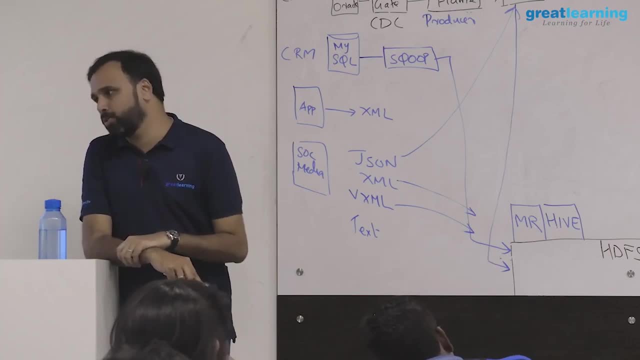 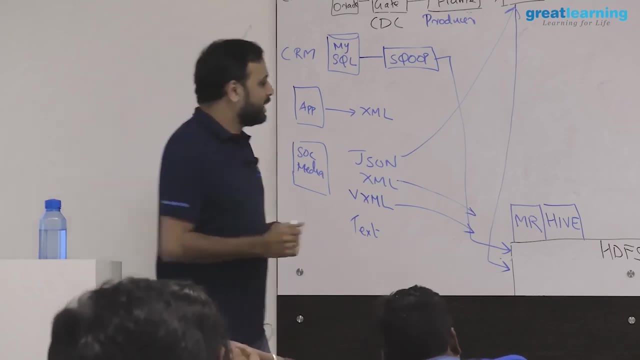 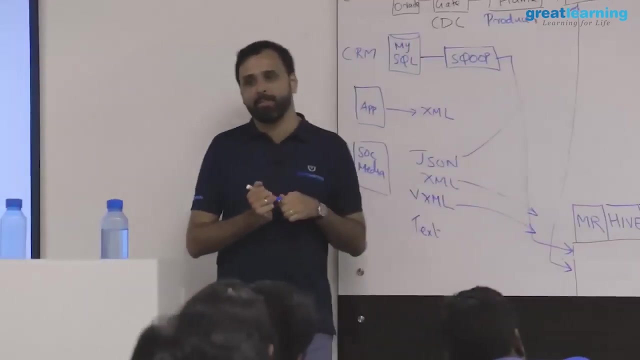 because MapReduce is already slow And it takes some time for this conversion also. So, but still, people are happy because you are using SQL, So no need to learn anything. And there is also another guy called Peeble- Peeble- the animal, Peeble. 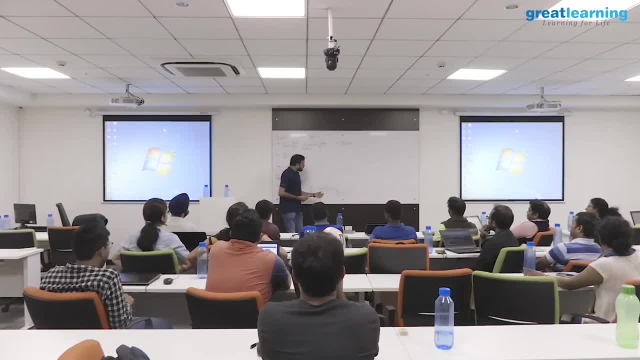 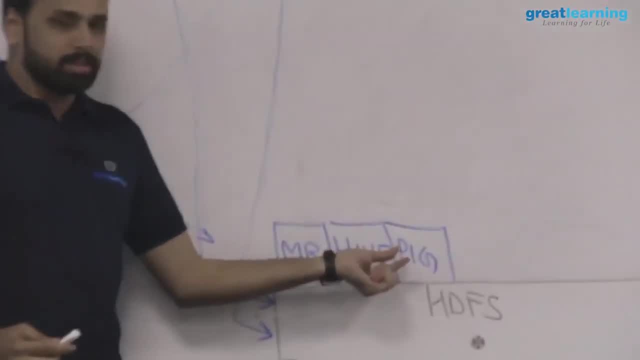 Peeble is a scripting language, basically Same effect as Hive. You write a script using Peeble and say run, it will convert to MapReduce. So this Peeble scripts are easy to learn, Not like Java program. anybody can learn. very easy to learn. 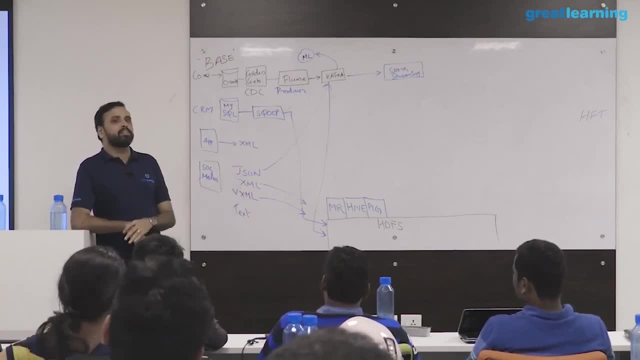 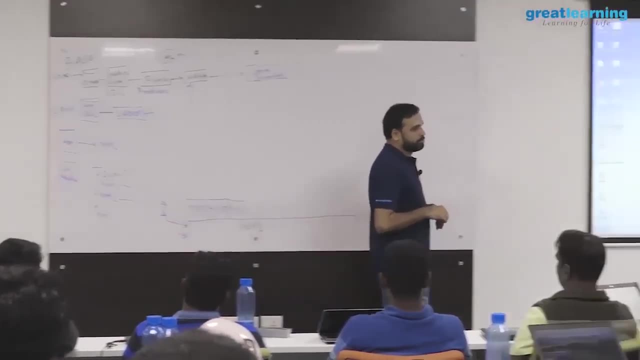 So people started using Hive and Peeble a lot. So if you are a person coming from SQL background, you may prefer Hive because you know SQL. If you are a hardcore programmer, like you, are not really good at SQL, but you are a coding guy, you can easily learn Peeble. 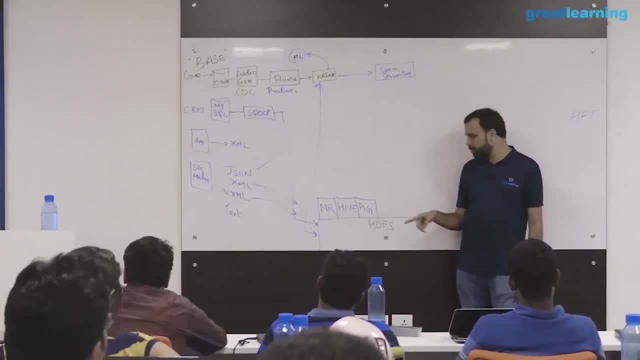 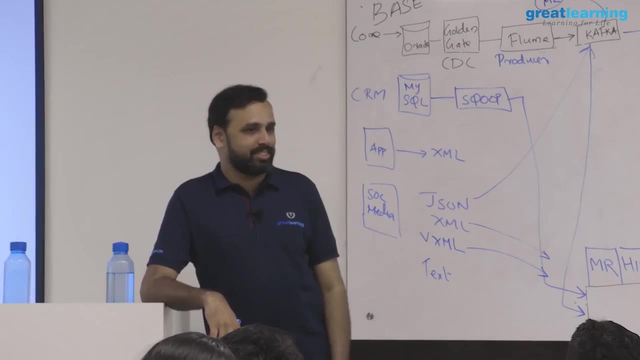 It's a script, actually very two, three lines. you can do analysis. So Peeble and Hive became very, very popular. There will be a tool, like you will say: OK, we'll analyze this data and we will do it actually for you. 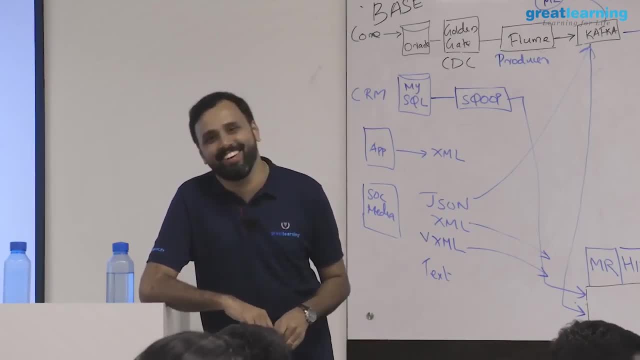 Do the data cleansing, Because data cleansing is the biggest challenge. After that, you can write in SQL code: and Yeah, so do the data cleansing. I think Google has a project which does this. Oh Yeah, Google has an AI project. 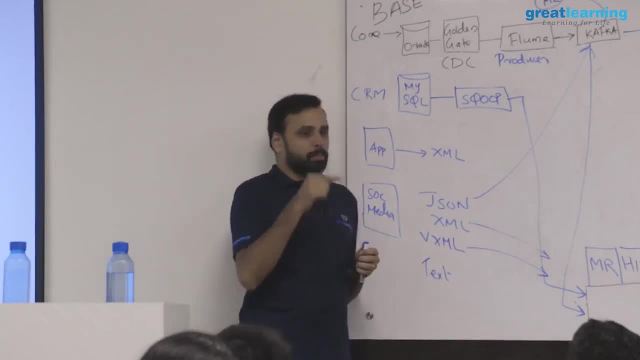 They are automating building a model. Building a machine learning model is a challenge, So they are automating that process. So there is a machine learning to build machine learning. like the movie Inception, There is a conference where all these companies will showcase. 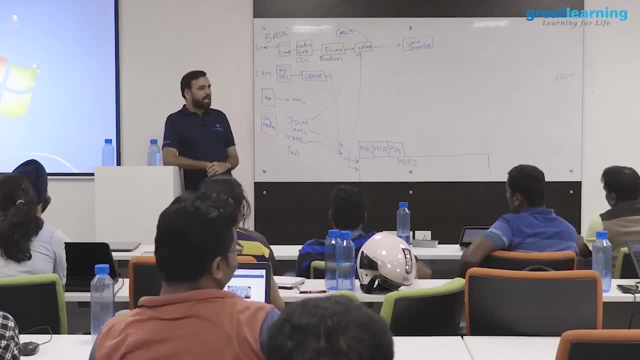 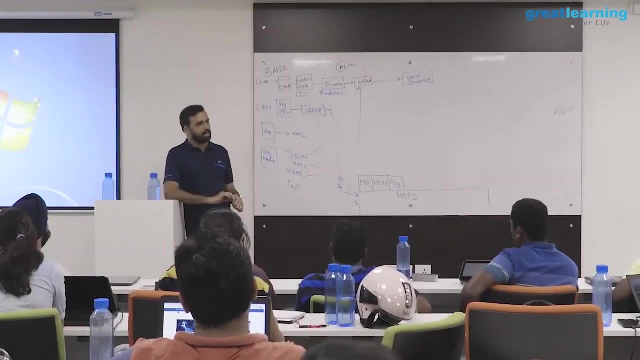 their products, like Sony, LG. So LG had a fridge, a refrigerator. It's not something new, but they have an AI-based refrigerator. Everything is AI, Including a refrigerator, So the refrigerator will now think for you. OK, So you don't have to think. 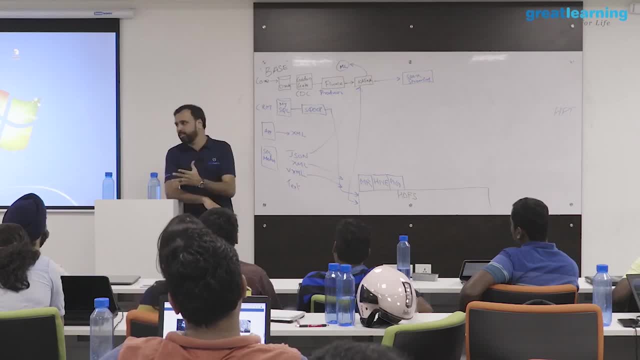 Now this refrigerator. if you keep food like chicken, you keep. it can understand whether chicken is old or whether it is ruined. So if the chicken is getting old, what it will do, it will remind you. You have to prepare the chicken. 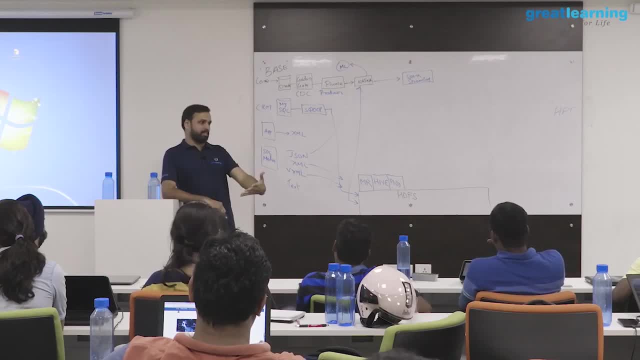 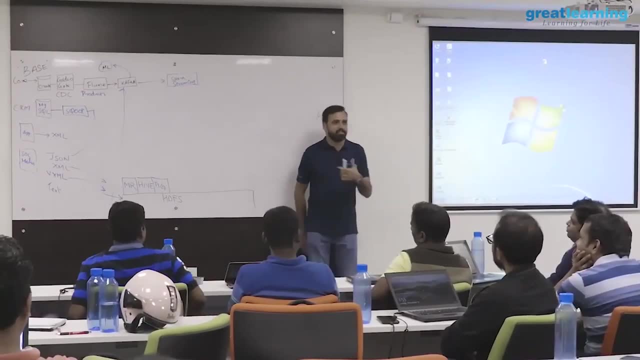 Now it will download a recipe and send it to your microwave oven, So you just need to take it from here and keep it there, And then the dish is ready. Microwave oven, no house to talk to, Fridge and a refrigerator. 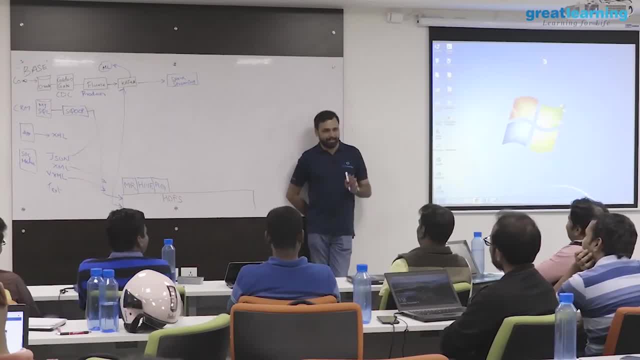 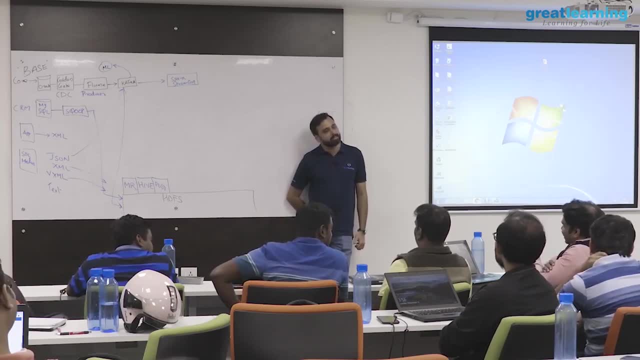 So they're all connected, except you. I don't know where they are heading. When you said that judgment of the opponent, I was just thinking I didn't ask the question, So is there an app that the judge should get an input? 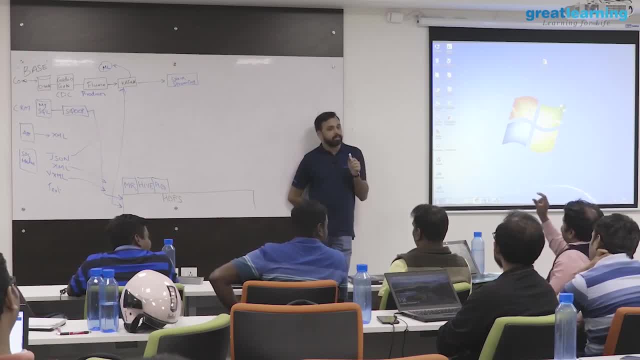 These are all the arguments, or whatever is there, So you can give these three judgments- Option one, two, three, like that, Not for the judge. That is already there. That is not for the judge. OK, The judge may not use it because the judge is human. 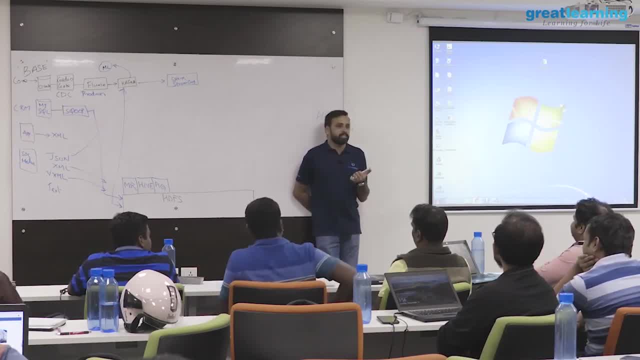 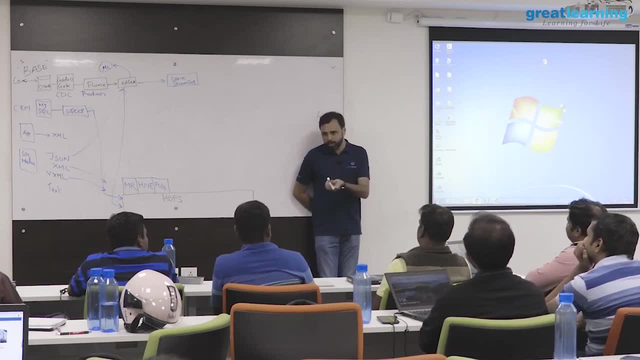 It's an option. So IBM has a product. It's called Watson, IBM Watson. That is for the people Like in the US. it is very popular. If you are in the US, this legal opinion is very costly. Let's say you want to sue somebody for $1 million. 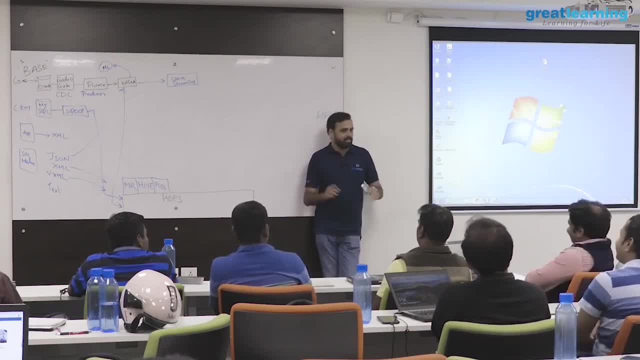 You first have to pay $2 million to the advocate, right? So it's very costly. You know that. So this IBM Watson, they have a robber lawyer, What it does. you go to Watson, You feed all the data. It will tell you the success rate of your case. 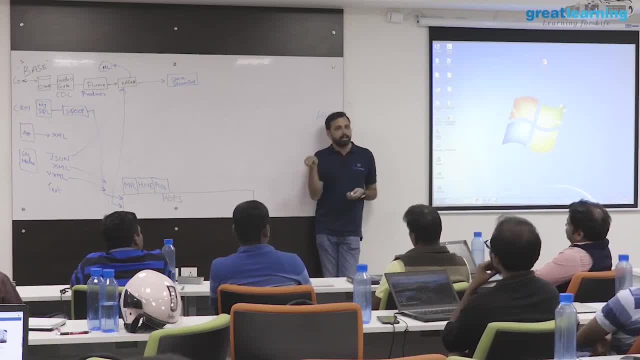 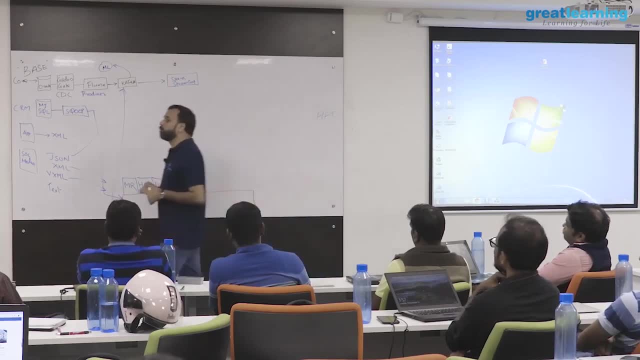 what you should produce in the court, et cetera, et cetera. by comparing all this, Now the startup company I said they are doing similar. They are doing the same thing on section 420, which is cheating. 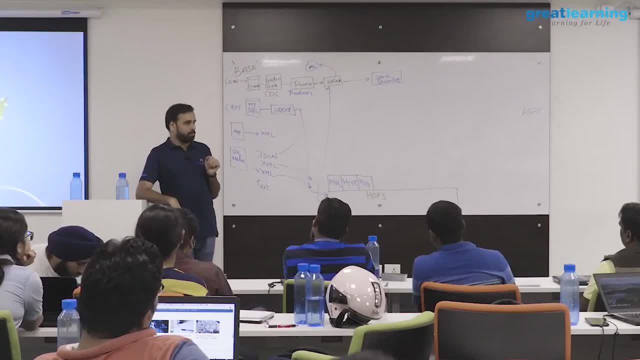 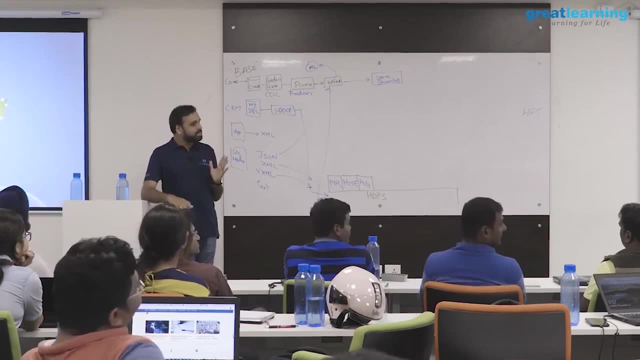 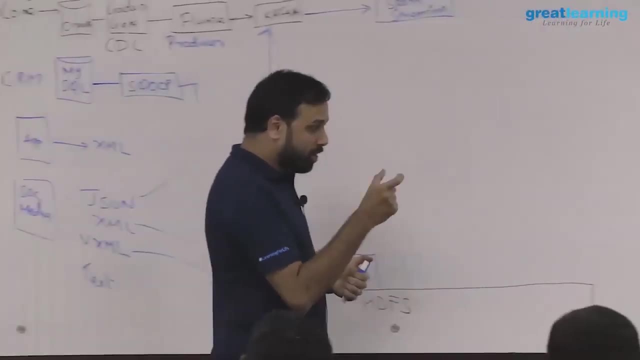 In India we have something called section 420, that is cheating, And cheating is very interesting. let me tell you: No, no, it's very interesting. I can say: You cheated me And you will go to jail. I mean, what I'm saying is that cheating is a very strong clause. 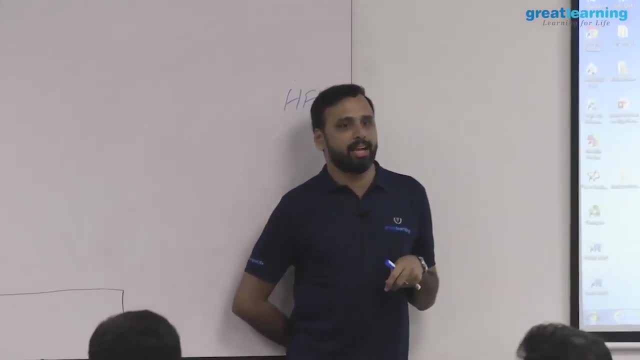 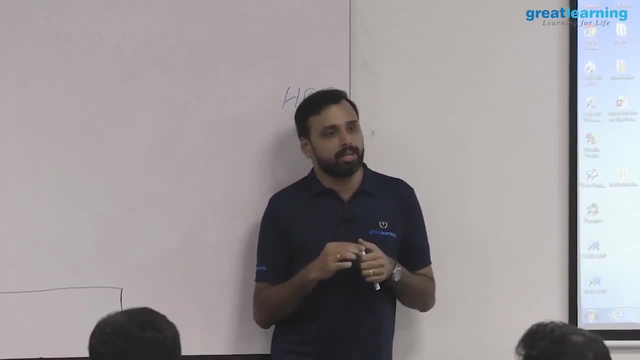 So if I give a request in the police station saying that I'm saying that you cheated me, So to some reason they have to take up a case. So now that is a bit of problem because, as per the government, cheating has to be taken very seriously. 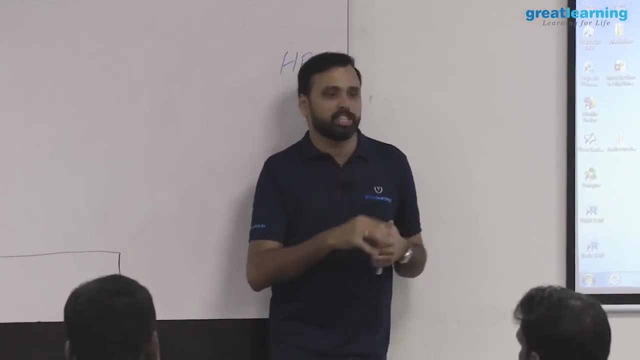 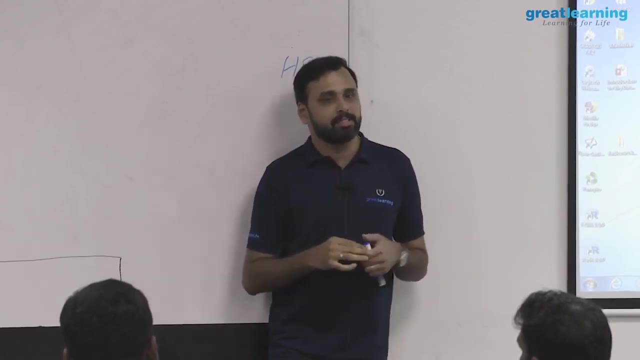 But a lot of people simply give a case saying that he cheated me. he cheated me. So these guys are now analyzing this 420. Whereas if in later case, if somebody files a case, the system can understand and predict that if you proceed with all this evidence. 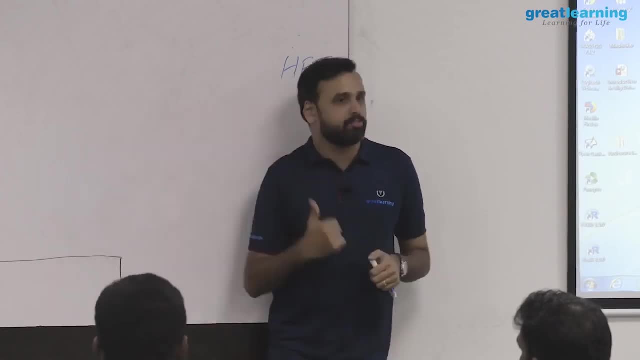 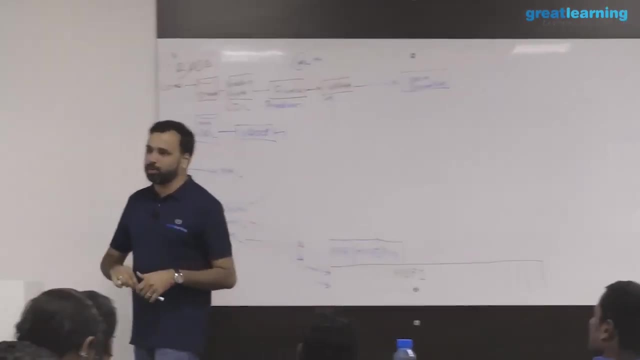 as per the record, you may not win or may win, This is a chance of winning, et cetera. That's already happening And since I am a trainer, I get to know a lot of this because I work independently. So many companies call me, many organizations call me for training. 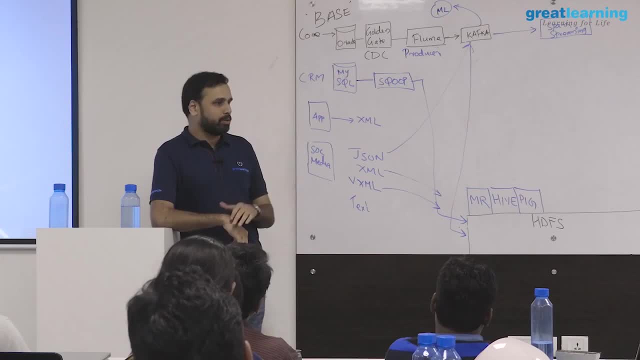 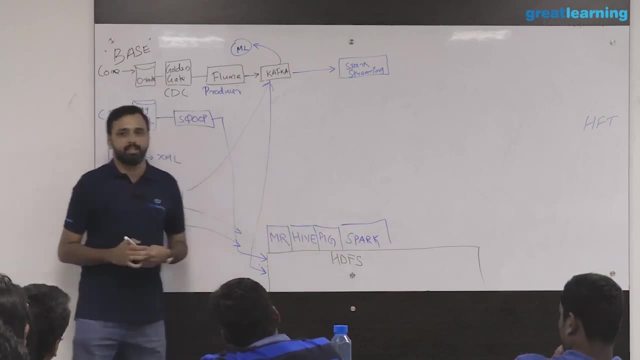 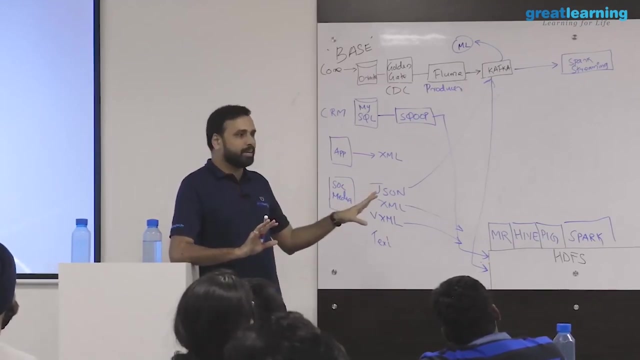 So, and usually I train on big data and cloud, but these are all connected. Yeah, so Spark streaming is there. This guy is very interesting. Why this is interesting? because Spark has a lot of advantages when it comes to big data. 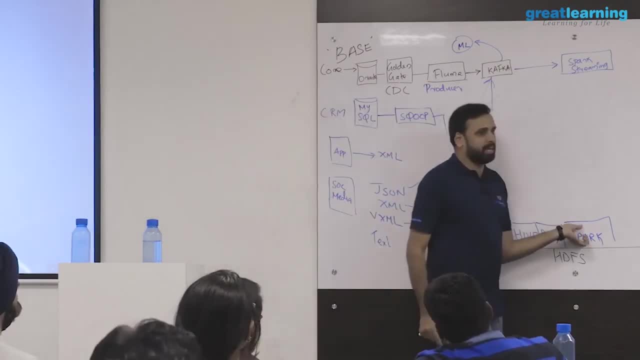 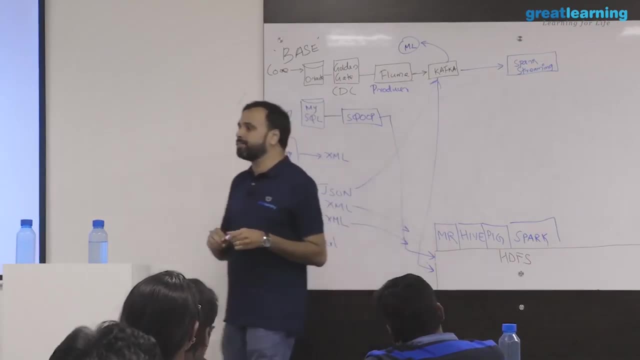 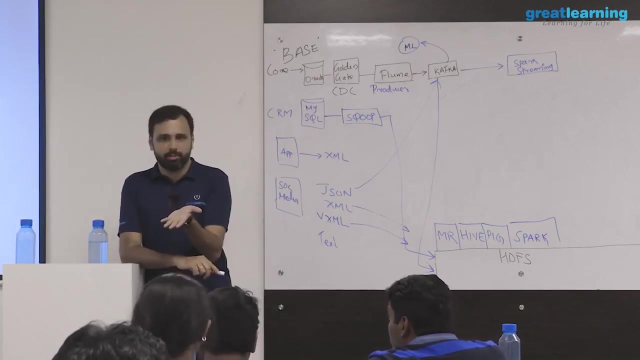 Spark is probably the fastest processing engine right now we have on big data And that is why people do use Spark a lot And also Spark has yeah. So another advantage is that Spark can do a variety of workloads. Using Spark, you can write SQL. 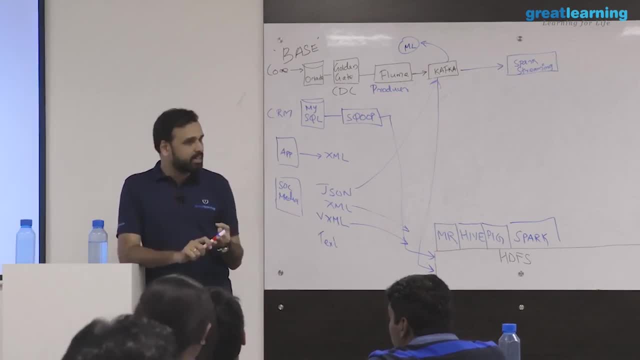 Yeah, So another advantage is that Spark can do a variety of workloads. Using Spark, you can write SQL, You can write SQL queries, You can do machine learning, You can do real-time analytics, You can do batch analytics- everything. 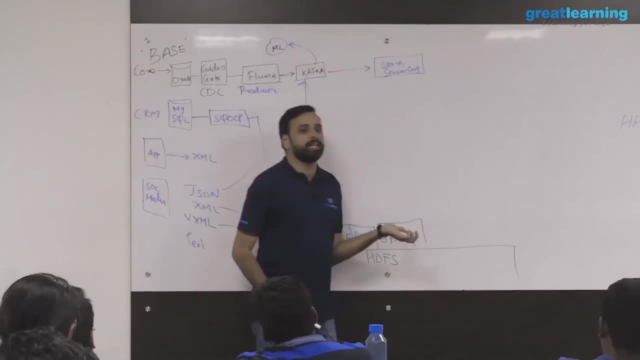 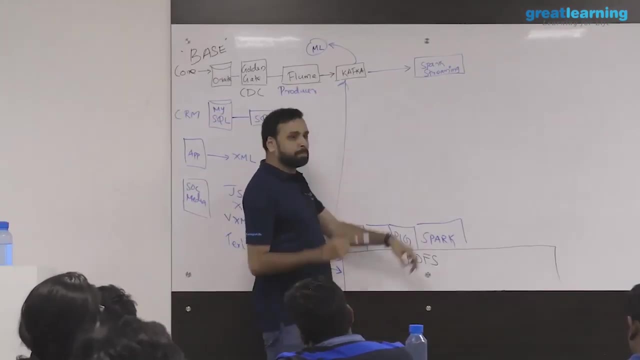 So you learn one framework and it can do many things. That is Spark. So Spark has become very popular. So that's what I'm saying. The real-time part of Spark is Spark streaming. Then you have Spark SQL and Spark R, So it has multiple components. 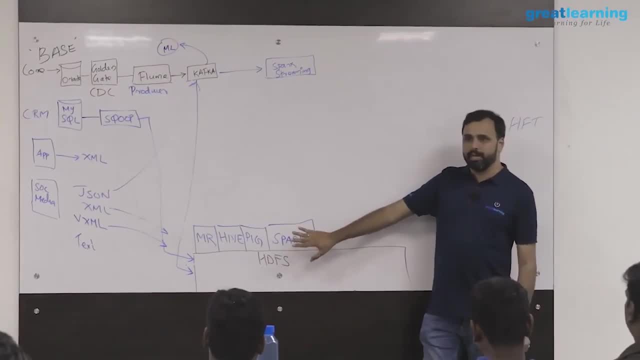 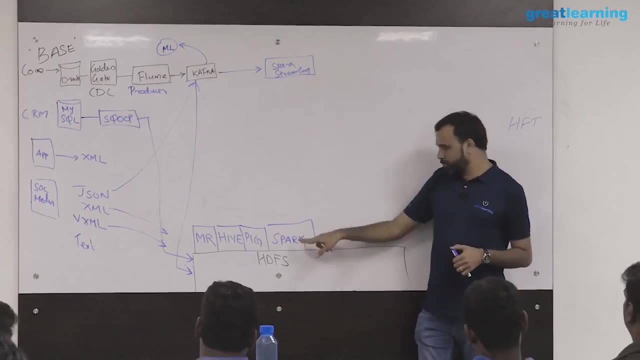 So if I simply say Spark, it is a batch processing system Like it takes the data process and give you output. Spark streaming is where it runs in real-time and give you the output. So my major area is big data right. 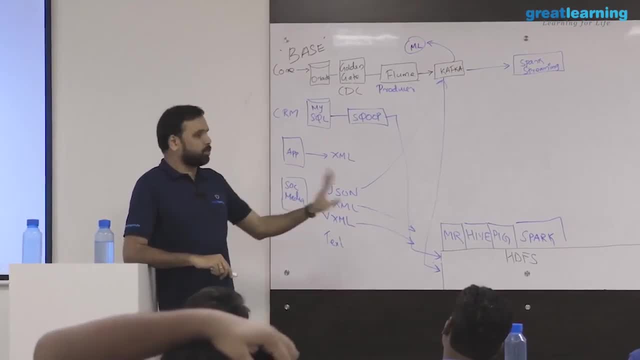 So for the last two, three years 90% of the trainings are on Spark. So when the client comes for a call, they will so previously. for the big data trainings they will say what are the topics you will cover. 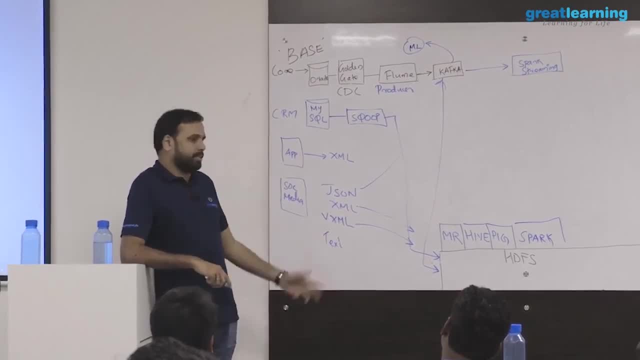 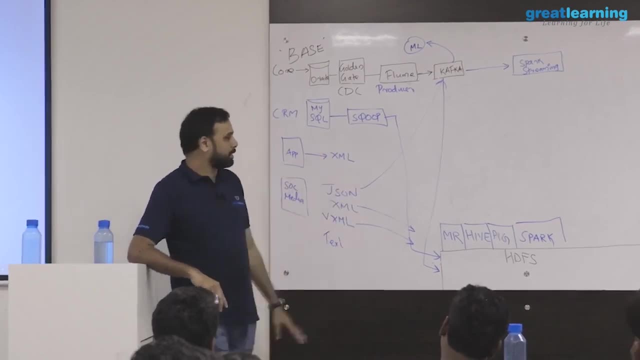 I will say: MapReduce is there, Hive is there, Piggy is there, okay, okay, Kafka is there. So now they will say: are you covering Spark? So the participants want 80% of Spark, Then you can cover other tools also. 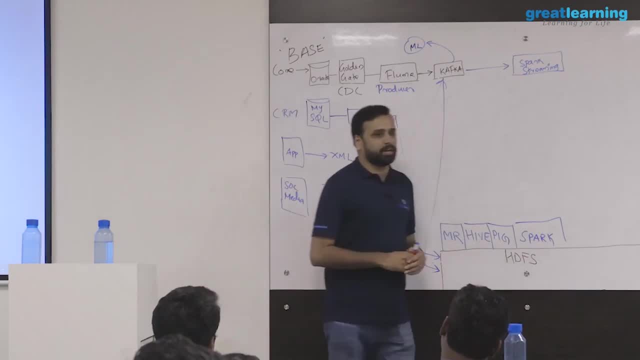 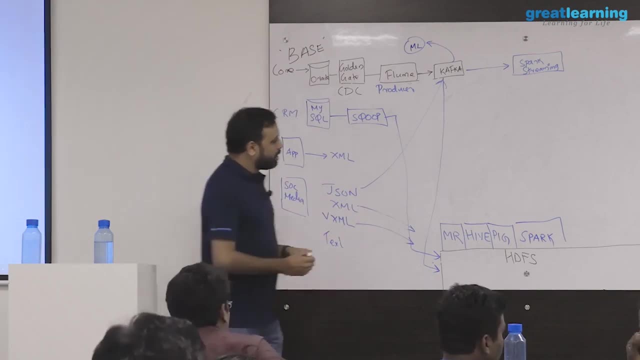 Spark is very popular. actually, these days, Most of my trainings are actually on Spark. It's very powerful also, So it's not just popular, it is very powerful also, right? So these are all the processing engines you can get in Hadoop. 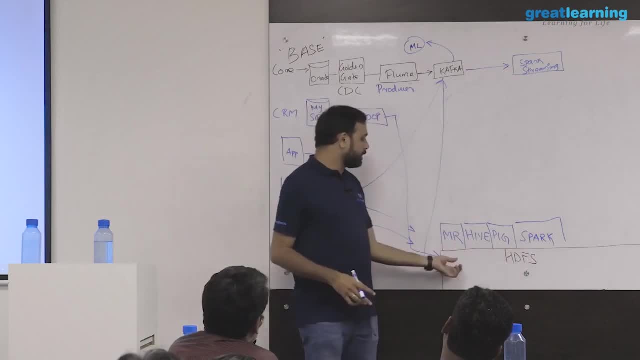 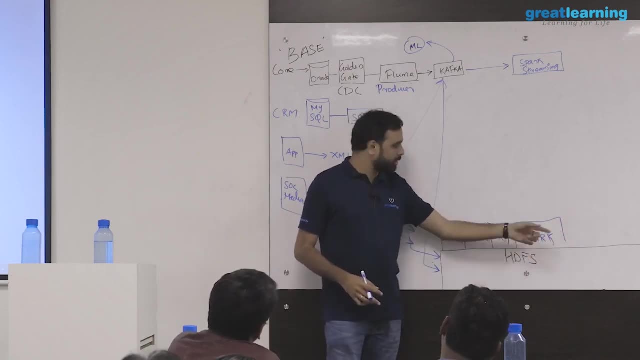 So when you download or get Hadoop, you don't get anything. And then you say that I want to analyze the data using Hive, using Pig, using Spark. There are a couple of more of them, but not so important. These are the execution engines which you know. 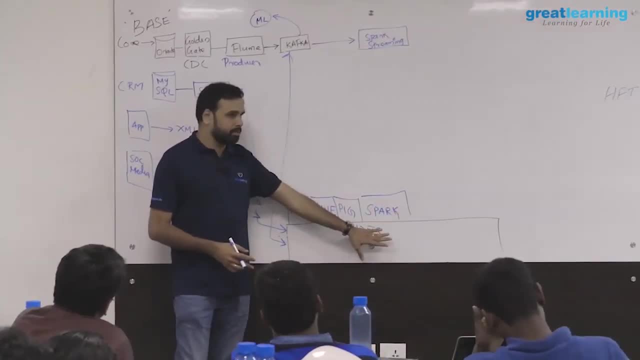 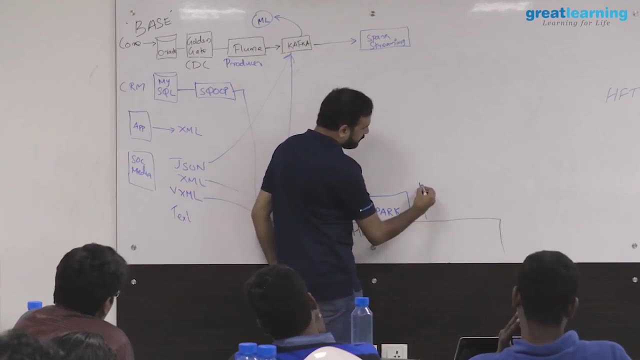 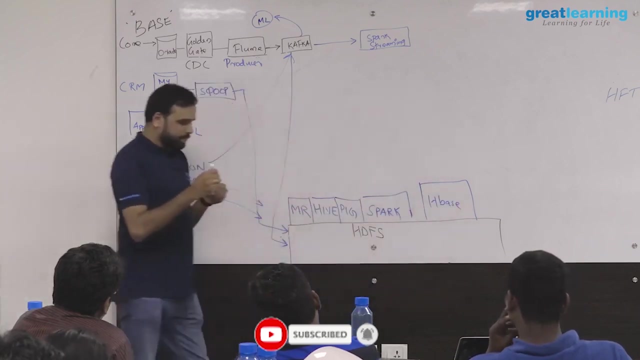 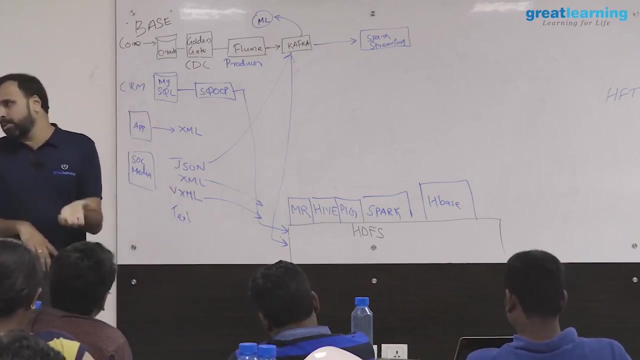 these are the execution engines which you get along with Hadoop normally. right Now there is also somebody called HBase. This is slightly different. HBase is the NoSQL database on Hadoop, the default NoSQL database. So if you want, I will talk a little bit about NoSQL later. 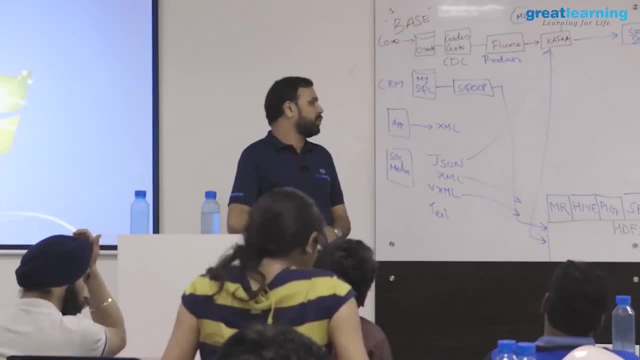 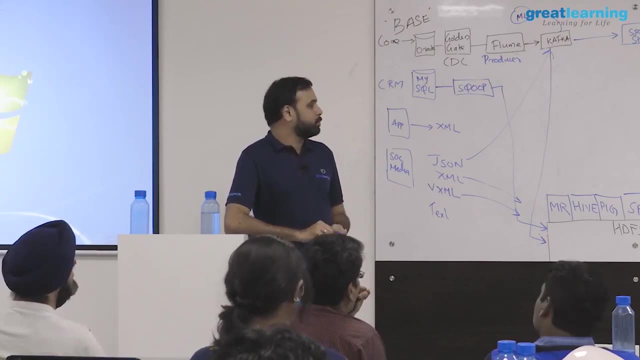 but if you want to use something called NoSQL, then you can use this tool called HBase. HBase is a default NoSQL database on Hadoop And HBase is also very popular. This Facebook Messenger is actually running using HBase. 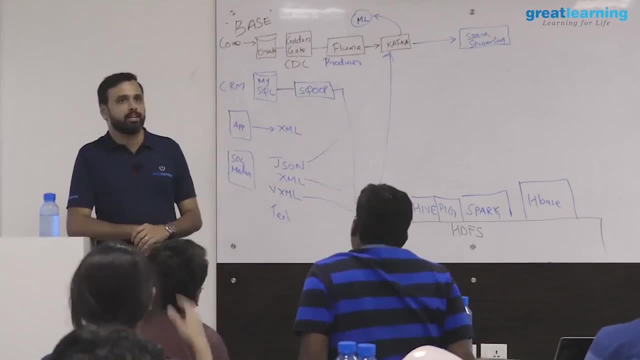 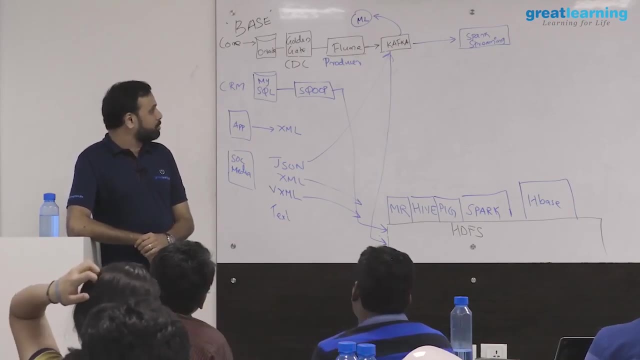 It's very powerful. also, All the messages you are exchanging right. Facebook Messenger that actually uses HBase. It's a NoSQL database- right? I will show you after the break. Another thing is that originally, when somebody say Hadoop, 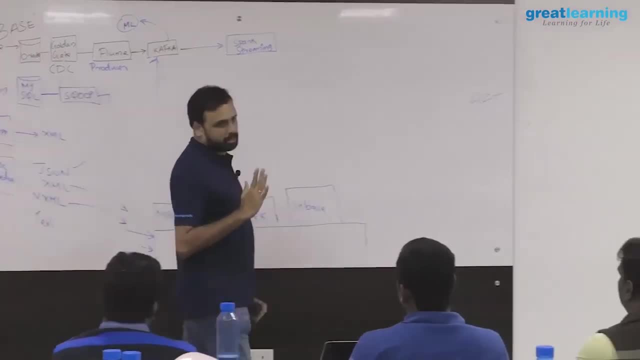 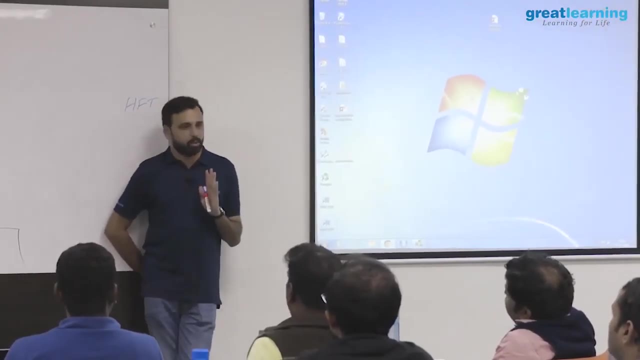 they will say Apache Hadoop. So that's the open source Hadoop right, The original thing which was created, and all. But if you are working in an organization, you will never use Apache Hadoop Because you know the reason. You will never get technical support or anything, right? 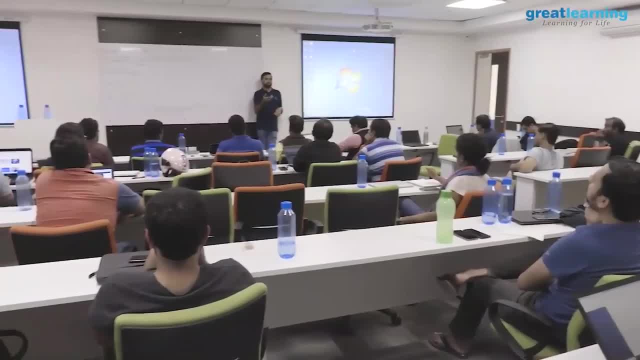 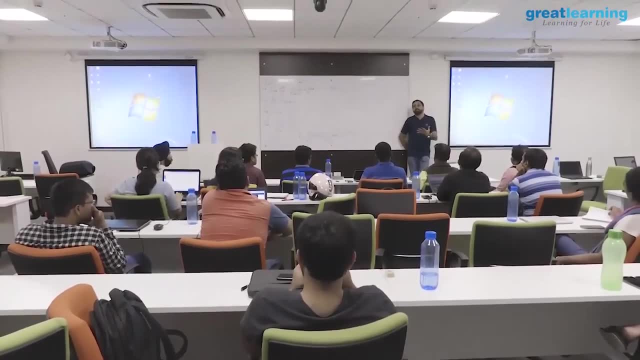 So, like in Linux, you have what Ubuntu right. So you have vendors for Hadoop. So there is companies like Cloudera, Hortonworks, MapR. These are the major vendors of Hadoop. So you go to them and say: give me Hadoop. 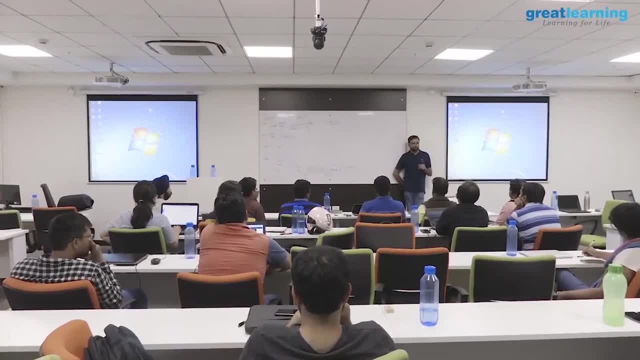 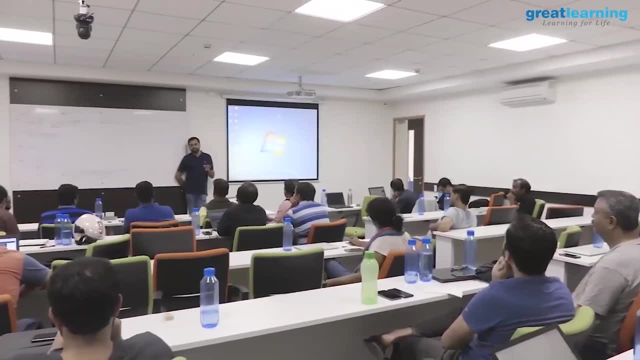 And they won't charge you for license. They charge you only for support. So it is considerably lesser pricing, I feel, comparing the traditional world. No licensing fee, support: they will charge. Permission: they will charge, So they will help you to set it up. 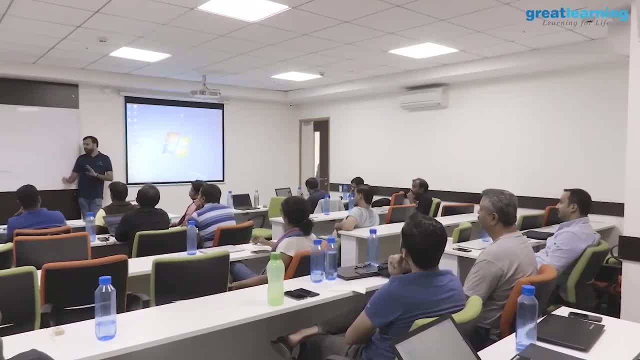 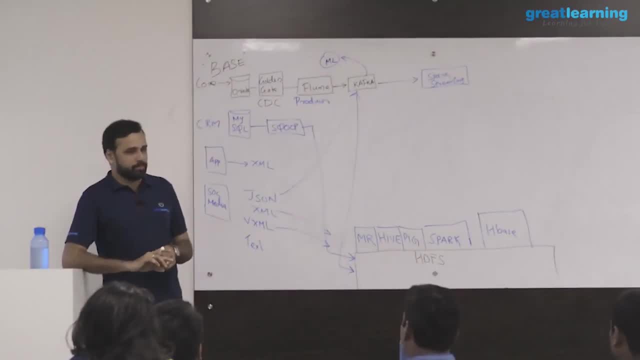 and then run the cluster and all. So any of these vendors you will be seeing. normally when you look at the Hadoop world There is something called MPP- Massive Parallel Processing. So MPP means faster SQL engines And you have many guys in that category. 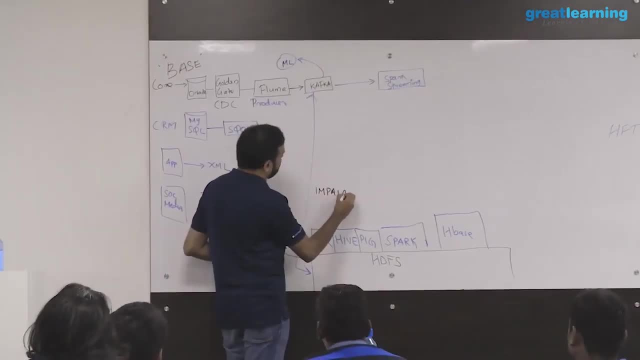 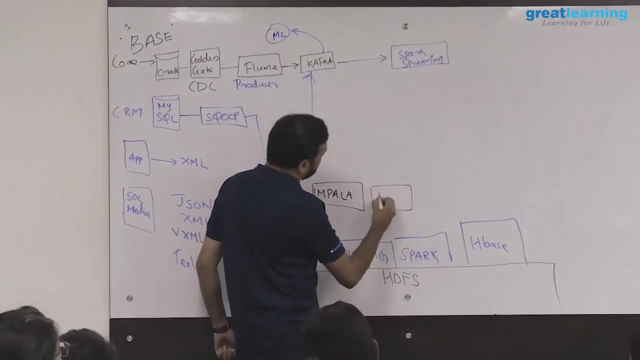 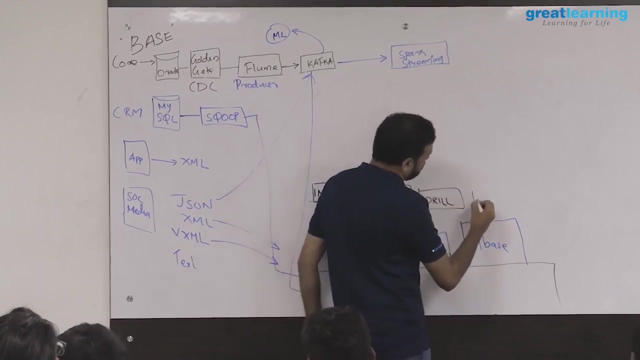 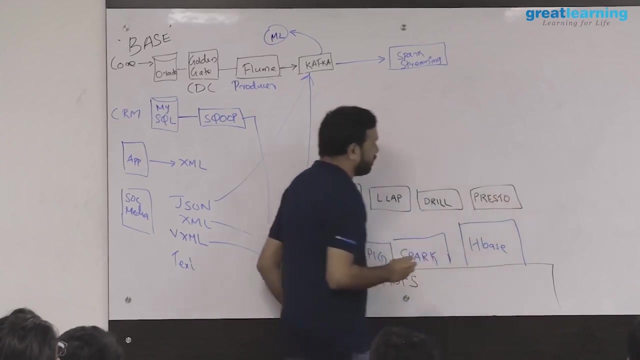 There is something called Impala- This is a SQL engine which is faster than Hive- And there is something called Hive with LLAP, And there is something called Drill And there is something called- what is its name? Presto. So all these guys are SQL engines. 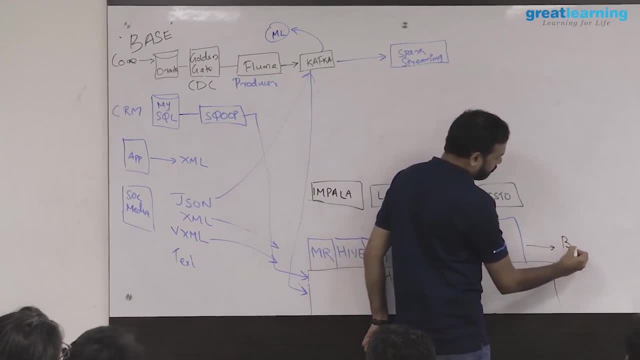 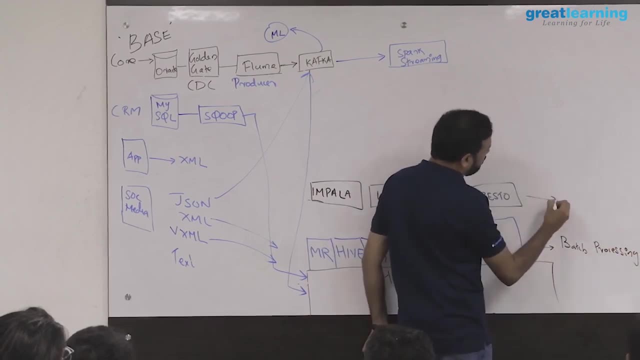 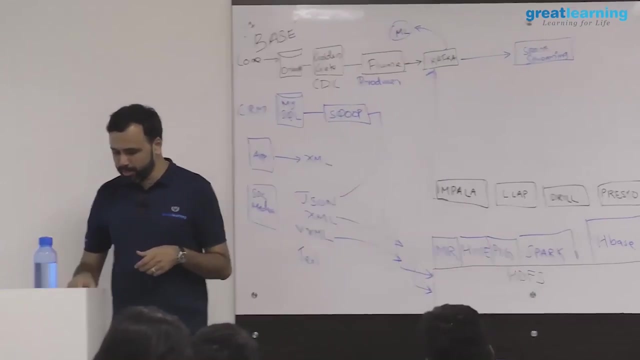 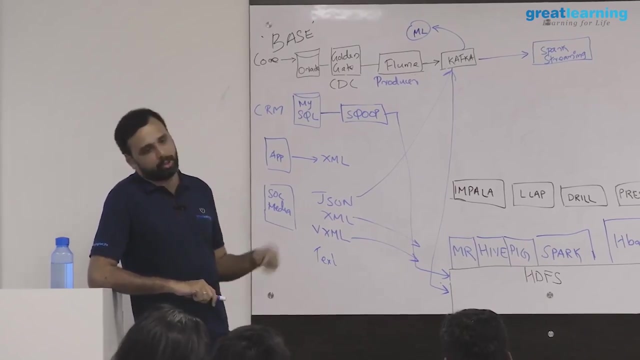 So this is basically batch processing. I can say These are MPP, Massive Parallel Processing, faster SQL engines. you can say So it depends on the use case. There is a definition as to whether somebody should use Impala or somebody should use Presto. 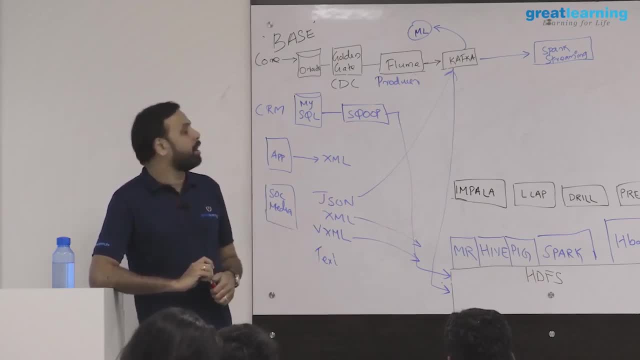 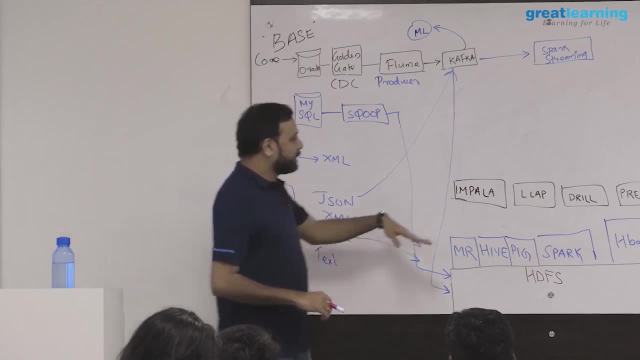 These are all tools which evolved over a period of time, But they allow you to run SQL queries So you can use them. It runs really fast on Hadoop. You can install them, So this is another layer where you can use SQL engines on big data. 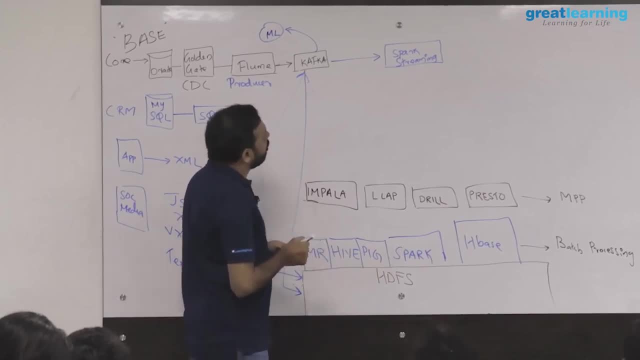 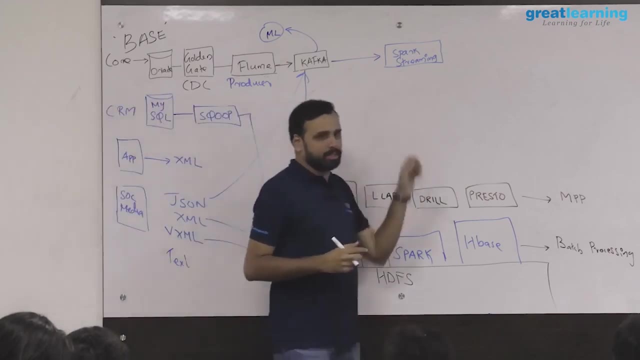 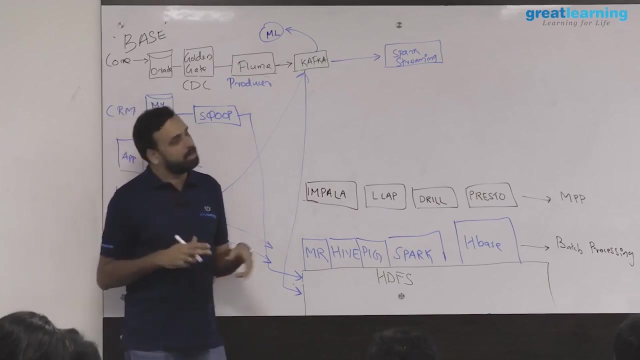 This is very popular. So when you come to this real-time analysis- so I was telling you that there is something called Spark Streaming, which is actually reading that credit card swipe and debit card swipe and then sending the SMS and all So this is done by somebody called Spark Streaming. real-time. 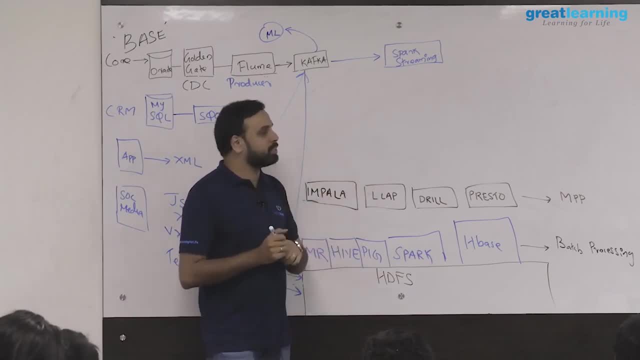 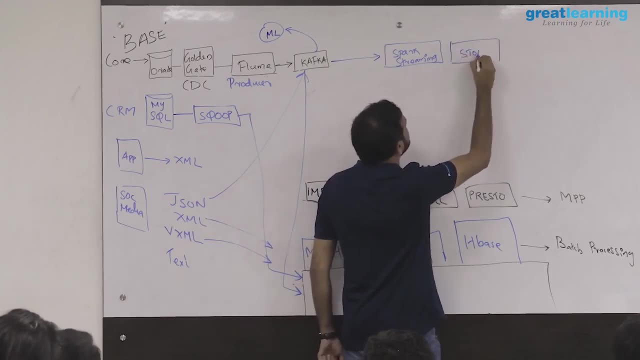 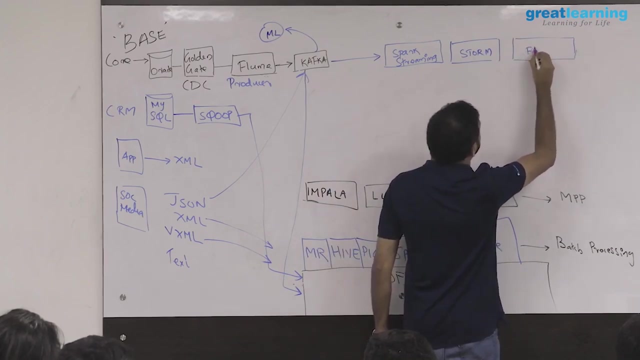 But Spark Streaming is a little bit different. Spark Streaming is not the only platform which does real-time analytics. You have something called, what is its name, STORM. STORM is a real-time analytics platform. There is also something called FLINK- FLINK. 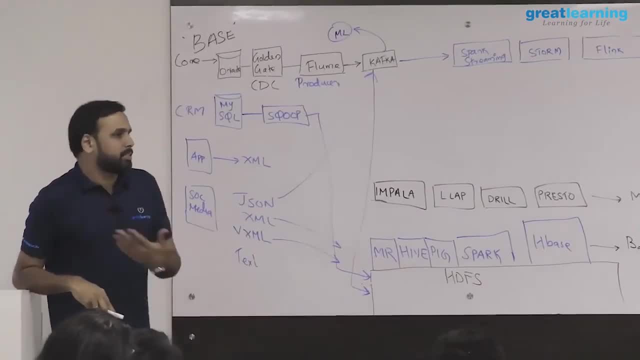 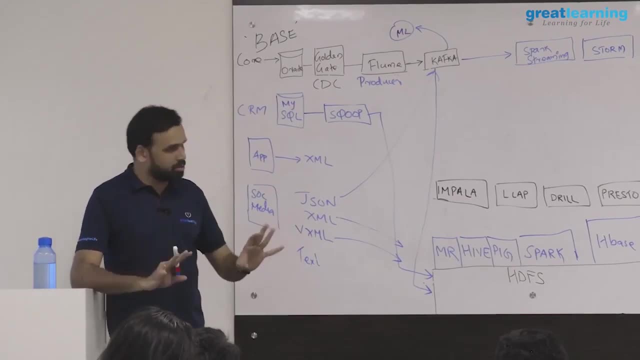 STORM and FLINK are again real-time analysis. So either you can use Spark Streaming or you can use STORM, or you can use FLINK. STORM and FLINK always have alternatives and they have some pros and cons on the other side. 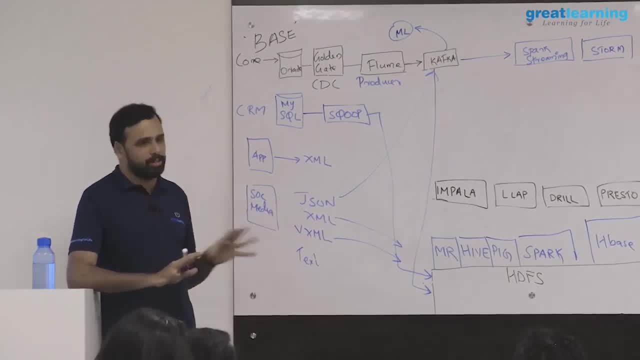 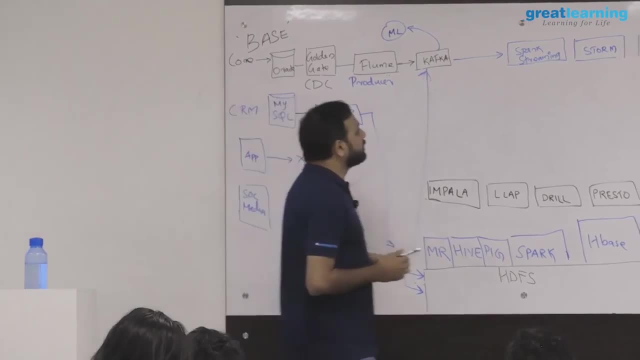 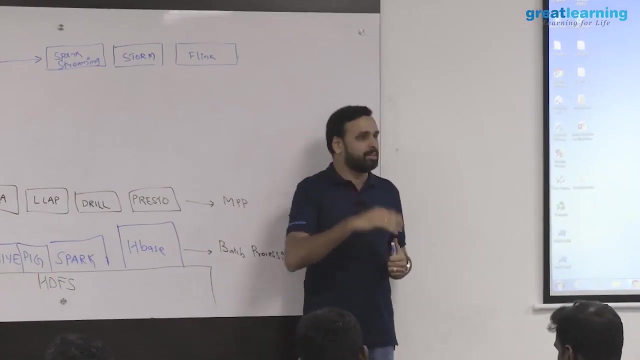 We don't want to discuss right now, but there are some pros and cons over each tool that you are using there And if you are interested in doing machine learning, so that is where you guys are more. So you want to do machine learning at scale, probably in a cluster. you want to use a huge amount of data and all. 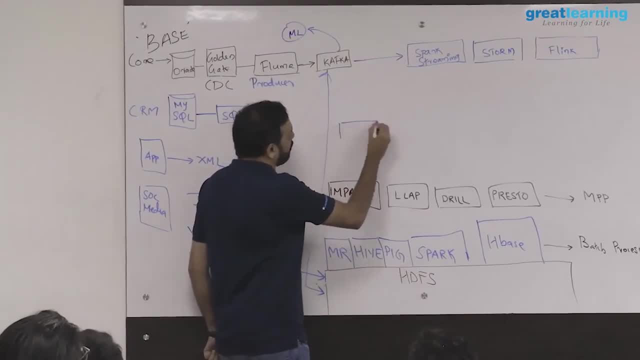 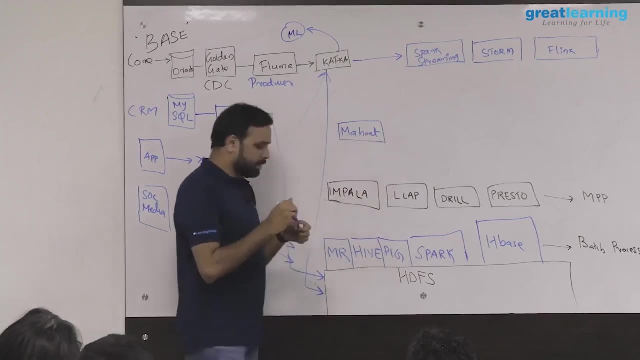 Then traditionally in Hadoop you can do this. In Hadoop there was something called MAHOOT. This is not something which people use now, But MAHOOT is a Hadoop ecosystem project where you can implement all your regression, classification, supervised, unsupervised, everything. 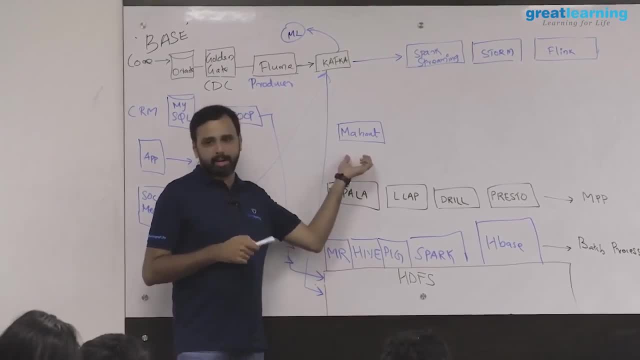 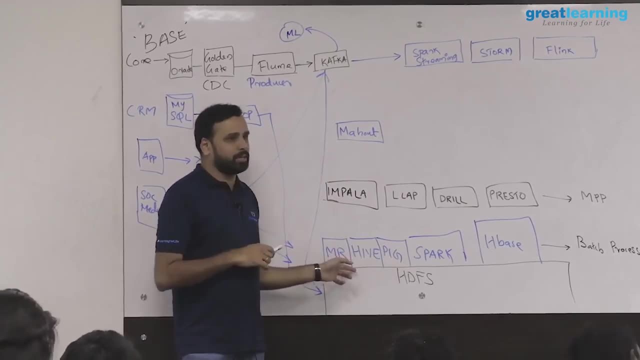 But the problem with MAHOOT is: if you are building a machine learning model using MAHOOT, it is going to internally depend on MapReduce for processing the data, And MapReduce is very slow. You know that, Yeah, Yeah. 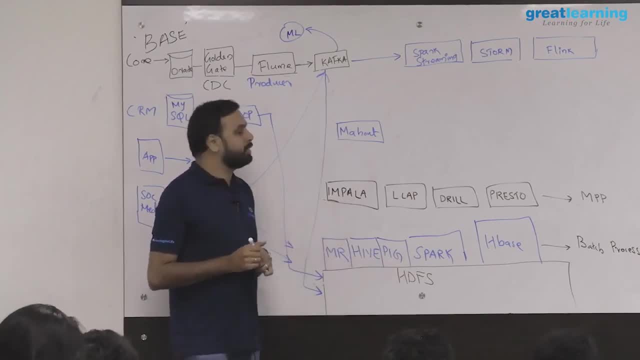 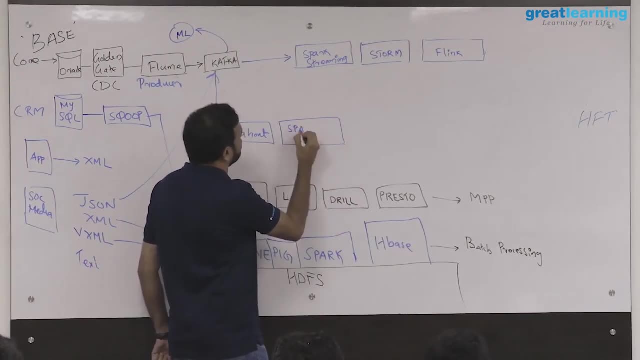 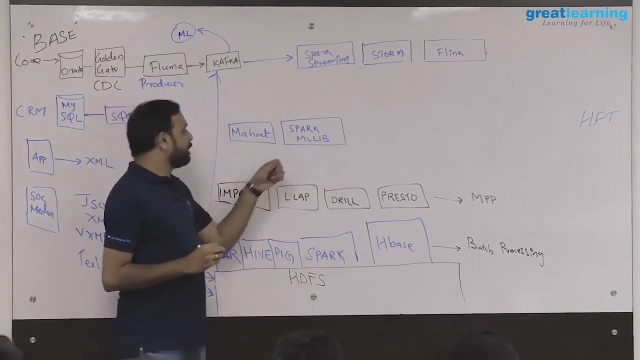 Yeah, So MAHOOT is not really popular these days. These days, most popular is Spark MLlib. Spark has a library. It's called Spark MLlib. OK, So Spark MLlib, our machine learning library, will allow you to build machine learning at scale. 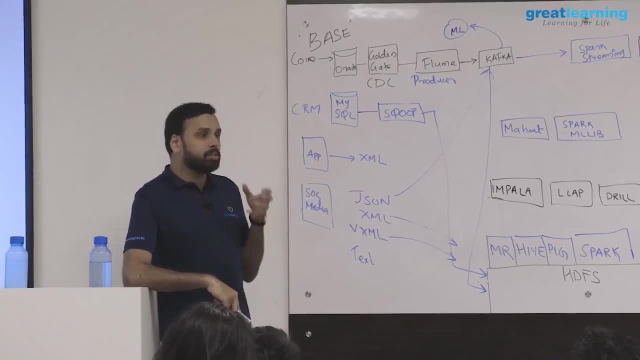 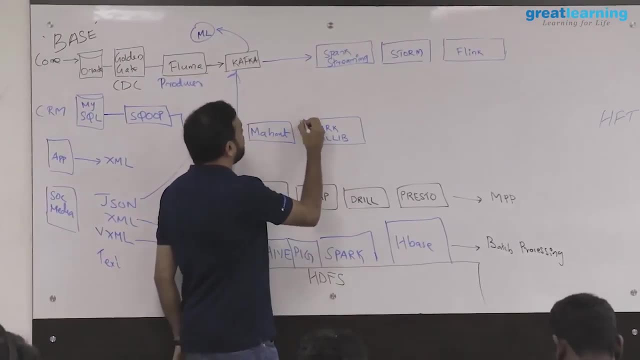 And also it is very fast. OK, And the beauty of Spark is, when you want to use Spark, you want to build it. When you want to use Spark, you can use any language you want. You can build using, let's say, Python, if you want, if you're comfortable. 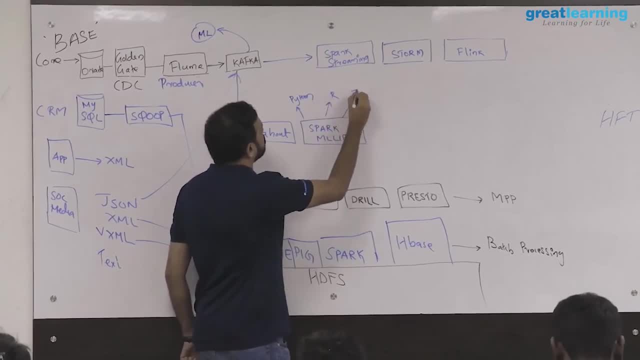 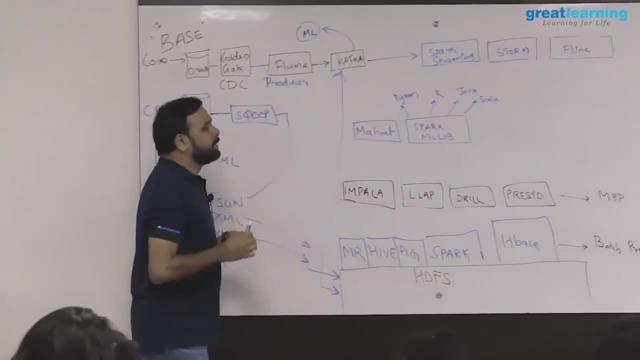 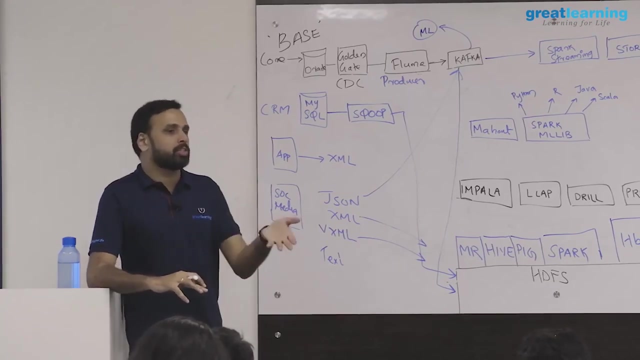 Or you can use R, or you can use Java, or you can use the language called Scala. So one of the cool features of Spark is that Spark allows you to program in many languages. So maybe I think your strong background is R, right? 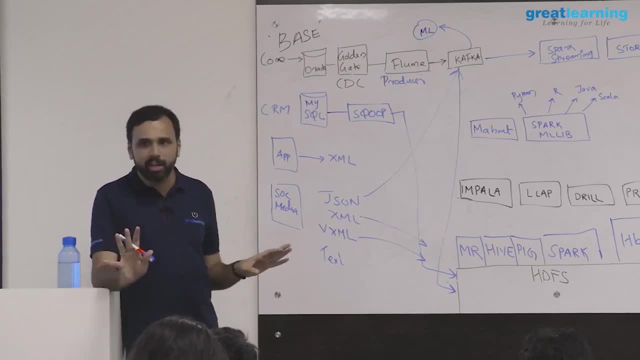 So when you start working with Spark, you can simply say: I want to use R only And you can do everything using R, whatever we were discussing. But maybe another guy is there who is coming from Python background. He can start doing the exact same things in Python. 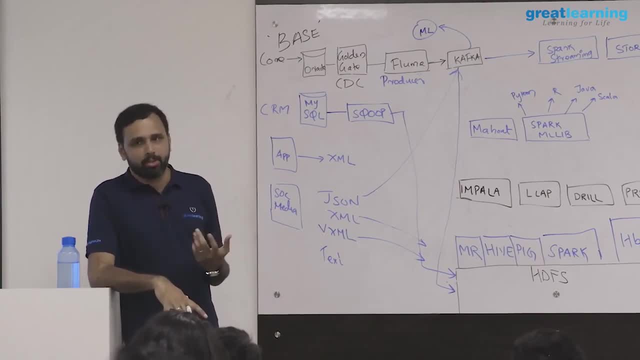 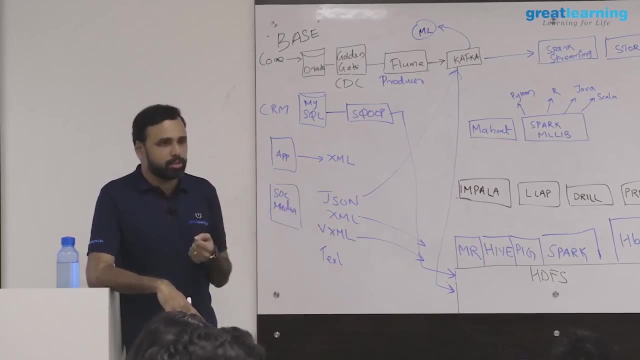 So that language capability is very high in Spark. So, especially for machine learning in Spark, people prefer R over Python. They are very good at it. So you have a Spark R module using that. There is a library called MLlib where you can do. 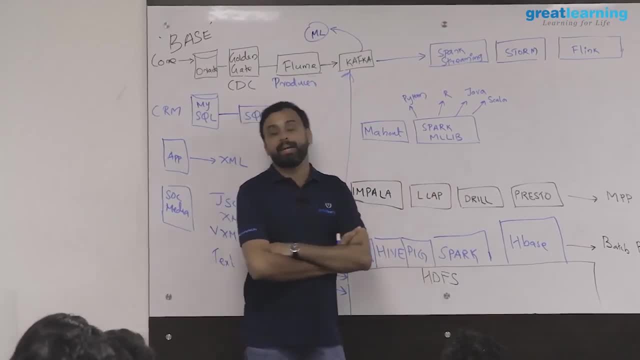 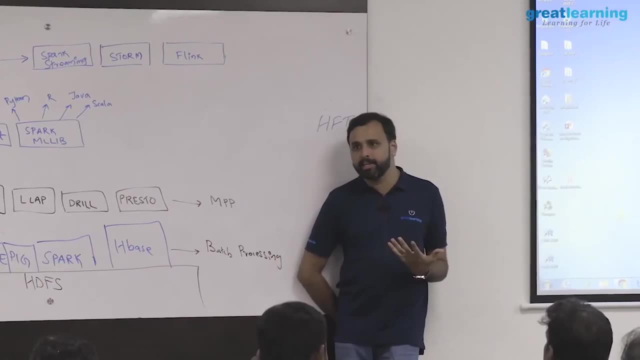 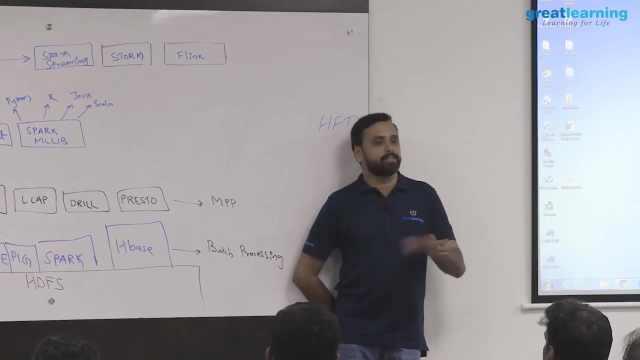 You can do machine learning at scale right. But again, when it comes to the very recent times, okay, a lot of the big data vendors have started supporting machine learning independently, In the sense they will say that you can run TensorFlow. 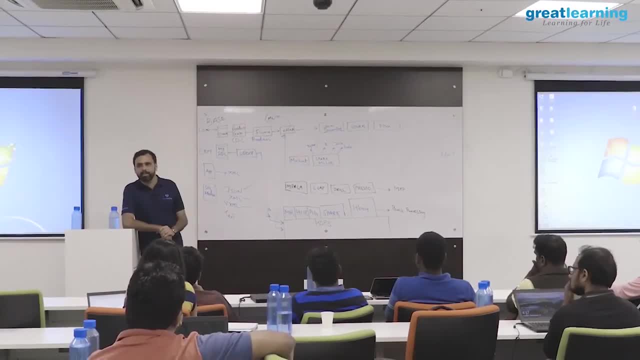 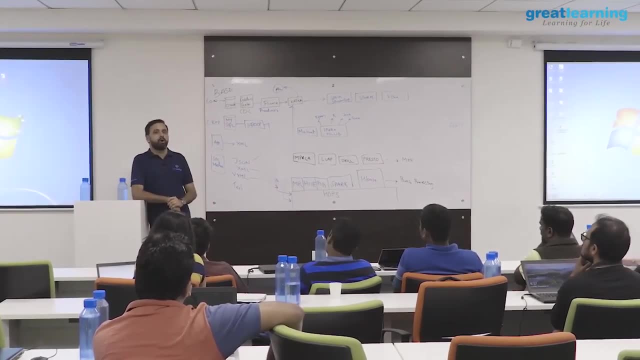 So TensorFlow is deep learning. right, There is a Spark and all are there, but you can independently start running. let's say, TensorFlow on our platform. They support it, right? So almost all the machine learning is supported. Almost all the machine learning libraries are now available on most of these vendors. 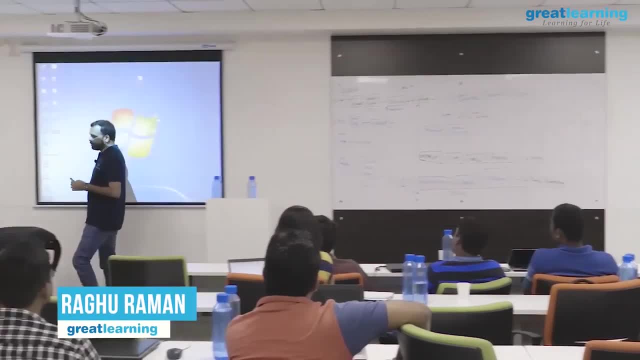 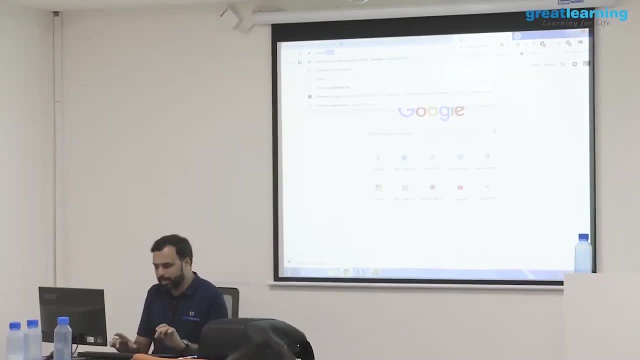 as well. I was talking about these vendors, right? So this is something probably makes some sense to you. So one thing which you can understand: there is a vendor called Cloudera. So there is a vendor called Cloudera, Clouderacom. 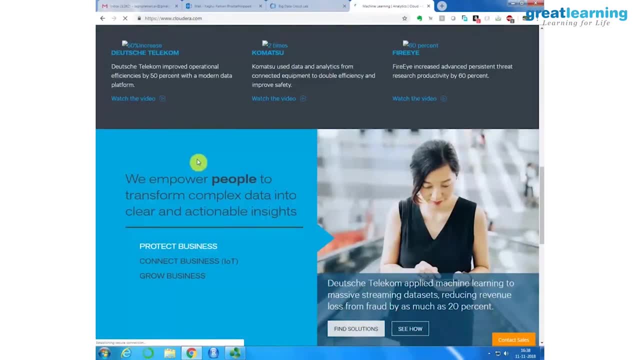 You can see from here, Cloudera was the first vendor for Hadoop. They came in 2008,. okay, And then they started selling Hadoop And, accordingly, most of the machine learning libraries are now available on most of these vendors as well. 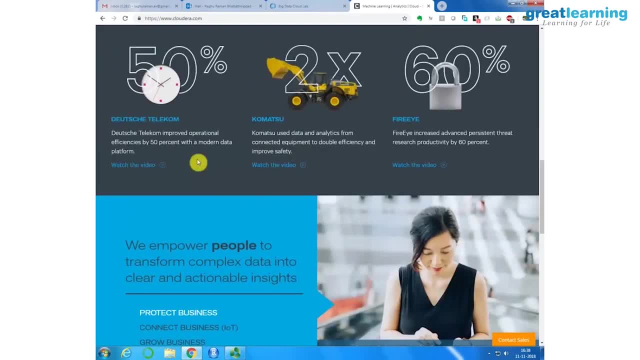 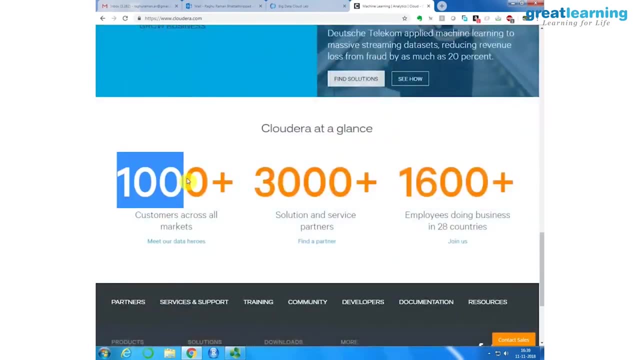 So most of the customers started using Cloudera because they are the first vendor, right? And Cloudera is very famous, probably the first vendor, like I said. So you have thousand plus customers and et cetera, et cetera. 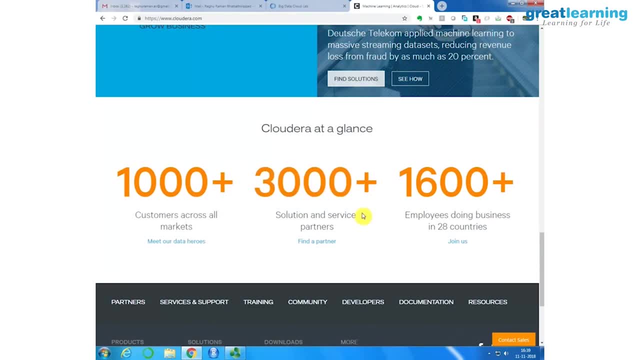 So if you buy Hadoop from Cloudera, like I said, there is a fee for support, okay, And Cloudera sells a modified version of Hadoop. So Cloudera is like Apple, so like proprietary. Okay, If you buy Cloudera product, you are not getting open source. 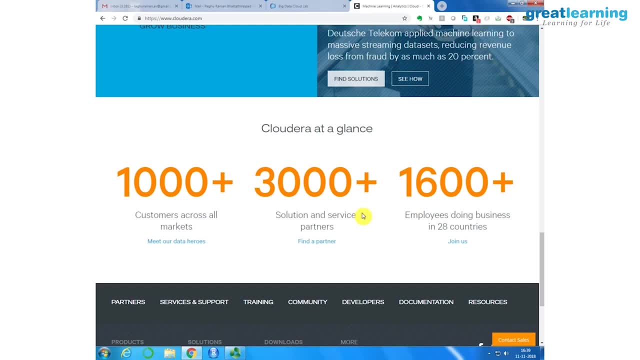 They have their own team. to what do you say? modify Hadoop and all these things speak, spark everything, But they claim it is very stable and all which is in fact very stable, You can use it. So Cloudera is one of the major vendor, right? 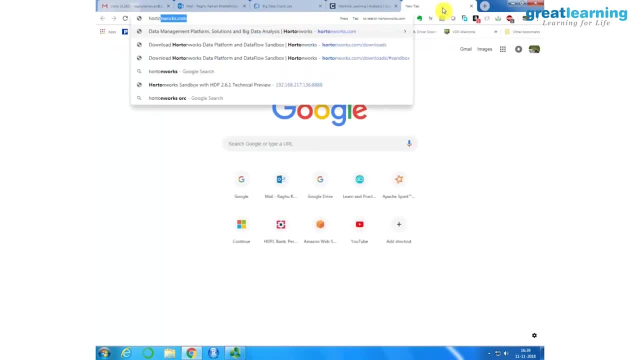 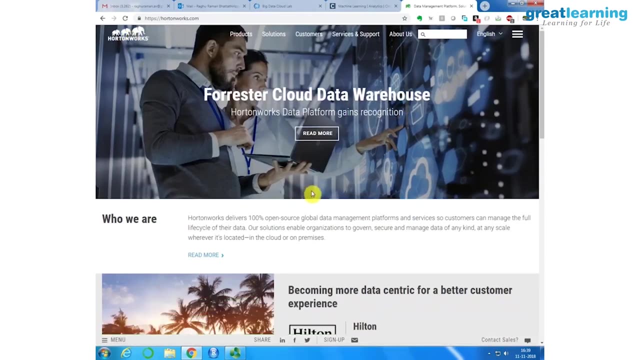 The second vendor, in case, if you are interested, is called Hortonworks. Hortonworks. Can you see here Hortonworks? right, Hortonworks came somewhere in 2008.. Okay, Okay, They started in 2012 or 2013.. 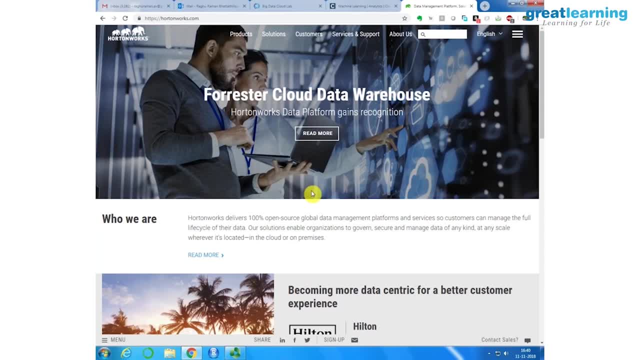 Their speciality is that they are selling open source Hadoop. They don't modify or do anything. Whatever Apache Kafka, Apache Hadoop, Apache Spark, anything, they will package it and sell it to you. So you are getting the hundred percentage original open source product right. 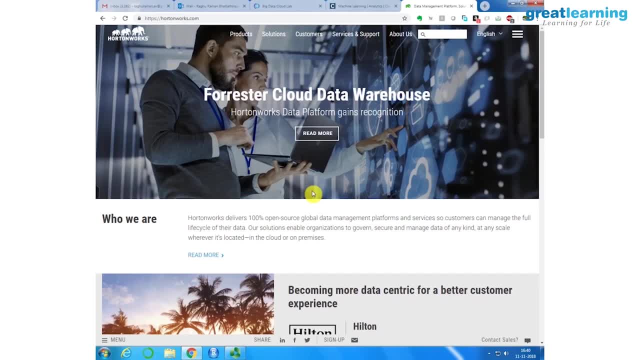 Now let me tell you a bit of history as well. So when Hortonworks came, they became a major competitor to Cloudera, because they were the only company And they were like rivals. So whenever even I go for training, the first question will be that: are you teaching Hortonworks? 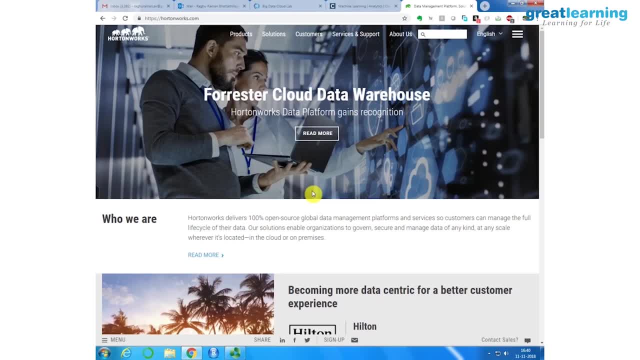 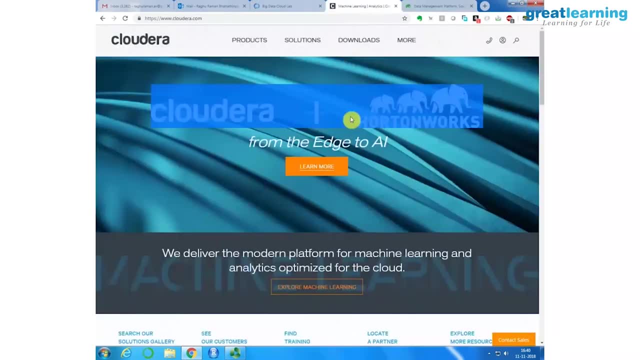 or Cloudera, Because they'll be using one vendor and you have to teach that vendor. So I train on both Cloudera and Hortonworks and it has been like this for first ever. This is like one day Apple coming out and saying that Apple and Android is one. 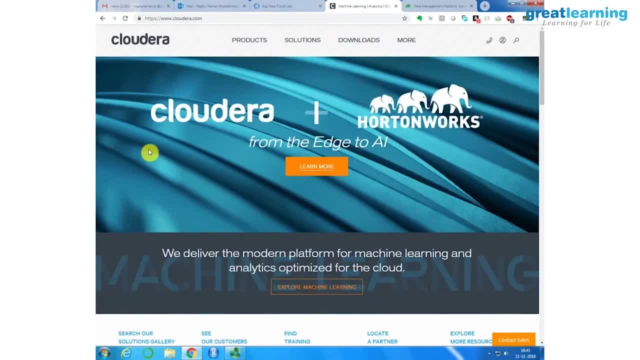 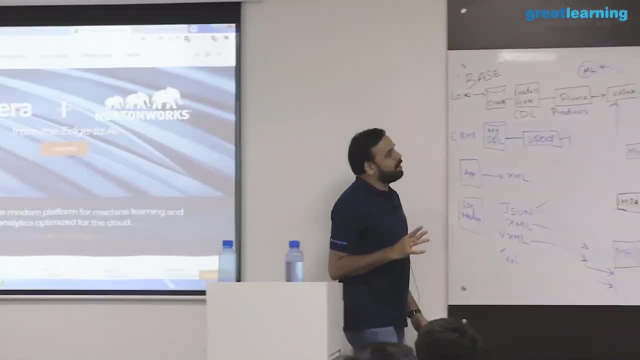 They did, They did, But they didn't meet up. They didn't've an agreement, They didn't have an agreement, They didn't sign anything with each other, and the two companies will merge, in fact, But the merger is announced now. 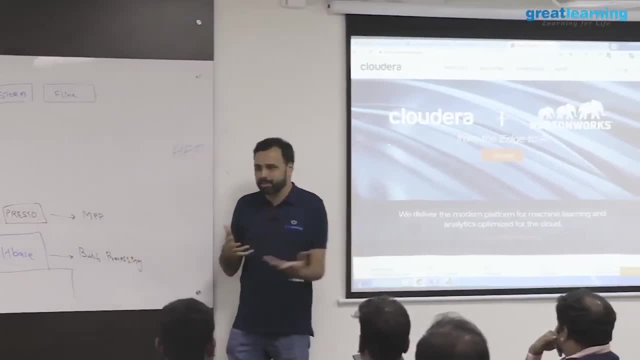 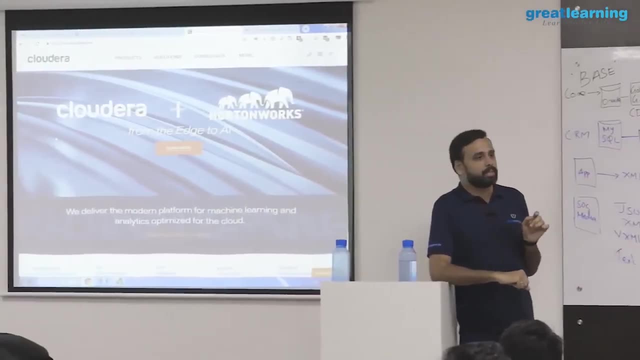 But what is the industry implication of the merger? or why the merger came? Because if there are such rivals, the merger should not happen. It can happen. but why the merger happened? The reason is these two companies were getting most of their revenue from on-premise Hadoop. 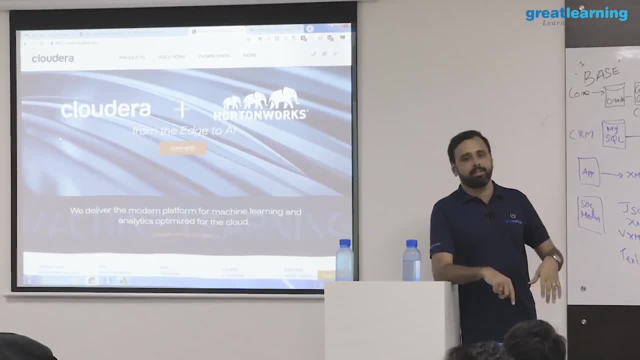 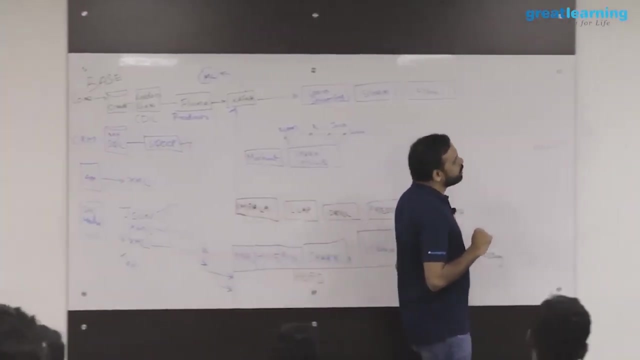 clusters that people will install their Hadoop cluster in the data center or inside their company, so these guys will sell their product. they were getting the money. now the situation has changed. now majority of the customers are using cloud correct, so majority of them migrated to cloud. 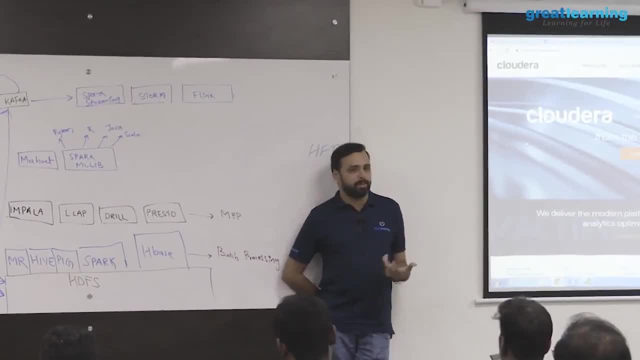 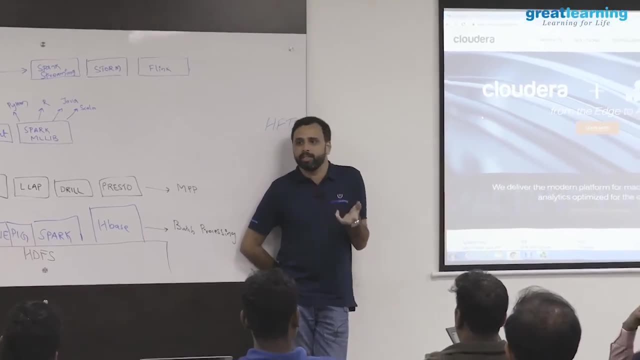 so the amount of money they are getting from on-premises considerably reduced. now. both these companies sell their products in cloud also, like if you are using azure or amazon, you can create a cloud era cluster, but they are not getting full money because most of the money 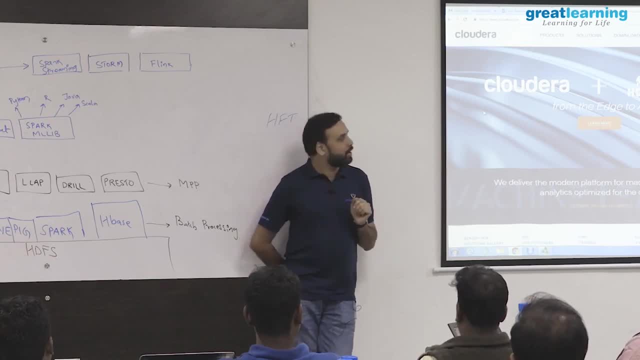 amazon will take. they will get some licensing fee only right now by the merger. what they mean is like they are creating a new product that will be available only in the cloud, no on-premise support. so the intention is to move to the cloud end of the day. so, but that does not mean these are the 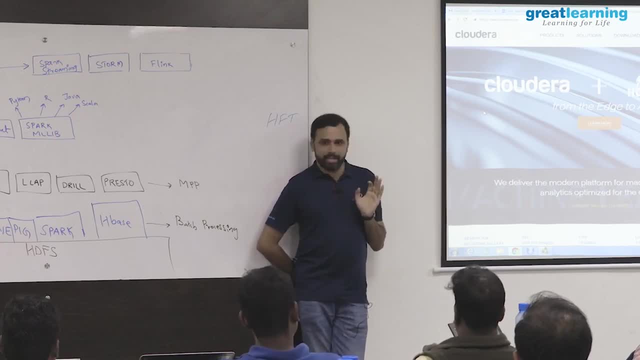 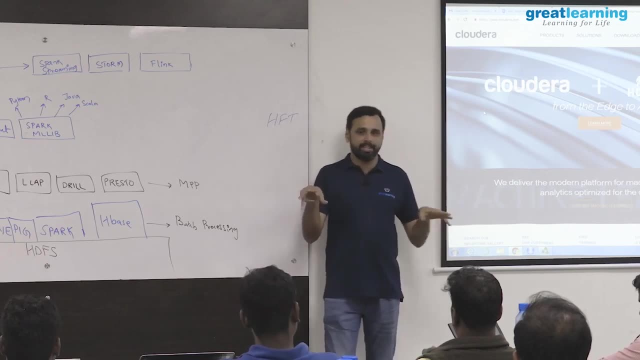 only two companies which are there in the market. there is a vendor called mapper mapper, so map is now the single enemy. so previously there are three companies: hartenberg, clouder and mapper. now these two merged one and mapper became a single enemy. right mapper is available in the cloud and 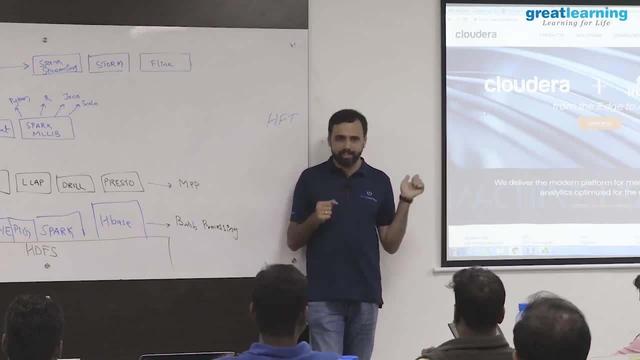 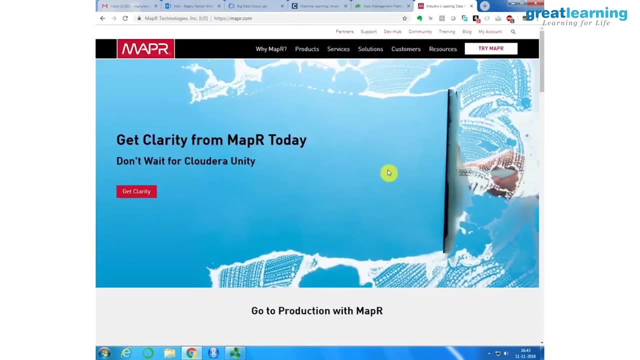 on-premise as well, but that is now the only major competitor to these companies. they actually had a very interesting home page for the merger. they had a halloween costume and all, and then they were saying that there, so don't wait for cloud, no, not, this is very nice actually, but they were. 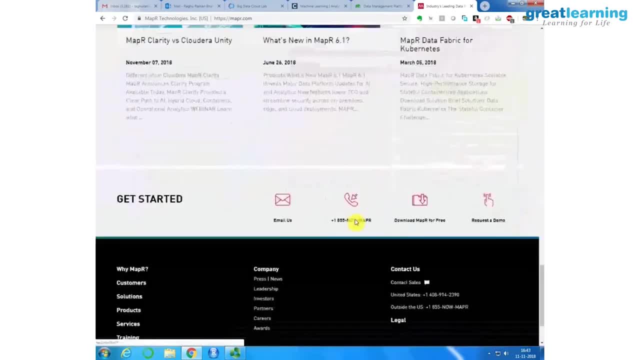 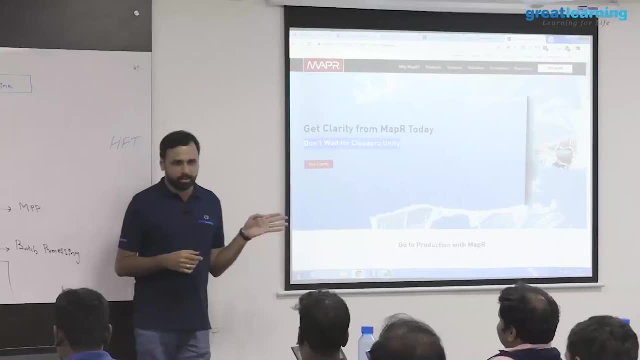 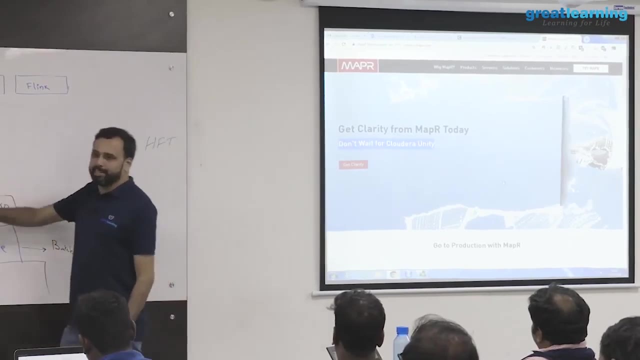 showing actually a very interesting web page. i don't know somewhere they had, but mapper is. mapper is basically an indian company in reality, right? so they are now the only threat to this vendors, because whenever you go for any of the big data platform, you have to trust a vendor. you're always 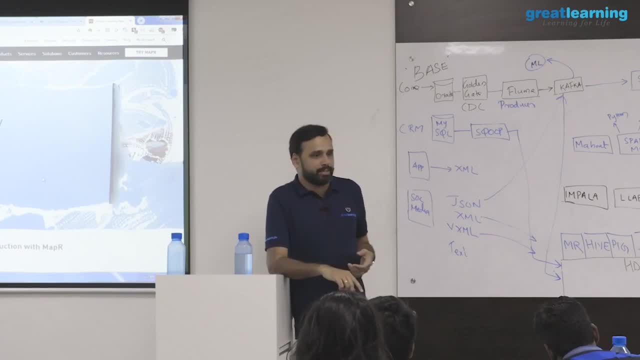 but this merger does not mean that tomorrow they will start selling the product. they are saying another three, four years it will take to build a product and sell. so far, everybody still on hartenbergs and cloud era to find out. merger is still going on because 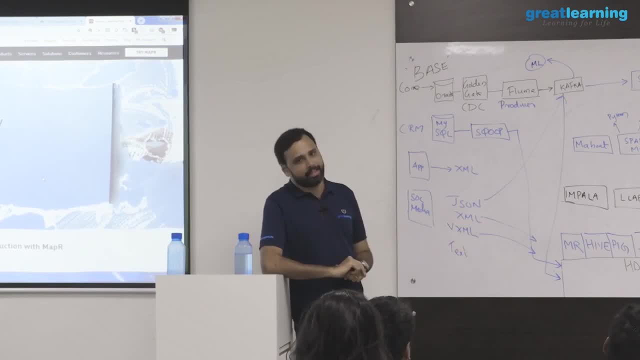 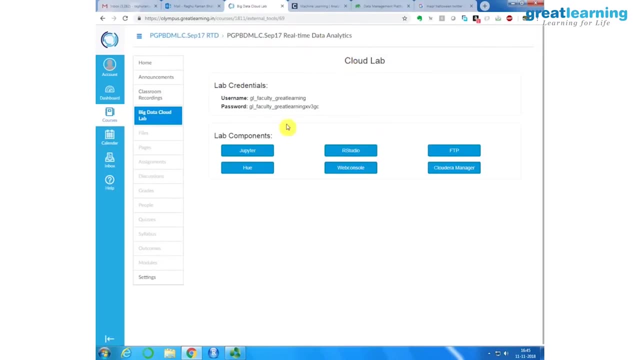 merger happened but still now mapper is on the cloud on our on some dates offered by einesco or some title: Bean Hog beğen zien. they are independent vendors. So this is the big data lab that we have in great learning to teach the big data course. 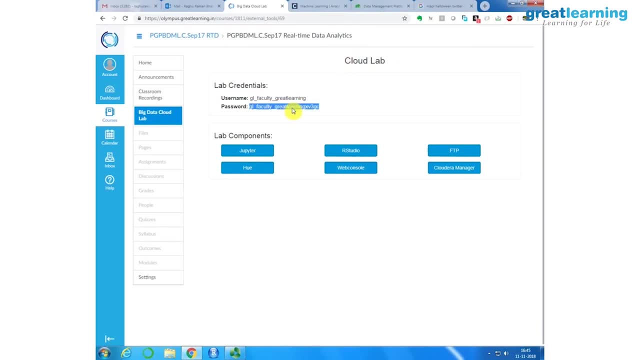 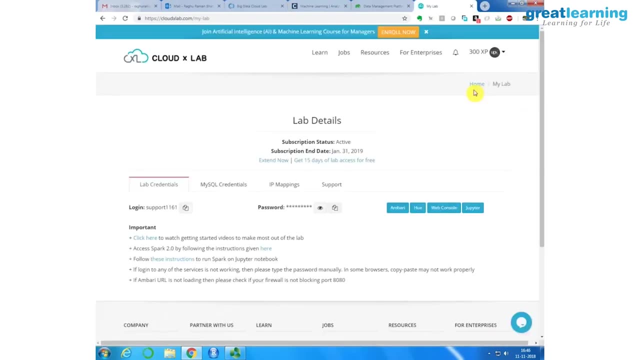 And this is a cloud lab, but as good as like an on-premise lab And this is running cloud data. Okay, and if I have to just show you, this lab is actually on Hortonworks And if you want to see the cluster. 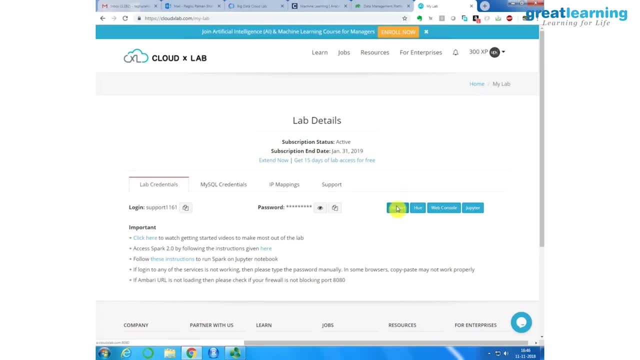 there is something called Ambari. can you see? Ambari is the administrator's tool for managing a Hadoop cluster. Like you want to add a machine, remove a machine, add user. the admin will be using this UI called Ambari. 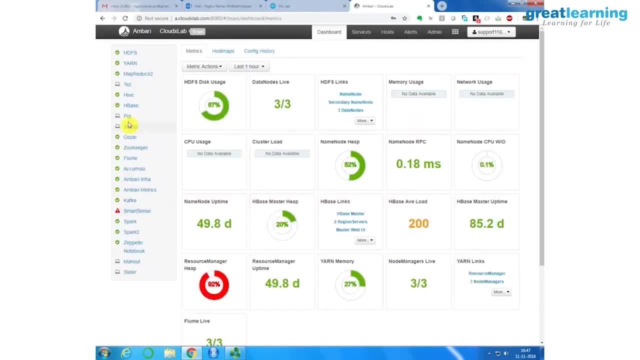 So I can just go to Ambari. So this is a UI to the cluster. Can you see? on the left-hand side There is HDFS, MapReduce, Hive, HBase, Pig Scoop. I'll tell you what is Uzi and Zookeeper. 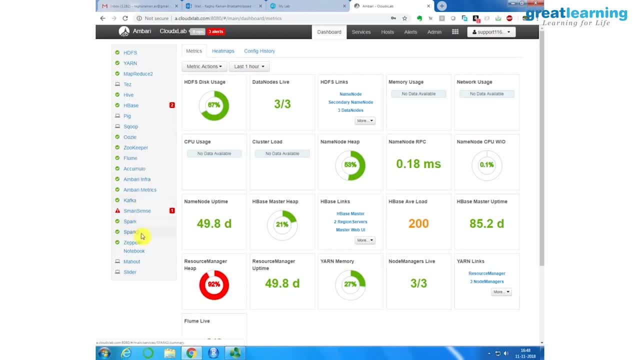 Flume, Kafka, Spark, Spark 2, Mahout Zeppelin, Mahout, Mahout is machine learning right. So all this is installed. It's a cluster. You can see three by three, There are three machines in this cluster. 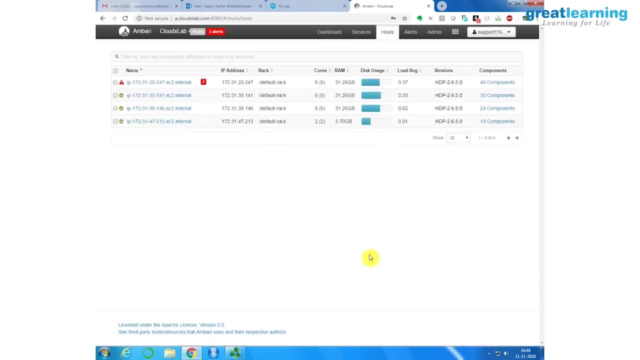 It's a lab, So I can just go to the host menu. And these are the three machines. There are four machines. One machine is down- this guy, I don't know why, But remaining three machines are active. This is their cluster. 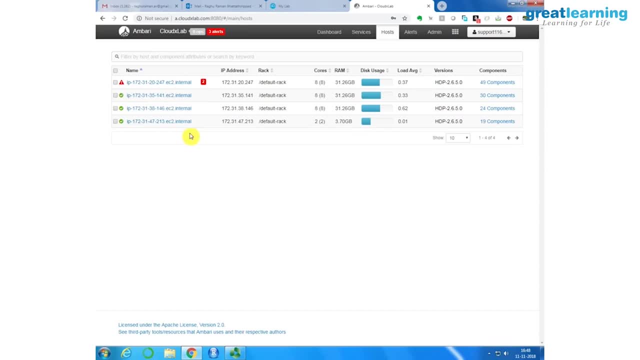 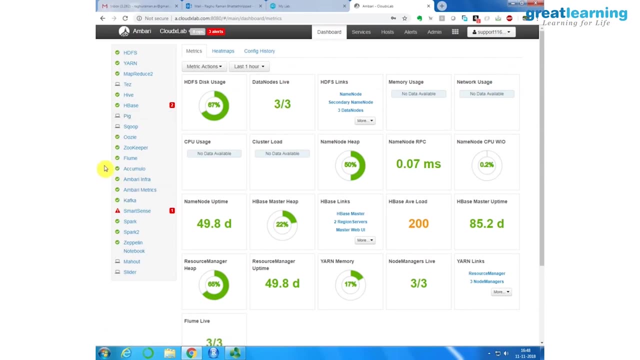 This is just a lab for practicing. We use for a lot of courses and all. But you can see, all these services which we were talking about is installed in this cluster. I think I did not. we used to speak about Uzi and Zookeeper. 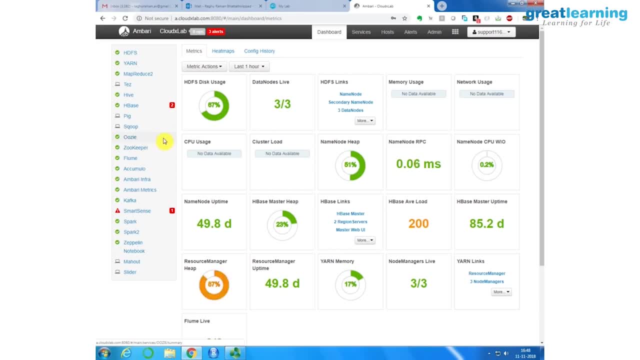 Uzi is a scheduler, workflow scheduler. Like, let's say, you want to run a program every day at 10 o'clock, scheduler, typical lab. So that is Uzi. Zookeeper is a coordination service. It is used to coordinate all the services together. 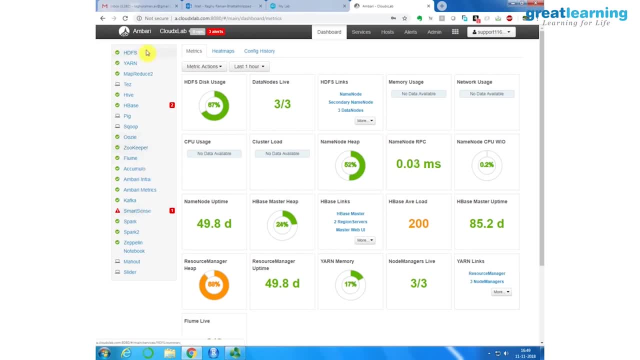 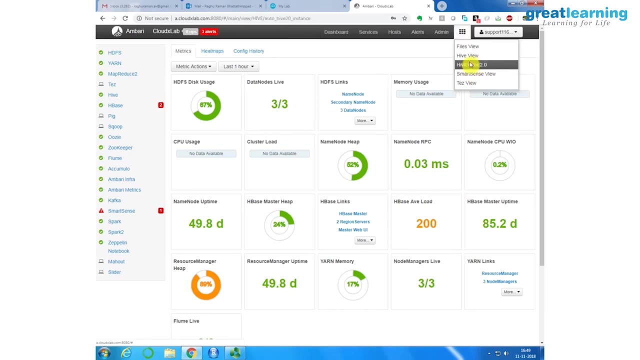 So more or less like an admin thing, And Ambari, like I said, is the UI which we use And you can see the host and all, And here you can actually access Hive and all. For example, there is something called Hive View. 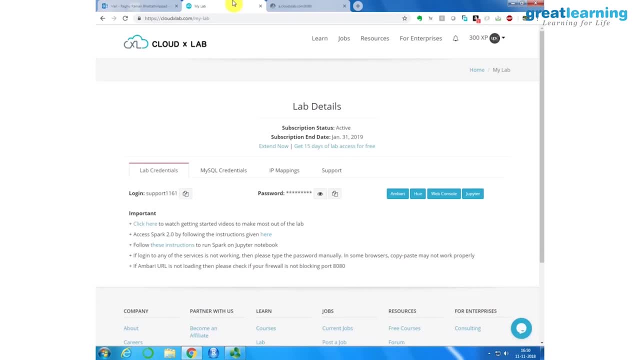 So when somebody want to work with the lab right, Or when somebody want to actually run some analysis or something, they will not be using the web UI. You can use the web UI, but in companies and all, they don't allow you to use the web UI. 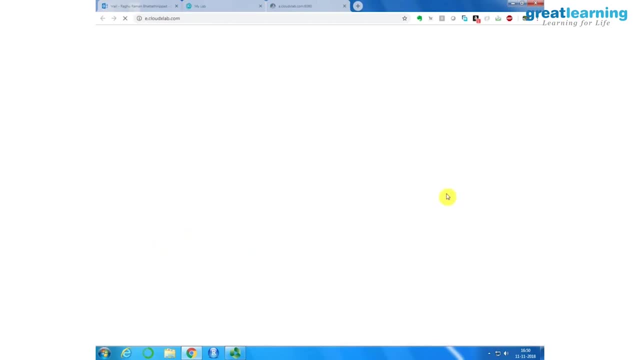 That is when you will be using this command line. So you actually has a web console And just click on this And I can connect with one of the machines in the cluster. Let me just show you. Yeah, so I just logged into the cluster. 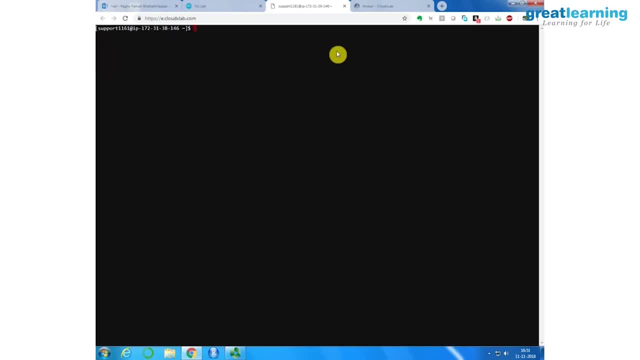 So I'm actually on one machine, but part of the cluster, And I told you that Hive is the SQL engine, right? So if I just want to use, I can simply say Hive and it will start Hive Shell for me. So Hive is actually having an interactive shell. 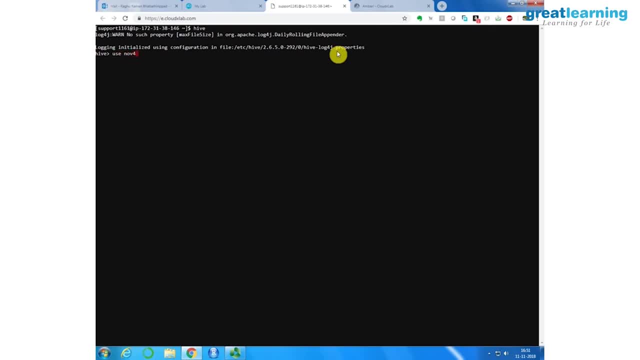 So this is Hive Shell And I can simply say: use November 4.. Now, this is the Hive Shell. This is the Hive Shell. November 4 is a database I created. okay, And this looks like typical RDDMS. Then I can simply say: show tables. 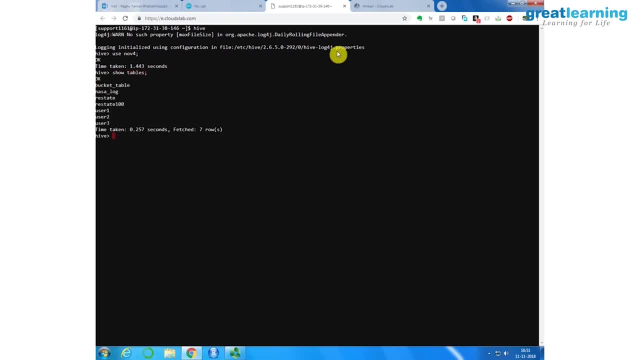 if I want to see all the tables, These are all the tables I have, And if I want to query a table, I can simply say select. it says select, count star. So I just want to know how many rows are there in the table? 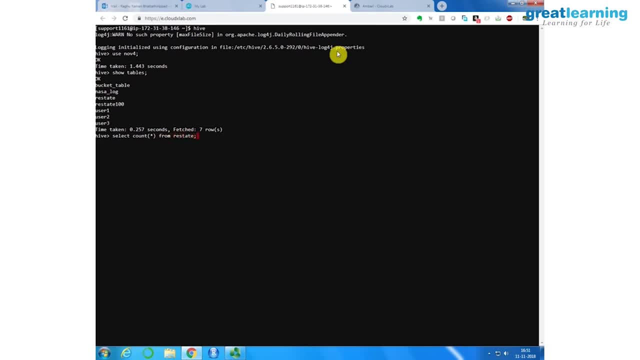 Select count star from re state. So this is the query I'm running and you will see if I run this query. it will convert this query into MapReduce program. This is actually a MapReduce job. How do I know? It will show MapReduce two faces. 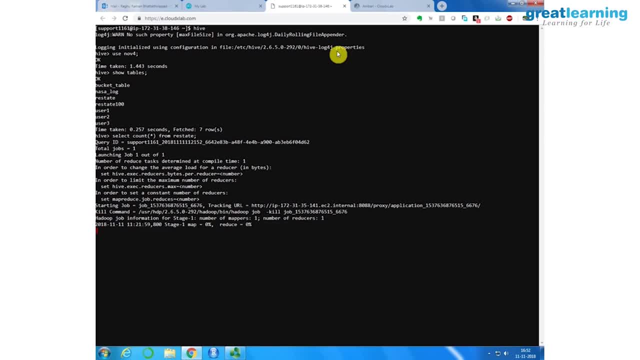 See Map zero, reduced zero, it comes Should start with the MapReduce job, actually, And Map 100, reduce zero, And then it will do over Map 100. And this is the answer. So even if I write a simple query like this here, 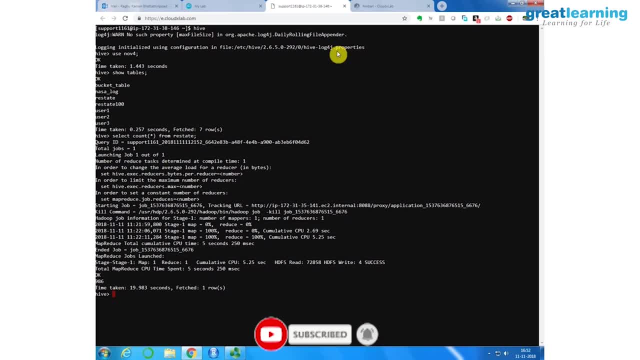 it will convert to a MapReduce job. and convert to a MapReduce job and run it, and then only I'll see the final output is here: I think 686 or some number is there right? So all the hive queries actually gets converted to. 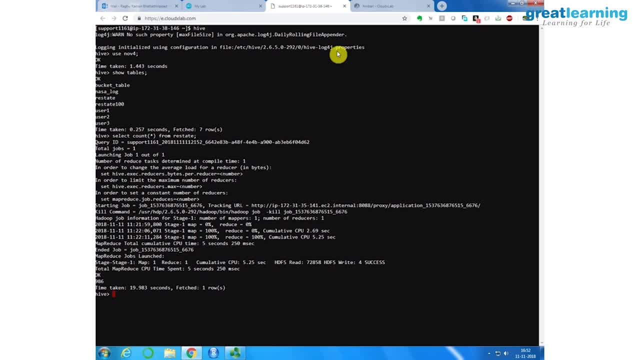 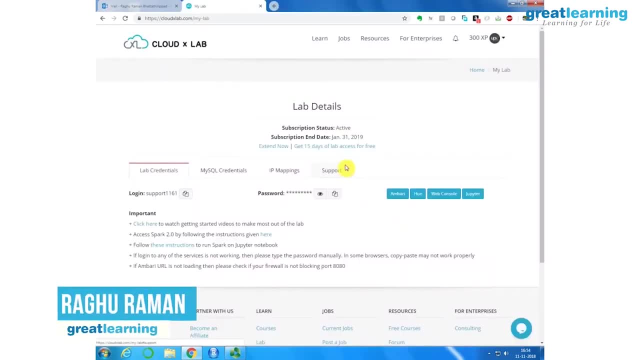 so it's very slow, right? So normally in a RDBMS, if you run this query within a second, you will see the answer, but it is slow. Maybe it is MapReduce. it is expected to be slow. CloudX lab is actually a Bangalore-based startup company. 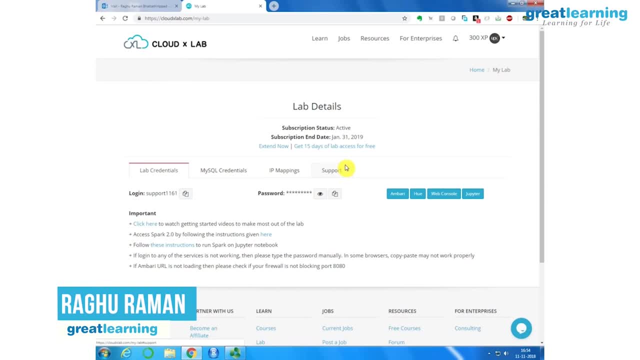 So what they do? they have a cluster, They sell it to students to learn, Like, if, let's say, I want to learn big data, I can pay some money and they will allow me to access. So from anywhere you can connect. it's very easy, right? 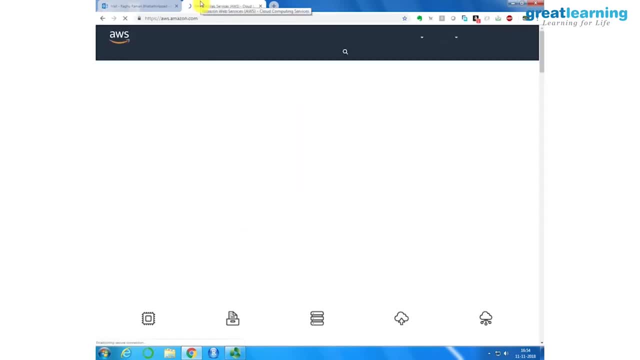 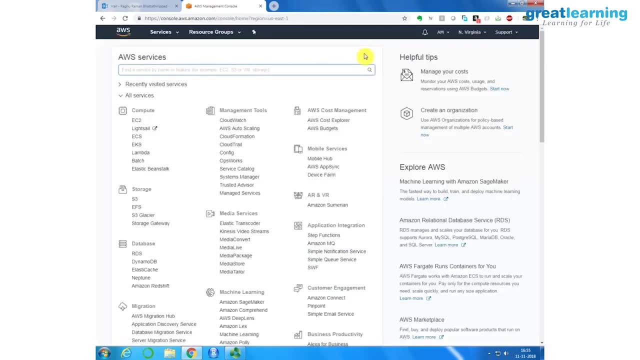 If you have a browser in Amazon, So I will just log on to AWS Amazon Cloud. okay, I just want to show you one small thing. Yeah, so this is basically the Amazon's homepage where you can see all the services are listed, right? 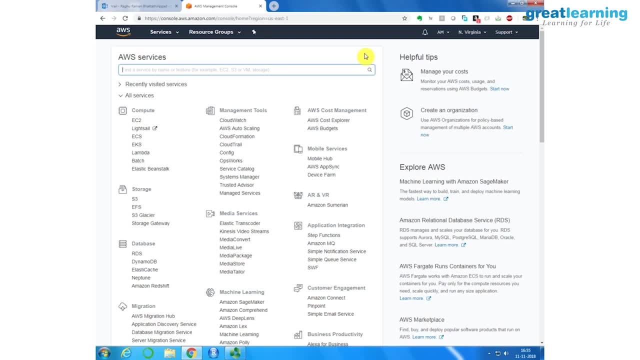 And we are not interested in all the services. right, We are particularly interested in Amazon, but we are also interested in big data services. So Amazon has a service called EMR, So you can simply search for EMR here. So Amazon has a service called Elastic MapReduce. 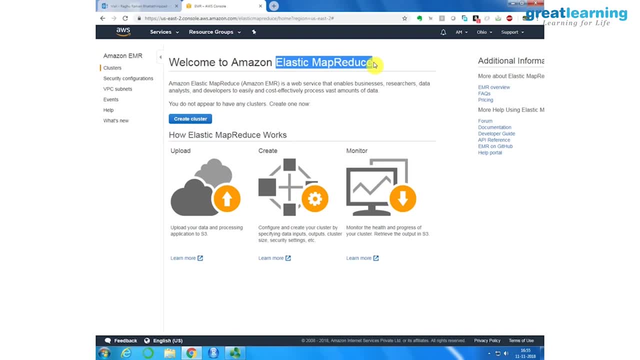 Well, the service has the least to do with MapReduce. They're just calling it as Elastic MapReduce. okay, And this is particularly a very, very useful service these days. Many organizations, like I said, are using this service. What is this service? 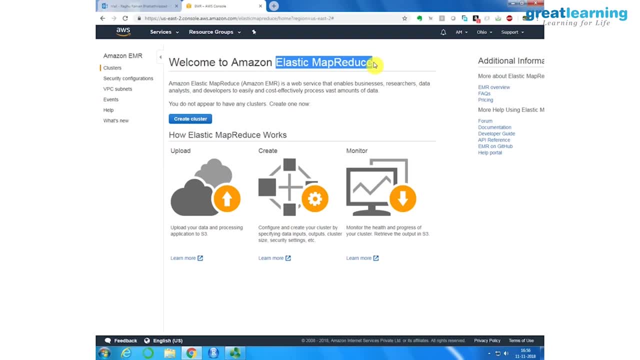 It will allow you to create a big data cluster on the cloud within five to 10 minutes. So if somebody want to create a cluster, then analyze some data and then delete the cluster. thereafter you can set it up. It's very easy to do. 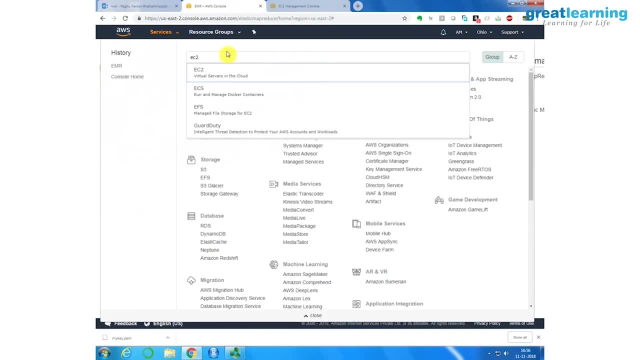 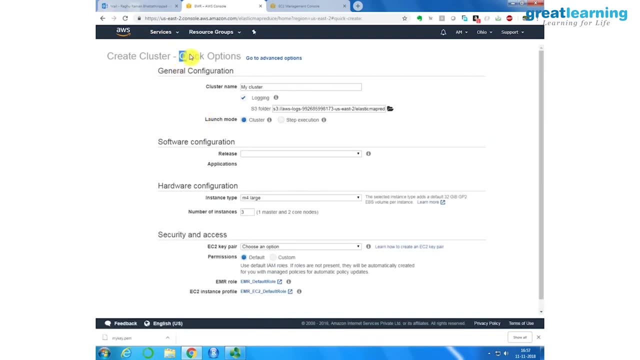 So all you need to do is that click on this create cluster. So what you need to do is that, if you have landed in the EMR page, you can click on this create cluster, okay, And by default, you will land in something called create. 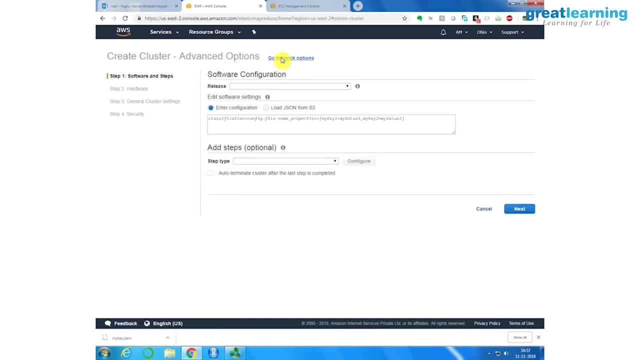 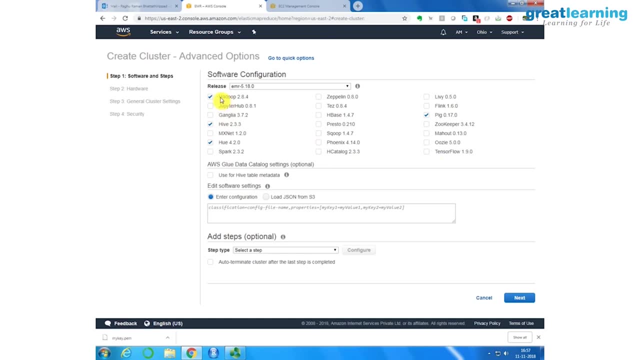 So click options. You can click on this advanced option right And you can see what tools you need to install. in the cluster, See, Hadoop is by default picked. So you are getting Hadoop version 2.8.4,. you will get. 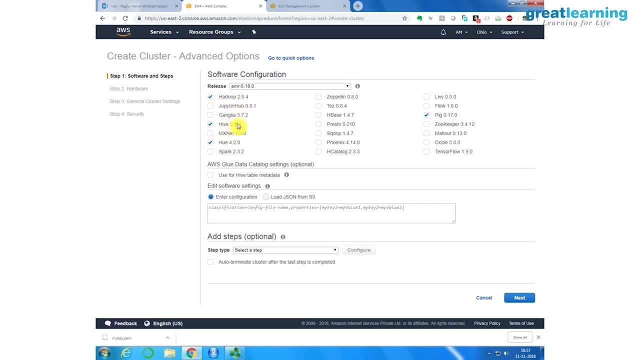 Do you want Jupyter? Do you want Hive? Yes, I picked Hive. Do you want Spark? Yes, probably I want Spark. pick this Zeppelin. Paste Hspace: probably I want Hspace Scoop Hcatalog. 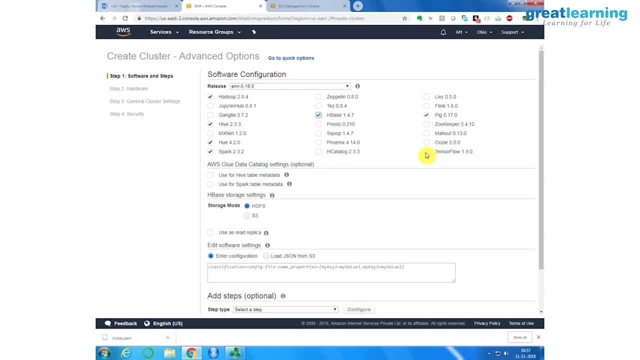 Pig Zookeeper. so TensorFlow see. So now TensorFlow is also there. So you want to do ML kind of stuff, right, You can just say So. as of now, I will say that I just want Hadoop Hive. 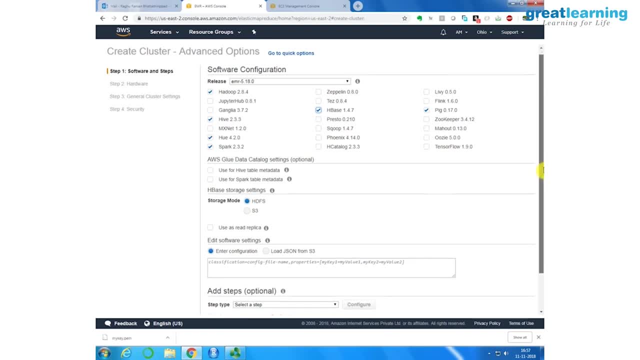 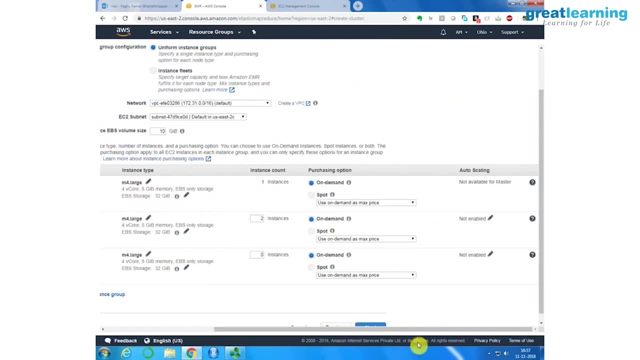 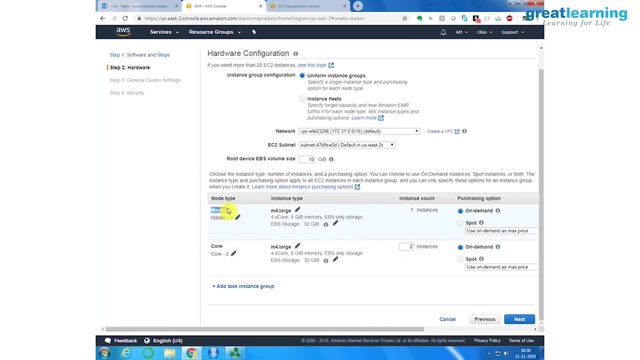 these tools, okay. And then you scroll down a bit and then you say next, And in the next page, oops, you can ask how many machines you want in the cluster. So you see there is a much more. There is a master machine here, okay. 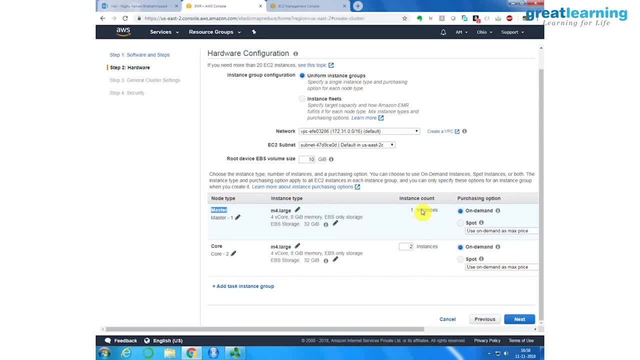 And by default you will get one master machine- That is default- And core machines. so Hadoop works in a master-slave architecture. There'll be one master and many slave machines to do the job. So core machines are your slave machines. 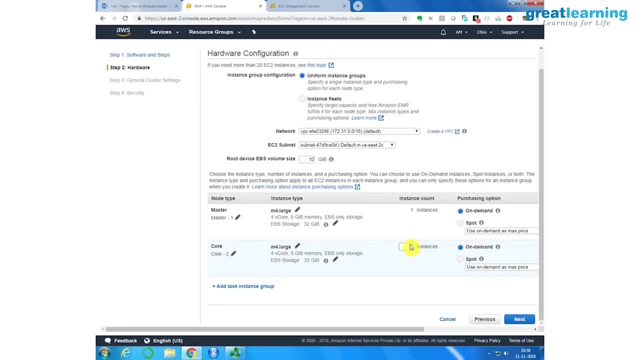 And how many slave machines you need. by default it is selected two, So that means I can change this to 90 or 100, depending on your account limit you will get. So I will say that I want one master instance and two slave machines. 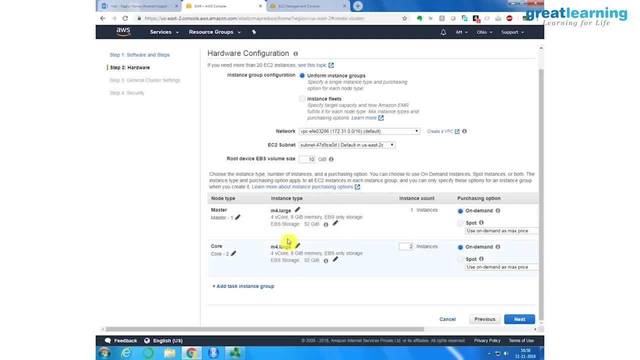 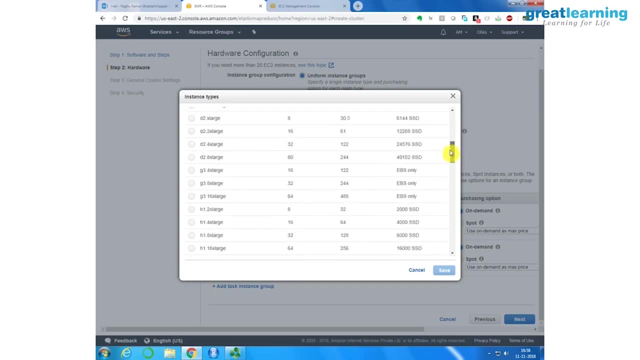 Two slave instances, okay. And what kind of a machine you want, you can select from here. So these are the hardware options you will get right And, for example, if I select the first machine, I will get two CPU 3.8 GB RAM. 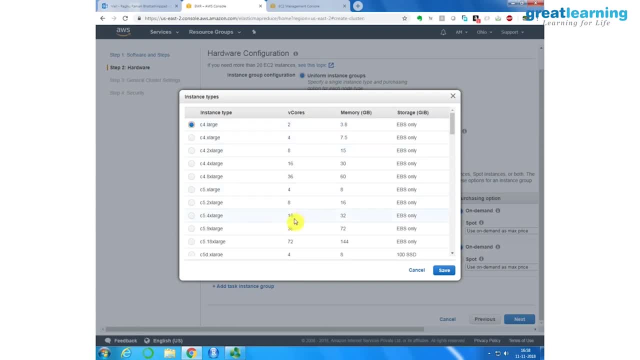 But here it is four CPU, 8 GB RAM, et cetera, et cetera. So probably we will stick with a smaller machine like four CPU and 8 GB RAM, something like this. Even for this I will say: this machine I want. 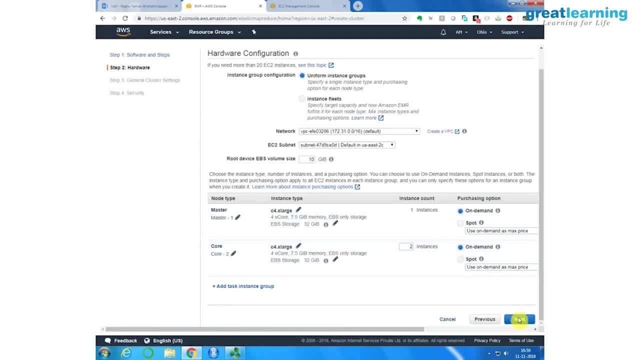 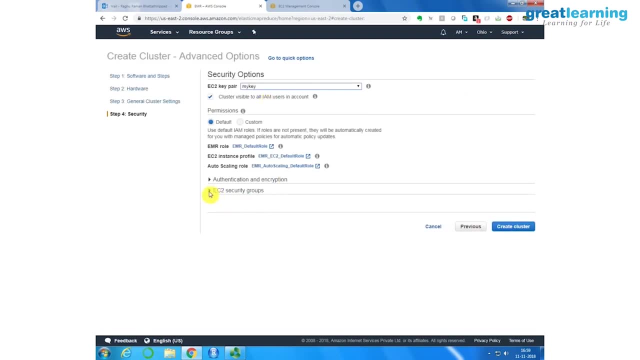 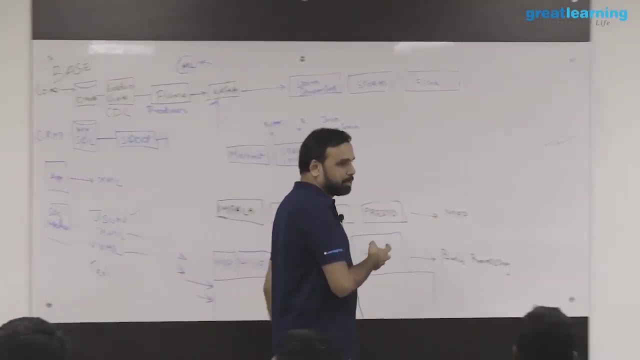 I can just save it So you can decide the configuration here and I can say next, I can say next, I can say this: and security groups, And you can say starting, just say starting, And probably in another five minutes or something, 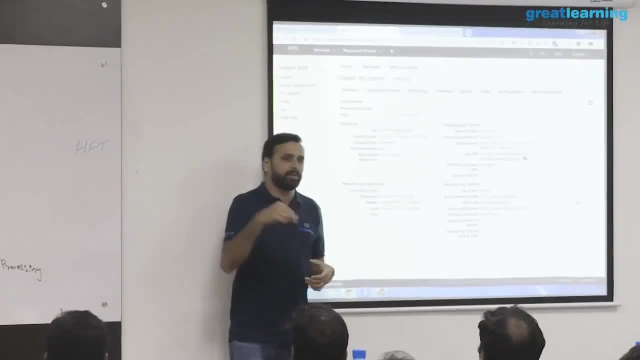 it will create a three-nought cluster and give it to me, and all the tools will be installed, whichever I pick. Then I can simply say, okay, I want this. So I can simply upload the data and analyze the data. So this is the disposable cluster. 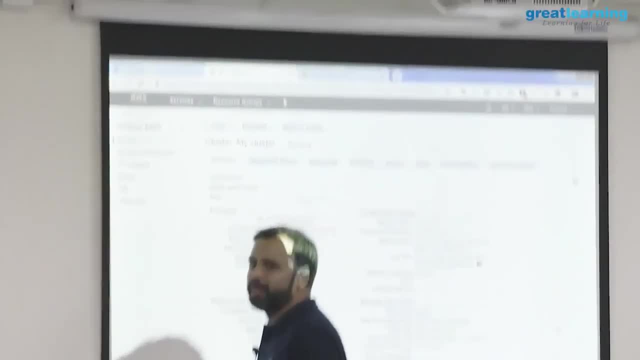 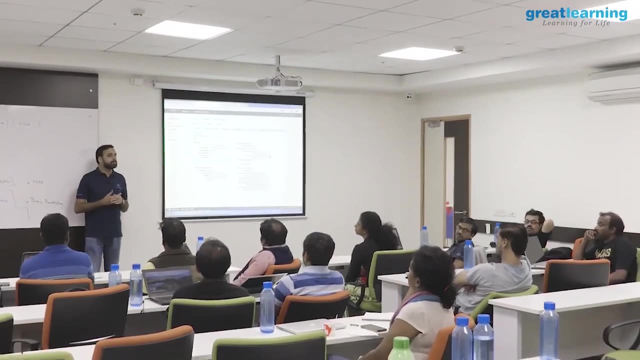 There is a button called the terminator here, So once you are done with your activity, you terminate it. There is nothing else you can do. I think we have to check. It's a free account, right? Amazon actually gives you a 12-month free account. Yes, one year, Yeah, but that does not cover a lot of things. Yeah, I mean, it's very limited to So the machines. So when you sign up with Amazon, they will say that they will give you a one-year free subscription. 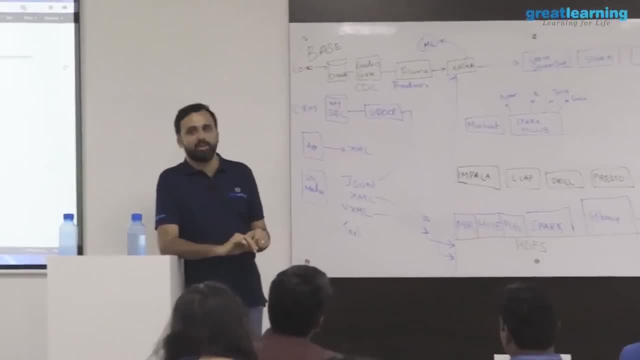 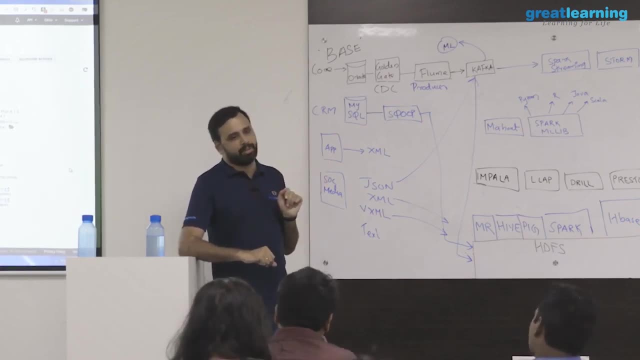 And that's nice, except it is not So in that it is a very limited usage. So they will allow you to create machines with, let's say, one GB RAM. If you want two GB RAM, you have to pay. 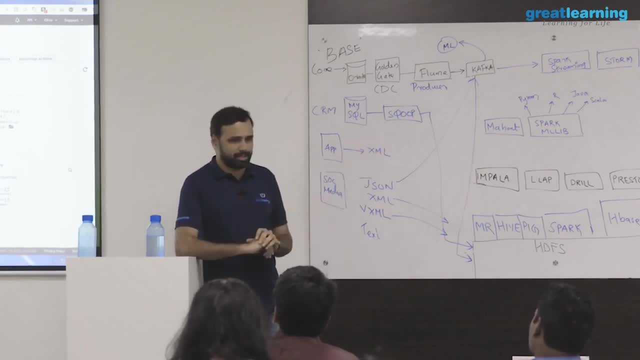 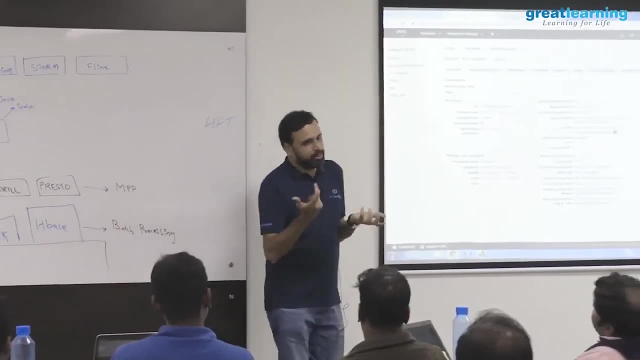 So my machines are actually eight GB RAM. They will charge for sure, right? So in the free tier or the 12 months free access, you will have only limited the free access. You have only limited resources which you can use free. 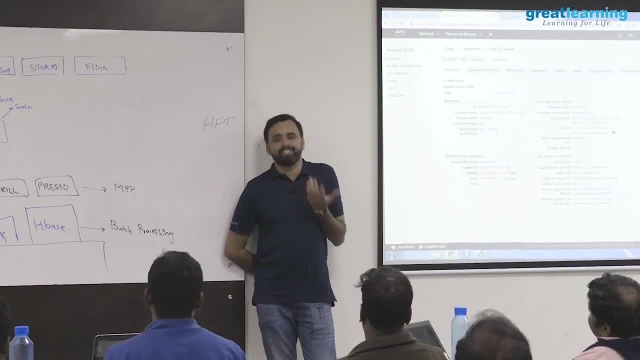 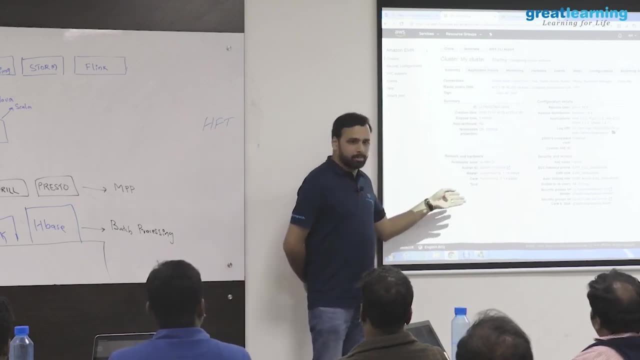 Everything else will be chargeable. actually right, But that is just to test Amazon. you know You cannot really run any production workload in that machines, So this will be chargeable, this, so how much charge you have to pay? 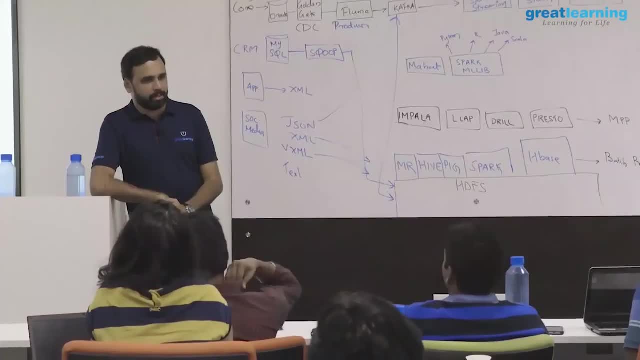 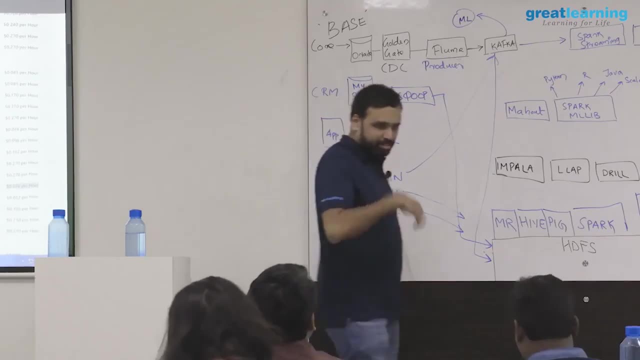 you have to check before creating the cluster. How do you check? Oh, that means I create and kept it. When you start, there is only one option: terminate. If you terminate, no charge. So in Amazon you have upfront purchase. 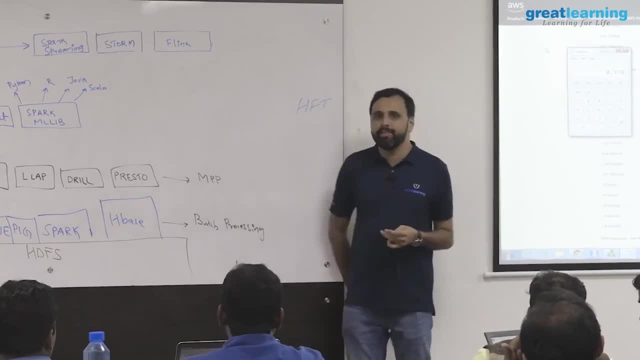 You can say I want to. I want to. you know, I want to, you know, I want to, you know, I want to run this for one year. They will give you the total bill- let's say it is $1,000, they will give you a discount. 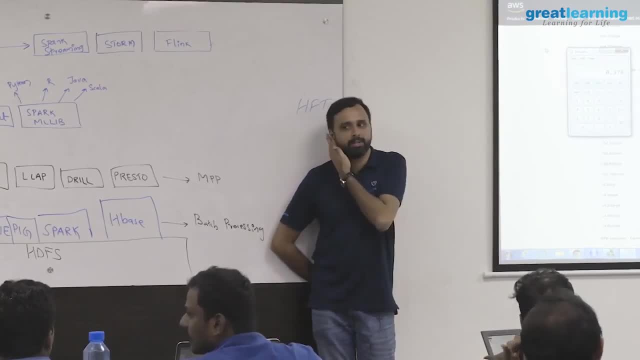 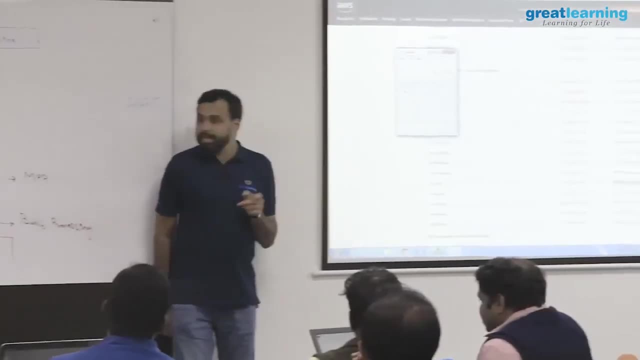 on that. They'll say: pay 800 or 600, something lesser amount, But I do not think that is applicable for everything. So the more important point is, even though I created an EMR cluster, now there is one problem with my cluster. 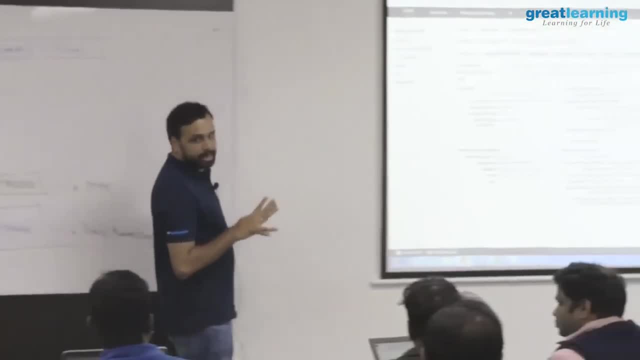 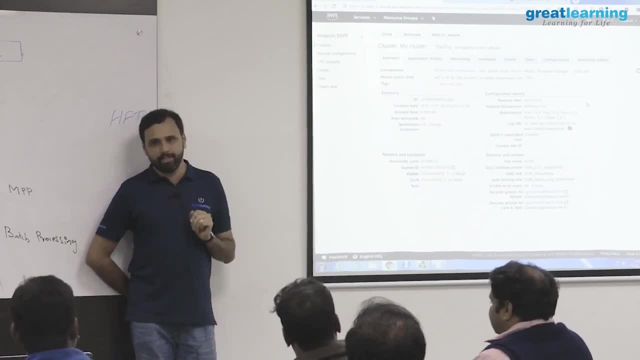 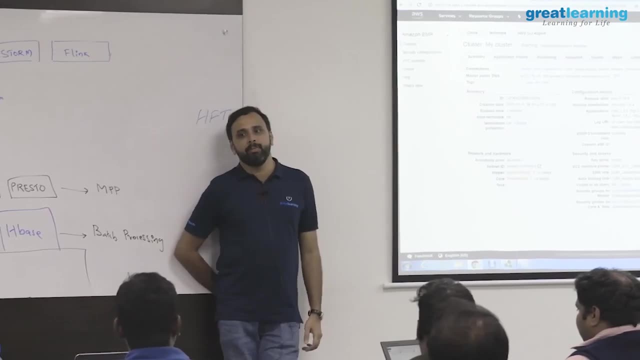 I don't have any administrative access in the cluster. That is bad, So this is not what people do. This is for occasions where you just want to create a cluster and do something. But if in your company, if somebody says that, okay, we need to create our own Hadoop cluster, 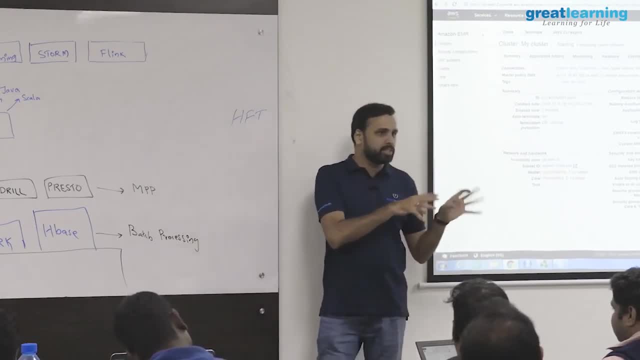 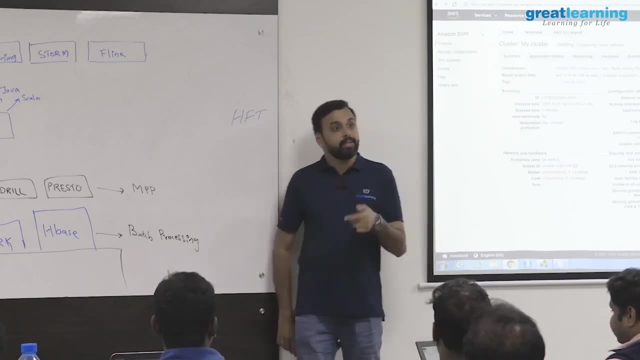 then what you do is that you will bring up, let's say, 10 machines individually. you will install Linux in them, then you will install Hadoop in them manually, you will set it. that is possible, And then you will have full control. 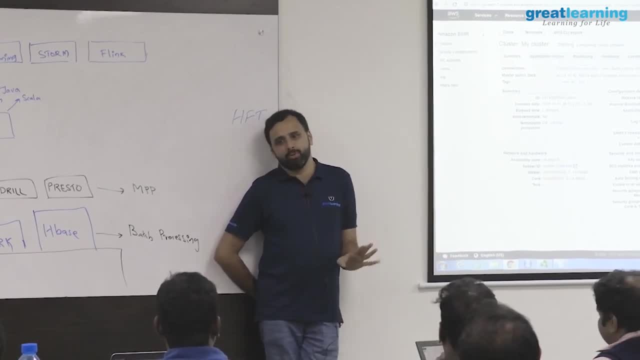 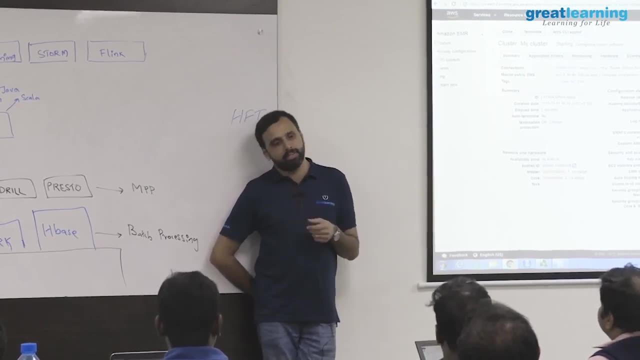 You will install Spark. you will install the most part Here. everything is Amazon is doing. You are just asking for a cluster, So that is not really what people do in production setup. This is for ad hoc cluster. We call it as ad hoc cluster. 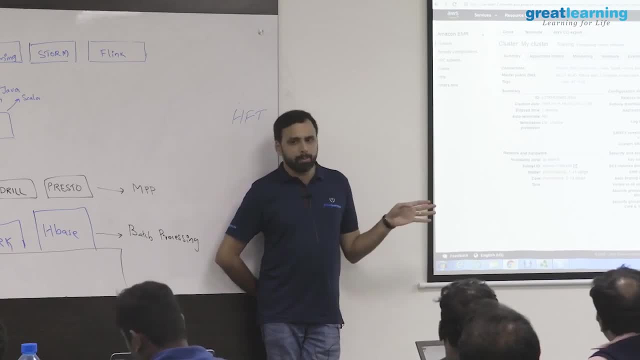 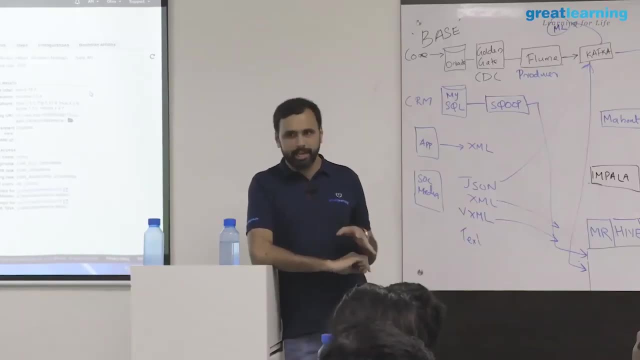 You get it when you want it. then you delete it. But this is also popular. EMR is very popular these days. Even a person without Hadoop knowledge can create it. That is at least that is what they say. whatever data that you store. 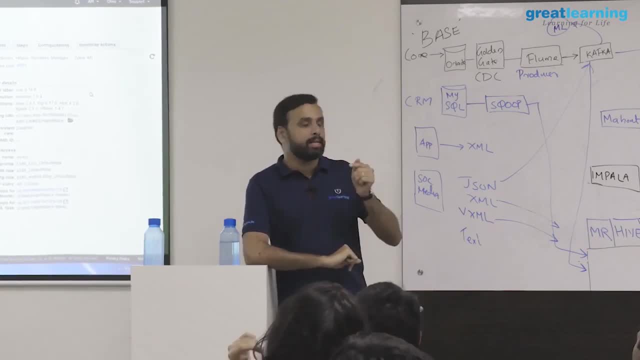 they don't have any access to the data. But another point is: if you are doing EMR and all your data must be in Amazon Cloud, Otherwise it doesn't make any sense. Let's say, all my data is in my laptop. Let's say, one terabyte data. 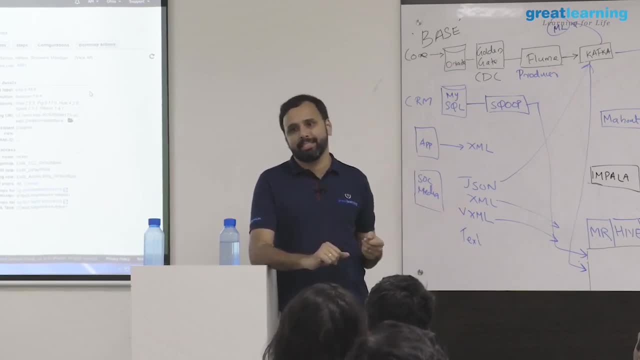 I have to first upload it right, So that doesn't make any sense. So this is good for customers whose product is already in Amazon. And many customers are there like Flipkart, And Flipkart is in Amazon, So for them it is easy. 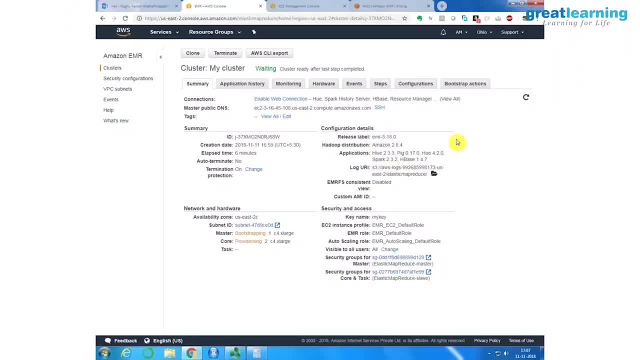 Everything is in Amazon. They add a service. So it says cluster ready after last step completed. So now we have a cluster. Now we have the full-fledged cluster right, You can connect with the cluster, do the analysis, everything that you want. 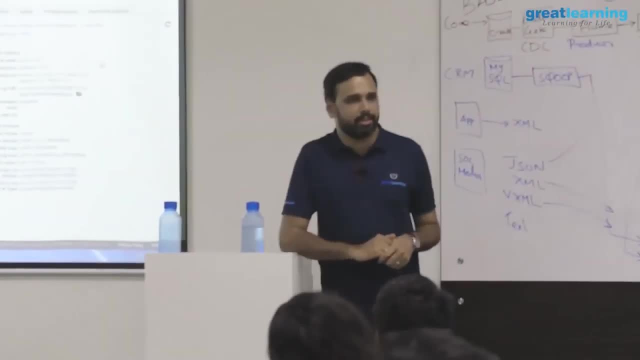 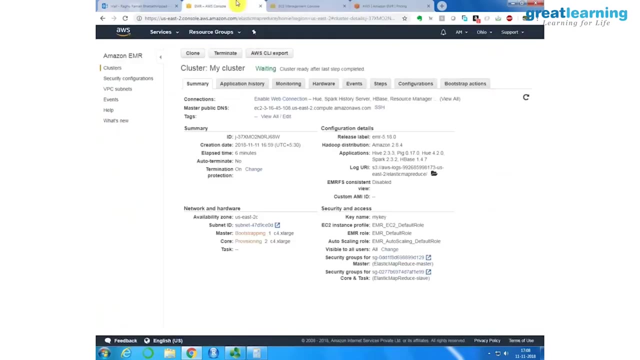 You have three machines in the cluster and they're running right And we can do all the analysis that we want. If I go to the cluster, it's already done. but what I can do, I can say I want one more cluster. 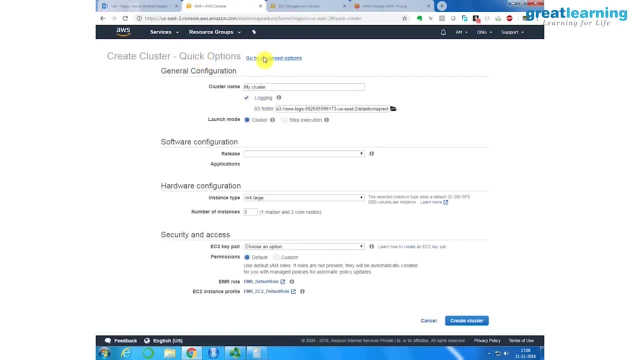 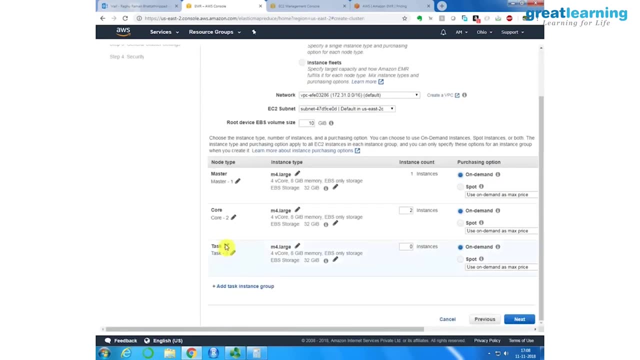 I'll go to clusters and I say: create cluster. And this is the place where we were doing right. So I will just say next, And if I scroll down, very interestingly I would not show you this, because I mean: 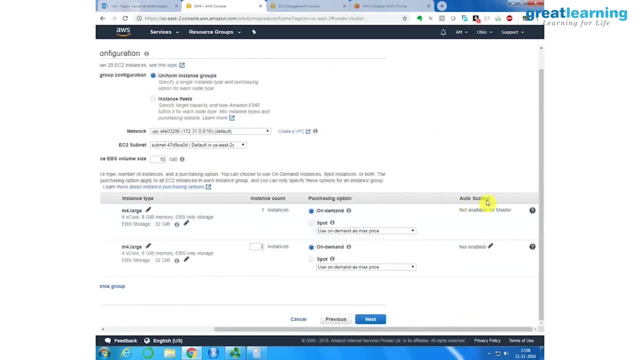 I scroll here. Can you see this? autoscaling Not enabled. So by default, this feature called autoscaling is not enabled, which means it will not work. but I can simply say I want to enable it. If I enable it, it will ask me. 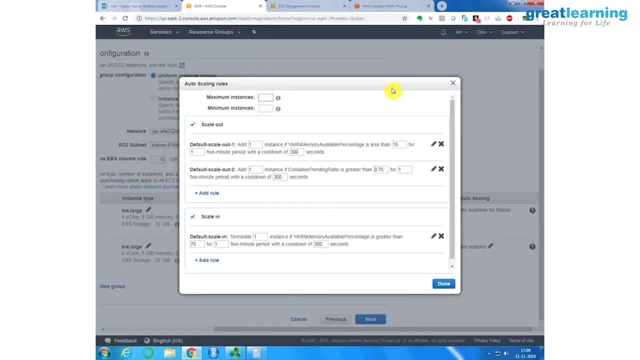 when do you want to add one machine? When do you want to remove one machine? That's the rule: One machine Or more than one machine. So here by default it says when you want all. the machine will ask you when to знаешь c. 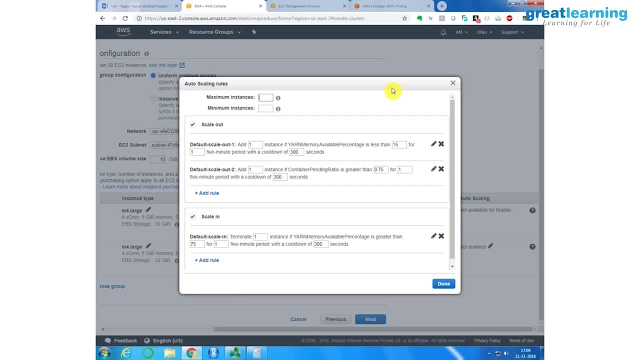 Yarn memory is less than so. there is something called Yarn memory Or I can add any rule. I can say that if the CPU, if the total CPU of two machines are more than 90%, then add one machine. Same concept here we are using. 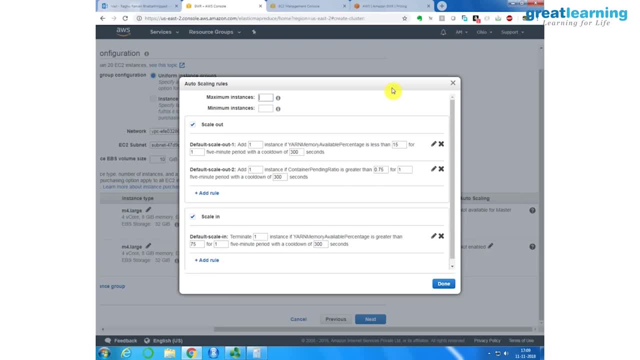 but here the only difference is that when you enable the rule, it is depending on the Hadoop resource utilization. That is where this Yarn and all are coming. So you say if more programs are running or something, or my analytics is taking too long. 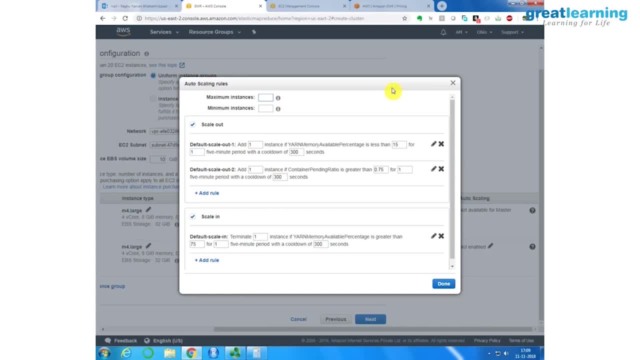 let's say my query is taking one hour: add one more machine or remove one more machine? The beauty is that you can scale out and scale back, So when the load is less they will automatically delete the machines. This you cannot do on premise. 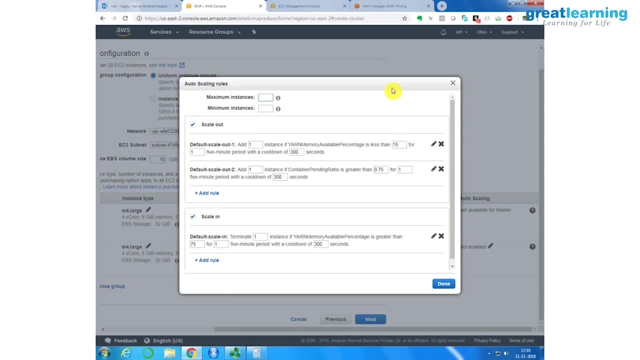 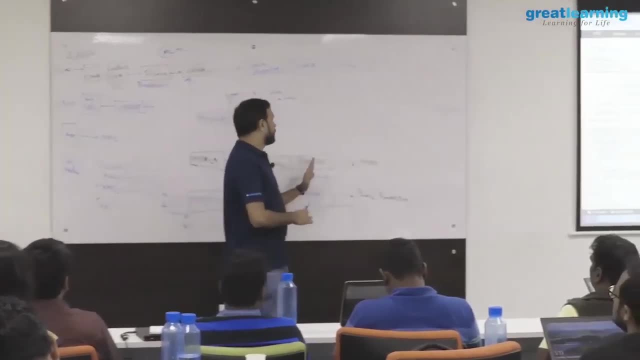 This. so I do not enable it, because when I just created a cluster- but this is possible, Autoscaling is possible on EMR by default- What we do is that let's say this is the Hadoop cluster, One of the very common problems. 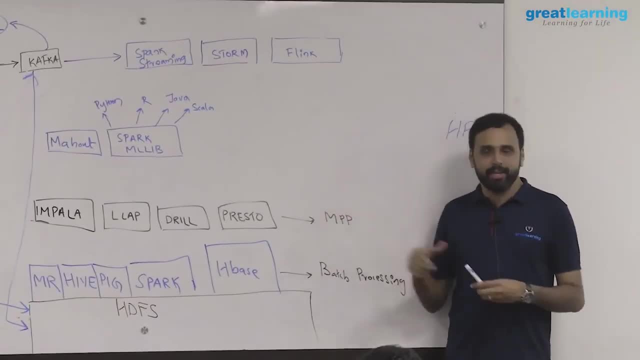 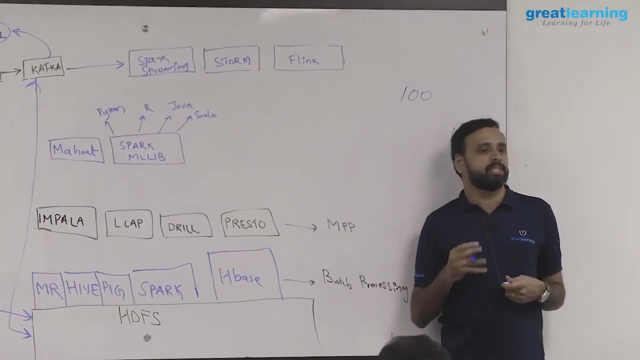 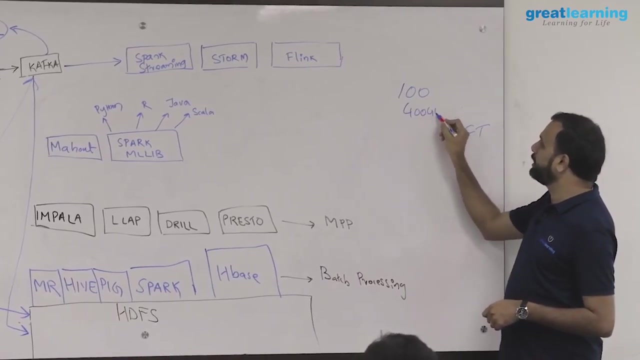 in every Hadoop cluster is resource management Meaning. let's say you're running with 100 machines in the cluster. 100 machines means each machine will have some RAM. Imagine 4 GB RAM. So total RAM will be what You have: 400 GB RAM, correct? 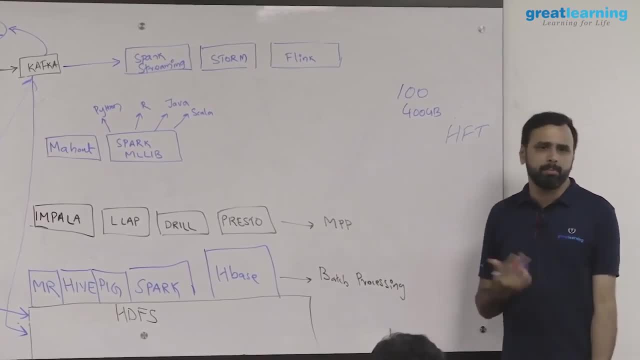 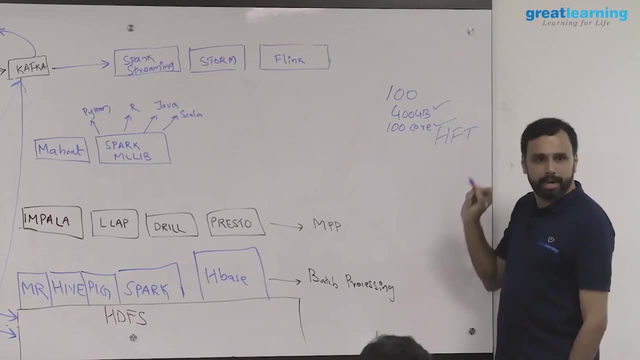 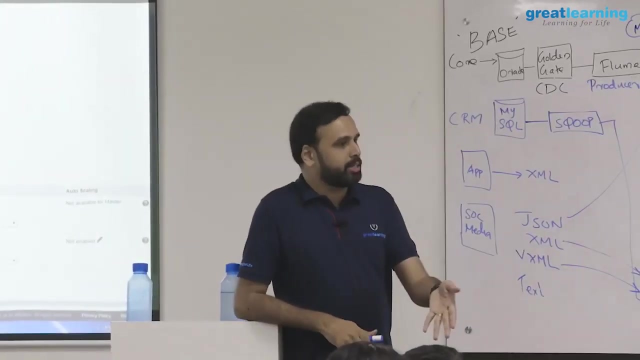 And CPU is also there. And let's say, one processor- simple example- So you will have 100 processor core. All right Now. so these are some of the things which can help you, even in machine learning or anywhere you go, because this is a concept which nobody understands. 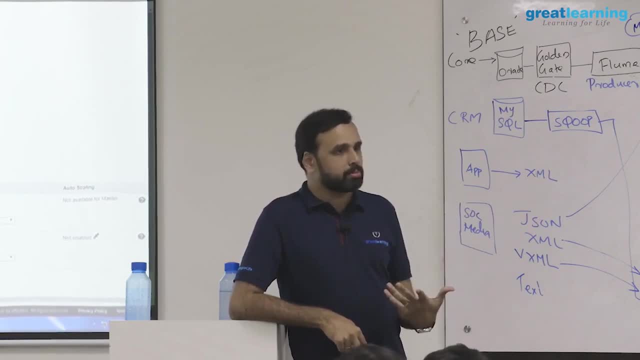 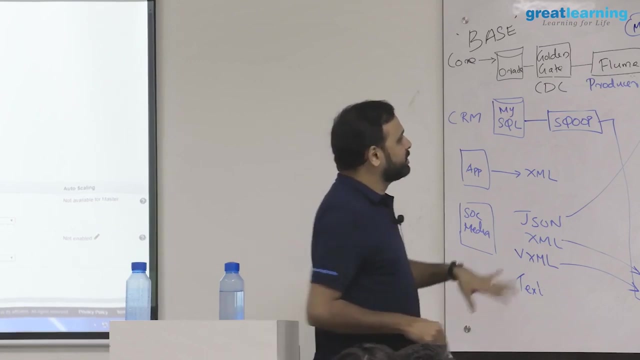 but probably the most important concept when you start working, which is called resource management. Whenever you write any program, be it machine learning or normal learning, whatever you write, if it needs to be executed, it needs resources. All right, Now imagine this is a cluster. you are a developer, you wrote a program, you wrote a SQL query. 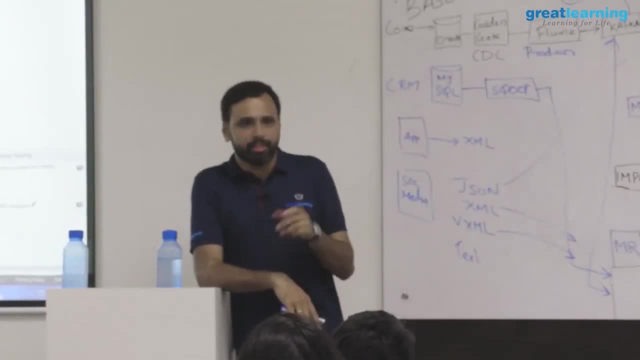 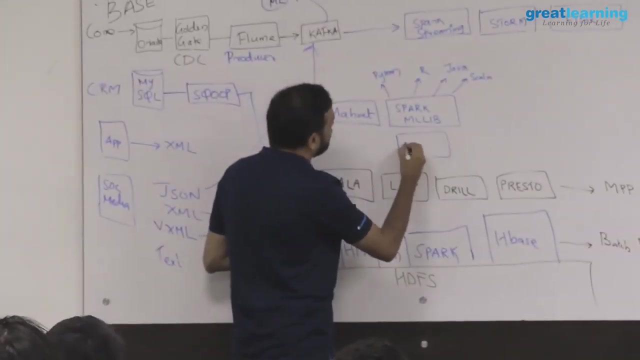 The SQL query is analyzing one terabyte of data. So if the SQL query want to run it requires some RAM, some CPU from the cluster. who will give this? how this will give, so on and so forth. So by default in Hadoop there is a component called YARN. 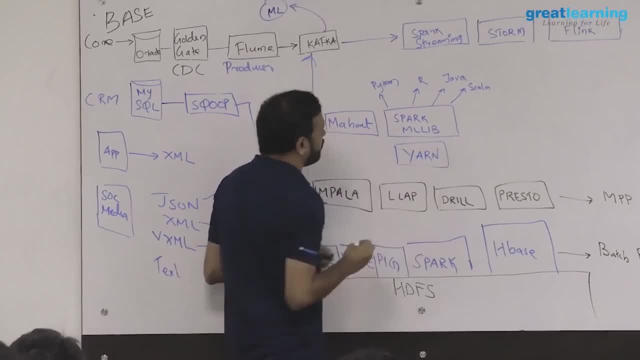 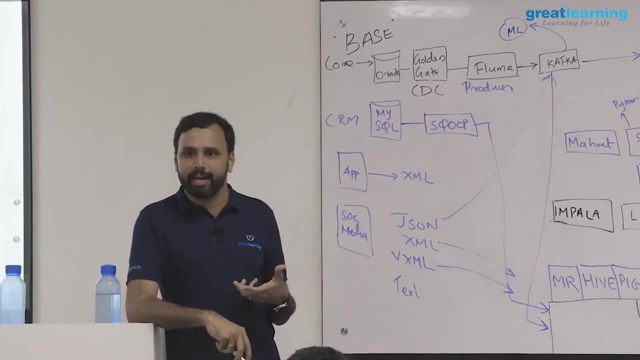 I did not talk about this, but there is a component called YARN in Hadoop it is an integral part. YARN is the resource manager, So YARN will decide resource management normally. So in a very normal cluster where there are not many programs running, you will not have 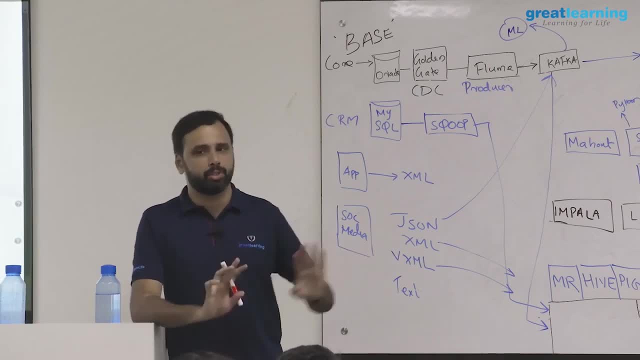 to bother. If you submit a query or a program, YARN will allocate the resources to run. But in very hefty clusters like in this, 24 bus, 7 and all, they have only 60 nodes And lot of developers are there. 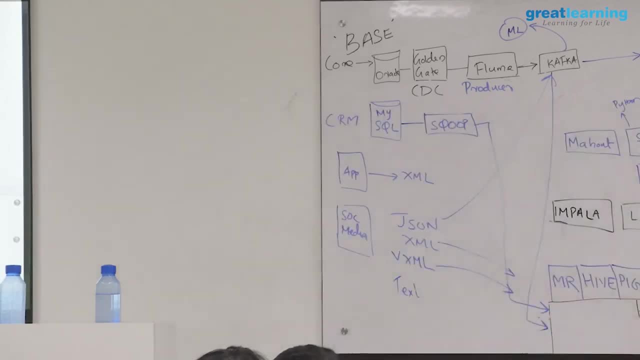 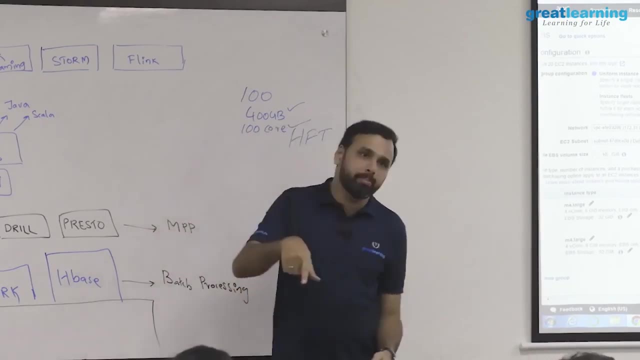 So what will happen if everybody starts submitting programs? your cluster capacity will be reduced, Your capacity will become full. So then what will happen then? the cluster is full. then if one guy again submit a program, by default, what will happen? his program will wait in a queue. 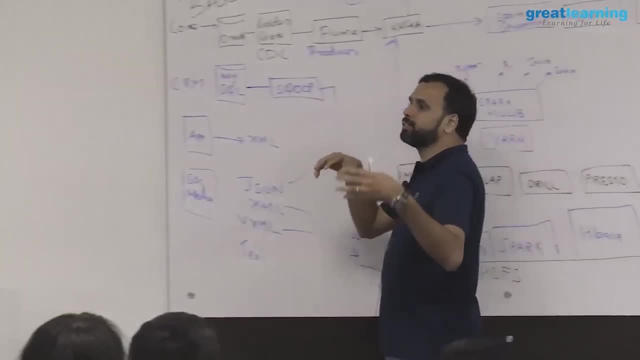 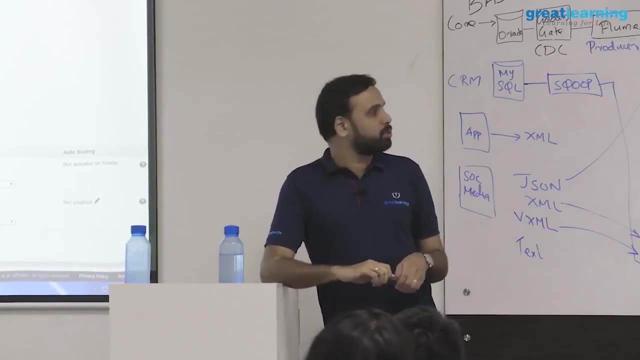 The program will not be cancelled. it will wait in a queue And then some program finishes and the resource becomes available, his program will start running. In order to manage this, you can do something called scheduling, So we do this all the time. 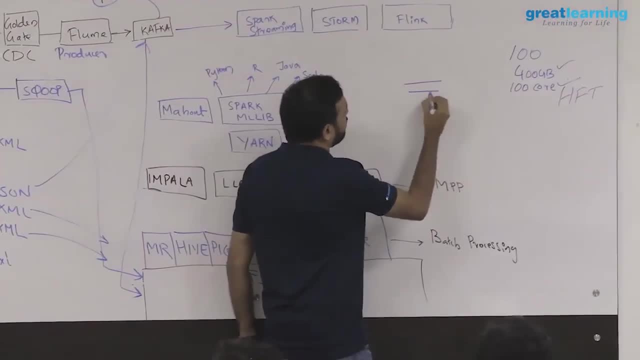 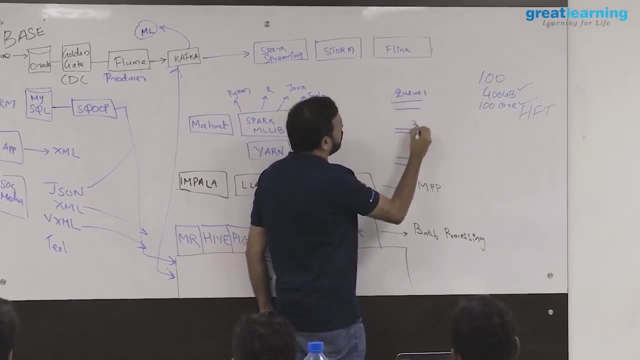 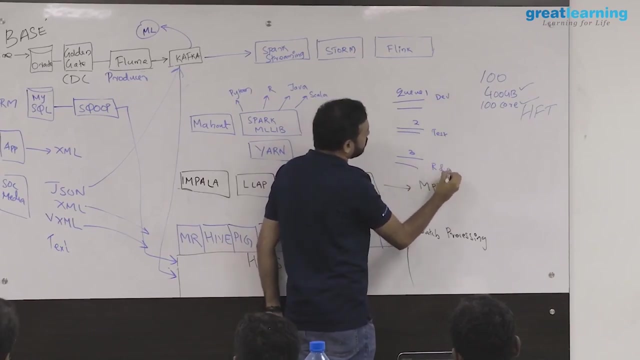 So we will split the cluster into three queues. Okay, We will say there is queue 1, queue 2, queue 3.. So this is queue 1, 2, 3.. This is all the developers. this is all the testers. this is all the R&D team. 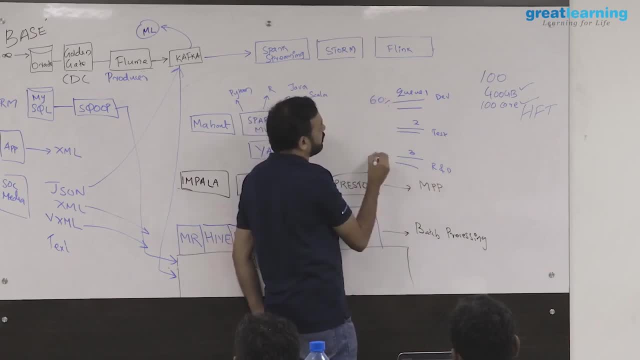 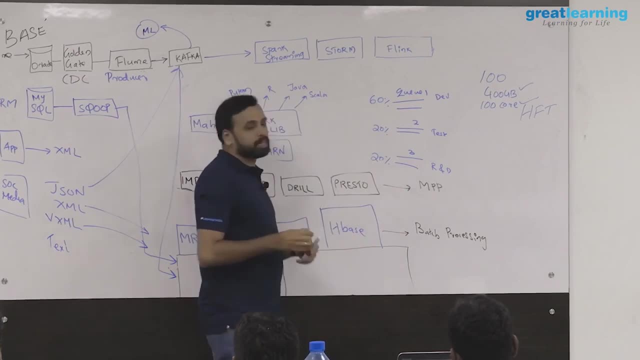 And developers, we will say they will get 60% of the resources, Testing team get 20% and R&D get 20.. So if you are a developer when you submit your query, automatically the query will go to the developer queue. 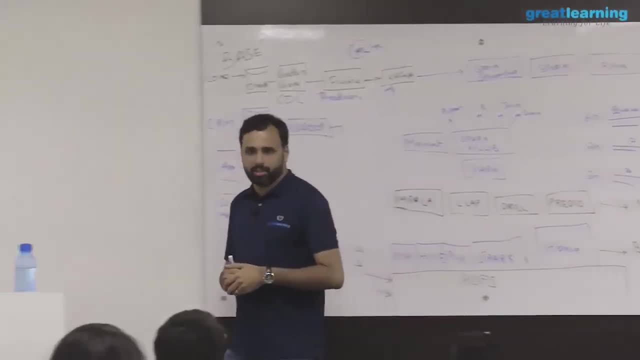 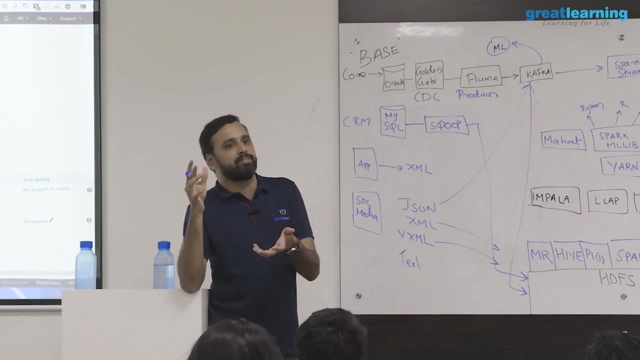 Okay, Which has 60% of the tester resource, right? or if you are a tester you get only 20%. So that way you have to control, and that is very important when in production, because writing a program may not be the big deal in production, setup running it is very big. 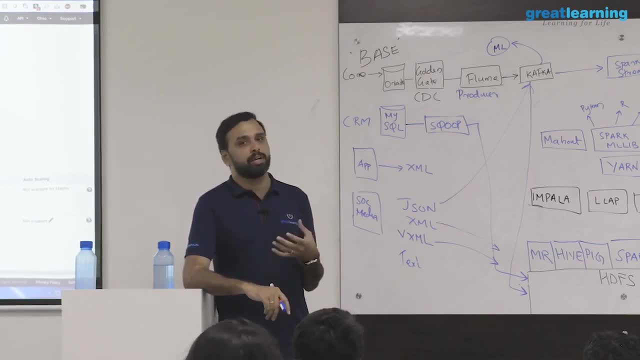 deal actually, And there are many programs which are not very critical. So if you have non-critical programs, you will schedule. this is a way to manage the total resources among multiple users. Okay, User management basically Right, Considering on-premise cluster. 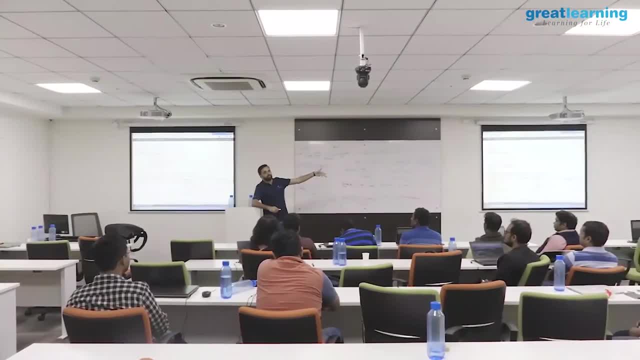 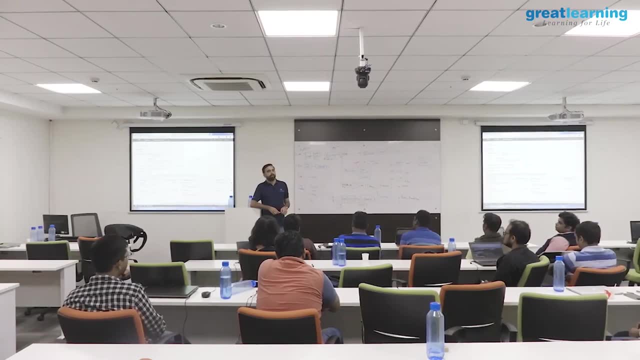 Right. And then there are rules who can take which queue how much resource you can take, Otherwise everybody starts submitting their program And you can also have priorities. So one of your customers want a report every day, 10 o'clock. Now, to generate that report, your BI tool has to connect with Hive. 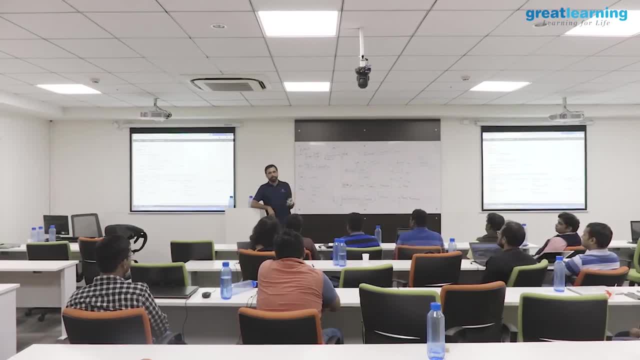 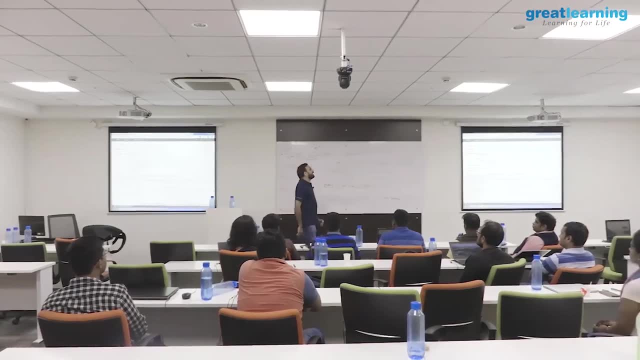 So your Tableau right Tableau has a Hive connector. Tableau can connect with Hive. So if you have a table in Hive, Tableau can fire a query and visualize the data. So your customer is saying that I need a Tableau report every day 10 o'clock. 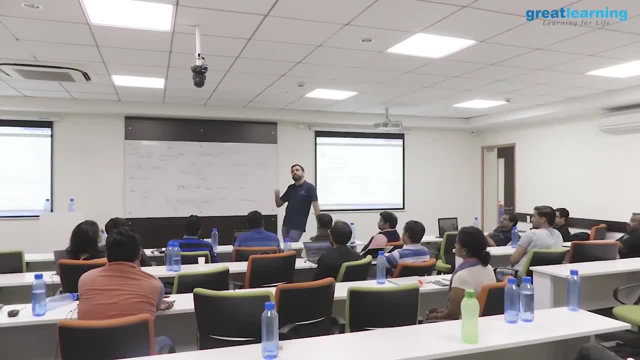 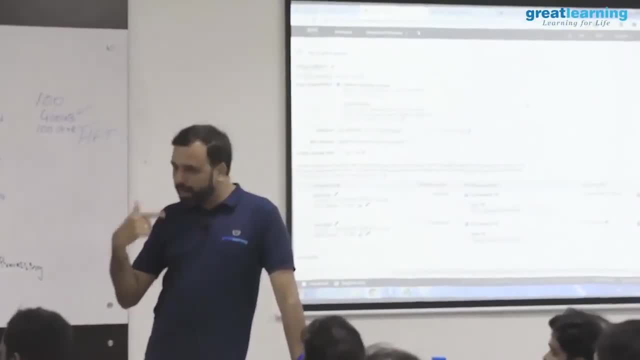 So Tableau has to connect with Hive and fire a query. So at 10 o'clock, if your cluster is busy, what will happen? Your customer will not get the report. SLA will be broken right, So that time you can have priority. 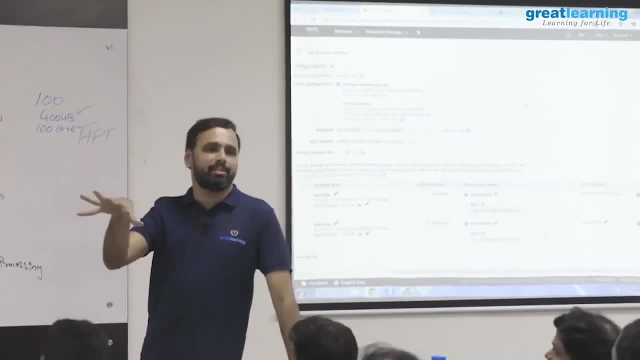 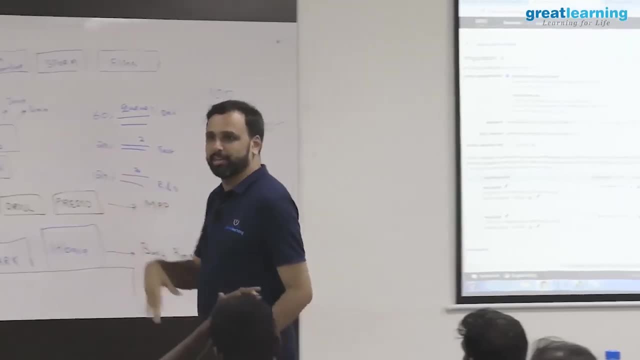 For this customer, this query it will run. Other jobs can wait, So resource management is a great headache. I have worked as a Hadoop admin for an year and a half, Not because of my passion, because of the circumstances, because the existing admin quit. 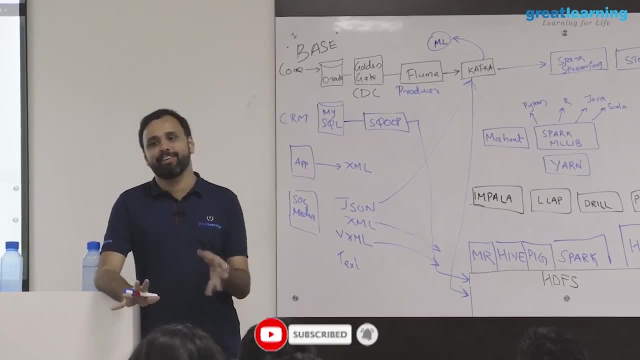 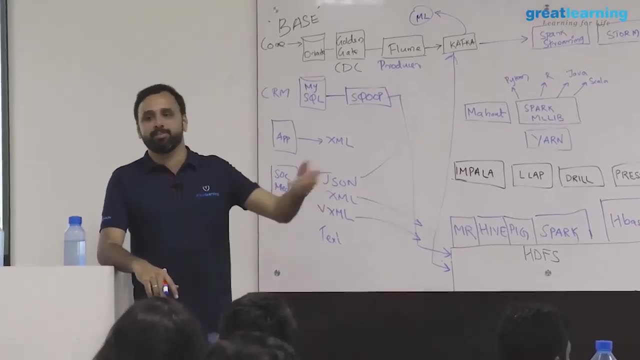 and there was nobody else, so I became the admin. I had no clue. what is the role of an admin? Everybody will start complaining. Here's our query: the result is not coming Because another is a customer is creating problem. There is only one cluster, right. 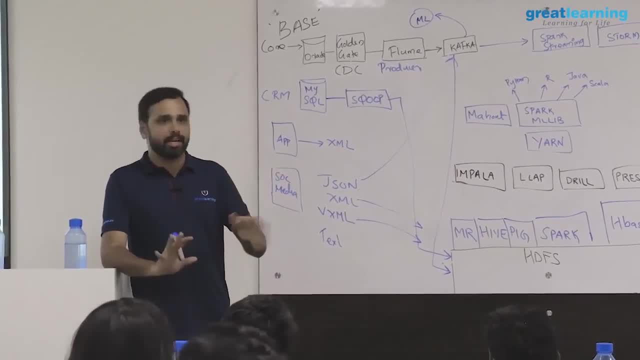 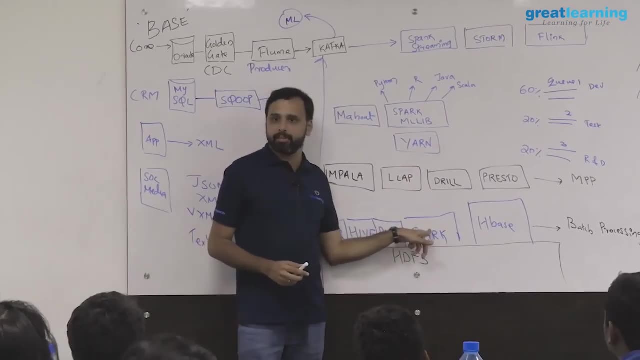 So resource management is the biggest headache. in a Hadoop cluster. Everything else can run, And especially when you're running Spark and other programs- and all Spark is very memory intensive- The moment you run this it will grab RAM like anything, So other programs will have to release it. 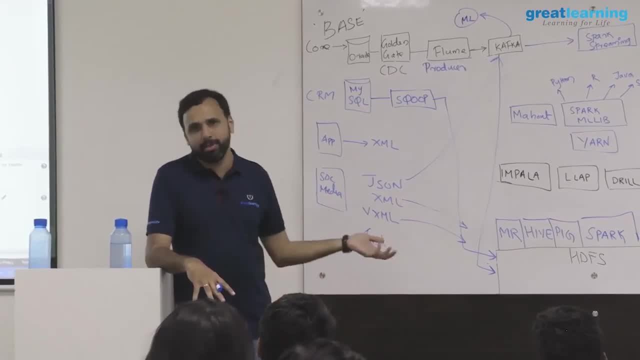 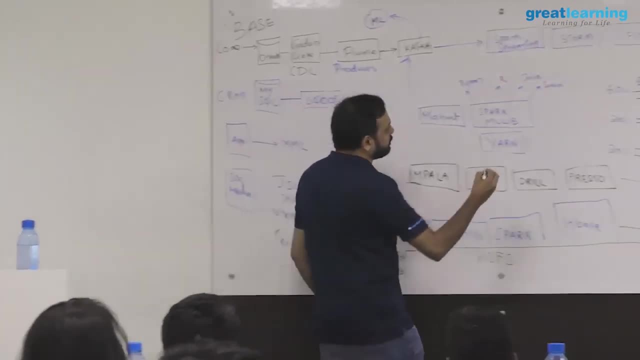 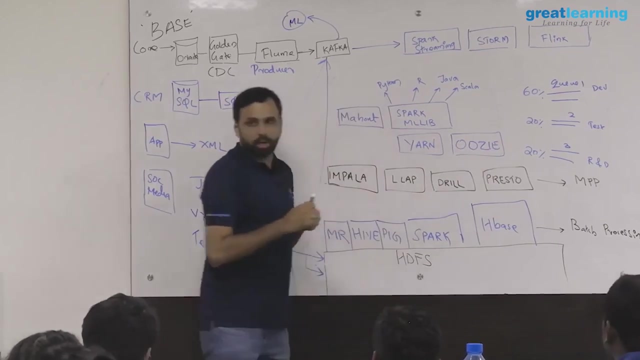 They have to wait right, And you cannot kill this program also because somebody might be doing some analytics right. So then you need to figure out a way in which- so that is where we are using this- Uzi Uzi Uzi is like your cron. 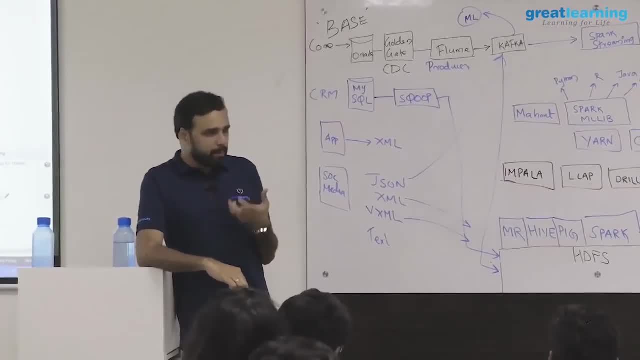 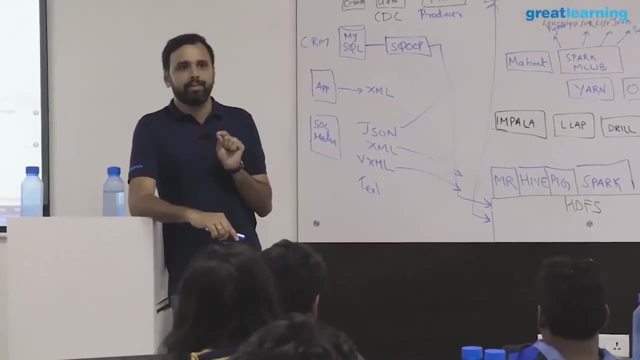 In Linux you have cron job right. So what typically administrators will do? so developers will come and say that I want to run this job, this program. So they will ask: is it critical? No More than 25 by seven. 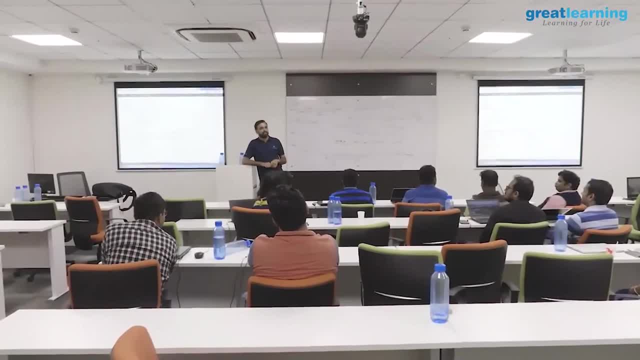 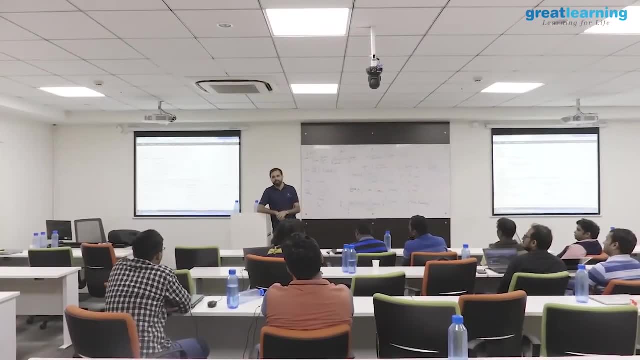 If I get one more hour, I'll schedule there also. It'll be totally busy, Because another problem is that people don't want to invest a lot of money. You go to your management- Ah, you go to your management there and say that. 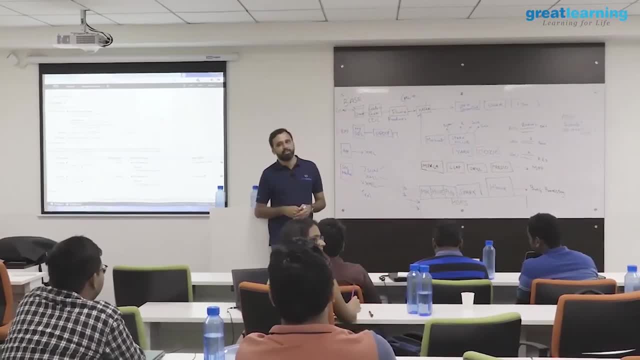 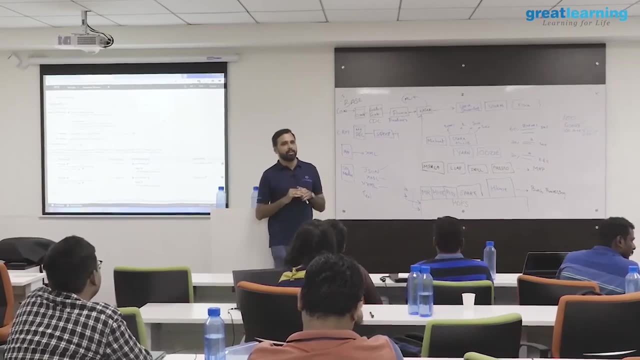 I want to add 10 more machines to the cluster. Why? What is the problem now? Where is your total cost of investment has gone? There's 100 questions you will get. So here you say: what are the problem of the existing? 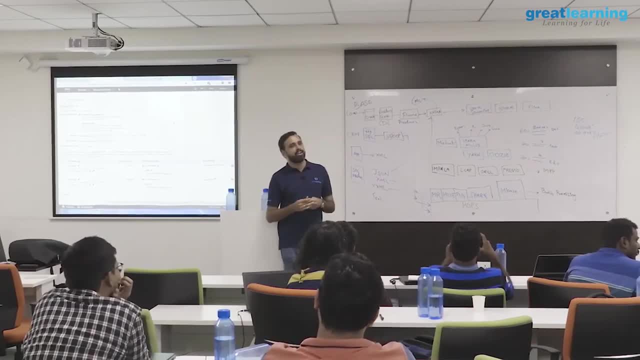 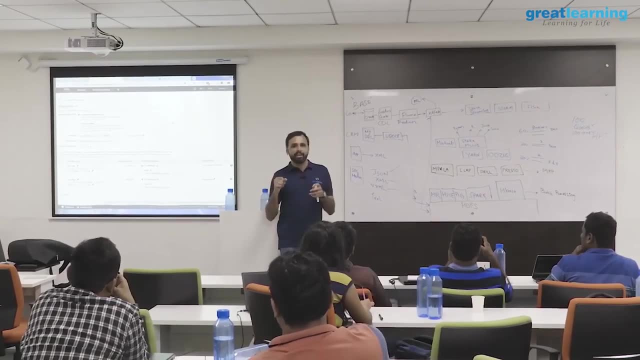 cluster. That is why I'm telling you: You are the admin right, So then, but your developer or not, they're restless. They're saying that my programs are slow. So that is when you are figuring out each and every slot. 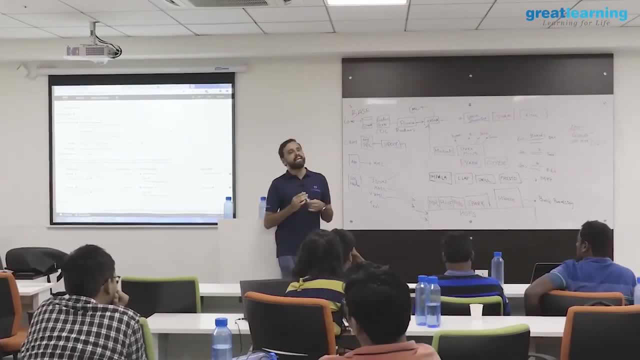 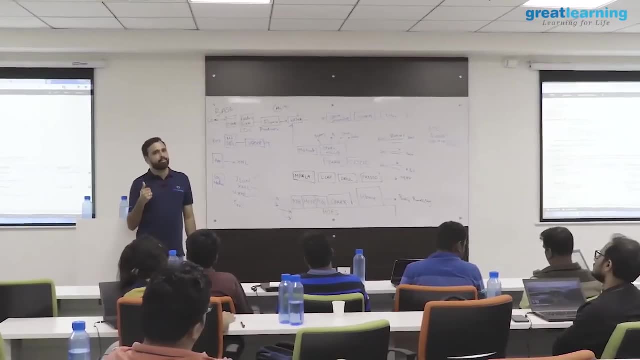 and the program is running or not. You have to make sure. But again, it is customer centric, Okay. So if the customers are very strong, they will say that we are ready to pay money and all you can- if it is your own projects and all you. 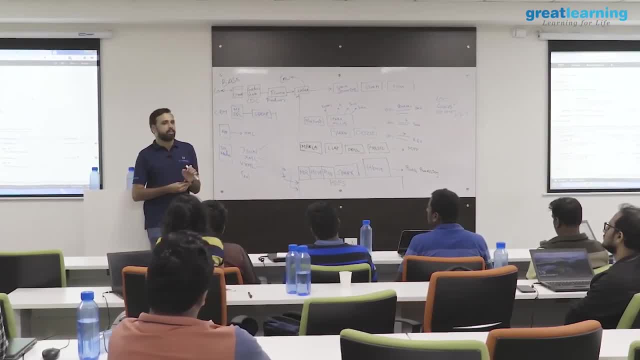 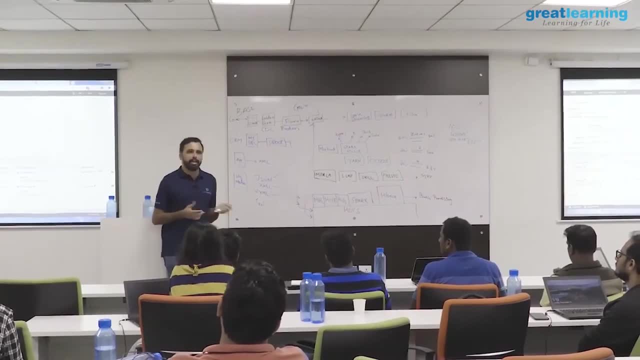 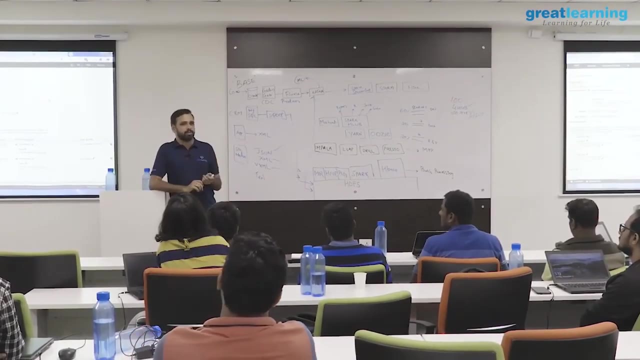 don't really bother. like bank of america and all they are, like they are ready to invest. any amount doesn't care, they want the results fast, right. so there, you don't have any other choice. they will say that we are not ready to wait. whatever you do, we need the results fast. that's what. but some 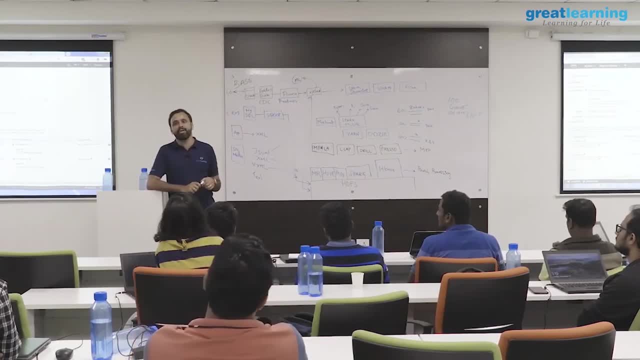 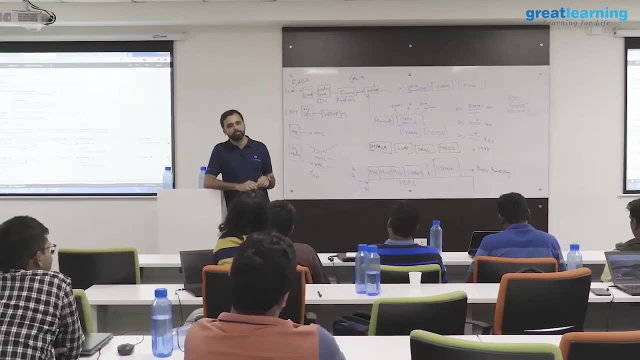 customers are like, so some some of your managers will be like: why are you expanding the cluster from where all these users came now? what queries are you running this, that, etc. is there a way in which you can analyze the performance of different programs in a cluster like, for example, if i have? 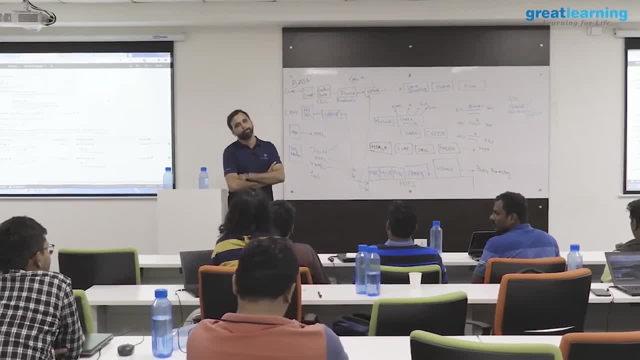 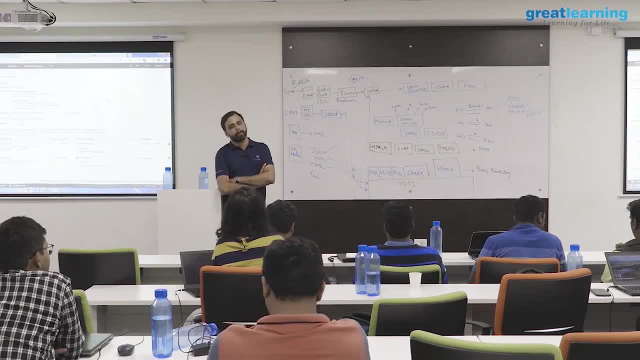 a program which is running on a cluster, will i be able to find out whether it's low because it's in a huge state, or because it is taking up a lot of resources, or because my program itself is coded really badly? no, so there are multiple things. one is that certain programs when you run a 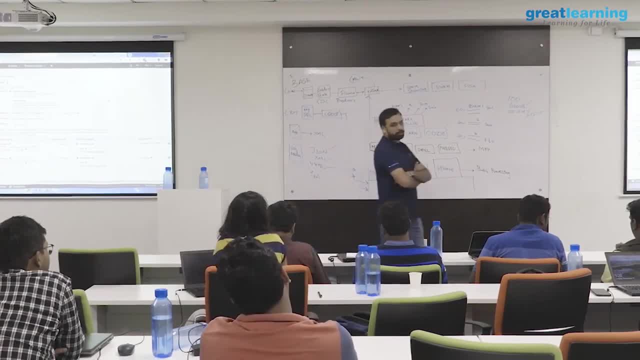 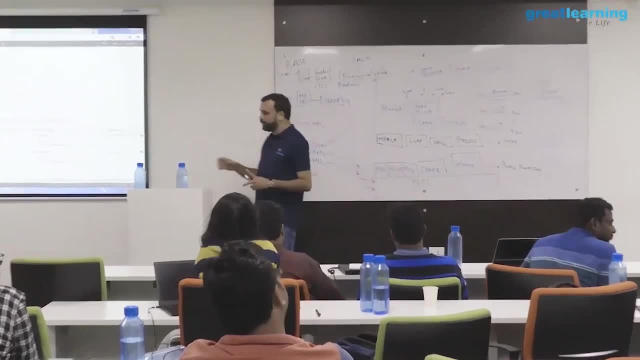 run in the cluster. you can choose the resources for the program. Certain programs you cannot. So certain programs you have to fine tune before you run the program in a cluster, For example if you're running a hive query. a hive is a SQL query. 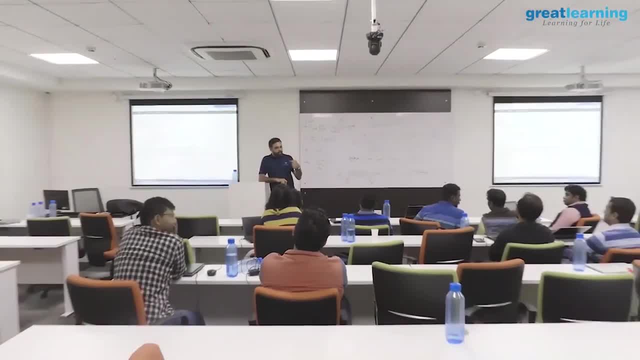 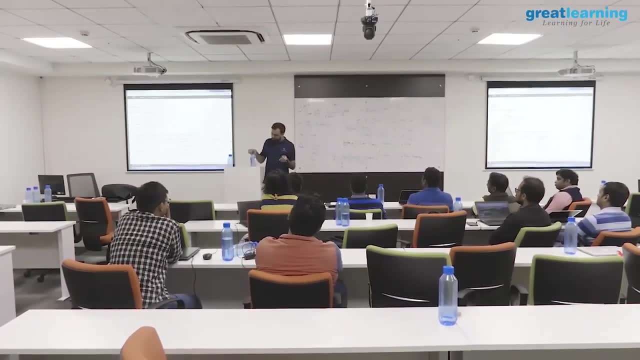 So first you have to make sure your query is tuned And then I don't know if you're coming from database background, not sure, Yeah, so if you're running a hive query, there is column-based statistics, there is table-based statistics. 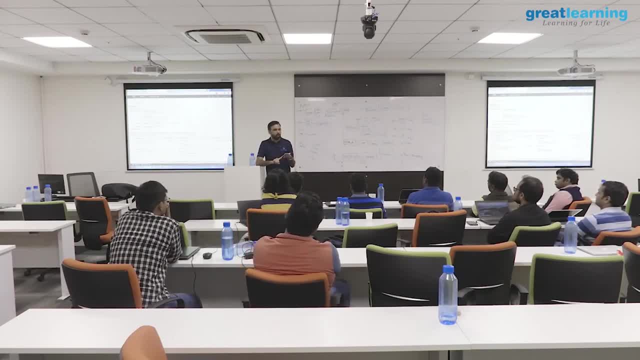 there is indexing and there is partitioning. So these are all things you will do. You will make sure all this is working And internally, Hive uses something called CBO- cost-based optimizer. The CBO works on all these parameters. 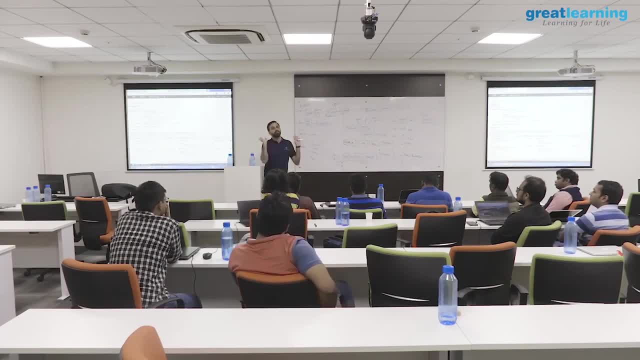 And then you tell CBO, I've done all this, optimize my query, and then it is not, So your query part is done. I mean, your query is maximum optimized. You can never have an error in the query. then. Then, while running that, if you're getting the resource, 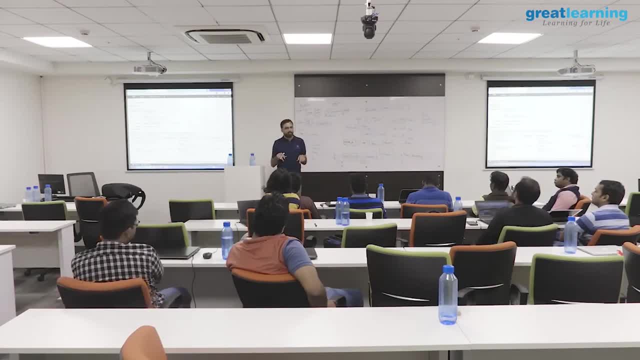 or not that you have to. you have a UI for this yarn. This yarn has a UI where you can see all the programs running and how much time it took, And once the program completes, you get the complete log file where you can say what happened in the program. 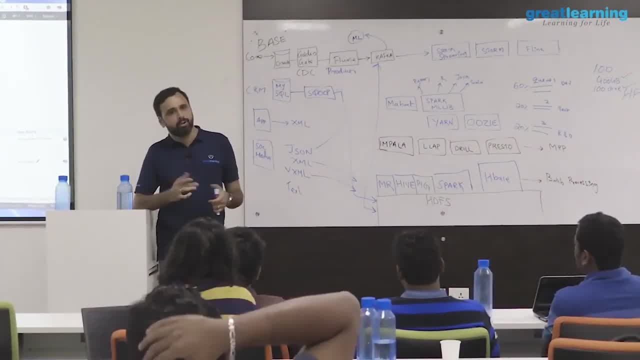 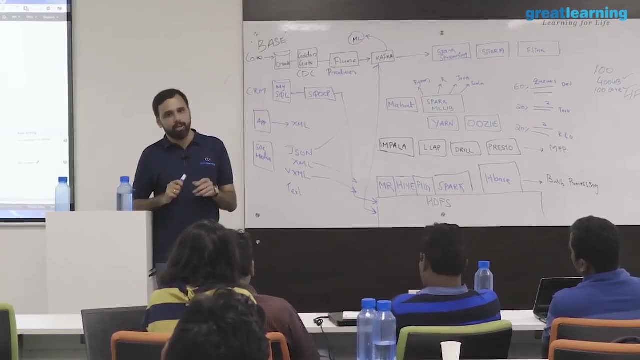 So running state is fine. If the program crashes or did not work, if a query gets aborted, then you need to look at the log and see why it went down. On the other hand, if you go for Spark and all, you have to ask for resources. 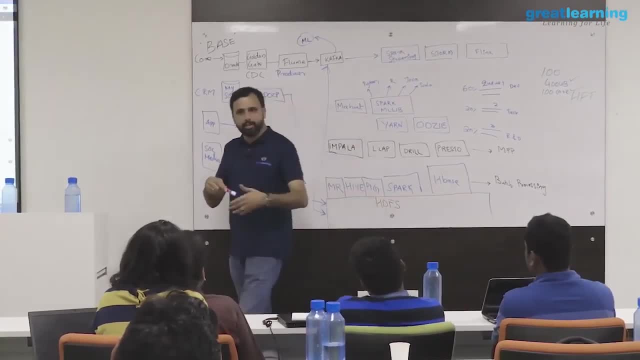 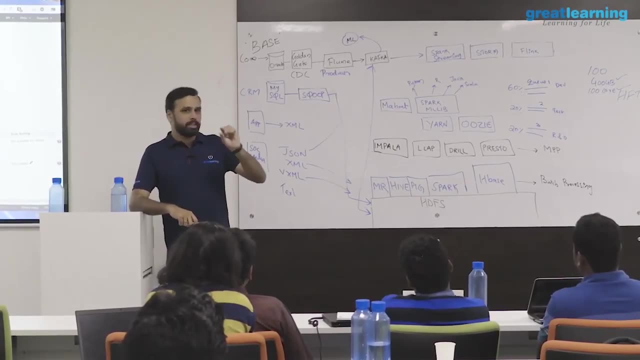 Meaning if I write a Spark program, if I run, I have to go to Yarn and ask Yarn specifically: give me this much amount of RAM, this much, these many processor cores, depending on the data I'm having. So there the developer has a responsibility. 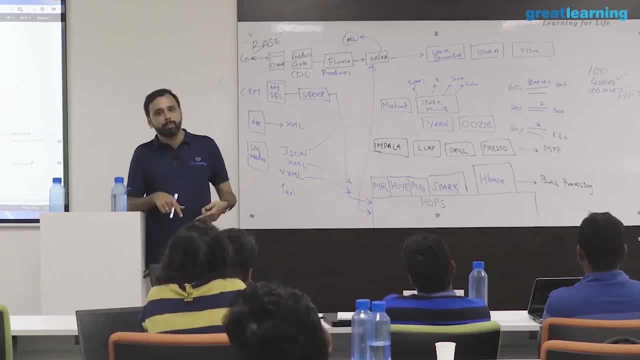 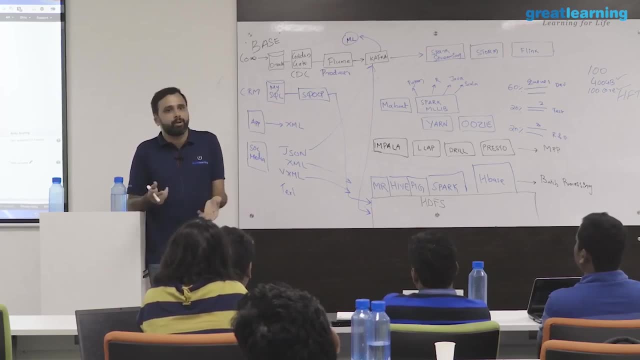 because he is writing how much resources he want. So if you screw up your program and, instead of asking for 10GB of RAM, you simply ask 20GB, You will get 20GB, but you're actually using only 10GB. 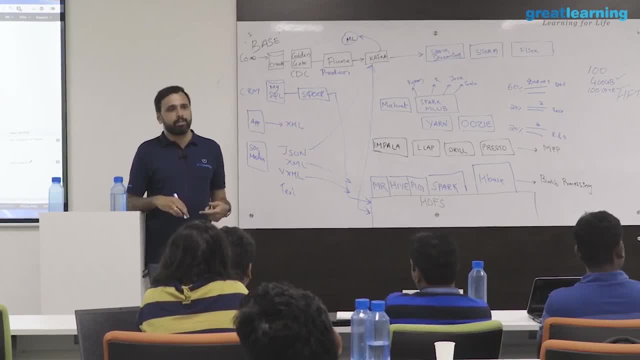 So that is your responsibility. And then you try to analyze the data that is being used, So that is your responsibility. headache, all right. so you have to figure out. so that is always a classic fight between developer and admin. so he could have written something and admin could. 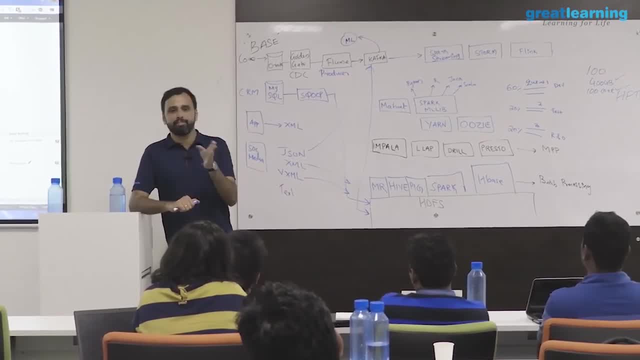 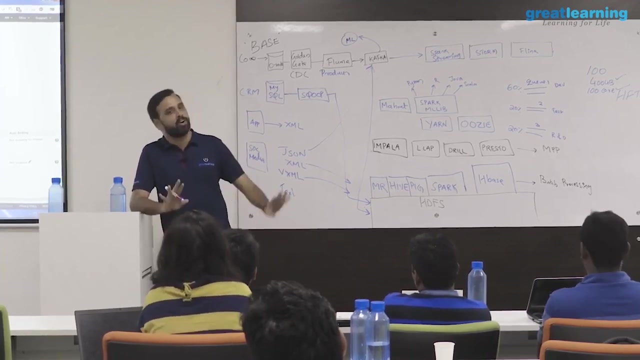 have thought about something, but you have to troubleshoot it at different levels and typically in every big data project there will be somebody called a big data architect. there is a role called big data architect. that will be like a big shot in the company. he never speak to anybody. he is like the God. 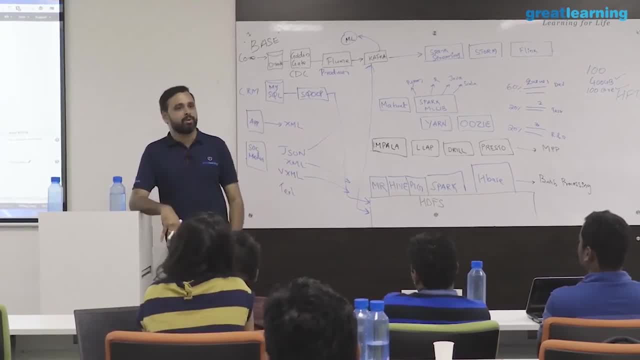 right. so that's called a big data architect. okay, so the big data architect is the guy who knows everything about the cluster. so anything that you run has to be passed by him. he has to vet it, say that it will run, then only it will run. so he is the guy who decides he knows right. he knows the admin side and developer side. 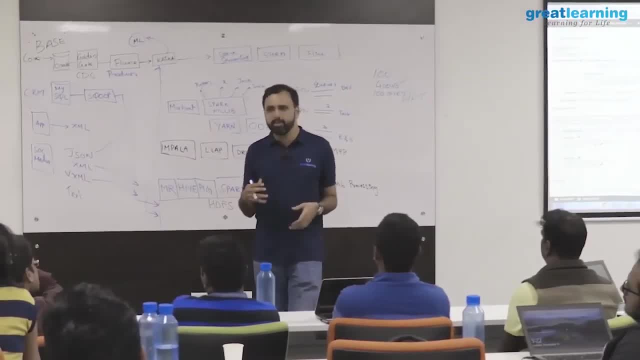 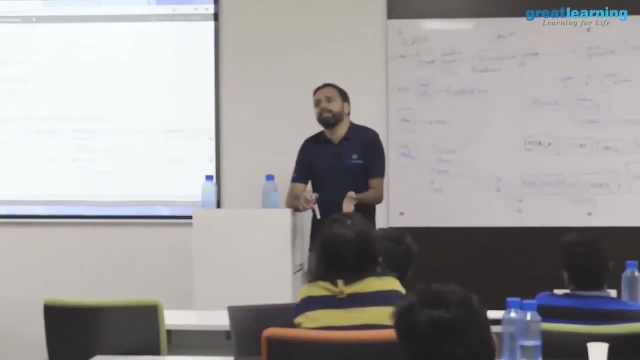 and he will ask: why you wrote it, why didn't you optimize it? or he knows in and out of what you have written. so everything has to be usually- I mean again company to company- it can always happen. some companies allow independently. you write your own program. he may, they may. 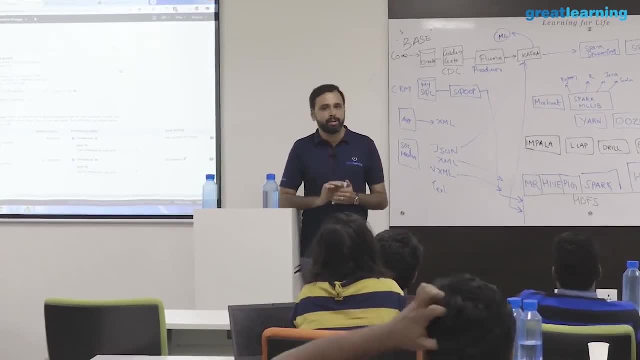 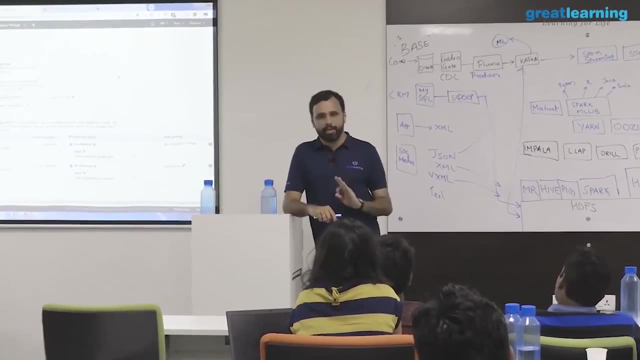 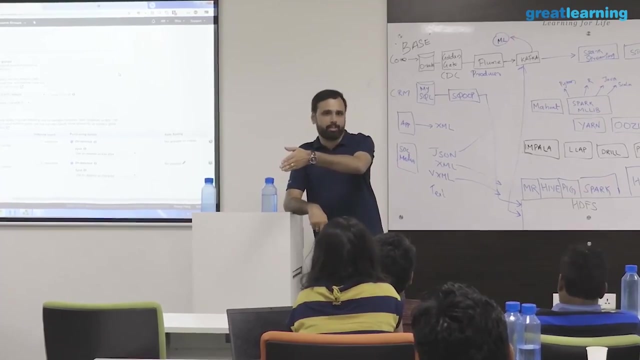 not have money to hire an architect at all. right, so they say you run it. but in typical client facing projects we have an architect and everything that you write has to be vet by him. and some projects actually use these three stages: dev test production. the typical dev test production is there. some projects do not. 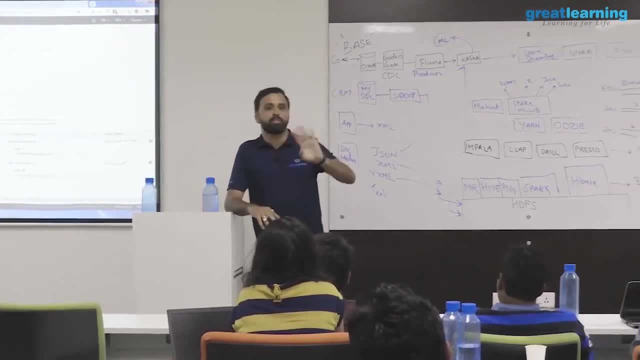 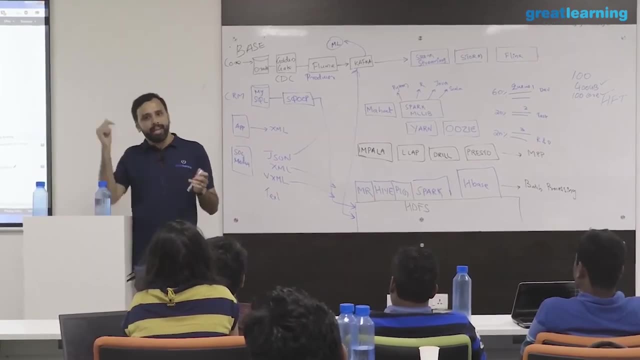 use it two types of there. so if you have dev test, it is much more easy because it is running through all three phases. you are almost certain that it is going to work right. so many aspects are there when you work in that project, right? I have actually worked with many. 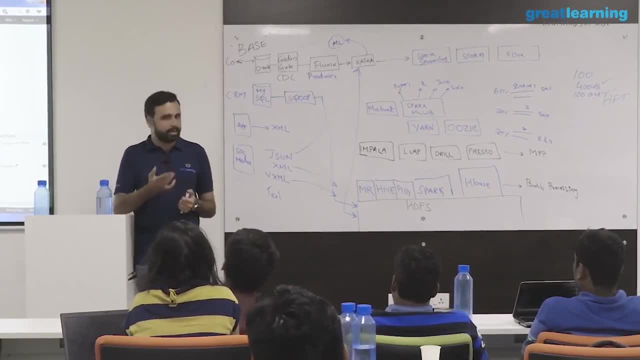 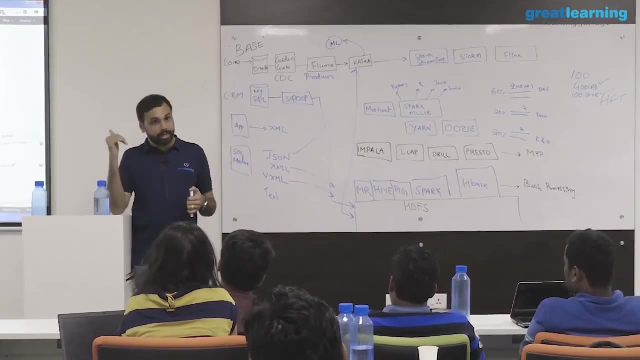 architects. actually, I mean, in my due course many architects have worked. so there, I mean I'm just joking, they're like really knowledgeable people. they know in and out of the entire system, right, because if you design something like this, if one finder and nothing is working, you should at least 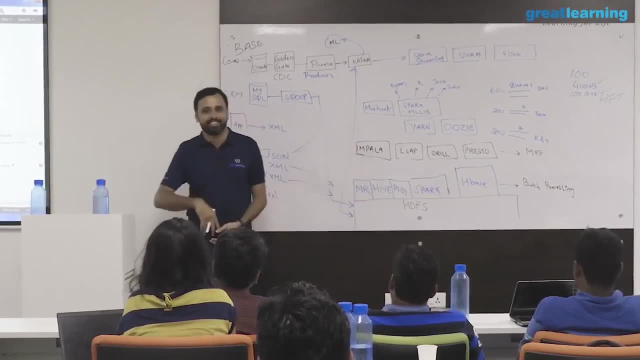 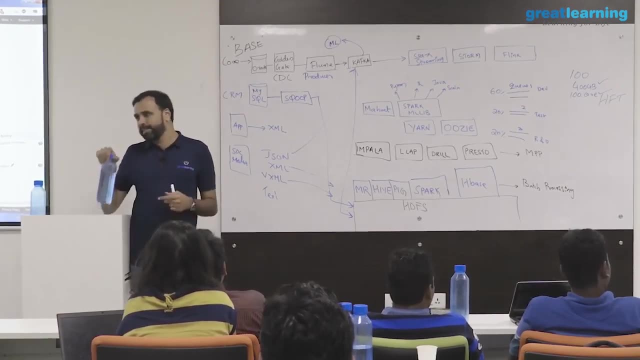 know what to look into, right, otherwise how do you know what is not working? so they will know which component has failed, how it has failed, etc. etc. right, so admin will be there, architect also will be there. usually you will have an architect who will design the workflows. and all now one more. 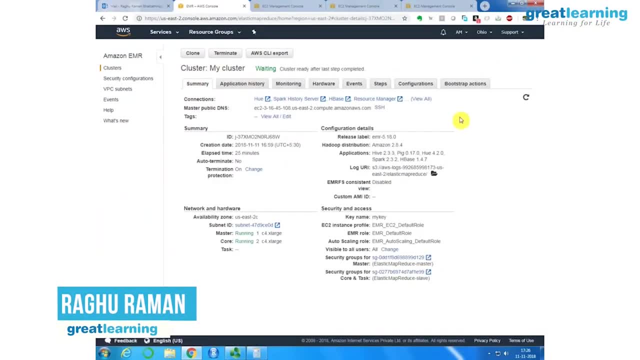 interesting thing about this EMR cluster is that it also has a GUI where you can easily upload the data to a root cluster and download the data. so one thing you may be wondering is: how do you upload the data? so one thing you may be wondering is that if this cluster is here, how do I upload? 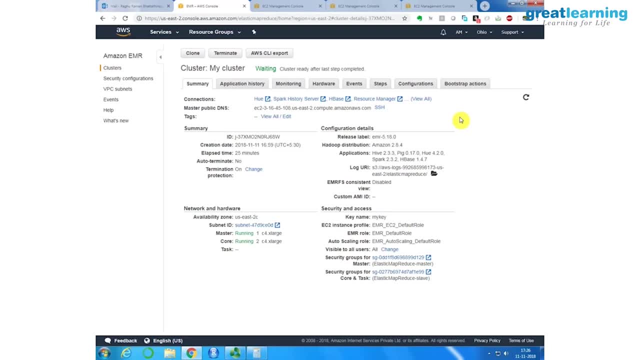 the data you can use, flume and all. but if I have a file? so let's say I have a file, I just want to upload it- how do I do it? so let's say we have a file, so I'll just go to my google drive. 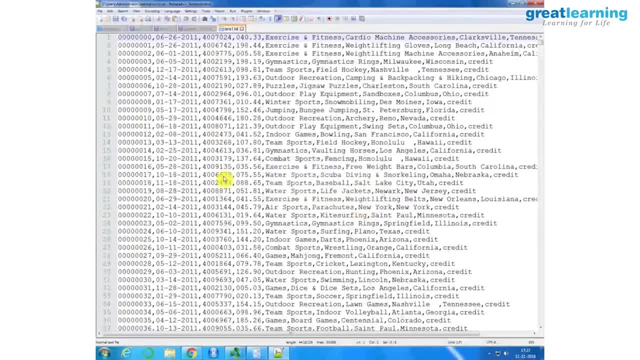 I should have some file. so this is a typical transaction data from a retail store. you have a transaction id, then there is a transaction date. a transaction date. you have a customer id. amount spent. category of item: he bought puzzles. within that he bought jigsaw puzzle. city of Charleston, uh. state of South Carolina and a. 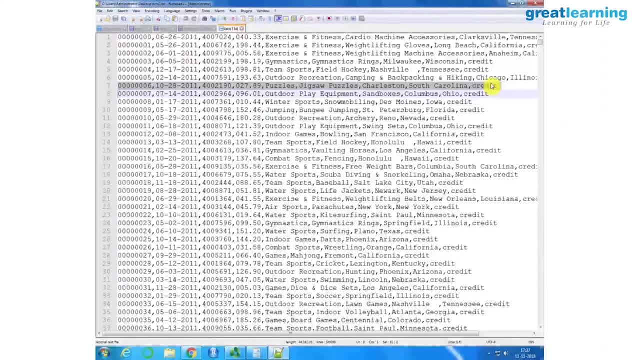 credit transaction. so it's a typical transaction data. now, let's say, in our emr cluster, you want to, and you want to create a table from this file, probably analyze some data. right, let me see, let me show you how easy it is to do so. all you need to do is: 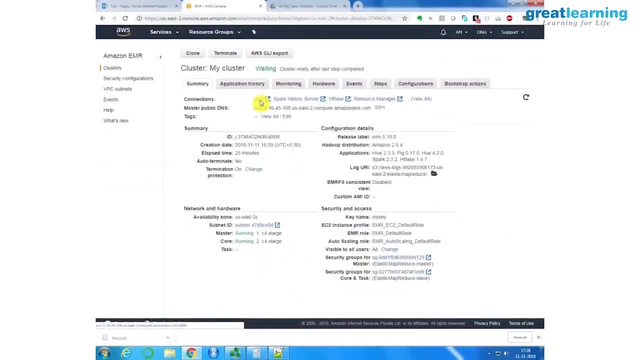 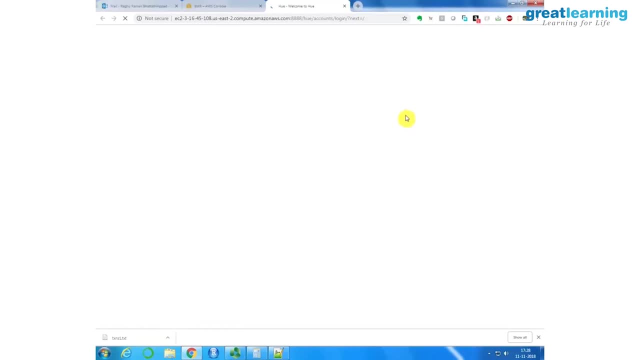 If I go to EMR there is something called Hue. Can you see H-U-E? Just click on this Hue, And Hue is basically a developer's UI to the cluster. So I can just open Hue And it will ask me to create a user account. 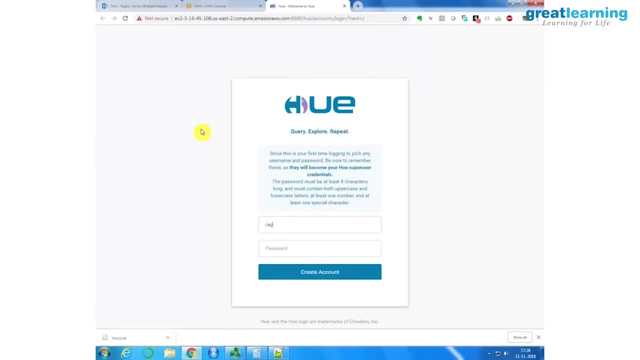 since I'm doing this for the first time, So I will say my username is Raghu and the password is some secure password. I will say create an account. Account created, I logged in and I will just switch the version because this is, I think, Hue 4, which is bad. 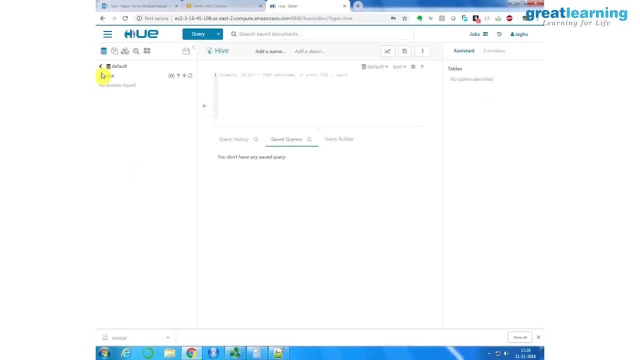 I need Hue 3.. What I can do is that I can go to. So Hive is already here, You can see this right, And I can create a table very easily here. So let me see browser tables. I can go to table. 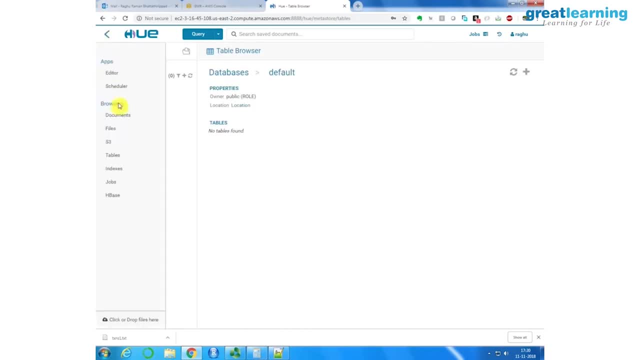 Before that, what I will do? I will go to files, And this is my Hadoop. This user, Raghu, this folder is actually my Hadoop, And if I want to upload a file, I can just drag and drop it here. 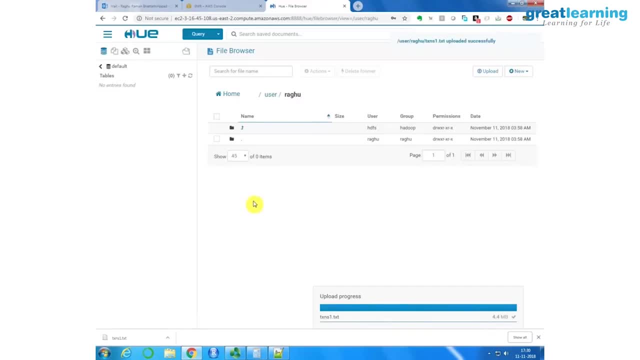 So you can see the file is getting uploaded. So now this file is available in Hadoop And my intention is: I want to create a table from this file. Then I want to query the data. To do that I can simply go here. 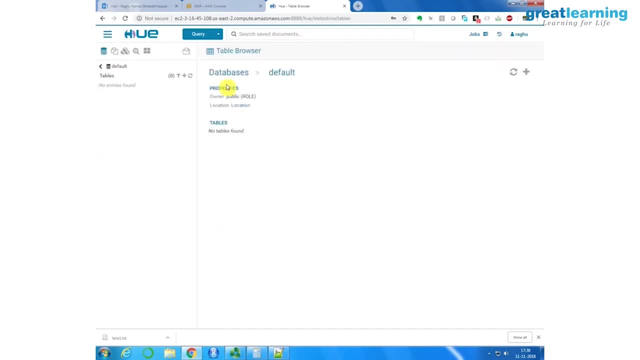 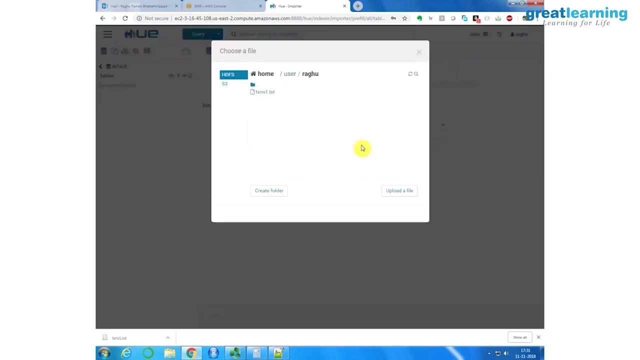 This is something called tables and go to tables And there is a default database. I can say this plus button, create a new table And it will ask: where is your data? My data is in a file And where is the file. 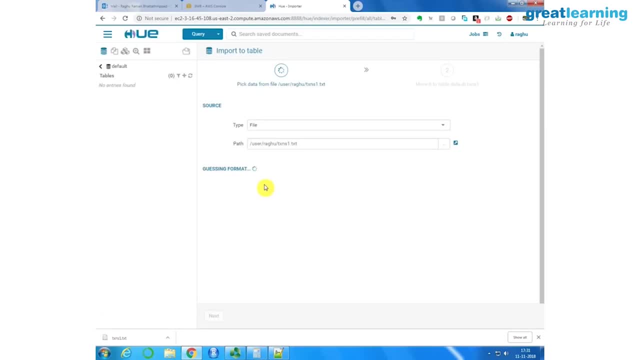 We just uploaded right This transaction. I'll select it And once you add the file, it will automatically figure out the format. This is like Alexa thing, right? So like automated. So see, it is saying that there is a field one. 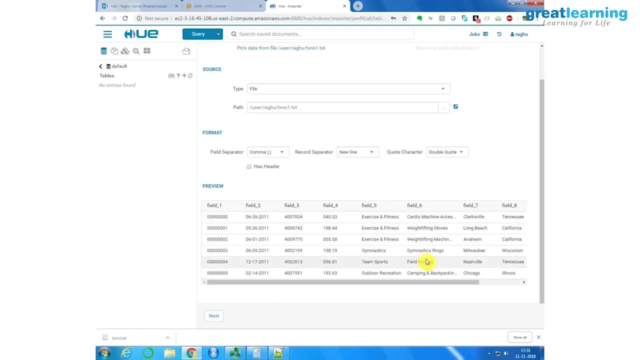 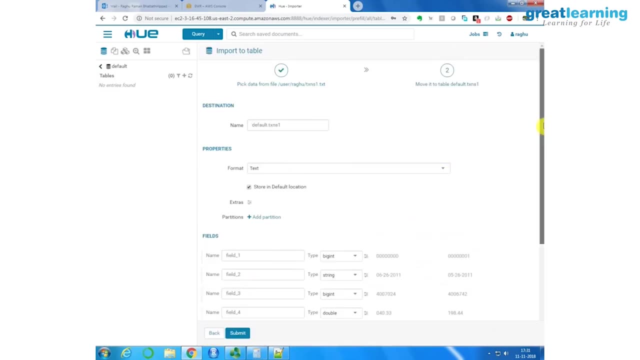 field two, field three: These are all the values you are having. Is this correct? Yes, it is correct. So I can simply say next, And it is going to automatically assign all the data types, String double, to all the columns. 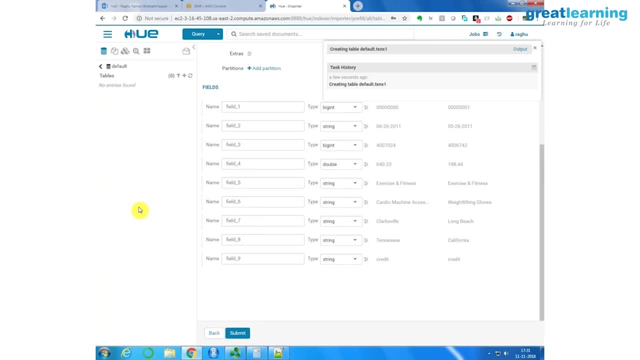 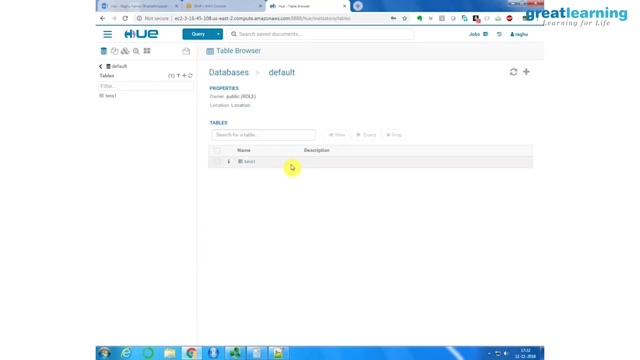 I say submit, So I just click the submit. It is saying: creating table default of transactions Already exists. Yeah, the table already exists. Now I can just go here and again go to my tables menu And there is a table for transaction. 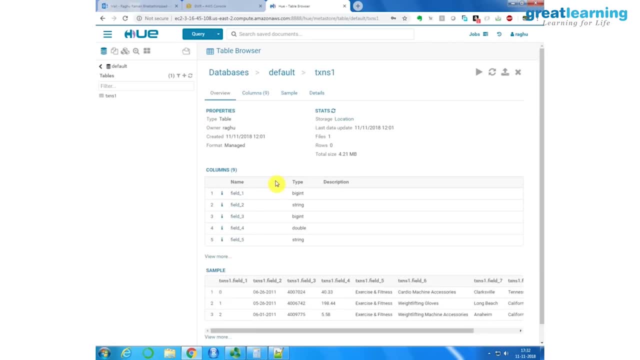 If I open this table, this is the sample data. right And okay. so now the table is created. So you did not write the DDL statement. It automatically created. It internally wrote it. Now, if I want to query that, I can simply go to query. 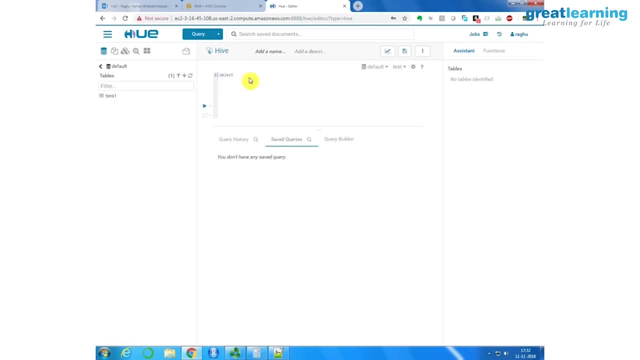 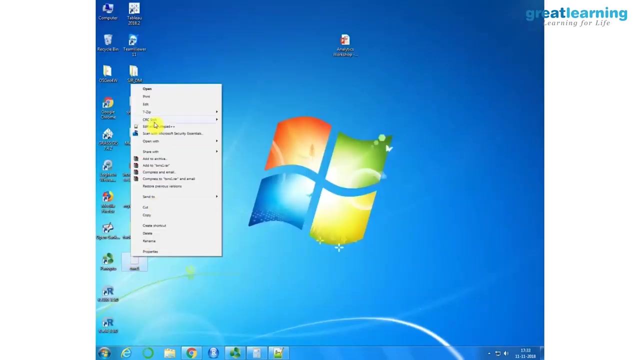 Okay, And here I can say: select: Start from TXNS1.. Limit: I don't know. Now the beauty is, let's look at the data. So I want to just query something different. I want to select all the data where? 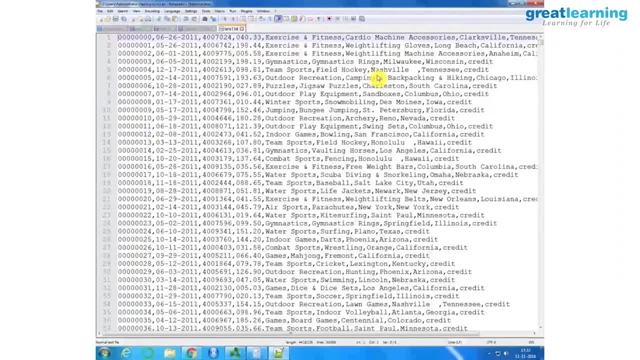 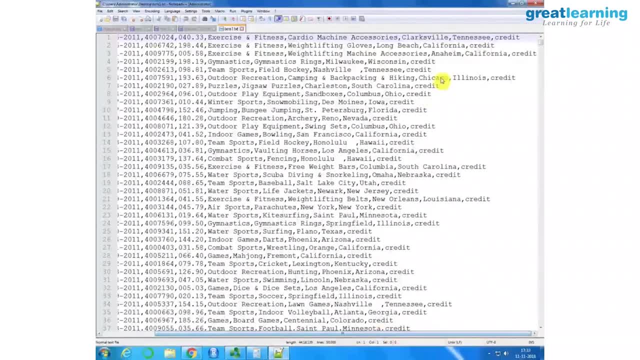 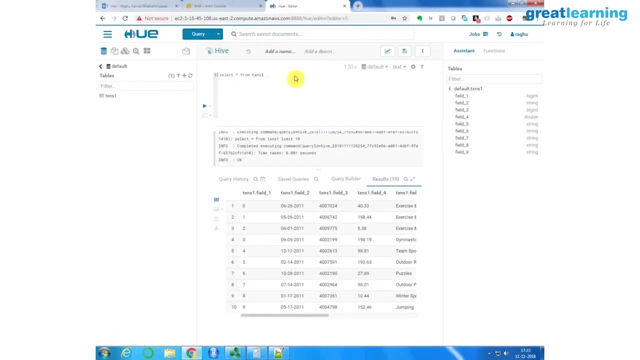 You can do it in the I don't know. You can say where the state is: California, right? Yeah, So that is which column Last, but one column. So here it is field eight, right, So I can say select star from transaction S1.. 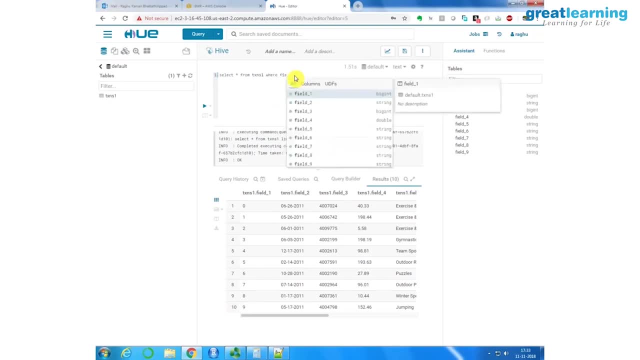 Then what you say Where Field eight, Field eight equal to single quotes or double quotes. I think single quotes, single quotes, right, California. So I want to show you something. If I run this query, I will get the data. 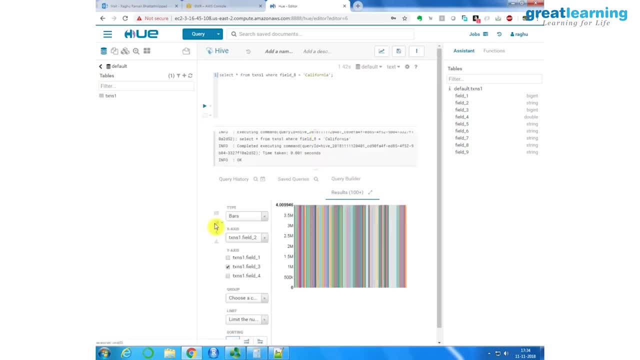 Now you can also visualize the data here. I can go here. okay, See, I can set up the type of visualization: pie chart. Well, this does not show anything because the query is simple, but you can have all the sorts of visualizations in the data. 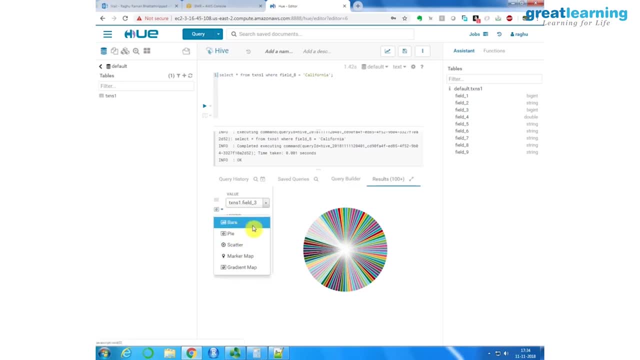 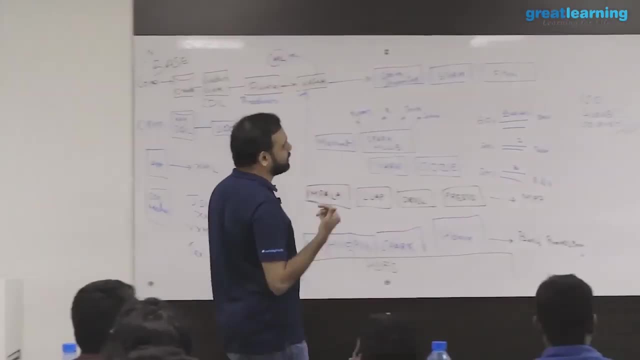 Scattered map, pie chart bars. Remember your BI class? So here by default, allows you to do the same things on big data, So it's really nice. You can also download the results as a CSV, as an Excel file, export as a PDF. 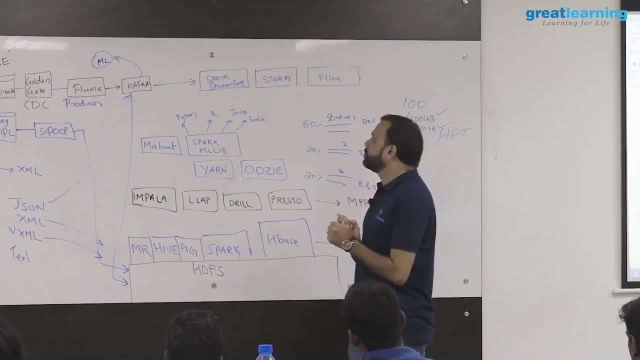 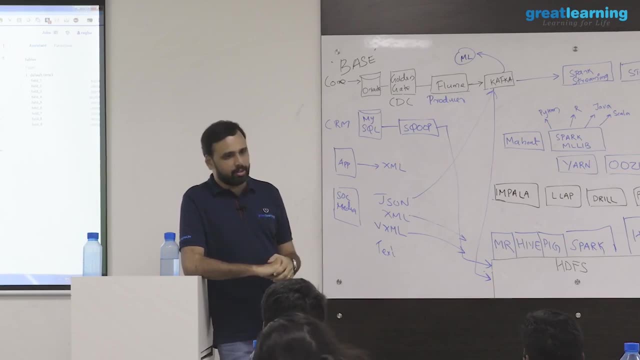 So this tool here is available on EMR. So in this cluster I mean, if you want to run Spark, you have to start a Spark shell. okay, You have to say Spark R, but I may not be able to show you it completely here. 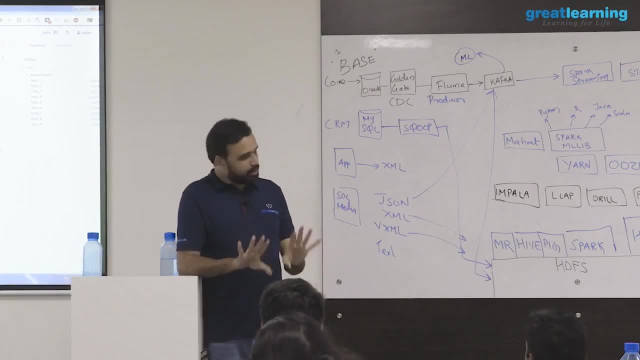 because it will take time. You need more. you need R knowledge, but you also need to understand Spark a little bit. So there's something called RDDs and data frames and we need some data also to build. But you have to start. so Spark works on the command line. 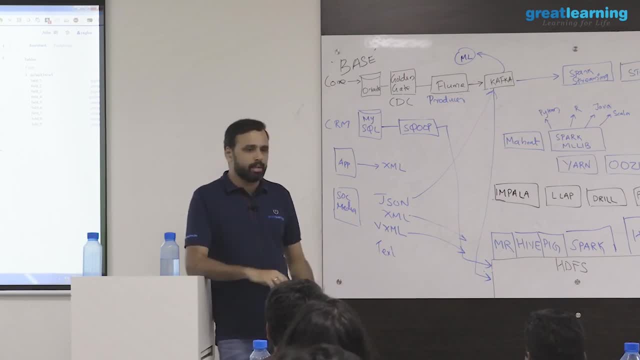 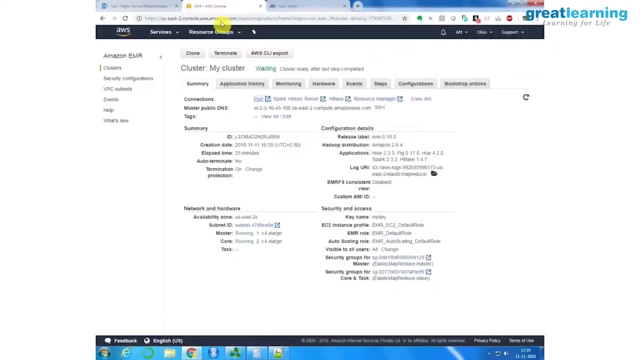 Normally you can use UI, but that's not very effective. There is a Spark shell. you have to start In that shell. you have to type the commands that you require. Okay, I want to show you one more thing. I told you there is a UI for a resource manager. 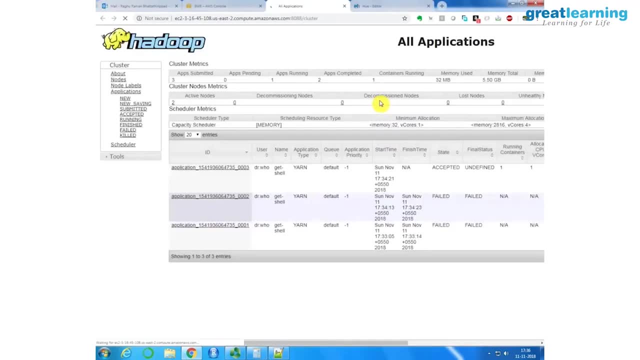 Here it is. You are asking: how do you look at the jobs you are running right? Can you see here Yan yan yan? So three queries. we ran all three here. Can you see Some of them failed. 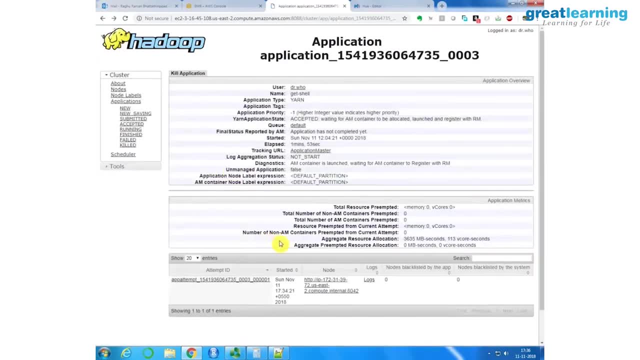 So this, if you look at here, it's not showing that because it is an internal IP. That is why it is throwing an error, But it says accepted default and all. So you can troubleshoot from the logs For EMR. there is a problem with logs actually. 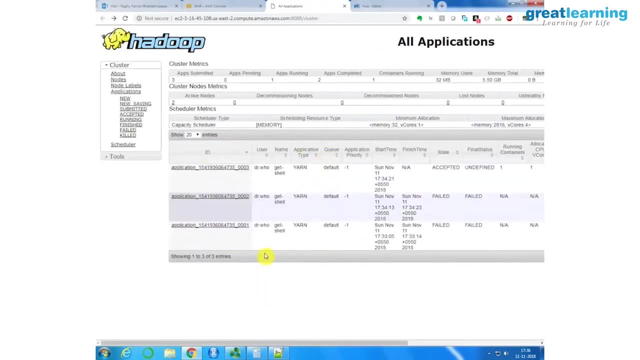 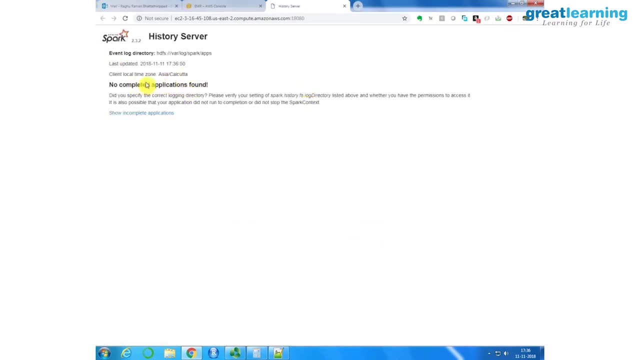 but in the Yan window you can see that You can run the queries and see the output here. So this is the Spark history server. There is something called Spark history server where all the so no application found If you're doing something. 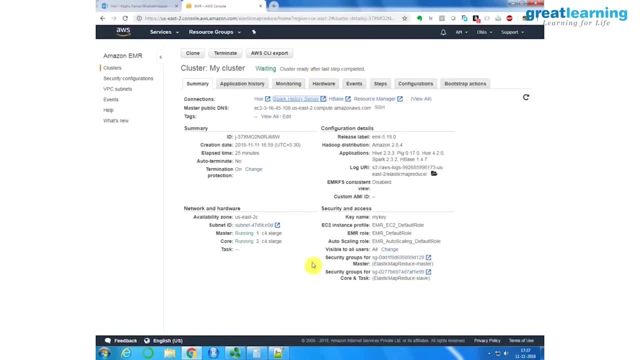 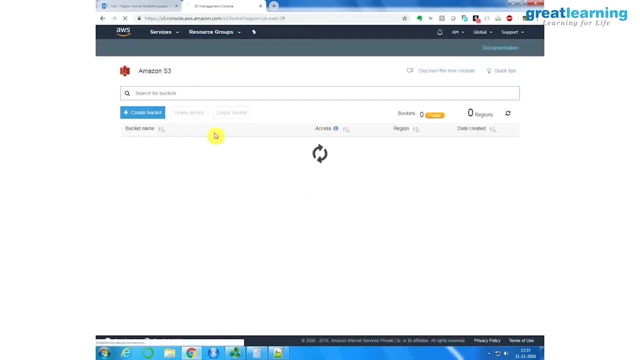 in Spark and you close it, it should come here. So I will terminate the cluster In Amazon. I told you there is something called S3 also, This is Amazon S3. This is where you can store, like I said, unlimited data. 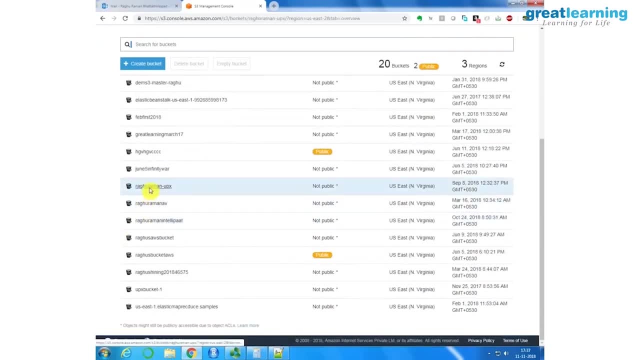 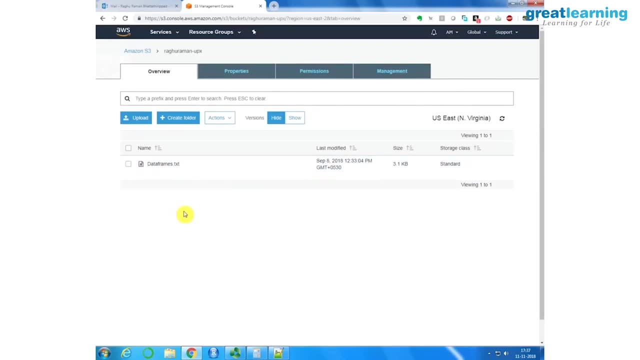 You can see all this data right, But I don't have much data. but if you open, you can just upload the data like this. So very easily you can upload the data And S3 is like an FTP server: You just upload it and keep it there. 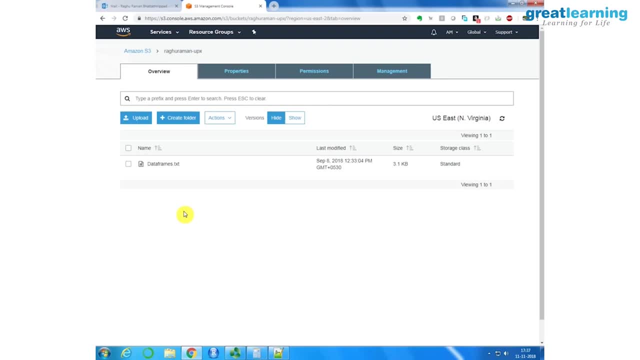 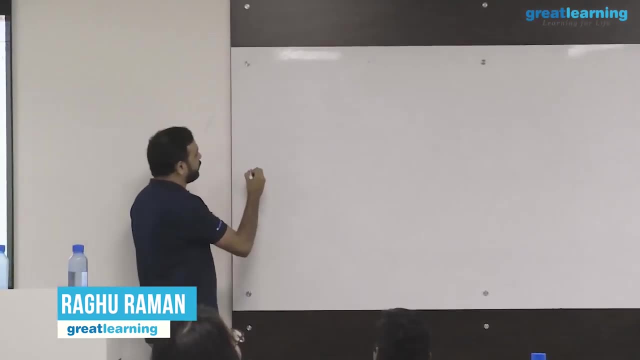 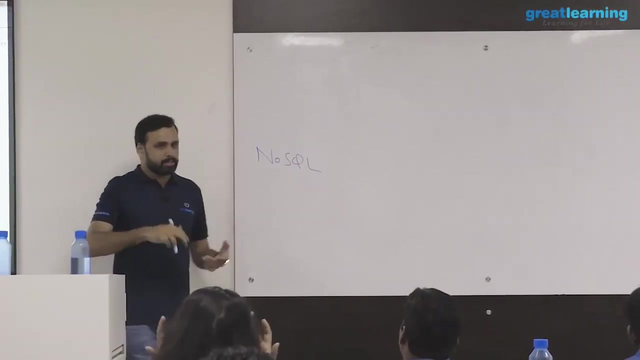 You cannot modify the data, Just dump it and download it. That's all. The idea is to talk about big data, right? So I must also tell you at least a bit about something called NoSQL, right? Maybe not in depth, but like many people, 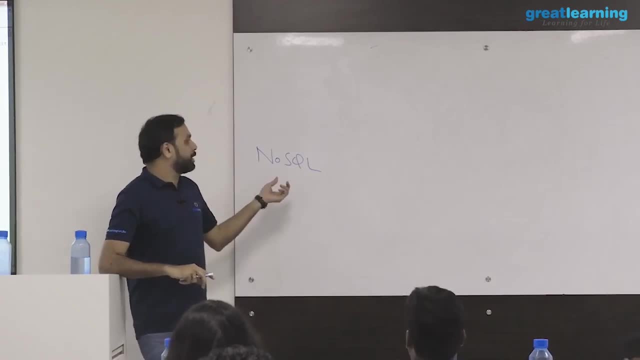 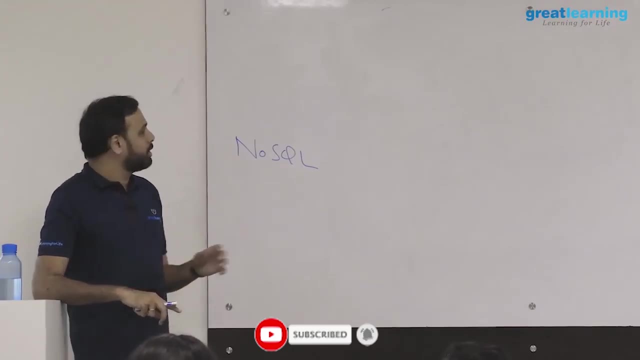 asked questions also. So normally your RDBMS systems and all are built on the idea of SQL. You know what it is. I don't have to teach right Now. NoSQL databases are the databases we use in the world of big data. 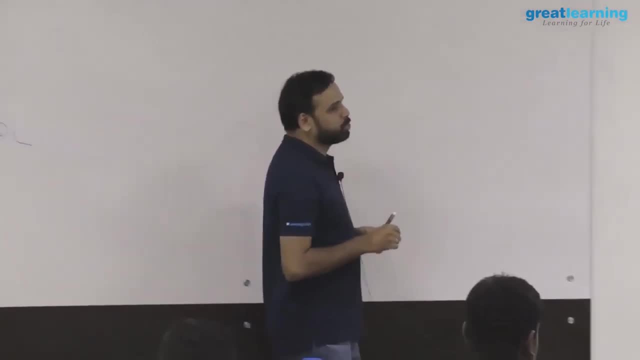 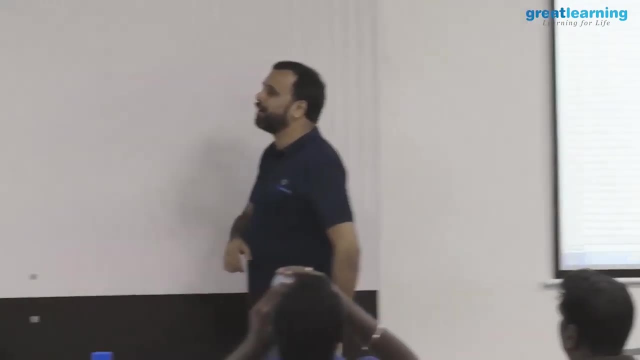 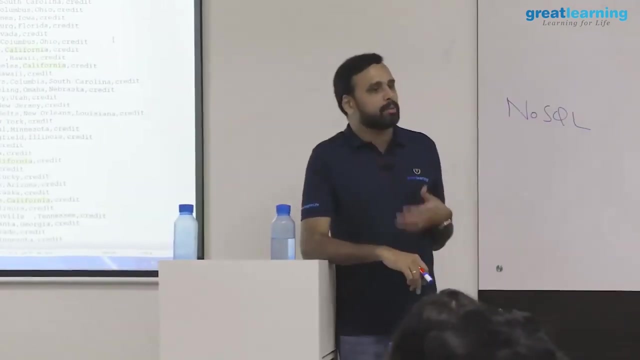 So the simple definition is that this is a database which you use in big data. Why? Because Hadoop and all are not databases. Hadoop and all are analytical platforms. So what if you have a requirement where you need a real-time response? 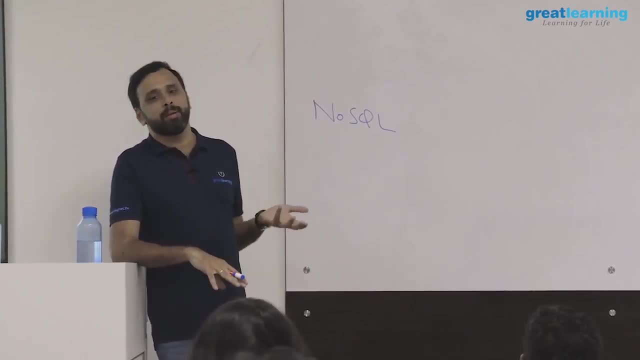 For huge amount of data like an RDBMS. So what is the primary purpose of an RDBMS? Client interaction? Somebody is interacting. they should get the output very fast, right? What is the same thing you want to achieve with big data? 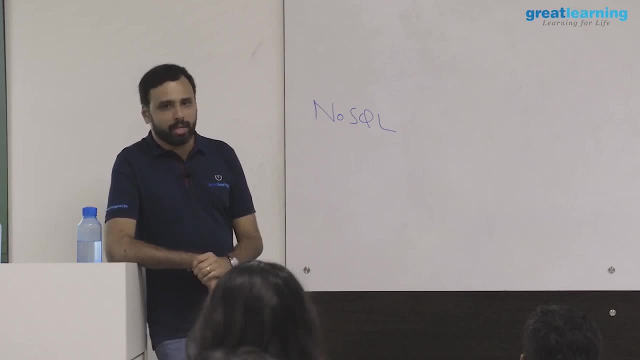 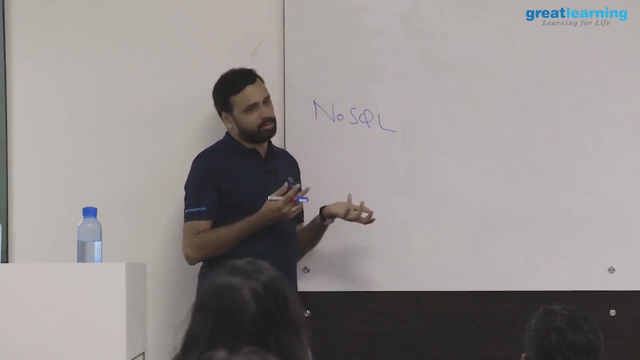 Then you will be using something called NoSQL databases. Now, this is a very huge topic and I may not be doing justice by covering this in half an hour or something. So somebody see that then. So it's actually a very pretty huge topic, okay. 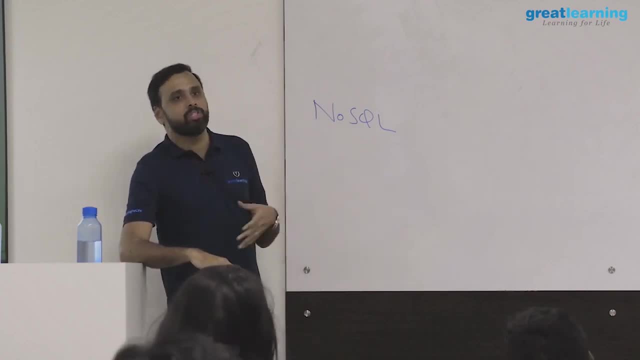 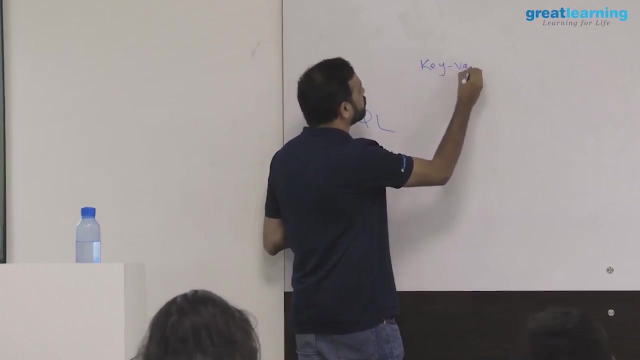 And there are too many things inside this, but just to give you some basic pointers. whenever somebody say NoSQL, there are four categories, and that is something very important. So you have something called a key value store or key value base. 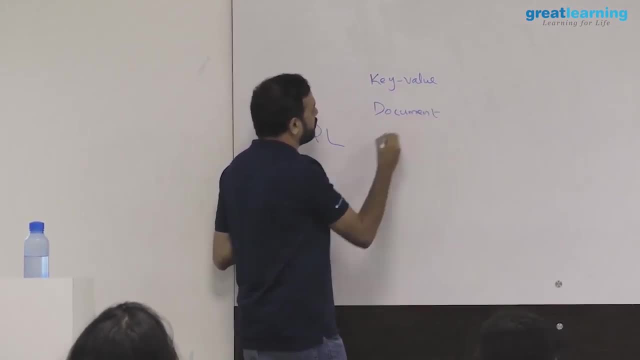 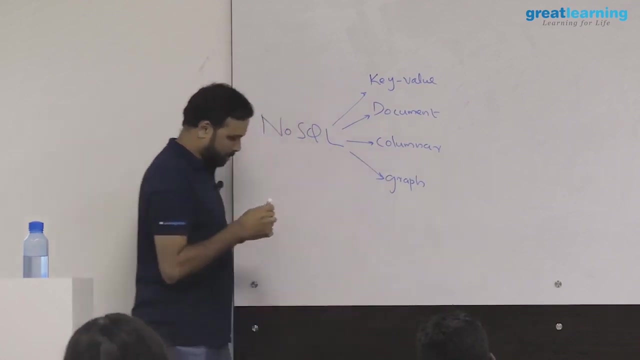 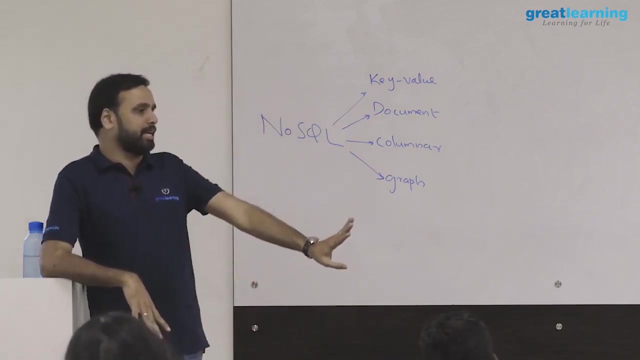 and then there is something called document based, Then there is something called columnar And then there is something called graph. So four major categories are there in NoSQL. So first question you need to ask is: somebody is saying that, okay, I'm using NoSQL database, which category? 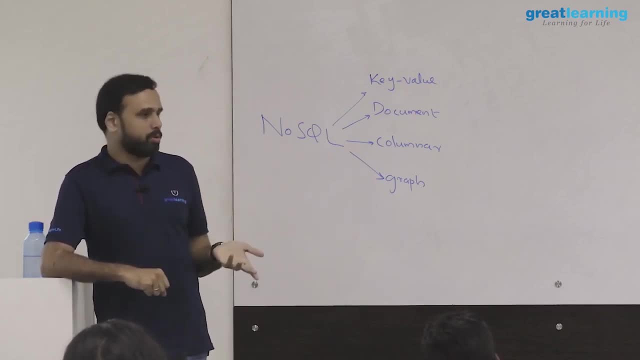 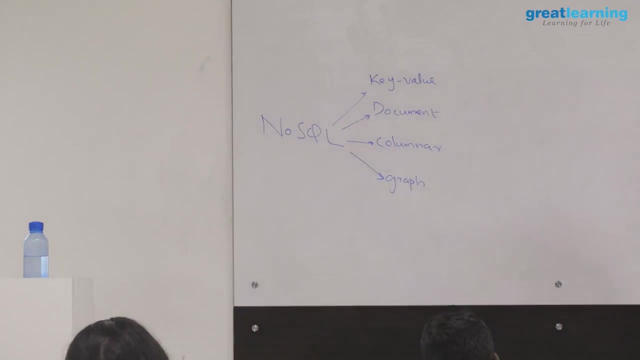 And they must be able to tell you one of this: There are more than four, actually, But and how many normal SQL vendors you know, Like normal RDBMS? how many vendors you know? So let's say, Microsoft is there, right? 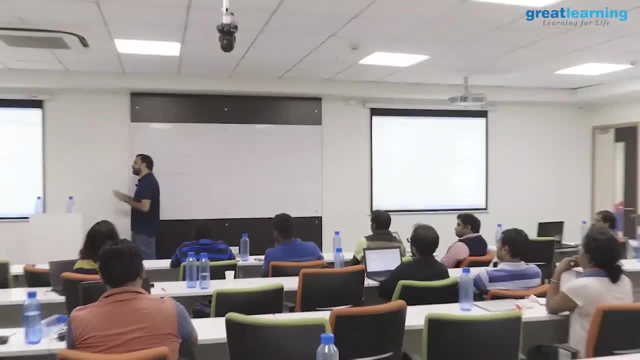 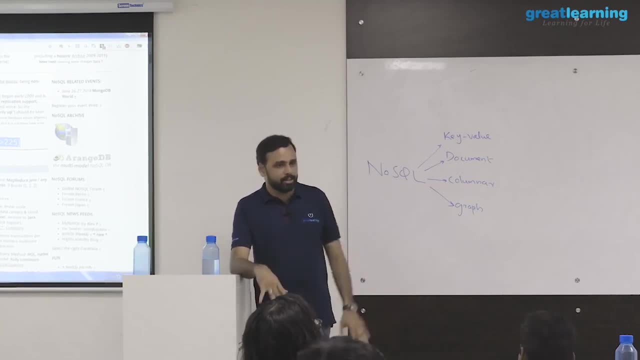 Who else is there? All right, like that. how many will be there? What do you think? Because of another reason, because NoSQL is not a mandatory concept. It's not like everybody should learn. If your company is using it, you learn. 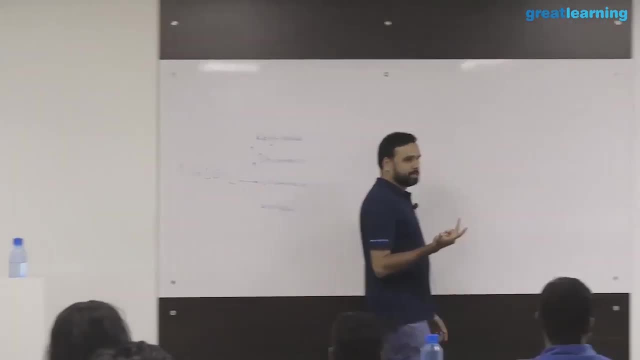 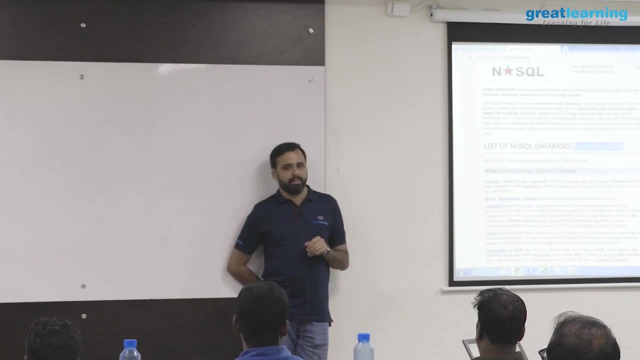 And in many companies when I have gone, they are using NoSQL databases And the developers who are working on them do not have a complete idea, and that's perfectly fine. Nobody's asking you to sit and learn the complete NoSQL. So many companies use NoSQL. 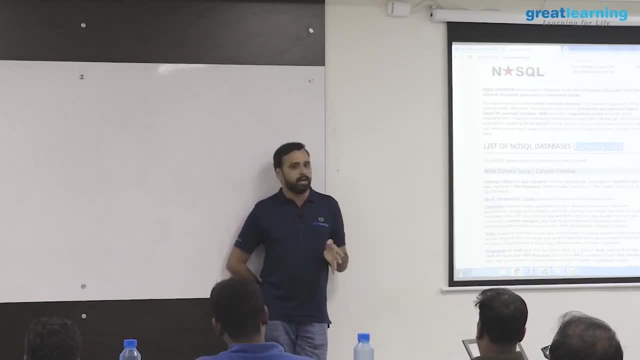 They know how to ingest the data, how to store the data, how to get the data and some very basic idea how to connect it and all That's enough. So it's not like RDBMS, where you learn theory and sit and understand internal of RDBMS. 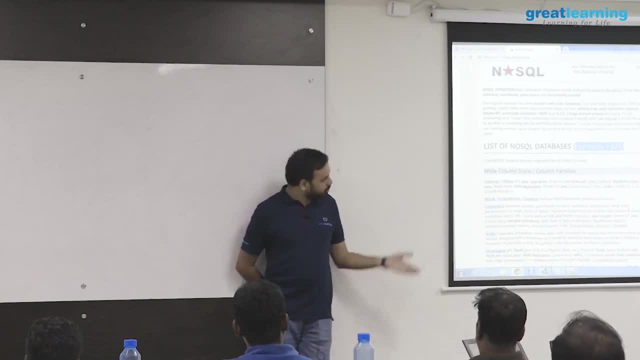 where the query is firing. That's not required, okay, And it is not possible. also, practically Humanly, I don't think it is possible to learn all this. 225 vendors are there as of now. okay, And majorly, there are four categories. 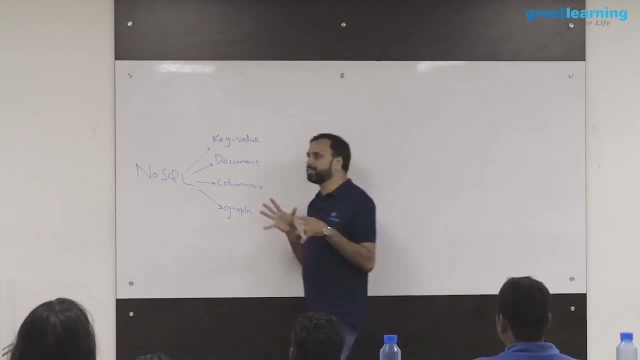 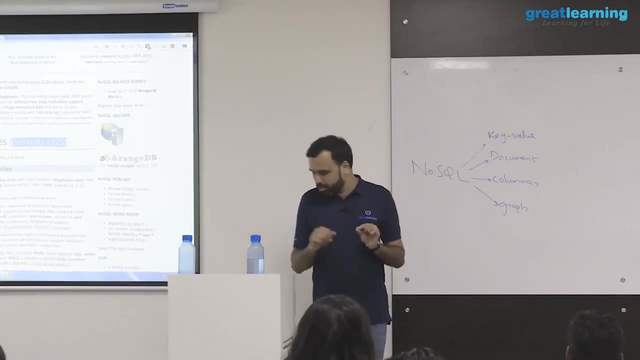 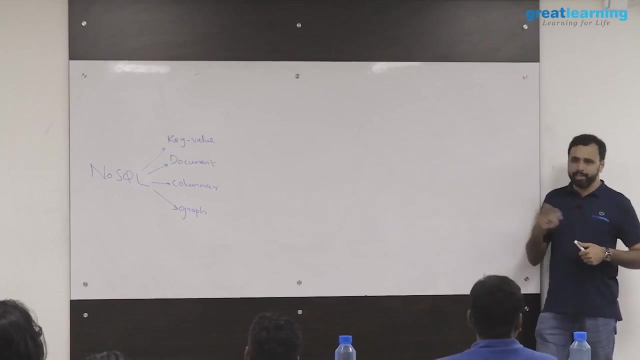 There are more than four, But commonly when people discuss theory they will say there are four categories. What is the basic difference in SQL and NoSQL? Let me ask you this: In SQL, let's say you are working for a production company. 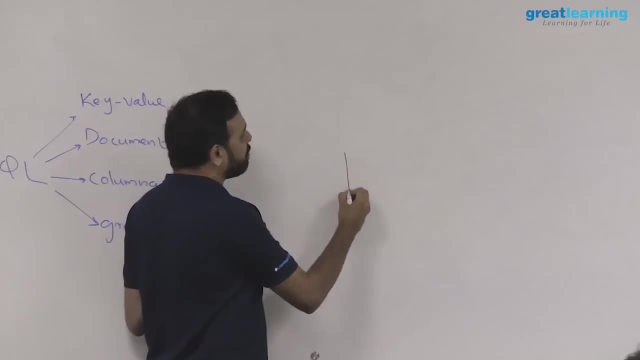 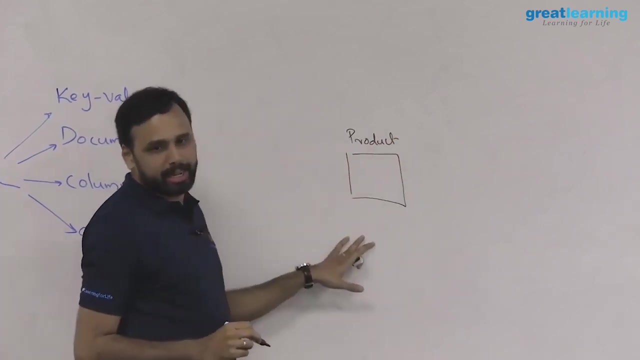 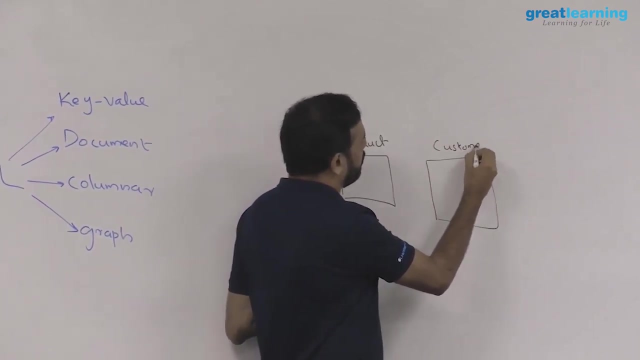 So you always do this right. You will have a product table. You will create something called a- I'm just giving an example. okay, A product table. Then there will be a customer table, right, Then there will be a orders table, correct? 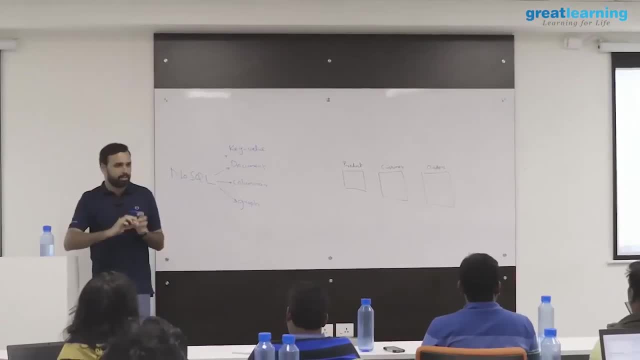 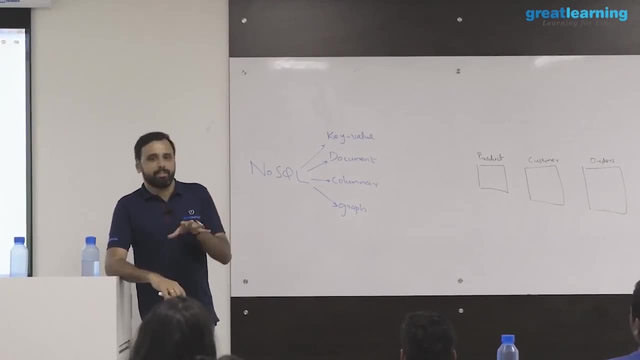 So whenever you define your schema in the RDBMS world, you always do what: Normalization or denormalization. Normalization, Yeah, it depends, But normally you will normalize it right And the basic idea is that you represent your data right. 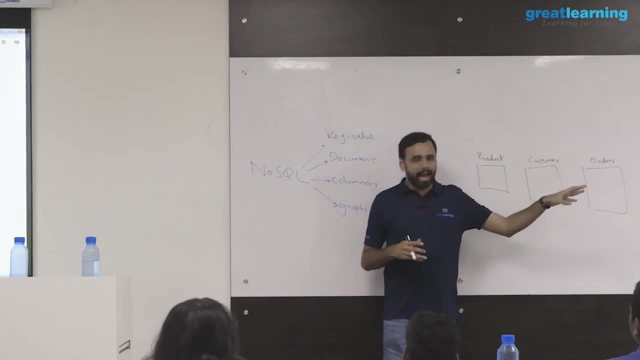 And the basic idea is that you represent your data right. And the basic idea is that you represent your data right. You represent your data in multiple tables And whenever somebody wants to get some answer, you write a join query, correct? 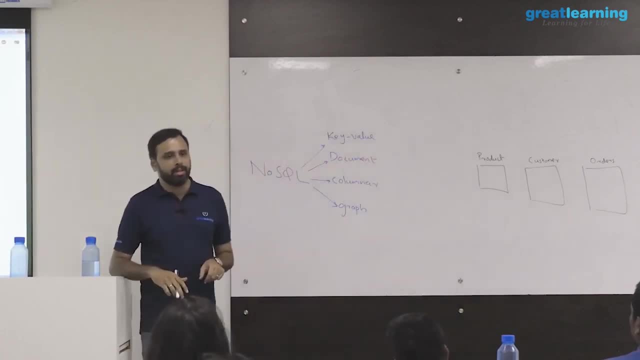 This has been the foundation for every RDBMS. In NoSQL, there is nothing called a join. You cannot find the word join first of all, And they don't follow this concept. That is the starting point of discussion. Now, this concept itself, we can discuss for a day, right? 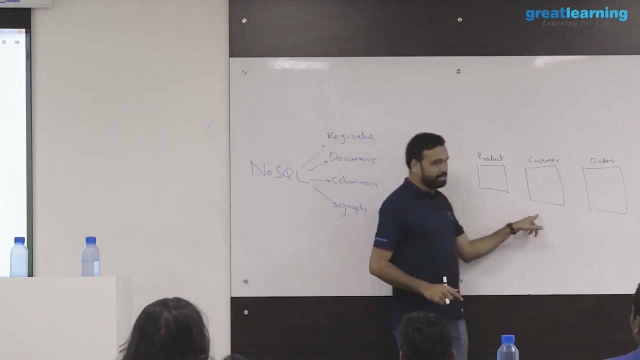 So basic idea is that you don't represent the data like this. Why? Because if you're having small amount of data, this is nice. But what if each table is one terabyte? Then every time you have to do a join query. 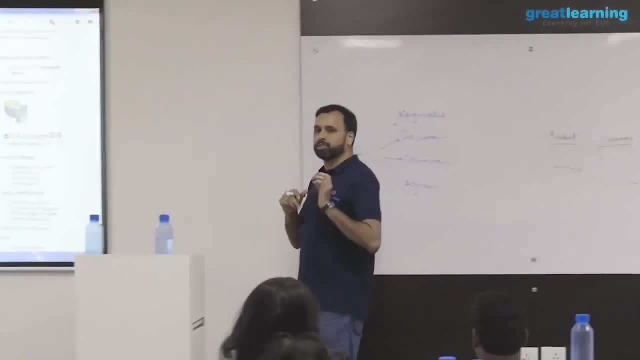 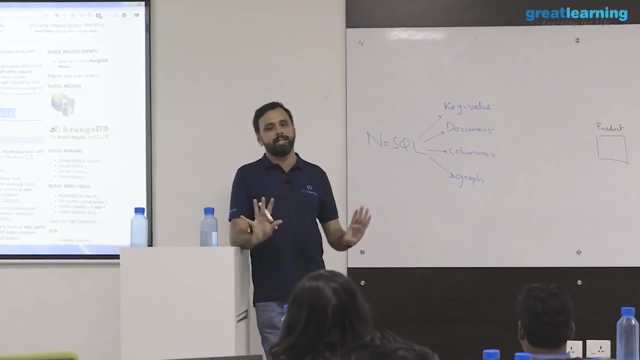 every time these three tables have to be joined, So that is not possible for me. So when I come to the world of big data, my data is big, my tables are big- I want to eliminate join operations. So what we do in NoSQL is that we create a single table. 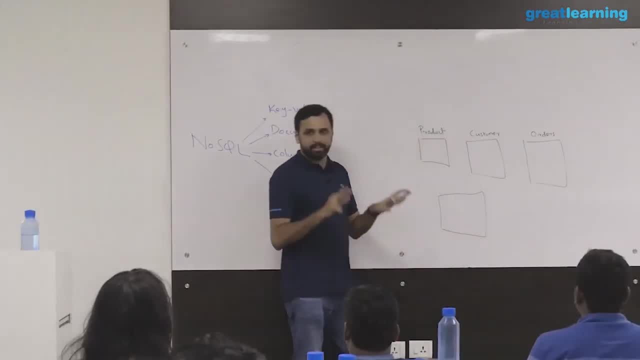 We don't even call it a table, something. We create a single thing. We create a single thing where all these three things are present: Complete denormalization. There is nothing called normalization. This is the basic principle in which NoSQL is built. 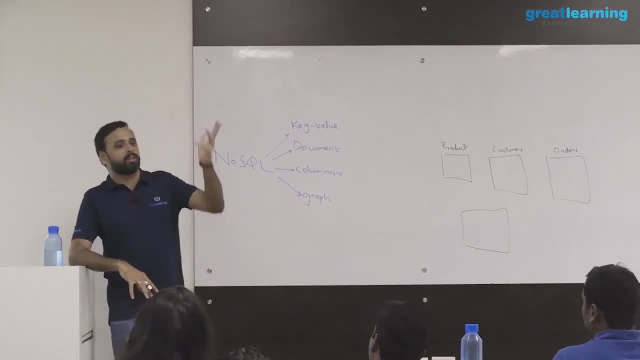 Which also poses a lot of questions. I know how this is possible. What on earth are you talking about? and all But understand. No, that's what there. all the concepts are different. So in normal RDBMS, of course. 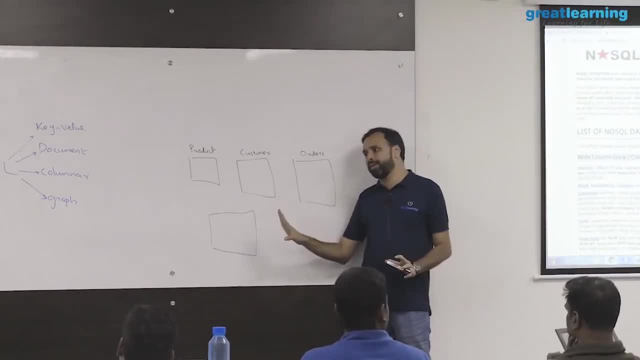 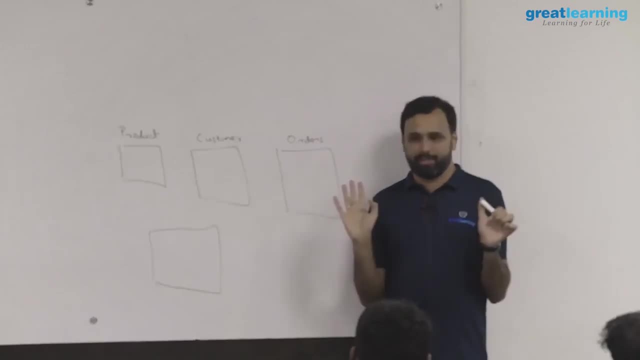 first thing, you are using a language called SQL. Here there is nothing called SQL, So by itself, all the concepts that we learned are gone. Any concepts you learn is gone because no SQL. And so here another interesting point which people never understand is that 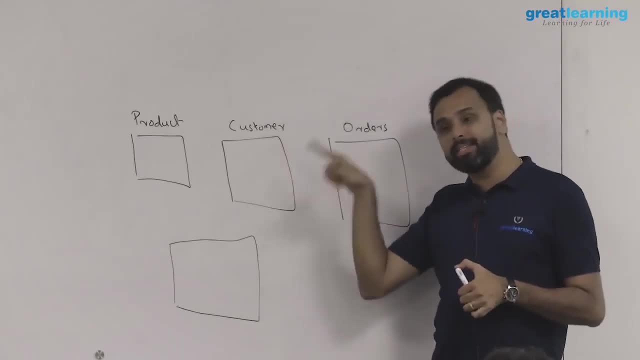 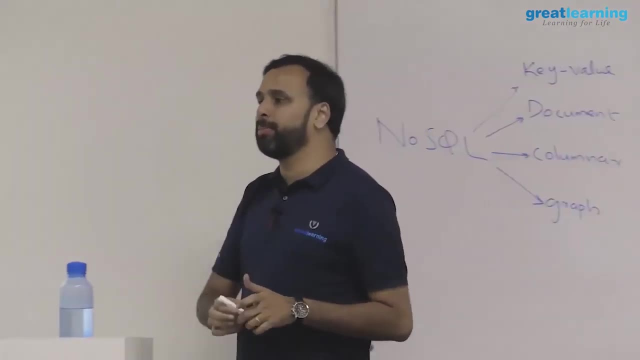 if you are firing a SQL query, who is actually doing the job is the SQL engine. Meaning I'm writing a join query And the intention of the join query may be to produce top 10 records or something. Right Now, who is actually doing the hard work is the SQL engine. 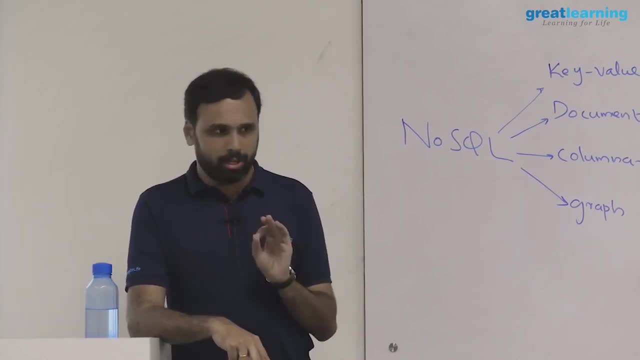 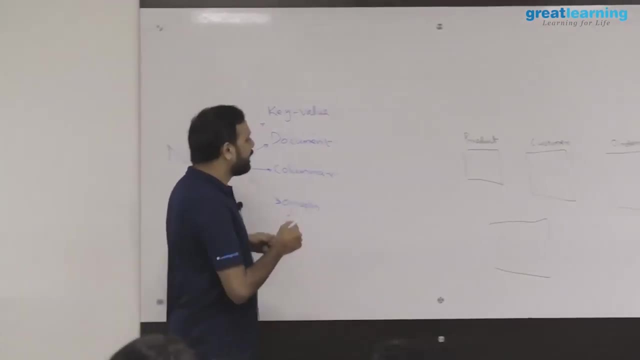 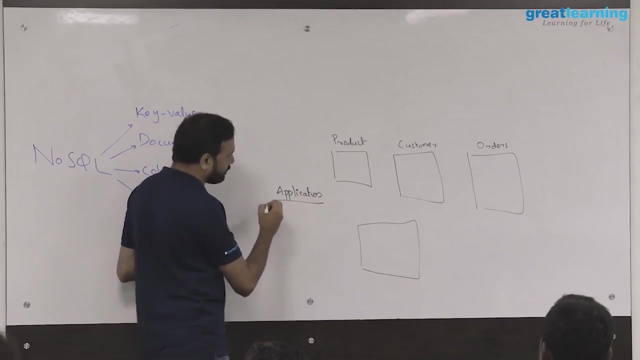 Right. That is why it is slow In a NoSQL database. the NoSQL database will never do a hard job, Meaning you will have an application. Have you ever thought about this? You open Amazon webpage, right. You open Amazon webpage when you click on a product. 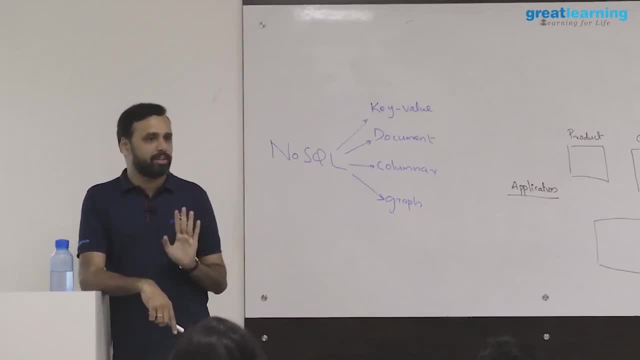 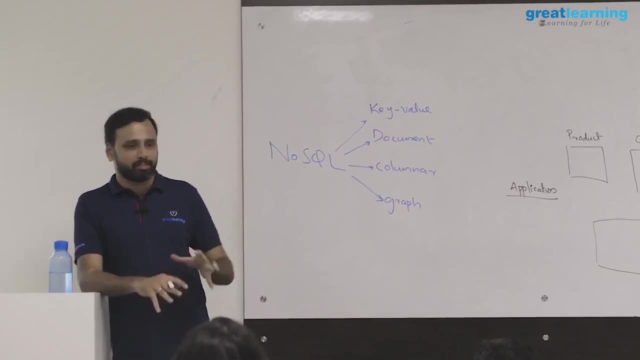 The product page loads so fast. But have you ever thought? Millions of customers are accessing Amazon And millions of them are clicking on different, different product page. Did it ever happen to you that takes five minutes to load a product page? No, 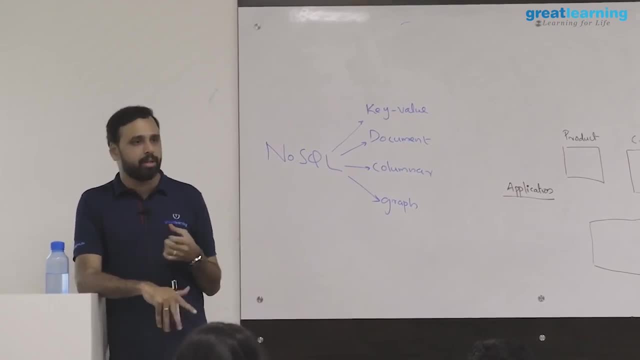 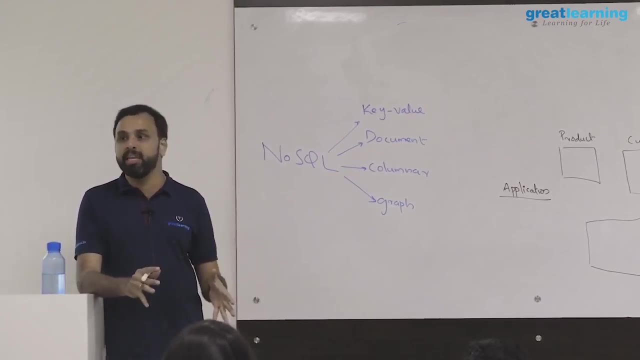 And look at the amount of information you have in a product page: Amazon, The images, reviews, ratings, blah, blah, blah, Like. if I have to represent it as a table, minimum 500 columns will be there, Correct? Have you ever scrolled through a product page? 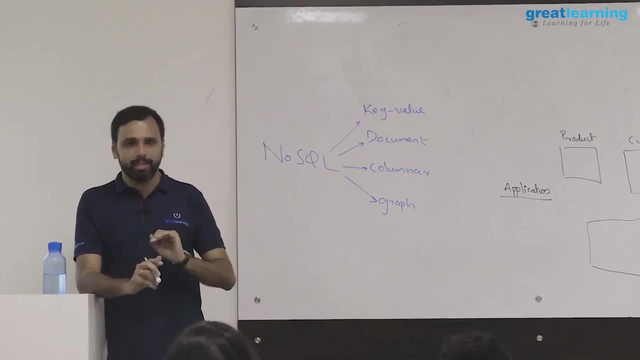 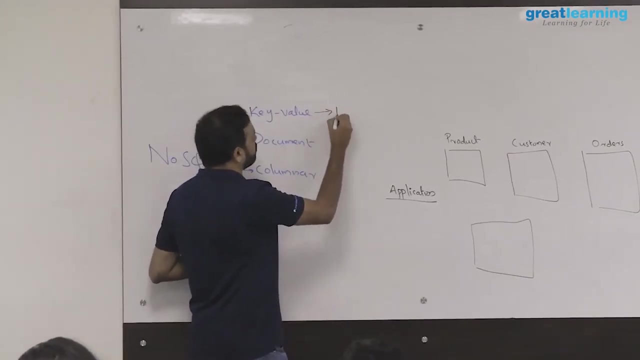 and see what amount of information it has. So what Amazon does is that Amazon uses something called DynamoDB. Amazon's NoSQL database is called DynamoDB. DynamoDB is a homegrown database. it's Amazon's own product. DynamoDB comes in this part. it's a key value store. 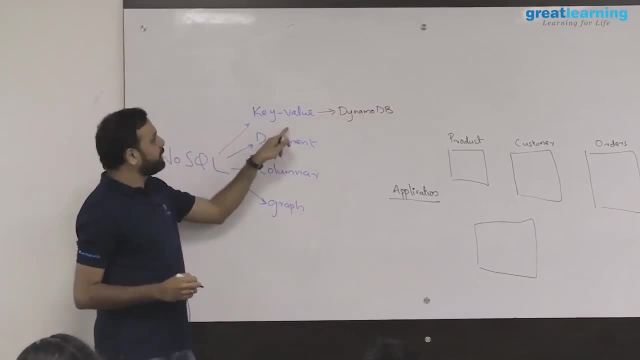 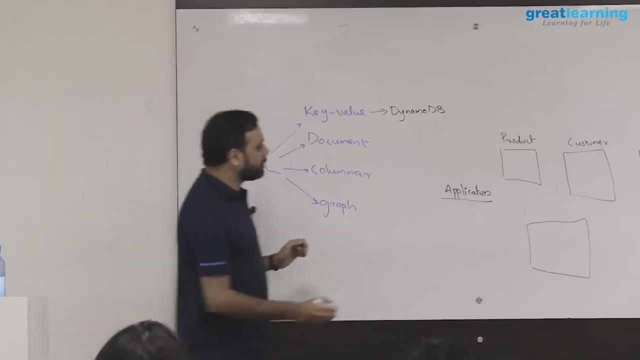 DynamoDB comes in this part. Now, just to give you an idea, what key value stores does they store the data in the database as a key and value. So Amazon has, let's say, a table-like structure where there is a key and a value. 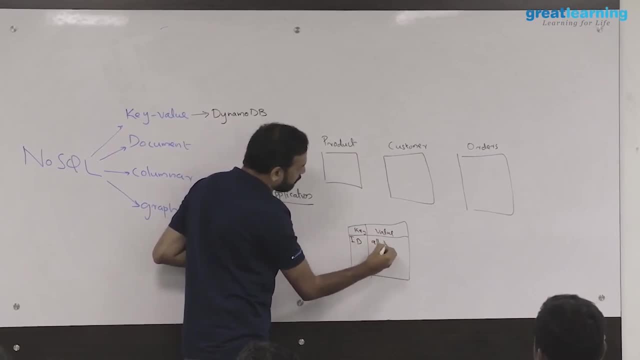 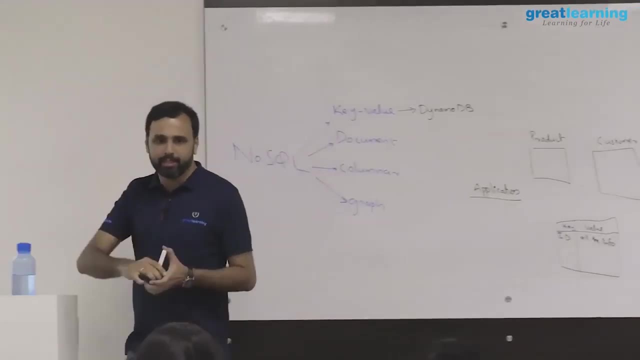 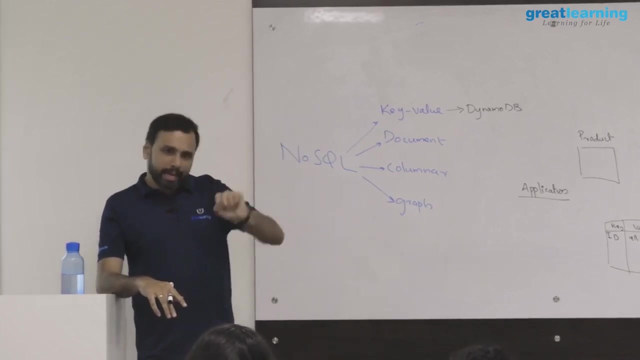 The key is the product ID. The value is all the info, Meaning if you are, when you're clicking on the product page, product link, that product ID is the key And all the data is in the value. Now, when you click, it is firing a query on DynamoDB. 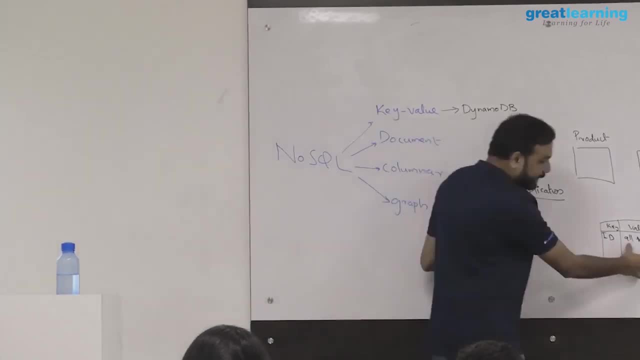 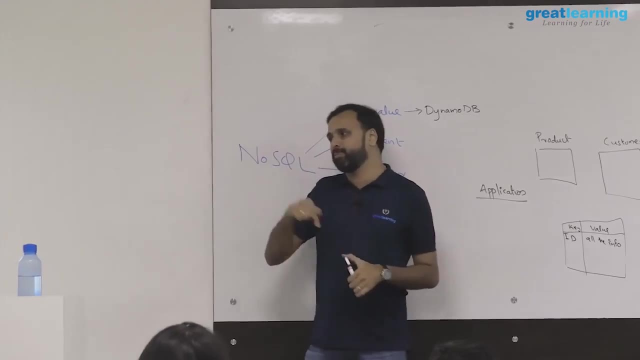 Okay. Now the beauty is it is just dumping all this data. Okay, And what to make sense from the data? the application layer has to decide, not the database. Are you getting the difference? In RDBMS, the database has to decide what should be shown. 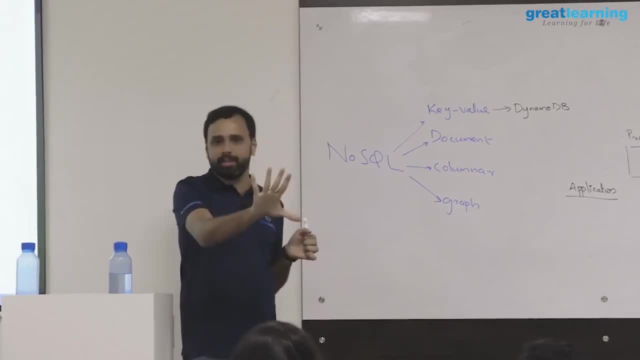 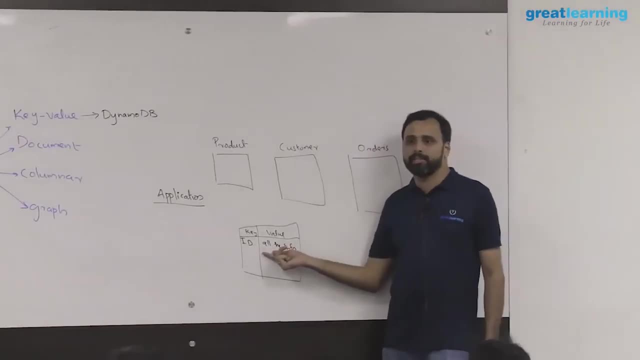 Here. NoSQL database is just like storing and producing the result. They don't do the analytics Meaning in this ID, the value part. it will have a lot of things like maybe the images or the location to the images, or URLs and everything. 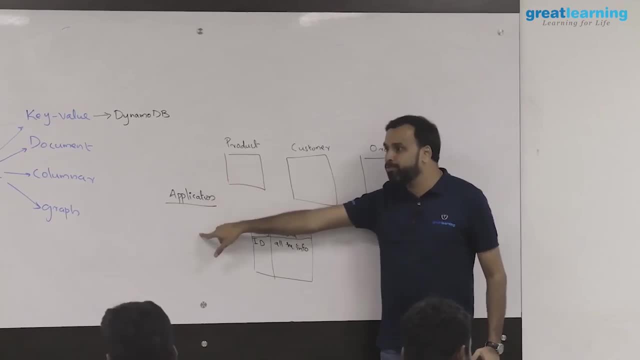 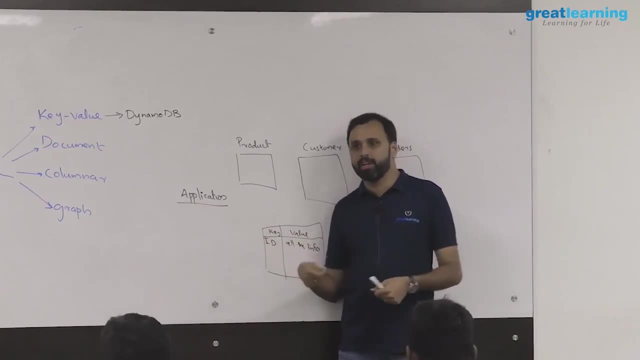 But we just have to push the application. The application has to be powerful, The application has to be powerful to display that. So the speed and all will come here, not here. Here also, speed should be there for the lookup, faster lookup. but that's okay, because otherwise 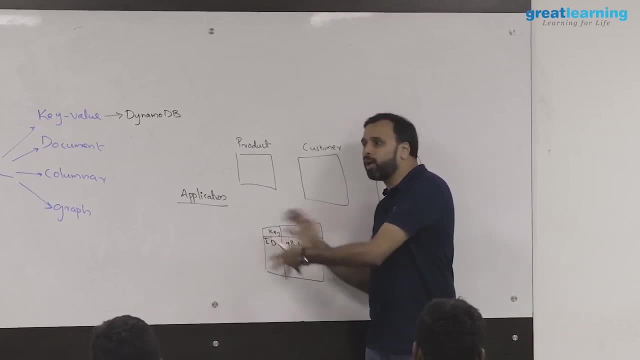 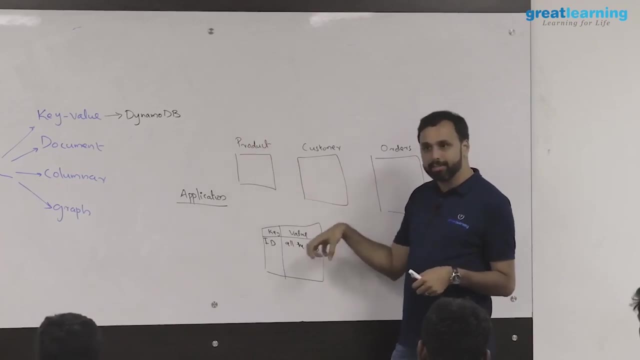 I should have created 10 tables for my single product and did a join operation every time somebody is clicking. That's impossible. I'm only talking about key value stores. okay, Others database also does similar, but this is the idea. So a lot of analytics did not go here. 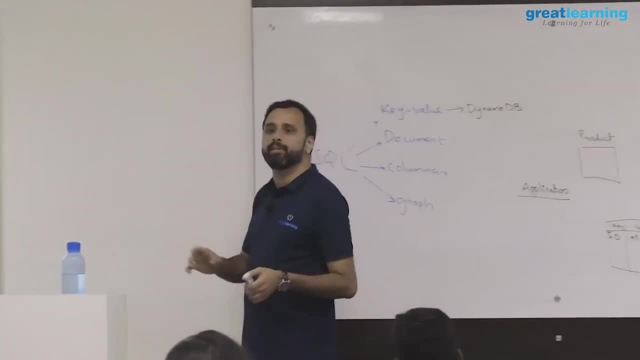 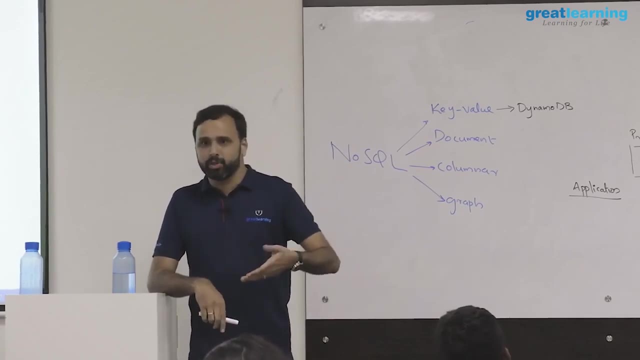 And accordingly, your queries are very simple. In fact, there are no queries at all. It is more like a select queries. So it's like scanning the data. So you should be easily able to find the data, get the data, What to do with the data, your application has to decide. 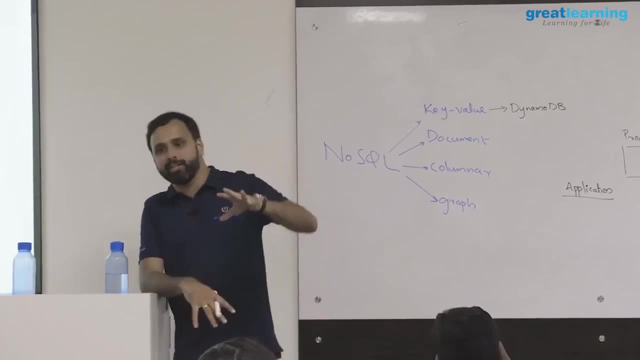 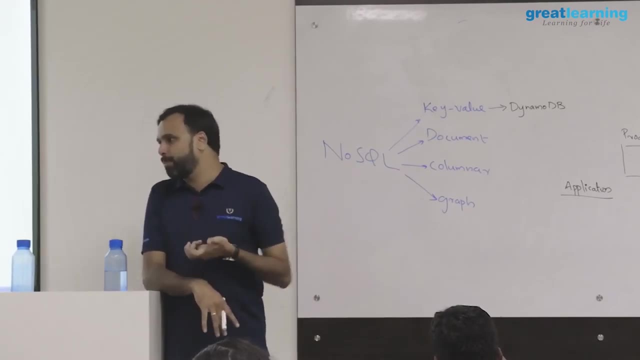 Not like SQL. In SQL, I'm like group then order, then join, then sort nothing, nothing. Give me the data, I'll do whatever I want. Now, who will do this? once you get the data? That is your application layer. 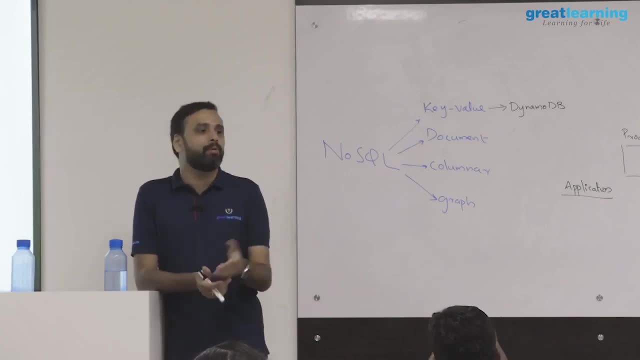 Your application layer may have anything. it depends. It may even have big data technologies, or you know it may even have big data technologies, or you know anything else, or very powerful applications, And that can- Any type of. so there is no specific type of applications. 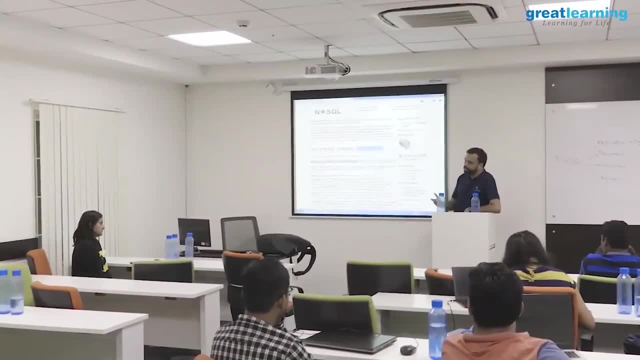 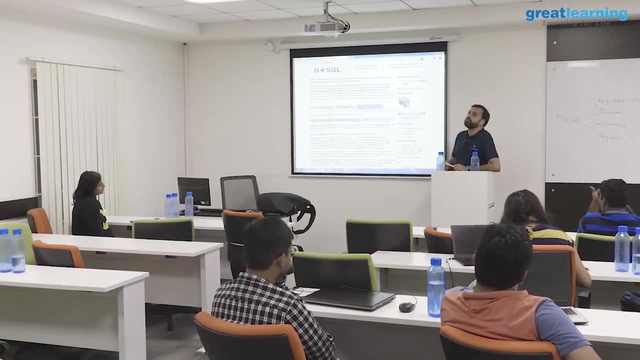 you can run any type of application you can run, Like from any programming framework. you can connect to NowSQL, right? This so the Java based applications and Python based applications. but here application framework has to be very powerful to serve the need immediately. 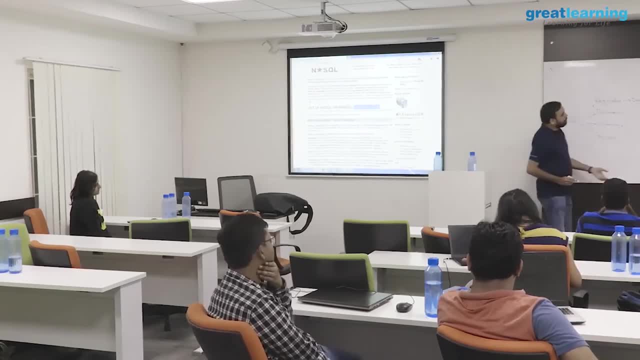 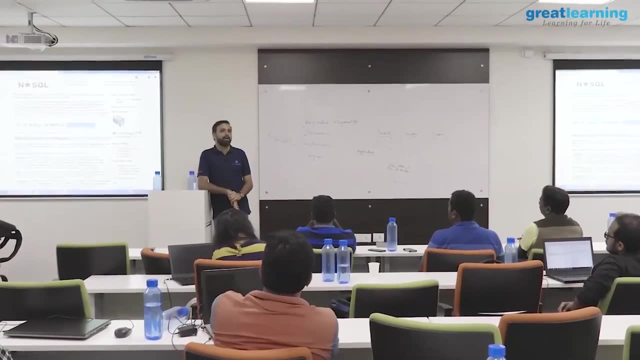 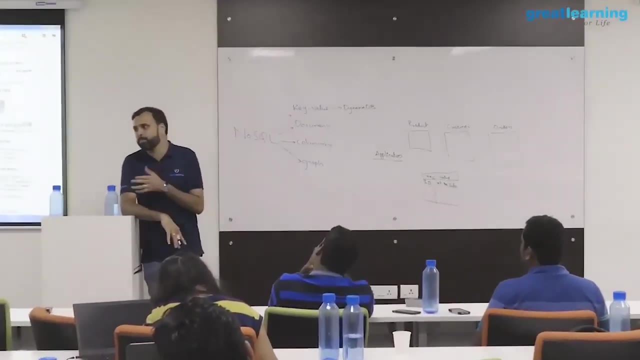 And another thing is that this may not be reliable. When it comes to reliability, NoSQL databases are not 100% reliable. You cannot say There are certain NoSQL databases which are reliable which you preference to reliability- Not reliable in the sense. 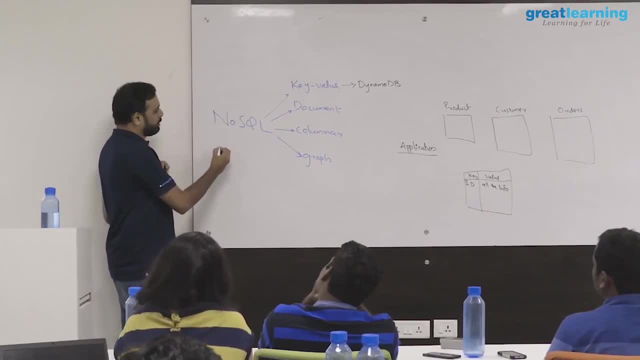 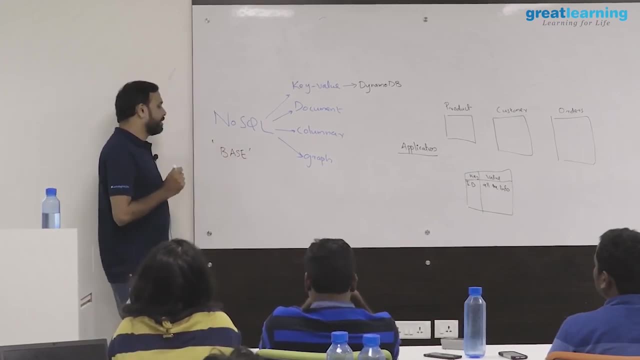 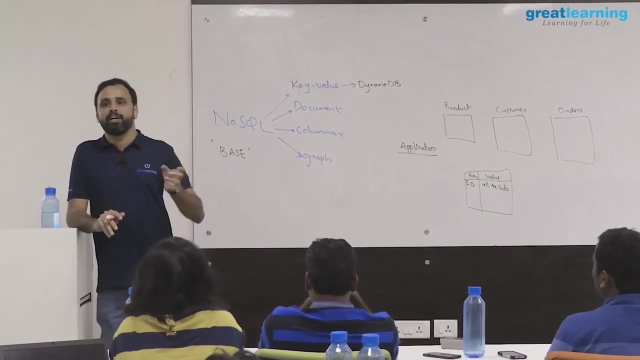 well, the reliability is actually built using something called a base. So, like I said, in ACID, here there is something called base, Basically available, soft state, eventual consistency. I think they just made it up to fit the. So ACID, the opposite of ACID, is what. 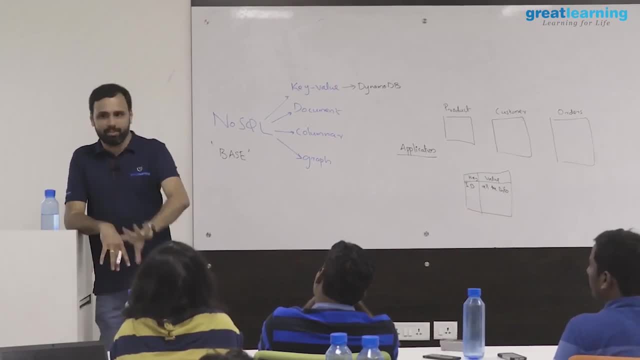 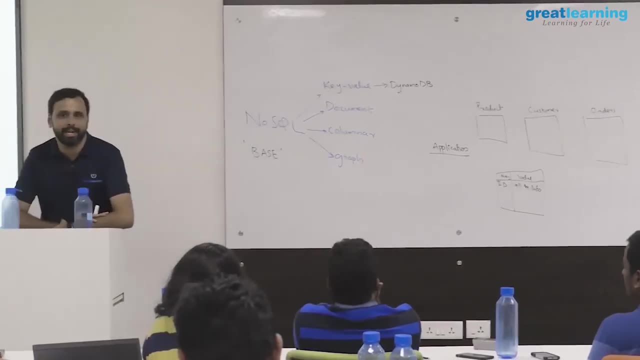 Base. Then they figured out the what each letter stands for. all right, So it is basically available, soft state, eventual consistency basically. But that is a principle which guides NoSQL databases. When I say not reliable, these NoSQL data are not reliable. 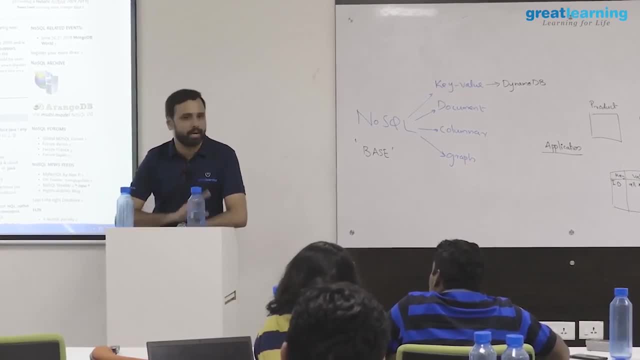 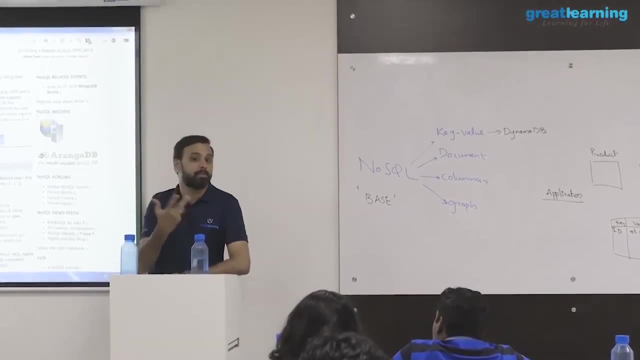 Some NoSQL databases are usually installed in a cluster, Very much like Hadoop, like 50 machines, 30 machines and all. So when some of the machines crashes, will your service be available or not, So that they can sacrifice? So there are some NoSQL databases. in which you may get a connection timed out error. the query may not run, but they may have sacrificed that for speed. They may be really faster right. On the other hand, there are some NoSQL databases which are very reliable but probably not reliable. 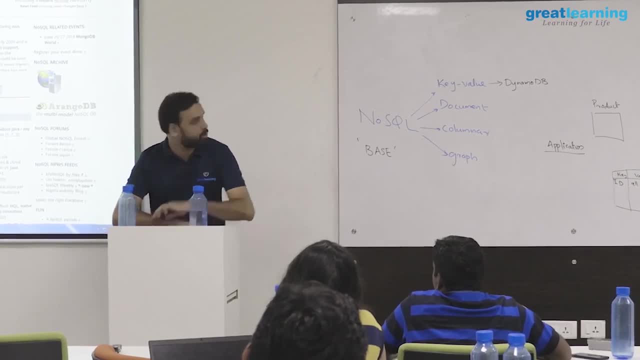 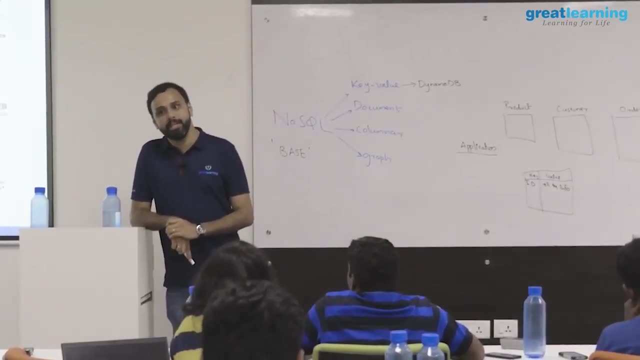 Probably the queries may be a bit slow. right, So you have an option. So these four categories: right, So they have options like whether that has to be reliable or unreliable, You want speed or you want consistency, et cetera. 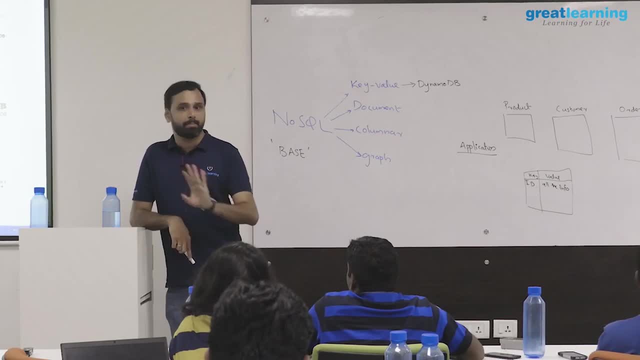 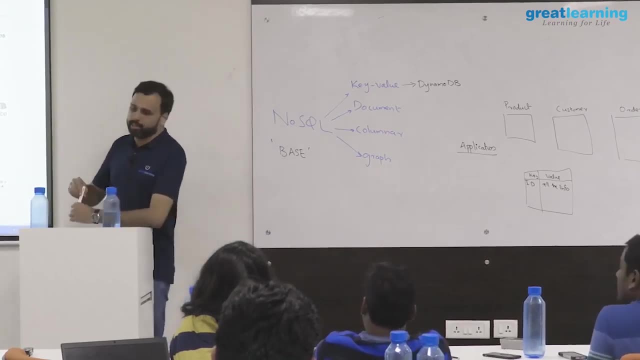 In simple ways, they don't follow SQL standards at all. You don't have ACID properties at all, okay, And so where is the classic use case of NoSQL? The classic use case is that you are storing unstructured data, first of all. 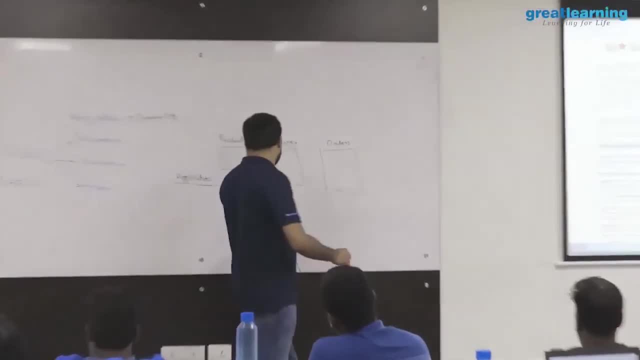 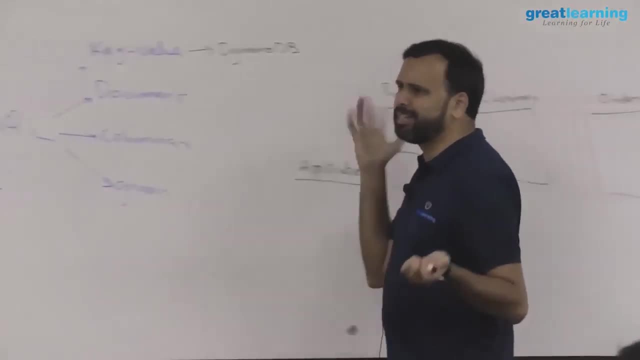 So, for example, if you are having DynamoDB, this value can be anything. I don't care, It's not a table right. So the value can be anything. So I can store images or links or anything I want, because what to do with the value? 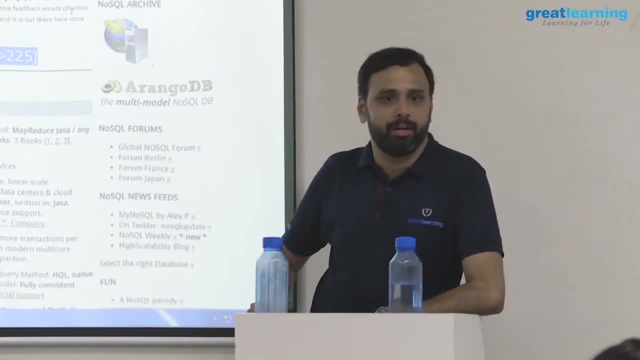 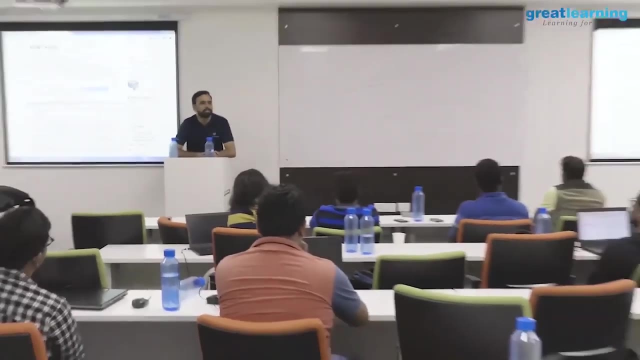 my application will decide On RDBMS. that is not possible. I need my strict schema. Again, the schema is very loose in NoSQL. Many NoSQL databases do not support the idea of a schema. They don't need it because it's all like dumping the data. 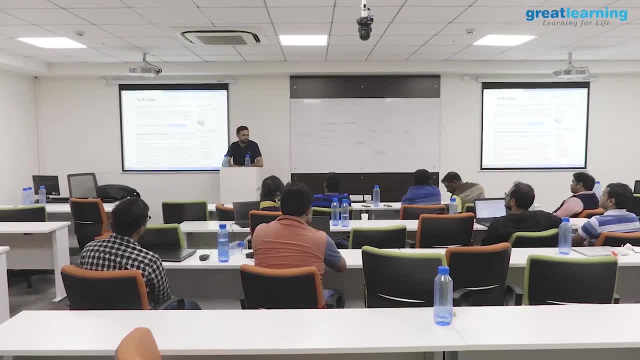 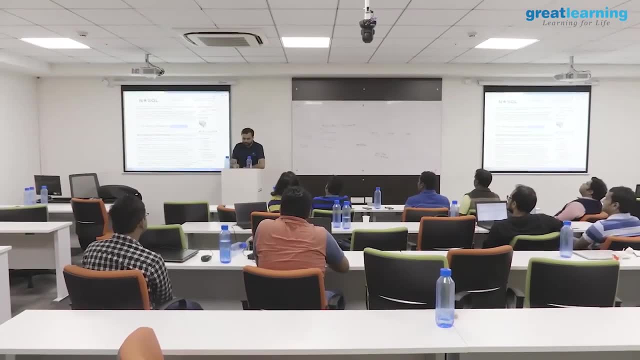 and getting it And getting the data fast right. The rest things will be handled, And so I was working with this Ola Ola company, right So one of their big data project. So Ola uses a NoSQL database. 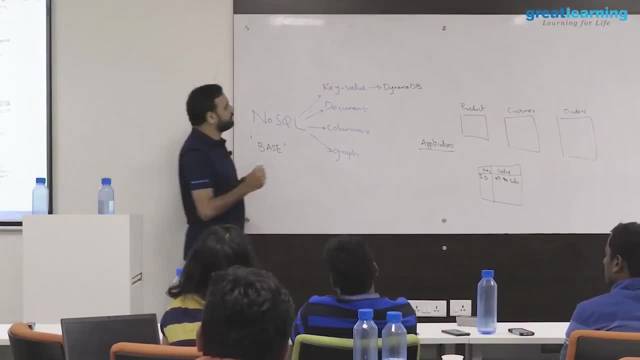 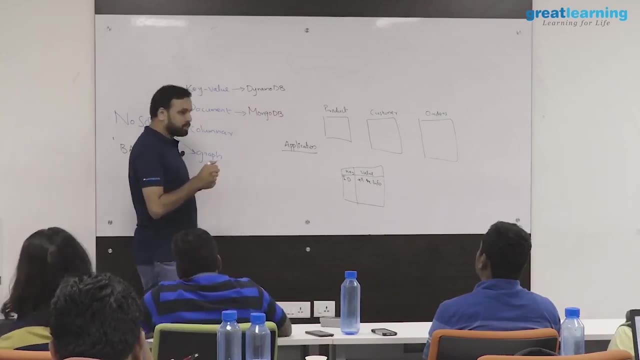 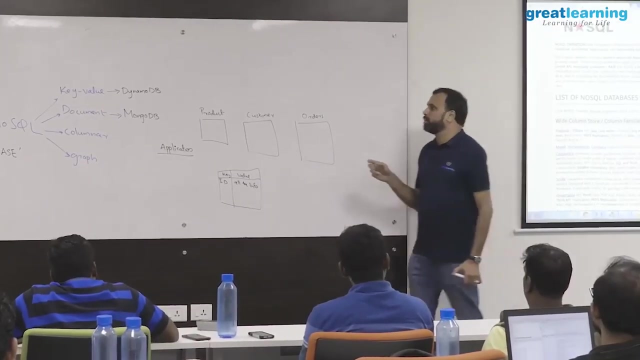 They use a NoSQL database called MongoDB. MongoDB falls in document category. What is the speciality of MongoDB? MongoDB stores the data as JSON document. That is why it is called document-based NoSQL. So in MongoDB, if you search for your data, 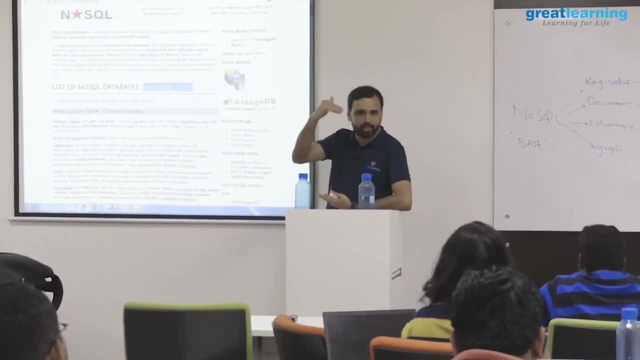 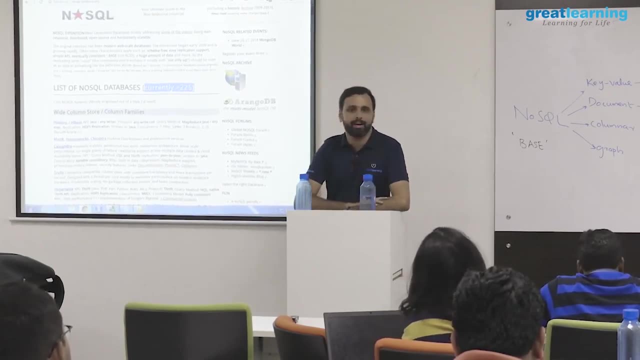 you can see that everything will get key value, key value, key value. It's like a JSON document. That is why it is called a document-based DB, So I'm giving you a real use case, right? So what Ola does, what is Ola's requirement? 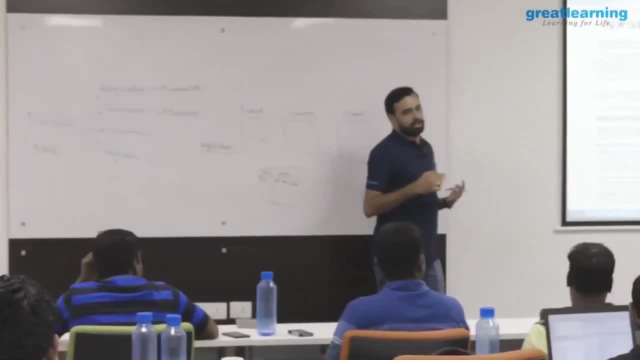 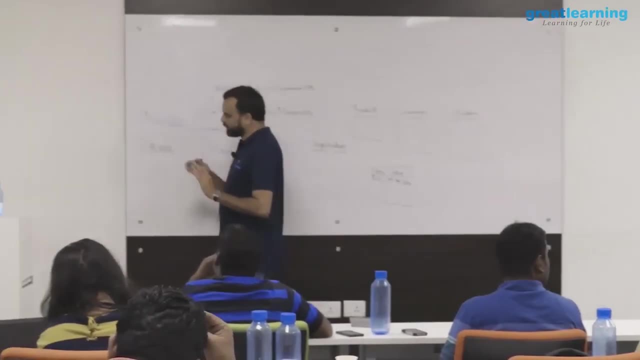 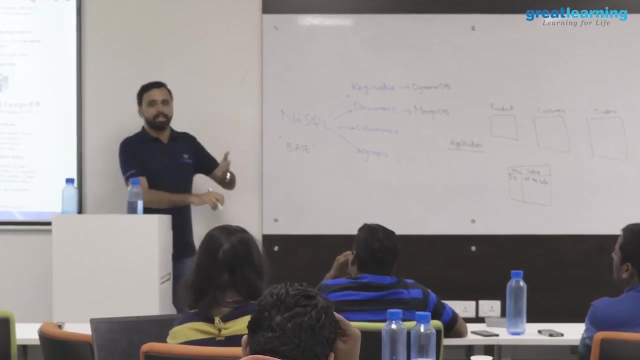 If somebody is using their app, you start the app. the app starts. The only requirement is that a person should see the homepage of the app and how many cars are available. So if you're opening the app and at that point in time, 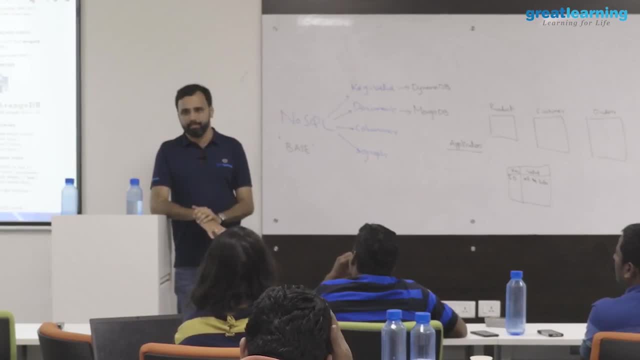 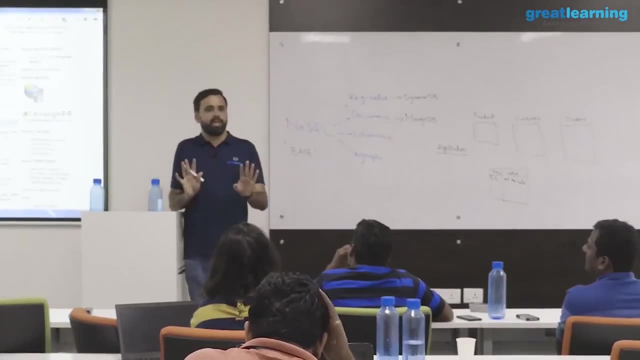 it says the app is not opening, it is getting stuck. you will hate, Ola, But if you're able to open the app, see the cab. and if there are no cabs or the cab says I'll take half an hour, you are okay with it. 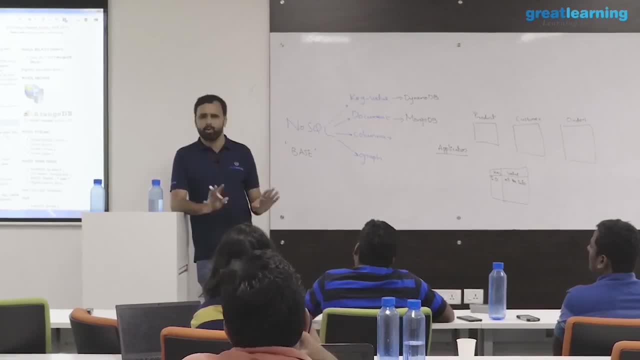 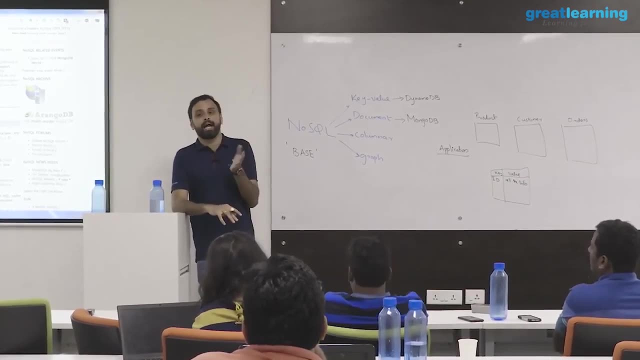 You don't mind. Even if you call a cab, he cancels in the middle. you are okay because you are stuck right. You will use Ola or Uber, But you will want a situation that the app itself is not opening. 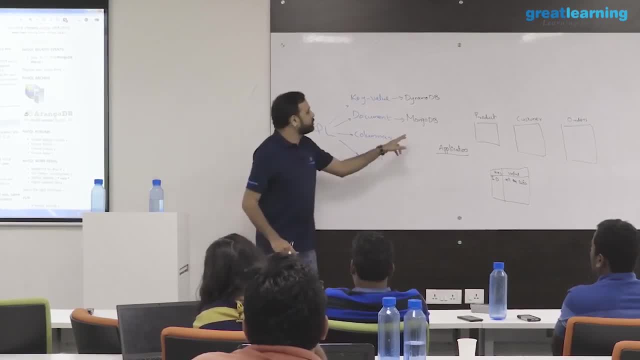 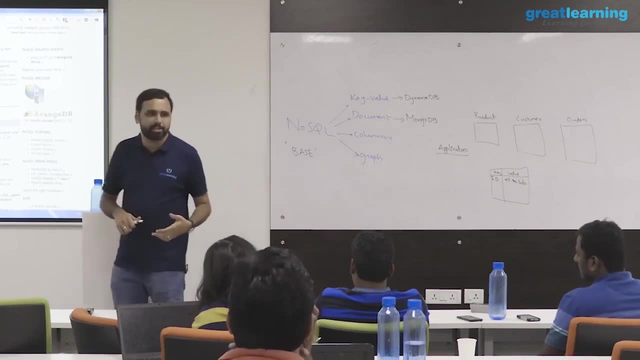 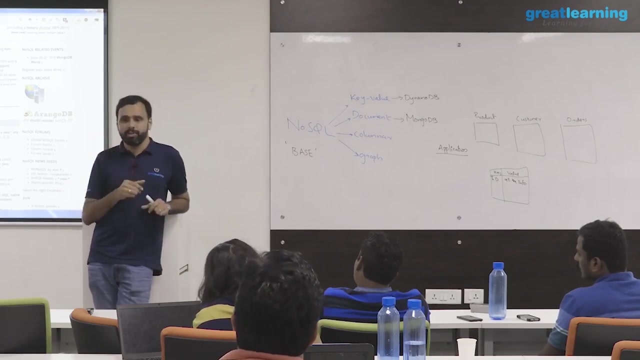 So what Ola does? MongoDB is used to manage the connections, initial connections, meaning they are all the driver data: How many drivers are there, How many cabs are there, with their location stored in MongoDB And all of the user data also. 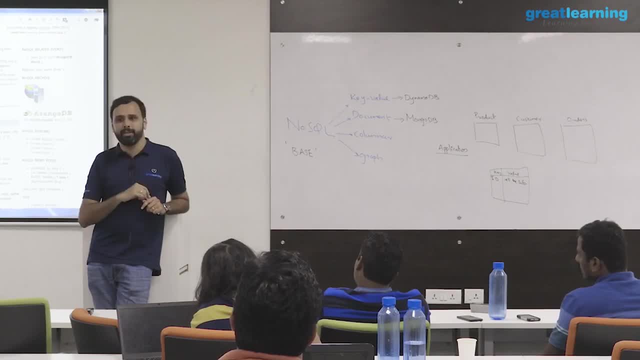 So when you're opening the app, your connection is actually hitting MongoDB And since MongoDB is a distributed data, so MongoDB is not a distributor. So when you're opening your app, your connection is actually hitting MongoDB And since MongoDB is a distributed data, 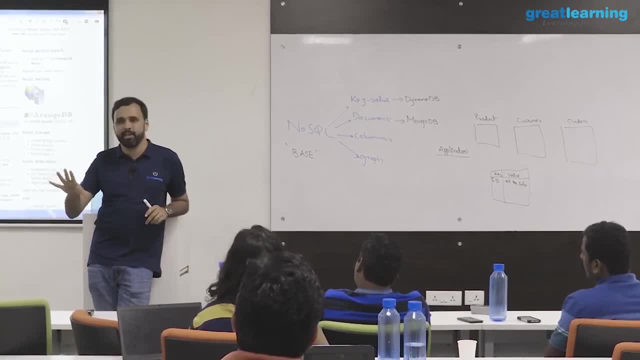 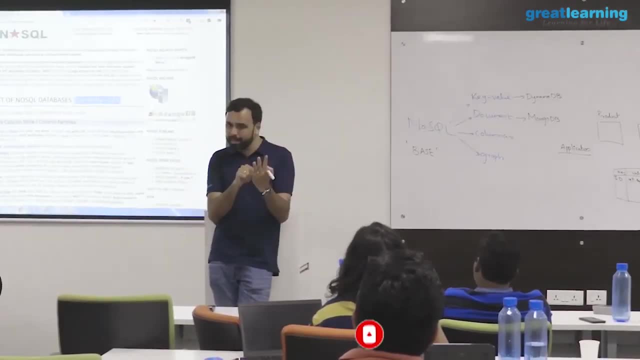 How many cabs are there? How many cabs are there? it can accept 1 billion connections simultaneously, No problem, And the queries are faster. So you're able to open the app, see the cab and you're happy. But when you actually book the cab, 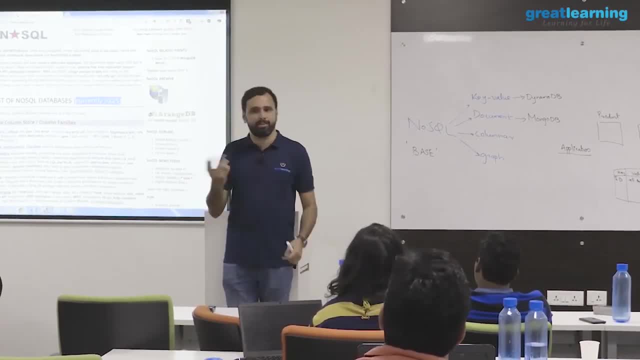 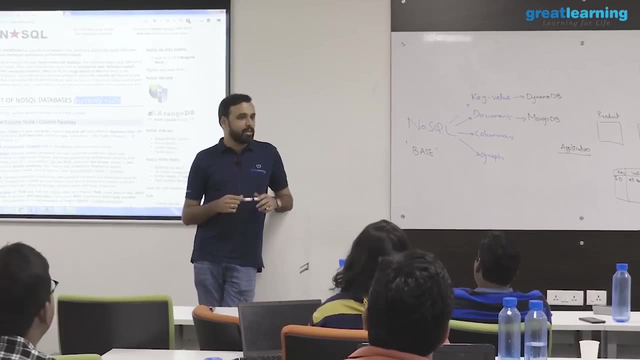 and then you pay money and all MongoDB is not in picture, It's RDBMS, Because you cannot say that the money is halfway. You need reliability, Right. So MongoDB is giving the best shot. In a worse situation, maybe you will not see any cab. also, 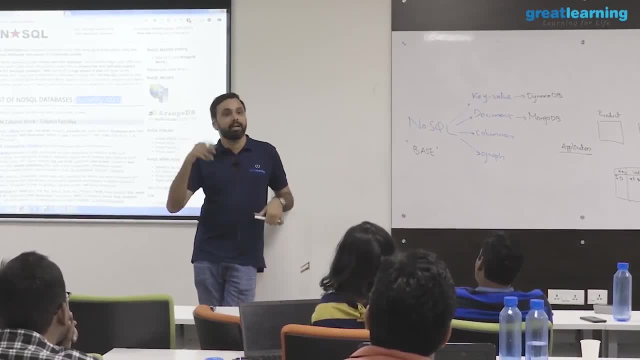 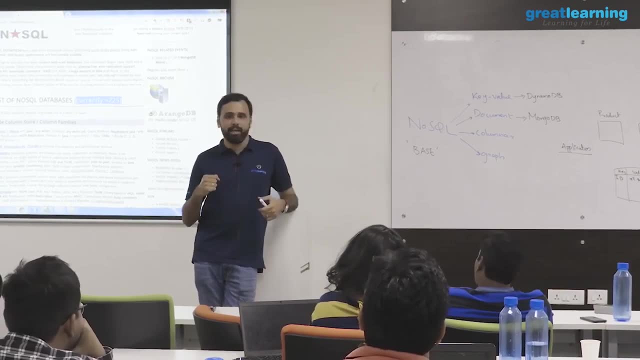 Possible app may get stuck, But that's okay Because I want so. there my requirement, business requirement, is that I want a lot of customers to be served at the same time, Like even if 1 million customer open app connection should be established. 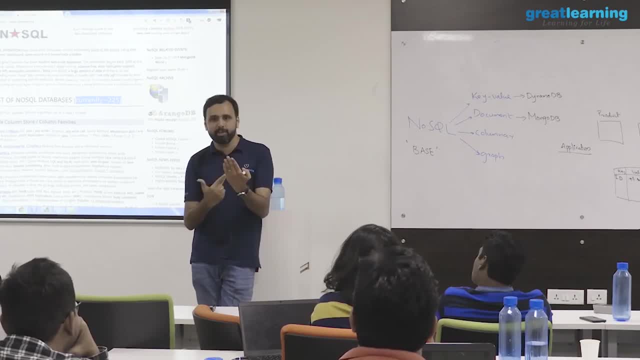 And they should be able to. so when you're opening the app, it's a query. You are searching for cab, So that query is handled by MongoDB. So, since it is a distributed database, it is really fast. So the queries will work. you will see that. 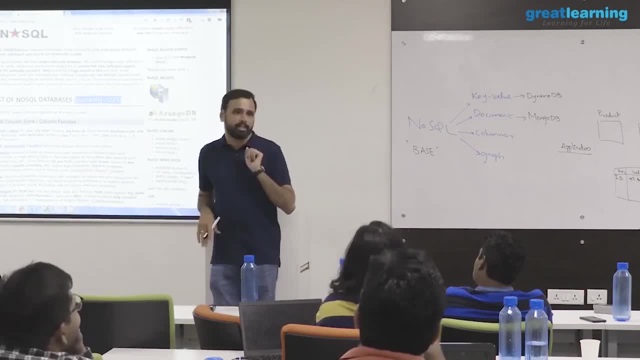 I have never seen any time when all the app gets stuck, But you can see the cars and all initially. Later it's a different story, Right? So there, they don't really care about reliability and all. All they care is the user should be able to use it. 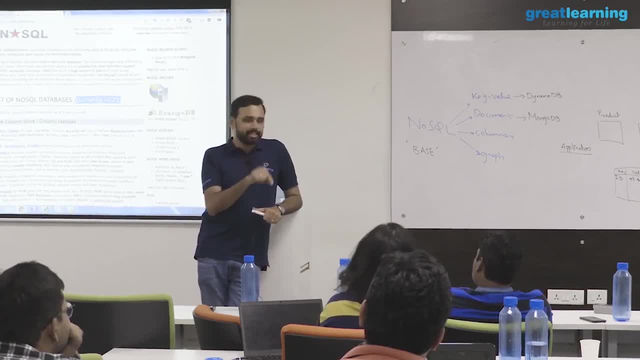 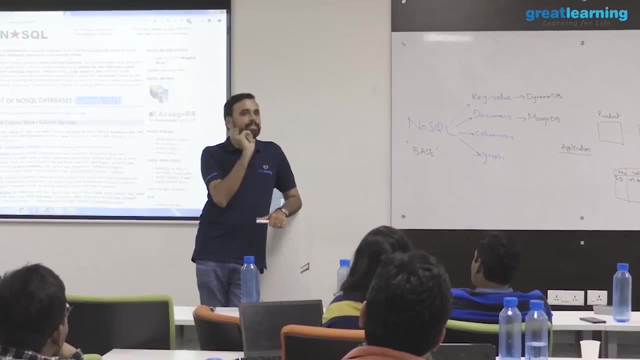 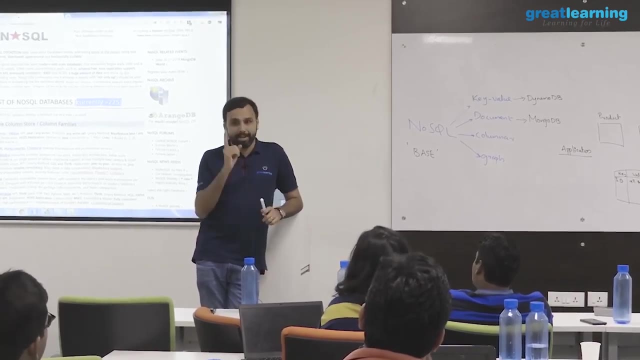 The same story applies to IRCTC. IRCTC was on traditional platform. Now they are either on MongoDB or Cassandra. You can see the difference if you log in. Only different, only reason is this thing. But again, I'm telling you, I'm logging into IRCTC. 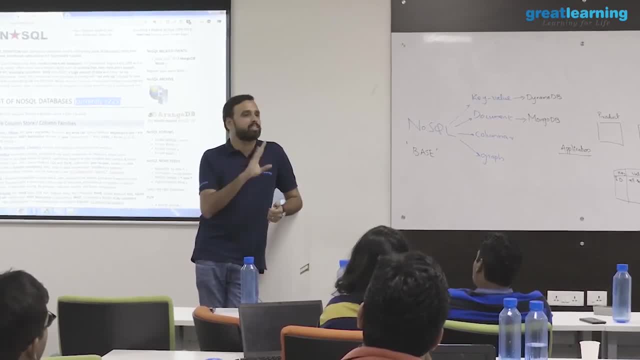 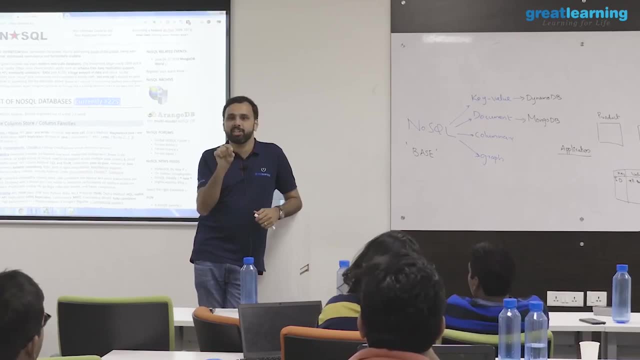 But again, I'm telling you, I'm logging into IRCTC, Right, And I want to book a train. We are in Bangalore, I want to go from Bangalore to Chennai. imagine, Right. So I'm doing searching, Connection, searching, everything is nice. 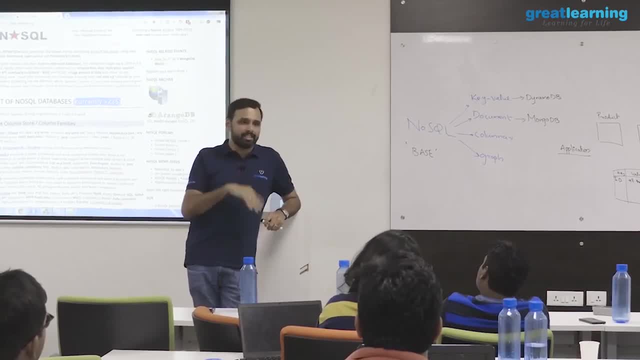 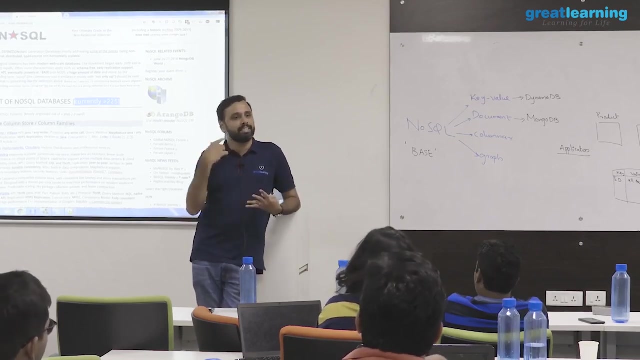 And when I search there is like 20 tickets in third AC. Then I go to transaction I booked, I'm in waiting list 100. There is no. what do you say? there is no relation between them, Because my initial search and connection. 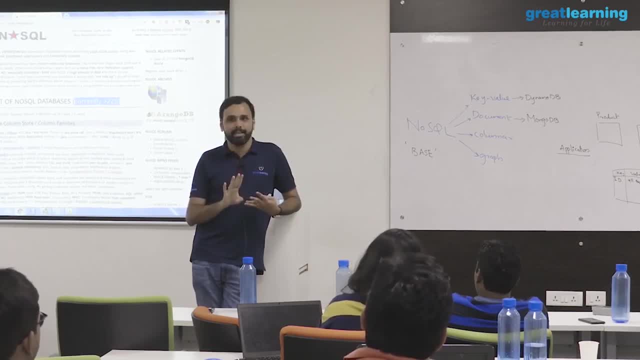 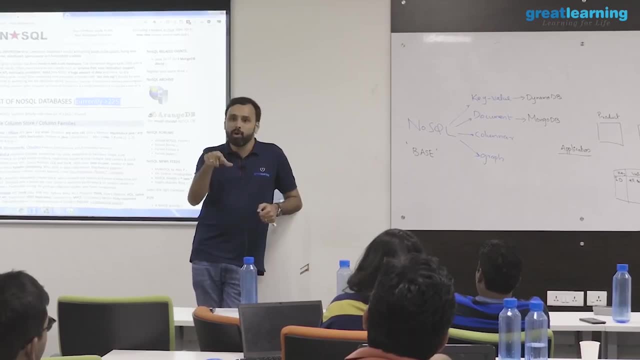 and everything is handled by NoSQL right And the type of NoSQL IRCT uses. they sacrifice consistency. That is why, if you log in, you will see 100 seats available. I'll see 20 seats available. That's okay. 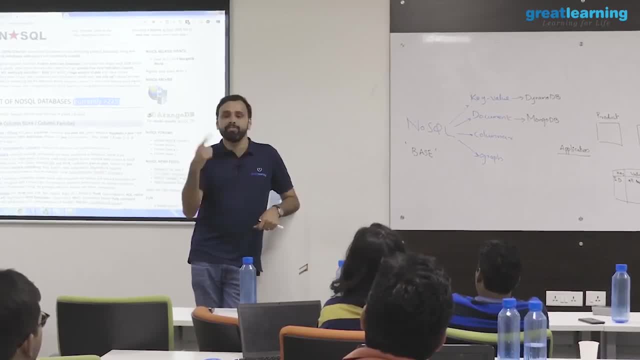 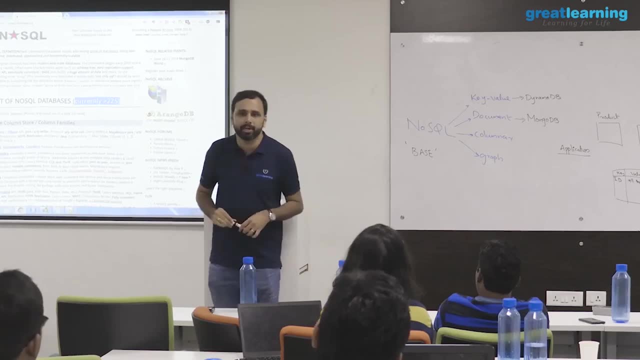 Consistency is sacrificed, but connection speed is there. So, end of the day, when a transaction happens, it is IDBMS. It cannot say 100 is there, 20 is there. It will look at the current seats and book it. 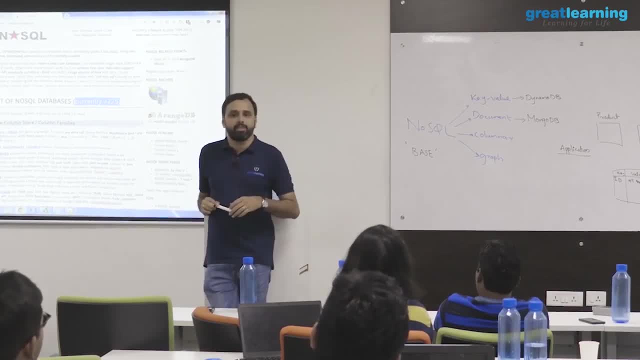 That is why you'll end up in a waiting list, even if you see what you say. So consistency initially, But later you will have IDBMS will kick in and it will say that your actual ticket is this. But problem solved, right. 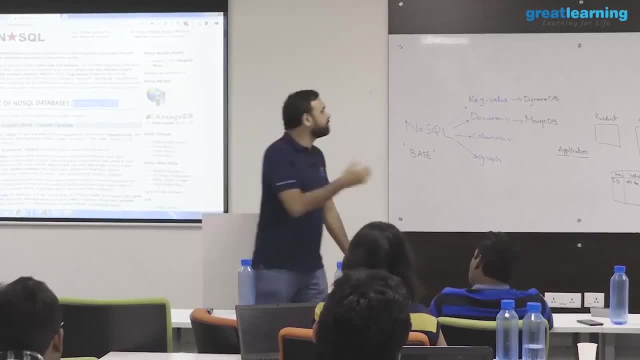 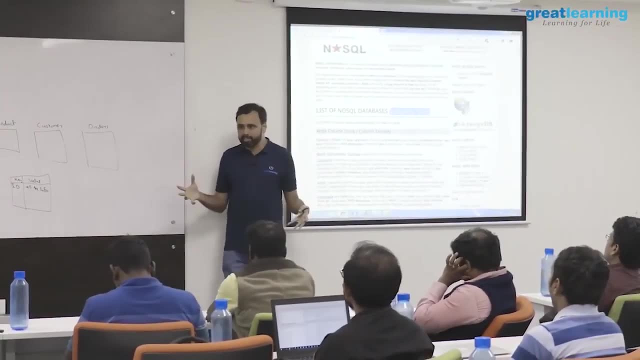 People are able to log in right. So that's what I'm saying. Most of the use cases of NoSQL. it is kind of like a dead shot right Where you are able to serve a lot of customers in real time. 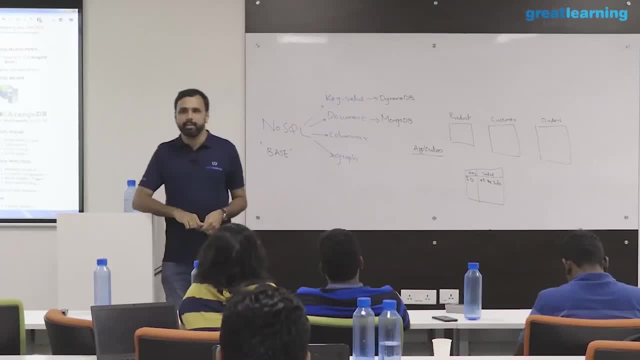 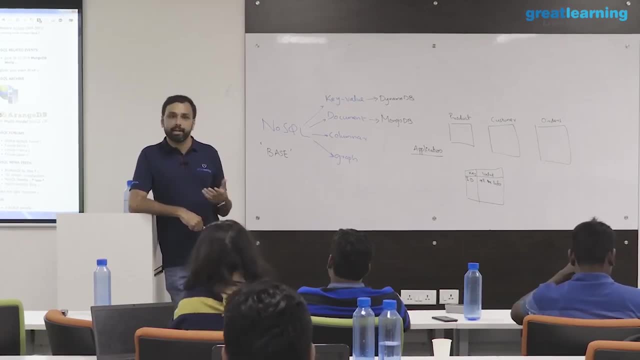 but there are NoSQL databases which are highly reliable, like Cassandra. I was saying, Cassandra and other are highly reliable, Not like this. okay, So you can do that, So you can even use it for transactions. There are many customers who use Cassandra. 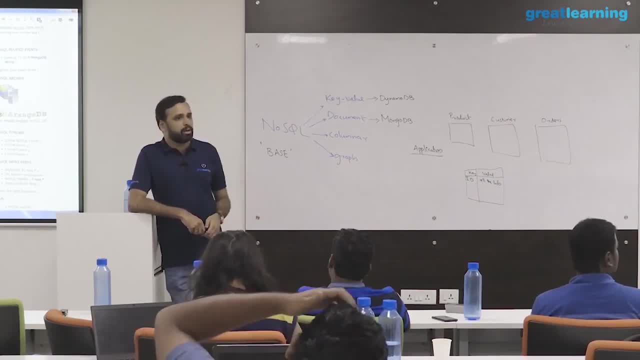 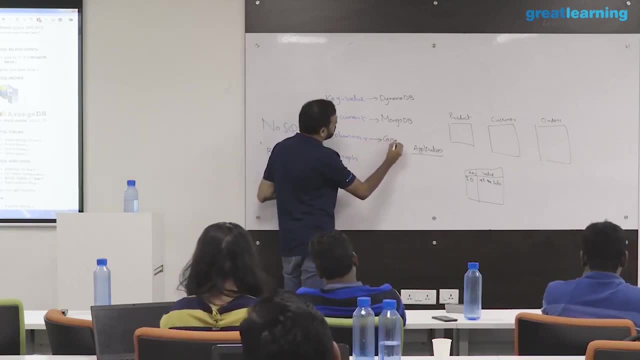 and all for transactions, Not financial, I'm saying, but very reliable and all So. columnar is where Cassandra comes in, Cassandra HBase and all comes in. Graph is where Neo4j comes in, So in columnar database. 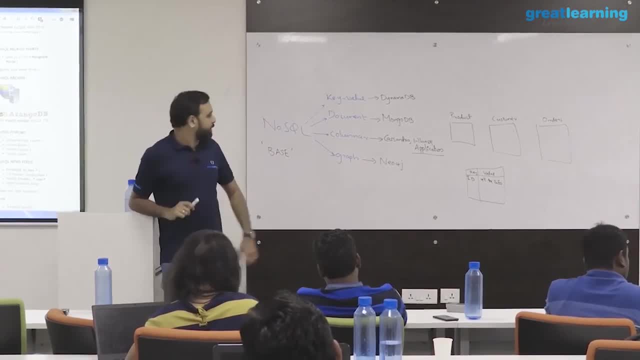 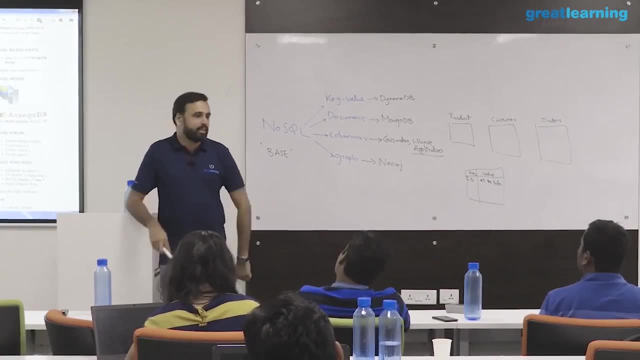 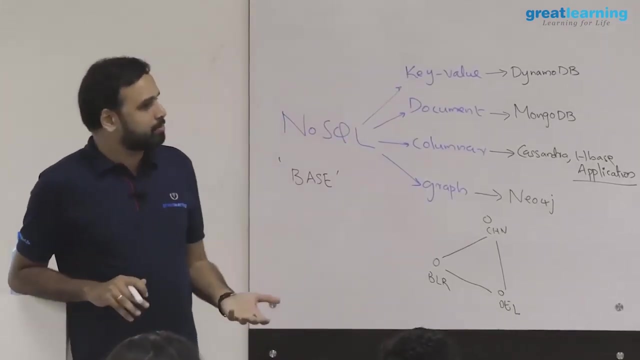 they represent the data in a column format. That's why it's called columnar. In graph databases, the data is in graph format. Do you have you learned graph theory? So I want to build a model wherein I am analyzing all the flight data. 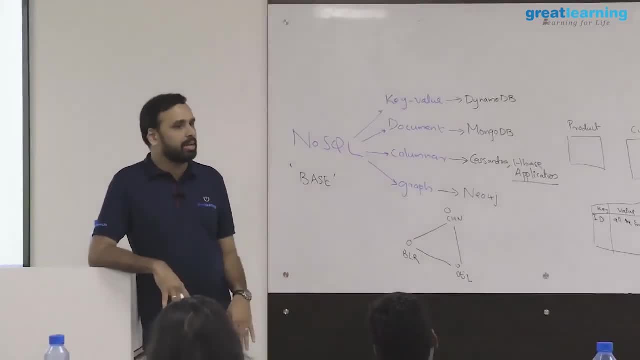 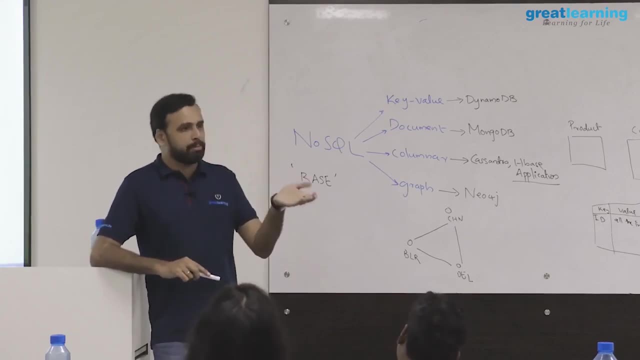 How many flights are flying, how many delayed, how many canceled, et cetera, et cetera, around all the airports in the world. imagine Now I can create a table. no doubt about it. Airport name- airport, that's fine. 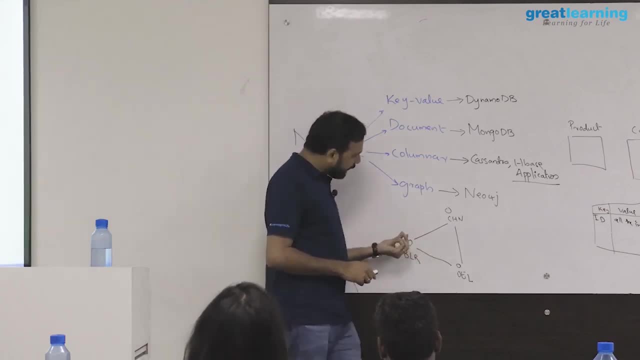 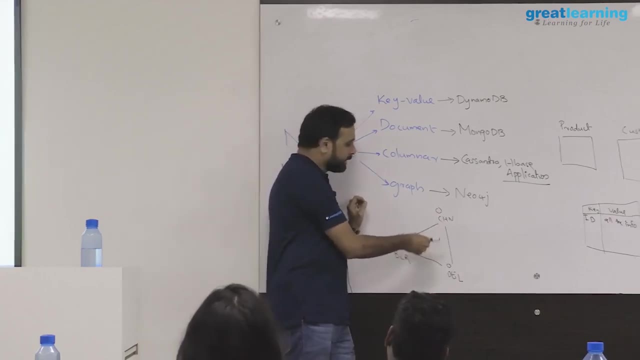 But a graph database will be a better solution for me. I can have all these edges as airports and the routes and then I can add, add attributes to the routes. I can say: in this route these many flights are flying and why this flight got canceled. 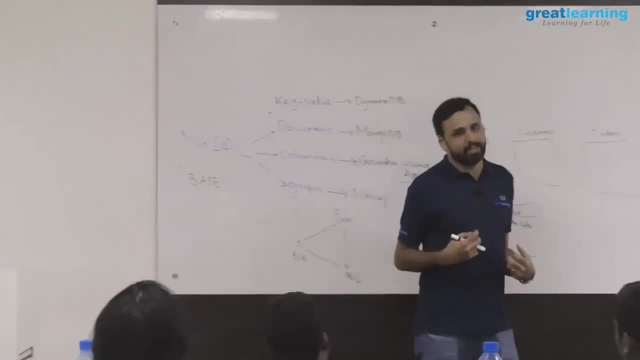 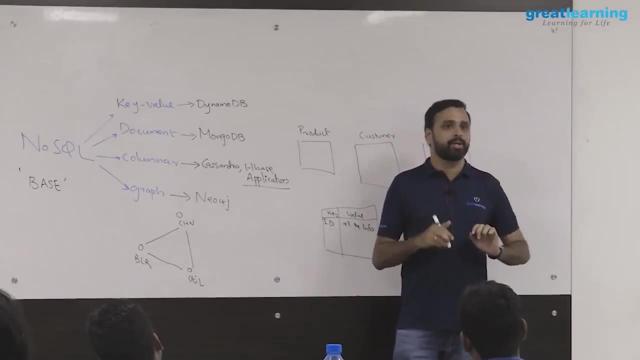 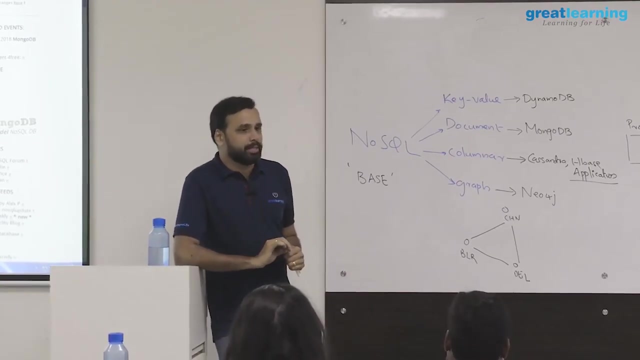 So your entire data becomes represented in a graph format and then you can write graph queries, not SQL queries. It'll run on graph and it is much faster, So in certain use cases people prefer graph databases to speed up. Twitter uses graph database. 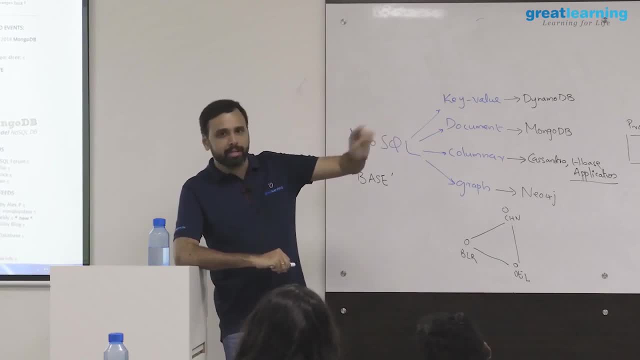 You have this person, then he follows someone and he follows someone. he tweeted, he retweeted, So this connection is actually graph. The entire Twitter is actually on graph database, So if you represent it like that, the queries can be faster. 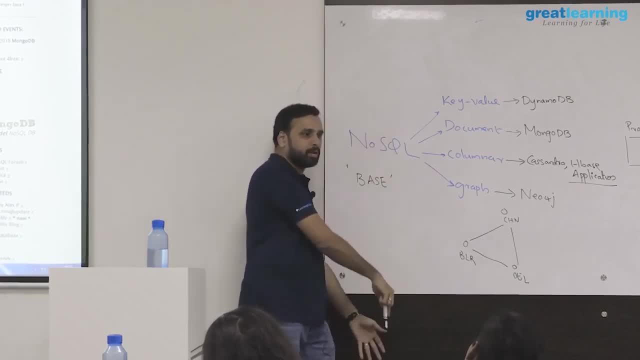 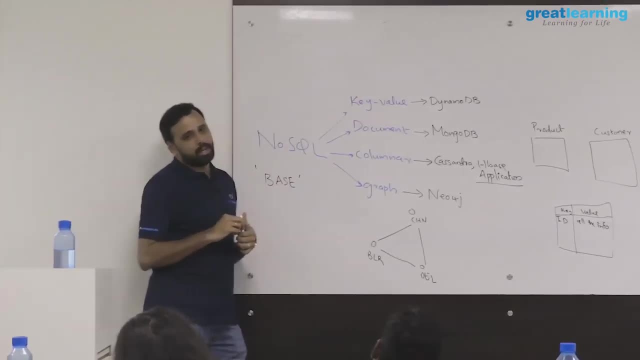 Because normally if I create a table the table length will be like one million or two million or three million. Graph can reuse it right, So the relations can reuse it And the queries are much faster there. So they use their own format of queries and all. 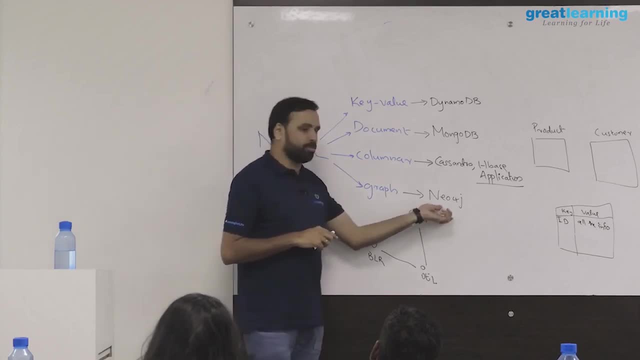 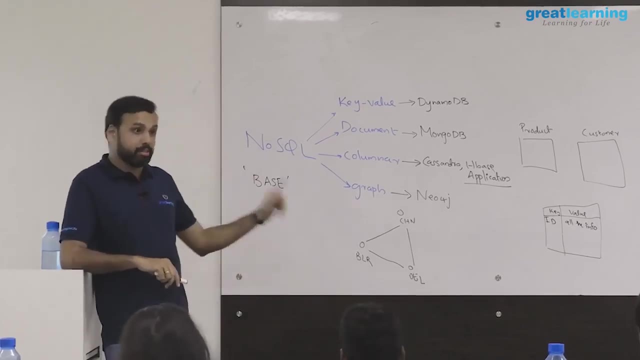 It's not SQL and all Graph database. one classic example is Neo4j. Neo4j is actually the first company to come up with a NoSQL solution. They were the first company to start this thing back in 2004, or something. 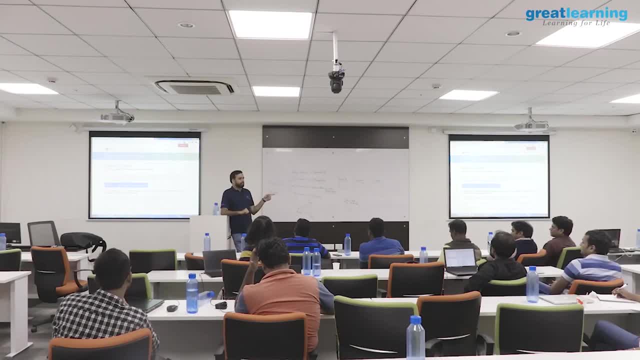 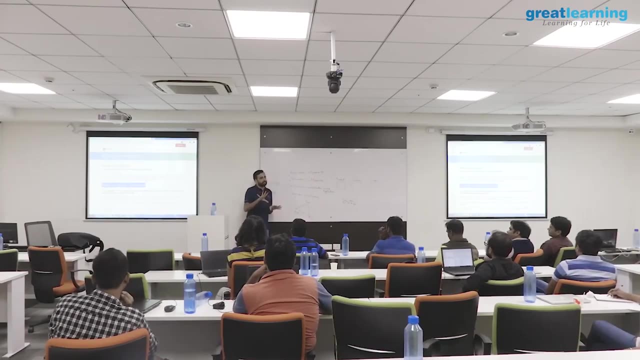 The point is, you cannot practically replace RDBMS with this. You may be able to do it, but with very careful observation. right, Because these two guys have nothing in common. But they have invented a new category of NoSQL which is similar to SQL.